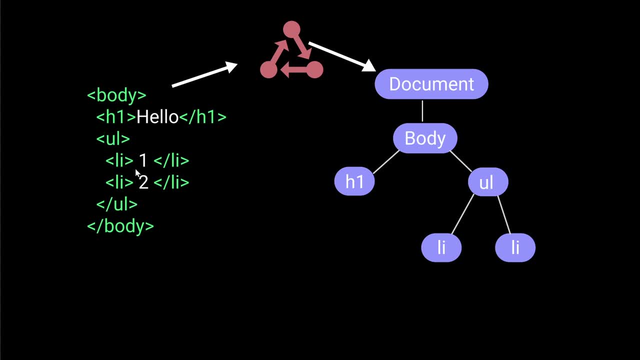 So this is our code. We save our file. Everything is working the way we expect them to work. We open that file in the browser. I want you to consider this is like a browser. Okay, so we open that file inside our browser So that browser will convert our coding into Document Object Model. So it will just create a huge Document Object And it will just create object for body, object for H1, for UL LI, if you have section article navigation, a footer a. 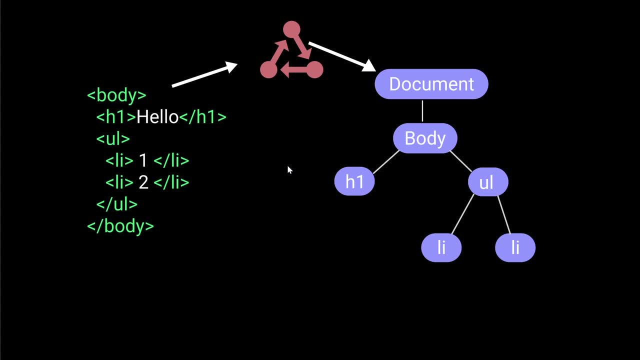 sidebars, all of that stuff. it will just create object for all of that stuff which we have inside our files. Okay, so I want you to just stick their structure in your mind. So whenever we visit to some site, so that browser will convert their web page to something called Document Object Model. So that was just a quick definition of Document Object Model. So now let me just show you everything in a coding, then you will get to know what I'm talking about. So, attached to this video, you will find a link which will bring you 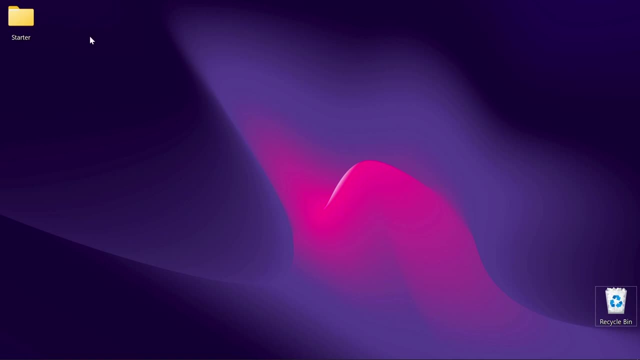 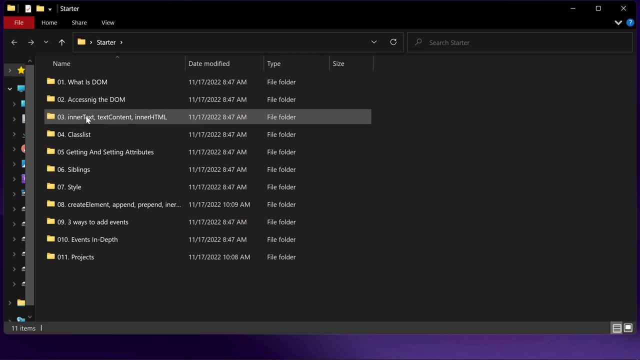 to my GitHub repository. So you can either clone my repository or you can download the starter files And you can also download the finished file as well. So if you just open this folder right here, so we have a few other folders like we have. what is a DOM? accessing the DOM, inner text, content, HTML, classless, getting and setting attributes, saving, style, blah, blah, blah. And we also have this folder for projects as well. So I want you to just download the starter folder. then I'm going to be just right clicking on it and click on this: get back. 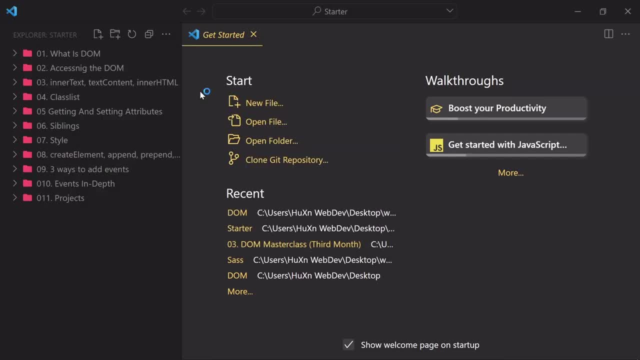 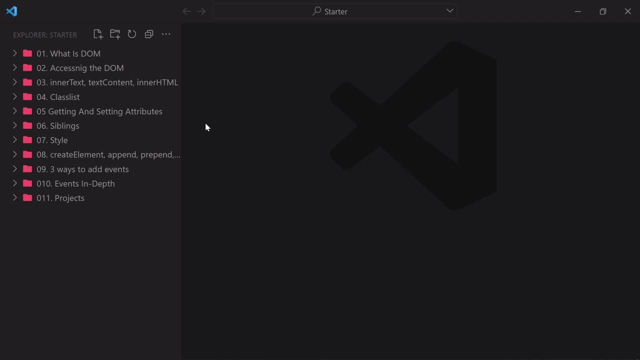 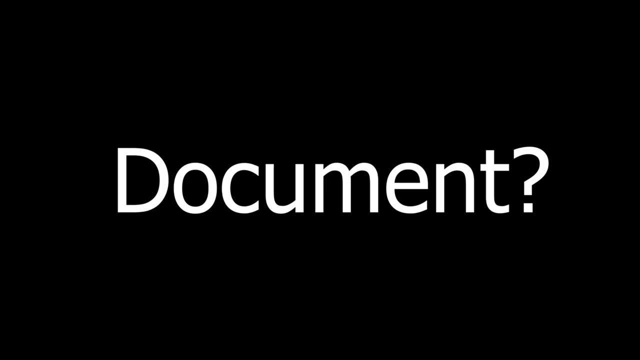 And then I'm going to just write code and period And throughout this course I'm going to be using a Visual Story Coder as my coder And as a web browser I'm going to be using a Google Chrome, And if you want to use some other web browser or some other coders, you're totally free to use that, But for me, I'm going to be using a Visual Story Coder and a Google Chrome as my browser. Okay, so I'm going to just get into it. Let me just zoom in a bit. So, starting from the first thing is that: what is a DOM? we already learned. 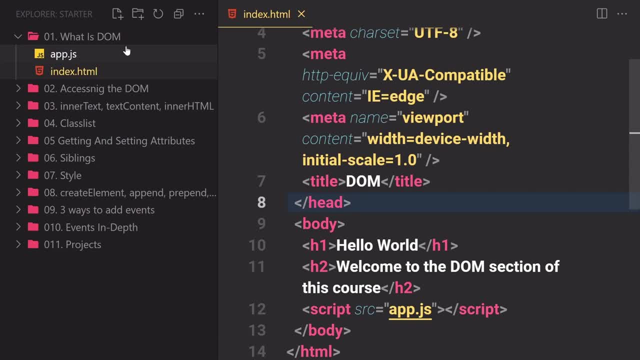 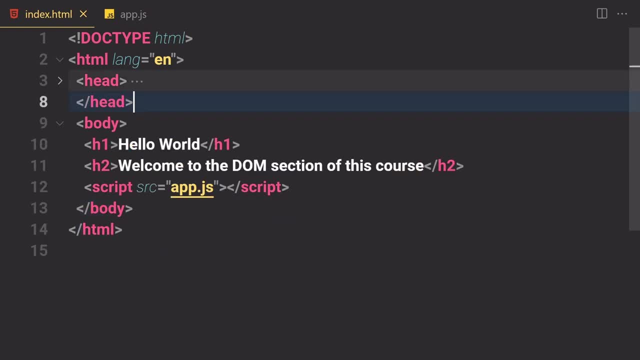 that. So we have this indexhtml file And we have this appjs file right here. So inside this indexhtml file we just have our basic HTML structure right here, And then, inside this body, we just have our h1 with the text of hello world, And then we have another h2, we have like hello, not, not hello. welcome to the DOM section of this course. And then, finally, we just link our JavaScript to our HTML. So I'm going to just right click on it and open it for the live server. So it will now open. 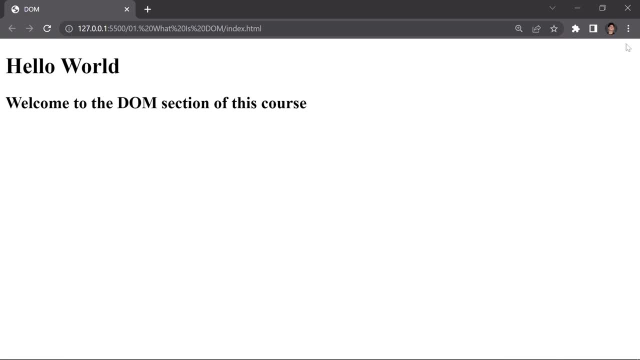 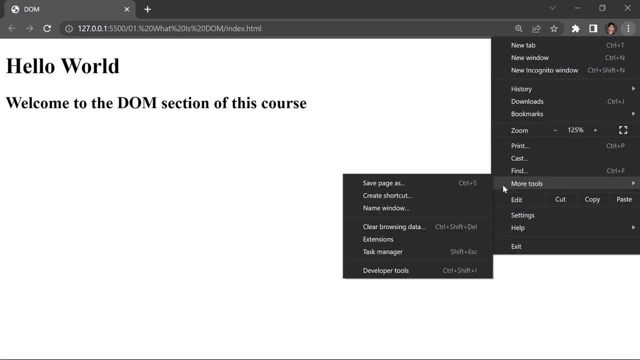 this file in a live server. So the next thing which I'm going to do is that I want you to just click on these three dots, And then I want you to just click on or hover over your mouse over to these more tools, And then I want you to just click on these developer tools, Or you can also. 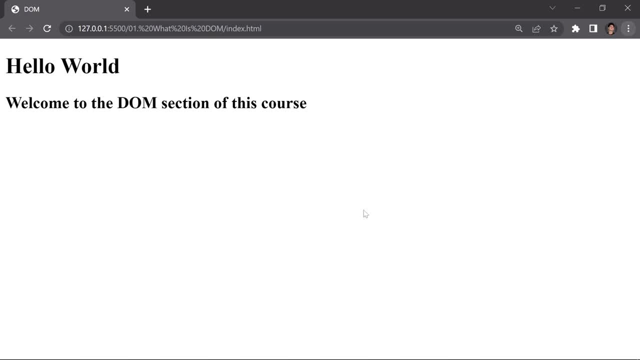 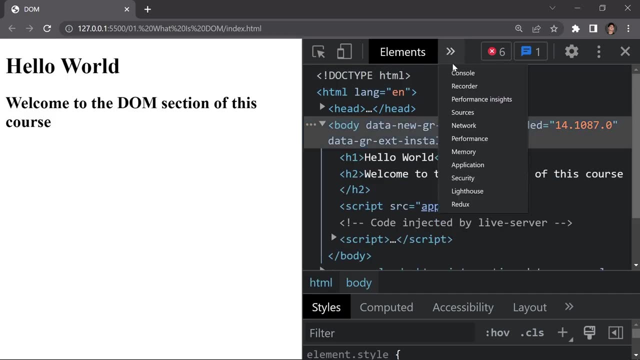 use this shortcut if you want to, And throughout the course I'm going to be using a shortcut, So chances are you will be set to elements. So if it's set to elements, you just have to click on the console. Okay, so it will just open a console for you, Anyways. so now let me just 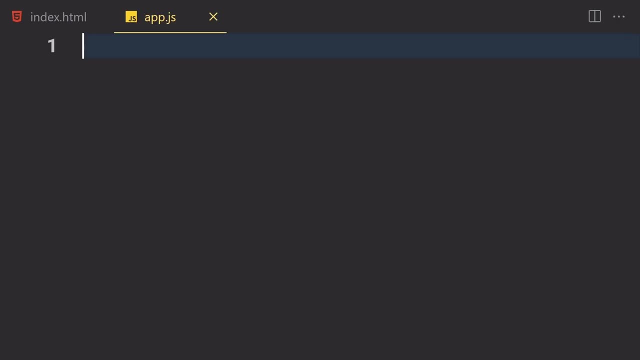 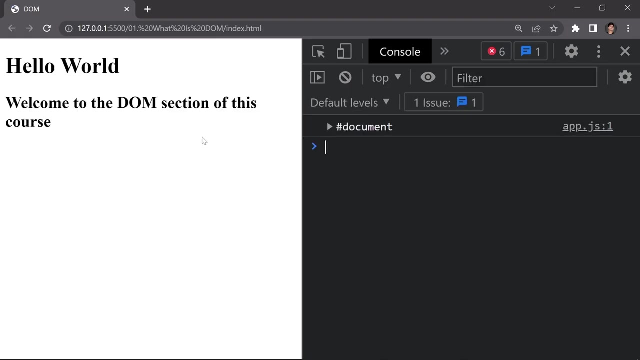 prove my point about the document. So what do I have to do? I'm going to just write consolelog of documents. if you just write consolelog of document and if you sell a file, and here you can see, we get a document right here. So if you expand that, and now here you can see we are. 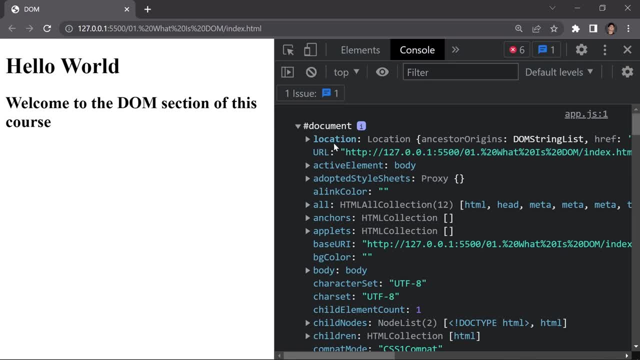 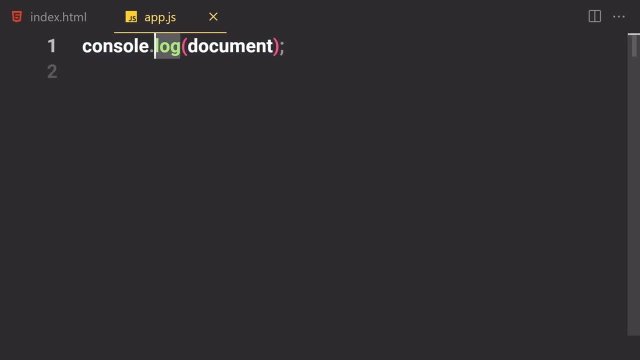 getting all of that properties and its value, different kind of values. And, by the way, if you're not getting all of these properties and its values, so what do you have to do? you just have to write: instead of consolelog, you just have to write consoledir for directory or whatever. 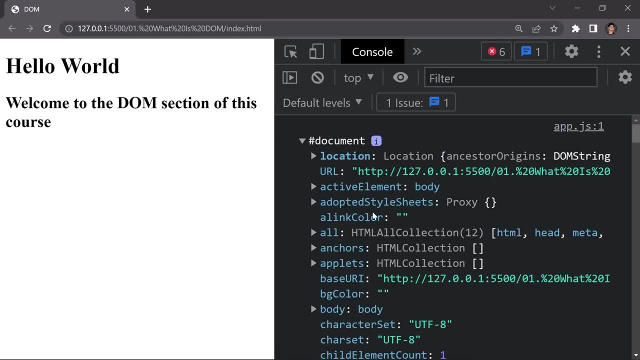 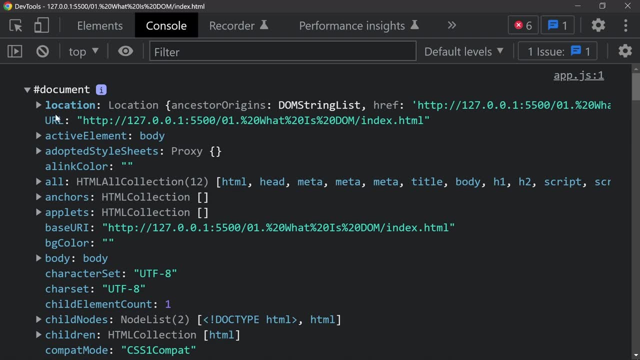 So if you sell a file, so it will now gives us that same result right here. Okay, so what I'm going to do? I'm going to just click on these three dots and like so. So now, here you can see. I just proved my point. like here you can see, we have a location property URL and we have countless 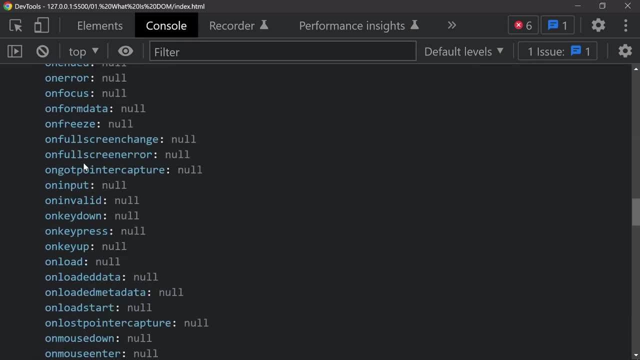 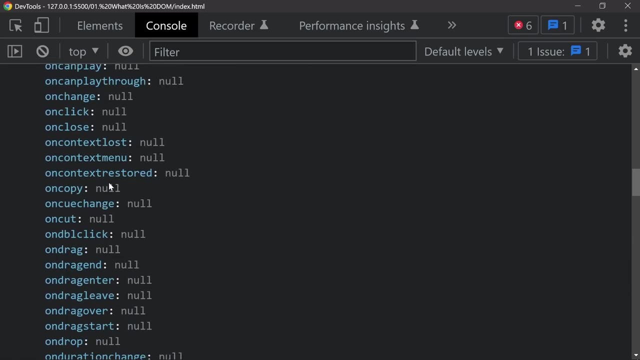 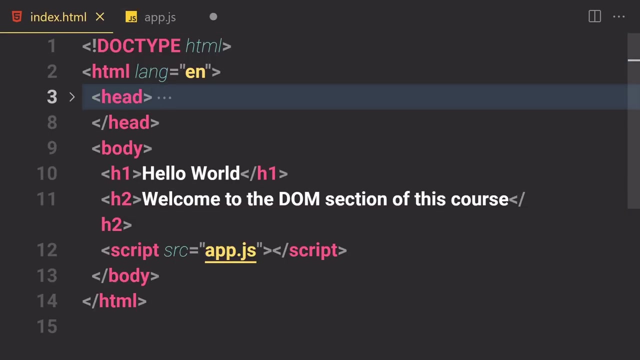 other, and I will highly encourage you to spend a little bit of your time on this document object, and we are going to be also using this document object throughout this course. So now let's suppose if you want to get your body like you know what you want to get, like a head area, like this head area which we have right, so head. 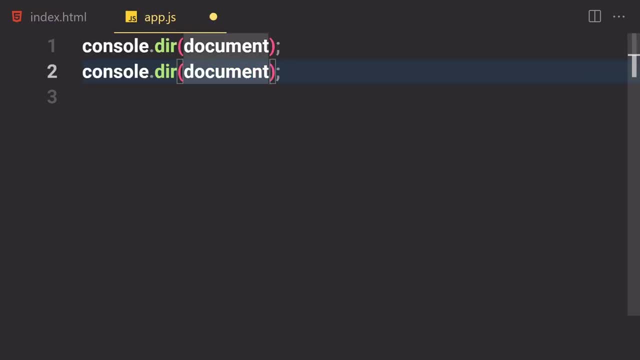 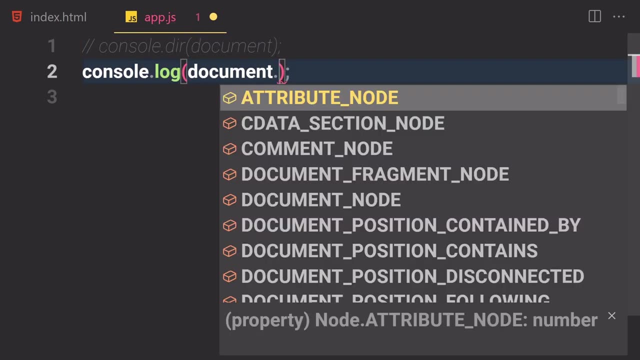 opening tag and head closing tag. So if you want to get there. so I'm going to just write, instead of consoledir, I'm going to write consolelog And I'm going to comment that first line And I'm going to just write period. this document is object, so we can access our properties and its 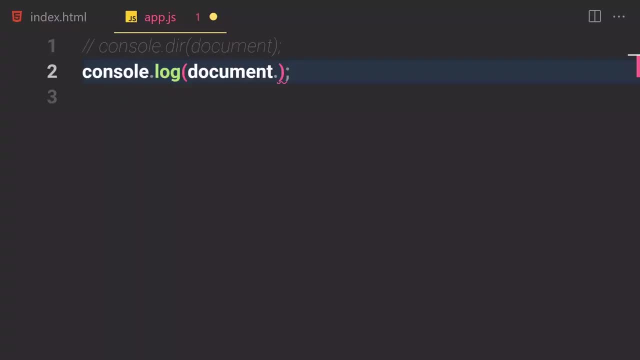 method which we have inside this document. object: right here. So I'm going to just write period to access some sort of a property or element. I'm interested in a head property, So I'm going to just write head and knife is so there And now. 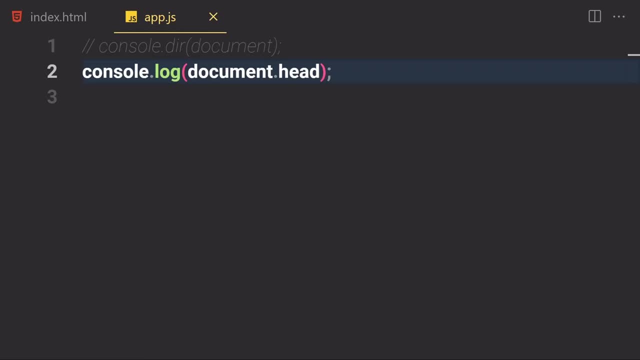 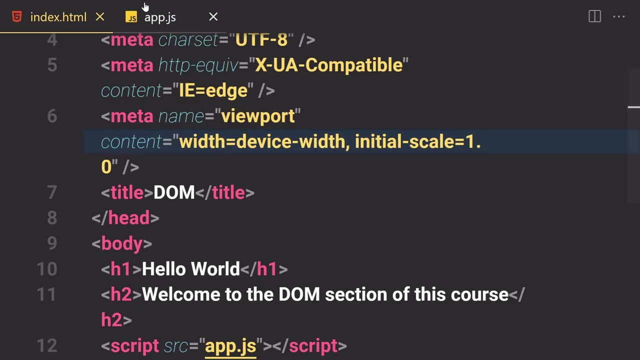 here. you can see it will log uses that head area right here. So we don't have nothing inside that. that's not true. Let's just see we have a metadata experts not showing it anyways, you know what? we can also get a title. So I'm going to just duplicate this line of code And instead of head, 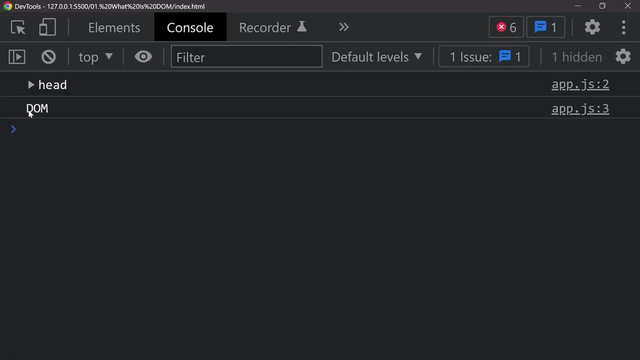 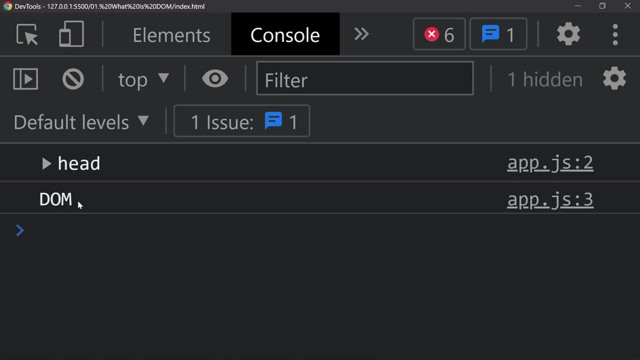 I'm going to just write title And if you say that it will log, uses the title of DOM right here. So we provide a title of DOM in this HTML, So it will gives us their DOM in our console. Okay, so I'm going to just duplicate that And let me just write a body. let's 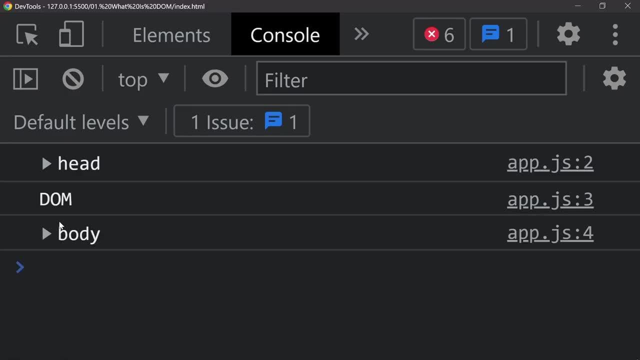 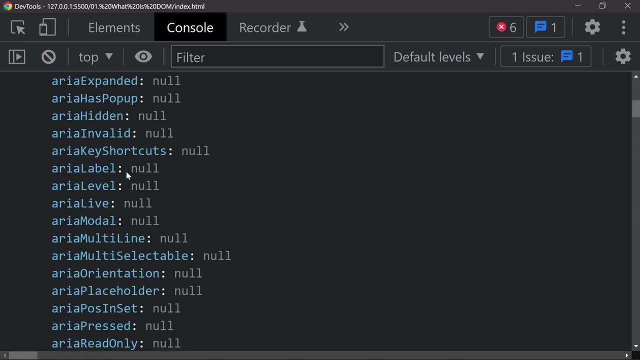 suppose you want to get body someone to send my file, And now, here you can see we have this body. if you expand that And here you can see it will log uses all of the properties and its values and a different kind of methods related to this body right here. Okay, so we have countless properties. 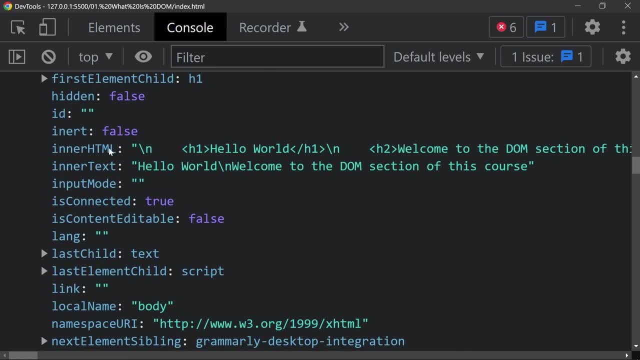 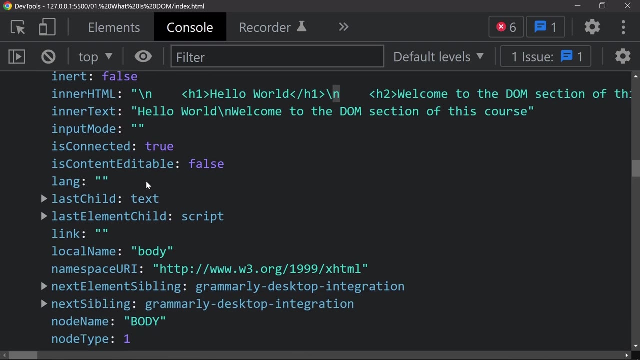 and its methods and all of that good stuff. So we have inner HTML of that h1 of Hello world, And then the new line of then h2, of Welcome to the DOM section of this course, And you can also see the inner HTML. I mean, like inner text and inner HTML, the input mode is set to empty string and you can 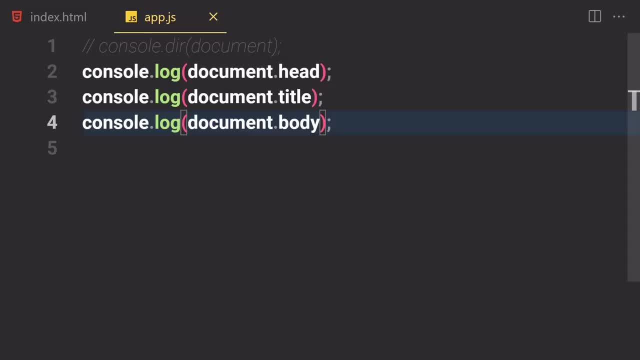 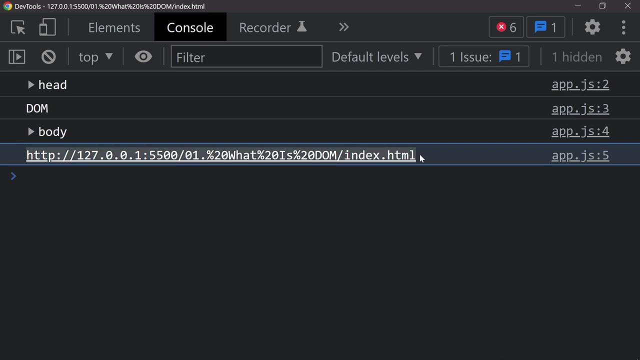 explore all of that in your spare time. Okay, so let's suppose if you want to get like best URIs, So you just have to write document dot best, not best URL, but you just have to write document that you are high. So if you sell that and now here you can see it on log uses, that URL in which 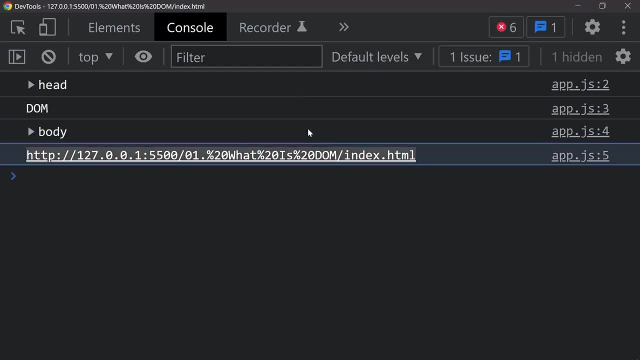 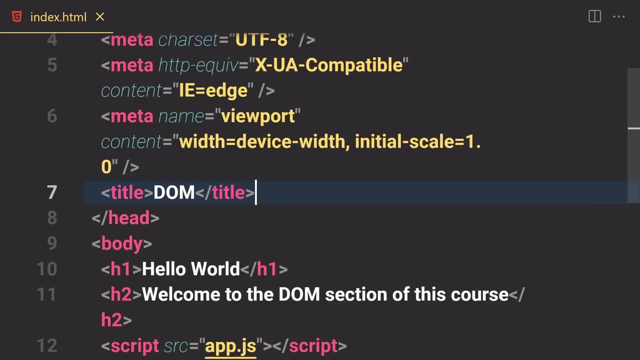 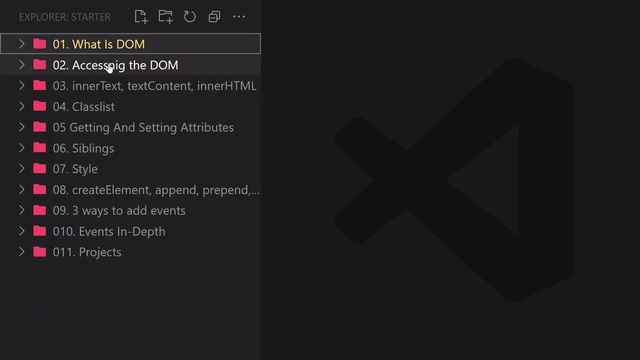 we are using our application. So this one right here, okay, So real long uses that. So that was it about definition of our document object model. So I'm going to just close this file, close that file as well, And I am going to close that folder And I'm going to expand the second folder, which is 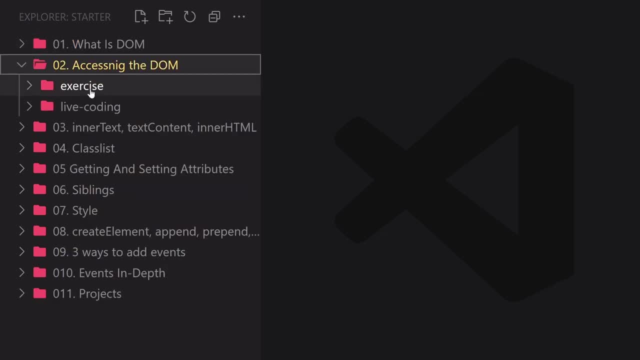 accessing the DOM. Okay, so we have two files, So we have two other folders. inside this accessing the DOM folder, we have exercise one, which you're going to be doing that By yourself And of course, I'm going to also give you my solution as well, But I will highly. 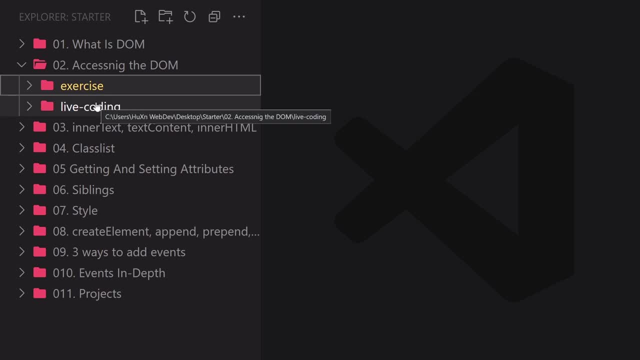 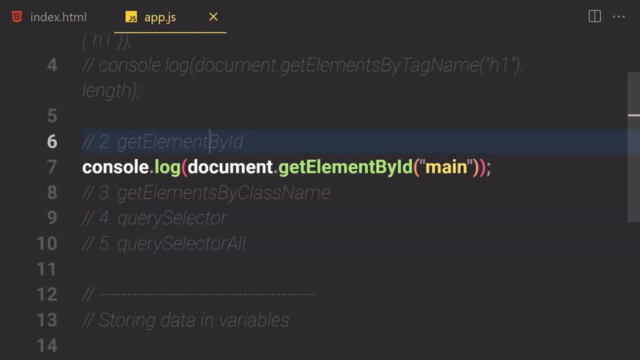 encourage you to solve this exercise by yourself. Now I'm going to expand this one. So we have this index dot HTML file And then we have our app dot JS file right here. Okay, so close that one. Okay, we wrote a little bit of code in there. I'm going to close that one, like so. 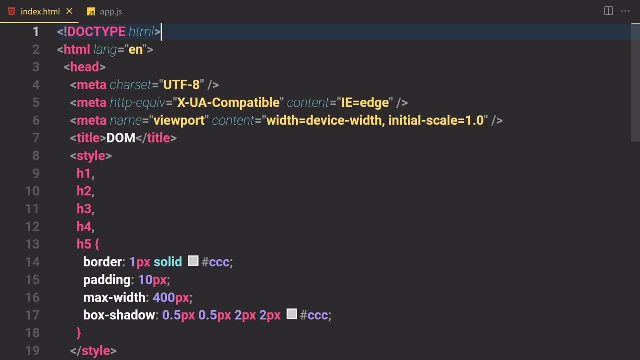 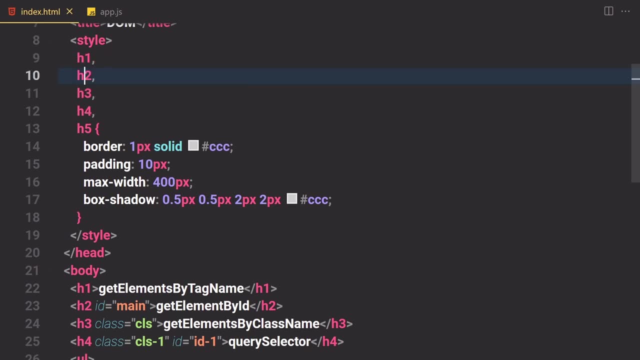 And now let's just get back And here you can see we have a basic setup or for HTML right here, But a little bit of styling right here. So we select our h1, h2, h3,, h4, h5.. And what we did? we just 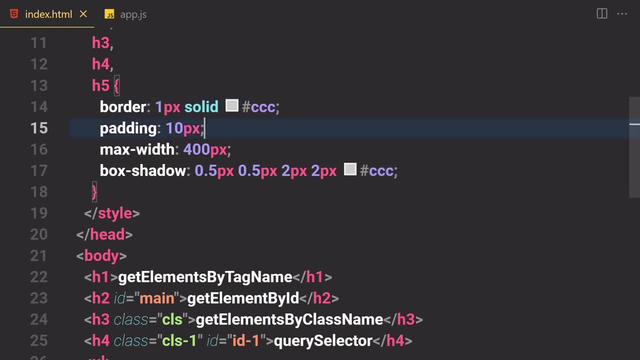 provide a little bit of border of CCC, one pixel solid. we provide 10 pixel of padding and we also give him the max width of 400 pixel, And we also provide a box shadow of 0.5 and blah, blah, blah of. 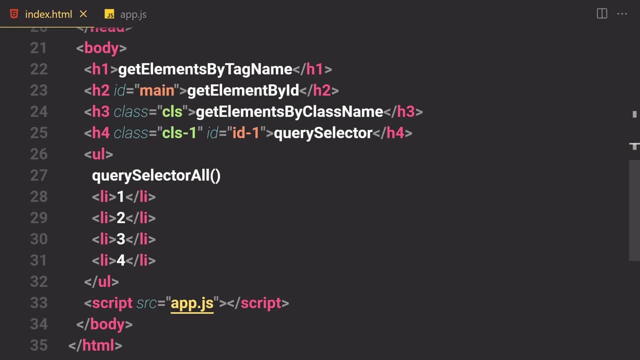 CCC. you will see the result just in a second. But inside the body area we have our h1 with the level of get elements by tag name. then we have our h2 with the ID of main and we have a level of get. 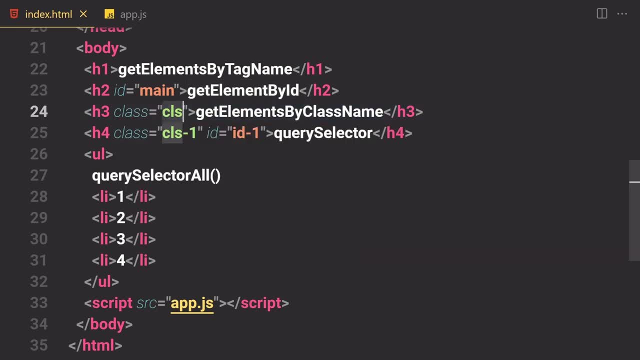 element by ID. then we have h3 with a class of CLS get. element by class name. then we have a h4 with a class of CLS one and also the ID of one And we have a query selector. then we have our ul. 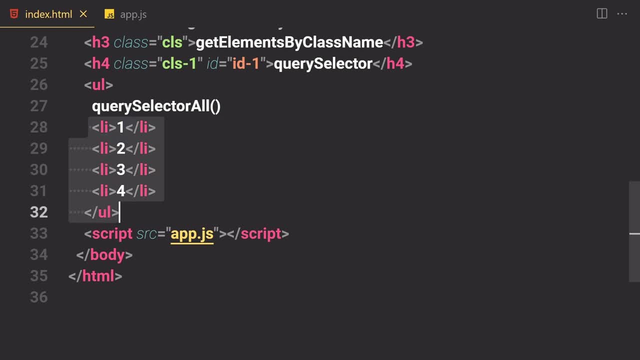 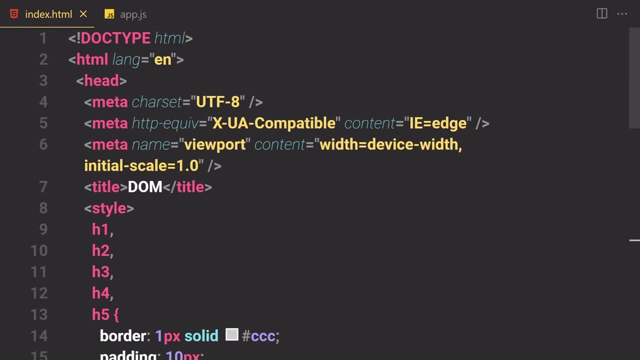 then we have a level of query selector all and a few allies, and each of these allies will have one, two, three, four- yeah, just four. And finally we just add our script area right there. So if you just right click on it and open it for the live server, it will open. 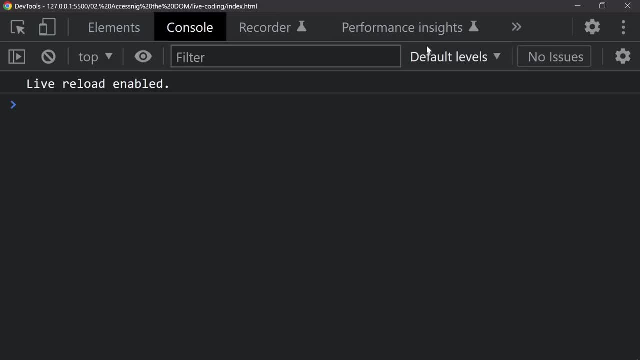 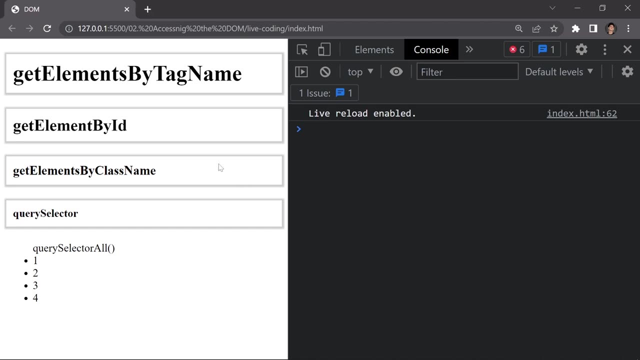 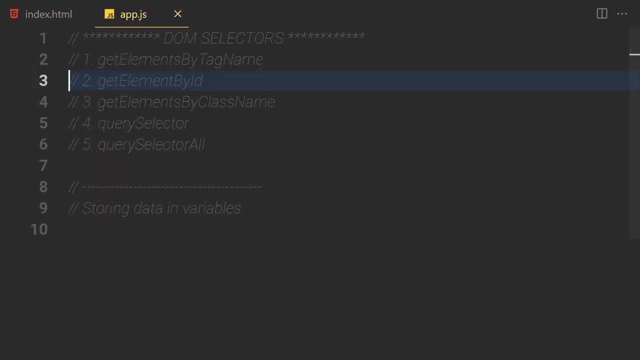 our file in a live server And I'm going to be also opening my developer tools. I'm going to stick that to the right, like so, And this is how it looks like right now. Okay, so say bye, bye to the other one, And now we are going to be working on, or accessing or DOM elements, So I want you to just 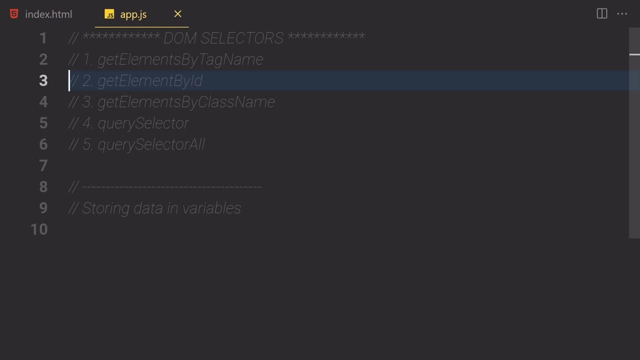 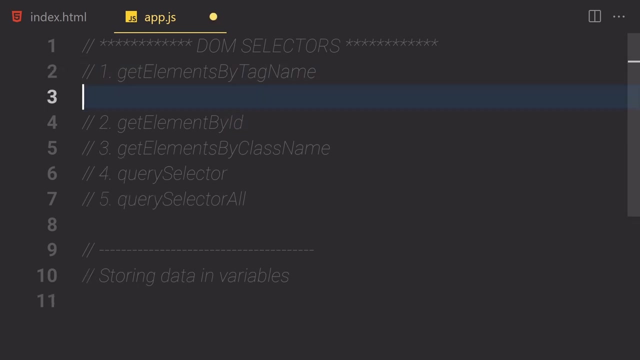 go to your index dot, not index dot HTML file, but app dot JS file. I'm going to just zoom in a bit. So if you have previously worked to the CSS, you already know that first of all you have to select something And then you can. 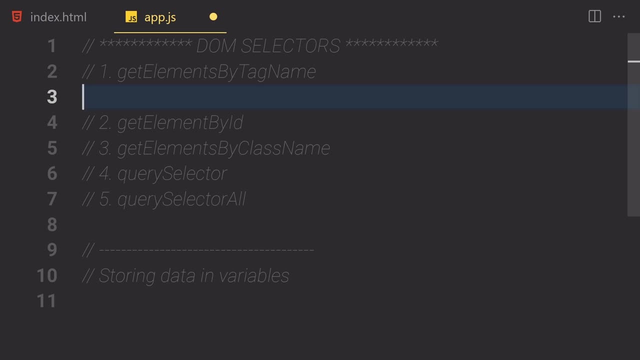 play around with that like, let's suppose, if you want to select something like I don't know CSS selector, like some sort of a selector selector, And then you can just provide a property and a value specifically to that property. Okay, so you already know this. So the 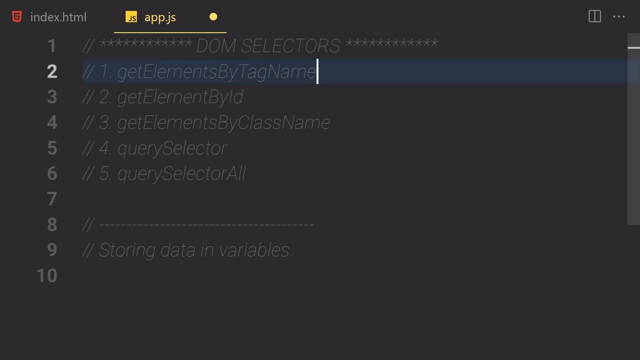 same will apply in JavaScript as well. So, like the DOM, So we have a few methods to access or elements. So if you want to access something by using JavaScript, so we have a few methods right here. So we have get elements by tag name. 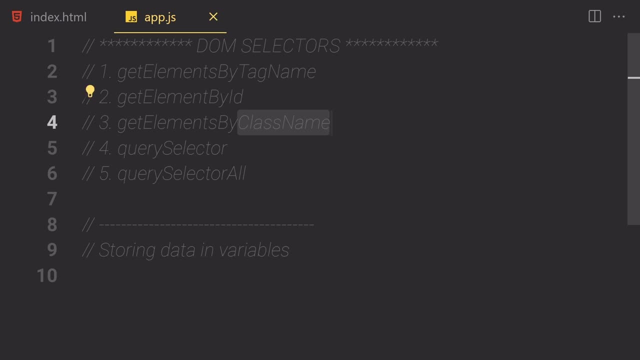 get elements by ID. get elements by class name, get, not get query selector and query selector all, And you don't have to worry about this one for now. So, as the name suggests, that get elements by tag name will allow us to select something by tag name. okay, like HTML: element by tag name. 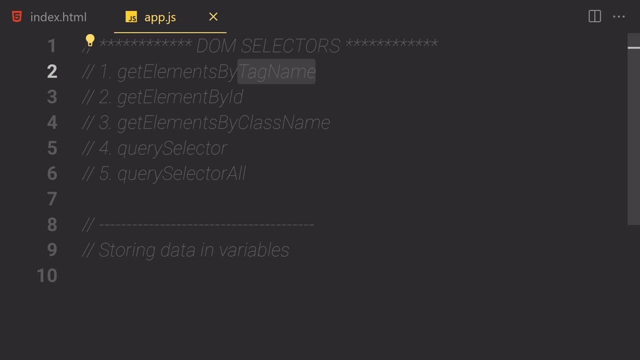 and then we have a get elements by ID, So it will allow us to select something HTML element by using ID. So then we have a get elements by class name. So, as the name suggests, it will allows us to select our HTML element by using a class name. Okay, so in CSS, if you want. 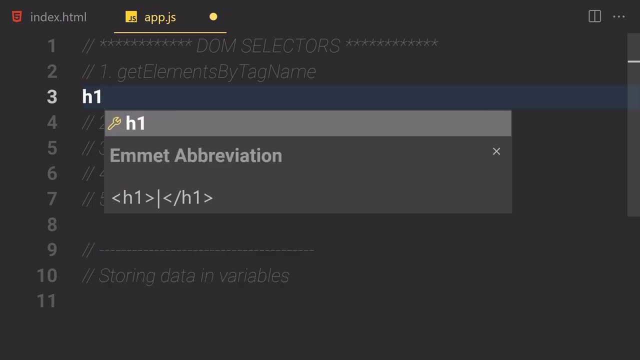 to select something like maybe by the tag name. so you're going to be first of all writing h1 or h2, or whatever the tag name is. So in my case I'm going to just stick to that h1. And then you can. 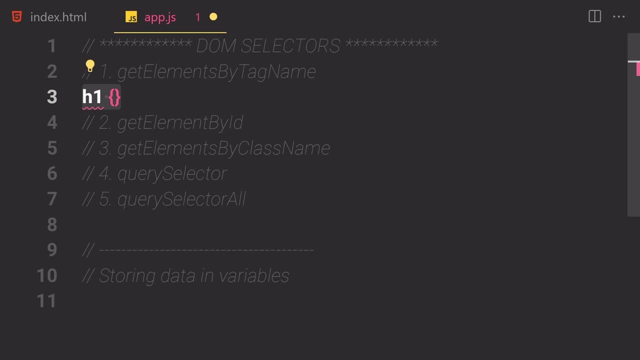 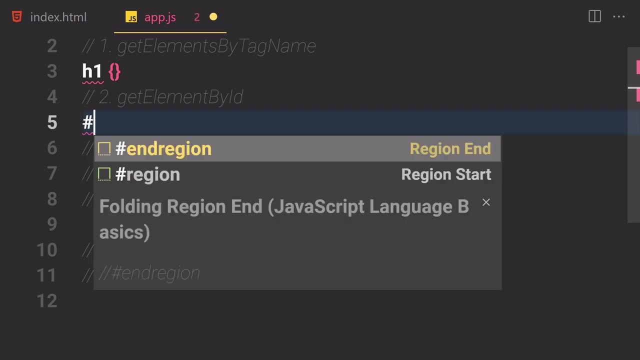 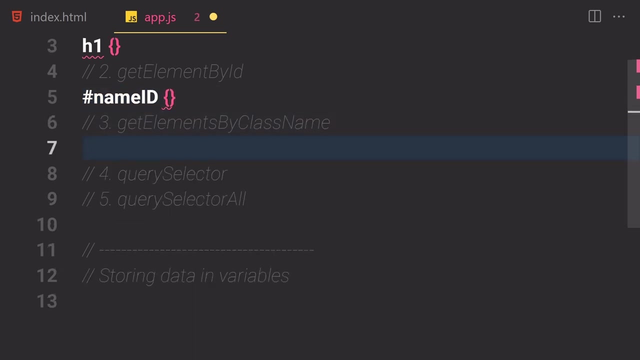 provide your content inside there. So this is the HTML. I mean like, this is the CSS tag selector. So if you want to select something by ID in CSS, you're going to be first of all writing a pound symbol and then the name of the ID. Okay, so then we have a class selectors. if you want to select. 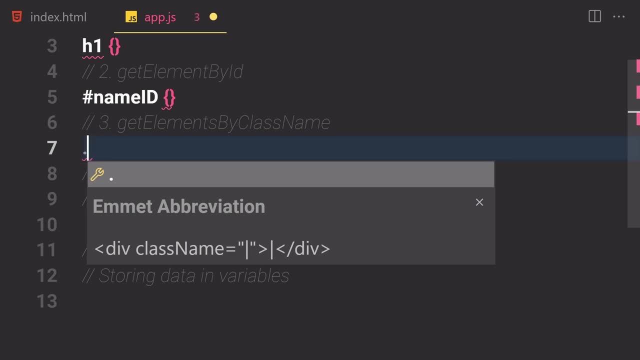 something by a clause. you're going to be writing a period or dot where you want to call it, and then the clause name, and then opening curly brace and closing curly brace, And you don't have to worry about these two for now. So this is a CSS selector, So I'm going to just remove that from here. I just 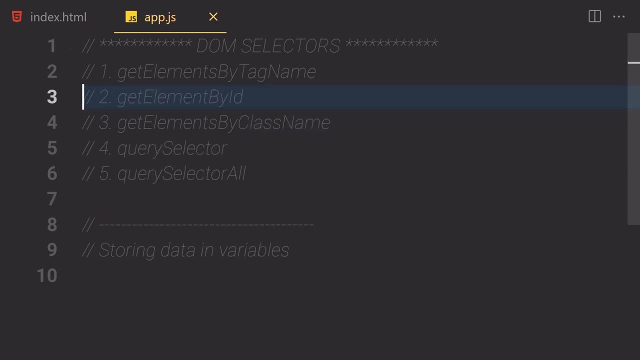 kind of wanted to show you, if you guys already don't know about that. so that was just kind of a css selector. so now if you want to select something by using a javascript, so we have a few methods, so now let's just use that. first of all, what do we have to do? i'm just asking you a question, so, like, what do we have to do? 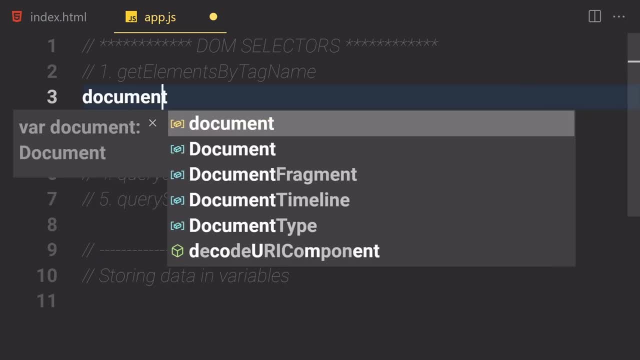 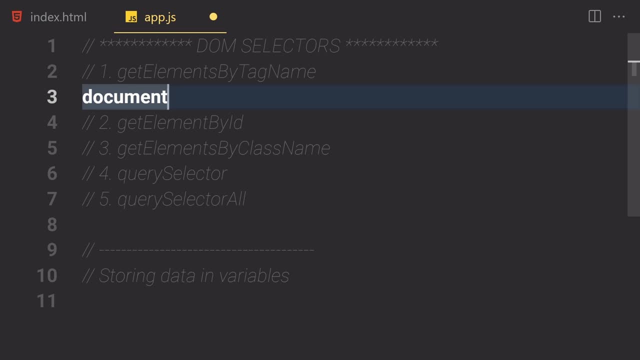 first of all, if you want to select something, so we are going to be writing our document, because this document is our main object, so we are going to be accessing all of our properties and method from this document. so now, if you want to access this method, like get elements by tag- 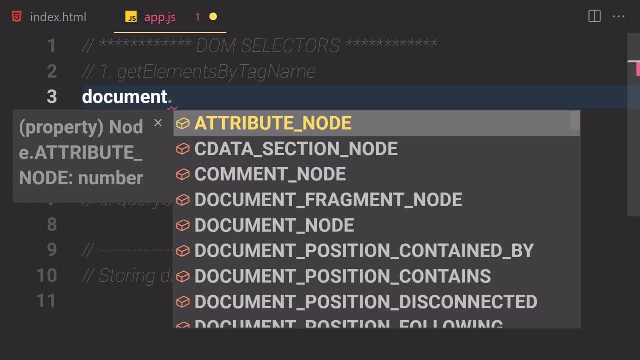 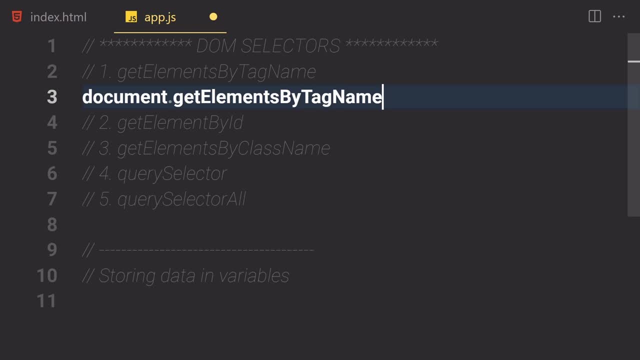 name. so what do i have to do? i'm going to just write dot or period, whatever you want to call it, and then i'm going to just use the name of that method, like get elements by tag name, okay, and then opening curly brace- not curly brace, but opening parentheses and closing parentheses. 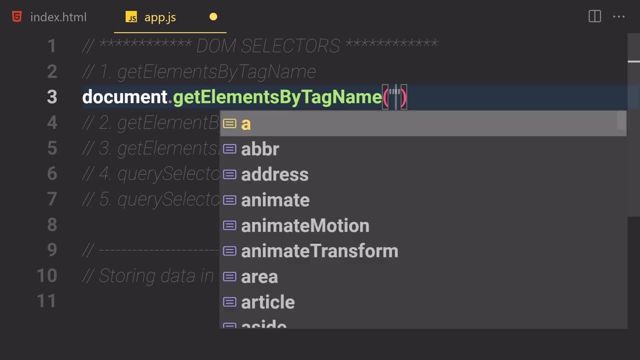 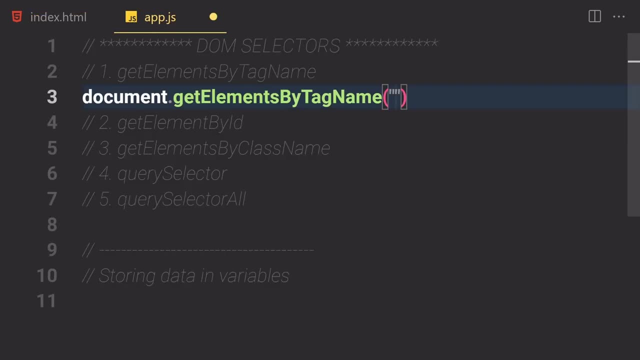 and inside these parentheses we just have to specify the element names, so which one we want to select. so if in this case we want to select that html, so i'm going to just write h1 in it, okay, so now let's just log there to the console real quick. 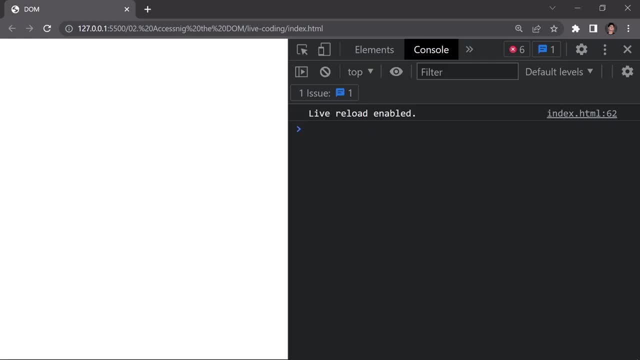 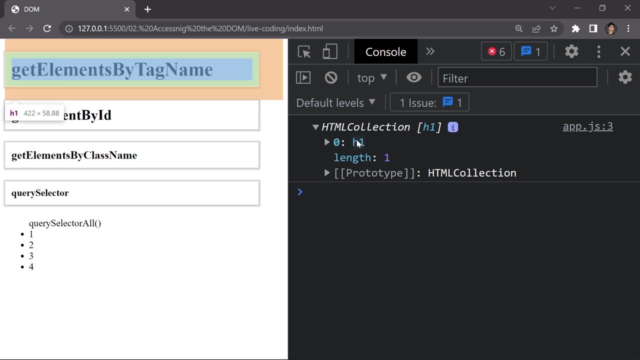 so consolelog and like so. so if you save that, and now here you can see, it now gives us the collection of that element. so we have, uh, zero value because there's some sort of array, but it's not an actual array, it's a collection if we hover our mouse over to it. so here you can see. 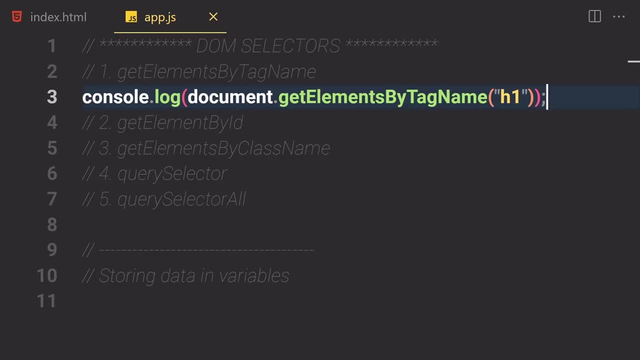 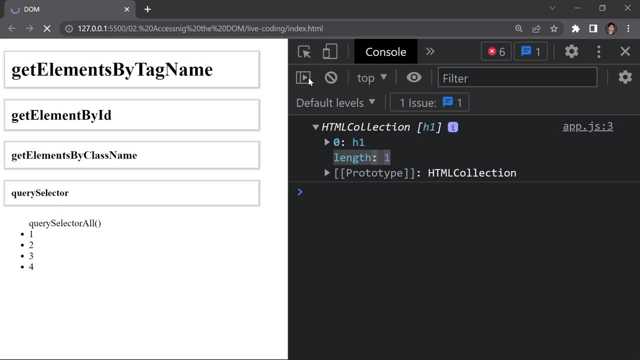 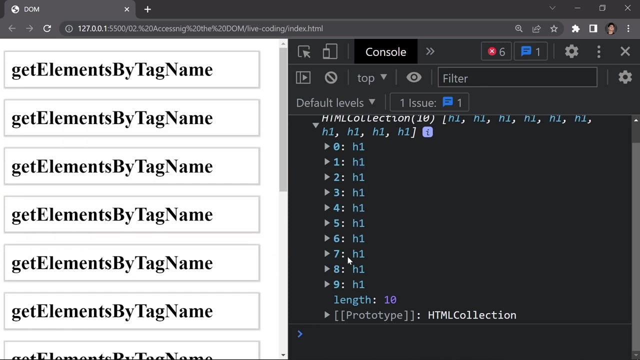 it will now select that h1 right here and the length is one. now, let's suppose, if we have more than one h1 inside our html document, so if you just duplicate that a few times and now, if you save that, and now here you can see, inside this collection we are getting all of that h1s right here. so we have one, two and 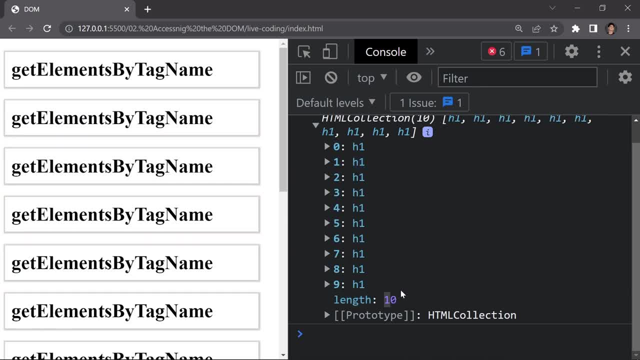 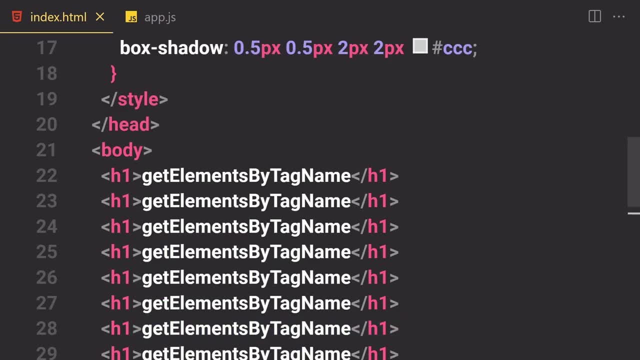 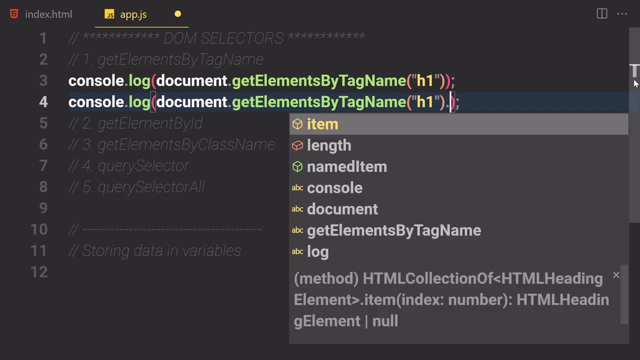 blah, blah, blah through nine and here you can see the length is 10 right here and you can also see the inside or web page right here. so i'm going to also get a length. so in some cases you would need the length of our html selector so we can just duplicate this line and we can just write a length. 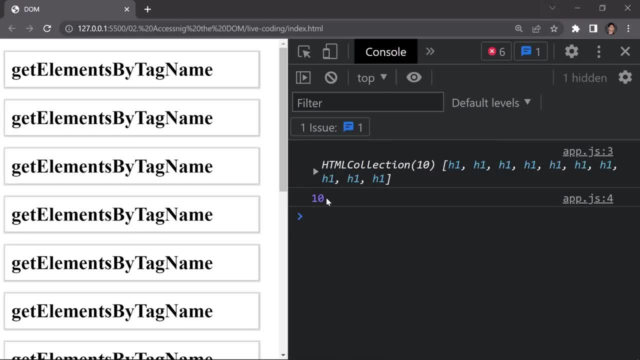 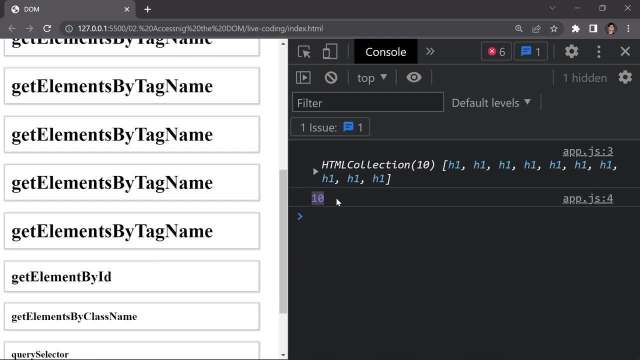 property on there. so if you sell that and now here you can see it will now gives us 10, like the length is 10, so we have 10 items starting from the zero through 10, so it will just gives us 10 uh values, whatever you want to call it. so that was the first selector about get elements by. 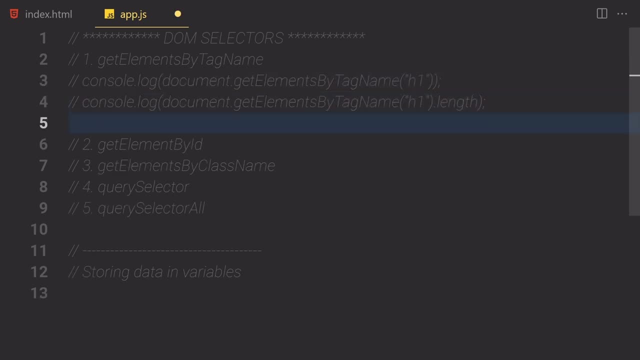 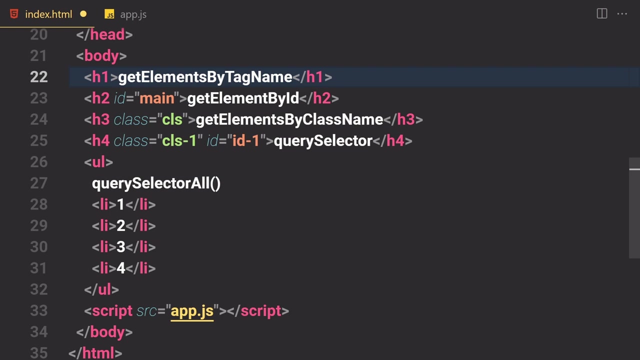 tag name. i'm going to comment these and i'm going to hit enter right here just for separation purposes, and i'm going to remove, uh, all of these. i just want to accept that first line and zoom it out to the right, but that was just a first selector. like get elements by tag name, if you want. 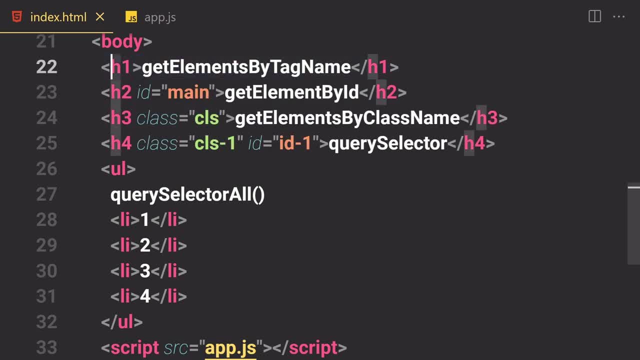 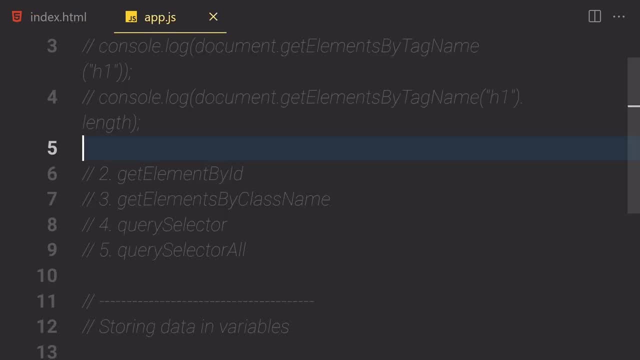 to select something by a tag name, so you can just specify the tag name. it doesn't matter if you provide like h1, h2, h3 for ul, span, article, section aside, header, footer, etc. etc. you just have to provide it inside these double quotes right here. okay, so it will just select it for you so that. 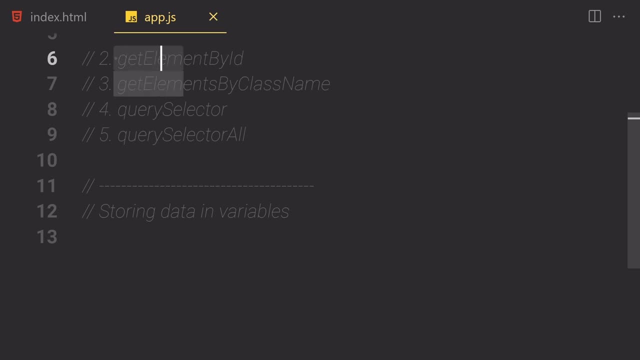 was just it about for first selector. now, the next selector we have is a get element by id selector. uh, it's a method, but it allows us to select something by tag name. so that was just. a first selector we have is a get element by id selector. it's a method, but it allows us to select something. 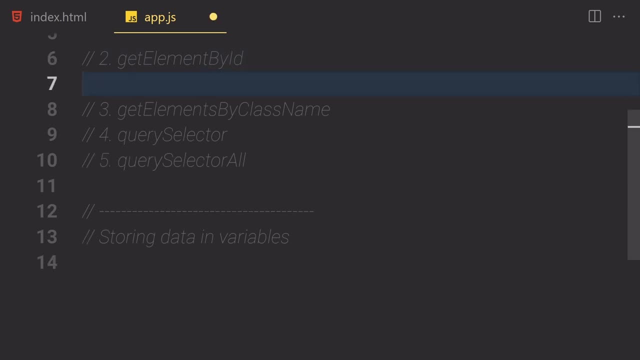 something by using ID. So what do we have to do? I already give you the answer, So I want you to give me the answer. What do we have to do to access this element? Well, first of all we just have to write document and then we can access or get element by ID method on there. So what do we? 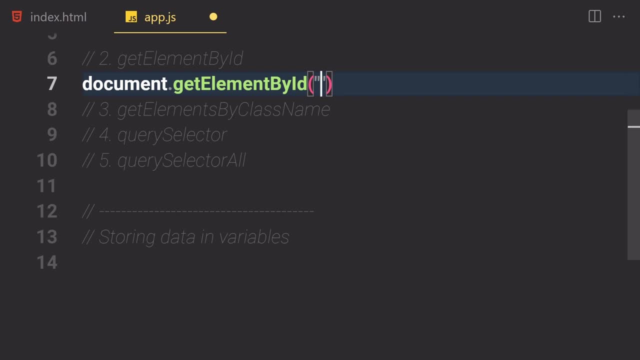 have to do in this case. we just have to give them the ID name right here. So what is the ID name? the ID name is man, So I'm going to just copy there And I'm going to put it right here. 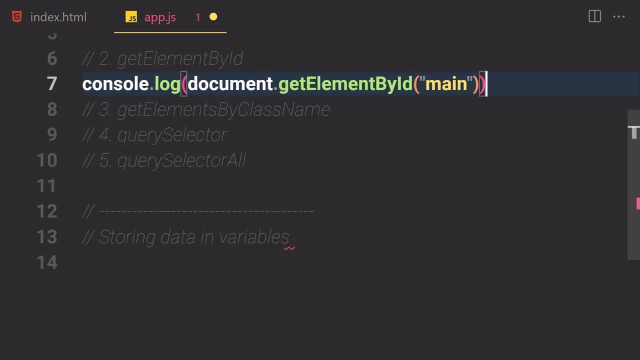 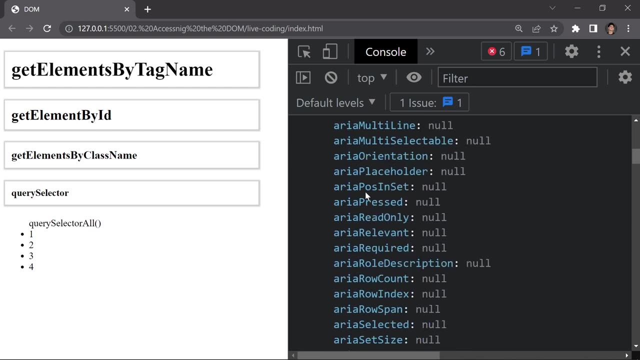 And let's just log there to the console and see what will we get And if you sell that. and now, here you can see, we have that H2 with the ID of man right here. So if you click on that, we have different kind of properties and its values for this H2 right here. Okay, so this is. 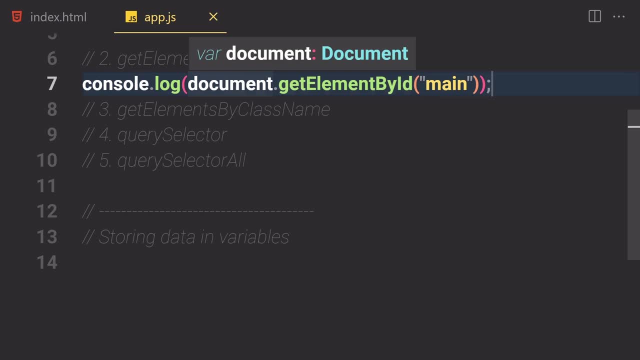 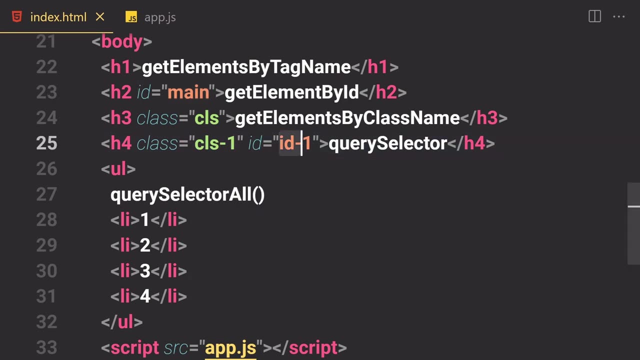 our H2.. And this is how we can select something by using get element by ID method, right here. So if you have another ID, like I don't know, maybe if you want to select this one, so I'm going to just copy this ID and I want to pass it right here. So I'm going to copy this ID and I'm going. 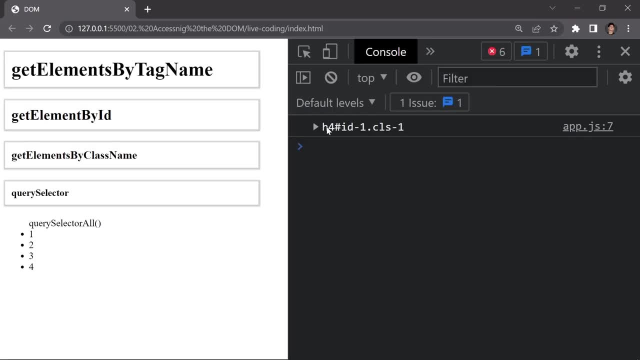 to pass it right here And I'm going to just send my file And here you can. it will now give us that H4 with the ID of one and also the class of one, So like CLS one. So here you can see we have. 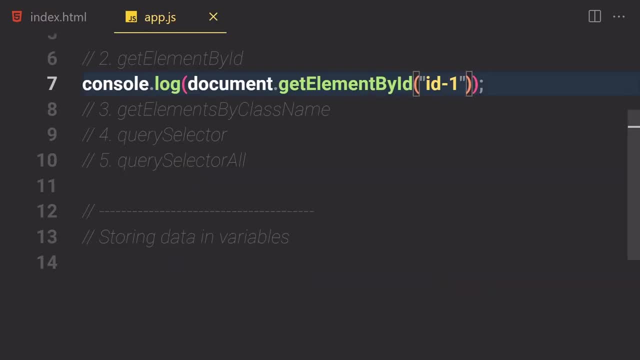 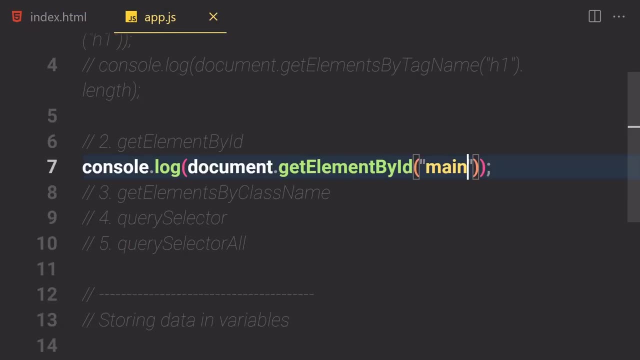 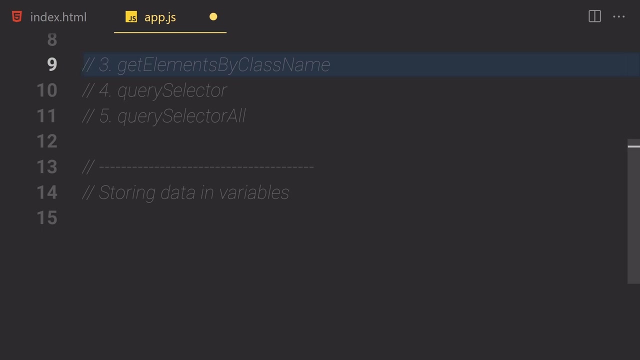 a class of CLS one. Okay, so this is how we can select something by using ID, get element by ID selector. So I'm going to copy this main And I'm going to pass this man right here. it will not give us that man right here. I'm going to comment this line out as well. Let's just start working. 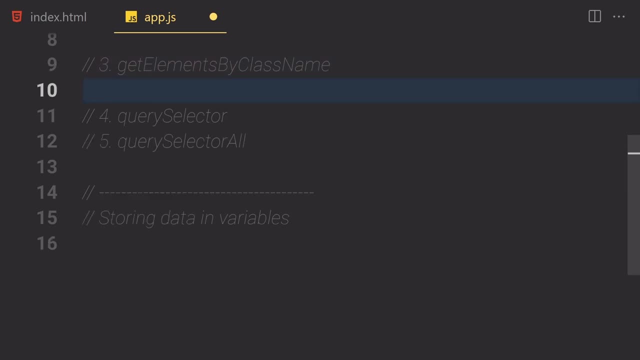 on our next one, like get element by ID selector. So I'm going to copy this main and I'm going to pass this one right here, And here you can see the class of all of our classes- and I'm going to get element by ID selector. So I'm going to tell you a little bit about what I mean by get element. 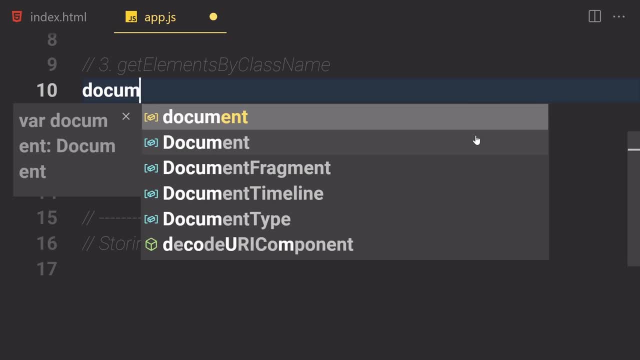 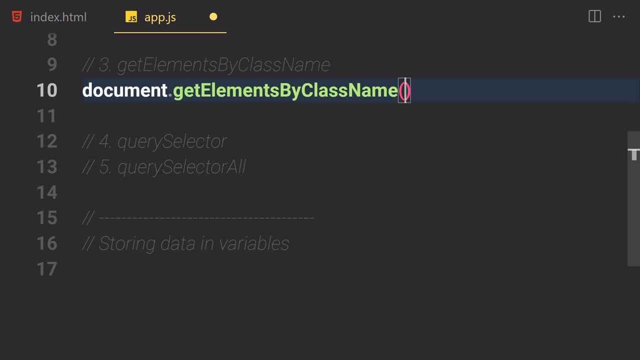 by ID Files. a lot of us are used to getting all our elements by class name and, as the name suggests that it will, allows us to select our element by using a classes. So first of all we have to write a document, So then we want to get our get element by class name. kind of a long 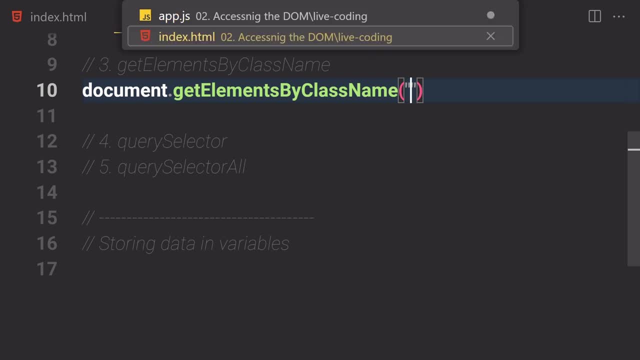 method right here. But here we have to specify our class name in a quote. So which kind of clause we want to select? So we want to select the CLS clause. I'm going to copy that And I'm going to paste it right here. So if you save file, then we have to log there to the console so that we can. 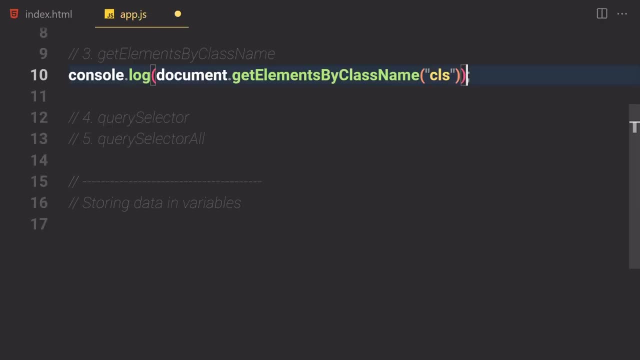 see everything thing a bit better. i'm going to zoom out and this is how it looks like. so we have consolelog, then we have our document and we are accessing this method on this document. okay, so the value we provide, or cls, and now you want to check if that value is available or not. so if you sell file, 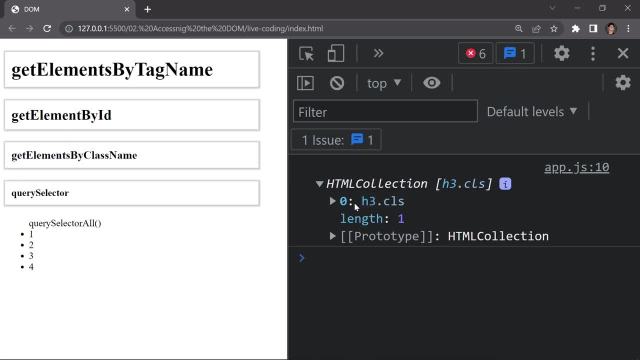 and now here you can see, the log uses that um value right here. so we have this h3 with the class of cls and now if you hover mouse over to it, it will now select or highlight there in that kind of orange color right there. okay, so we are now selecting this one. what if you don't have like? 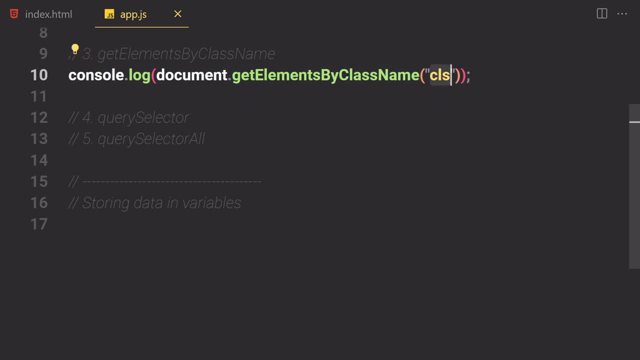 uh, that clause, if you just provide uh invalid class, like i don't know, maybe if i just provide apple and if you save that, it will now gives us nothing, because this html collection did not found. uh, that apple class certainly now gives us empty collection, right here. okay. 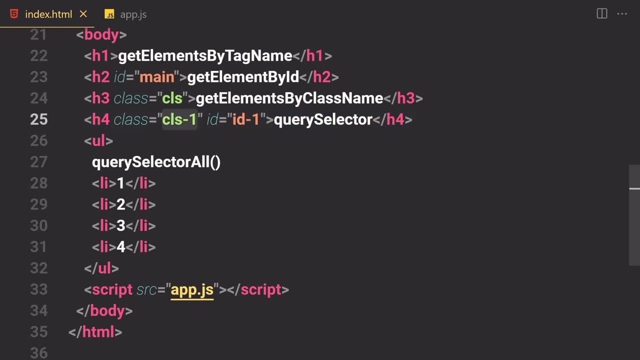 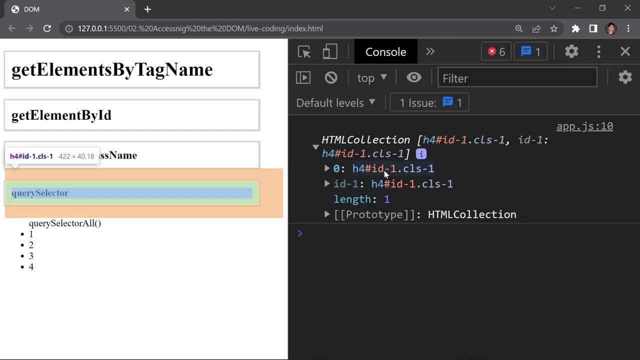 so what if we provide uh, this class right here, so like cls one, copy there and i'm gonna paste it right here. save is server file and now here you can see, it will now select that h4 with the idea of uh id one and also the class of cls one right here. okay, 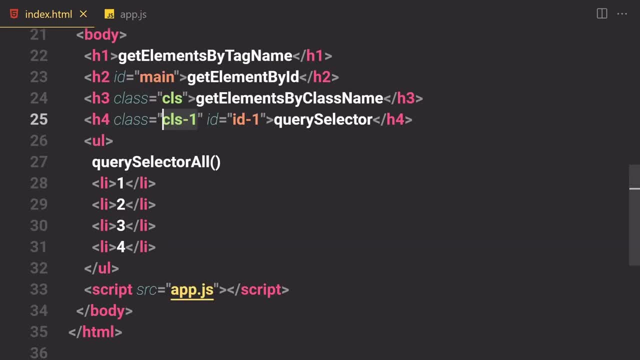 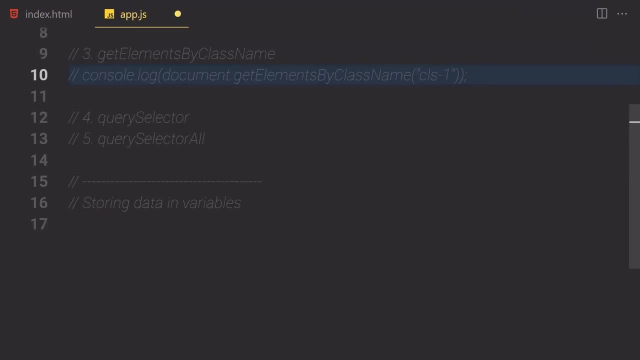 so it will now select this cls one right there. anyways, that was just it about, for get element by tag name, get element by id and get elements by class name. so now, what about this query selector and this query selector, all so? now let's just discuss that a bit. i'm going to comment this line. 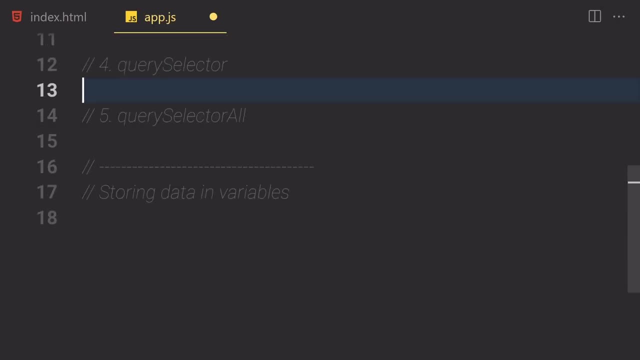 out and then let's give group a name after that. so let's give class name a name and give class name. I'm going to start working on our query selector. So query selector is the most used one and my favorite one- selectors. So throughout the course you're going to see me using query selector If 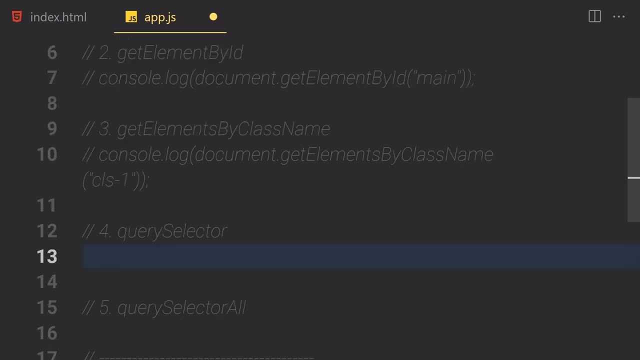 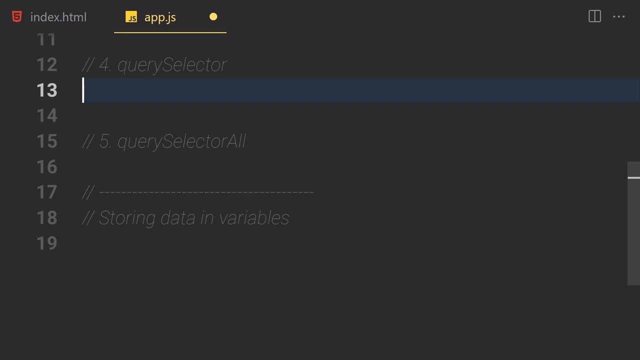 you want to use, like some other selector, like maybe tag name, ID name, blah, blah, blah, which we already learned, So you can also use that. But for me, I'm going to be using this one And I'm not saying that you don't have to use the other one And you should use this one. I'm just 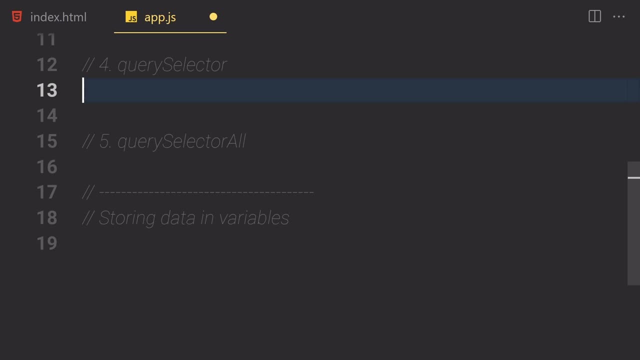 saying like I really like query selector because it allows us to select something, or select or elements by using just a CSS selector. So if you want to select something by query selector, so you just have to write like I don't know. if you want to select like class, so we have to just 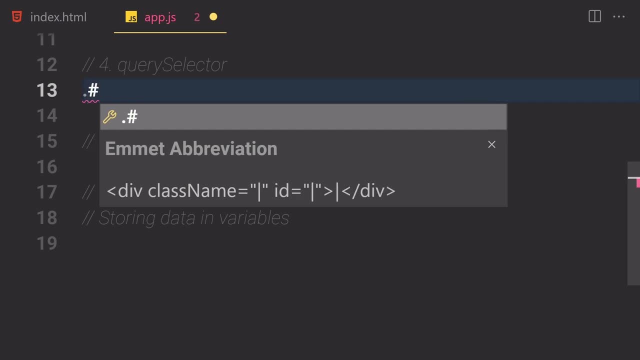 write a period. If you want to select ID, so we have right pound symbol. if you want to select a tag, so we just have to write a tag name. Okay, so I'm going to show you that just in a second. 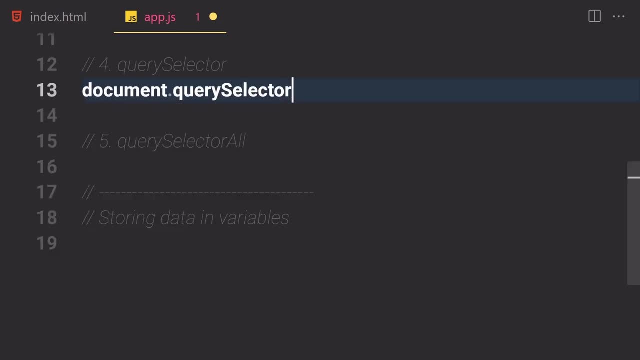 First of all, we have to just write document, then query and then selector. Okay, so query will be in lowercase, and then this s will be uppercase, and then the rest of them will be in lowercase. Okay, so this is how the syntax will look like. And then we have our opening parentheses. 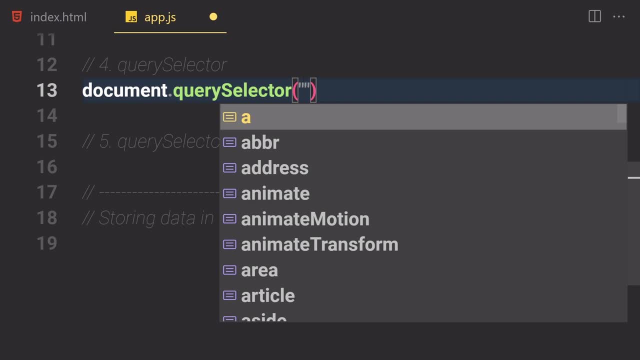 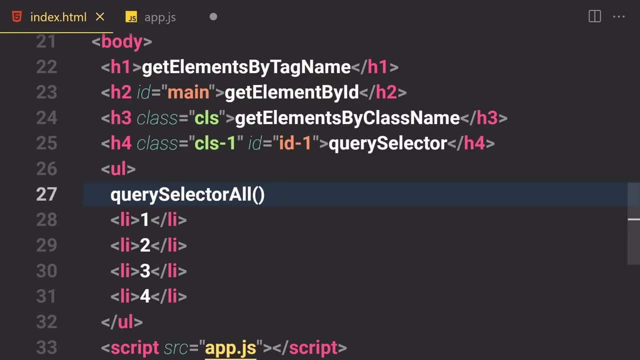 and closing parentheses, And inside these parentheses we are going to be writing our strings. So here, if you want to select something by tag name, let's suppose, so you just have to write a tag name like h1, maybe, if you want to select this h1, so we are going to be just writing. 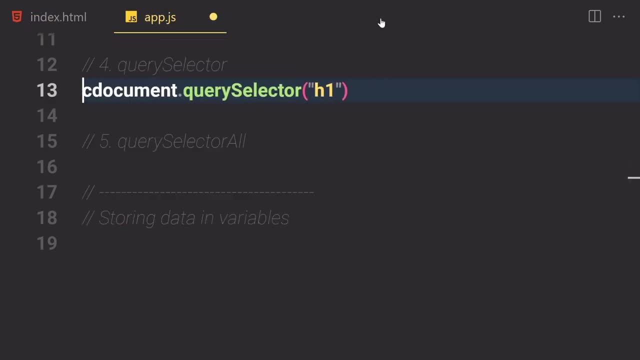 or h1.. And now let's just log that to the console real quick. So console dot log. And now, if you save our file, and now here you can see, it will not select that h1 right here. Okay, so if you want to select something by class, so you just have to write period or dot. 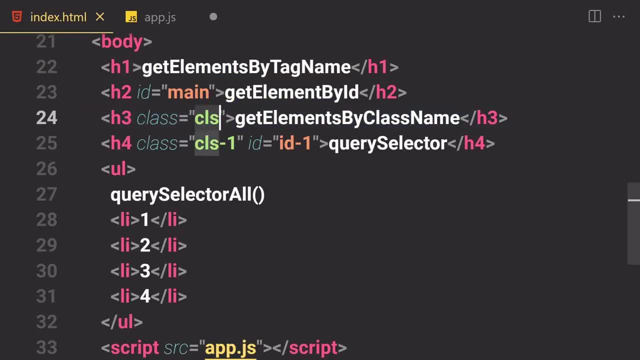 and then the class name. So what was the class name? the class name was CLS. I'm going to copy that And I'm going to paste it right here. So if you save our file, it will not use that h3 with. 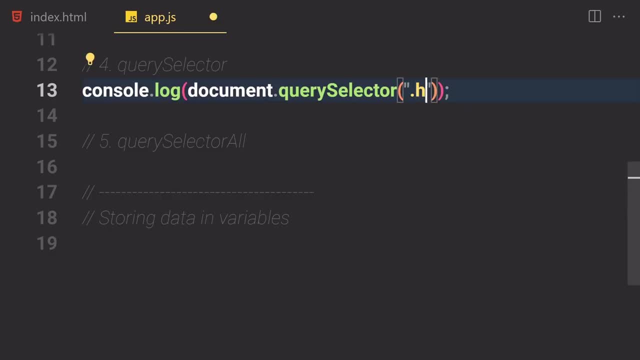 the class of this CLS. If you don't have some classes- like maybe I just want to write my own name, And if you save our file, it will not use this nil or null, whatever you want to call it. Let's suppose, if you do provide this class right here- but we forgot to include that period And 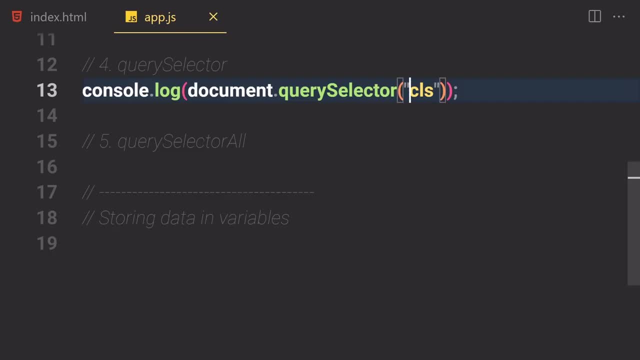 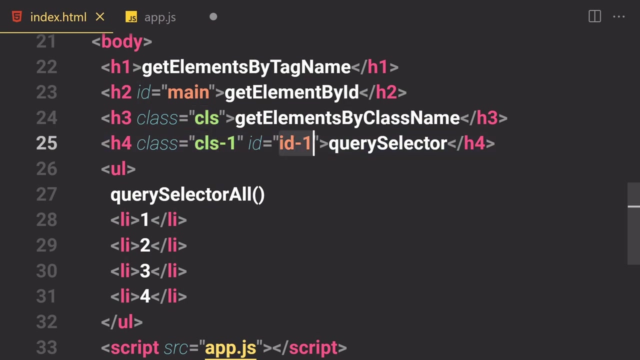 now, if you save that, it will still gives us that nil class right here. That's because we forgot to include that period right here. Okay, so that was it about how you can select something by tag name and class name. Now let's just learn about ID selector. So if you want to select this ID, so we 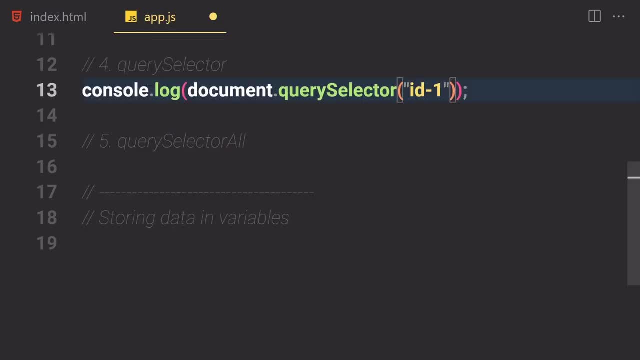 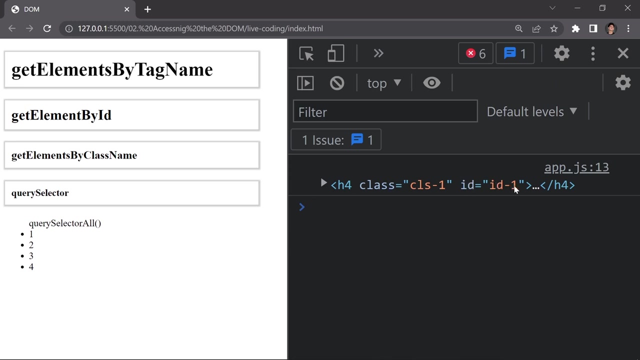 are going to be copying this name, paste right here. But first of all we have provide or pound symbol here, So we have to specify this pound symbol and then the ID name is just like a CSS selector And if you save our file it will not select that h4 right here. So here you can see, we have that ID. 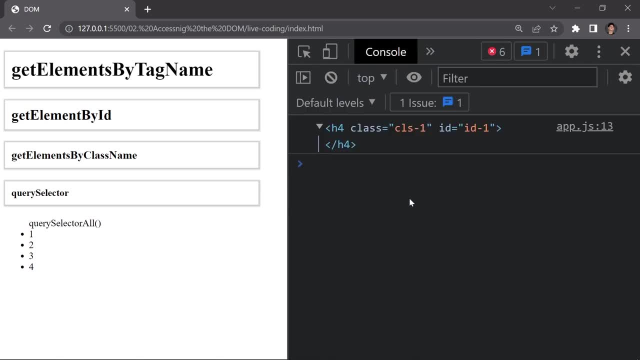 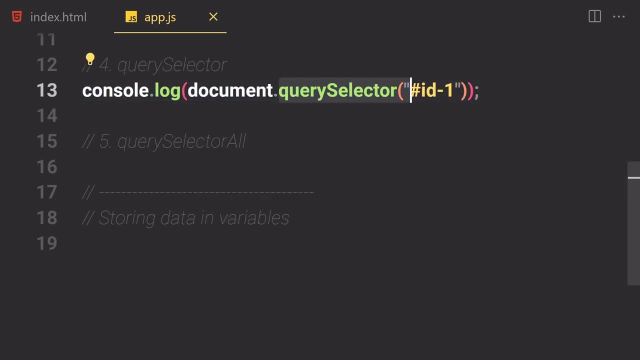 of one on the selector. So yeah, that, that's that Anyways. So that was it about query selector. but it will just gives us one element at a time. So if that selector like I know, let me just show you. 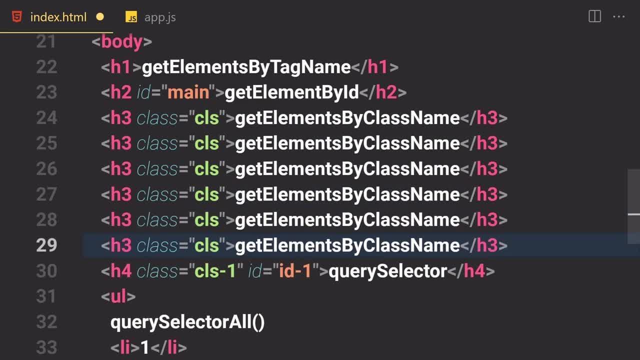 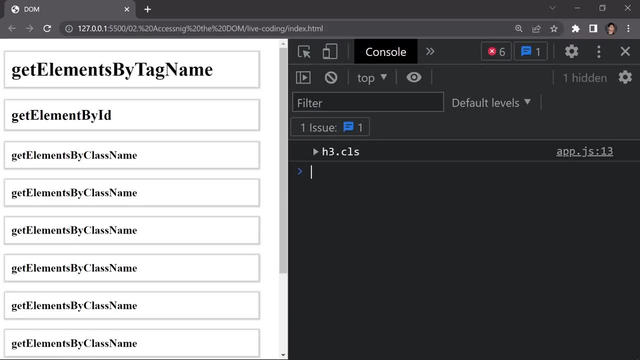 that You know I'm going to duplicate this line of code a lot of times And now, if you sell that, okay, so I'm going to put my CLS right there. So CLS and knife, you sell that, it will just select. 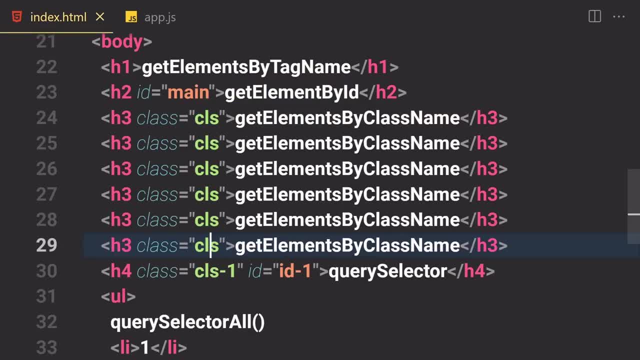 that first one. it will not select all of them. Here you can see we have like 123456 classes right here, So we we reuse this class like six time, but it will just select the first one, like this h3,. it will not select this one, this one, that one and 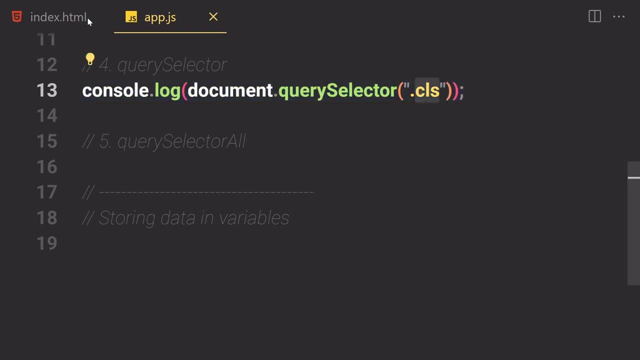 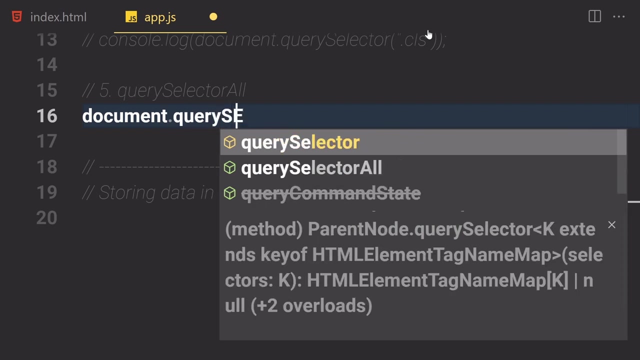 any of them, but it will just select the first one. So if you want to select all of them at once, so for that we have another method called query selector, and all right here. okay, so I'm going to comment this line out And instead I'm going to be just writing, like document dot: query selector. 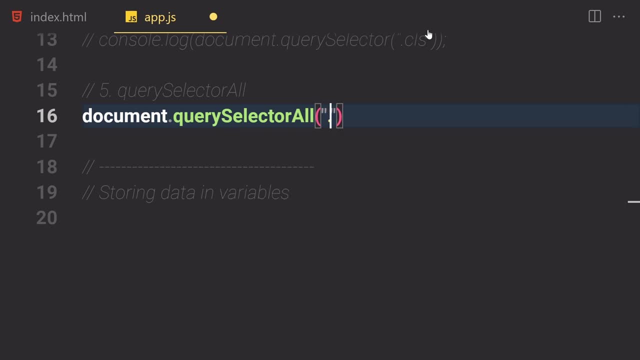 all and now let's just provide or query selector, all like just period and CLS. And, by the way, if you want to select something by using ID, so you just have to provide a pound symbol. If you want to select something by tag name, so you just have to provide a tag name like h1, or span, or 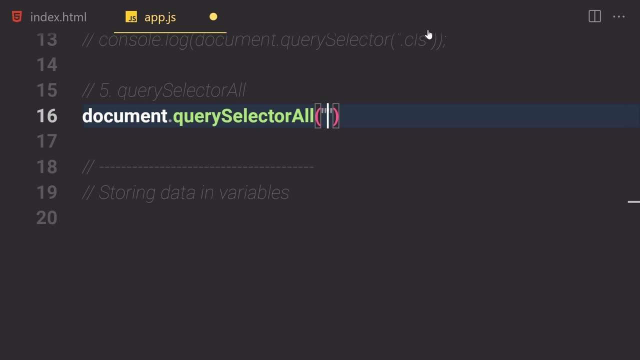 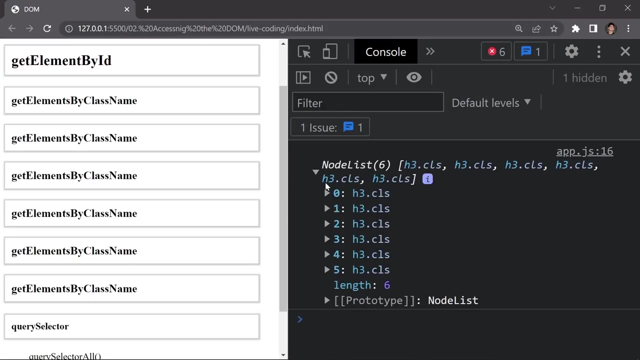 section or whatever. all of them will work in here as well, just like a CSS selector. But now, in this case, you want to select all of their allies. I'm like CLS classes, So you just provide CLS. I'm going to just write console log And if you sell a file, it will not select all of these CLS. 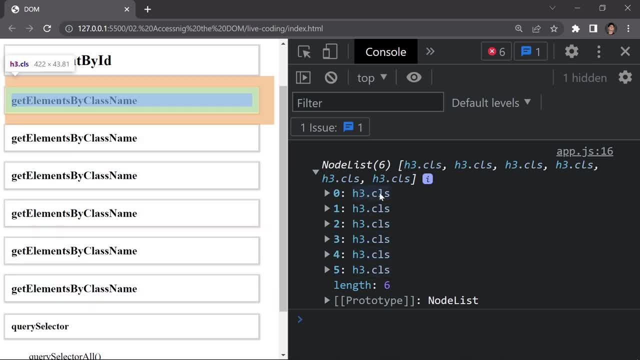 right here, Like I'm like: Why am I saying CLS? Yes, CLS is the class. That's what I'm saying. Okay, so we'll now select all of their CLS. I'm going to comment this line out, And now let's. 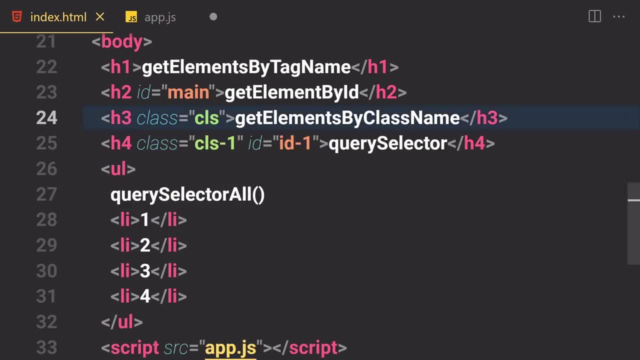 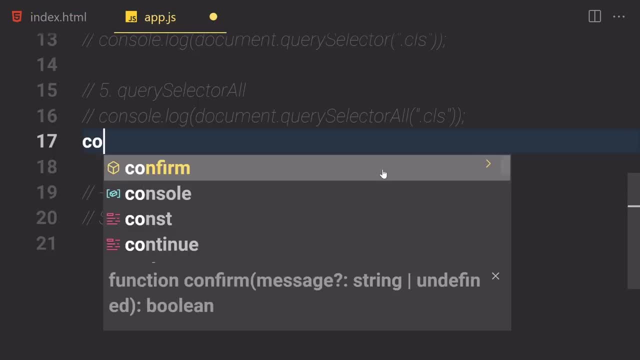 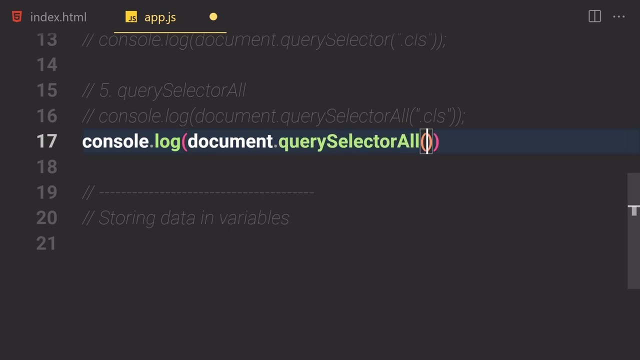 suppose if you want to, you know I'm going to remove that. Now, let's suppose if you want to select all of these allies at once, So for that we can use this query selector all as well. I'm going to just write console dot, log of document dot, query selector- all this method inside this query. 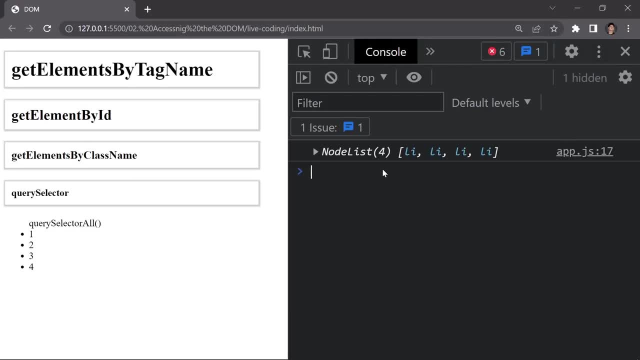 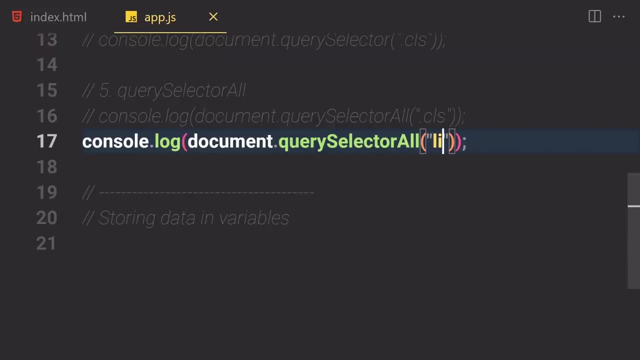 selector all I'm going to just provide a live right here. So if you sell that, it will not select all of these and I right here. We have a one, two, three, four right here And the length is also four And we can also provide. 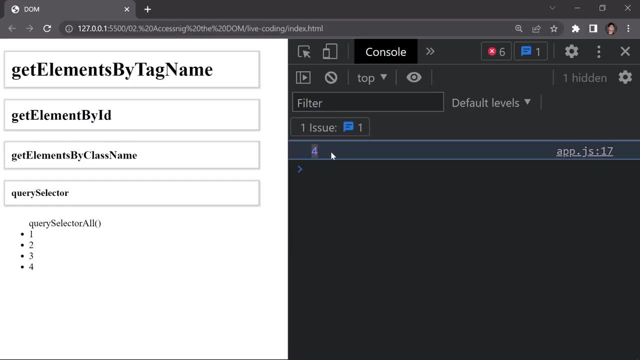 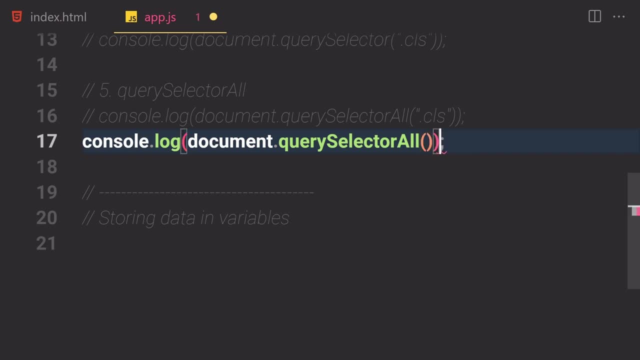 dot length property in this one as well, So it will not gives us the length of four Anyway. so that was it about a labor of query selectors and all of that kind of good stuff. Okay, we have to provide our quotes in there. What else I wanted to show you? Okay, so if I just write like Li, right? 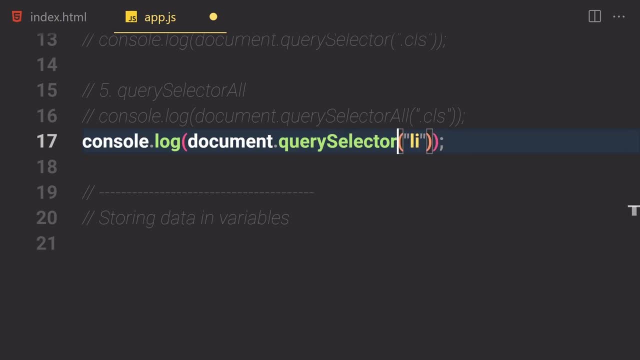 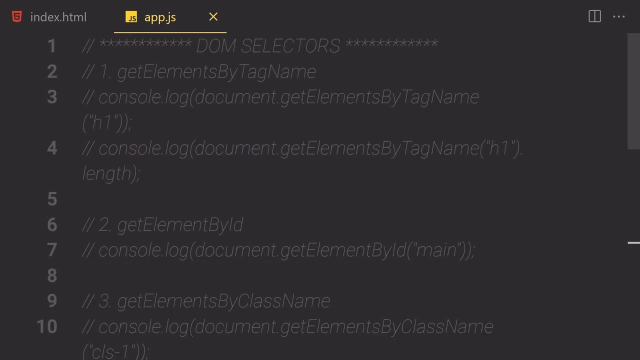 here and instead of query selector all, if I just remove that all and if you sell that and here you can see, it will not just select the first one right here, like this one, A lot of talking, I'm going to just provide query selector all. I'm going to comment this line out. So now, here you can see, we 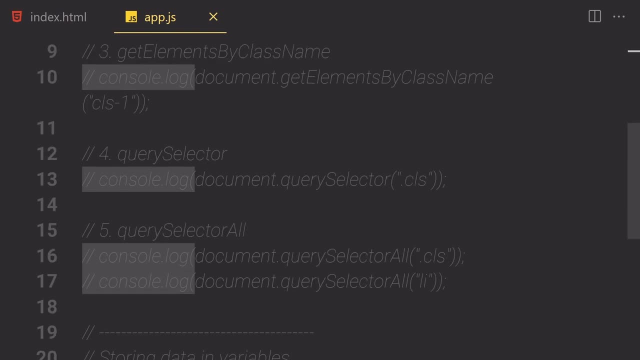 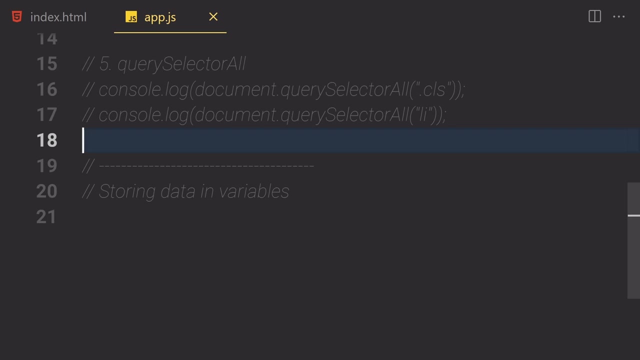 are just console logging all the time. we have like console log one, two and blah, blah, blah a lot of times right here. So instead of logging everything to the console, we can also store everything in variables, And I'm assuming that you already have a little bit of knowledge about JavaScript, if you 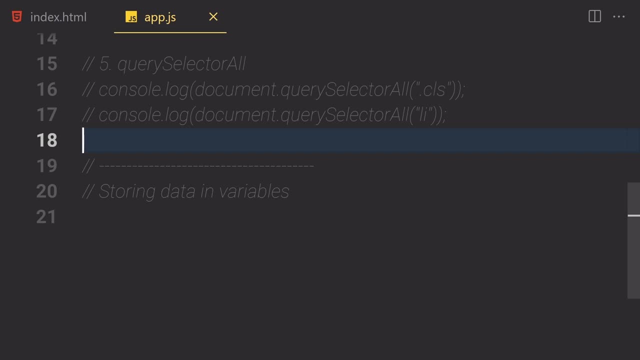 don't have a little bit of knowledge in JavaScript So you can check out my post or entire playlist. I've got totally entire playlist for you. you can check it out And it's totally for free. So now let's suppose if you want to select something and you want to store the value, 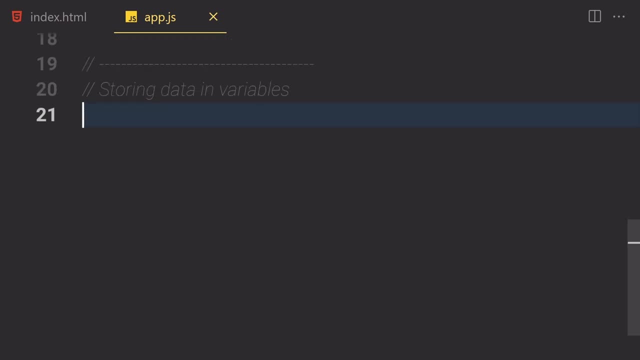 of that in some sort of a variable, So you can also do this. So let's suppose if I want to select that h1, so I'm going to just write const h1, or let h1 or war h1. So you can use whichever kind of. 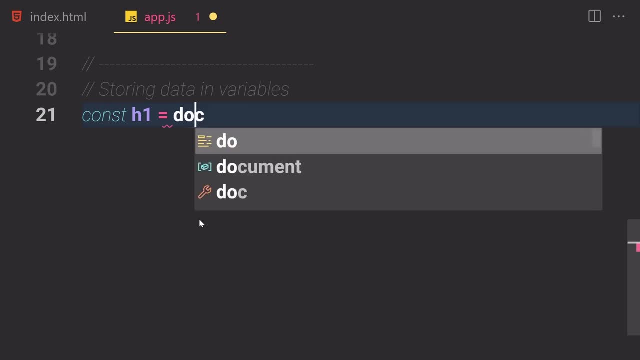 you like, but in my case I'm going to just select the h1.. And here I'm going to just write document, document, dot. query selector of our h1.. Okay, so we are using our tag selector. So if you just log, 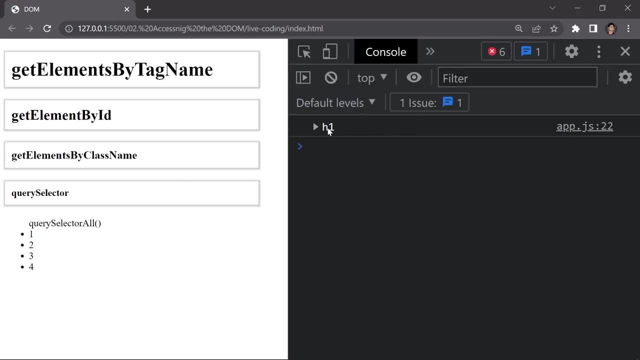 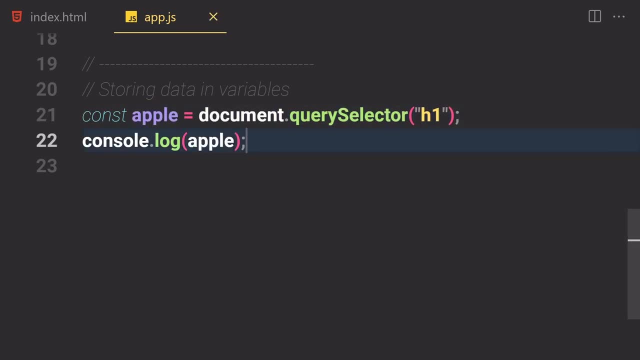 that to the console like h1, and if you sell that it will just log that h1 to the console And the name doesn't matter. you can give him like Apple name, let's just select that Apple and it will still work. But you have to specify the correct selector inside this method, right here. 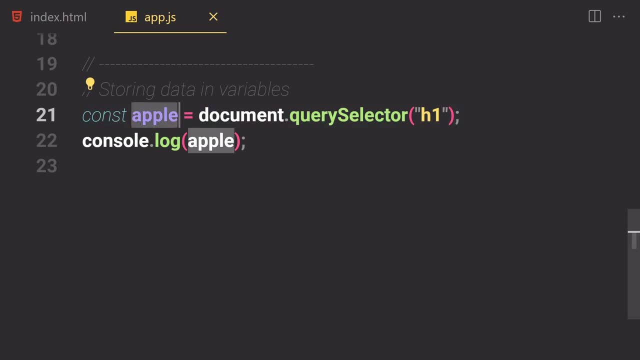 Okay, this is just a simple variable, So you can store your values inside this variable. So I'm going to set back there to h1.. So h1, you can also just set that, like I don't know, h1,, L or 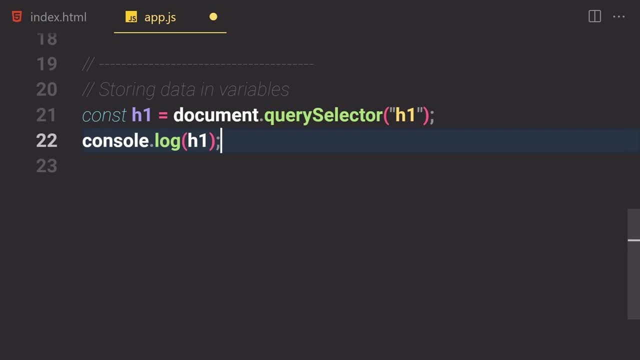 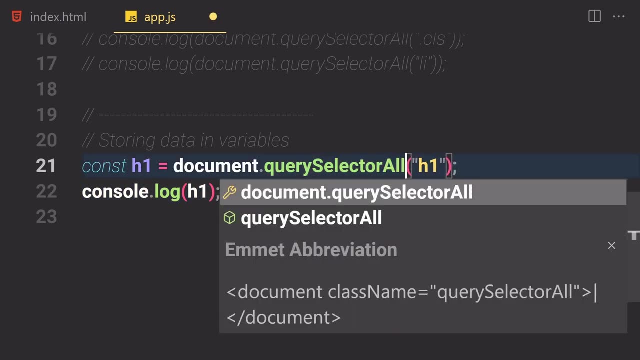 element if you want to, But in my case I'm going to just stick to that h1.. So if you save there, it will not give us that h1.. If you want to select, if you want to store multiple values, like query, selector, all, and you want to select their allies, So if you sell that it will not. 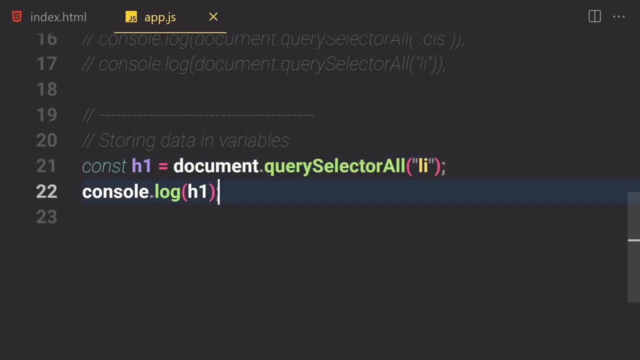 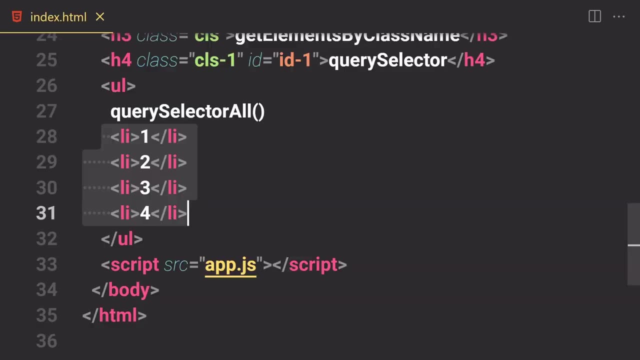 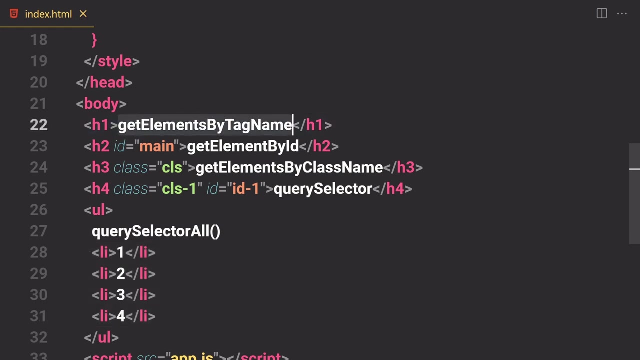 use the collection of all of these allies right here. Okay, so everything is working the way we expect them to work. Okay, so we are totally done with this section. So in this section we just learned about a few selectors. we learn about get element by tag name. it allows us to select something by using a tag. 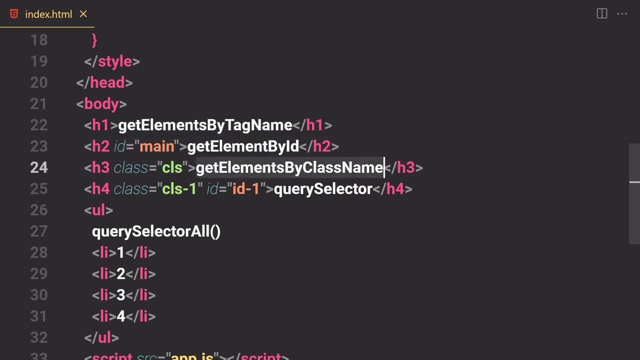 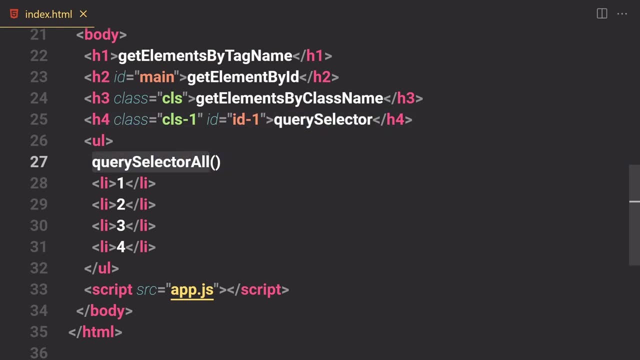 name. then we learn about get element by ID. we also learn about a get element by class name. we learn about a query selector and query selector all query selector, inquiry selector- all- will allow us to select or element by just using a CSS clauses like period, pound symbol and all of that. 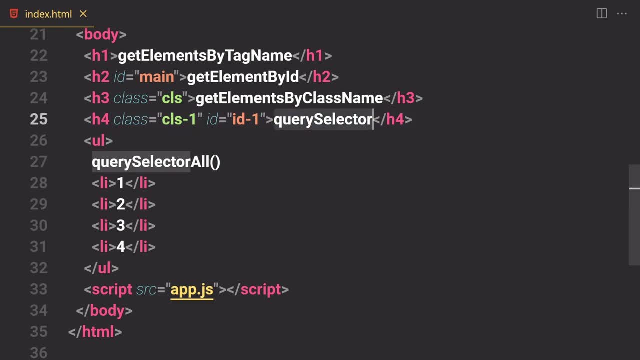 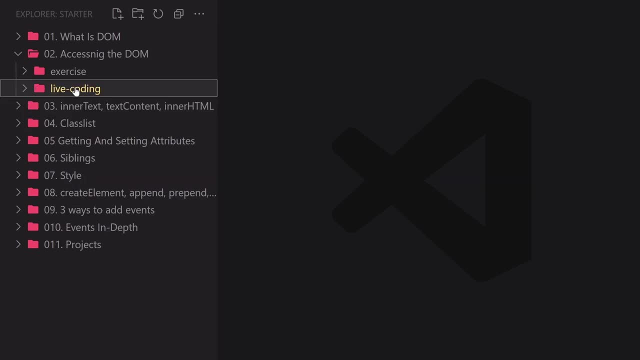 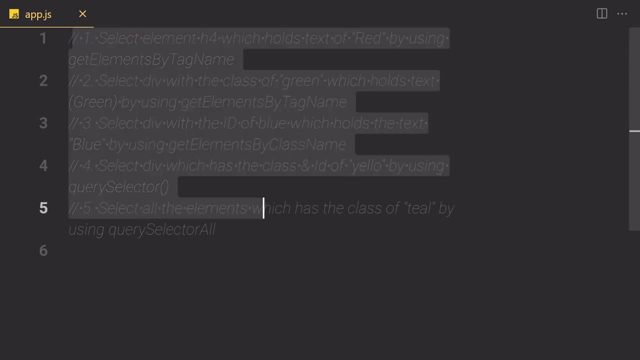 but this will just gives us the first element, but it will not use the collection, And this one will give us all of the collection, like so, Okay, so now it's challenge time. I want you to just open this file And I want you to just open this F dot j's file And I want you to just read through. 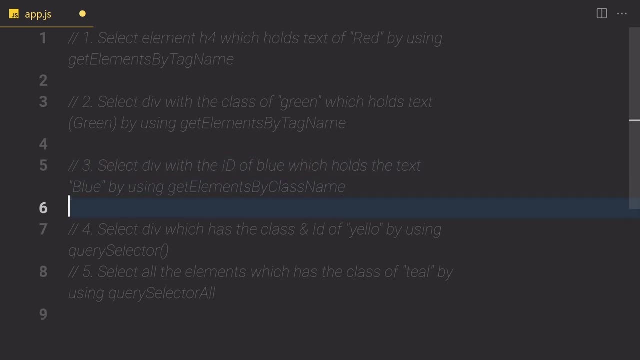 this instruction and solve this challenge by yourself. If you can do it, that's totally okay. Then I want you to come back and continue with the review, And now I'm going to give you my solution. So what are they saying? select element h4, which holds the text of red, by using get element by tag. 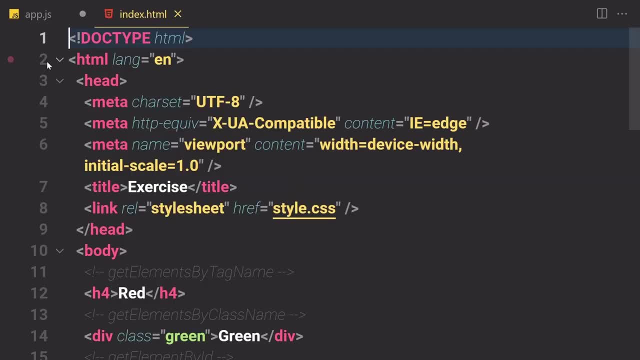 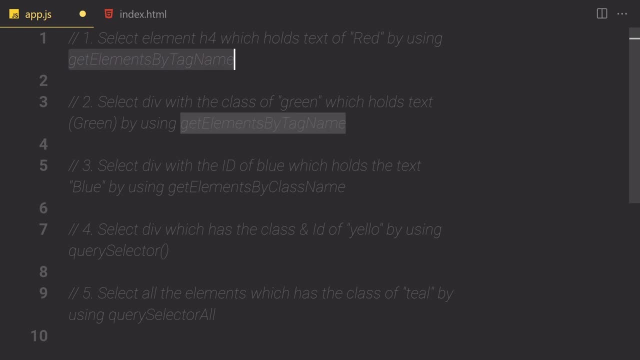 name. So let's just explore- or HTML- I'm going to hide this head area. So we have this h4 with the text of red right here. So what do we have to do? we have to select that by using get element by tag. 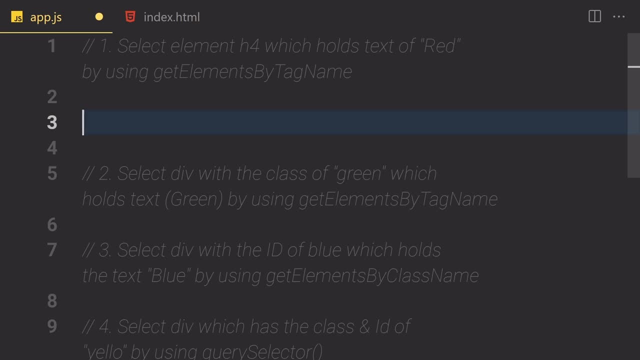 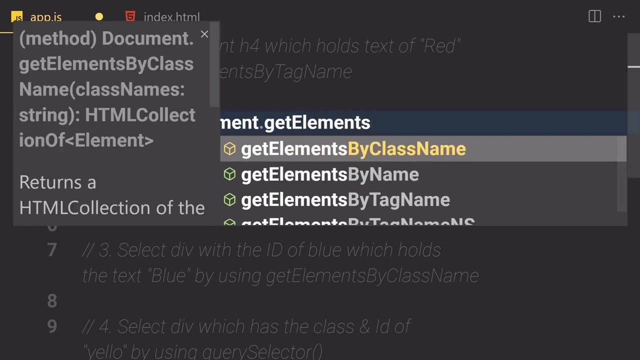 name. Oh, my goodness, is the most simplest, the most simplest challenge I can give you. So let's just write const And let's just store that inside h4.. And I'm going to just use document dot: get elements by tag name, elements by tag name, like so. Now let's 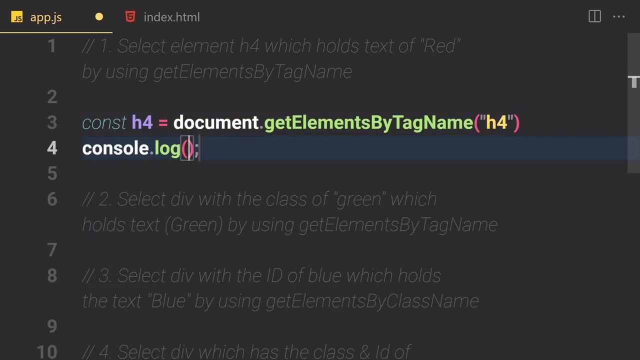 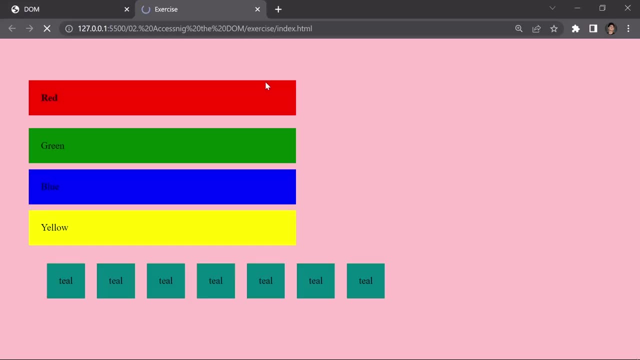 just put our h4 in it, And now let's just log that to the console like h4 and knife is out there and boom. Okay, so we have to launch this indexhtml file. my bad, launch this one. say bye, bye to the. 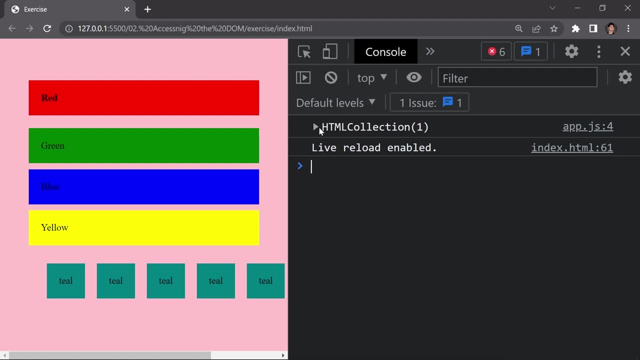 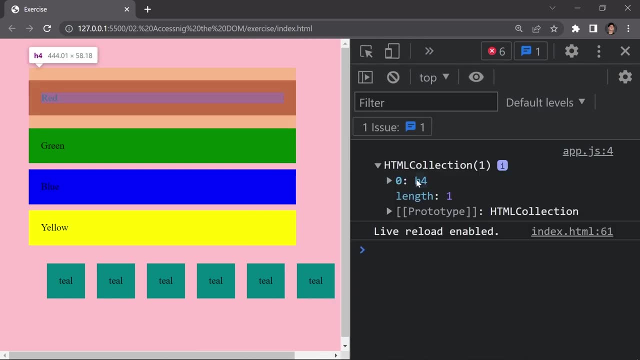 other one. Open our console, And here you go, We have our h1.. And we, I mean, like we have our h4 element selector right here. Okay, so let's just refresh that. Open it And there we go, We have our. 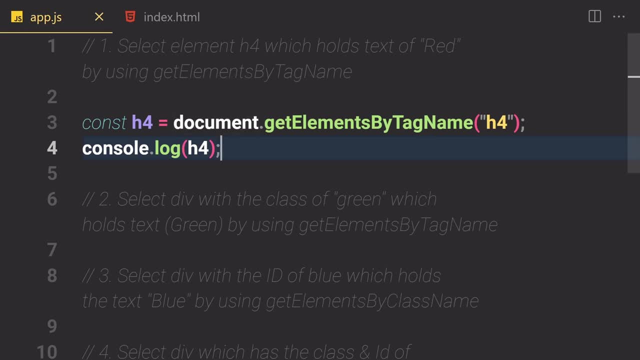 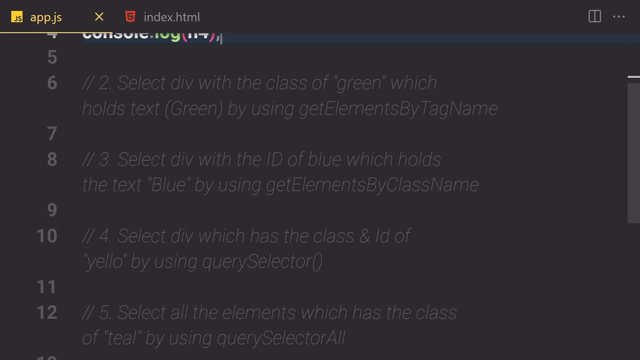 h1. I mean like h4.. Alright, so that was the first solution. Now, the next thing which you know, the next thing which you have to do, is that we have to select a div with a class of green which holds. 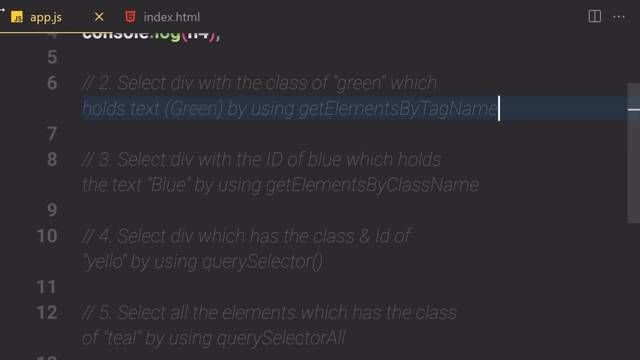 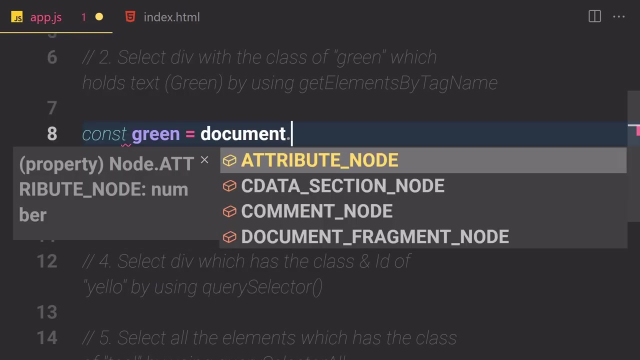 the text of green as well by using get element by tag name. So let's just explore that. we have a div with a class of green And we want to select them by using this get element by tag name. So let's just write or const, and then green in this case, and document dot. get elements by what? 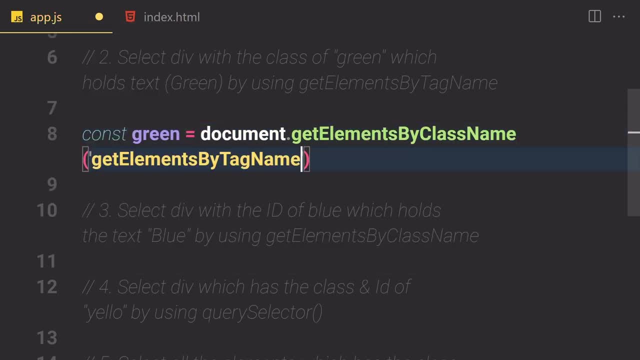 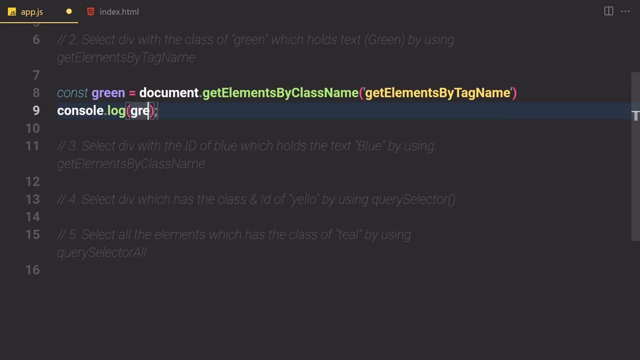 by class name. And now let's just put or not, period, but we just have to specify the name because we are not working on a query selector. And now let's just log that to the console like green, And if you sell that it will not Okay, so something isn't working. 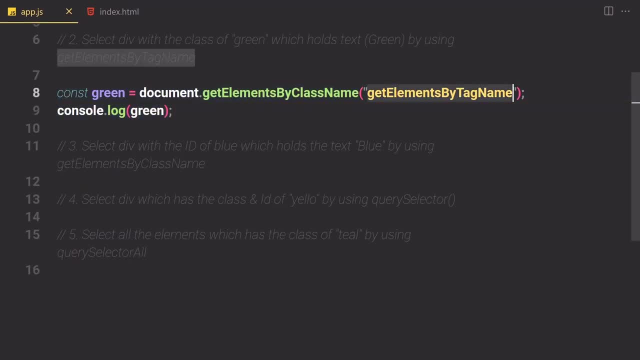 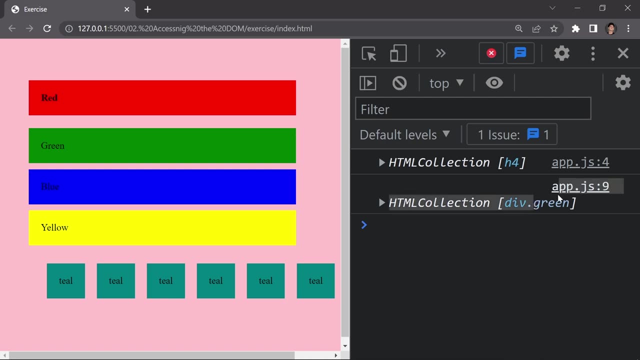 Get element by class name is a green- Oh my god, it's a green, And knife is so there, and it will not give us a div with a class of green right here. Okay, So the second challenge is also done. I'm going to comment both of these console logs from there. 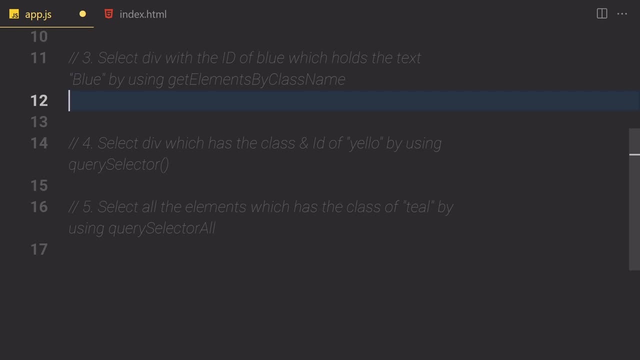 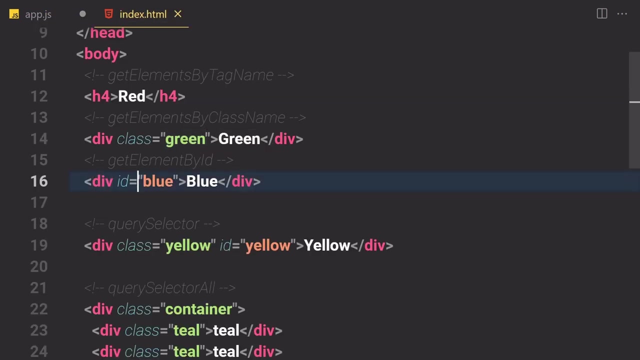 because we don't want to clutter or console. So the third thing which you have to do is that select div with the idea of blue, which holds a text of blue, by using get element by class name. Yeah, there we go. So let's just see, we have a div with a class- not class, but idea of blue. 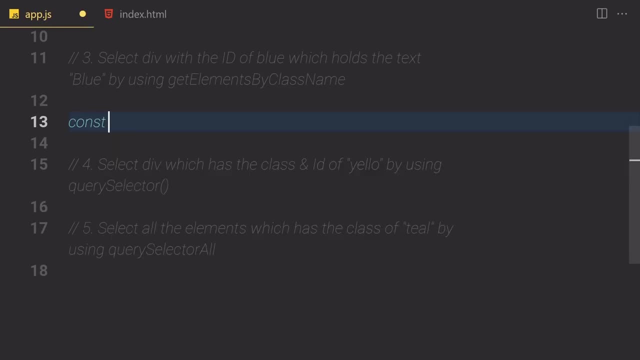 And the text is also blue. So we just have to write like cons blue and inside BL blue, and it will be equals to document dot this, get element by class name or just copy. there I cheated a bit. you can also do cheating if you want to. And now let's just log this blue. 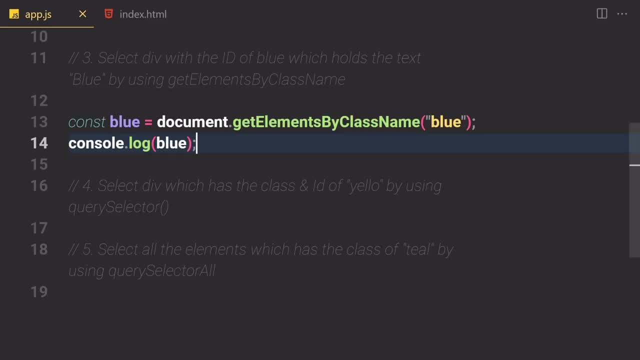 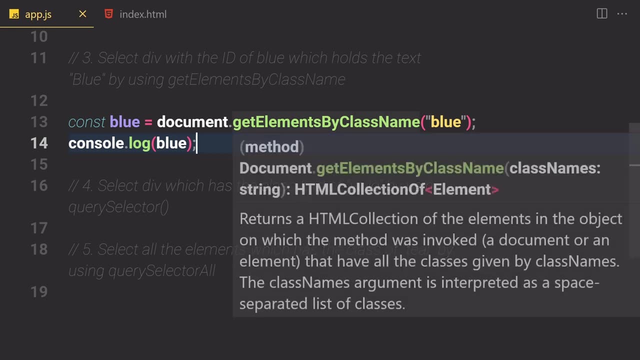 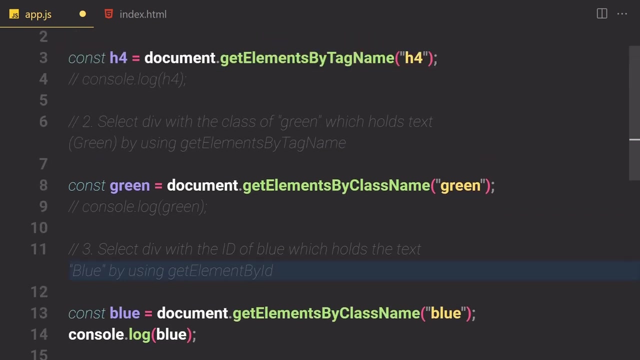 to the console and knife is so there. Okay, so the one, the class of one. select the div with the idea of blue. Okay, so we are using a class name, not a class name. get element by ID ID. my bad, sorry, This one is a tie And this one is a class. now. 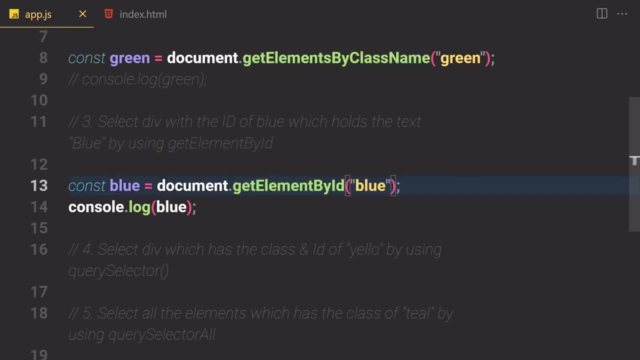 get element by ID copy there And I'm going to pass it right here, said art. So here you can see the log uses div with the class of blue And by the time you're watching this video you will get this correct instruction. you will not see that query selector or whatever that was. 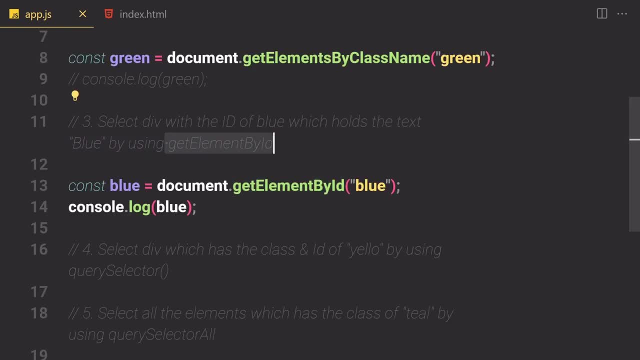 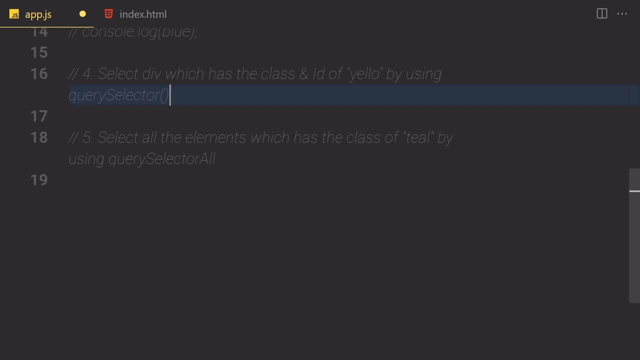 I mean, like I get element by class name, it will be a get element by ID. I'm going to comment This line out. And now what else do we have to do? select div which has the class and ID of yellow. 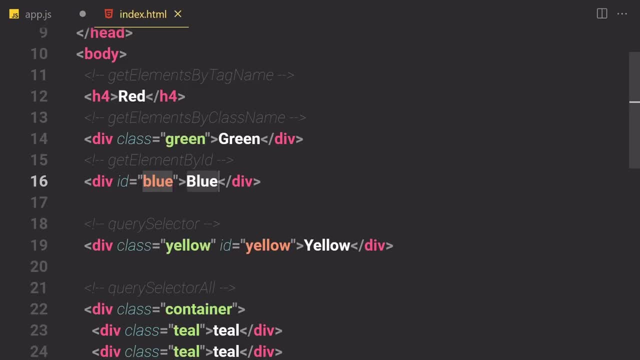 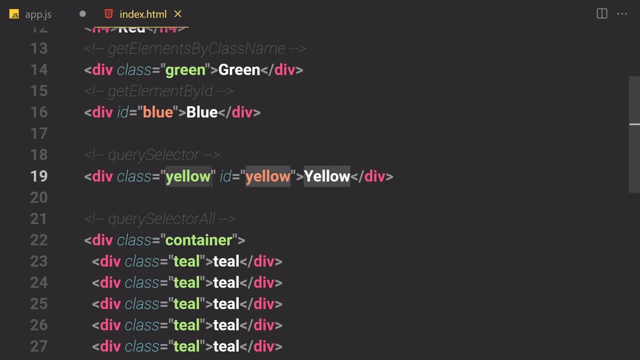 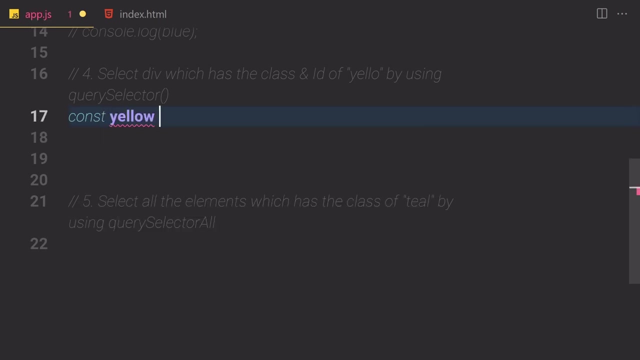 we yellow by using query selector. let's see, Okay, so this one do have a W at the end. So, David, the class of yellow, ID of yellow and text of yellow. So we are going to be using that, using a query selector. I'm going to just write cons a yellow and will be like us to document, dot what. 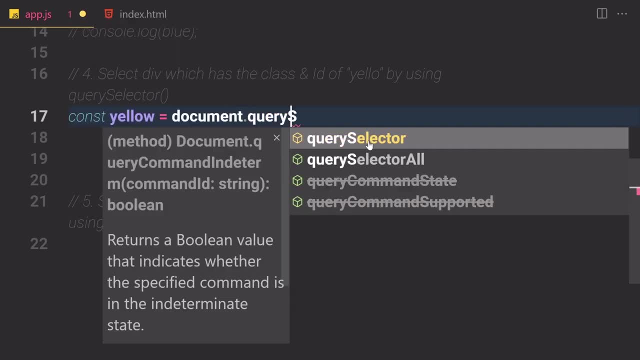 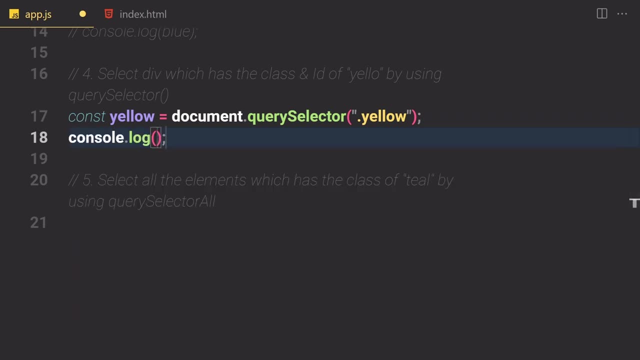 query selector- Document dot. query selector of just a yellow in the class And let's just log that to the console real quick like yo low, so them a lot. selected as a clause. we can also selected as ID, because we have a yellow ID as well. 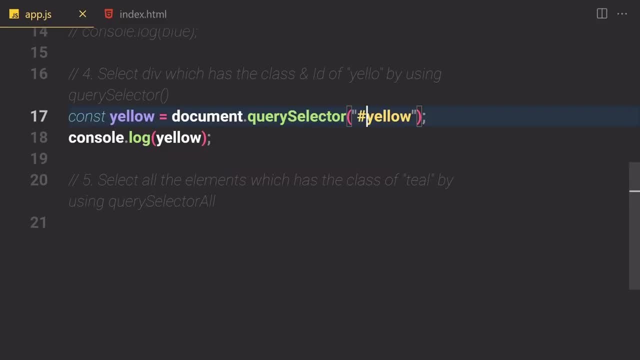 A and we can also select how we can also fing else. So we just have why they're selected by clause or by ID Arts. that's working less of. if you just forgot to include that pound symbol, save it, it will not give us nil. we already expected. 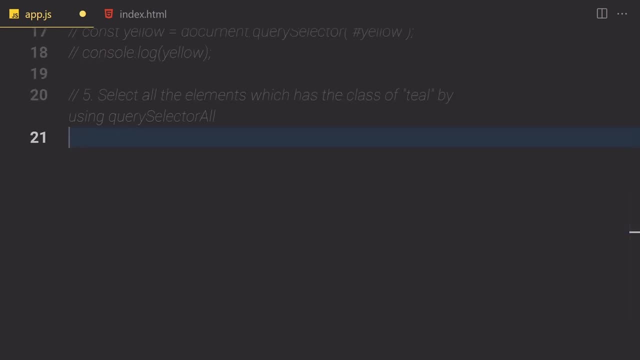 that comment this line out. so the final thing which you have to do for this exercise is that select all of the elements which has the class of deal by using query select row. okay, so let me just show you that and real quick: cons all deals. you can give any name you like: document, dot, query. 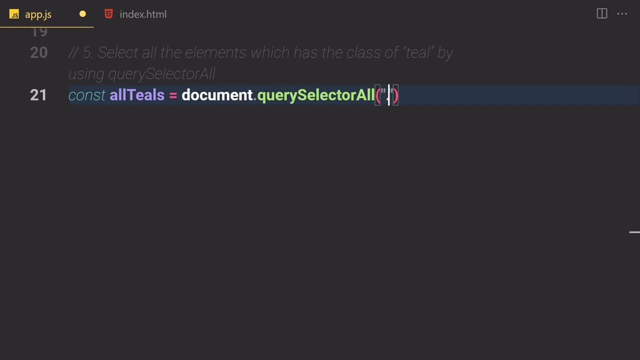 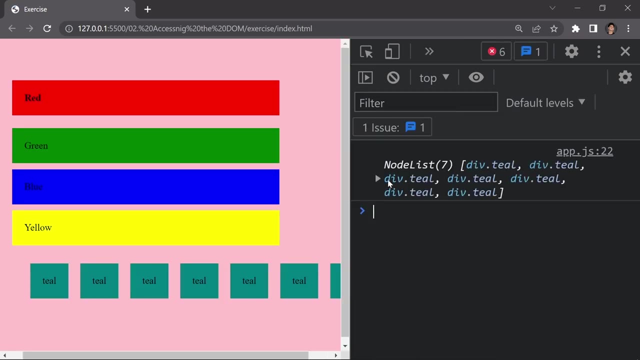 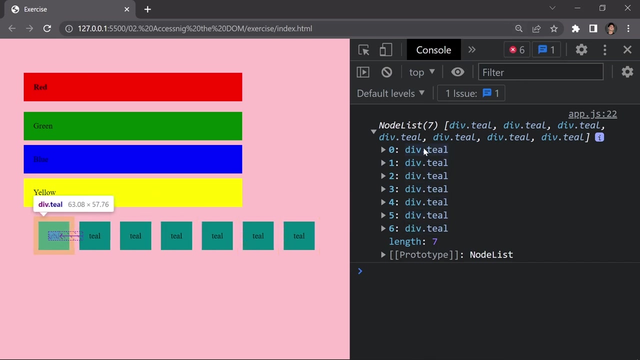 select row and inside there we are going to be selecting our teal. okay, so let's just log there to the console like all teals. and now, if you save that, it will now select all of these teals right here. so if i hover my mouse over to it, so it will now select all of these teals right here, okay so. 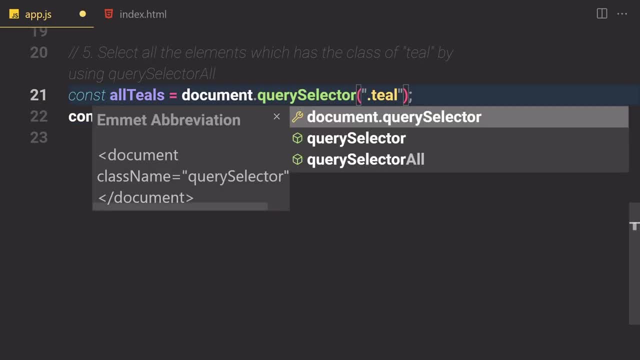 let's suppose if you just provide query selector instead of query selector all and if you save that, it will now just gives us the first one. it will not give us the rest of them. so that's just the difference between query selector and query selector all. so in this section we just learned. 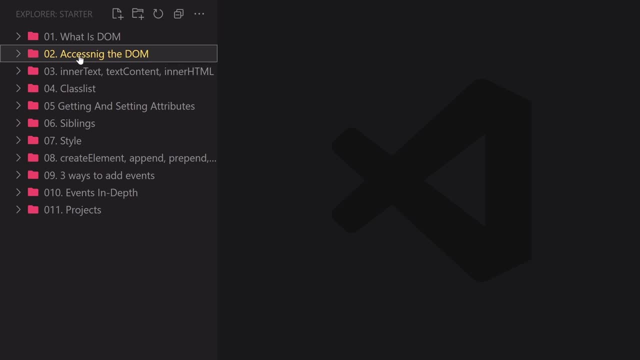 about accessing element by using query selector. all so in this section, we just learned about accessing element by using the dom, accessing the dom element by using javascript. there we go. so, now that we learned how we can access elements from a dom, the next topic which we are going to be: 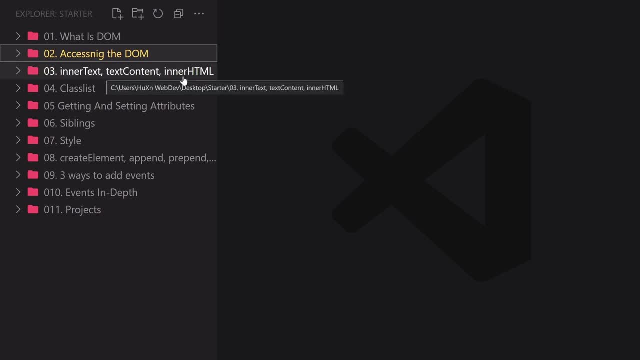 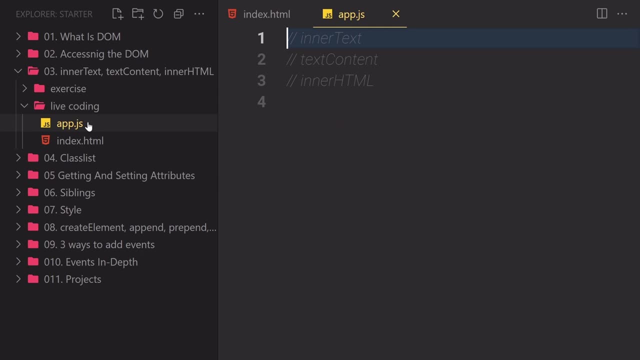 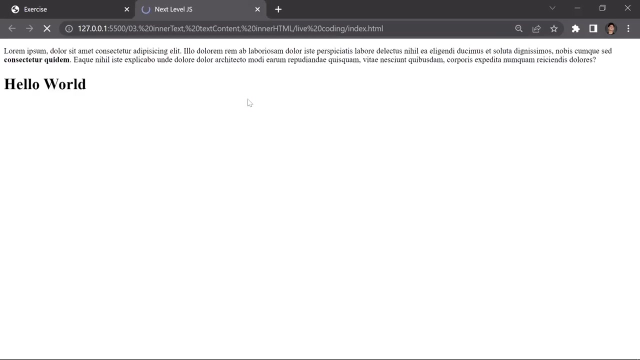 discussing is how we can get the inner text: inner content and inner html. so we have two folders, we have a live coding, so i'm going to just open my indexhtml file and also the appjs file and then we will have our exercise. okay, so just right click on it and open it with a live server. so now just 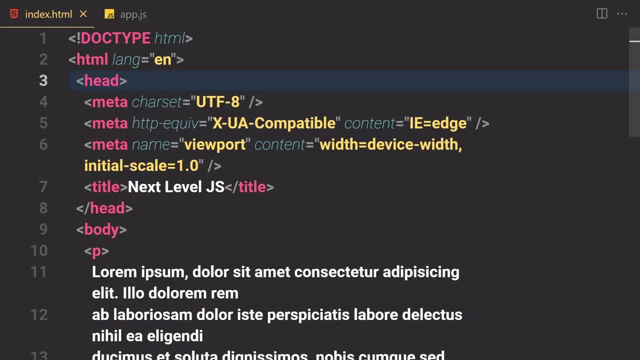 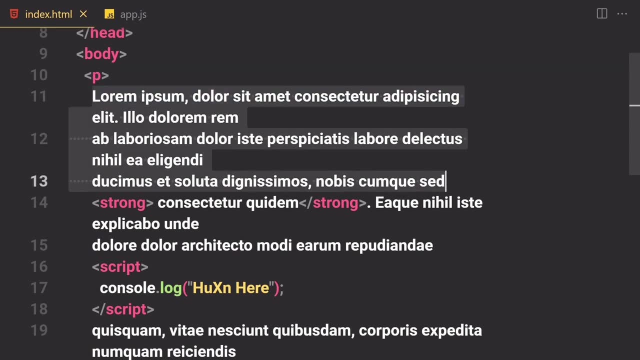 go to my server and i'm going to also open my dev tools as well. so now i'm going to just grab this head area for now. and now, here you can see, we have our p tag. inside this p tag we have a few- um, just random words right here, and we also have this strong tag right here, and we just put a little. 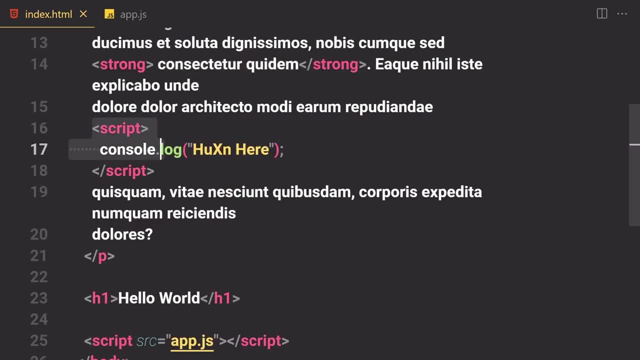 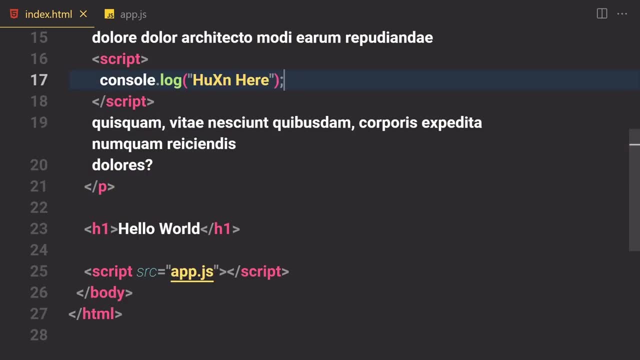 bit of text inside this strong tag as well, and then we have a script tag inside this paragraph as well, and then we just log that to a console like huzzan, here, right here, okay, and then finally, we just have our h1 with the text of hello world. 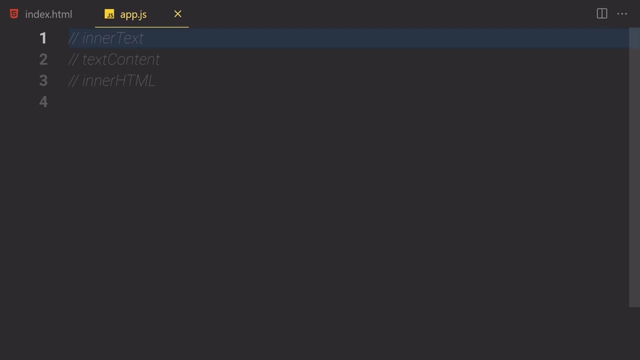 so in this video we are going to be learning about- i mean, like in this section- we are going to be learning about three properties. the first one will be inner text, the second one will be inner- uh, i mean like text- content, and the third one will be inner html. so this is what we are going to be. 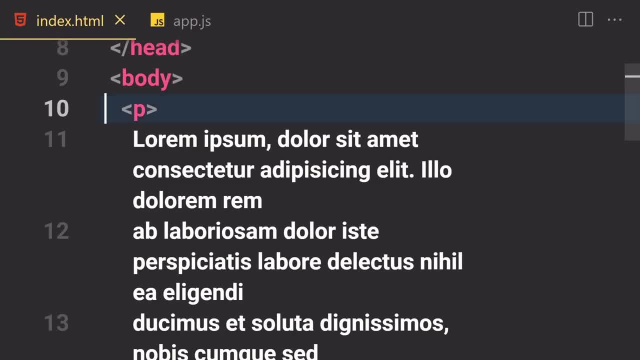 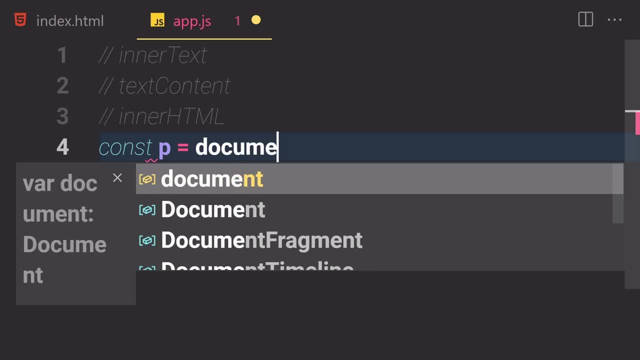 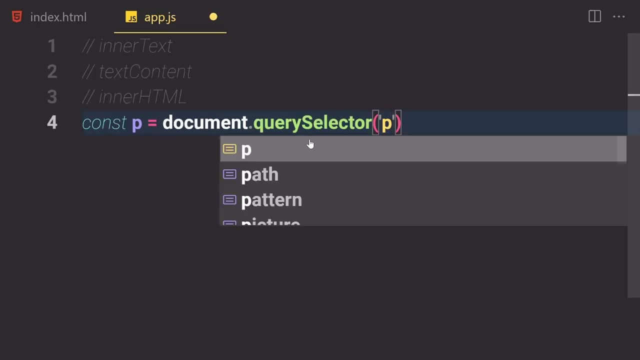 learning. so, first of all, we are going to be selecting our paragraphs, so you already know how to select that. we already learned a lot about selectors, so we are going to be writing p document dot. what query selector, and you can choose whichever kind of selection you like, but i just choose query selector. so now let's just start from the first one, which is that inner. 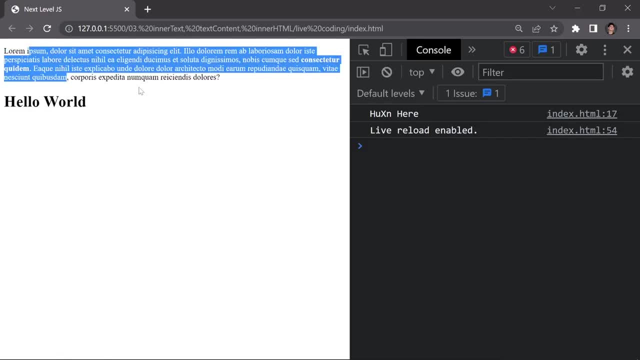 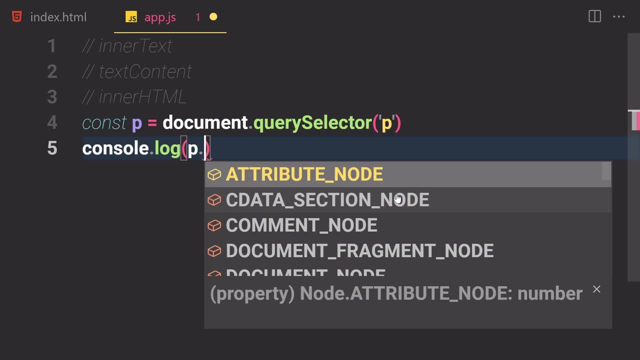 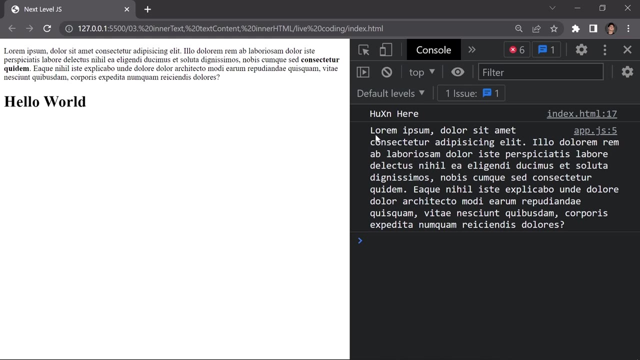 text. so if you want to get the inner text from some sort of element so we can just use the inner text property for that, let me just write a console dot log of paragraph and then dot inner text right here. so if you sell that and now here you can see it on log users, that inner text right here, poorly. 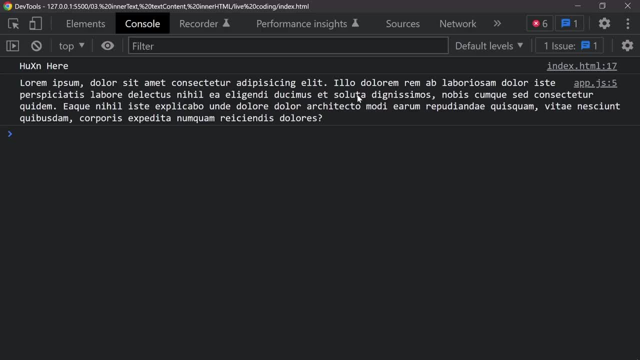 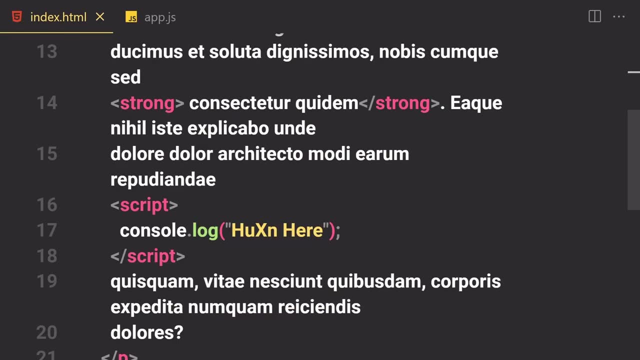 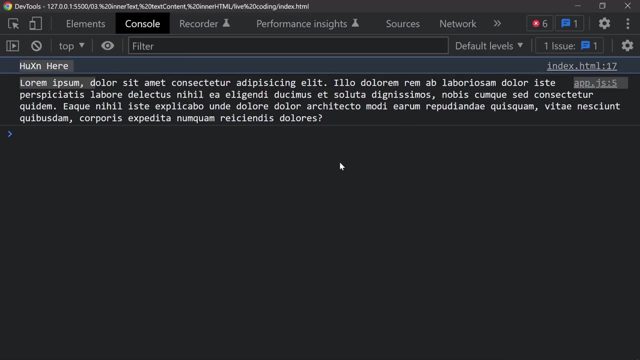 poorly formatted. you know. i'm going to open that in separate windows so you guys can see everything that is in here. that's because of this uh script tag right here. so we have like consolelog right here inside this consolelog. we just have hosan here right here and you cannot see that script. 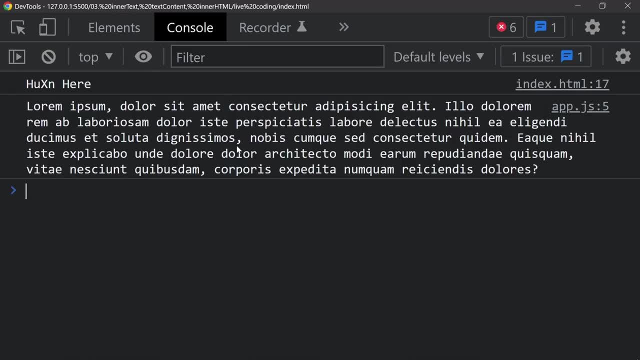 tags right here. it will gives us all of that html content right here, but we cannot see that uh script tag and we cannot see that hosan here. right here, if we just hit ctrl f and we can also search for a script and it will not give us any script tag right here because we don't have any. 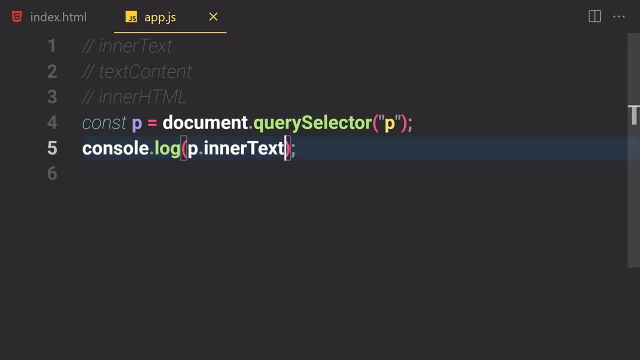 this inner text property will give us all of the text, but it will be totally formatted and it will not give us any uh content like any html and any javascript kind of a content. it will just give us a pure text right here, just a simple, pure text. all right, so that was the first one. now let me just 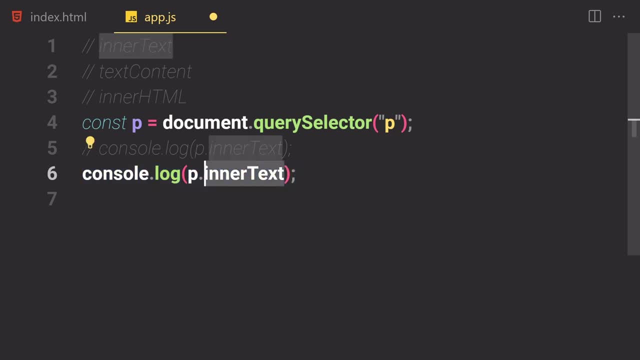 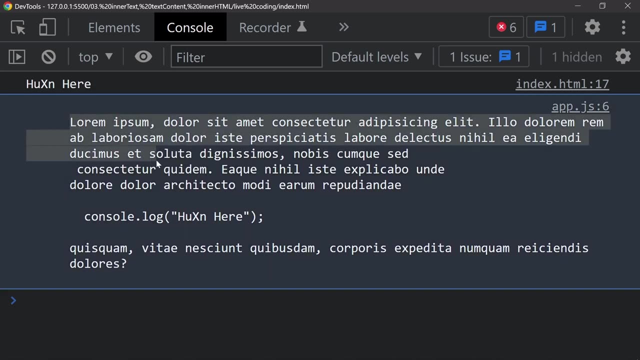 duplicate that and i'm going to comment this line out. and now let's just change that to something called a text content. so if you save that, and now here you can see, we are now getting this text right here, but it's totally unformatted. and we are also getting this consolelog right here, but we cannot see that script tag. that's. 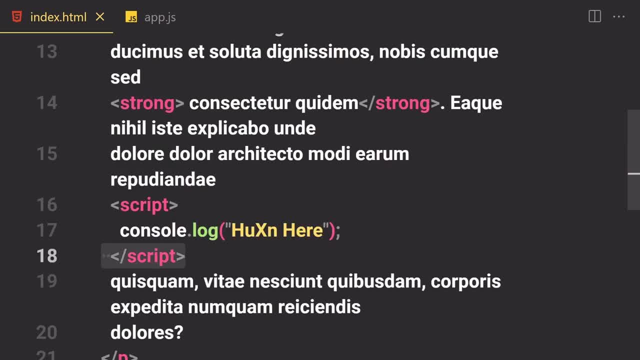 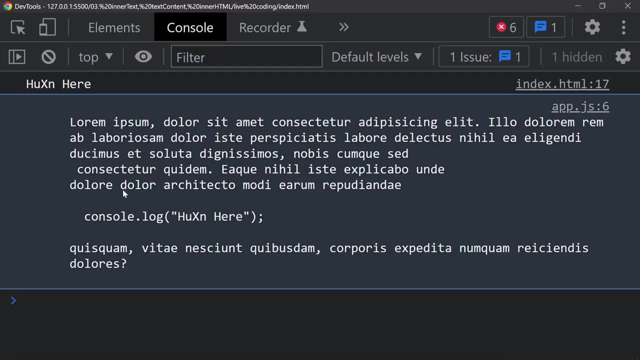 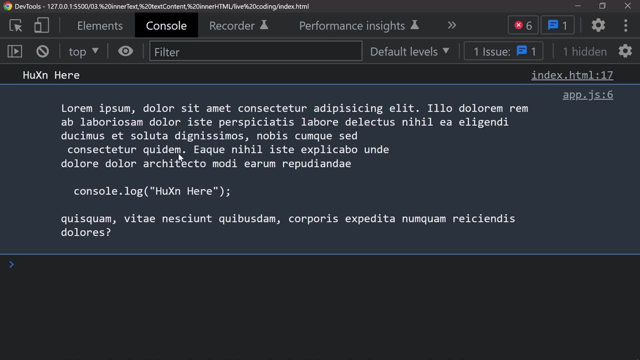 because the script opening tag and script closing tag is html elements and also these strong tags are also html elements. so we cannot see either a strong tag and we cannot also see that uh, script opening tag and script closing tag right here. so this text content property will just gives us the 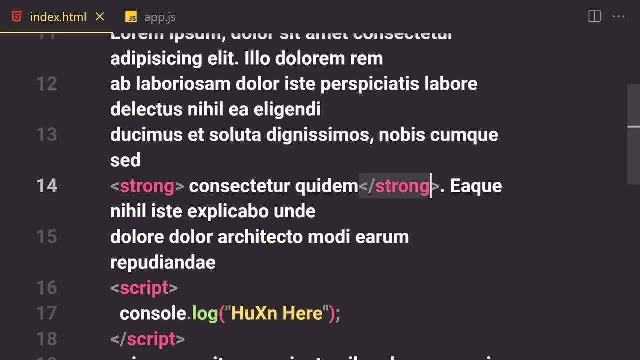 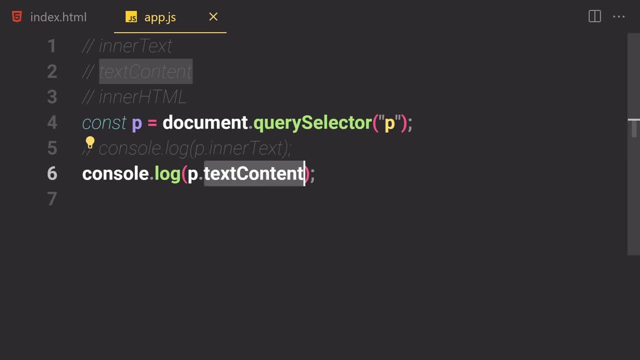 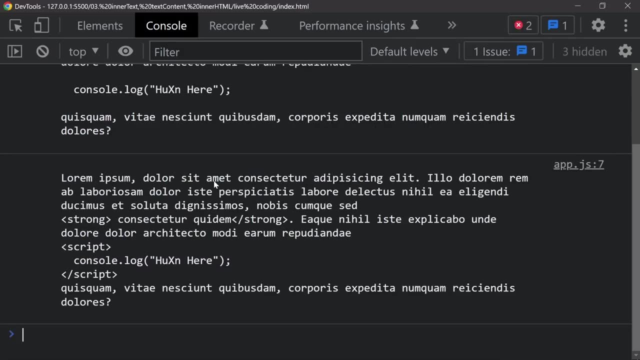 content which is inside our html document, so it will not give us the html elements and stuff like this. gives us a pure text. it will give us a pure content and this final property will give us everything. so we have an inner html field cell there and now, here you can see, it will also include this strong tag right here, like strong opening tag. 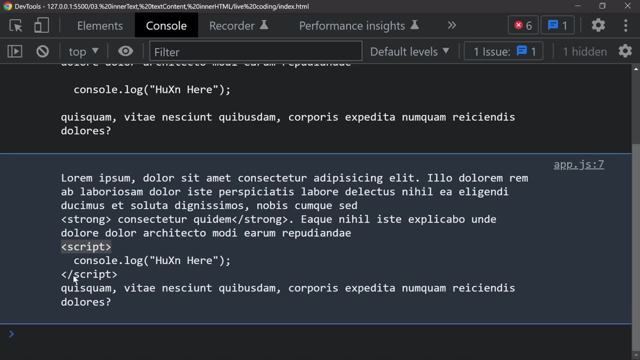 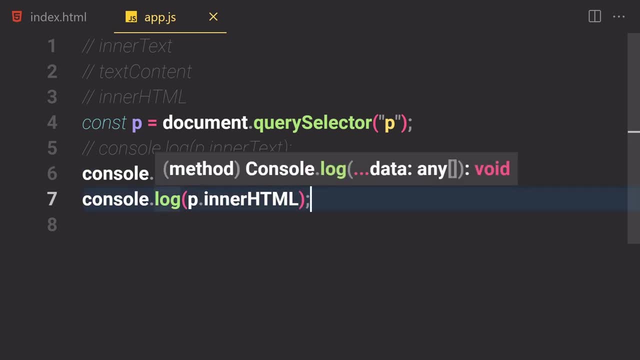 and str and strong closing tag, and it will also include the script opening tag, script closing tag and also this content inside the script tag and it will now give us everything. okay, so we can also change that, if you want to. you know what i'm going to come with both. 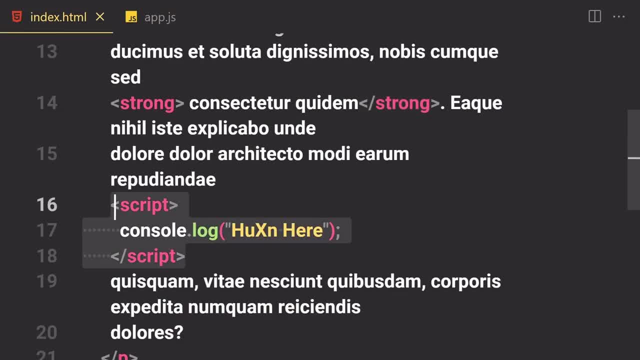 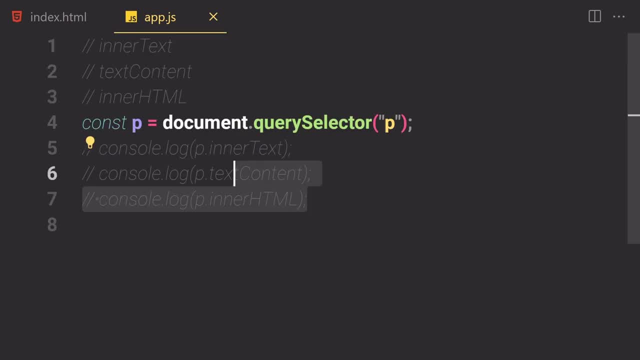 quays, we'll only use this html content content folder. first and finally, you can just remove the html content in the project folder or you can do that by without selecting or selecting the content group to an face template or anything else. so the face or theq element, for example, if you Ani text. 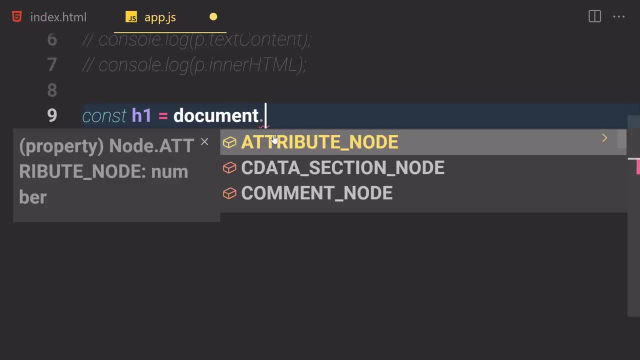 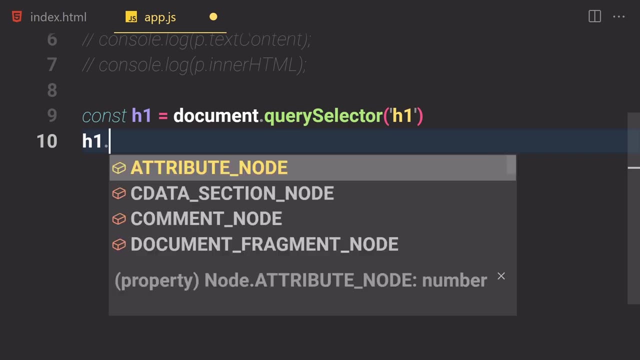 there, we are gonna set the text and we're gonna put it in the present here, so we're just going to just let that be. if we'd want to hit export, or if our system- we are actually using any apps that are working with it right nowле, just remove our clearéconsol andu net comes out and we just have. 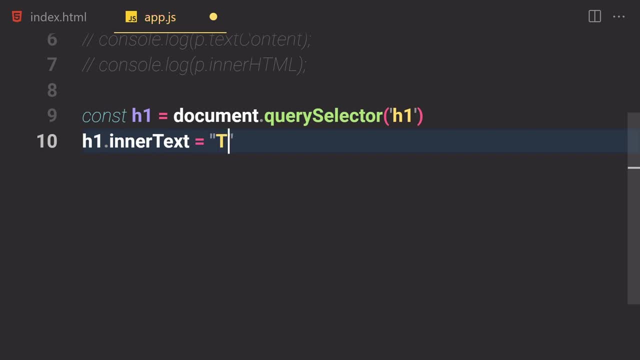 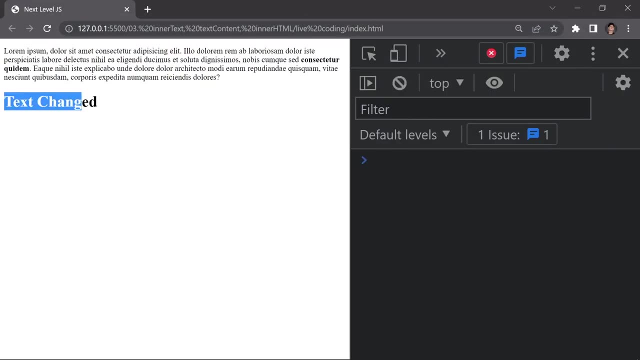 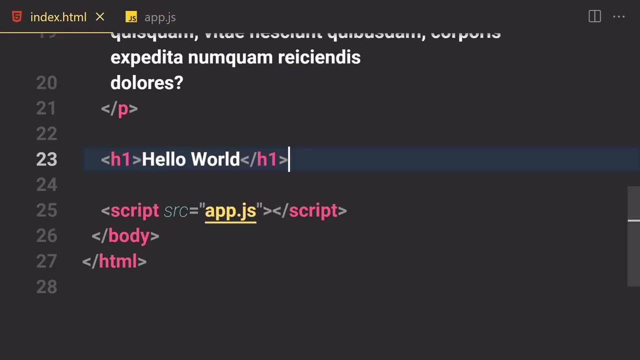 i'll just write t-e-x-t and it will be now set to text changed. okay, so if you save that, i'm gonna stick that to the right and here you can see we are now getting text change. if i comment this line out, and by default we are getting hello world, that's because of this h1 of hello world, and if 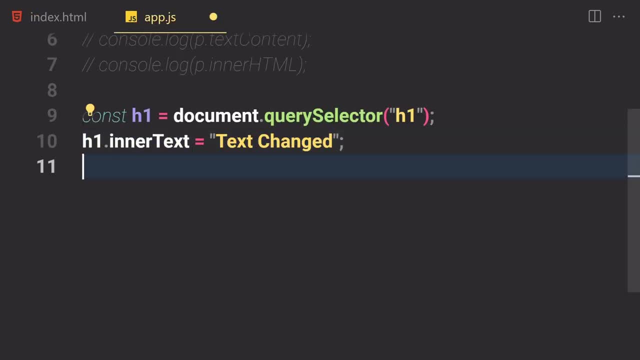 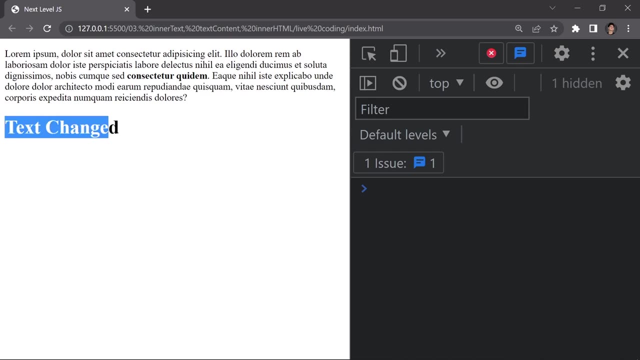 you want to change that. so you can just write dot inner h. so we can just put dot inner text property and we can change this text to anything we want. and if you save a file, it will now change this text to text changed. okay, so we can also change the html if you want to. so i'm going to just write. 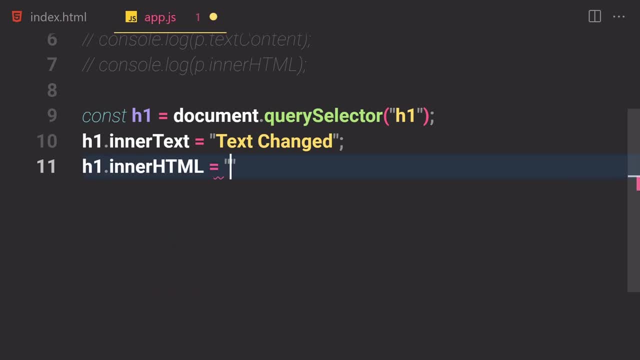 h1 dot, inner html, and it will be now equals to like, i don't know, emphasis would be fine, so i'm going to just use m. i'm going to just write one, two, three in it, okay, so let's just close that real quick like m opening tag and m closing tag and then this, as the name suggests, that it will. 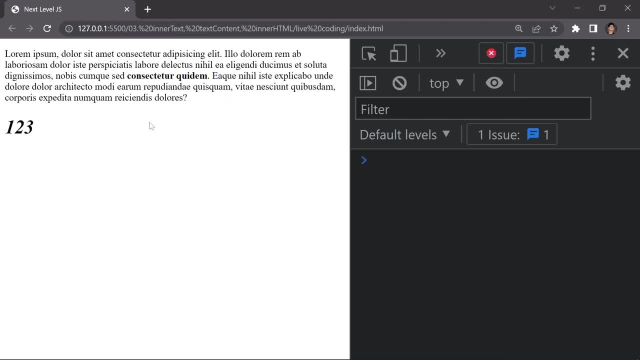 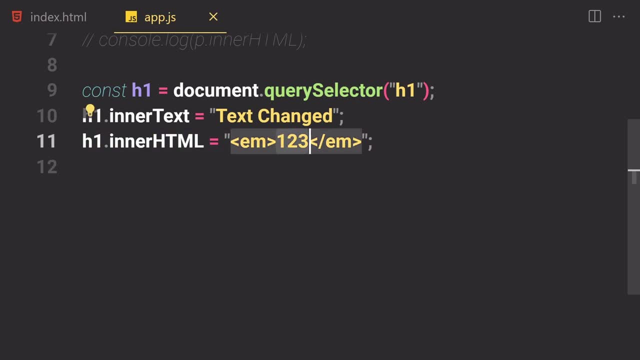 also provide the inner html. so if you save that and here you can see, it will first of all give us one, two, three and it will also italicize that right here. okay, so if you just pour like my own name, like huzzain web dev, and if you say over there, 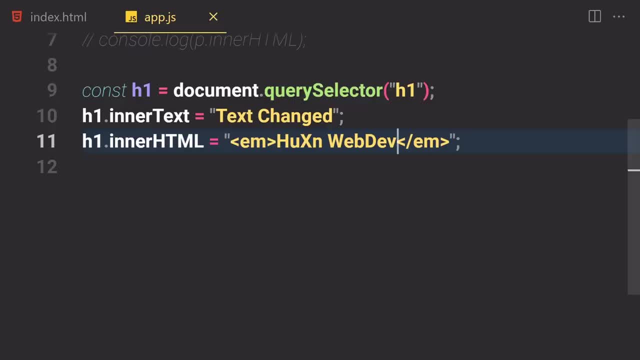 and it will just make it italic and also, uh, what do we call it? um, it will also change the text to be like huzzain web dev. okay, so we can also provide- uh, i don't know- a dell tag. so if you just provide a dell tag, del, and if you say that it will just line through, we can use our html. 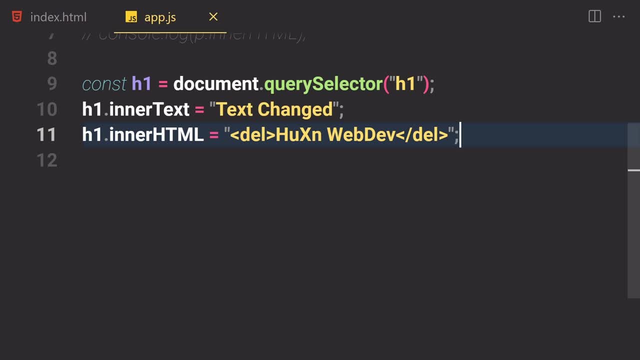 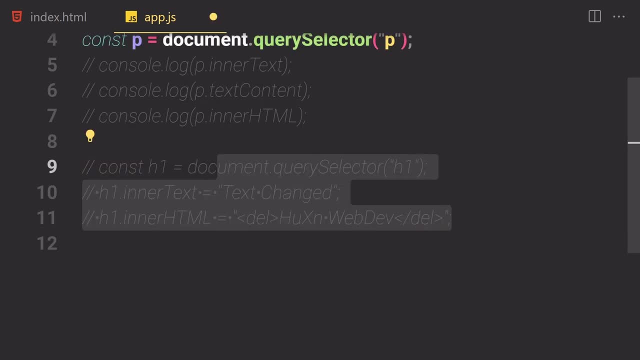 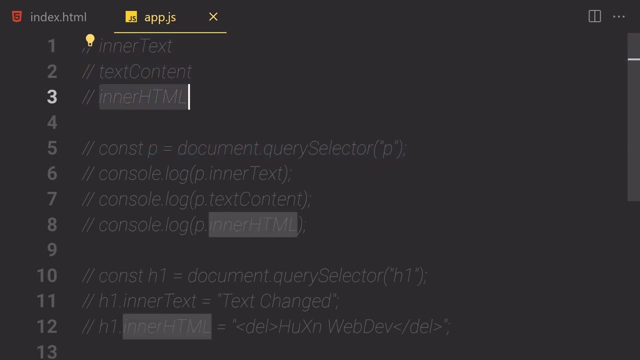 by using this inner html property. so these stuff can be very useful and very dangerous in some scenarios. but you don't have to worry about all of them for now. you're going to learn all of them once we jump into some sort of a project. so we are totally done with our inner text property, text content property and inner. 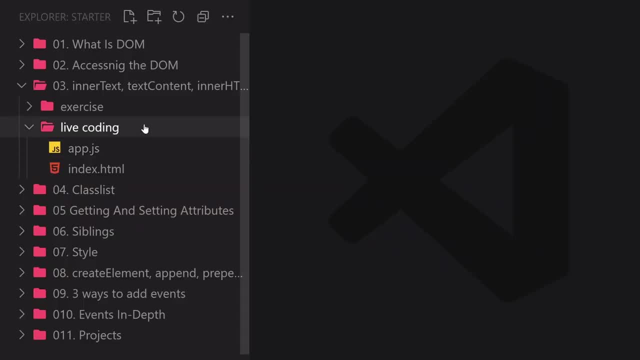 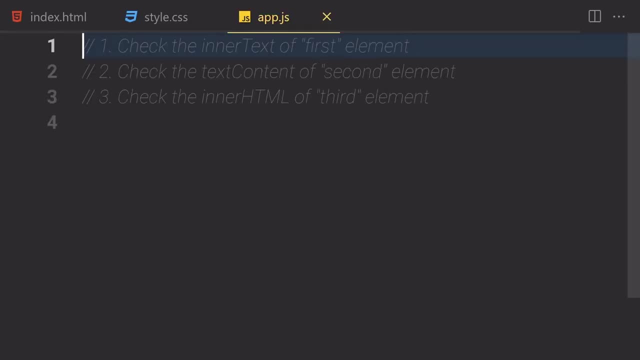 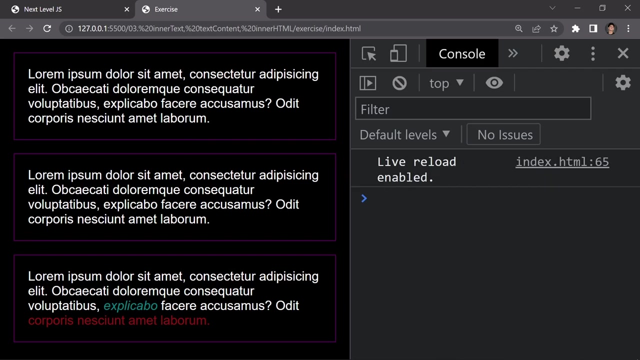 html property as well. so i'm going to just remove that. and now let's just get into our exercise. so i'm going to open this indexhtml file, stylecss file, appjs file, okay, so right click on it and open it for the live server, so we can see everything in a live server, like so. 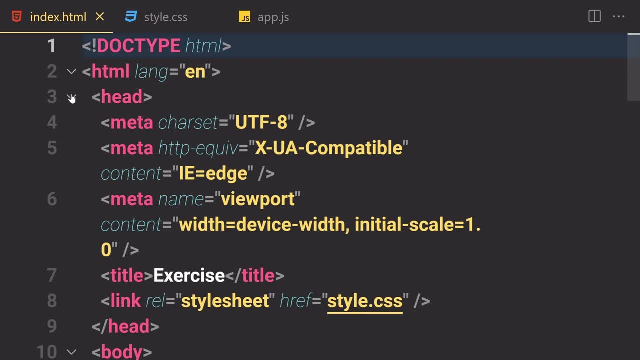 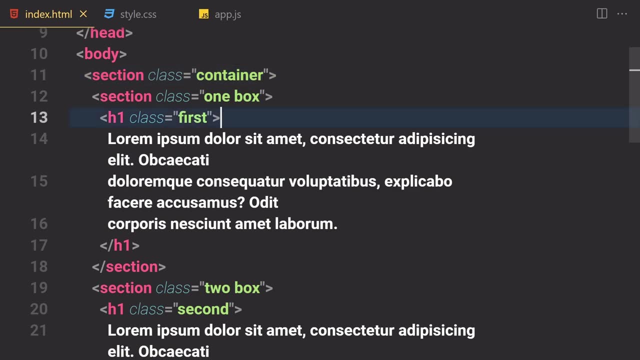 all right, so we have a few content. i'm going to collapse this head area from here, so let's just zoom out a bit. first of all, we have a section with a class of container. we have a section with box one and box two. inside of this box we have our h1 with a class of first. 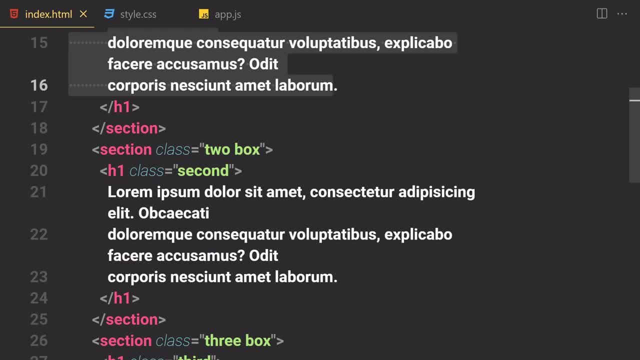 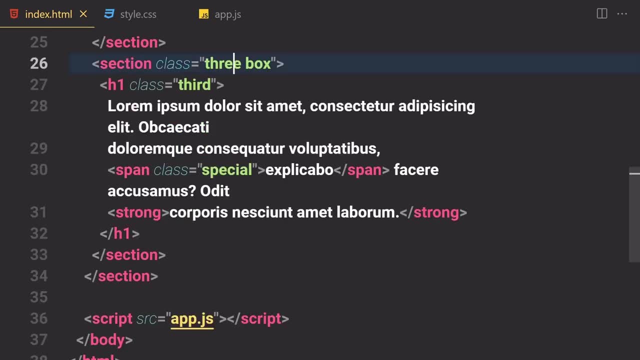 and we have a few lorem ipsum right here. okay, then we have a section two with a class of two and box. then we have h1, one of second, and we have a little bit of text in there. then we have box three and then we have h1. 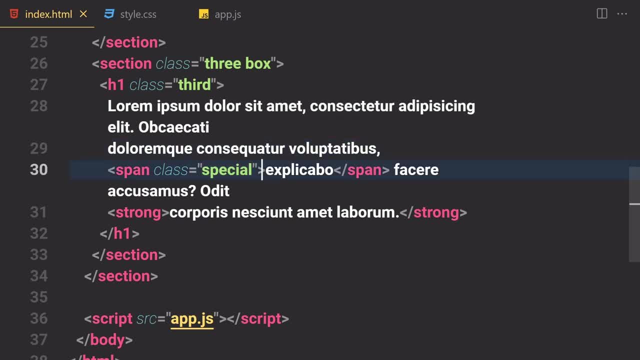 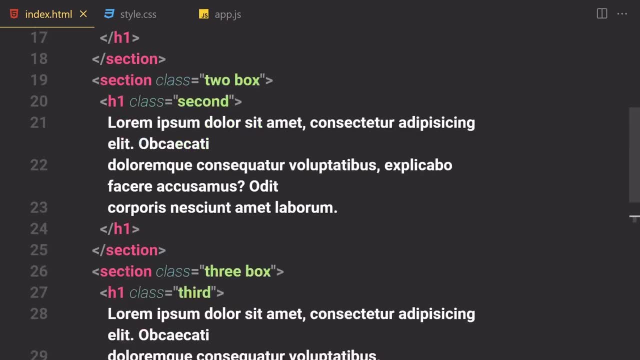 of third, and we also have a span of special right here and we just wrap this text inside that span and finally, we just have our strong tag right here, like strong opening tag and strong closing tag, and this is the result of all of that right here. okay, so in css we don't have crazy css, but first, 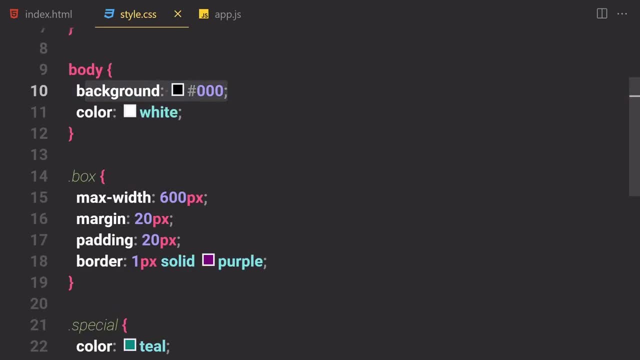 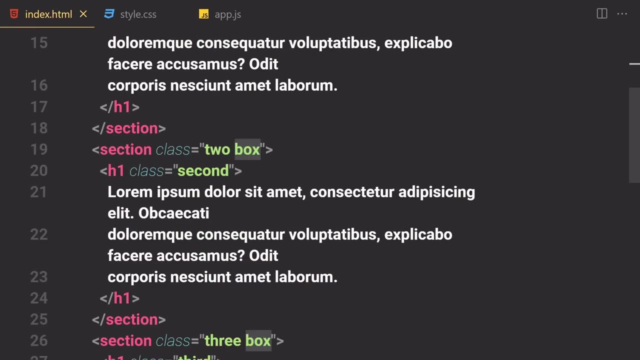 of all, we have our resets. then we just change the background color of the body to totally black. the text color will be white. we select our boxes, so all of these boxes, so we have box in here, this one is a box, this one is a box, and so on and so forth. we provide a max width of 600. 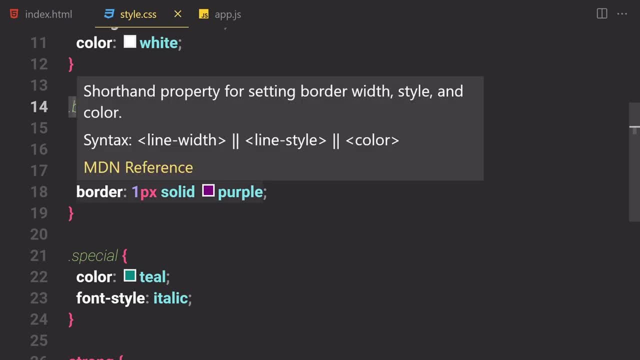 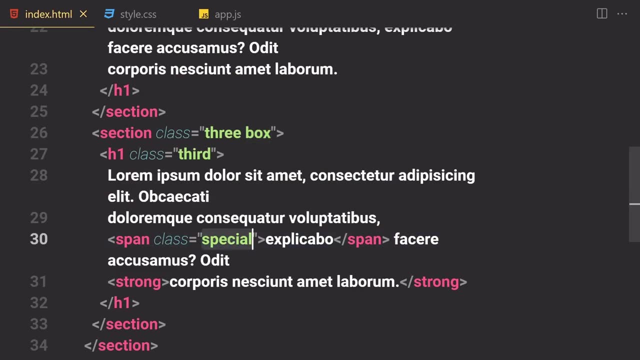 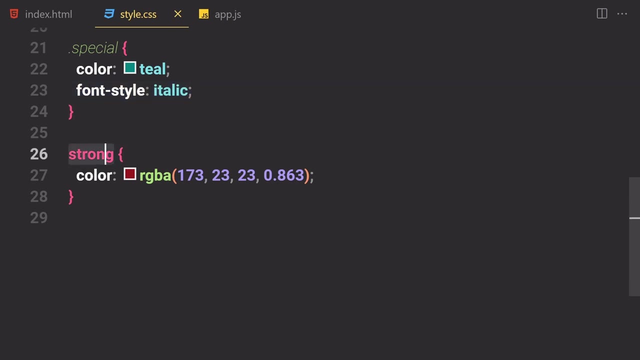 pixel margin will be 20 pixel, padding will be 20 pixel, border will be border will be one pixel all around. then we have a special class, which is this special class right here, like these spans, and we just provide a color of tl and font size, i mean like font style of italic. and then, finally, we 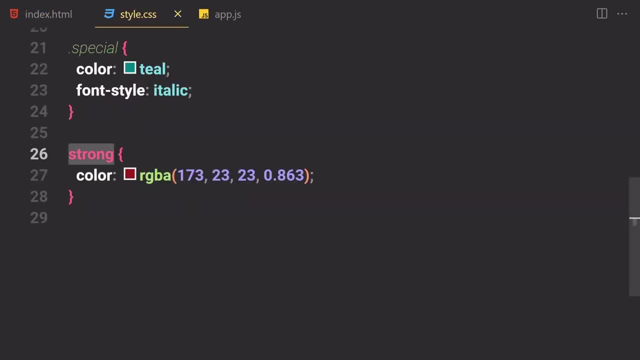 select word strong, which is that strong right here, and we just give them a little bit of color, of kind of a orangish or brownish or card, whatever you want, kind of a brownish color right here. so this is it about our html and this is it about our css. so what do we have to do in our javascript? check the inner. 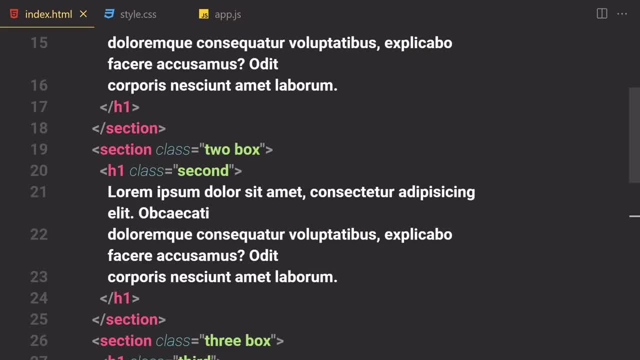 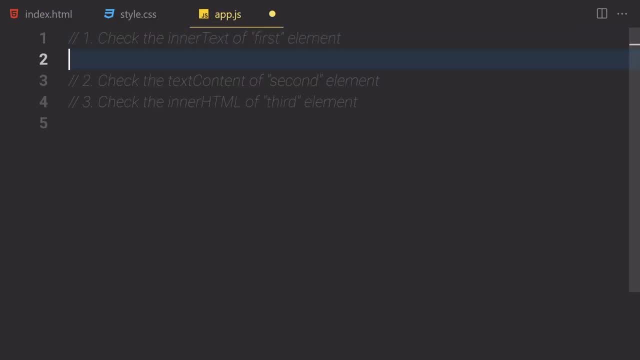 text of the first element. so what is the first element? let's just see. if you just hit, okay, so we have this first element right here. so if you want to check the text of that first element, so for that we just have to create our variable cons, first element, and then we have our text. 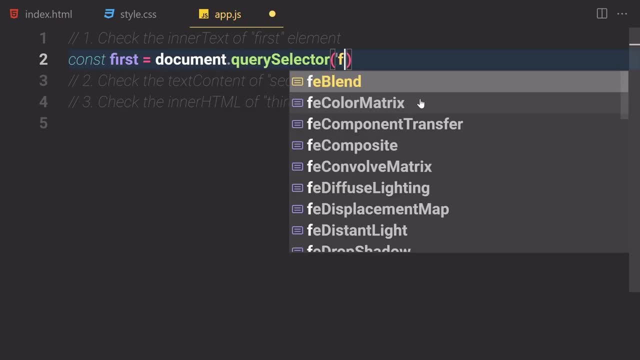 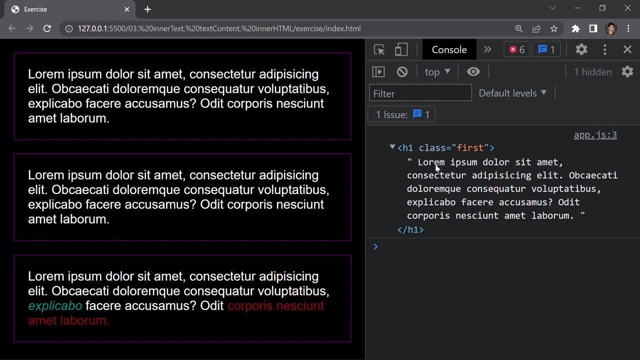 first, and it will now equal to documentquery, selector of period and first. okay, so now we get that. let's just log that to the console, save it, and here you can see we are now getting this h1 and we have a little bit of lorem ipsum inside there. so if you want to get a text of that first 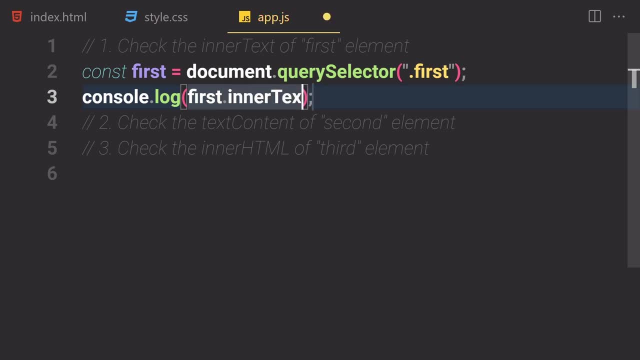 so for that we can just write like dot: inner text, so inner text. and now, if you save that and it will now give us the inner text of all of that h1 right here. okay, so that's it about our first step. so what do we have to do in a second step? so check the text content of the second element. so first of 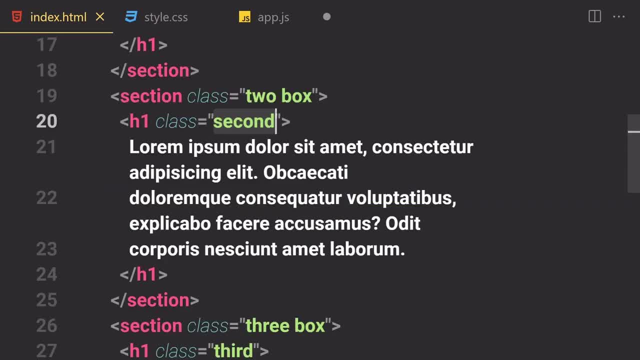 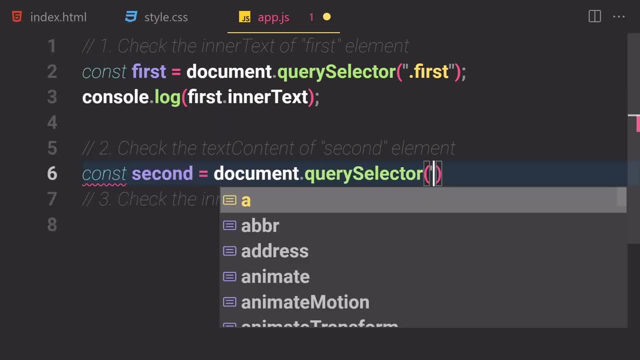 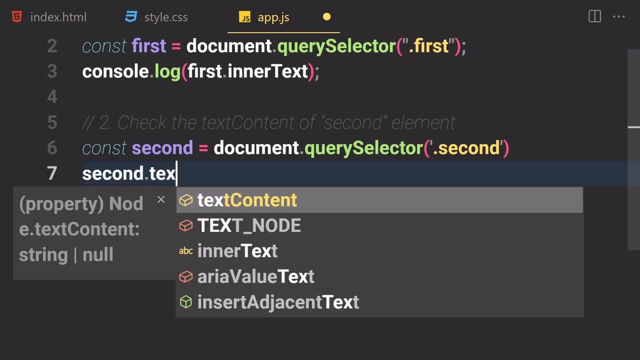 all we have to see. do we have word second? yeah, we do have that second right here. let's just select that. i'm going to just write con second and will. now equals to documentquery: selector of second. okay, so now, if you want to check the text content, so i'm going to just write second: uh, dot text. 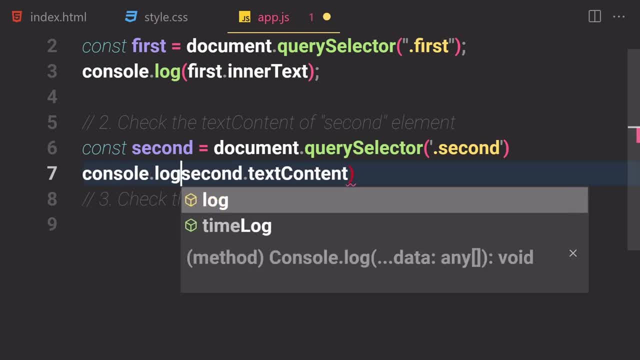 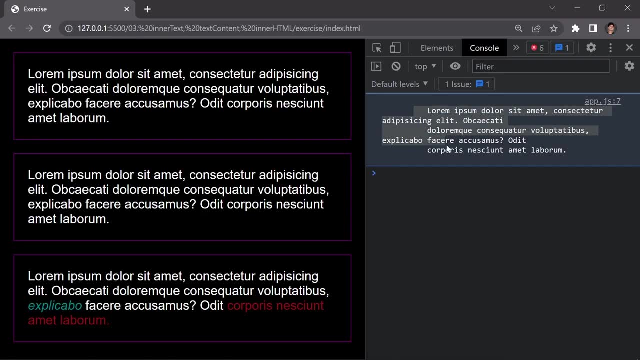 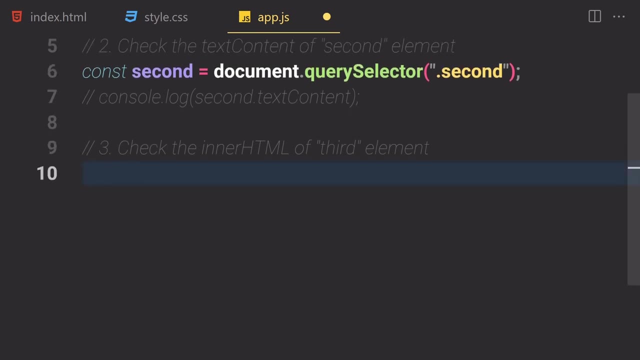 content, but we have to wrap that in or consolelog so we can see it. i'm going to comment this line: save my file. and now, here you can see it will not use the content, but without formatting whatsoever, right here. okay, comment this line out. the third thing which you have to do and the final thing. 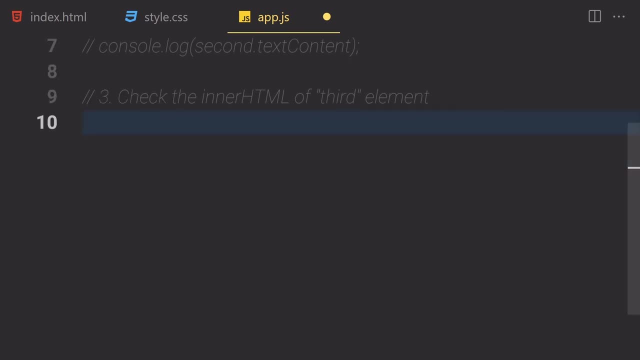 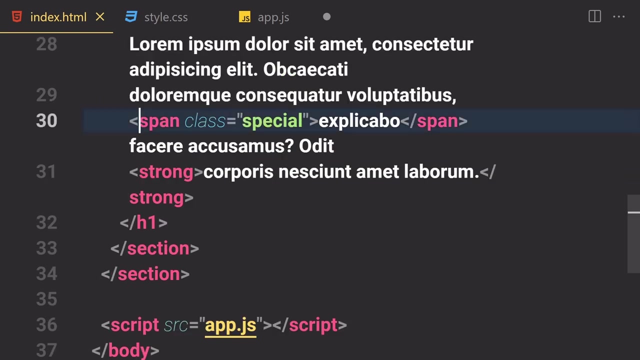 which you have to do for this uh exercise is check the inner html of the third element. so let's just see what do we have inside this third element. so inside this third element, we have our span with the class of- i mean like with, yeah, with the class of special, and then we have 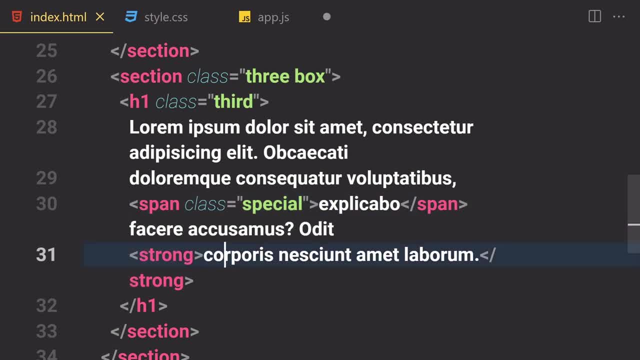 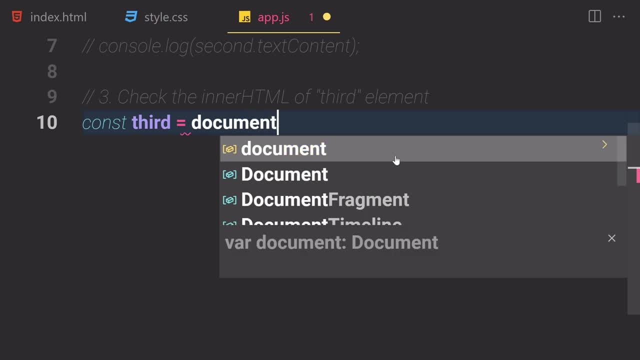 a strong opening tag and strong closing tag, so it will show up all of these spans and all of these gibberish. so let's just select that first of all. cons third, and it will be now equals to documentquery. selector of third. okay, so we just have to write consolelog third. 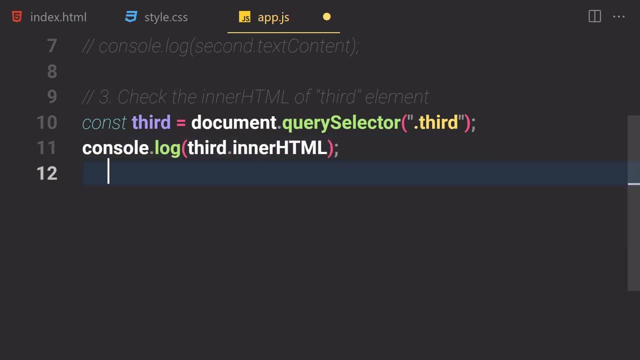 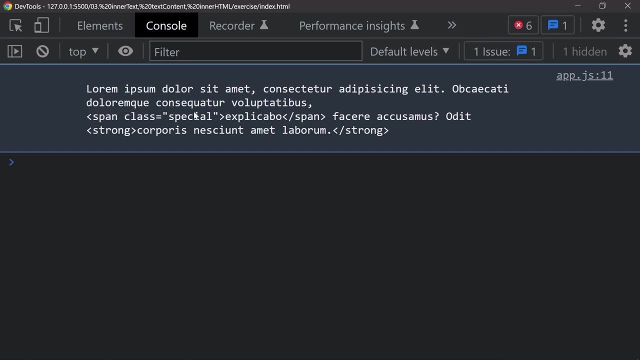 dot, uh, inner html in this case. and now, if you sell that, and now here, let me just um separate that. and now here you can see, we are now getting span with the class of special and the text of: i can't pronounce, and we also have this strong opening tag and strong. 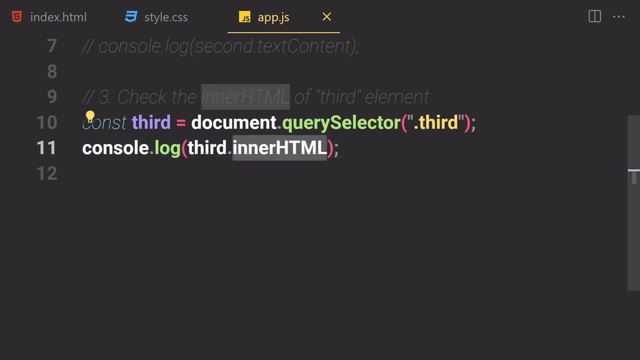 closing tag. if i change that to like, um, i don't know, uh, inner text right here. so if i just change that to inner text, so it will not include all of that, but it will give us it there in a formatted fashion. if you change that to inner, not in our text content, and if you save that, it will give us. 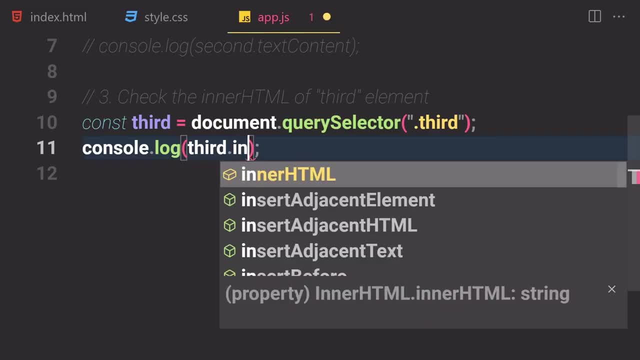 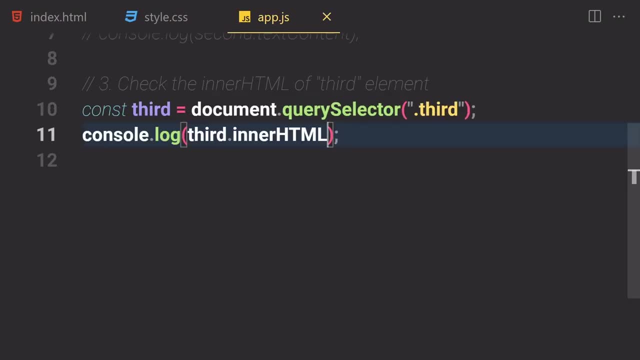 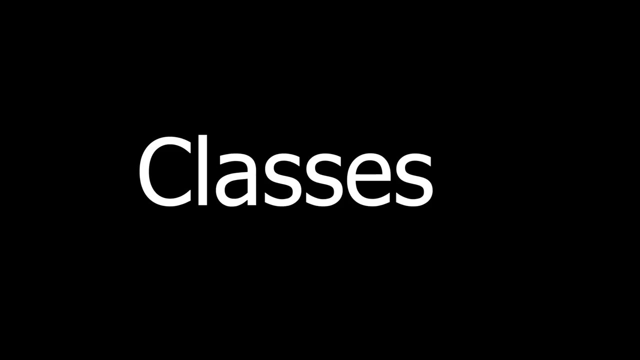 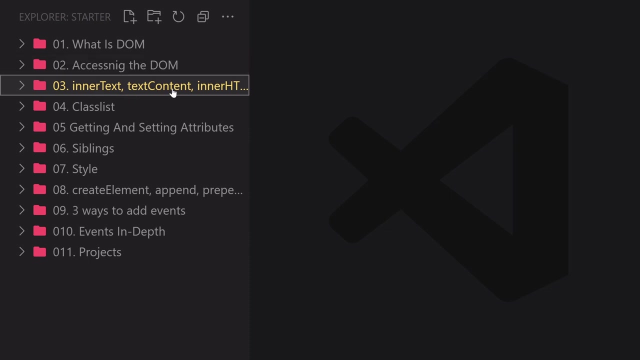 that like so, without any uh code, word search. so if you just write like inner html, save it, it will give us that another uh coding inside that, inside that text. so that was it about inner html text content and inner text right here: property. so now that we learned that what is a dom, how to access elements from a dom and how to see the text. 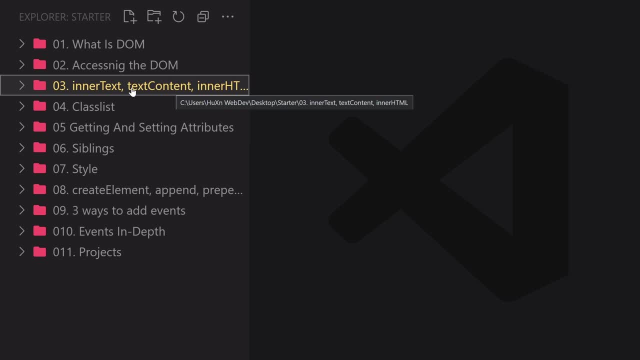 content, inner html and the text inside that element. now the next thing which you have to do is that we have to learn about a classless property and how we can add classes to our elements, and how we can remove clauses from our elements and how we can do toggling of our classes. so we just have uh app лишьigkeit and add classes and how to remove classes from our elements and how does we can do toggling of our classes. so we just have uh add students. So those are all our details, as you can see, if you see on theBigunt hours of view, we can click here within theADA environments page and check the electives to see the changes over theある Morning. 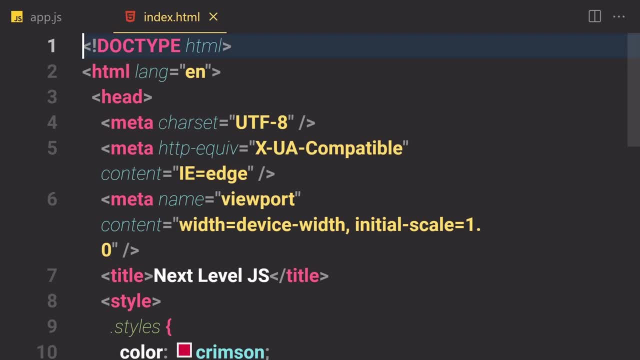 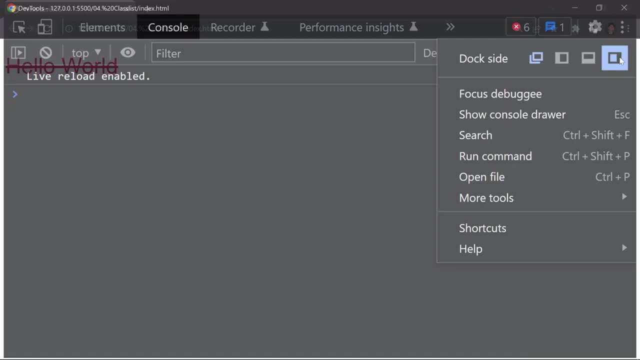 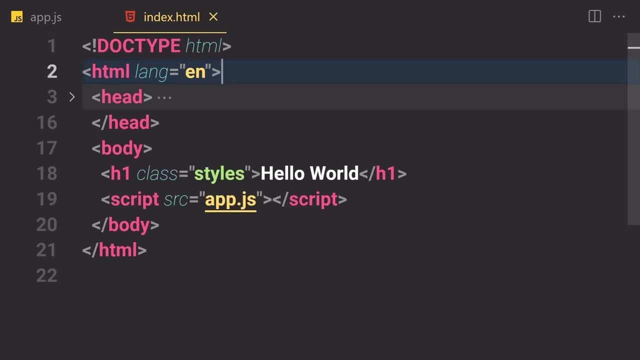 uh, appjs file and we have our indexhtml file. right click on it and open it with the live server. so it will now open this file in a live server. i'm going to open my dev tools set there to the right like. so i'm going to just hide my metadata from there and inside this body area we just have our 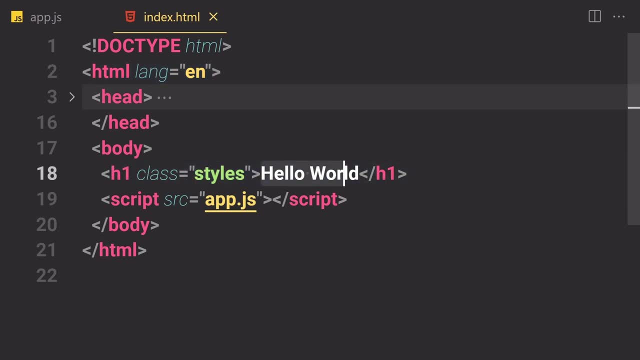 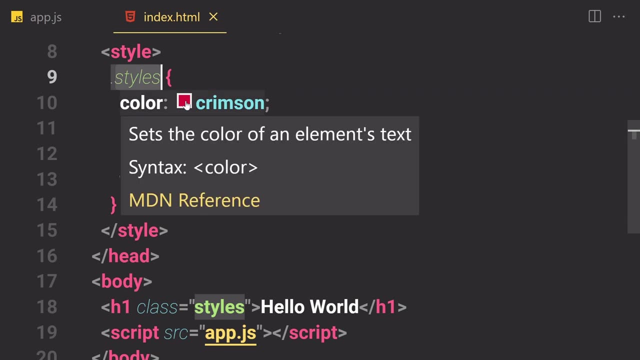 h1 with the class of styles and we just provide our hello world inside there and now, if i expand there and here, you can see inside this styling we have our styles, uh class right here and we just provide a color of crimson for where it will be totally normal font size, not font size, but font. 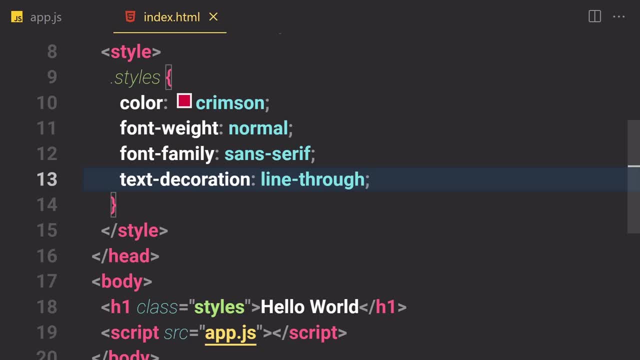 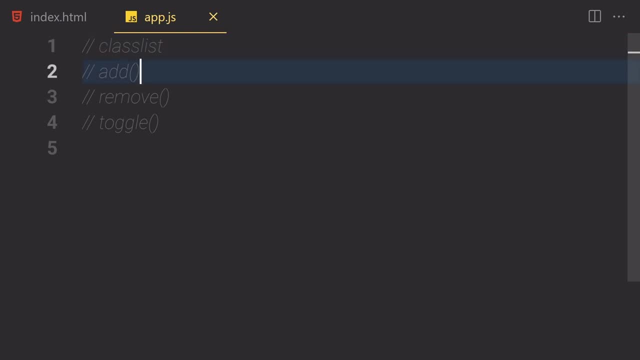 family will be sans serif and text decoration will be lying through, okay, and we are now getting all of these styles right here. okay, so now let's get into or class this property first of all. so now let's just select or h1, and then we can interact with that. so first of all, let's just 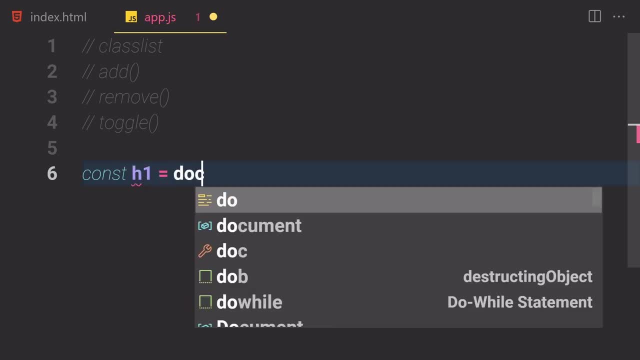 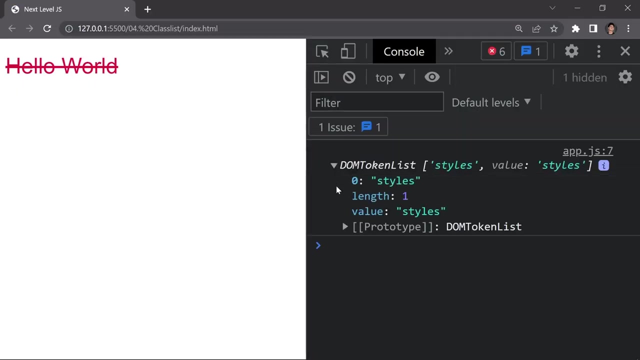 write or cons of h1. you can store it in let, in constants- i mean let and war as well- and now let's just select or h1 right here. so now let's just write like consolelog of h1.class list and now, if you save that, it will now give us the list of all of the classes which we provide to this specific. 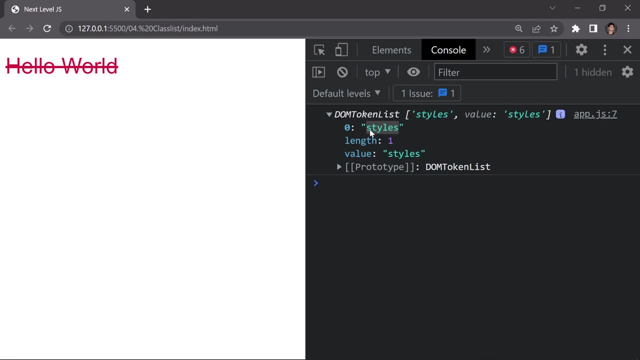 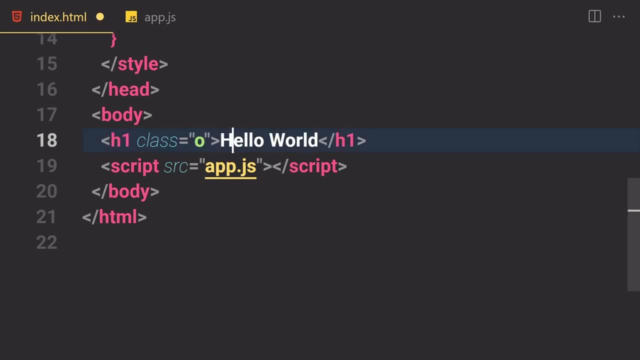 element right here, so we have just one class right here, so that's why we are getting the length of one right here. but if you have multiple classes- like i don't know if i just remove these tiles, if i change that one, two, three, four, five- and if you have a lot of classes, and now if we say over there, 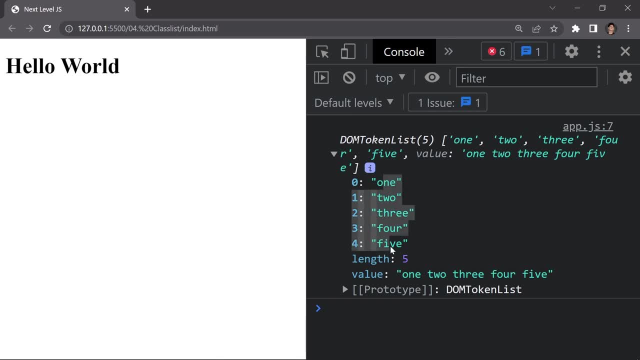 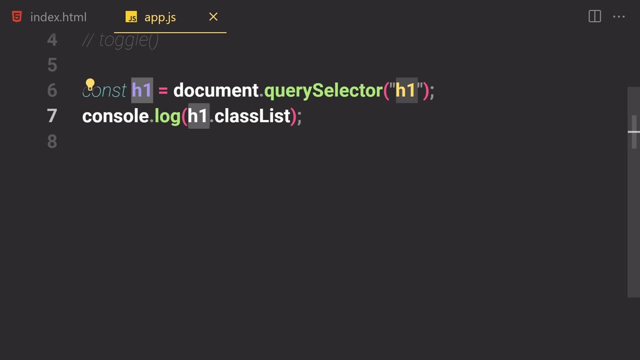 it will not give us all of their classes right here. all of the list of that class is right here, okay, so i'm going to just undo that to styles sale there and this is how it looks like right here. so this class list property will allows us to check all of the classes which this specific element has. 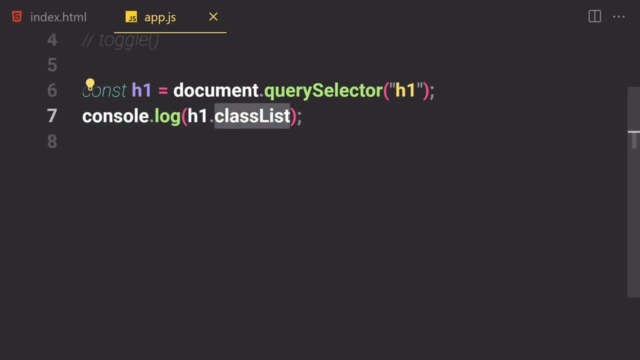 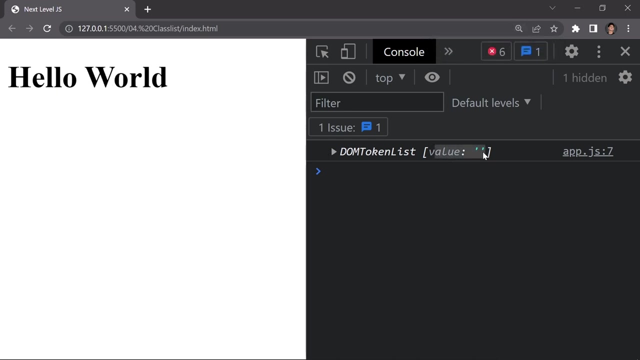 so we just have our selector and then we can just use this class, this property on there. okay, that class, now that it is not going to be a number like this, it is going to be a value along such a line, but it's just one of those nodes and then also says everything, and so we can save this. 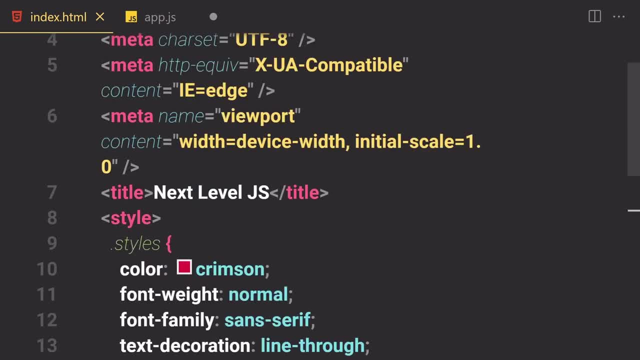 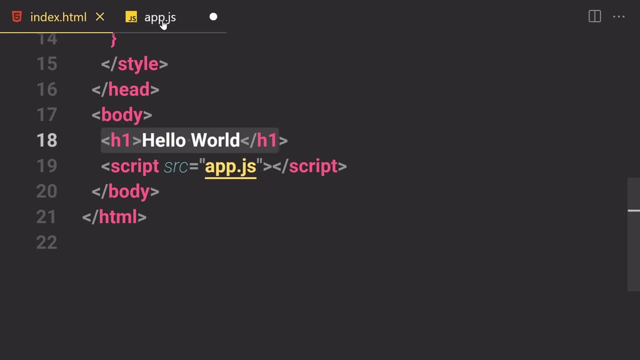 information at any time by just loaded inside of, stumble within our her, with our h1 logic, and we have everything now. so we have good problem. so now we let's just wrap around with this so that management to this h1 by using javascript and interacting with the dom, so for that we can just use that. 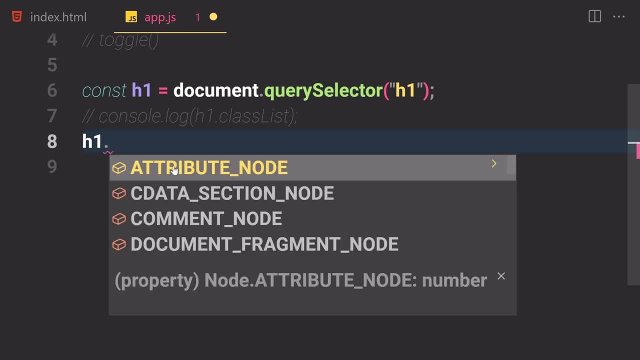 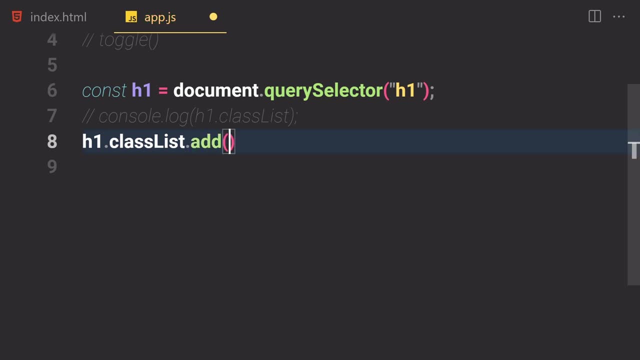 h1. first of all, we will just select our h1, and then we are going to be selecting our class list property, which allows us to give us the list of their property, and then we can use a useful method called add, so, as the name suggests, that it will just add class to our element. now we have to give. 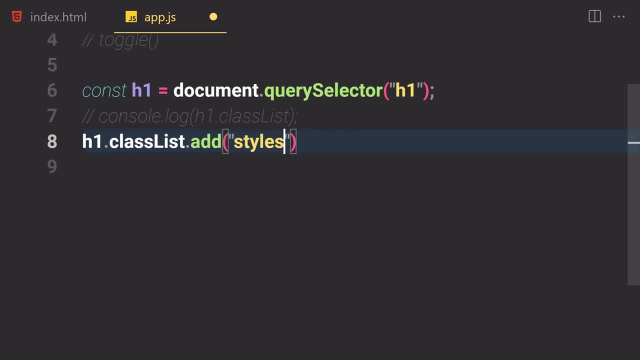 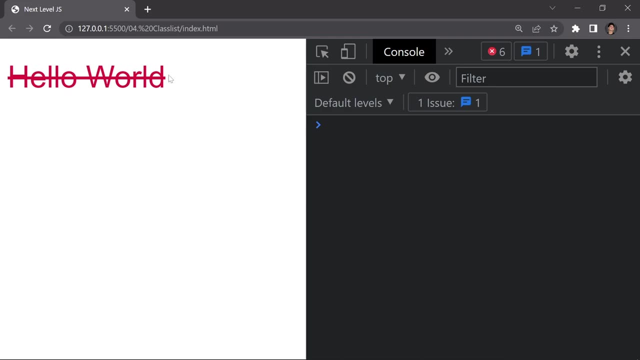 the name of that class inside double quotes. so i'm going to just write styles right here and knife is saved there and here you can see it will now apply that class to it right here. so here you can see we are now getting these styles. we don't have that class right here. on this element. 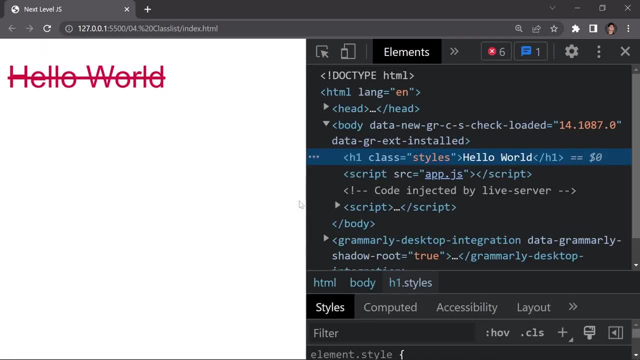 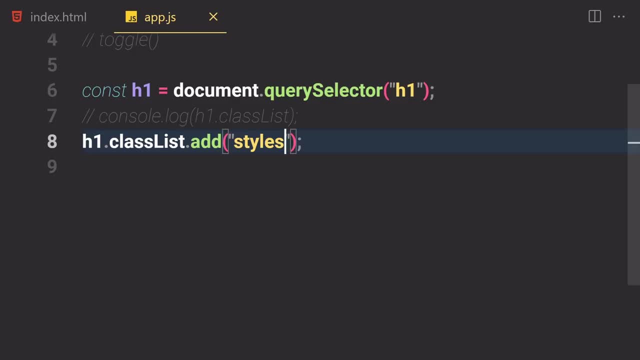 but if you just right click on it, click on inspect, here you can see it did provide that styles class to it right here. okay, let's just go back to the console. and now let's just see i'm going to copy this line out, paste it right here, i'm uncomment it and save it. and now here you can. 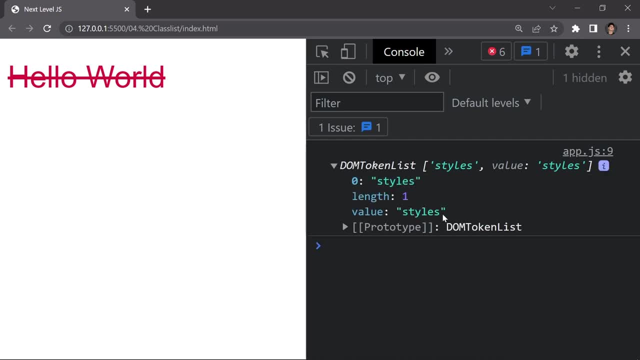 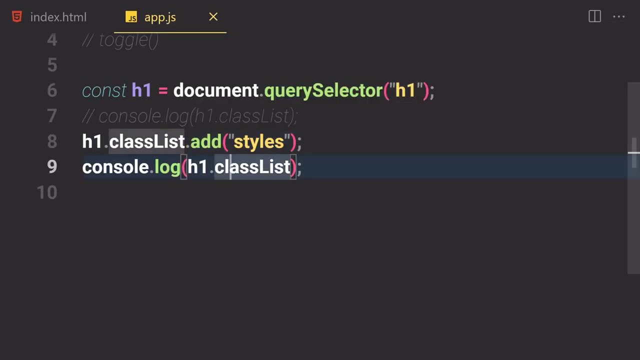 see, we are now getting the styles class right here, and the video value will be also styles and the length is set to one. okay, so this is how we can set classes to our elements. now the next thing which we have to do is that how we can remove classes from our 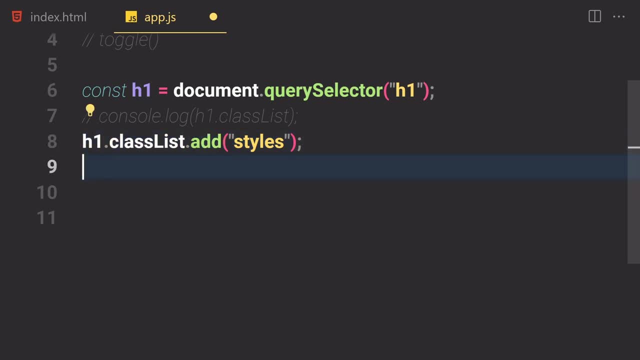 elements. so now, in this case, we attach this class right here. so now, if you want to remove this class from this h1, so what do we have to do? i'm going to duplicate this line of code and now, instead of add, i'm going to just write remove, right here, so remove, and then let me just write remove real. 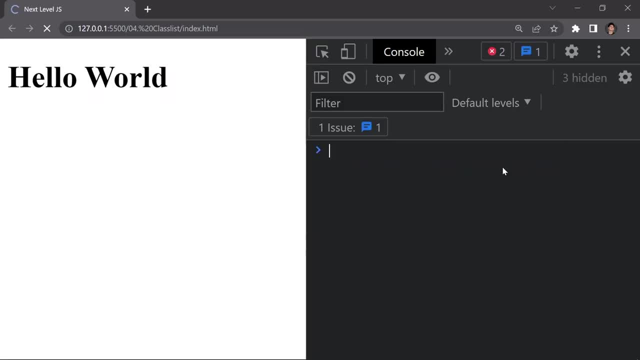 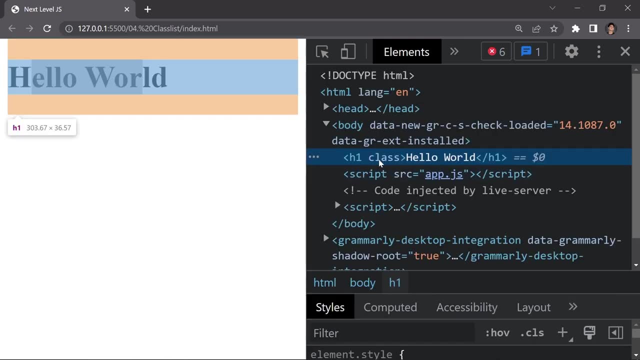 quick, so remove and then the class name. so now if you save that, and here you can see that styling is gone, and if you just right click on it and click on this inspect, so here you can see it also gone from here. so we do have that class keyword right here, but we don't have any value for that. 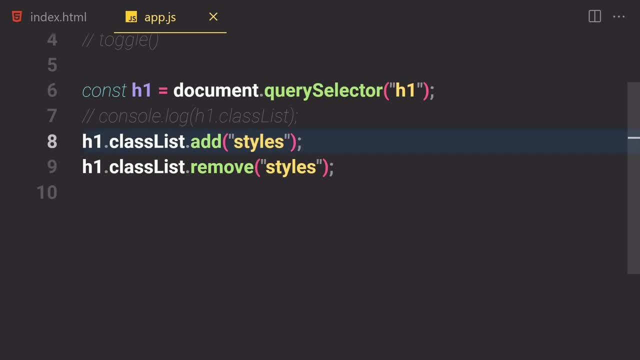 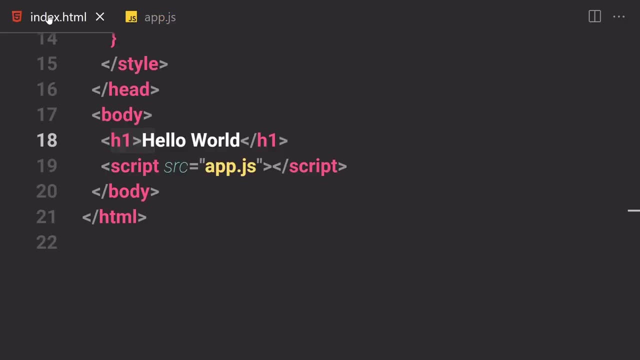 so that's why we are not getting that. let's suppose i'm going to comment this line out and save our file. so you already know that we don't have any classes on our h1 right here. but if i just add, you know i'm going to also comment this line out as well. save our file. 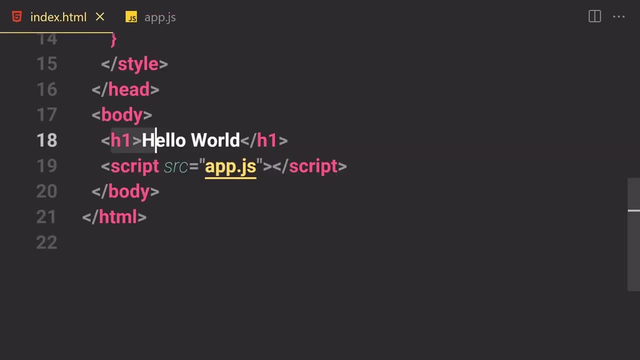 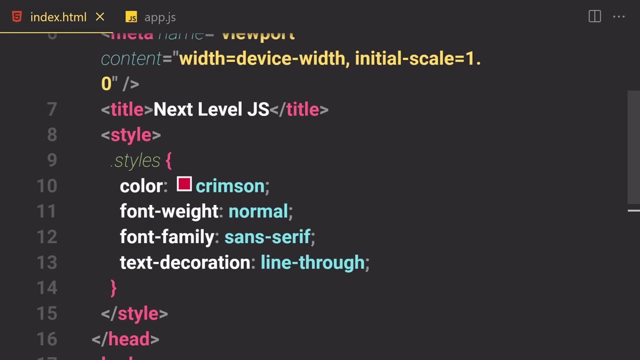 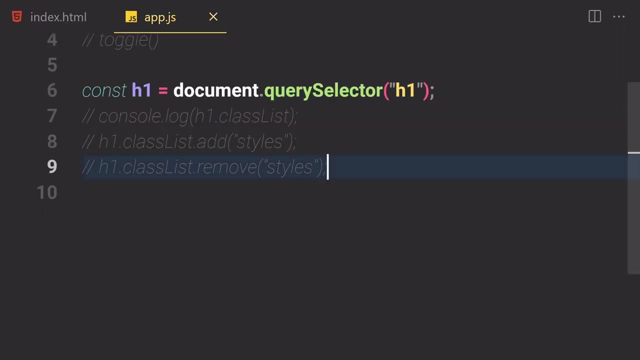 so we don't have any classes whatsoever on or h1, so let's just write: or a class right here of styles right here. so if you save that, okay, so i messed it up something, copy it, copy, paste it and now we are getting the styles all right. so now, if you want to remove that style from this h1. 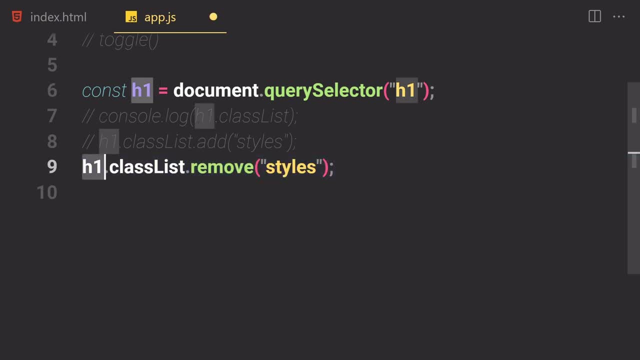 so we just have to uncomment this line of code. so we have first of all the selector, like the tag name, then we have a class list and now we are removing this specific class from this h1 element. so now, if you save that and now just remove that class from it, if you just provide apple in this, 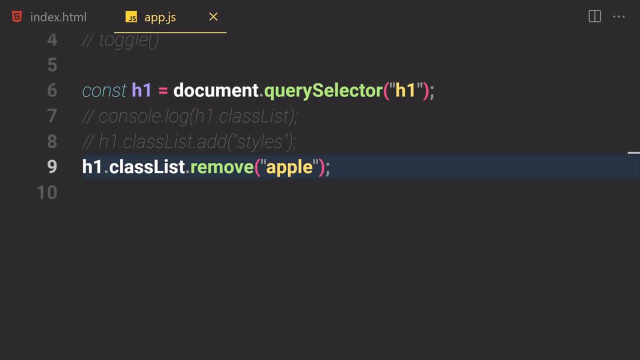 here. so if you save that, it will not remove that apple, because we don't have any apple class on this h1. we don't have any apple class in this class list, so that's why we cannot remove that. so let's just provide styles back and we'll now just remove that. and now, finally, let's just learn. 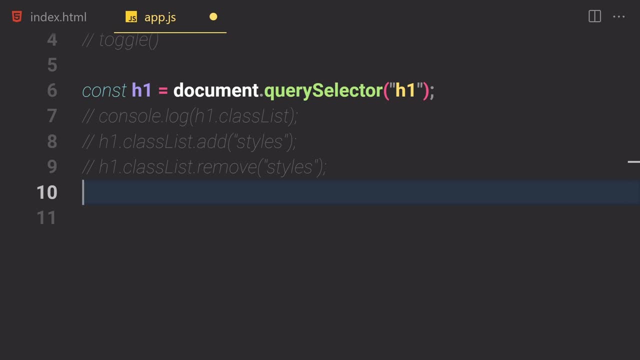 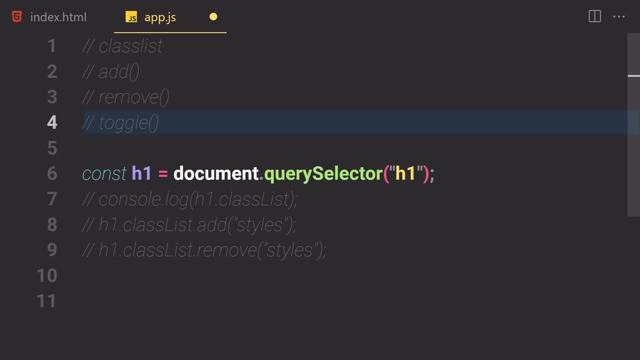 about my favorite property- or method to be precise, which is known as a toggle, so as the name suggests that it will just toggle the classes. if we have class, so it will just remove it. if you don't have a class, it will just add that specific cluster. so i'm going to just show you that just in a second. 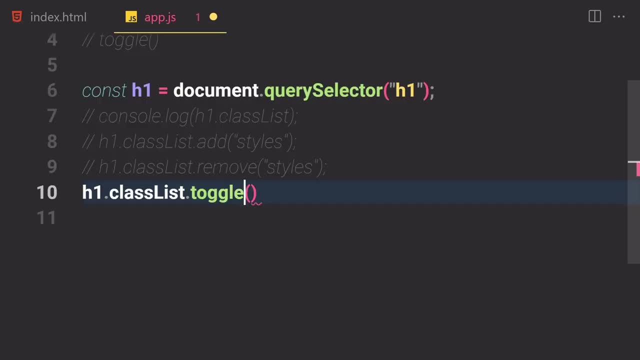 i'm going to write h1, then class list and then toggle. okay, so inside this toggle i'm going to give him a class of- like i don't know- apple and we don't have any apple classes anywhere. so if you save that and let's just see, okay, so let's. 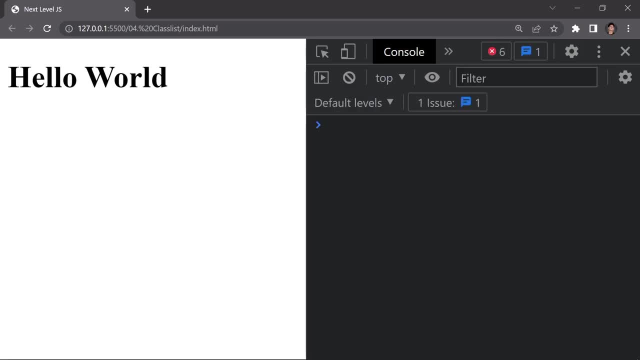 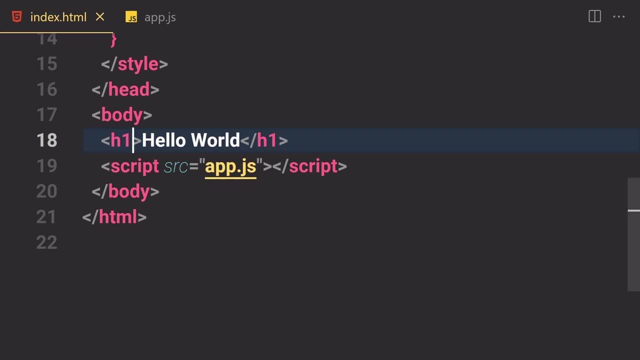 just remove that class from here and we don't have any apple class anywhere. i'm going to right click on it and go to inspect area and now, here you can see, it did provide that apple class right here. that's because we are using this toggle class right here. what if i just provide a styles to it? 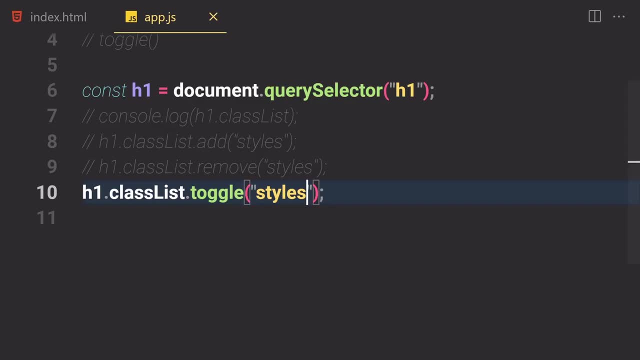 so if i just write styles, so now just add that style class right here, i removed it from, i removed that class from here, but we do provide it right here. and what if i just provide it right here? let's just write class of style and save that. it will just remove it. so it will just go the other way around. so if we have class, 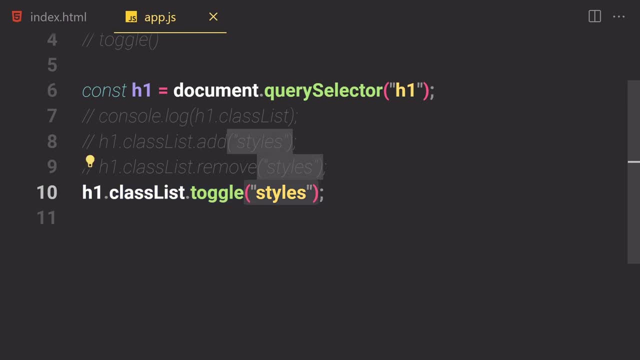 it will remove it if you don't have that specific class, so it will add it. this is how the toggling works. so how can i put that in other words? let's suppose if you have a class of um, you know what, you know what. that's why you just have to play around with that by yourself. so let me just say: 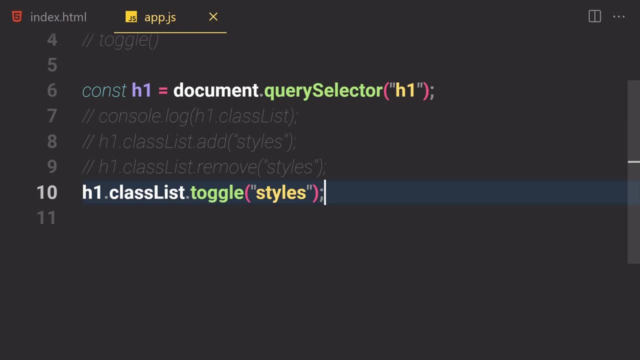 that one more time so you guys can just understand it a bit better. if we have the style class on this one, so it will remove it. it will just remove it. but if you don't have access to that style class on this h1, so it will just add it right here. so this is what a toggle do for us. so i'm going to 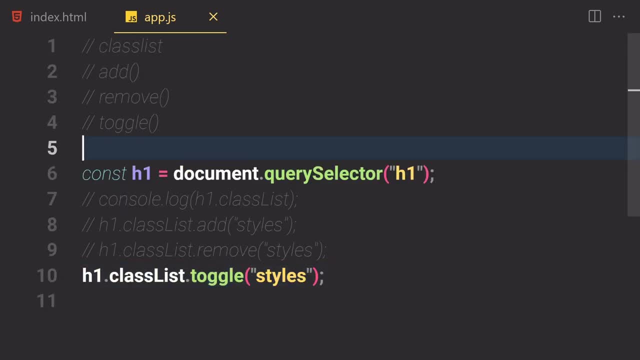 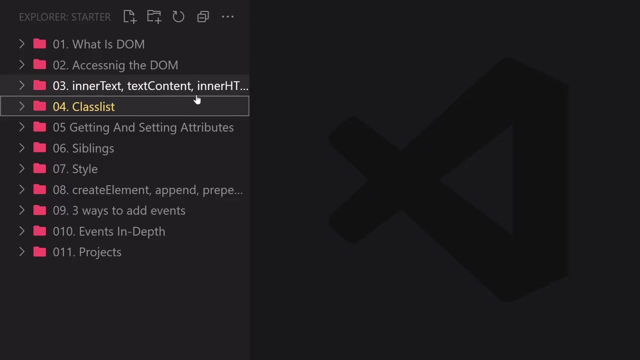 just comment this. oh, you know we're not going to be commenting anything, so we are totally done with this section as well. now what else do we have to do? the next topic which you are going to be learning about is something called getting and setting attributes. so this is what we are going. 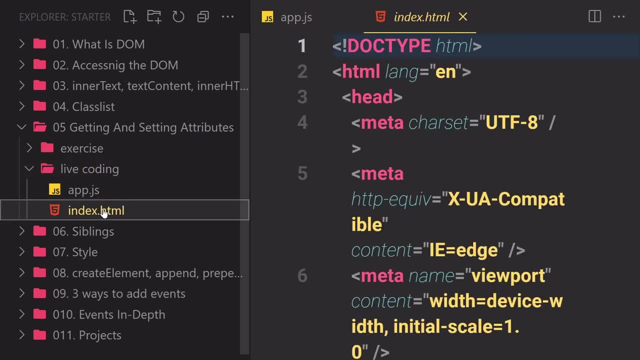 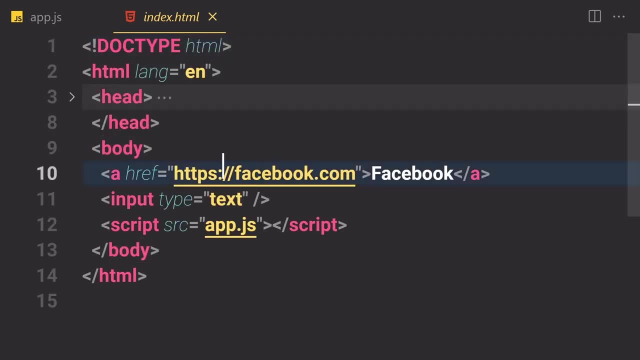 to do is: we are going to go to our html file. i'm going to click on this live coding, go to the appjs file and indexhtml file as well. i'm going to comment our collapses head area. and now, inside this body area, we have just one anchor tag which will just go to a facebook home page, and then we 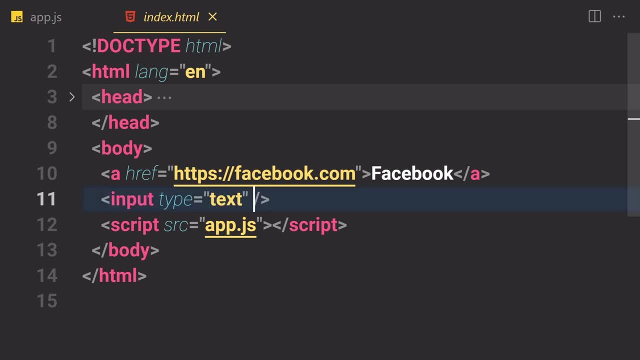 have our one input area right here with the type of text. so this is what we have so far. all right, that's it for indexhtml file. i'm going to right click on it and copy, open it with live server, and this is how it looks like. i'm going to also open it with live server and this is how it looks like. 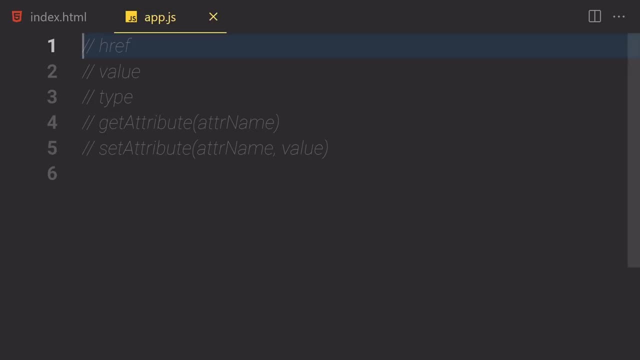 open my developer tools as well. so we are going to be learning about href- attribute value, attribute type and also get element. i mean like get attribute and then the attribute name and then set attribute the attribute name and its value. okay, so we have this href right here. so 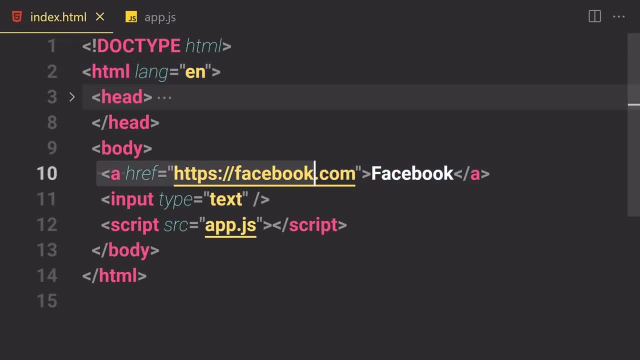 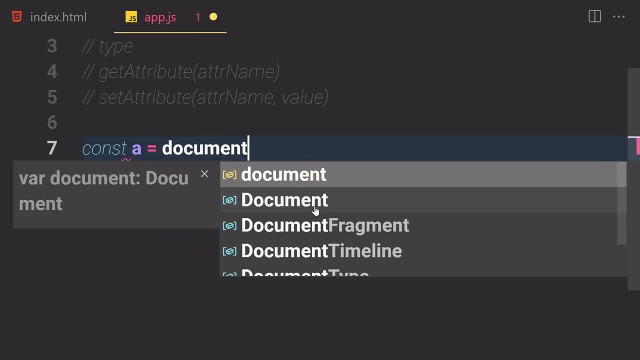 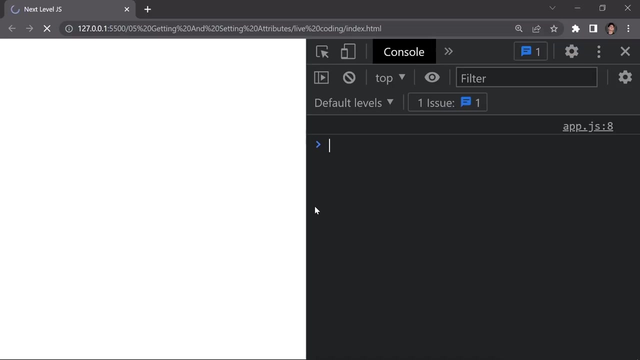 first of all, what do we have to do? we want to select that anchor tag and we want to get that href attribute from there. so first of all, we are going to be writing const and then a, and let's just get our a right here, okay. so if you just log that a to the console, you already know what we. 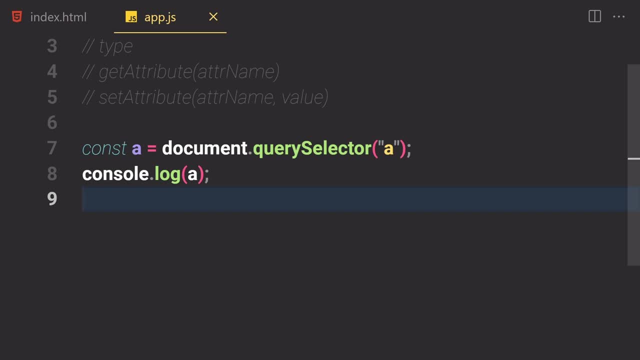 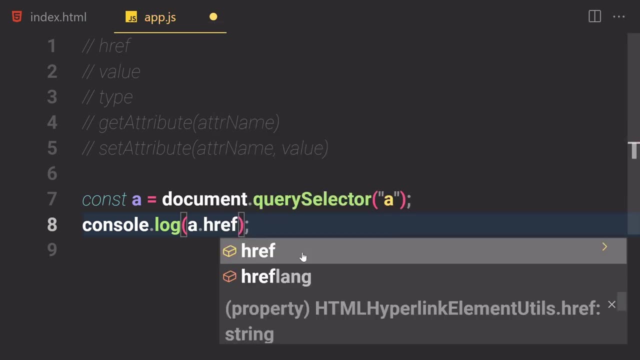 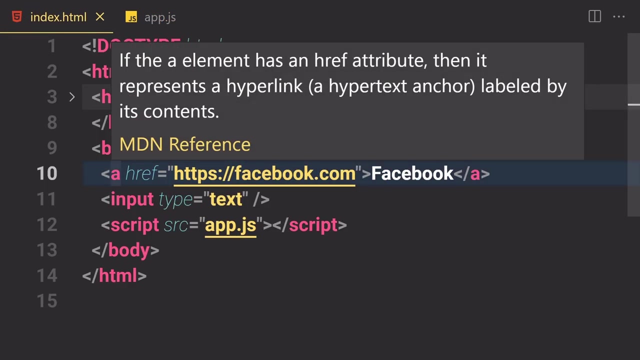 will get. so we will just get this anchor tag right here. so if you want to get an attribute from this anchor tag, so for that we can use dot href. so if we save our file it will not give us the value of that href right here. but if you don't have the value of that href, so let me just cut that from. 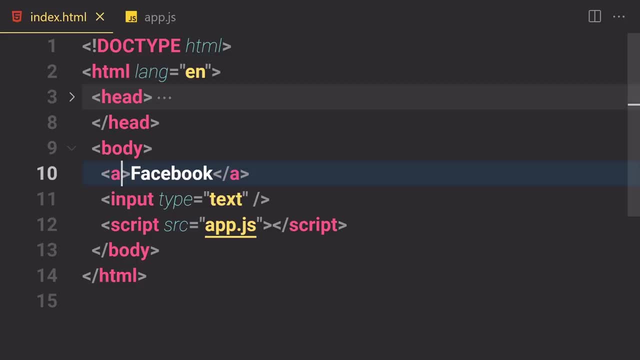 here, save it. it will not give us nothing right here, because we don't have access to the href, so it will not gives us nothing. i'm going to pass it one more time. so we do have this href value uh of just a facebookcom, so that's why we are getting this href uh right here. href value right. 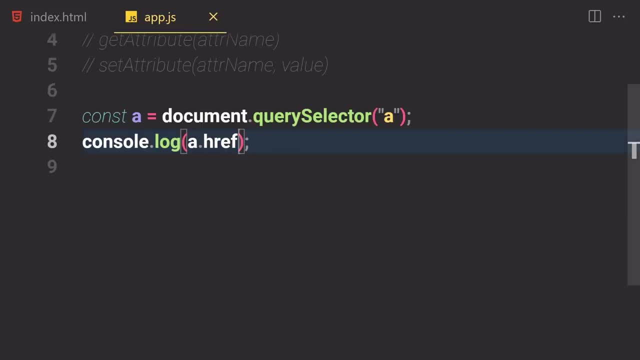 here. all right, so that is the first thing. you know what? we can also change that to something else, like maybe- uh, i don't know- wwwyoutubecom, and forward slash hosan web dev, my youtube link. okay, so let's just zoom out of it, and this is the href value that we want to get. so let's just 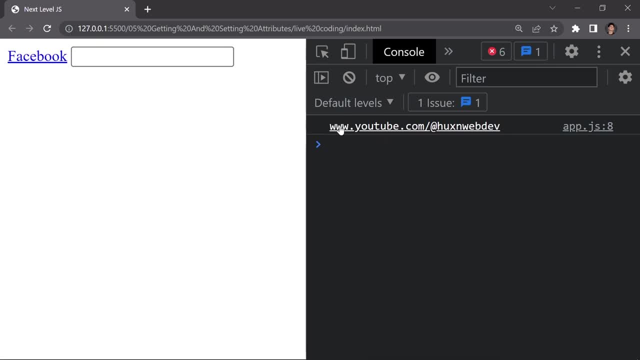 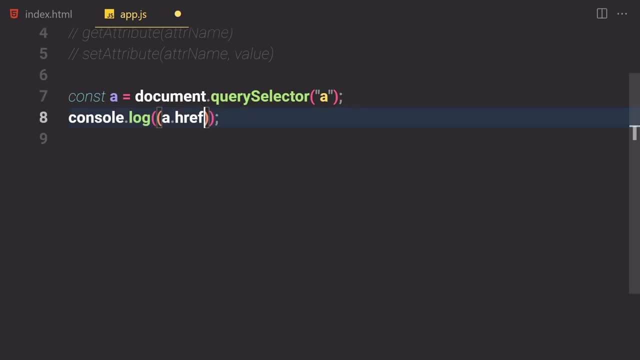 how it looks like. i'm going to save that. so here you can see it will not change that to youtubecom, okay. so this is how we can provide a new value to it and this is how we can get elements, or get values of our elements. so that's the first attribute. now let me just duplicate there. 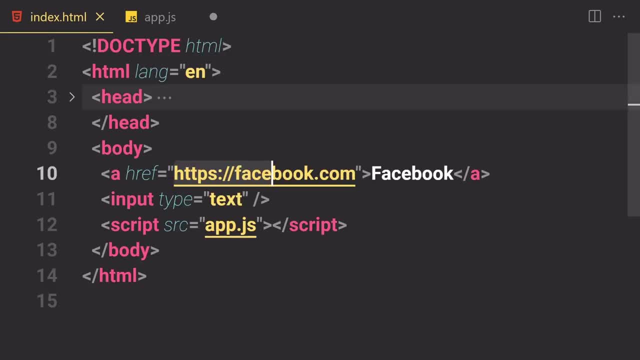 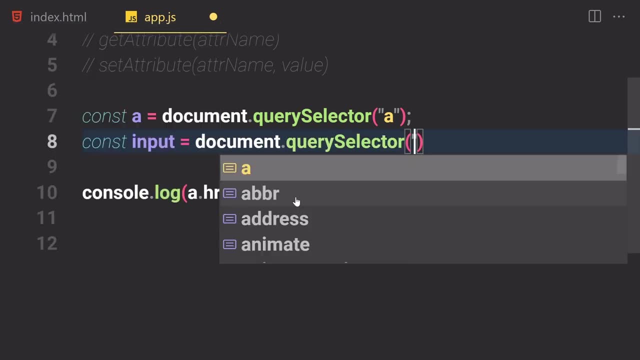 and you know what i'm going to also get my input tags as well. so this input i'm talking about, i'm going to write cons input and film set to documentquery selector of just a simple input right here. okay, so that's the first attribute. now the next attribute which you're going to be learning, 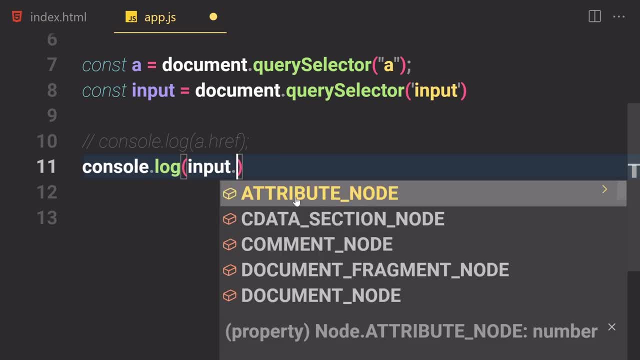 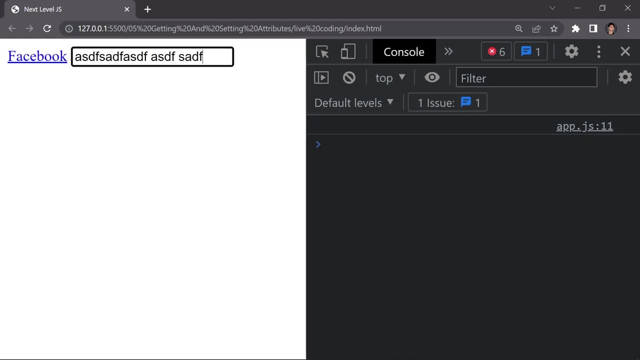 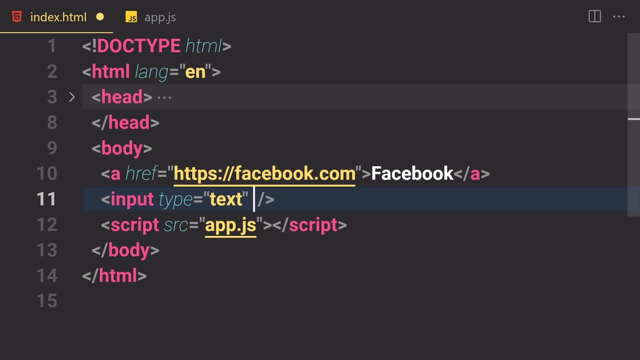 is that let's just log there to the console first of all input dot value cifis out there, and we will see nothing. that's because we don't have no values, nothing inside this input area right here, so we will get nothing. but if you do have a value, let's just put a value to it. so let's just write a value. 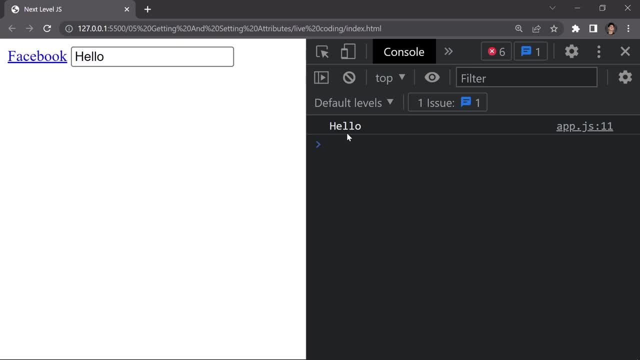 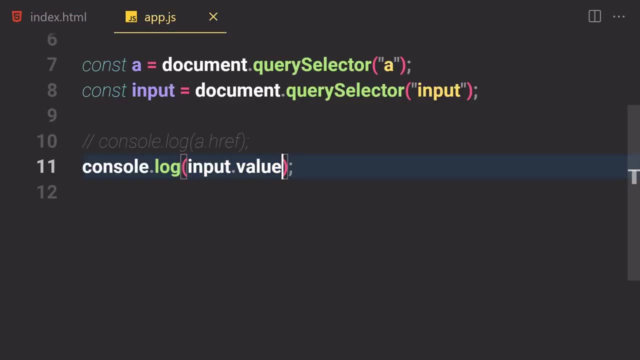 of, i don't know, hello, and now, if you so there, and we are not getting this header right here and this value which we provide right here. okay, so that's how we can get a value from our input. so that's the second attribute we get now. the next attribute which we are going to be getting is a type 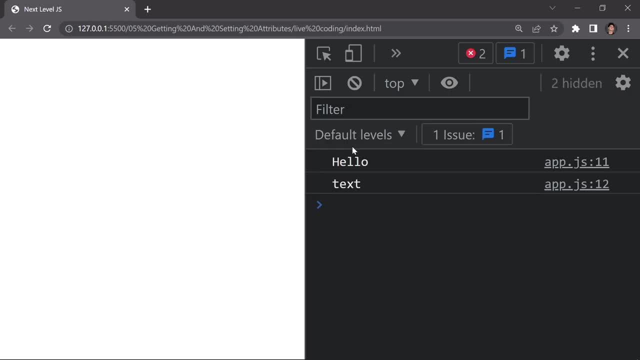 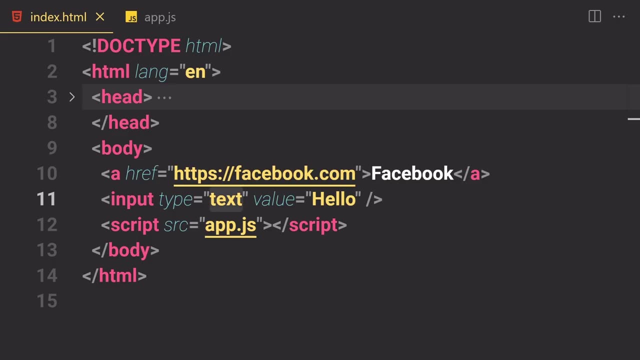 attribute. so i'm going to remove that value and set that to the type. and now if you save that and type is set to text, and we set the type to text right here, so that's why we are getting this text type right here. so if you just change that to like i don't know, email, save it. it will not. 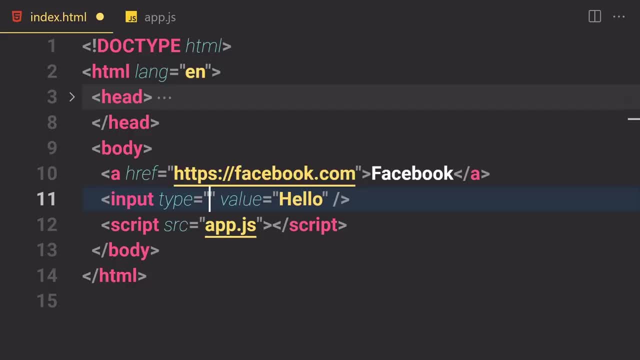 give us email. if you just write a password, it will not set it to password. it will if you just write something else, like something else. and now if you save that and it will give us a text because this something else is invalid, okay, and by default it will just set that to text. and now, if you save, 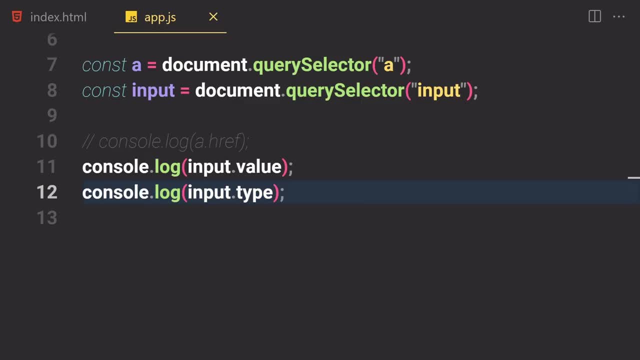 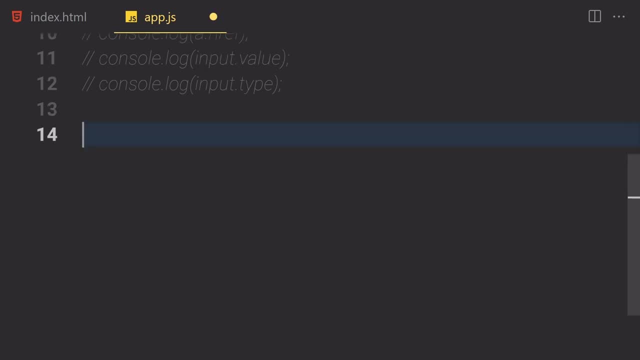 that, and everything is working the way we expect to work. so that's it about how we can get a different kind of attributes from different kind of elements. so now let's just learn about how we can set values to the different kind of elements. so now we have our anchor tag and now we 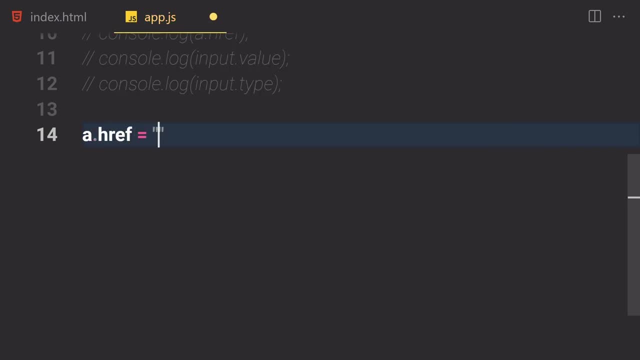 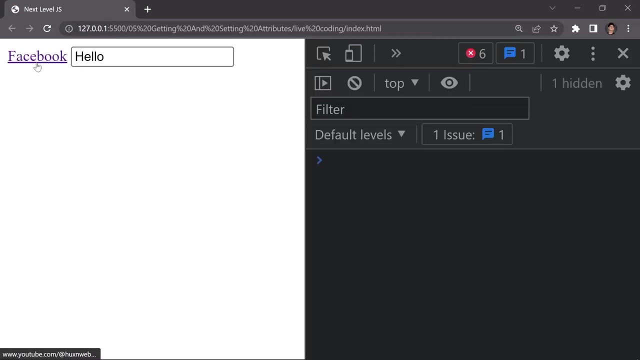 can just change this href to something else, like i don't know, maybe. uh, my own youtube name like, oh you know what, https, and then colon, colon, wwwyoutubecom, forward slash at the red huzzan web dev. okay, and now, if you save that, and now we have a facebook, so if you click on there, 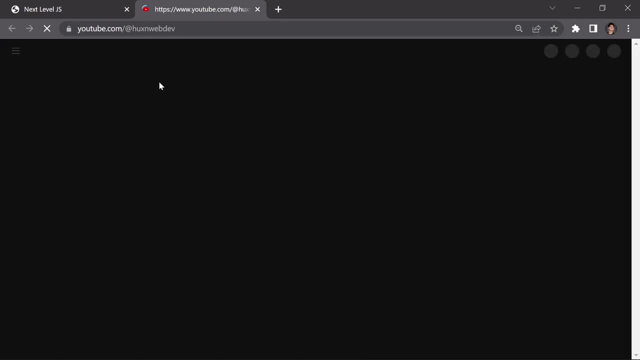 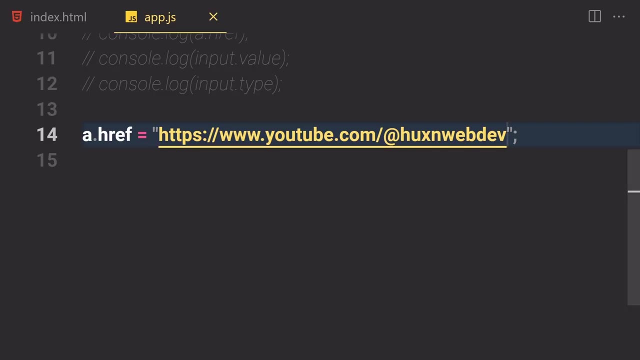 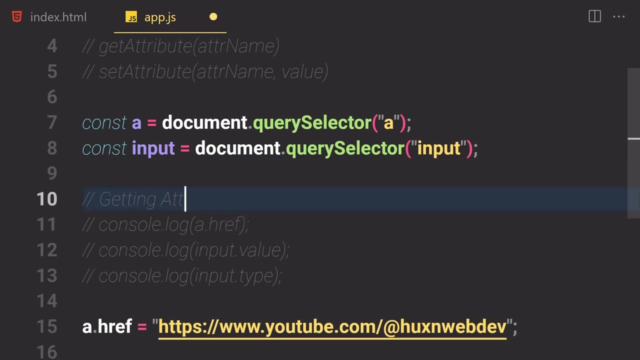 and it will. now brings us to my youtube channel right here. let's just wait for it to render all right. so here you can see that gorgeous cut. here i'm going to close that one. this is how we can get the values, or getting the attributes, or getting getting attributes, and this is about 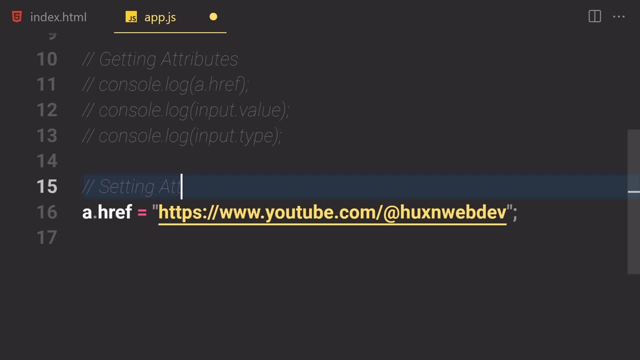 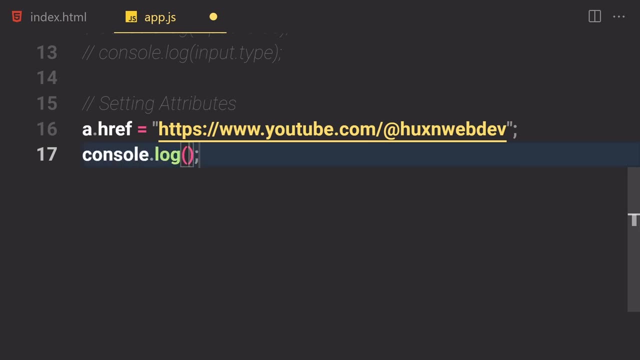 setting attributes like uh, setting attributes like so, all right. so now if you want to set the value of something else, like maybe this is right, consolelog of inputvalue. and if you want to change that to something else, like hello. and now if you save that and we're not, oh, we already have. 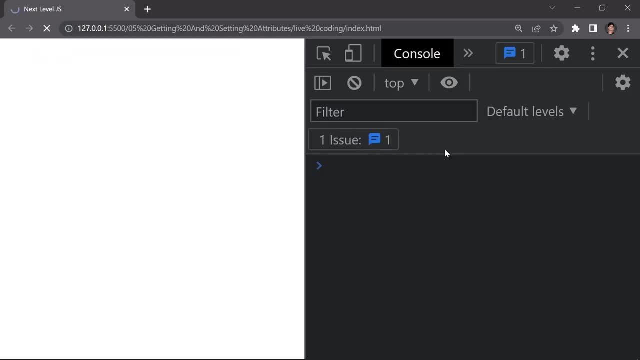 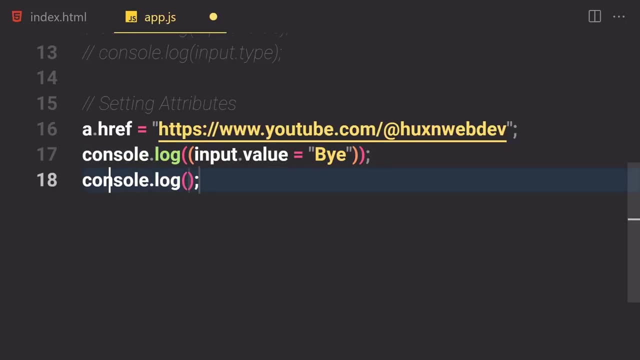 hello, if you want to just say that to like buy, save it. and we are now getting buy in here and also in here. so let's just log the type to the console real quick. so inputtype is already set to text, but if you want to change that to password, 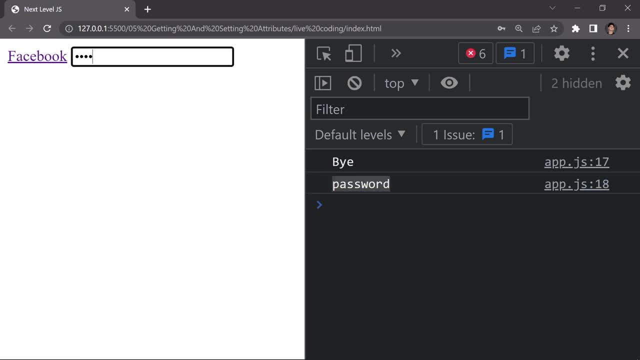 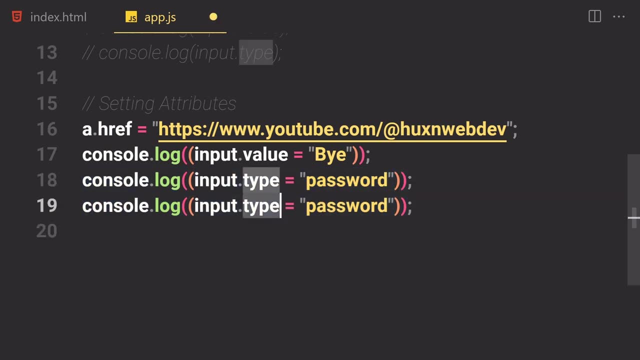 and if you save that- i don't want to change it to password in here and here you can see this will also be affected right here. okay, so this is how we can set the attribute, and now let's just learn about a placeholder, so we can also just provide a placeholder to our forms and inputs. so, um, 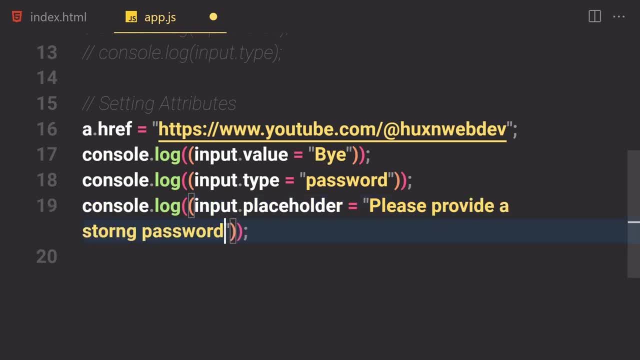 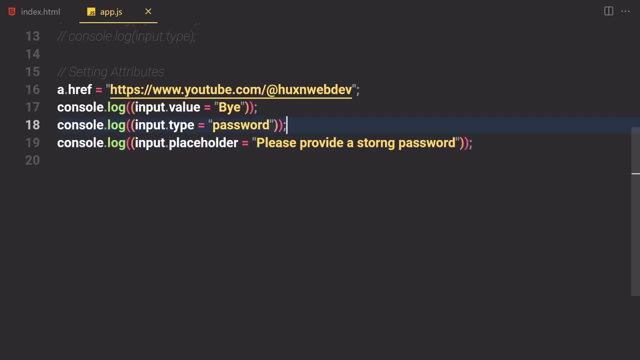 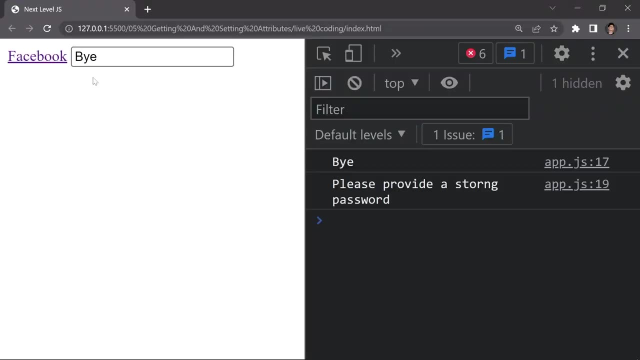 please provide a strong password would be fine. okay, so let's just zoom out. let's just zoom out a bit. and now, if you sell that, but we have to comment this line out. and now, if you say there, and let's just remove this value from there, save it. oh my god, we already. 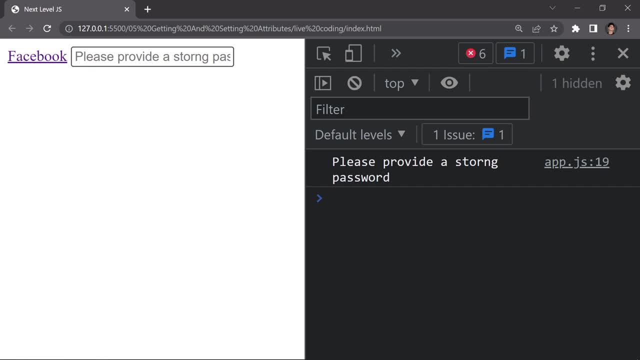 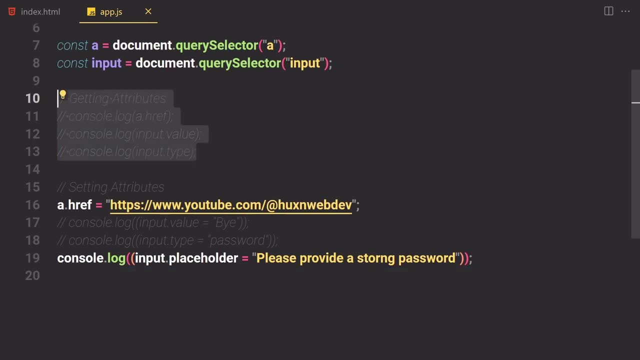 set up real you in here. so, coming this line out, and now you're getting like: please provide a strong password. that's because of this placeholder attribute. so this is how we can get attribute, and this is how we can get attributes. and now i'm going to show you how we can get attributes. so 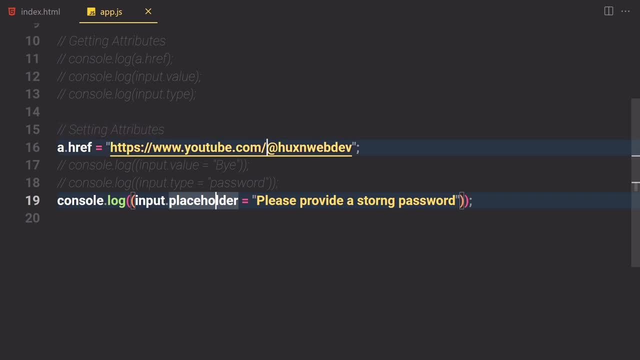 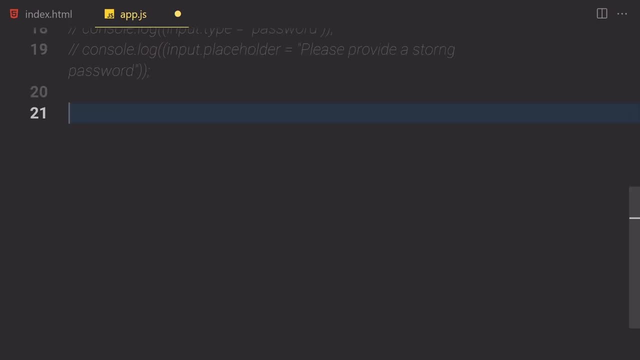 we can set new attributes, so i'm going to comment both of these line out as well. all right, so now the next thing which you have to do is that we are going to be learning about a method called get attribute and then the attribute now, so let me just write that in here. oh, my god, let's just write. 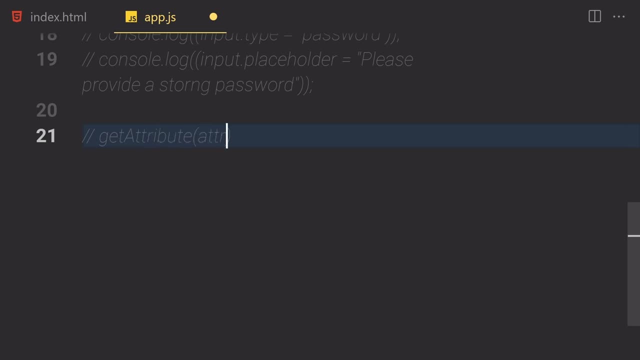 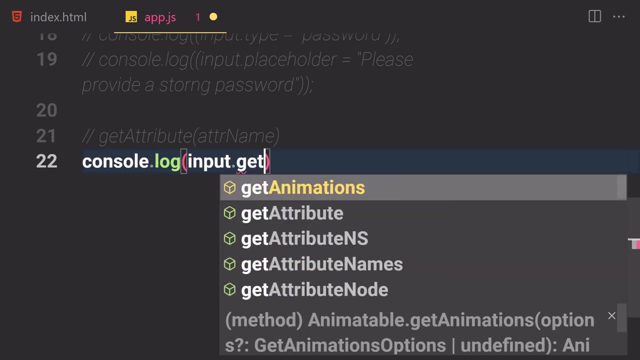 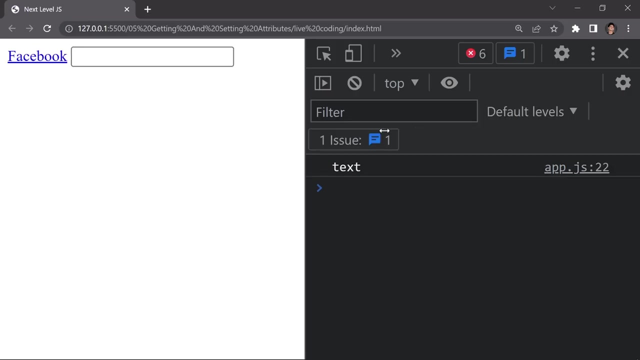 get attribute and then the editor name like a attribute name in here. so i'm going to just write consolelogin here and then let me just select my input and we can just write get attribute method right here and now. let's suppose, if you want to get a type, so you just provide a type, save it and 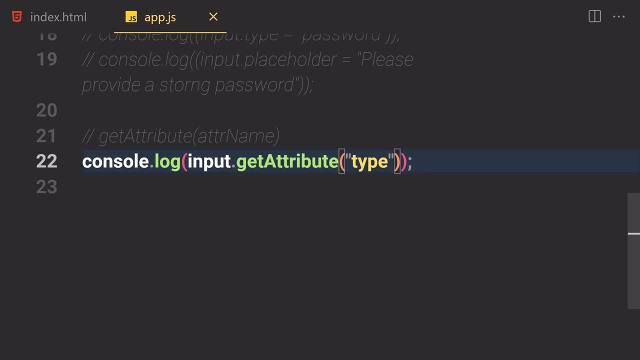 we will get like text right here. so let's suppose, if you want to get like i don't know, let's just provide a placeholder to it as well. so placeholder will be uh, email. so placeholder is now set to email. here you can see that. and now, if you want to get an email, so you can just write email, save it. 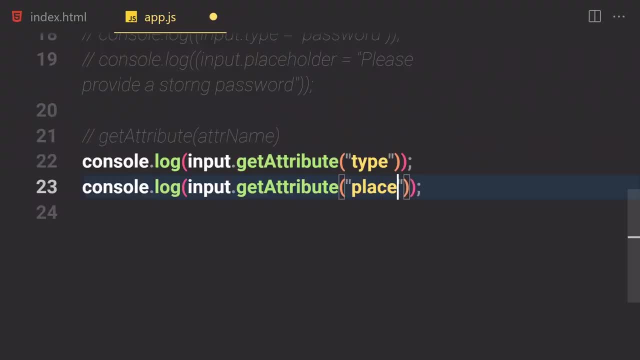 uh, okay, instead of writing email, we can just write a place older like so. and now, if you save that and we are now getting email right here? okay, so this property, or this method to be precise, will allows us to get attribute from a specific kind of elements. okay, so we can also set attribute. 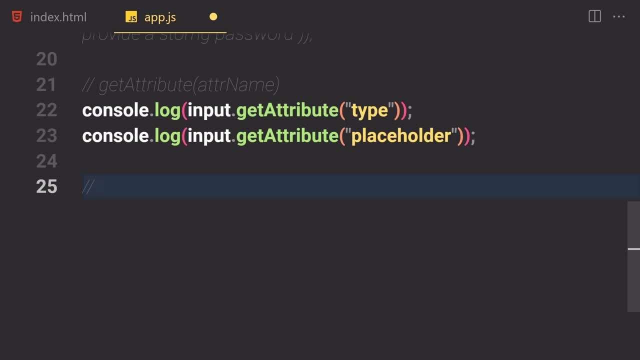 to elements. so that was it about for getting attribute. so now let's just learn about a set attribute. so set attribute a-double-t-r-i-b-u-t-e. did i spell it correctly? so set? and yeah, let's just copy that and i'm going to paste it right. 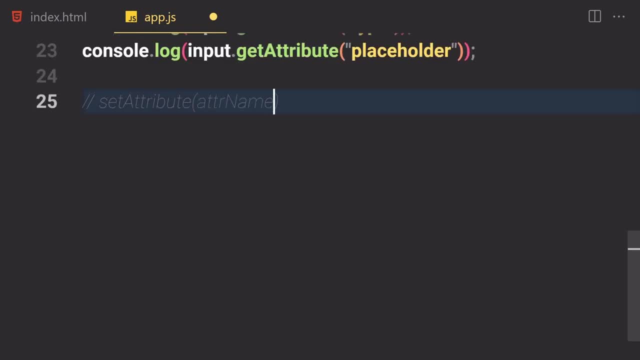 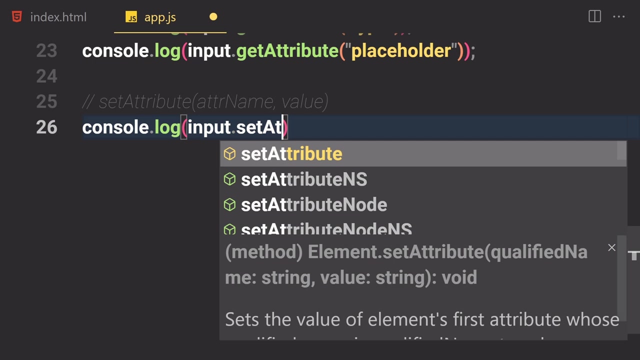 here and then the etcher name like the attribute name, and we can also provide different kind of values to it. so, uh, let's just write consolelog. let's just write consolelog of input. first of all we have to get our input and now let's just use set attribute method on it. and here we want: 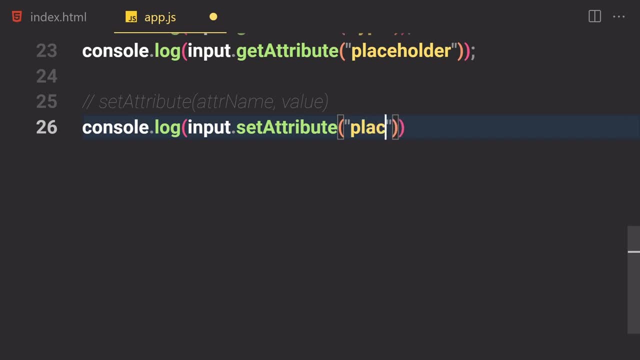 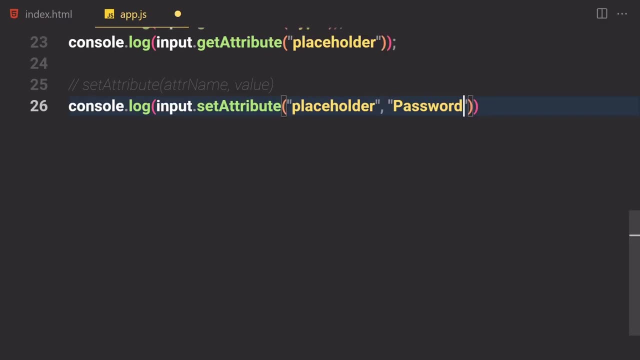 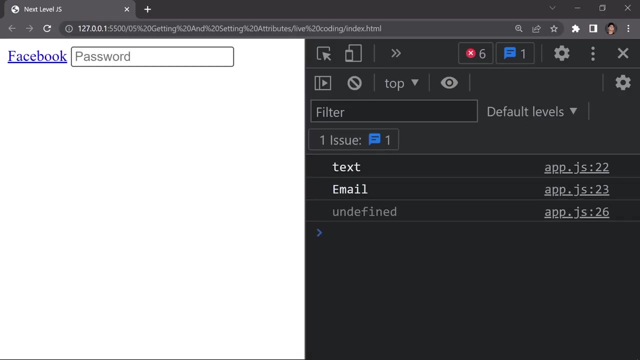 to get like place holder p-l-a-c-e holder right here and now. you want to provide a value of like- uh, i don't know password, maybe so we can just provide a new value of password. it is currently email, so we can also change that to password. so if you save that and here you can see it will. 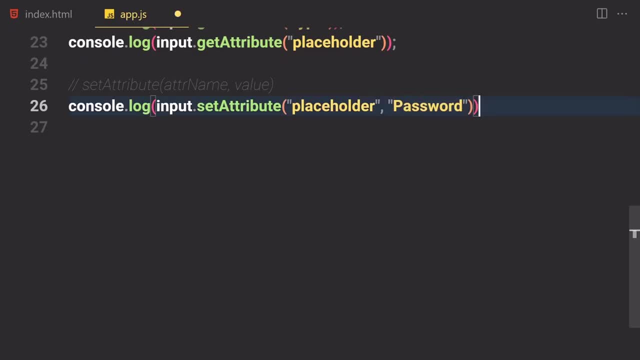 now change it to password and we don't have to provide that in console. so let's just remove this console from there and this is how we can set a new value. so now let's just change that to like a no type to be password as well. so i'm going to also change the time to be penciled. so if you 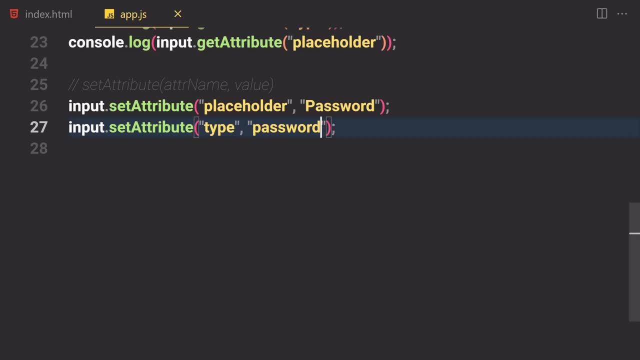 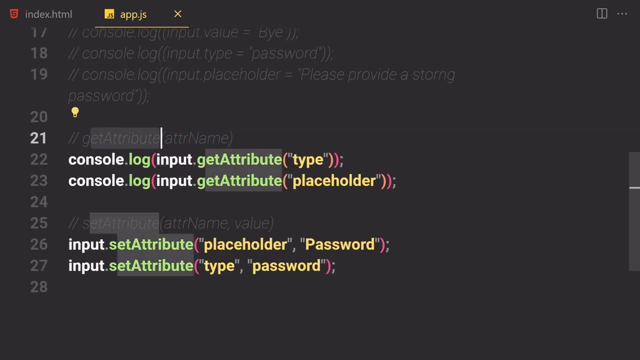 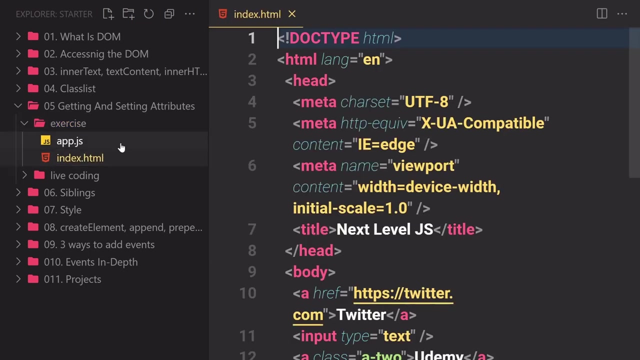 save that and the type will be also set to password. so this is how we can get attribute and this how we can set attribute, and these are the methods we have for getting attribute and setting attributes. all right, that was a lot of talking. now let's just get into our exercise. and now let's just tackle. 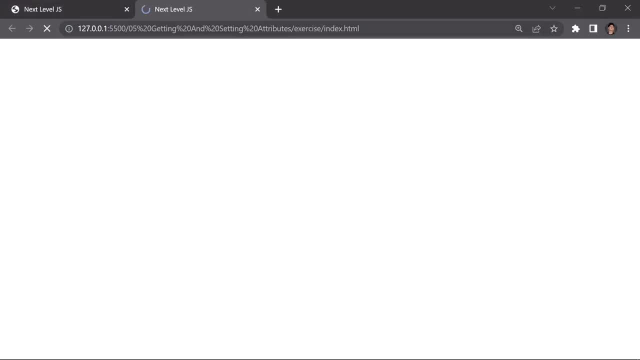 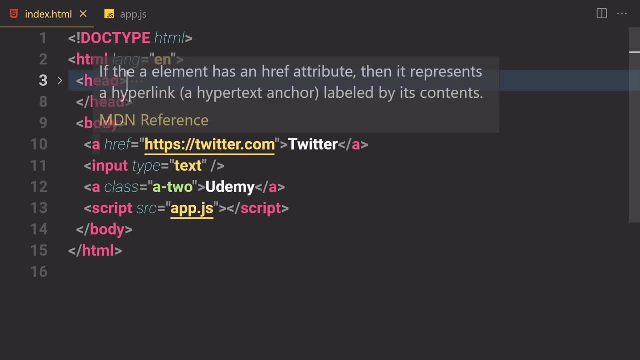 this exercise and i will highly encourage you to do that by yourself, but if you can do it, i'm already over right here. collapse this head area right here. so we have our anchor tag with the href of twitter and then we have our input area with the type of text. then we have anchor tag with the class of a2. 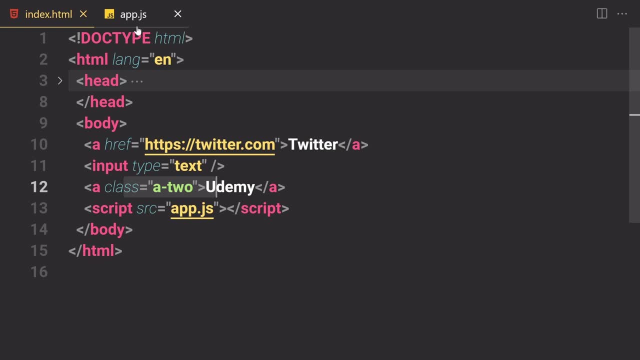 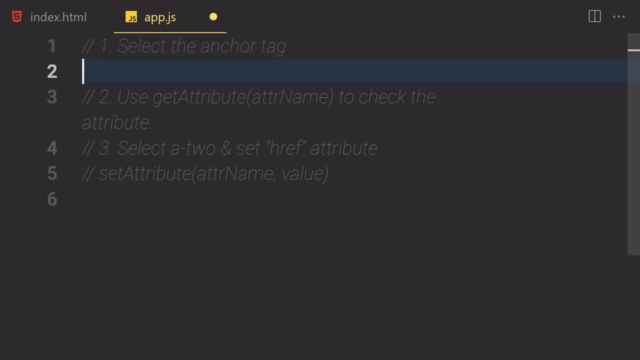 and no and no hrefs on this anchor tag. all right, so what do we have to do? first of all, let's just get into it, select the anchor tag. let's just select that by using. what was that anchor tag? yeah, i'm gonna write: const. anchor tag will be now equals to documentcreate selector. 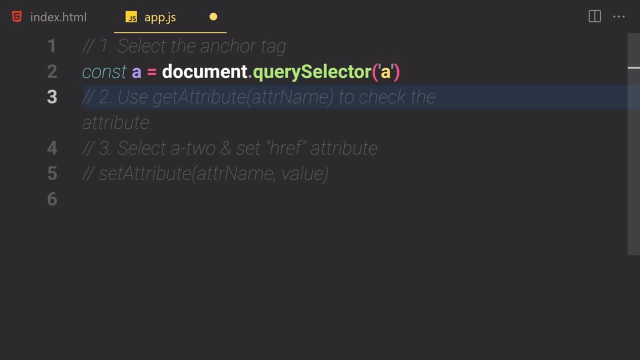 of anchor text. so the first step is finish boss. what else do we have to do? use a get attribute, attribute name to check the attribute, all right. so now let's just do that real quick. so consider log of aget attribute and let's just provide attribute name of like which kind of 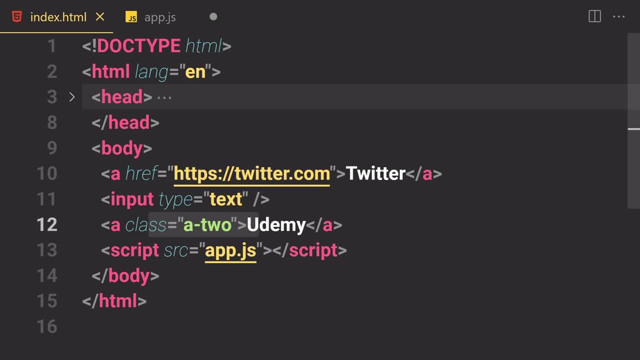 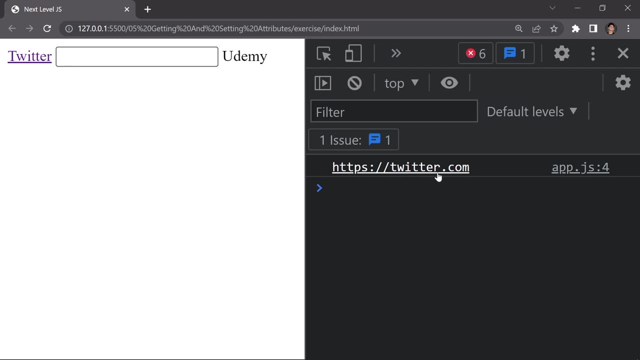 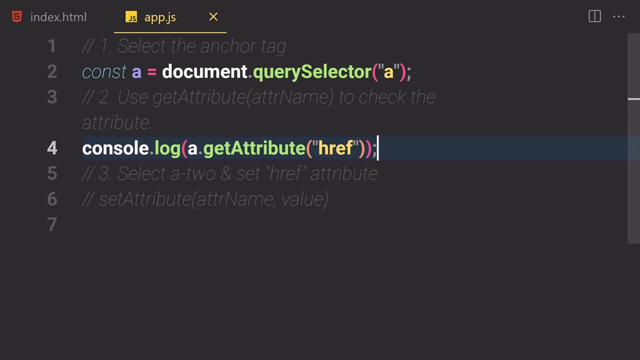 attribute. should we check? okay, so we have an attribute of href, so now let's just or href inside. then if you save that, it will now give us a strata right here. so that's correct. now what else do you have to do? select the a2 and set href attribute to it. that's kind of awesome. 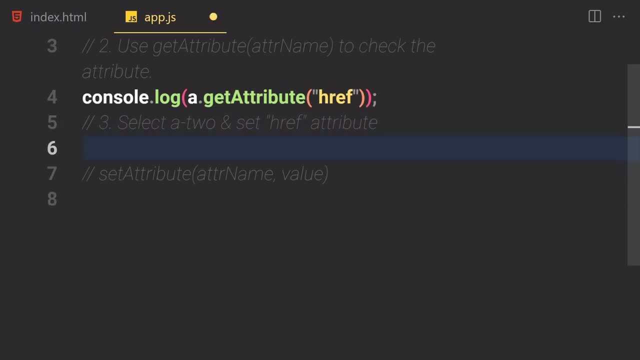 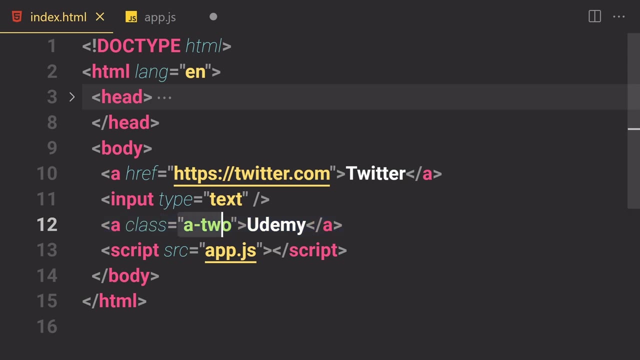 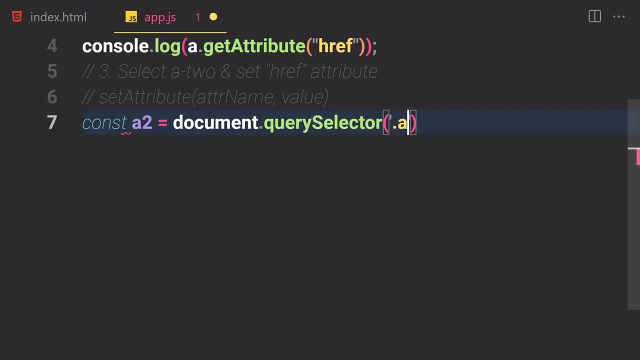 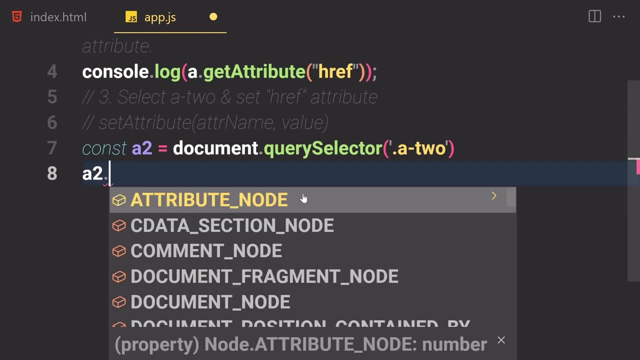 so we can just write like: uh, i don't know, let's just select this a2, where is that all right? so we have this a2 right here. let me just write: uh, const a2. and now we go to documentquerySelector of a-2. okay, so what do we have to do? set href attribute there, so a2.set attributes of like i. 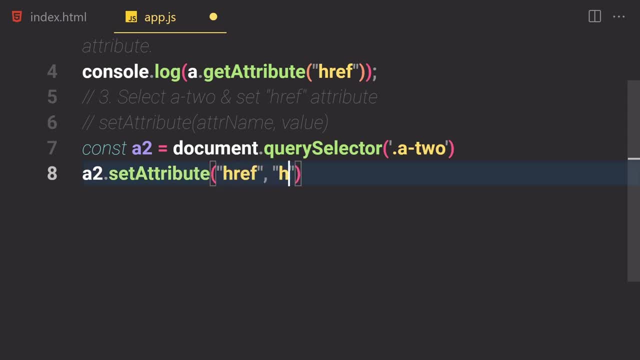 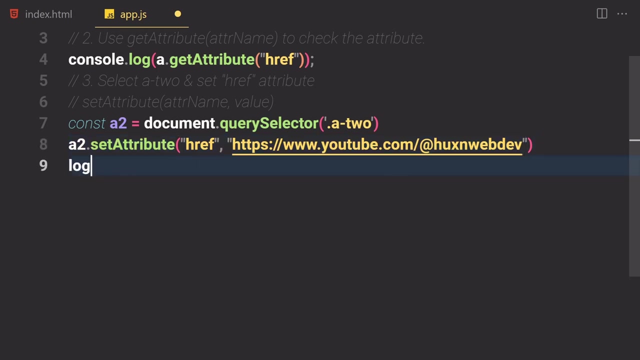 don't know, href will be fine and we can just give our own youtube channel links. so https//wwwyoutubecom, forward slash at third. third web dev my channel link and let's just log that h2 to the- not h2 but h2 to the console. so if you, 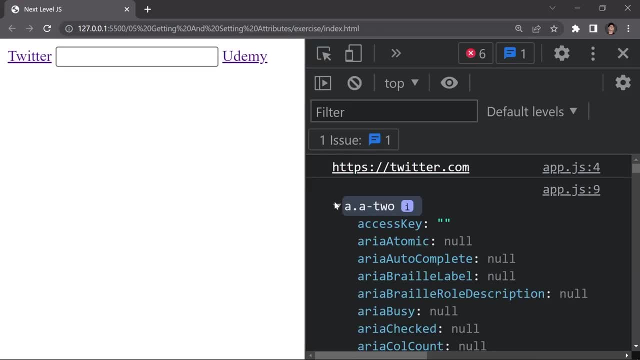 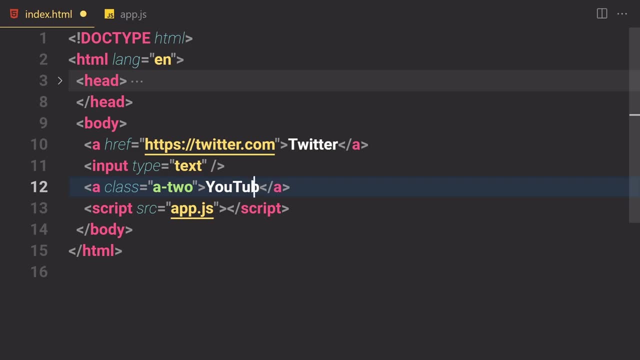 save that and we are now getting this a2. uh, okay, so it's a udemy. it's a udemy. i'm gonna change that to youtube. save it and now, if you click on that, it will now bring us to our youtube channel right here. okay, all right, so we are totally done with this. uh. 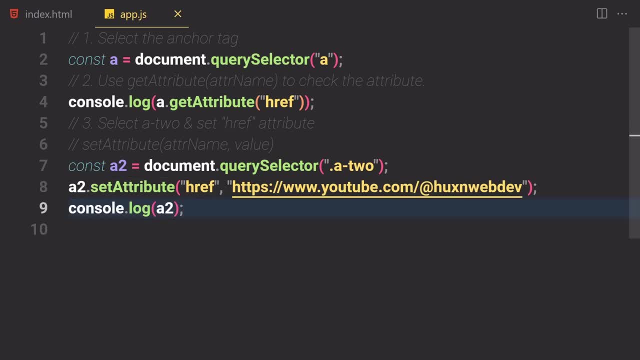 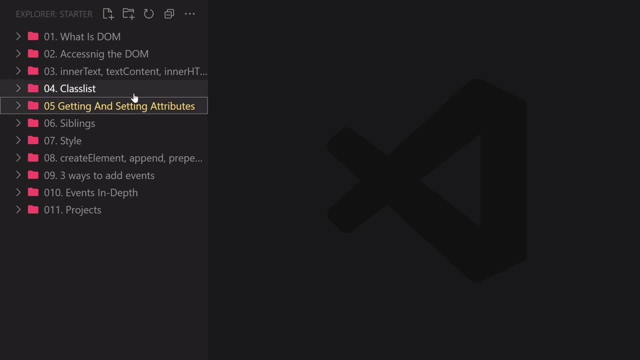 exercises as well, but for a bonus. yeah, you know i'm not gonna give you any bonus. you're not worthy of it, i'm just kidding. we don't have any bonuses, all right, so now we are totally done with the getting and setting attributes. so now the next topic which you are going to be learning about is something called siblings. 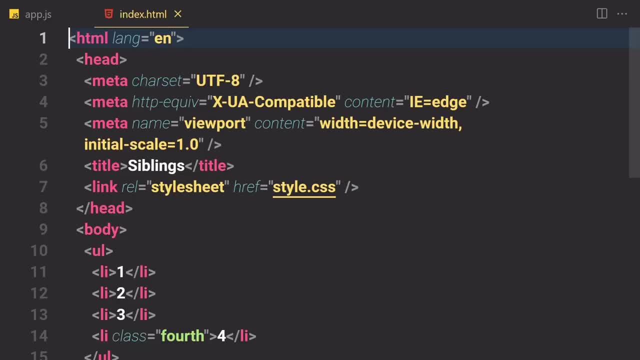 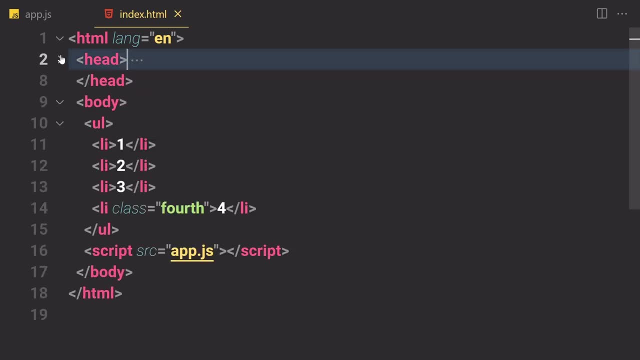 i'm going to open my indexhtml file and appjs file. right click on it and open it with the live server, hide the metadatas from there and let's just see: okay, so let's go ahead and let's just go ahead and run that. do it just now, all right, so now we have an utxt file, all right. so let's. 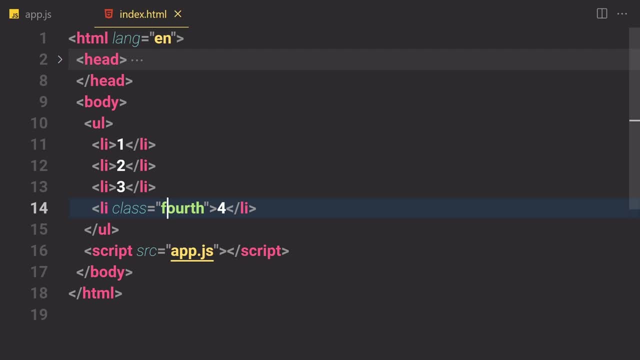 drop our this object into floor out, and i made a lot of sense for this evil class, so i'm gonna void it. okay, i gotta fine impactedals now and then i'm gonna follow along with this stuff and i can just provide to all of you. so let me look at let's. 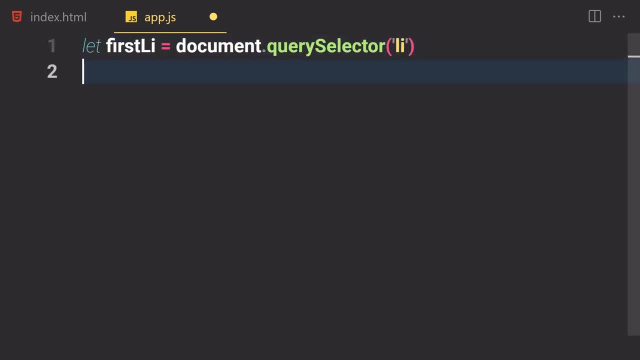 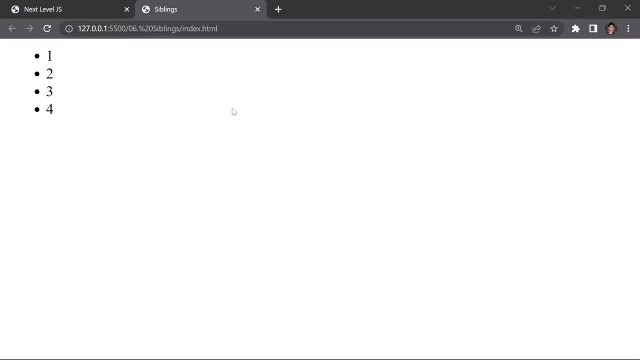 document, that query selector of or li. so we already know that it will just give us the first li. and now if you just log there to the console, like first li, and now if you sell there and open it with a console and say goodbye to that one. so here you can see, we are now getting our first ally right. 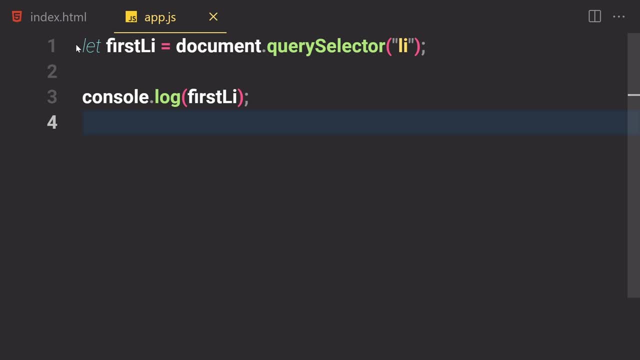 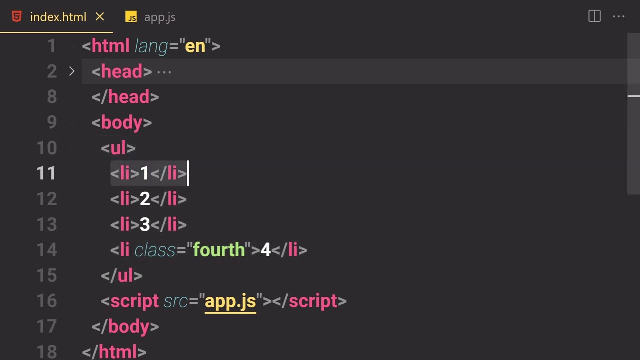 here. okay, so now, if you want to get the parent of this ally, so like, what will be the parent of this alli? the parent of this ally will be this ul. so what will be the parent of this ul? the parent of this ul will be this body. so what will be the parent of this body? the parent of this body? 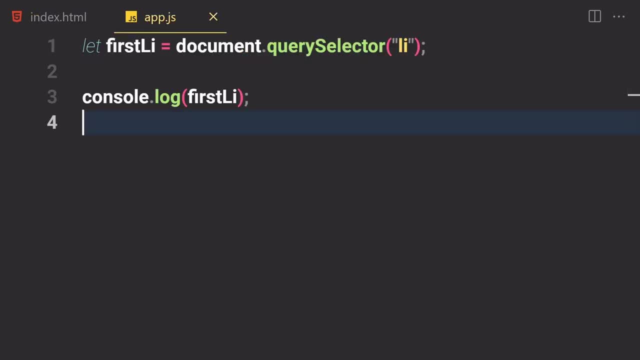 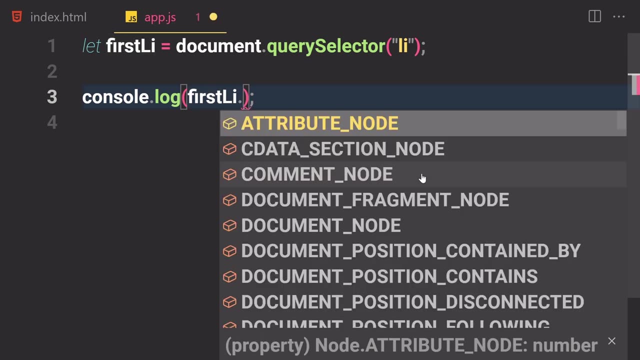 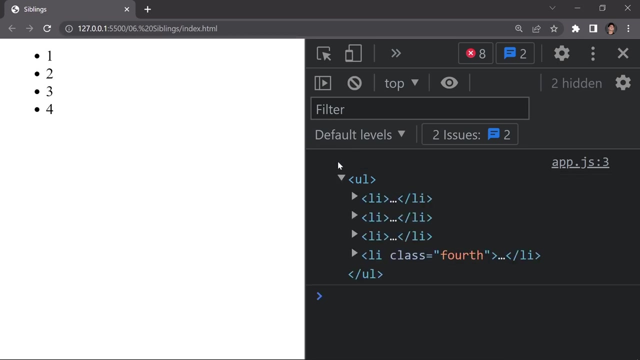 will be our document and then, finally, it will give us nail. so let's just see what will be the parent of this first ally. so i'm gonna just write um parent elements so it will give us the first parent of that element. so if you saw that. so here you can see, we are now getting a ul right. 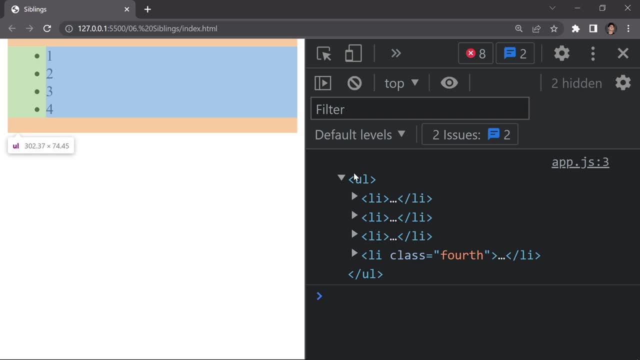 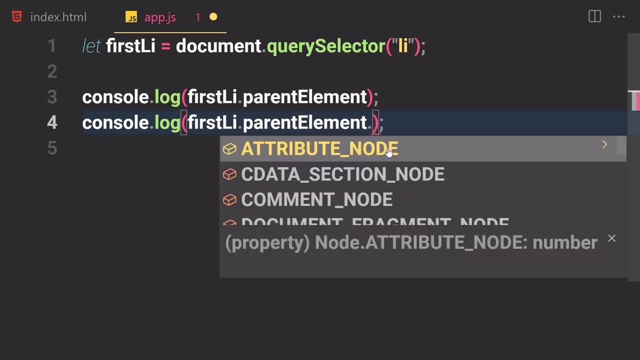 right here, so let's paste it in, but of course we will get the 같은 element of the first parent so here. so the parent of this ally is this ul, so that's why we are getting this ul right here. what if you just duplicate this line of code and we just use that same method? i mean like same. 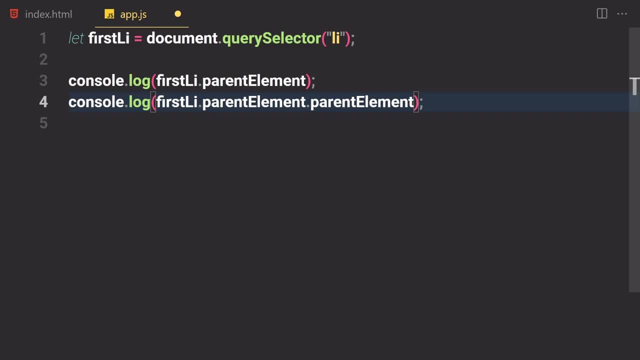 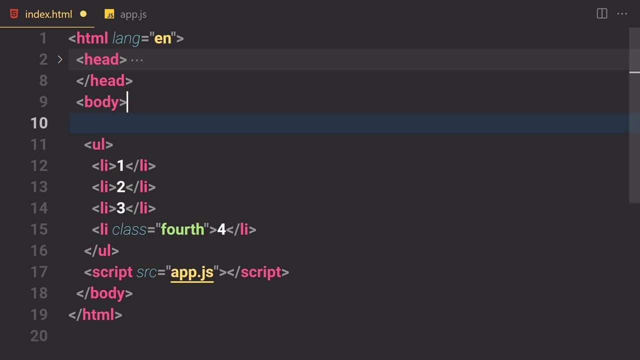 property as well like parent element. one more time, i'm going to zoom out a bit. and now, if you save that, it will not use the body right here, because the parent of the ul is no body. if you just wrap that in a section, let's just write a section, cut that from there and i'm going to pass. 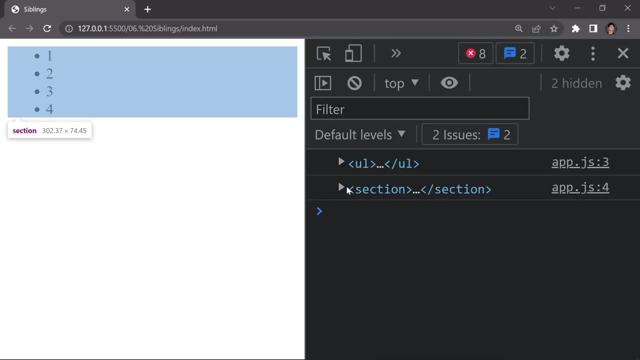 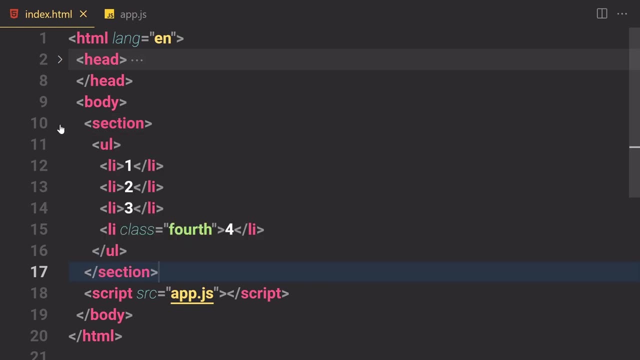 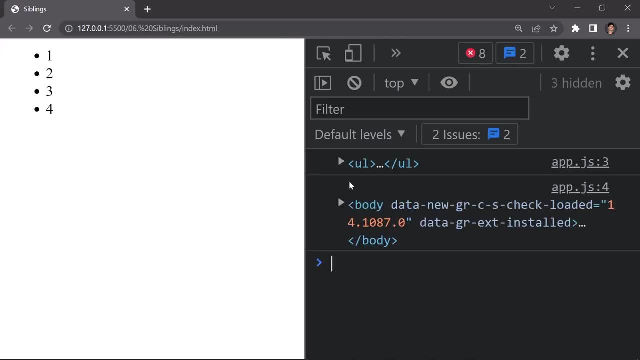 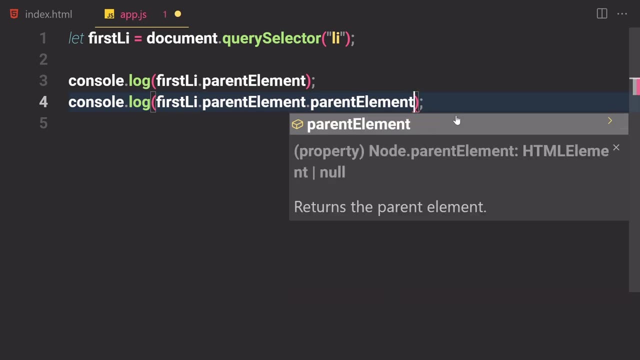 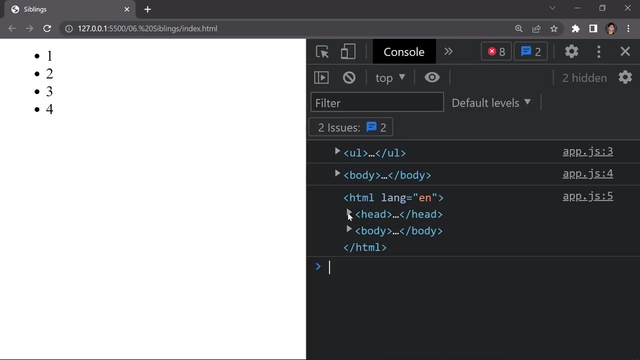 i'm going to just remove this sections from there and we already know that we have the parent of body. but if you want to check the parent of this body, i'm going to just duplicate this line of code and i'm going to just change that to parent one more time: parent element. and now we are getting this html right here like a. 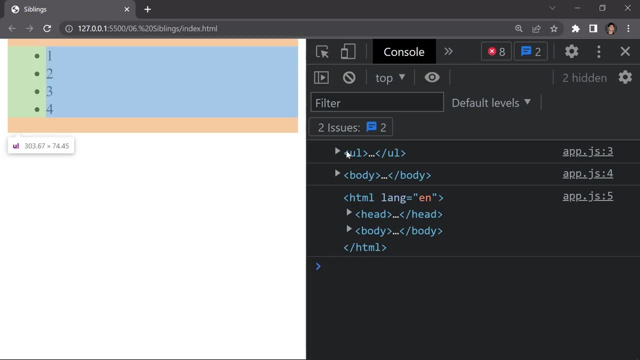 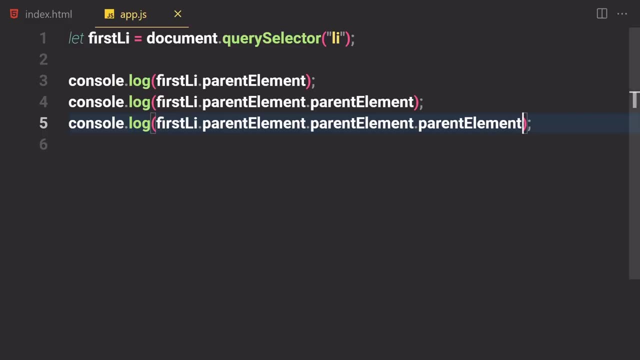 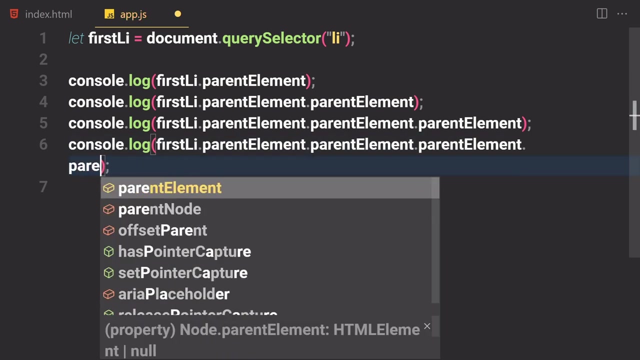 root, uh html. so we have uh first of all ul, uh, then we have first of all we have a ul, and then we have a body and then we have our html document. but finally, let's just check and let's just use that parent element one more time like parent element one more time. i'm gonna just zoom out a bit. so if 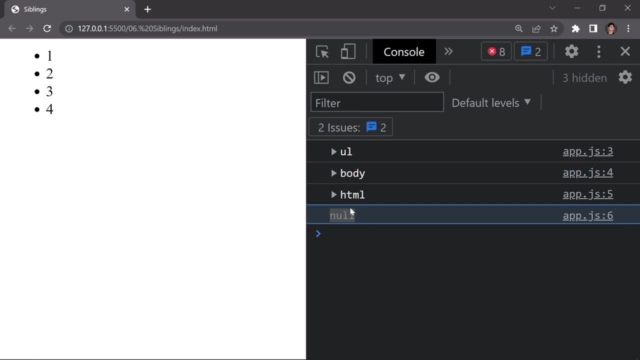 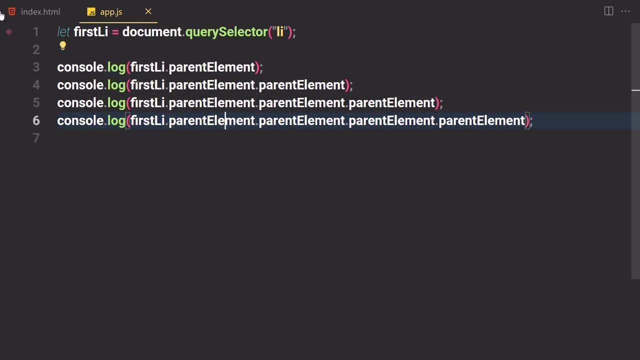 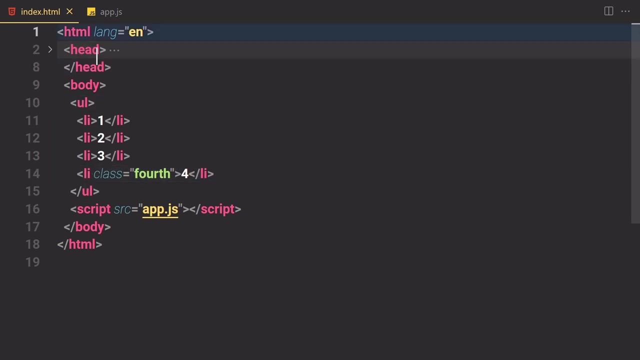 you save there and it will now give us nil, because we don't have any parents for this html, so it will now give us nil. okay, so this is how we can get a parent for each of the elements. so, uh, this is the, so we can also just go from this one, so the parent of this one will be ul, and so on and so forth. 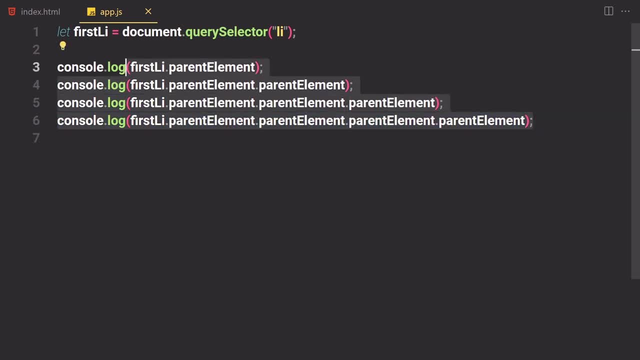 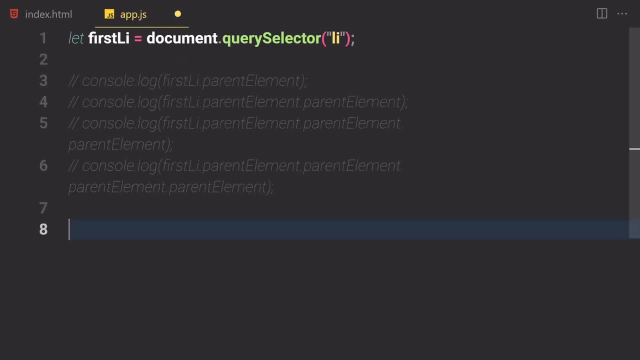 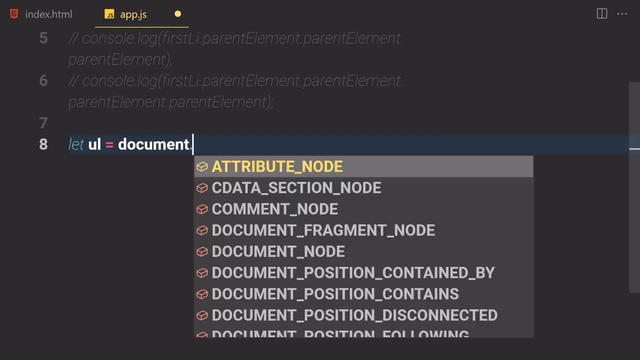 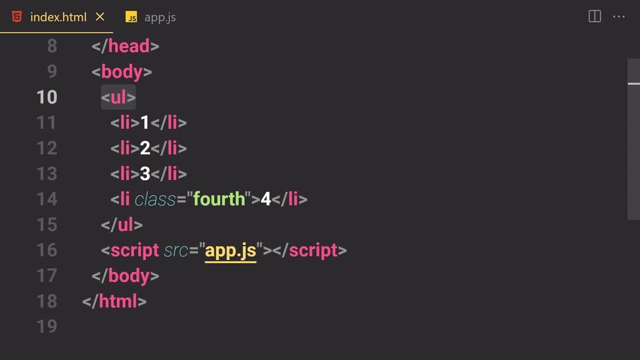 let's just write first of all that ul and documentquery selector, and we are now selecting this ul right here. okay, zoom in a bit. we are now selecting this ul and now if you want to access the children, so for that we have our children property. so i'm going to just write consolelog. 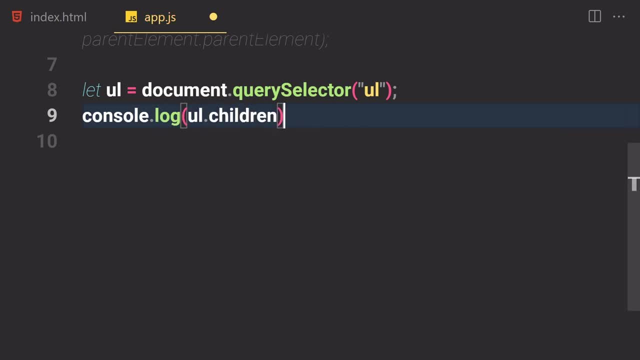 of ulchildren. so if you just write children and now if you save there, it will now give us the collection of all of these la's right here. okay, so we can also access each children if you want to, like i said earlier. so we can also access each children if you want to, like i said earlier. 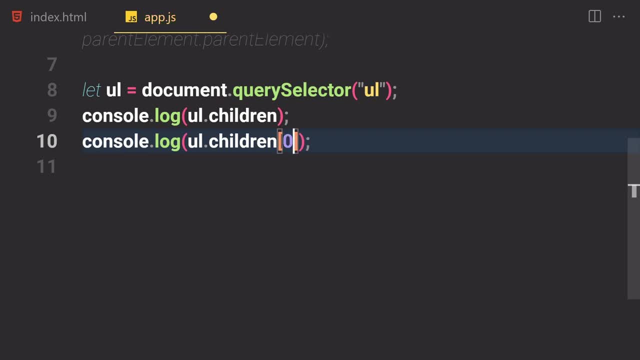 we can just specify the index of zero, it will not use the first one. so to outside in, like i said earlier, we can just specify the index of zero, it will not use the first one. so if we sell that into the collection of all of this, and now here we can see if a log is the first one, we can also 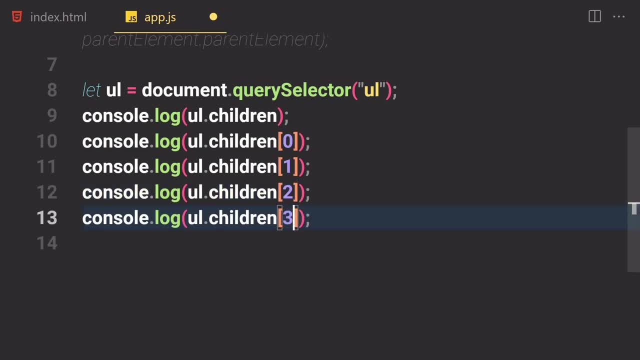 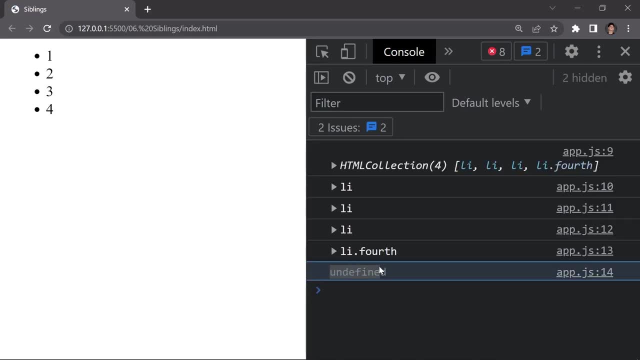 get like the second 1, the third one, the fourth one if you want to be. so there after everything is all of this, but if you try to access the fourth one in this case, so it will not give us and applied because we just have la's for one to four, we don't have more. 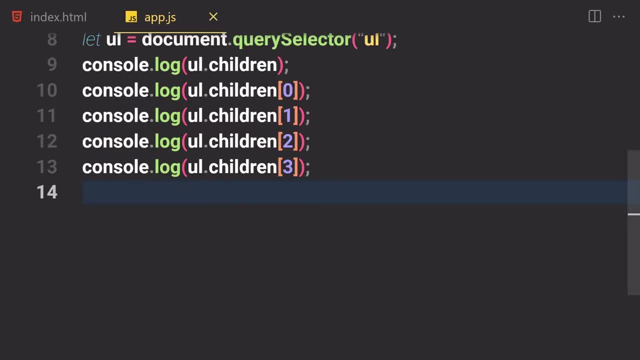 than that. so that's why we are getting this. I'm drying right here. I'm going to remove, move that. all right, so now we can also change the inner text to be like something else, maybe, or we can also get the inner text if you want to. so let's just write consolelog of maybe, ul and then 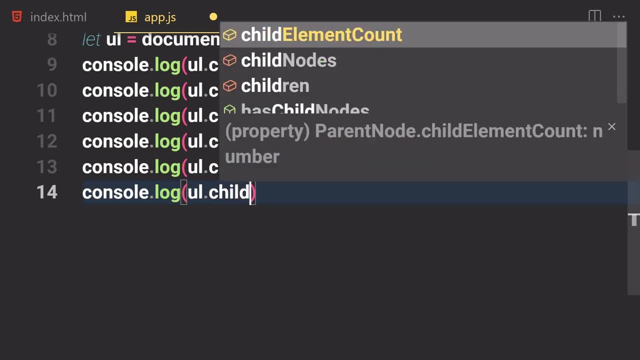 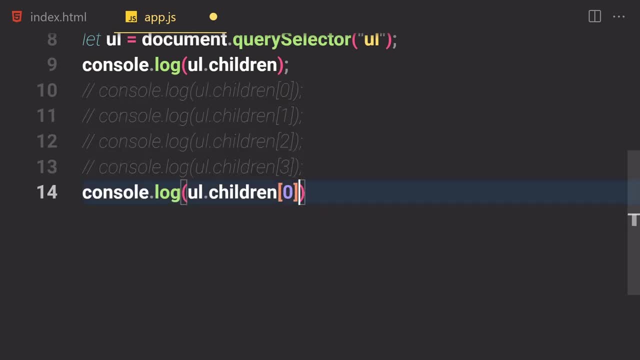 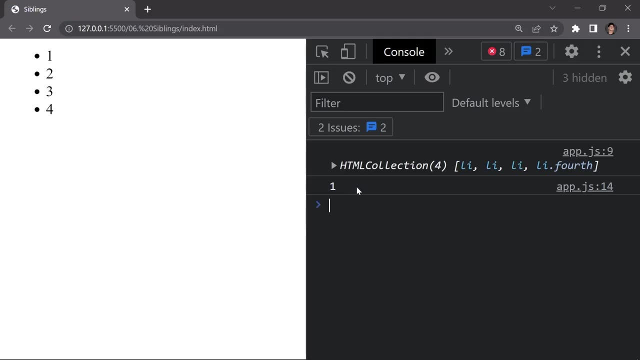 children, chill, come on, children. oh my god, children, there we go. and now let's just select the first one. i'm going to comment the other one, and now let's just get like inner uh text, inner txt, like so, and now, if you save that, so the inner text is set to one, so we are now getting one. so if you 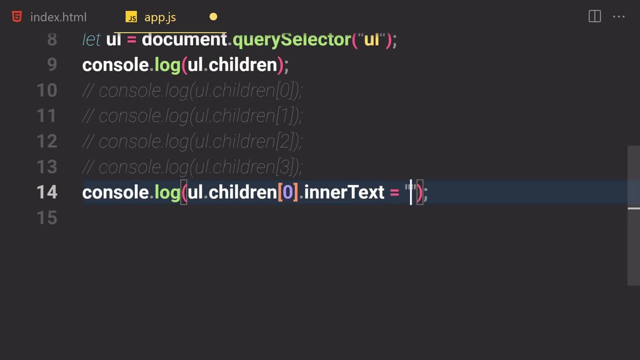 just change that to something else, like uh, i don't know, uh one as letters, and so if you save that certain, i'll change it to one. like: so we already learned about text and stuff like that. i'm going comment this line out. so this is good about how we can get a parent and this is about how we can. 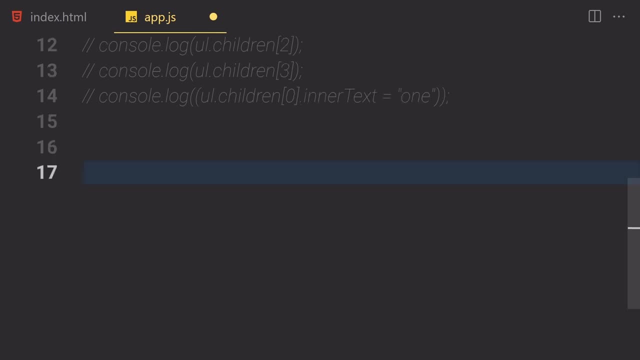 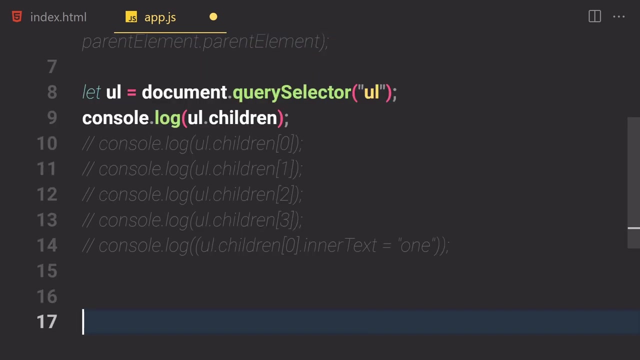 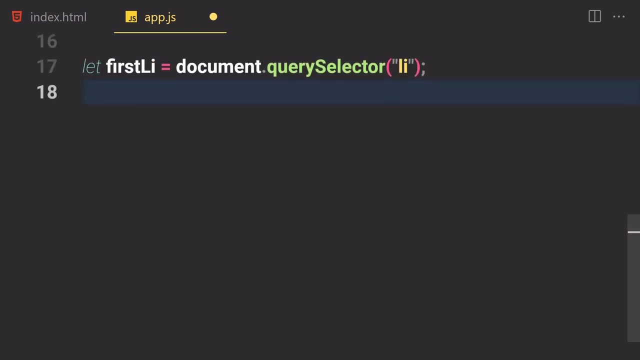 get a children. so now, let's just learn about a siblings as well. so, uh, we have a first ally. i'm going to comment: or you, i'm going to copy this line of code, comment this line out, and i'm going to also comment this line out as well. so now, let's just learn about a sibling. so we have our first line. one more time. 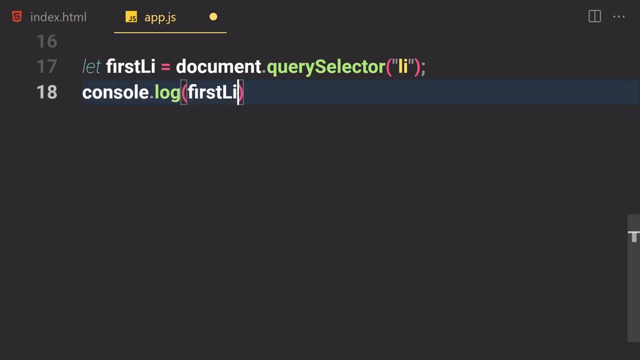 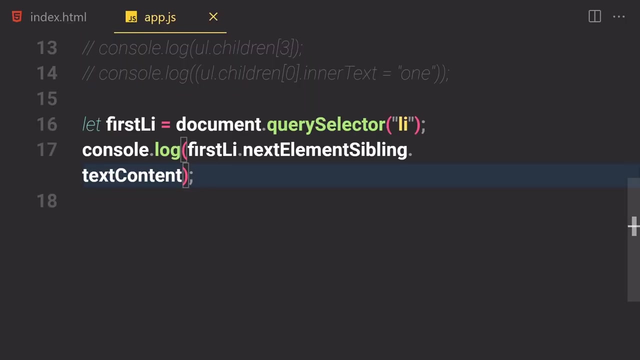 and now let's just write consolelog of first ally dot one next element, sibling. certain log gives the next element sibling. and now, if you save that, uh, let's just write text content so that we get to see our content. so we are now getting the second one right here, so this one is the first. 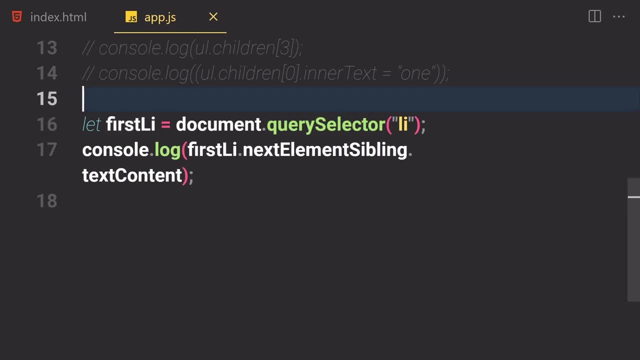 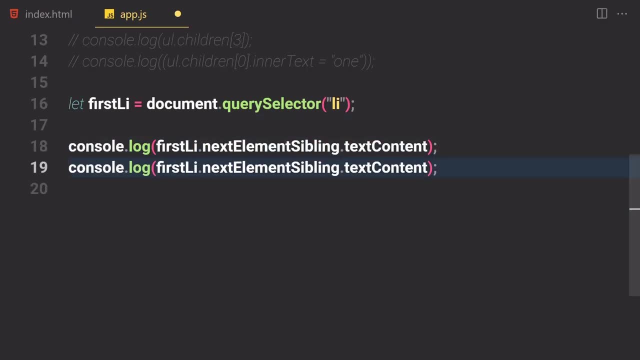 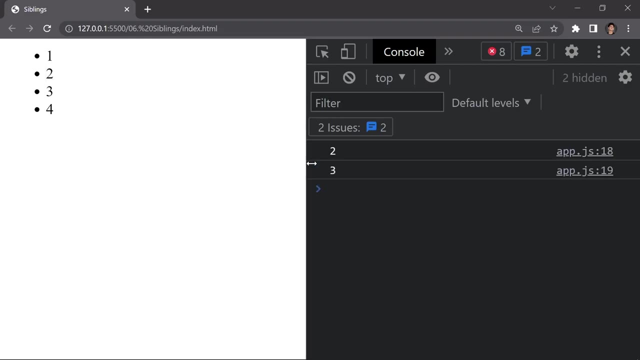 element and if you just use that next element sibling property on there, certain log uses the second property. so i'm going to hit enter right here, zoom out a bit and duplicate that. and now let's just use this next element sibling one more time and just write a dot in there, save it and it. 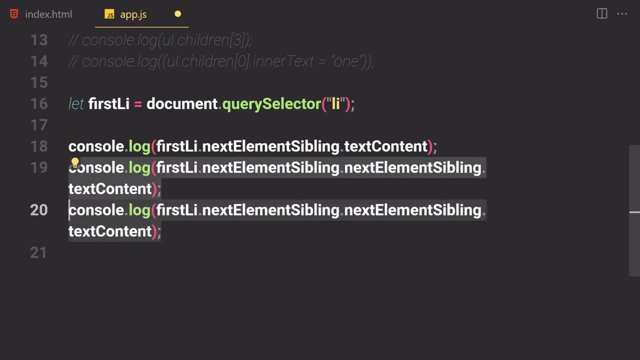 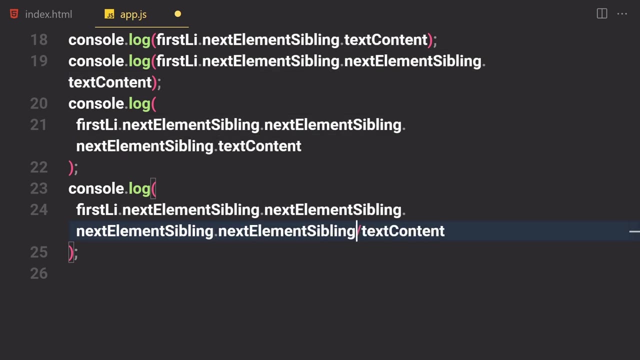 will now gives us three, and the list will go on and on and on. i wanted to show you everything, but you don't have to go like that much crazy. uh, okay, so save it. every log is four, but if you try to exit, this is one more time. uh like, so let me just write it: one more time period. 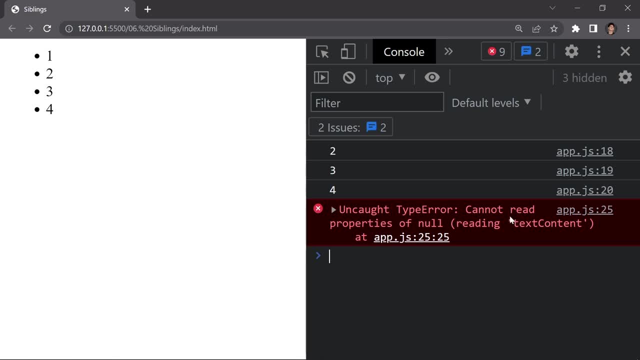 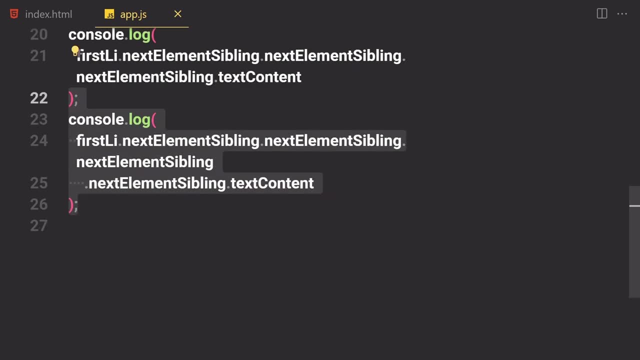 save it. it will not use uncut type. error. uh, cannot read a property of nail because this is a nail, so it will not use nail. okay, so this is how we can get all of that siblings. so i'm going to remove that final one, because this one is a little bit cluttered. so we already learned about how we can. 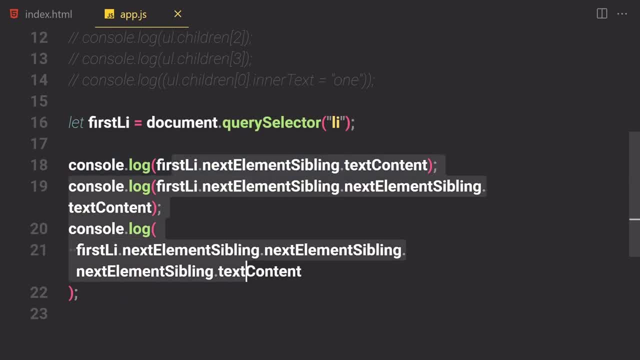 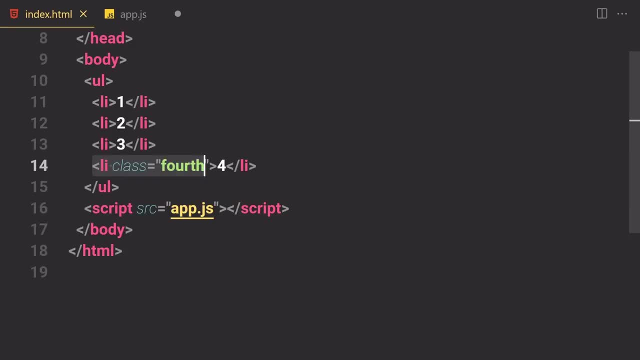 get a parent, how we can get children and how we can get a next element, sibling. so i'm going to both of these line out. uh, okay, and now let's just finally select our fourth ally, which is this one, and let's just learn about a previous elements, uh, sibling, real quick, let me just write, let. 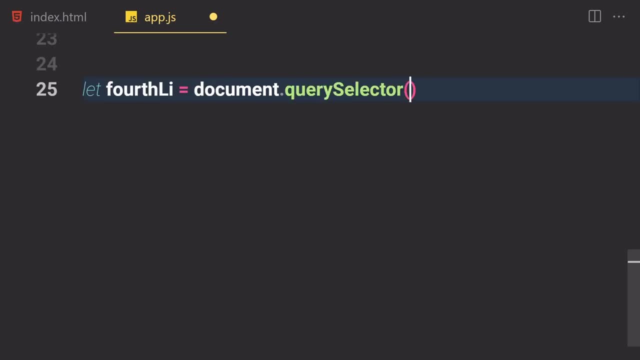 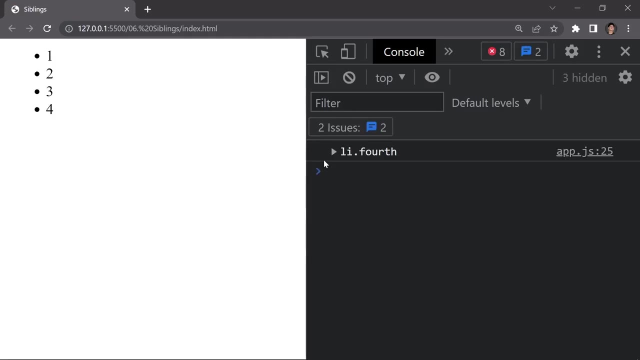 fourth ally and if you will, now you go to document that query selector of this fourth ally and i'm going to be just let's just log that to console like fourth ally. and now if you save that, and you already know that it's that fourth one, if you just write text: content of seven. 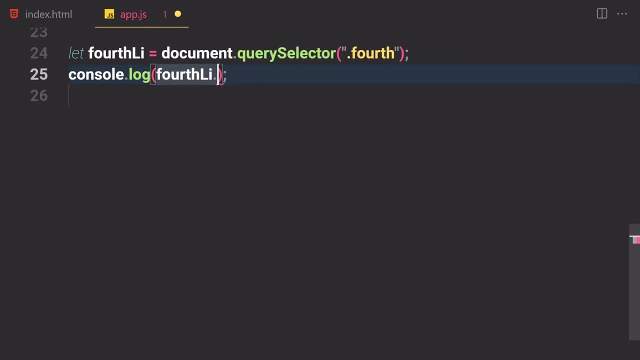 it will not give us four. okay, so if you want to just get a previous element sibling, so we can just write previous, let me just write the previous element siblings. so if you just write that and save it and it will now give us the third one, we can duplicate this line of code and we can reuse. 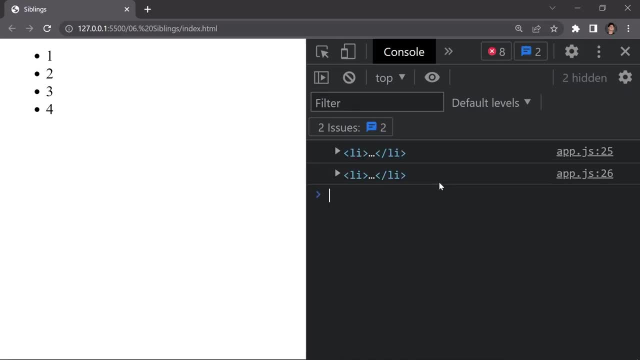 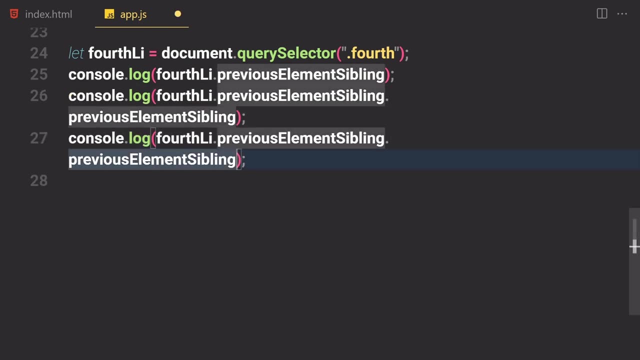 that property. copy there, pass it right here, save it. it will log users. the second one right here. we can still reuse that one more time. like this list can go on and on. if you have a lot of elements, one more time and save it. it will now give us the first one, but if we try to access the final time, 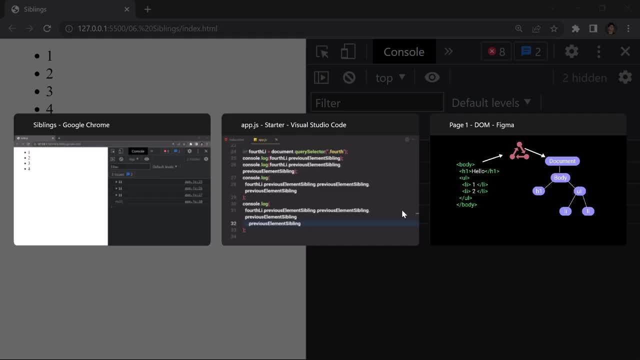 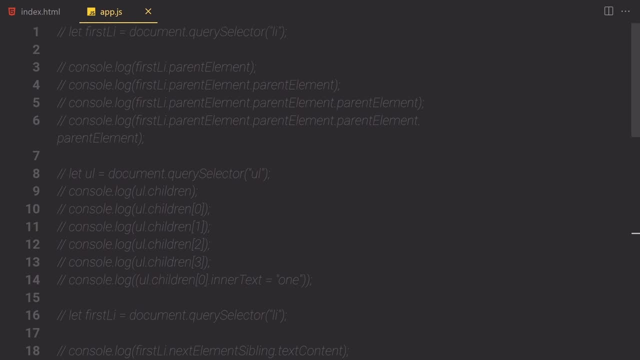 so save it and now it will now give us a nail. okay, so i know these are a lot of talking and a lot of typing and stuff, but you just have to remember that if you want to get a parent of some sort of element, so for that you just have to use a parent element property, and this list can go. 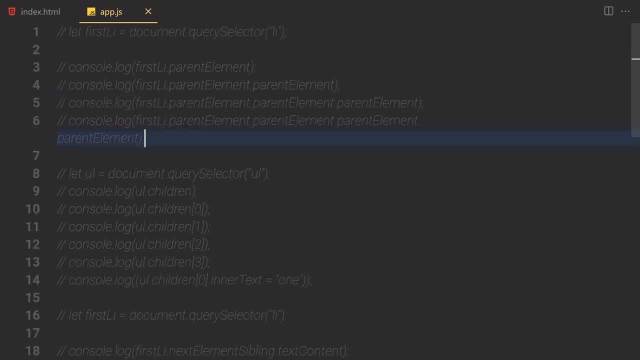 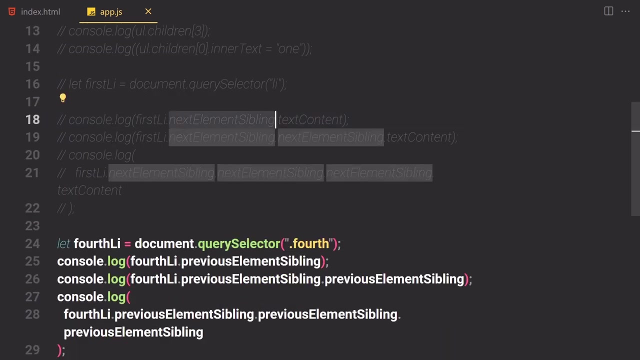 on and on, like you can go as much deep as you want, but i just kind of want to give you these examples now. if you want to get a children, so for that you have a children property. if you want to get a next element- sibling- so for that you have a next element sibling. if you want to get a previous, 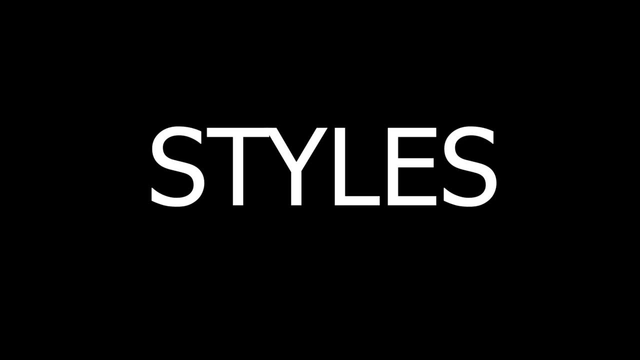 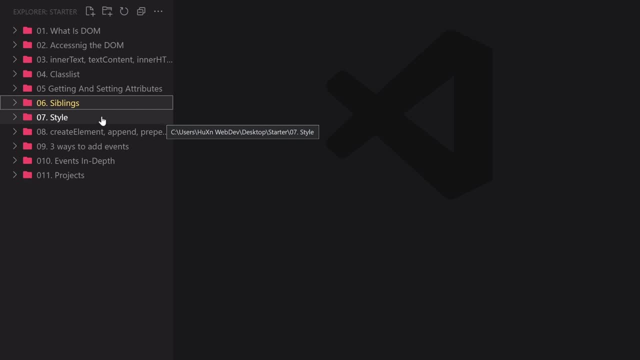 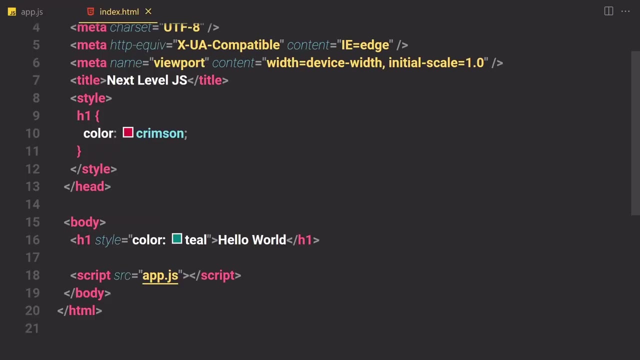 element. so for that you have a previous element, sibling property. so that was it for the siblings. now the next thing which you have to do is that we have to learn about styling, like: how can we apply styling using javascript, uh, and not css? we already learned how we can, uh, toggle classes and 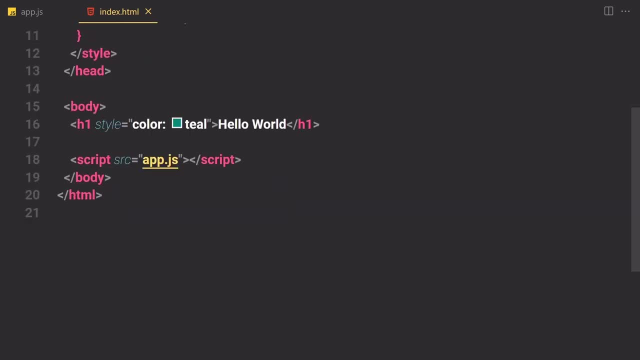 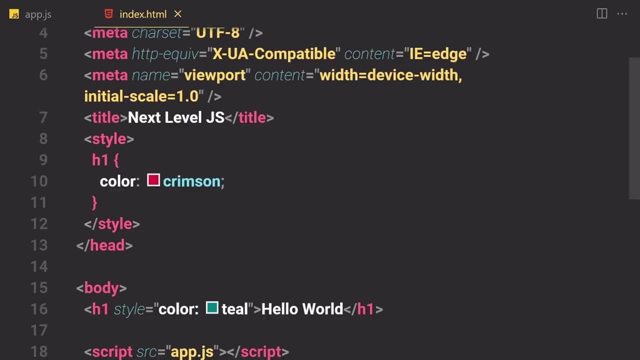 do all these things, but in this section we are going to be learning about how we can provide a styling through a specific element. i'm going to zoom in a bit, first of all, and then we have. we just have, you know, let me just launch that and you'll get to see what it is. so we have a 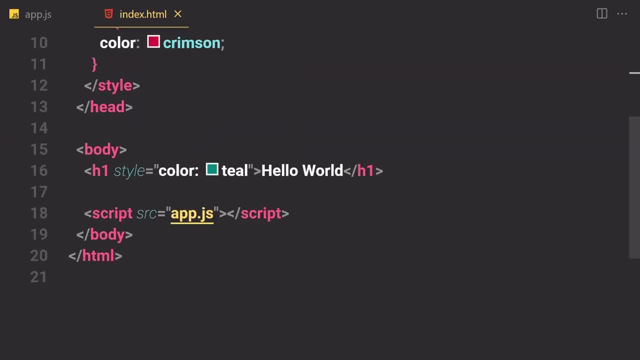 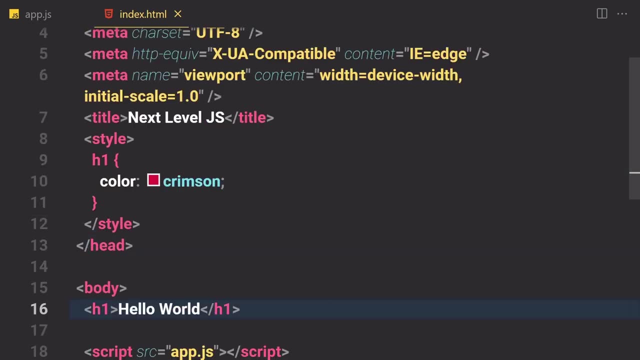 color of teal. let's just open our dev tool: zero quick. so that's because we are providing this teal class right here, so i'm going to just remove that from here and we have this hello world and it's taking the color of the styling right here. so we just selected that and we provide this style of the style. so do we want to follow this teal, to do our own design here, and we are going to add this color to this, to our own design. so we just select this error and then we are going to refresh in this section and we are going to write some new bias. 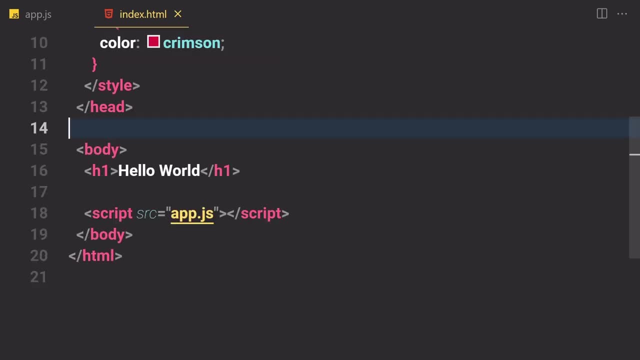 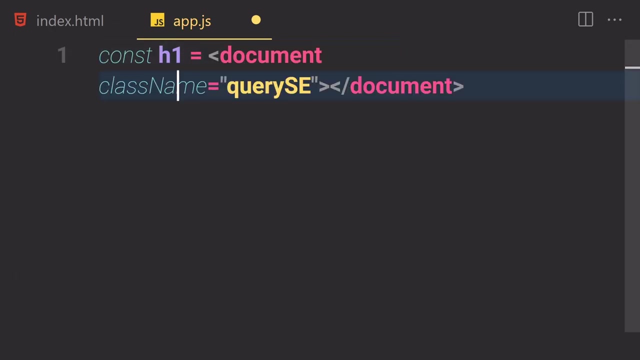 there and we provide a color of crimson right here. okay, but if you want to provide a styling using or javascript and interacting with a dom, so for that we can use just a styles property. let me just get my h1 real quick, so i'm going to write: documentqueryselector. oh my god, what is the? 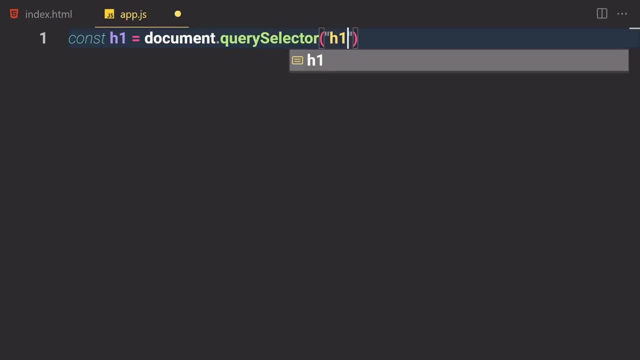 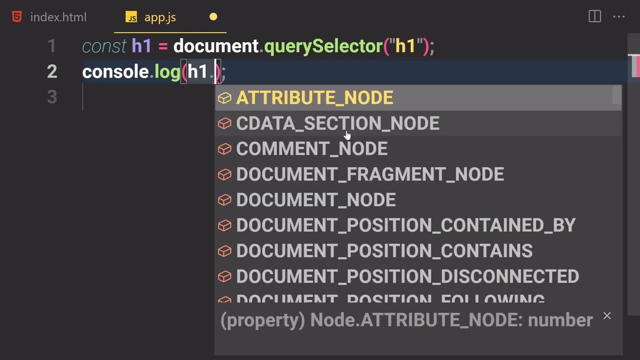 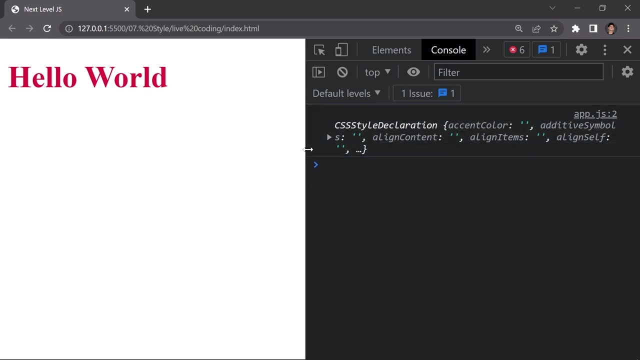 zoom in a bit and let's just select for h1. log that to the console real quick. and now, here you can see, we are now getting that h1. now let's just type dot and now let's just select what style. so if you save that and here you can see, it now gives us a css style declaration property. so if you just 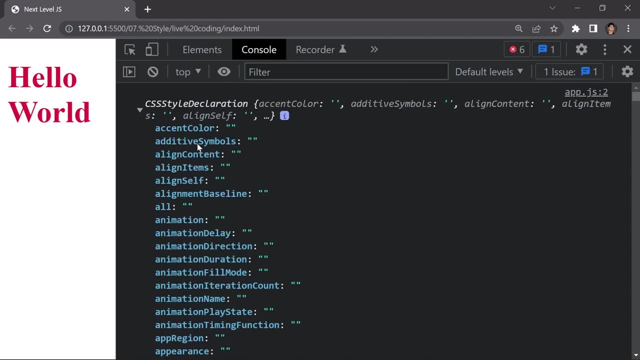 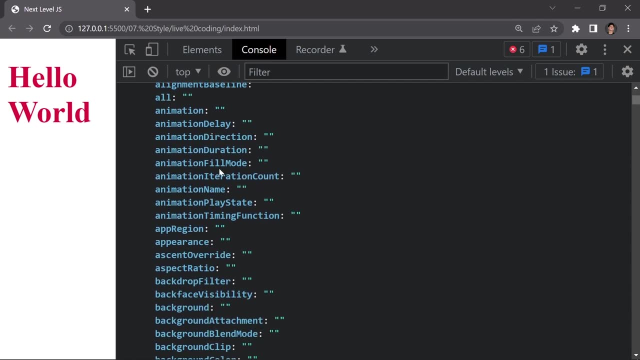 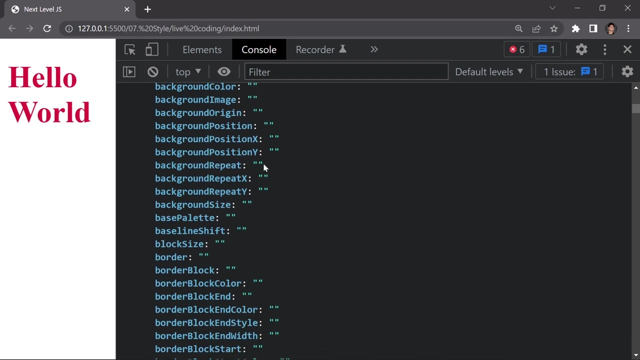 click on that and we have crazy amount of styling right here. we have uh, s and color, we have a line, current line, items a for animation, animation delay, direction, duration, film mode, iteration, count, name and all of different kinds of properties and its values to empty, because we don't provide any values to it. so let me just split there so that you 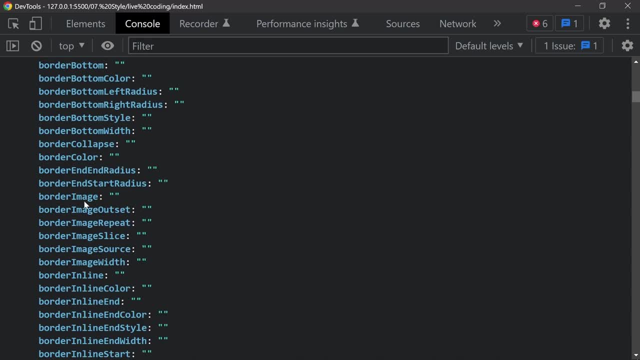 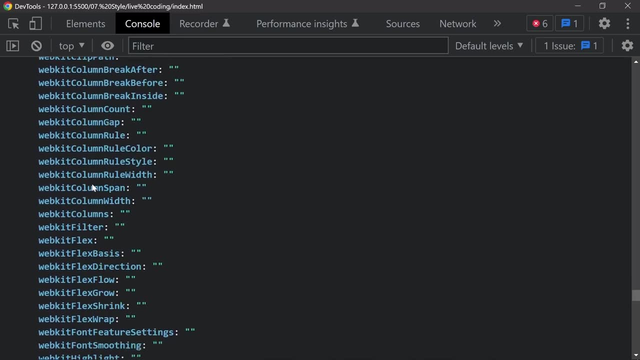 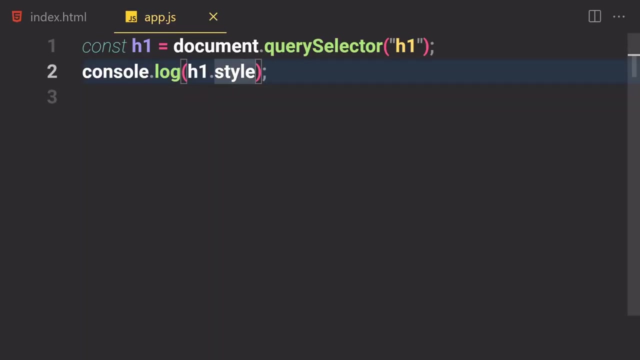 guys can see everything. so we have border, we have a background properties, we have like width and higher, the clear clip path property, columns, the display properties. so we have all of these css properties inside their style property, which we wrote right here. this one is very, very, very powerful, but my suggestion would be to do not use that. instead use. 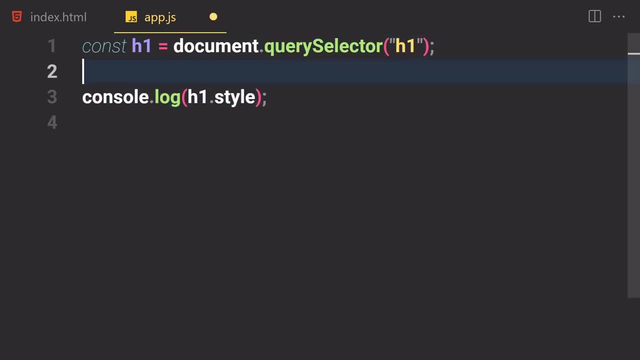 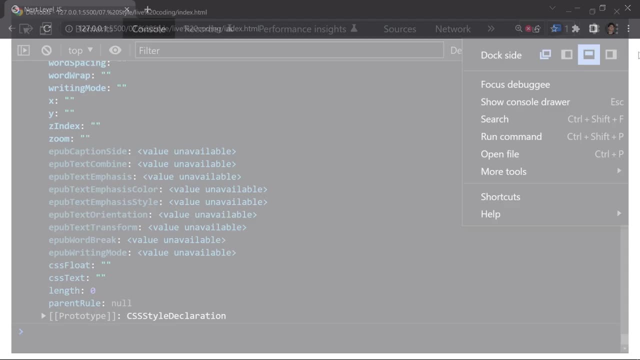 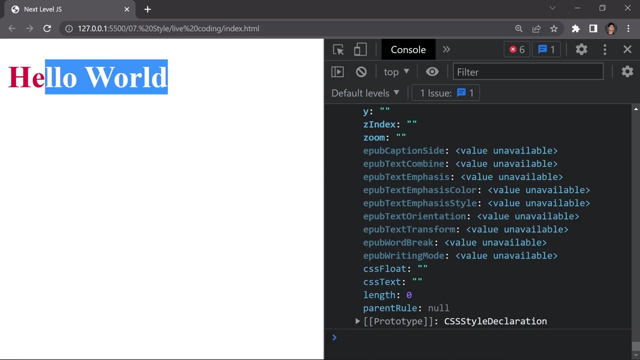 class and then toggle classes. but don't use that because it provides something called an inline style. so let's suppose, uh, the color is now changed to. let me just see the colors change to come on. oh my god, the color is changed to crimson right here. but now, if you want to change the color to be something, 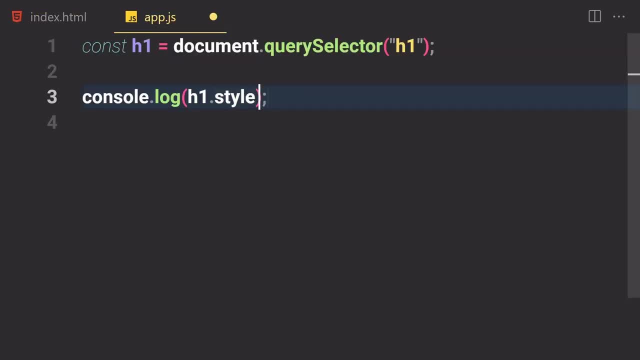 else, like maybe teal, so we can also provide that. so i'm going to just write, like you know, i'm going to remove this console log from here and write a dot, and now, let's suppose if i want to provide a color problem, so i'm going to just write color and change that to teal. and now if we save that- and it will now 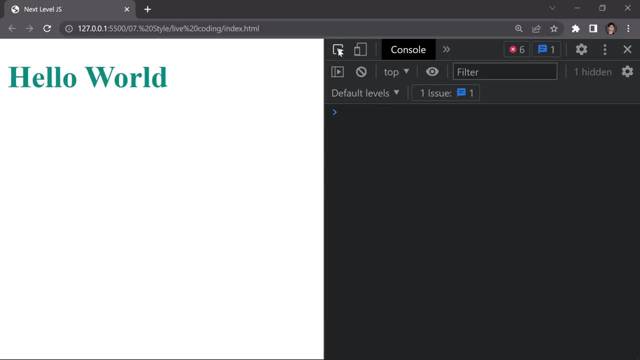 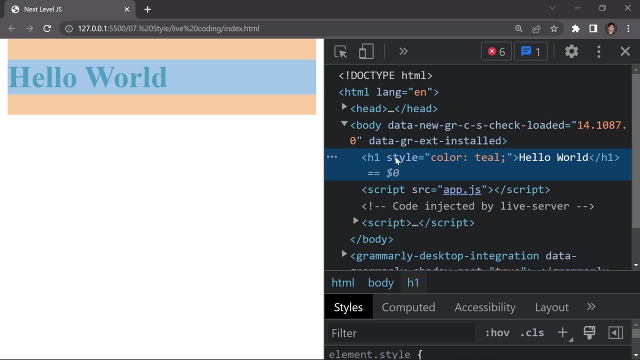 change the color to teal. so why is that? i'm going to just click on this mouse and i'm going to select that, and now, here you can see, it will not provide inline style to it. so we are now selecting and we are providing this inline style of color: teal. if you want to provide a background color. 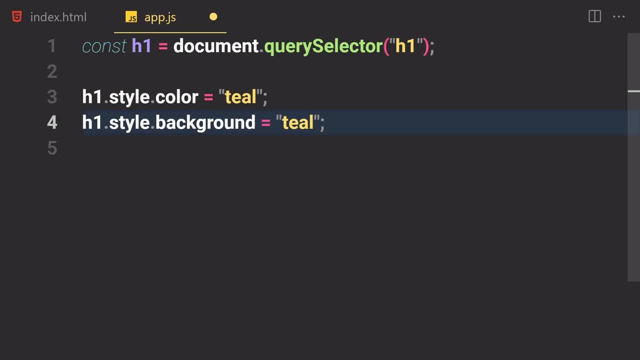 so you can just write a background background and, by the way, you are not allowed to write a css kind of styles like background dash color. it will just think it's just javascript, remember. it will just think like we have a background variable, then we have a color. 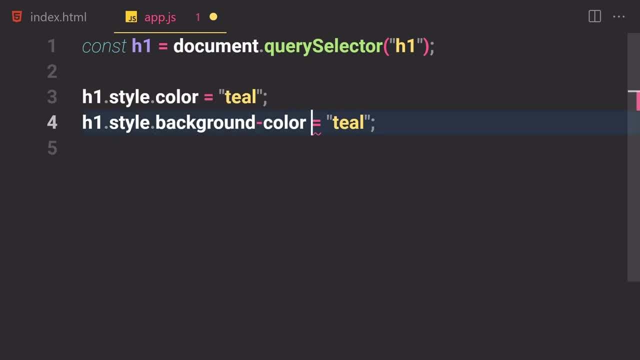 variable and we are just, uh, removing something from this color, like we are just subtracting something from a color and we are just adding that to a background. so we'll just think about that. i'm going to remove this dash and i'm going to just write a camel case right here. so background color. 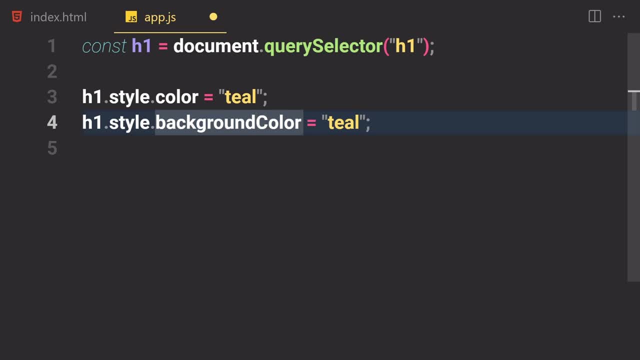 as a camel case. you can also go with- uh, no, you cannot go with a snack case, because this is a javascript and we are working on a style, so you have to write that camel case. so the background will be now, in this case, set to crimson. so if you save there, the background color will be now set. 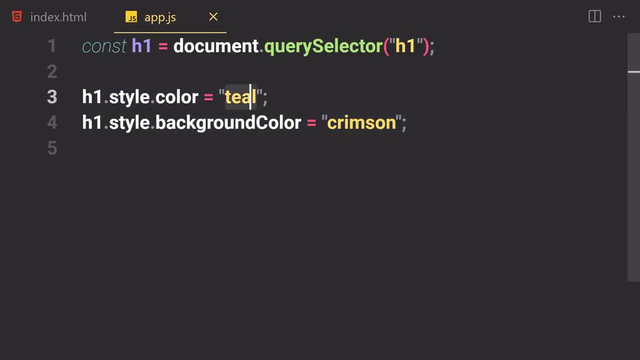 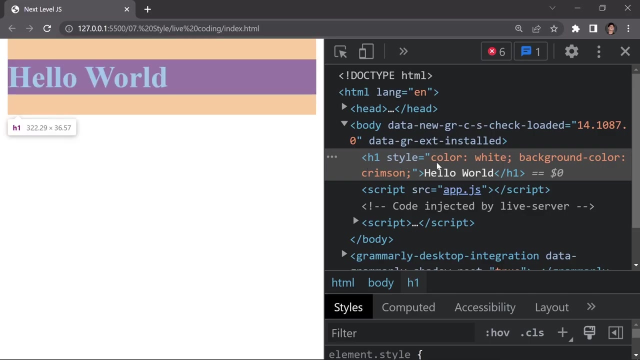 to crimson and the text color will be now set to teal. we can also change that to white, if you want to. we can provide hexadecimal values. we can do all of the css craziness by using this style property, but my suggestion will be to avoid using this style property, because it's very powerful and 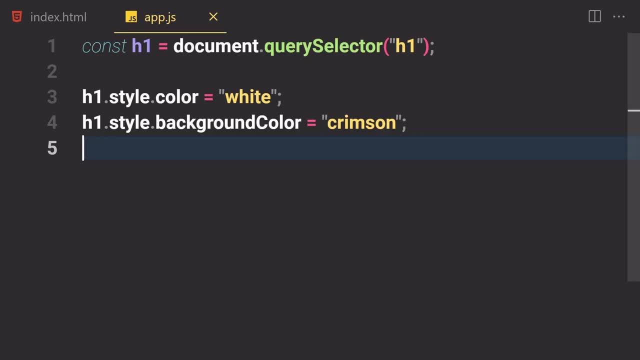 here you can see, it will provide the styling inline right here. okay, so i don't know. you can just play around with that. you know what. you can just go with that and that's it. so that's it, for you can just change that to like sky blue and this is how it looks like, and you can just provide a. 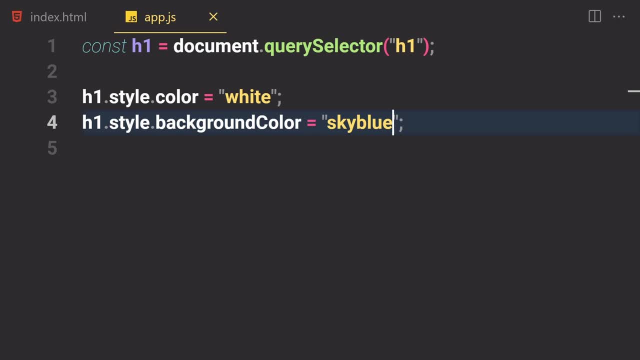 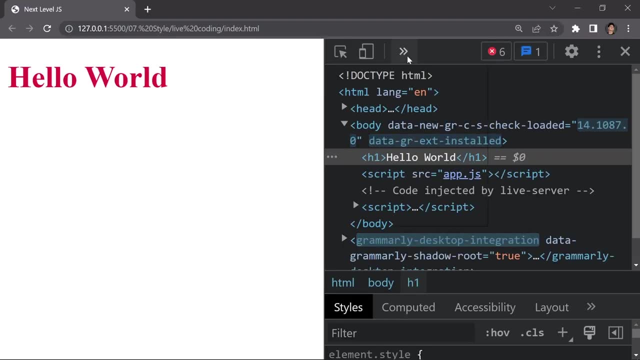 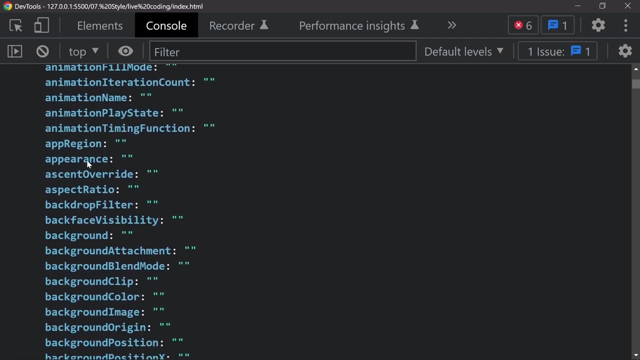 transformation, animation. you can use all of these properties which i show you. let me just show you that one more time: h1, dot, style, and let's just comment both of these properties. go to our console split there and just expand the css properties. so you can just change like whatever you like. 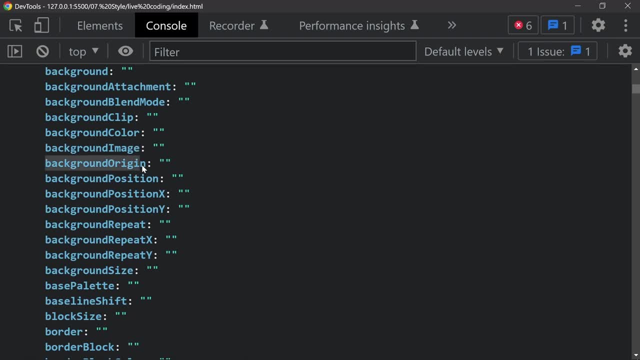 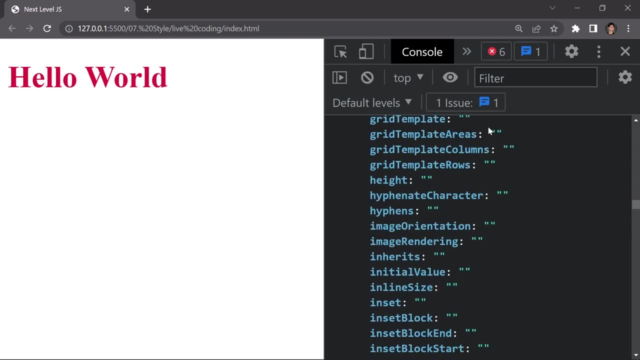 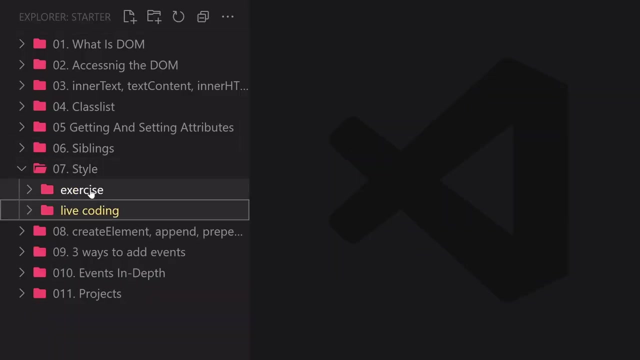 you can change the background image background or you can change the background origin. the position x is a repetition, the sizing of the background images or whatever. powerful and also very huge, like you can do whatever you want with that anyway. so enough talking, we are totally done with this styling and stuff. now let's just get into our styling. i mean like our exercise and 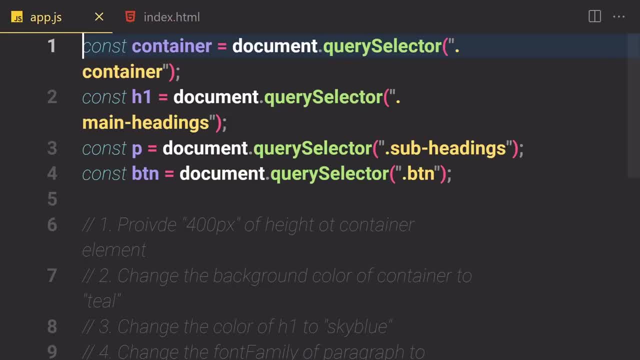 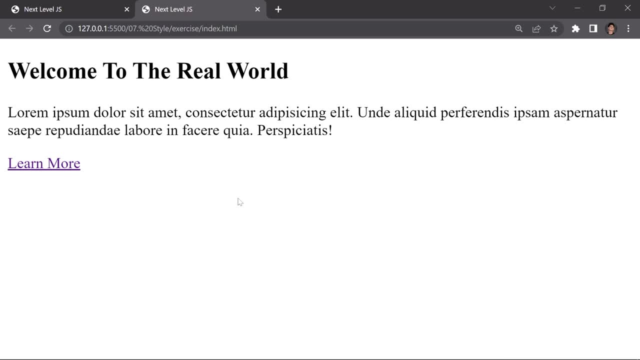 now i want you to do this exercise by yourself. uh, okay, so we do have a lot of selectors and stuff. let's just zoom out a bit and let's just see: open word console quick. oh, you know what? this is a styling tag, so you don't have to open order console for that. 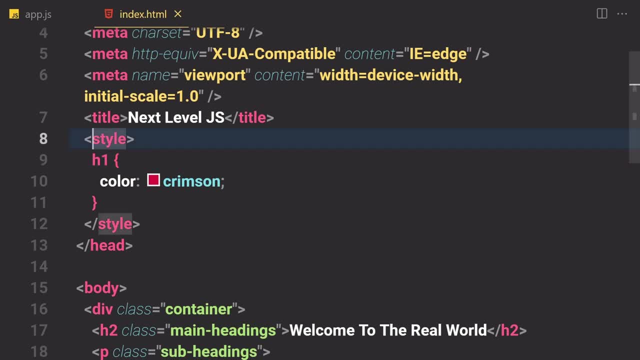 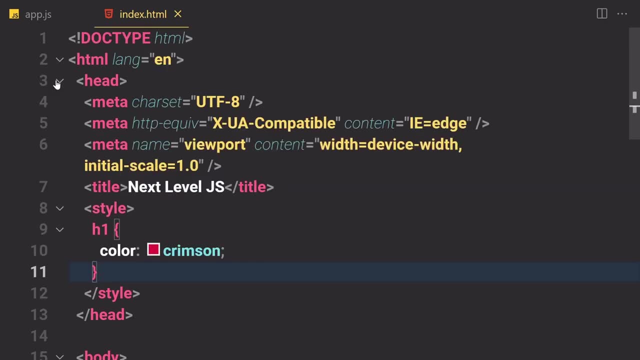 so in html we just have order, this style and we just we just have our style and we select or h1. we provide a color of crimson tiered, but i'm gonna just hide this head area from there. so inside the body we just have one container. inside this container we have a over h2 with 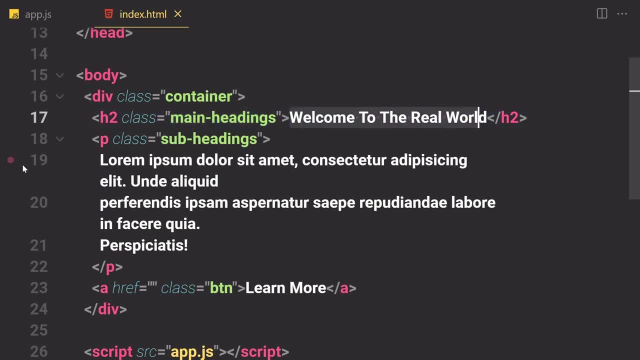 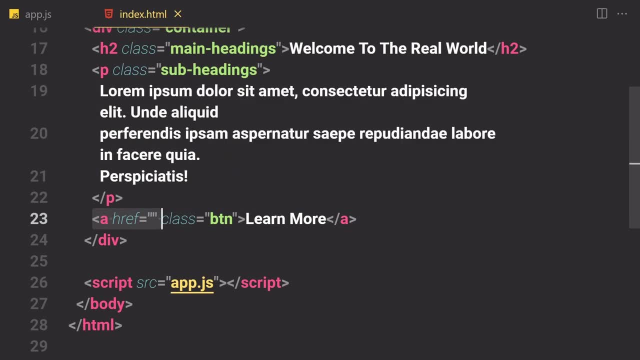 a class of main headings and we just say, like: welcome to the real world. then we have a paragraph with a class of subheading and we have a class of subheadings, and we have a class of subheadings and we have a little bit of lorem ipsum. then, finally, we have our anchor tag with the class of btn and 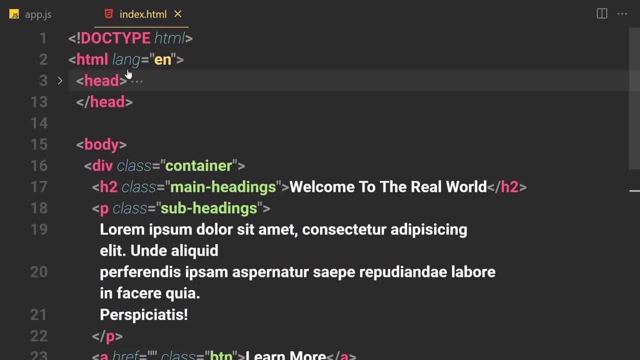 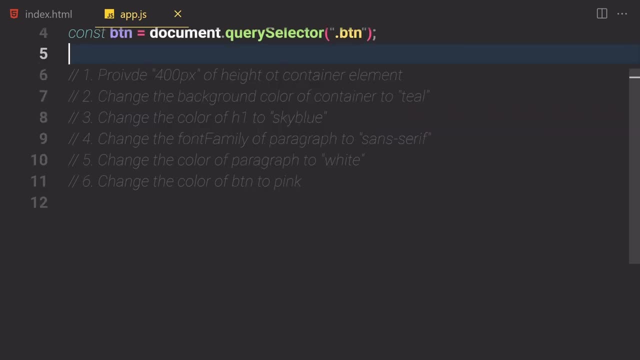 it will just say: learn more. and finally, we just add our scripts. so that's html. now, what else do we have to do? we are now selecting our container- uh, this container, right here. what else do we are doing? we are selecting h1 paragraph and also that button. so what do we have to do is a challenge. 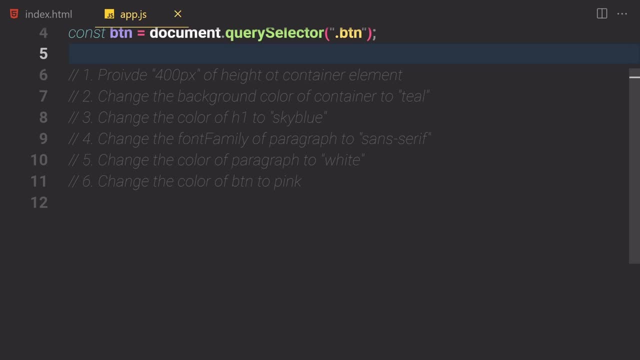 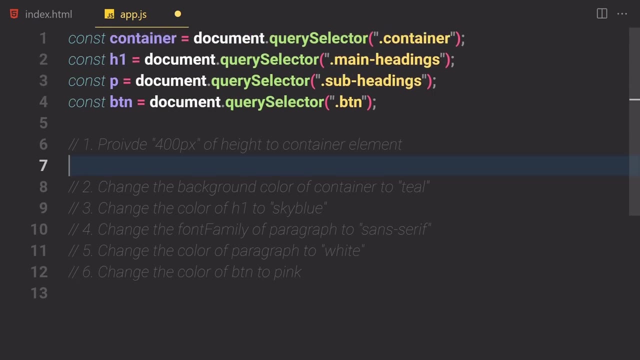 provide 400 pixel of height. what do? container element? so that's the first thing. we already select our container element right there. so provide a 400 pixel height to it. i'm going to just select first of all my container. i'm going to use style and then height. come on, not get element. 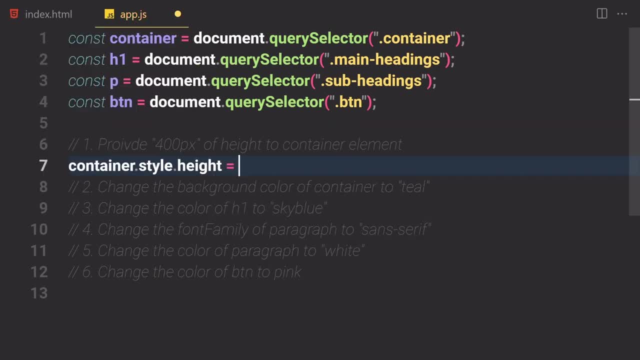 whatever but style, and i'm going to just provide a height to 400 pixels, so it will be on quotes, and now, if you save that, we cannot still see something because we don't have any background colors. all right, so what else do we have to do? change the background color of the. 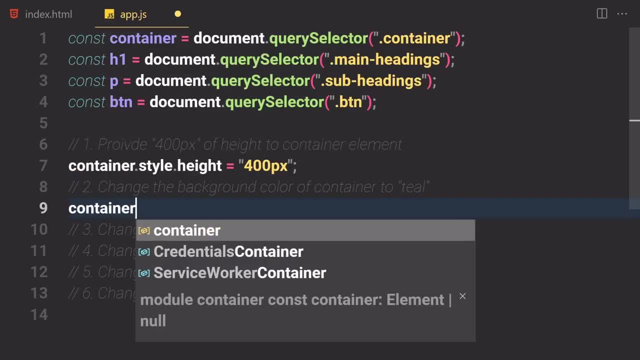 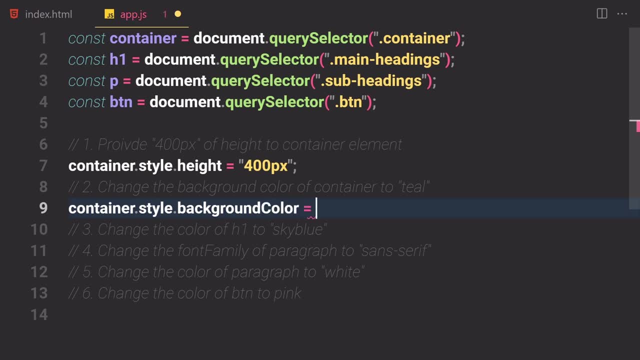 container to teal. let's just do that baby container dot style, dot background, and we can also just write a background color. but yeah, background color would be fine. we can go to just background if you want to, and now it will be set to teal and voila, we are now getting that. so then we have a 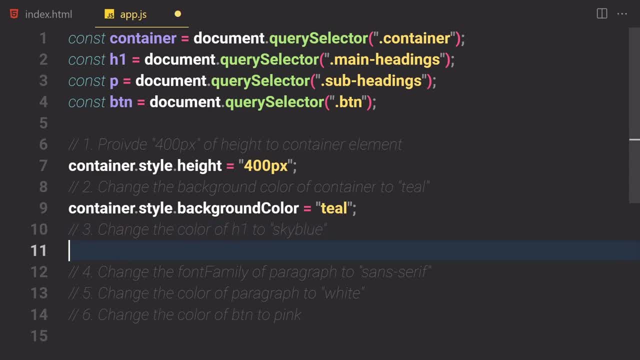 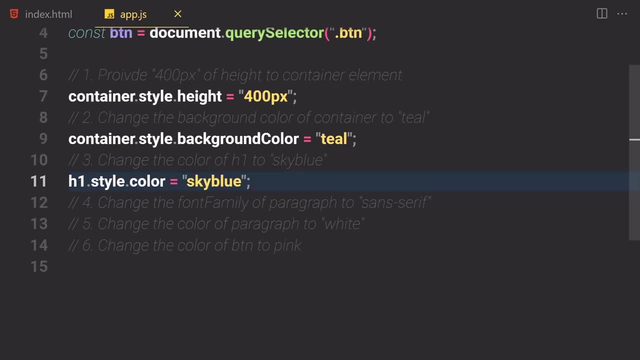 change the color of h1 to sky blue. so we already select that h1 right here. so let's just write h1 dot. style dot. what? what should we have to do? uh, to sky blue. so color will be now set to sky blue. and now, if you save that, it will now just change this text to sky blue. what else do we have? 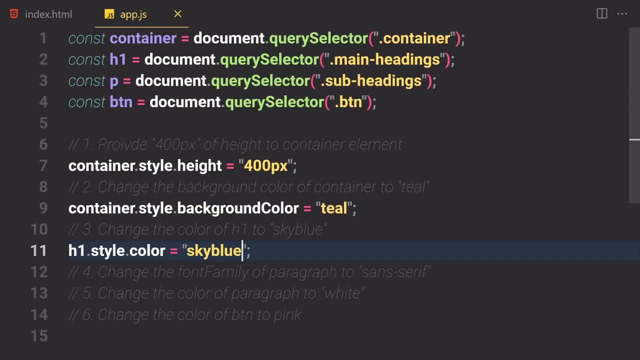 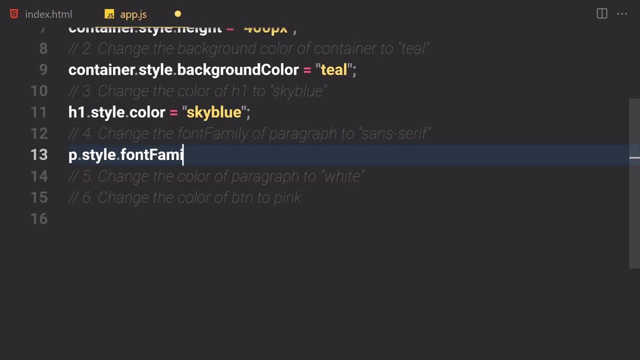 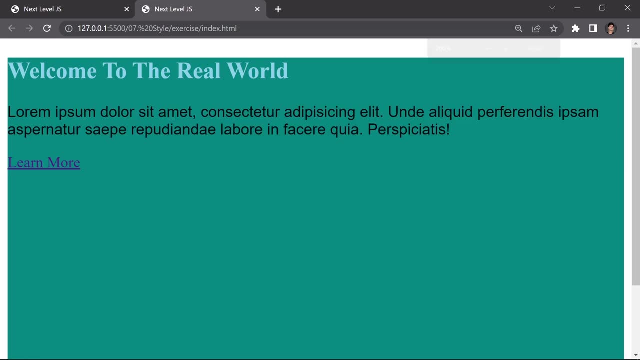 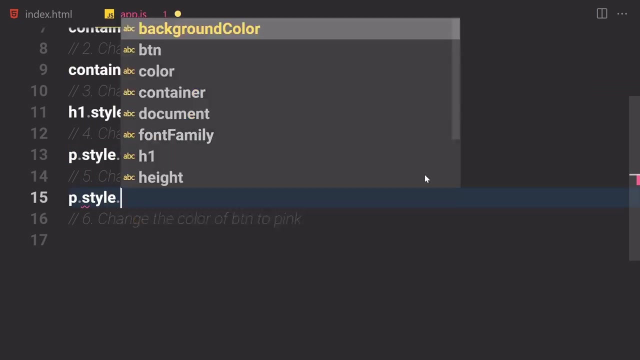 to do? change the font family of the paragraph to sense serif. so we already select that paragraph and let's just write paragraph dot: what style dot? font family to sense serif. save it and we'll now just change that to sense serif. it will remove that serif from this font. all right, so change the color of the paragraph to white. let's just do the p dot style. 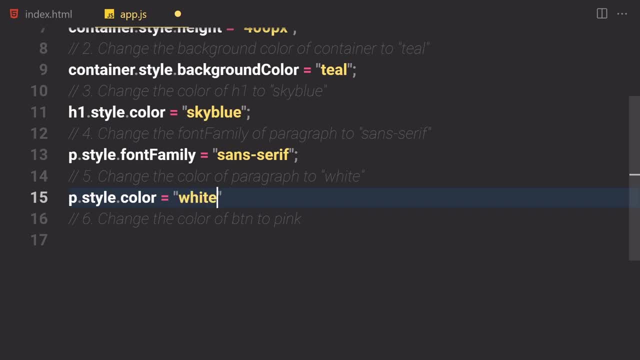 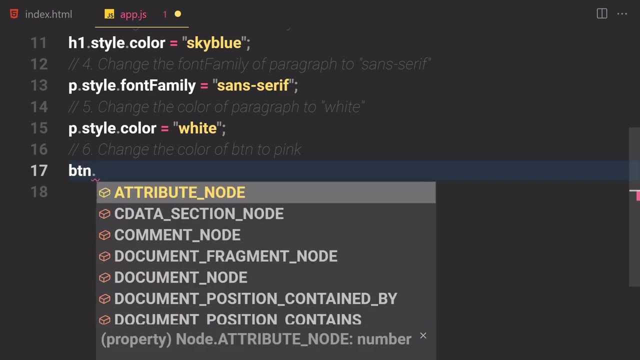 dot color and it will now set to totally white. save it and the color is now totally set to white and change the color of the button to pink. so let's just select- we already select that button right here. so btn that, uh, change the color of the btn to pink so that style dot color to totally. 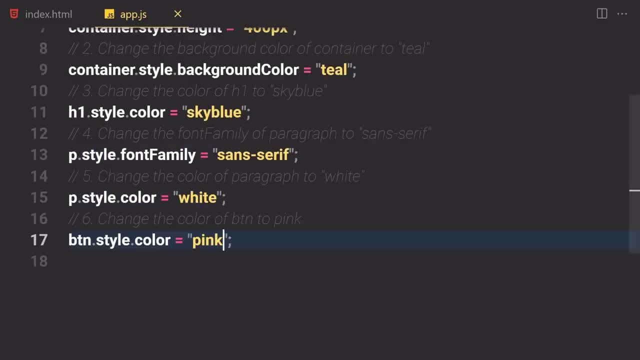 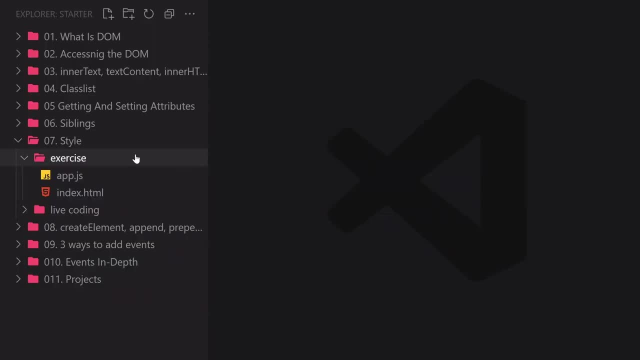 pink. so we have a little bit of awful styling right here, but guess what that's it? and we are totally done with our challenge, all right, so we now tackle this challenge. we learn about styling, and now let's just learn about a complicated topic called create element, append element. 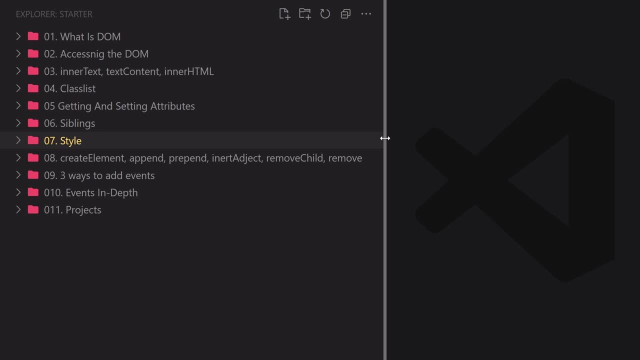 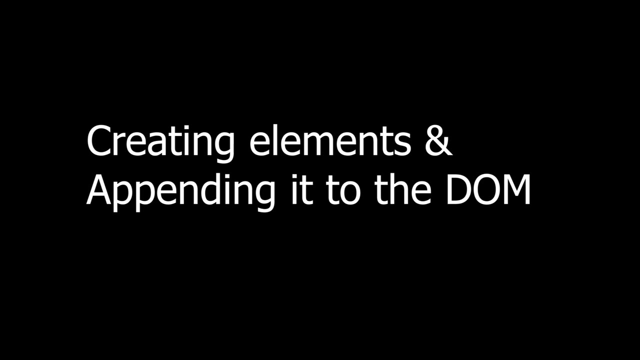 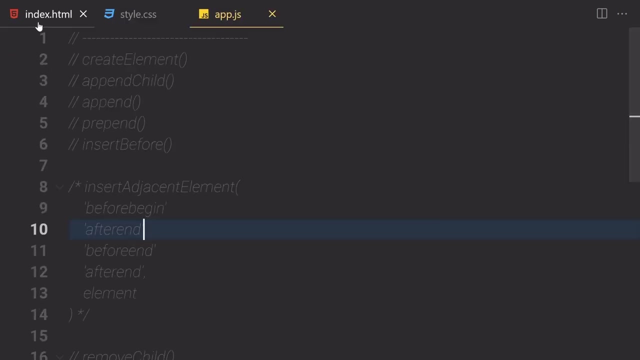 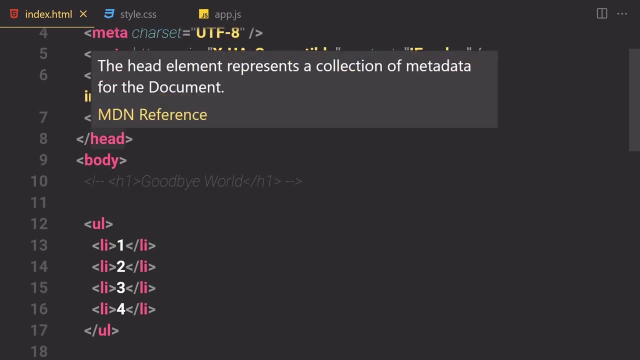 prepend element, insert adjacent, remove child and remove. these are a lot of methods we have inside word dom. i'm going to open my index dot html file, style dot css file and appjs file. so we don't have anything inside any of them. and inside this h, inside this h, inside this html file, we just have our basic stuff. i'm going to 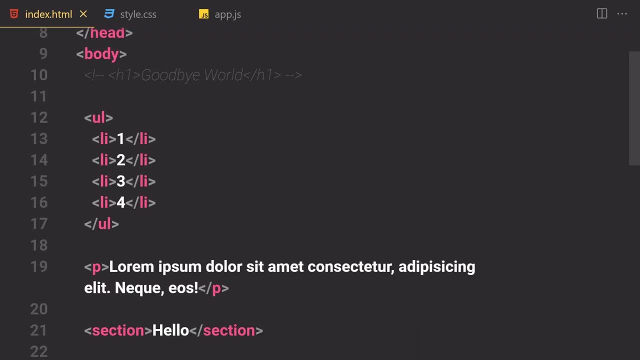 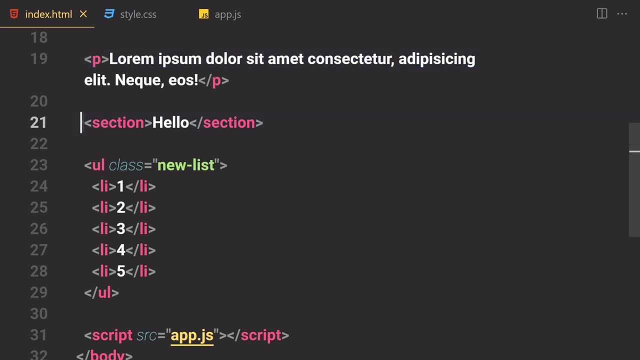 comment or you know, i'm going to collapse this head area. we have a ul. inside this ul we have a four allies. then we have a paragraph with a little bit of lorem ipsum in there, then we have a section, then we have a new list and then we have a little bit of allies inside. 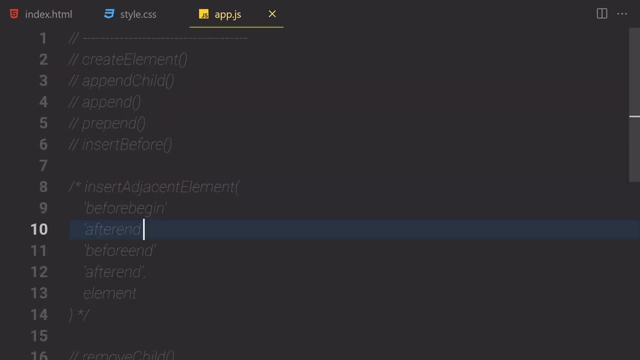 there, all right, so let's get into that. so in javascript, we just have a little bit of comments. so the first thing which you are going to be learning in this section is how to create element and how to use this create element method. then we are going to be learning about how we can. 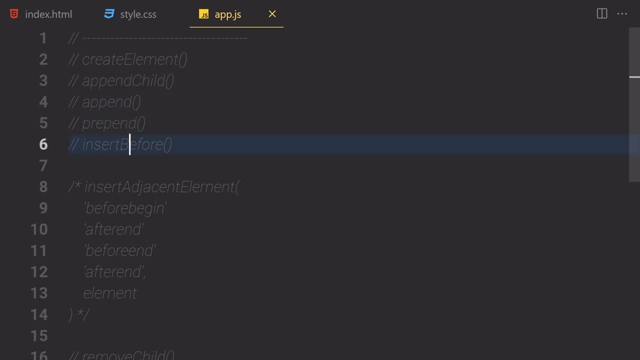 use this append child, append method, prepend, insert before insert element, insert adjacent element, remove child and remove. okay, so we are going to be learning these methods in this section. so, starting from the first thing, which is that create element, so if you want to create element using javascript, so first of all we are going to be writing our comments. 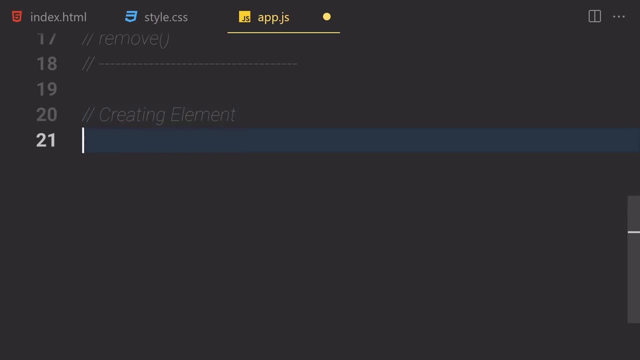 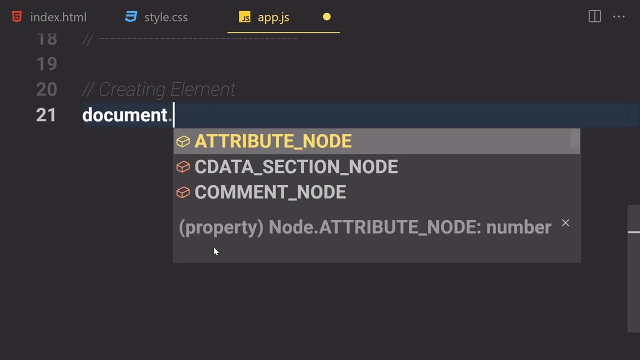 for yourself, like creating elements, or element to be precise, just a singular. so suppose, if you want to create a element, so first of all you are going to be writing a document and then you have a method called create element. it's self-explanatory. so if you want to create anchor tag, you can just 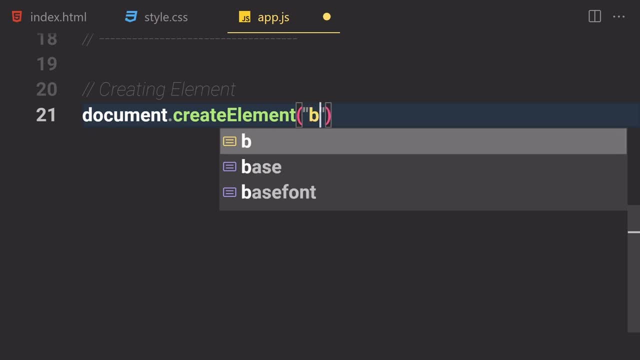 provide anchor tag if you want to create like bold tag, so you can just provide b. if you want to create h1, so you can just provide h1, and you can just provide section uh if you want to. you can provide article if you want to, but in my case i'm going to. 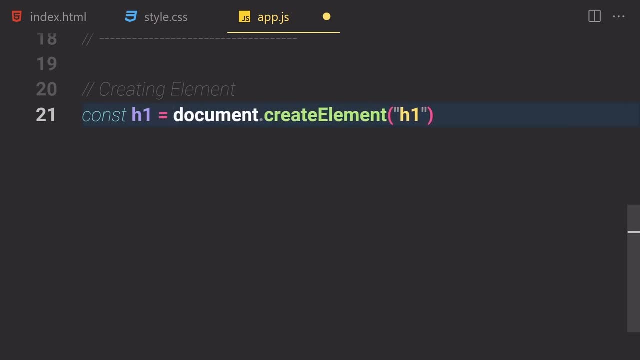 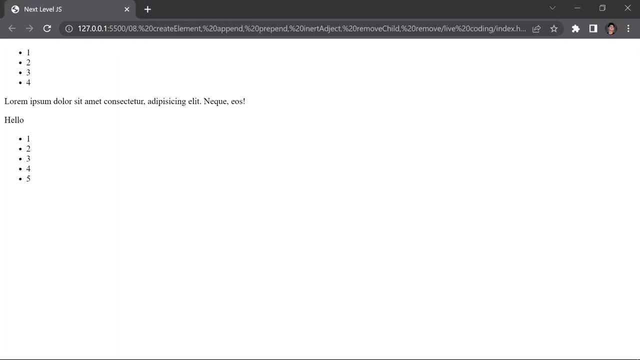 just write h1 in it and i want to store that in some sort of a variable like h1, so now we successfully create or h1. so now if you log there to the console consolelog, h1. and now if you save there and we have to launch this indexhtml file like so, save a byte to the other one, open. 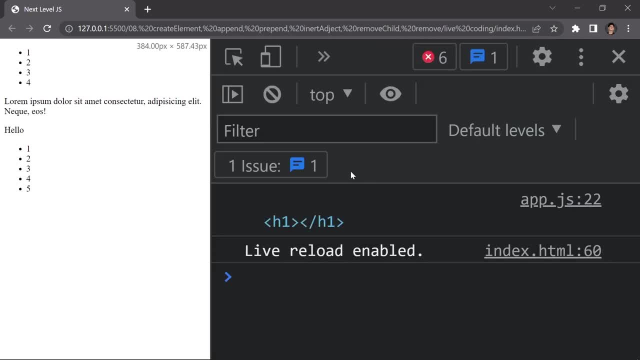 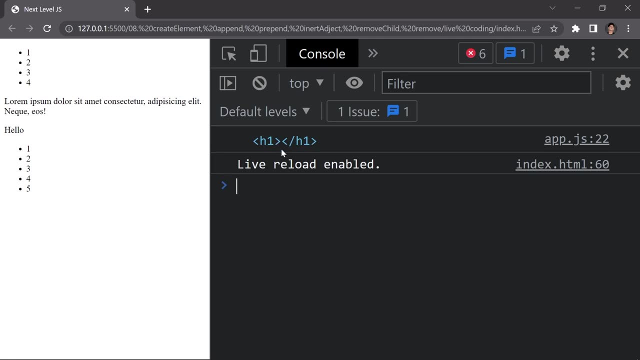 or console right here, all right. so now, here you can see, we just have our empty h1 right here. we don't have any classes, we don't have any ids, we don't have any content inside this h1 right here. okay, so basic h1, all right. so now we successfully create our h1. so 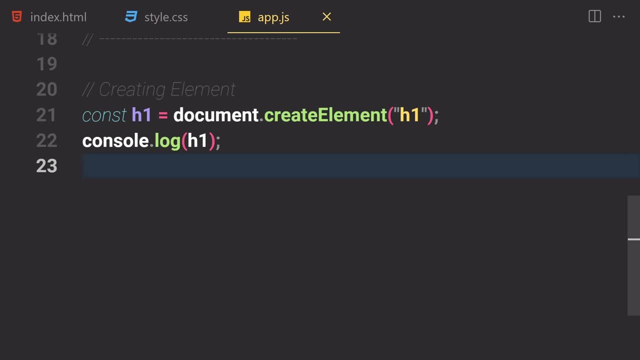 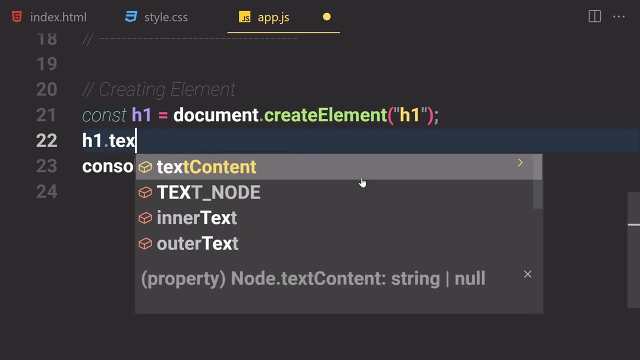 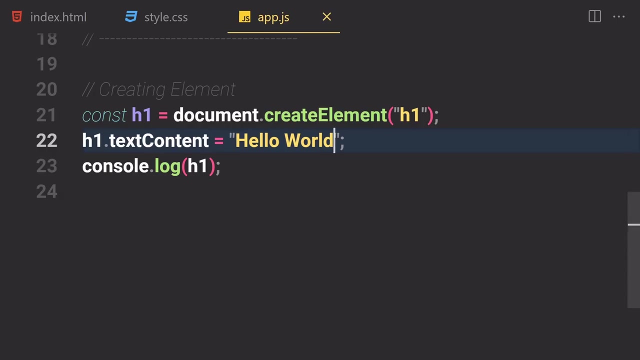 what else do we have to do now if you want to, uh, add content to this h1? so we already learned how we can add content to our elements. so for that we have h1.text content property and we can just provide like hello world. and now, if you save that and let's just check that text content, 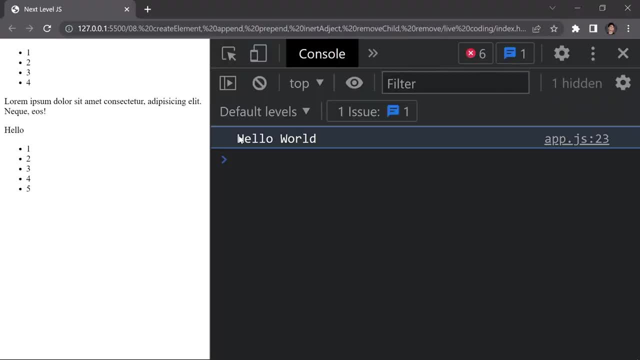 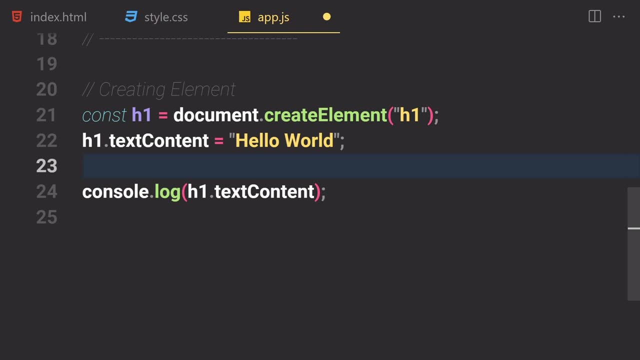 property like text content and now, if you save that, it will now gives us that text content right here. okay, so we can also provide classes to it, if you want to. we already learned how we can provide classes to it, so you can just write h1.classlistadd and we can just provide different kind. 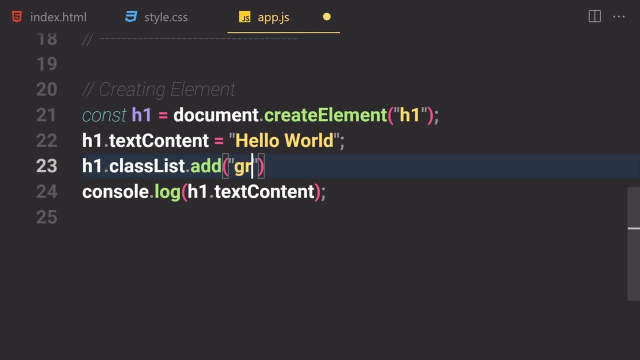 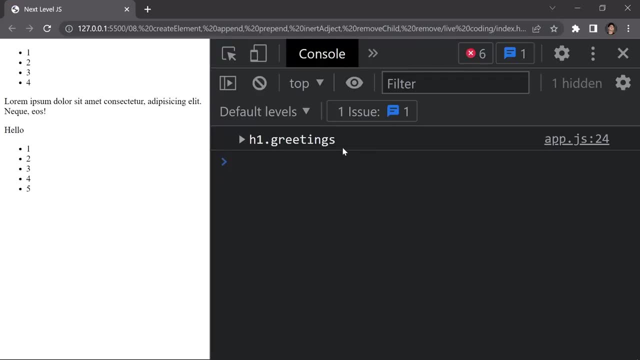 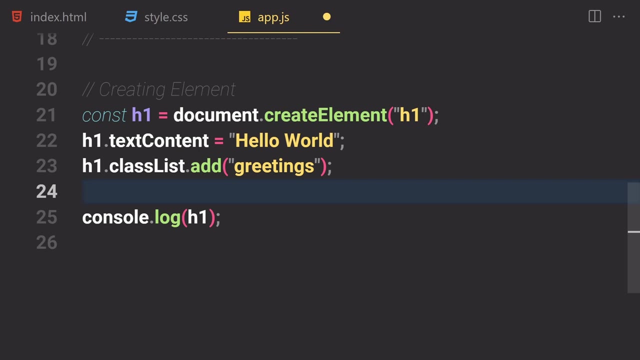 of classes to it, like i don't know. greetings would be fine, so greetings. so if you say over there let's just remove that text content and here you can see we have h1 with the class of greetings right here, and we can also do styling if you want to. so you can just write h1, but we cannot see the styling. 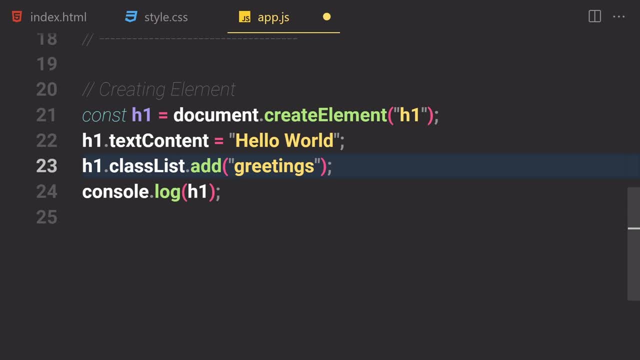 because we didn't append there to our dom. so this is it about: how we can create our element, how we can add text to our element, how we can attach classes to our element, how we can remove even clauses from our element, like just write, remove class, if you want to. so now the next method, which 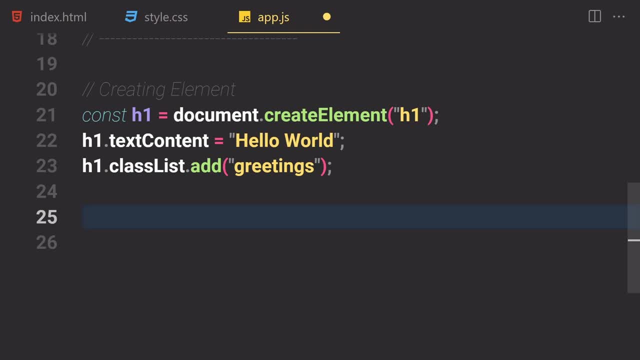 you are going to be learning about is append child method, and append child will just append, or whatever text we have or whatever thing we have, it will append it at the end of the list. so let me just select first of all the body. i'm going to just write const body and it will be now set to. 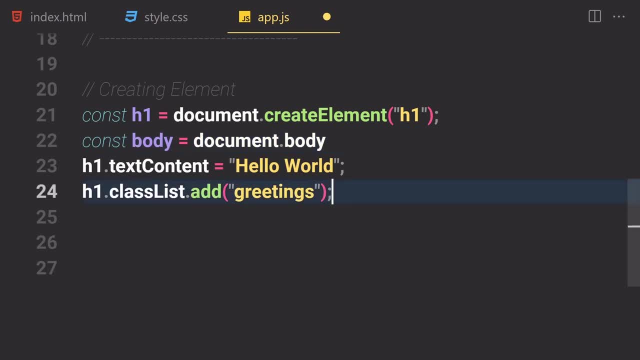 documentbody. so now we successfully select our body, now we create our element, we provide text to our element, we provide class to our element, but we don't have that element inside our body. so if you want to push that element, that newly created element, to this body, so for that we can. 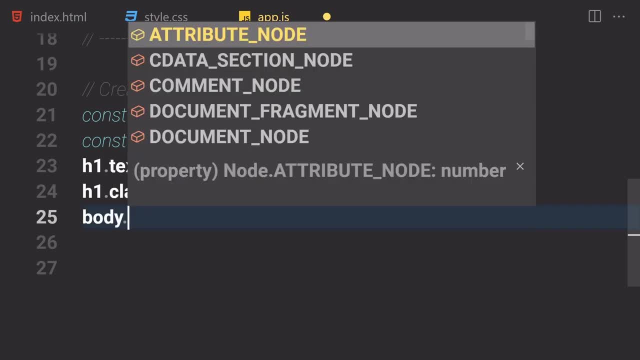 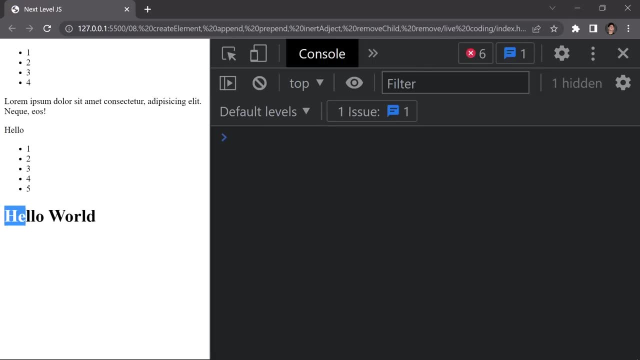 just use append, child. so i'm going to just write body dot element. so i'm going to just write body dot, append and then child. okay, so i'm going to just set that h1. so if you save that and here you can see, it will not use that hello world right here, but it will be at the end of this body, it will be. 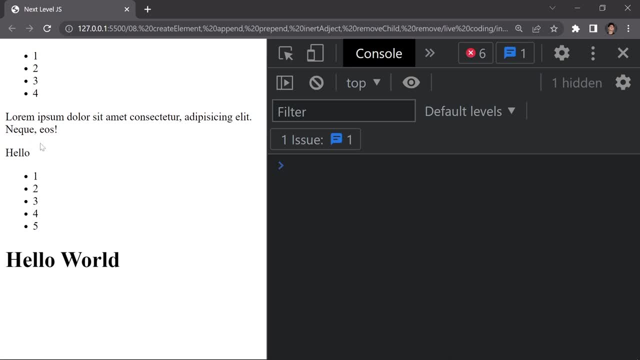 not, it will not be at the top, it will not be at the center, it will not be anywhere in here, but it will be at the bottom because, as the name suggests, that it will just append or element at the bottom of the list. so what is the bottom of the list? the bottom of the list is that 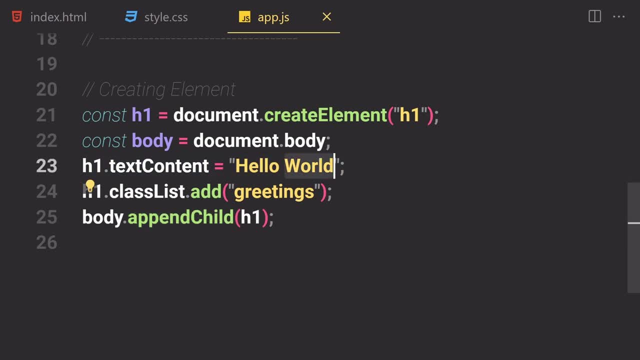 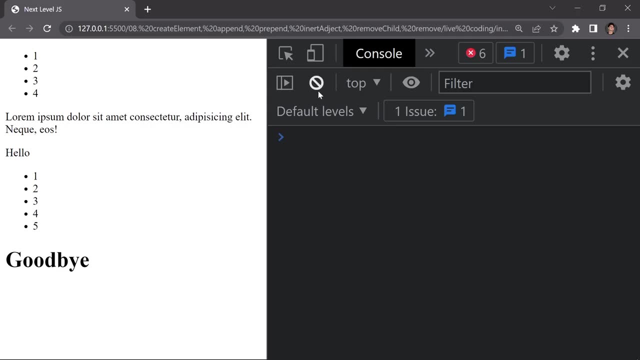 the final area right here, so it will just push it right here if you change the text to be like: uh, goodbye. so if you save that, it will now change the text to goodbye. and also, let's just make sure that we provide a classes to it. let's just click on it. 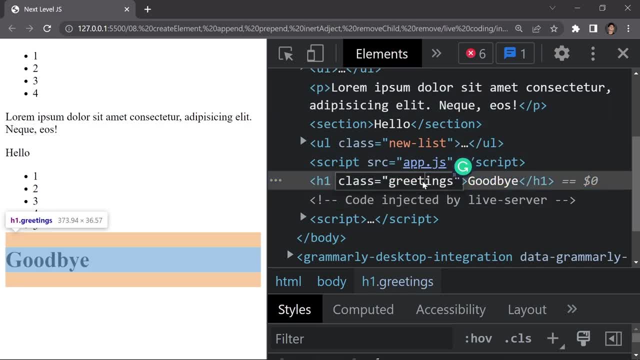 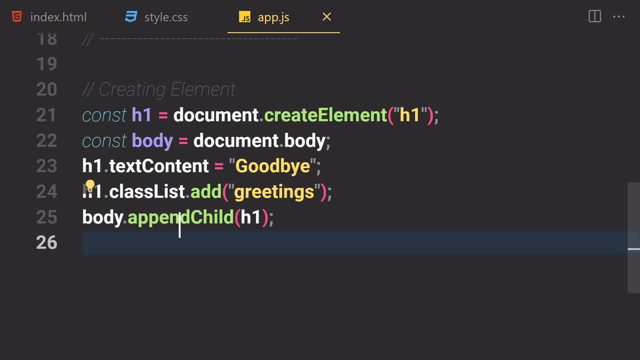 so here you can see, we are now getting this greetings- greetings class right here. okay, so everything is working the way we expect him to work. so this is how we can create our element and this is how we can append it to somewhere, so we can, like, append it to our ul and allies and all. 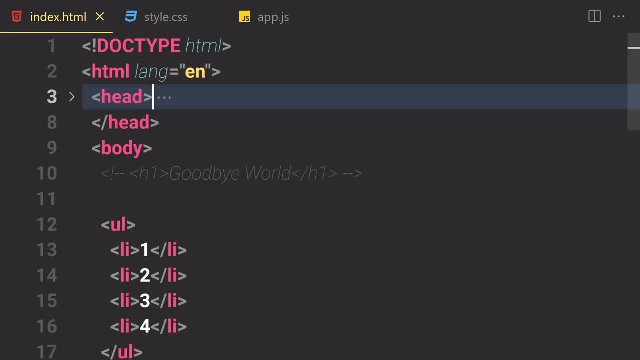 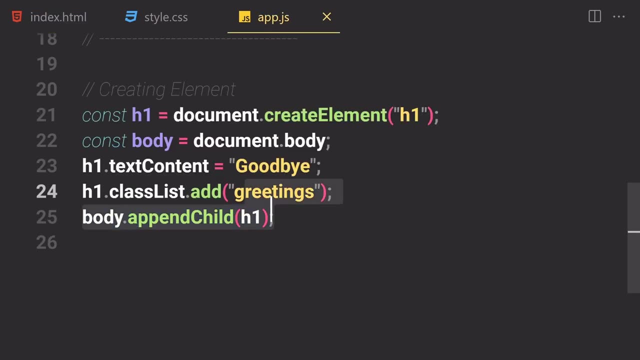 of that kind of good stuff which we learned. so you can just select, like this ul, and you can append it right here at the end of this. uh, allies, right there. so now let's just do that. you know what i'm going to comment all of this coding from now and i'm going to just 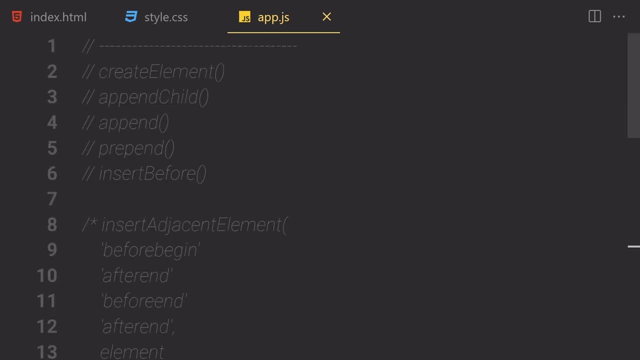 make a separator for ourselves. all right, so now that we learned about create element method and append child method, but now, in this case, we are going to be learning about insert before and then append, prepare and insert before and stuff like that. all right, so first of all, we 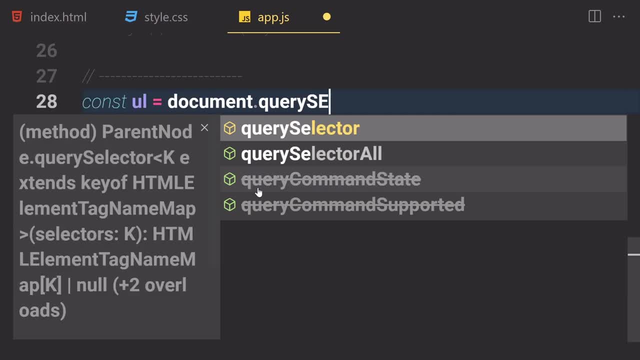 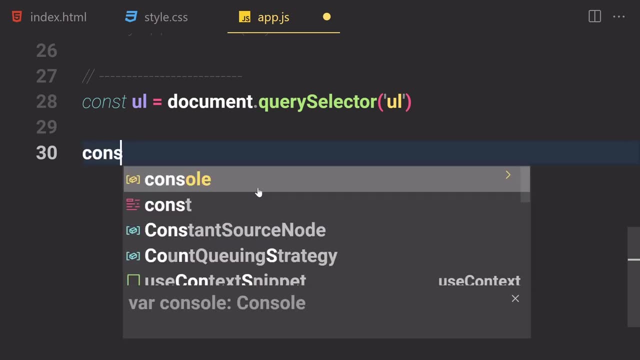 have to select or ul. so i'm going to just start: document dot- query- selector of the documentquery, this ul. okay, so now let's just create our new items. so new, oh you know what? let me just give a name of like new li, and it will be now set to document dot- create elements. so we want to create. 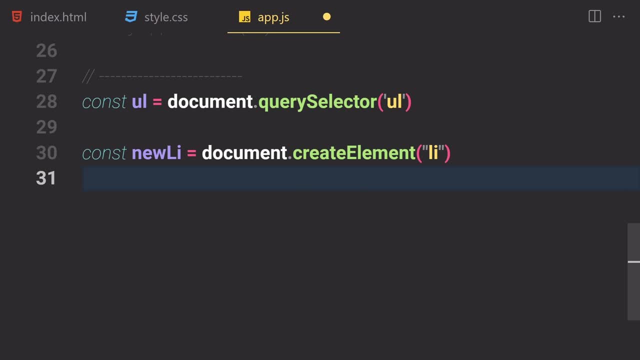 an element. we have to just provide li right here. okay, so we want to create an ally, so that's why we provide li. now let's just provide a text to it. so dot inner uh text to it. it will be now set to: i am li tag. okay, and now let's just append that to ul. so we already learned, like, how we can append. 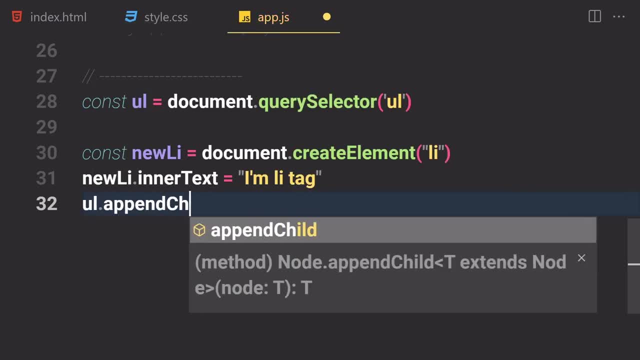 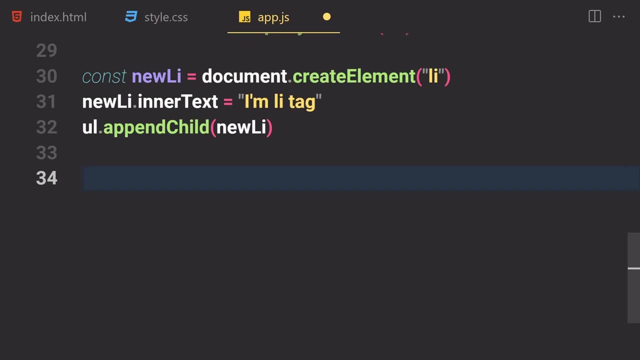 that ul so you can just use like ulappend child. this is kind of a review, so new li. so now we successfully append that to ul. okay, so now let's just get our first li. so const, first li and it will now equals to document that query selector. and we want to just select our first li, which is: 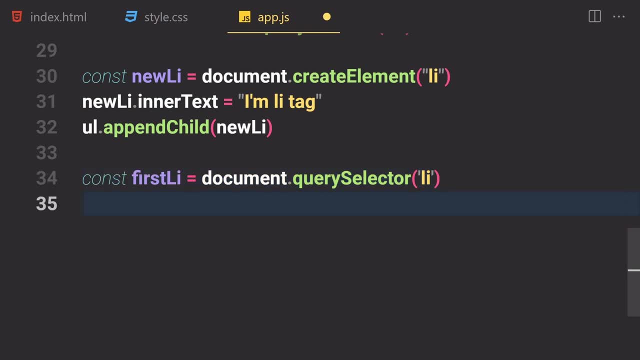 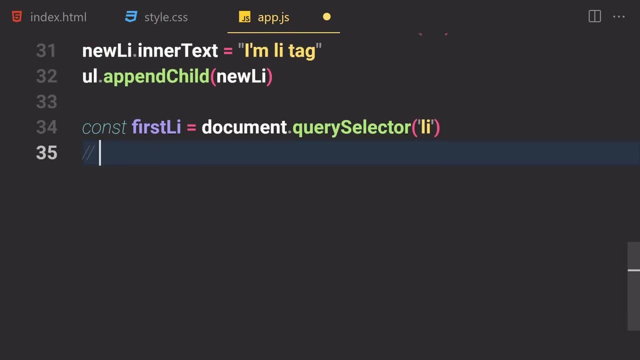 this one, okay, and now let's just learn about our. you insert before. it's kind of a weird one. so insert before method is a little bit weird one. you have to remember that. so first of all we have a selector, then we have insert before method on. 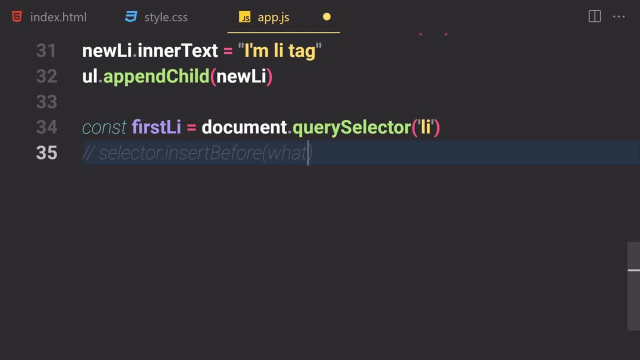 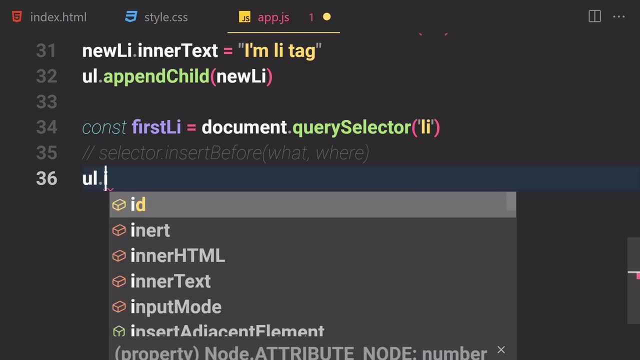 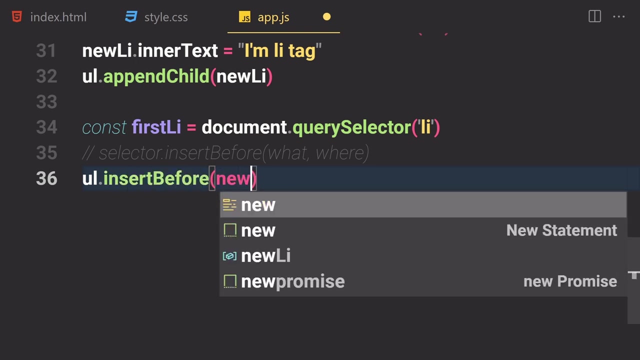 there. so it will just take two parameter, like what do you want to insert and then where do you want to insert it. so let me just show you that you know. so now let me just write ul and then insert uh. insert before and we want to provide uh, so we want to provide new. 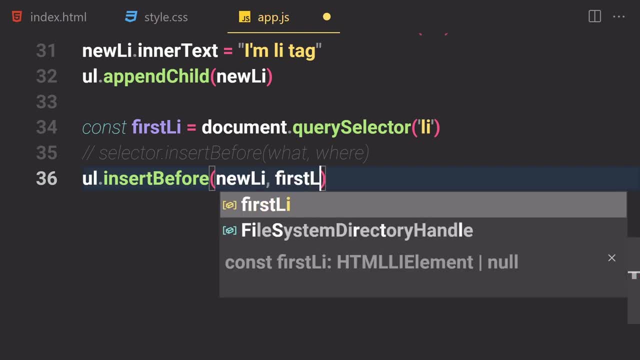 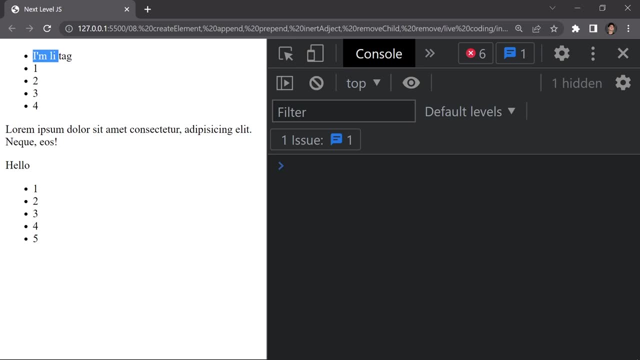 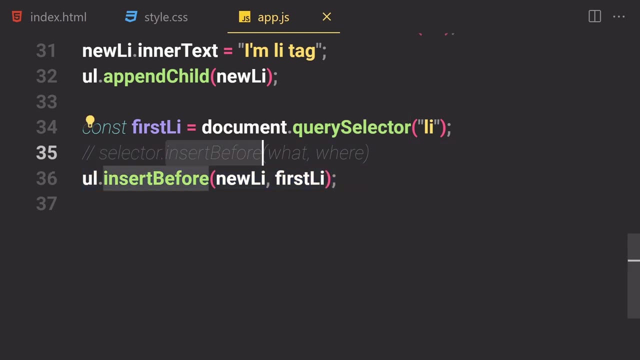 li and we want to put it in a first li. so if you just save that and we'll now just put it at the top right here, okay. so this is the first line and it will now insert it before this first li, right here. okay. so the syntax is a little bit weird. first of all we have to select something, then we 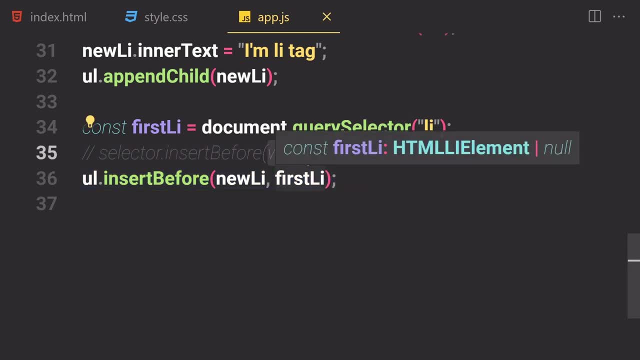 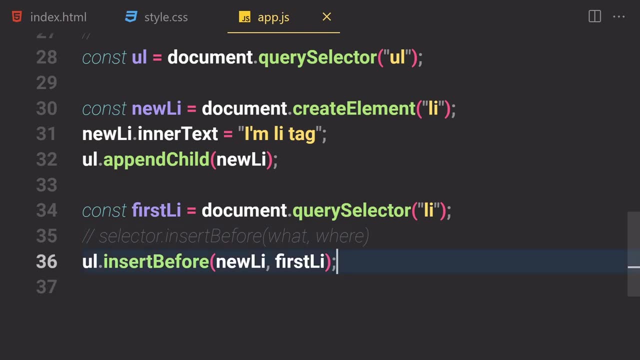 want to use this insert before and then: what do you want to insert and where do you want to insert it? okay, so that was just kind of a quick introduction about insert before element, and now let's just learn about insert adjacent elements. so let me just comment out all of these. 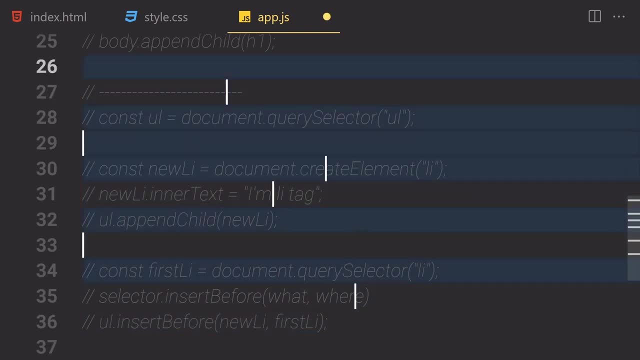 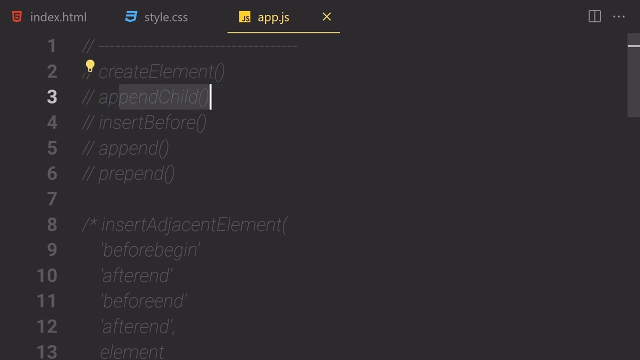 lines. for now i'm going to comment it out and let's just, uh, copy this line out and i'm going to paste this separate right here. so we just learned about create element append child insert before. now let's just learn about insert adjacent element right here. okay, so go to the bottom and 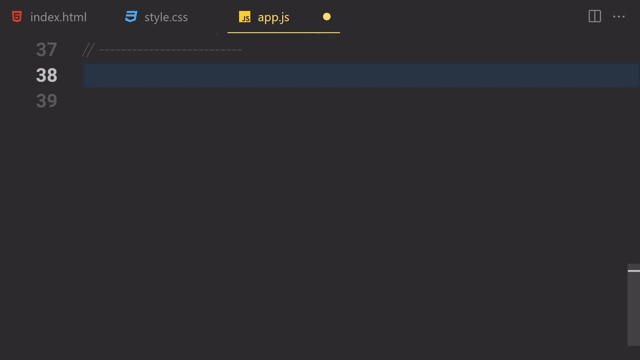 now let's just learn about insert adjacent. so first of all we have to select our paragraph, which is this paragraph right here. so so we are going to be writing cons, first paragraph. so we are going to be just writing document, create selector of paragraph. so we already select our paragraph. now let's just create our i tag. so i'm going to 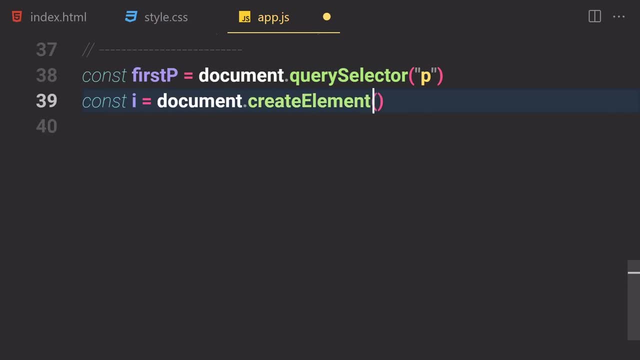 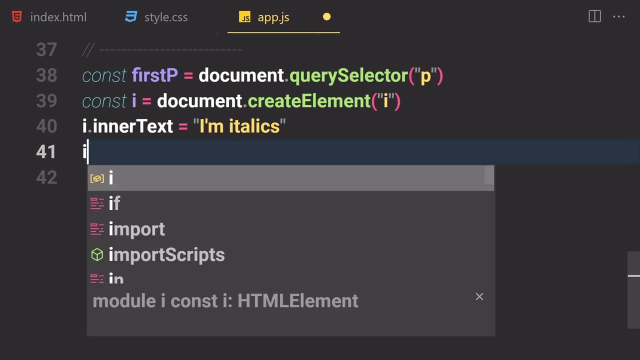 write i and then documentcreate element. so, as the name suggests that it allows us to create our element, awful i and then i dot. inner text will be now set to: i am italicized, italicized italics, or whatever you want to call it, and we can also provide a styling to it, so the style dot. 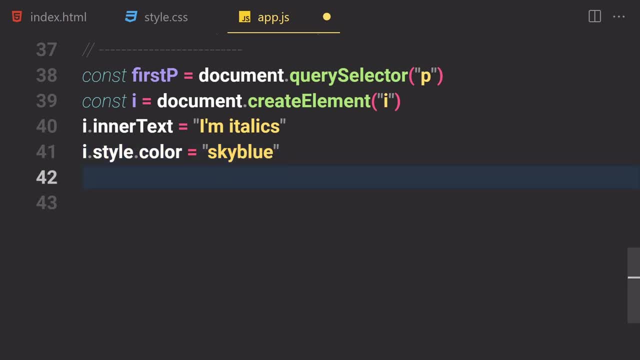 color will be now set to sky blue. okay, so now we successfully create our element, we provide a style. i mean, like we provide text to it and we also provide a style to it. okay, so now, if you want to insert that, so for that we can use a method called insert adjacent elements. so i'm going to 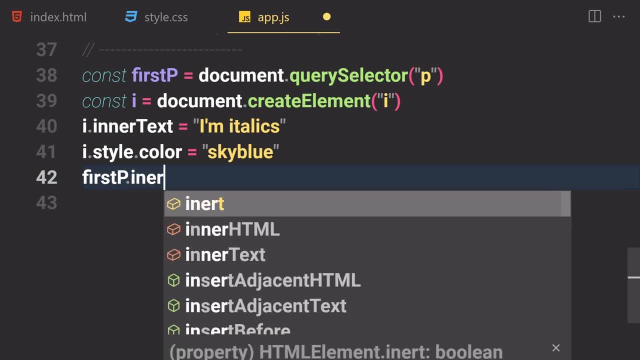 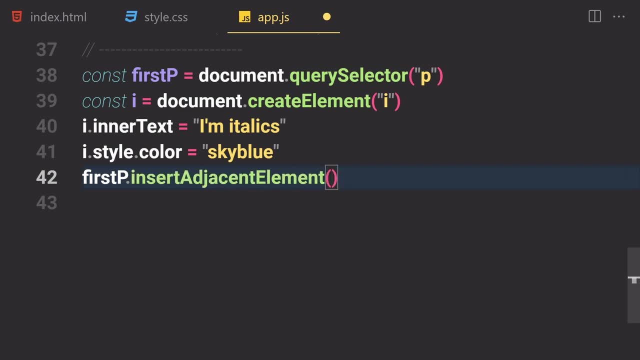 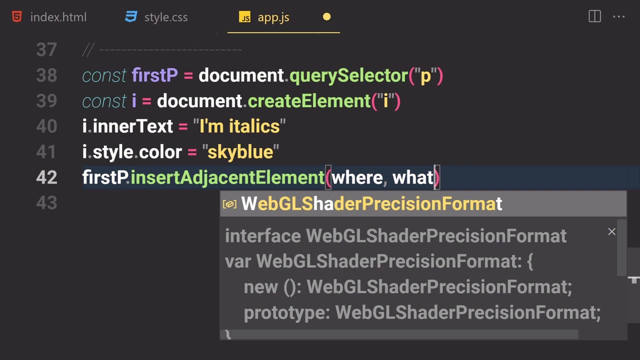 just first of all write a first paragraph and then insert adjacent not html, but elements, so element like so. okay, so it will just take like: where do you want to insert it and what do you want to insert it? okay, so it will also take two parameters, like: where do you want to insert it? 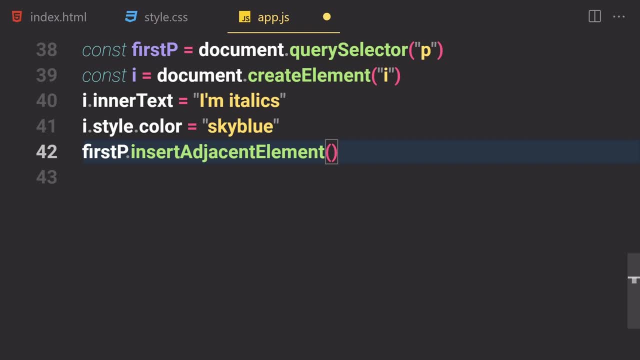 and what do you want to insert? so we have a few values for that. so we want to just write like before begin. so before begin, as the name suggests that it will just insert it before it begins. so if you just save that and it will now place it right here, i'm going to just remove that, so it will now. 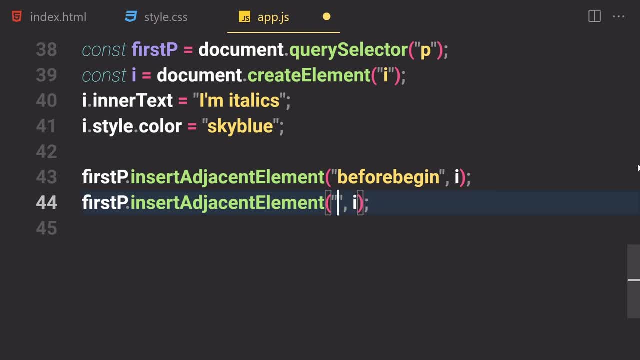 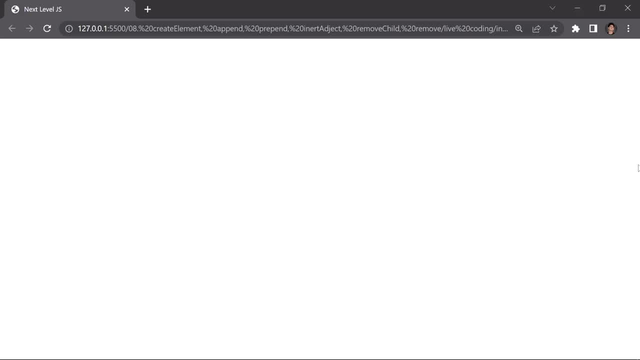 place it right here. i'm going to duplicate this line of code and i'm going to just change that to: after begin: uh, f-t-e-r-b-e-g-i-n. now. if you save that, it will now place it right here. okay, after it begins, i'm going to duplicate that one more time. 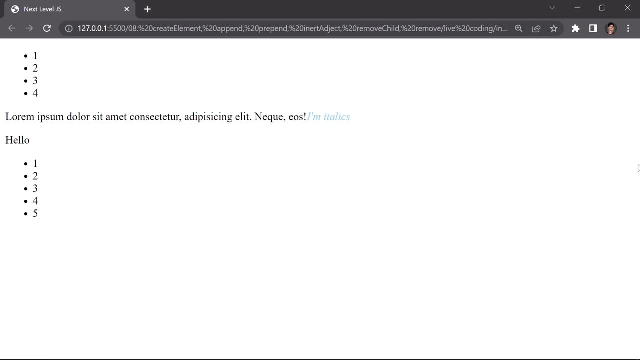 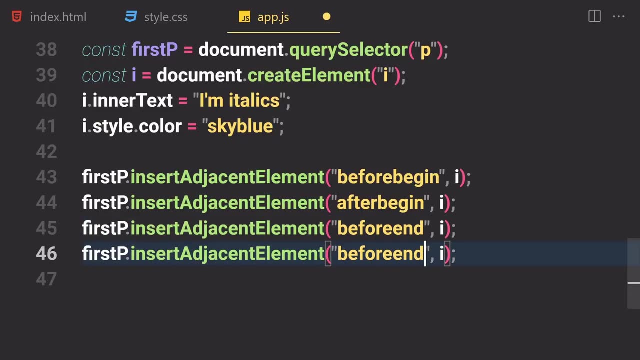 and then we have before end. and now, if you save that, it will now push it right here before the end of that uh line, right here, okay, so now if you duplicate that, and then we have a final parameter for that, like after end. and now, if you save that, 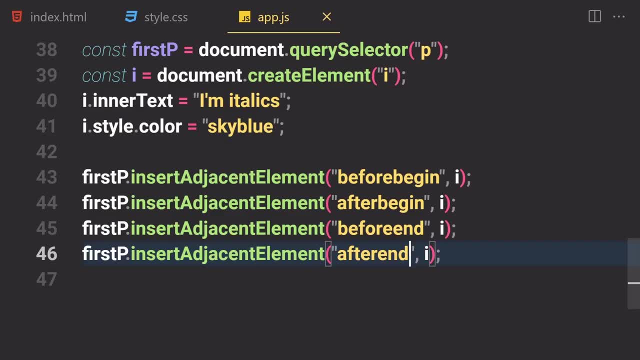 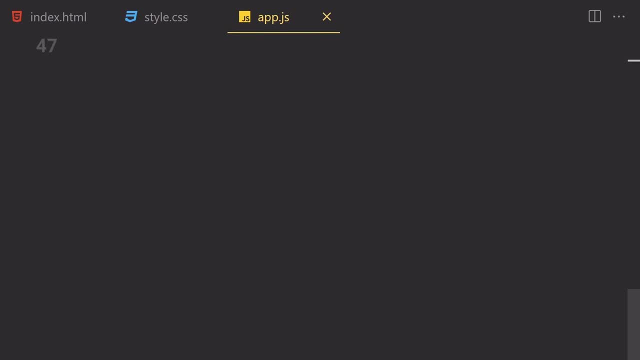 and it will now just put it after the end of that paragraph. so this is how you can work with the insert adjacent element. and then now let's just learn about this- append and then prepend. these are kind of a similar ones, so i'm going to just comment out this one. and now let's just place: 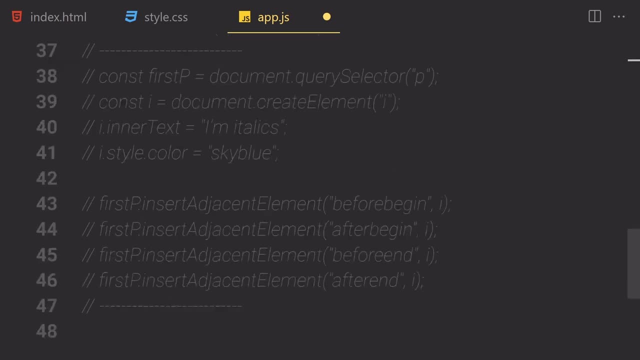 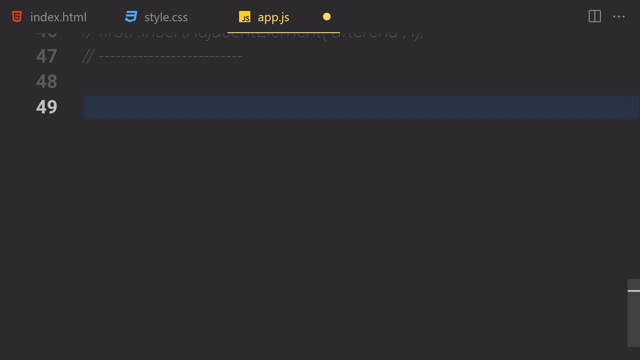 this separator for here and now. let's just learn about append and prepend. so, uh, for append and prepend, it's kind of a similar and simple one to learn. uh, let's just get our section first of all, so we have this section with the text of hello inside, and then we have the text of hello inside. 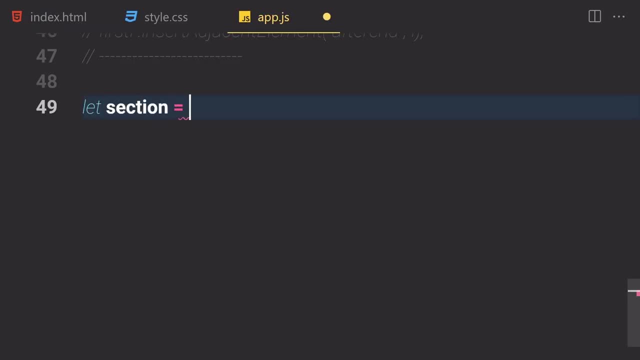 there. so now, if you want to get this, i'm going to just write section. it will be now equals to document dot query selector of section. okay, so now let's just uh append or ally to it. you know what i'm going to comment, uh, uncomment this line, or you know i'm going to copy this text from here. 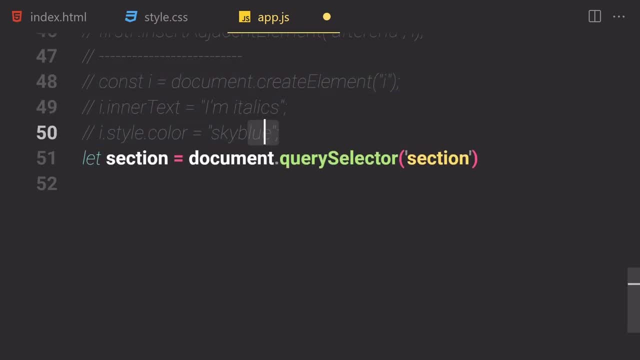 and i'm going to paste it right here. i'll cut that one paragraph and uncomment these. so now we successfully create, or i tag right here and we just, uh, provide an inner text to be like i'm italic, and we also provide a color, to be sky blue, and now let's just push that. you know i'm going to. 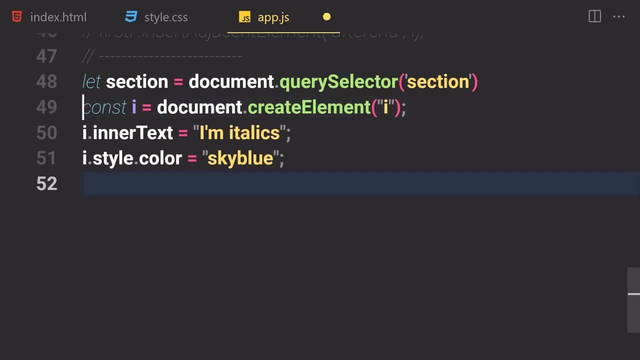 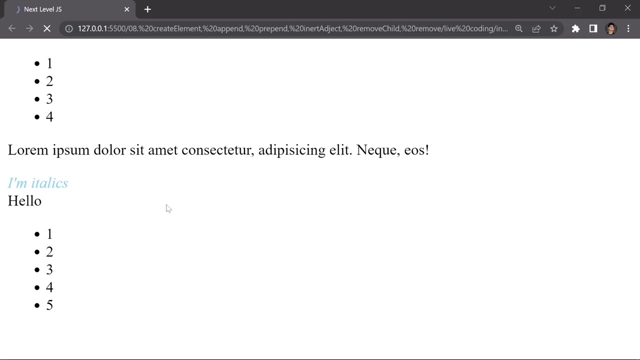 cut that from here. i'm going to paste it right here. okay, so now, if you want to push this i tag to this section by using a pen class, so we can also do that. so let me just write a section. let's just write section and then append off this. i. so, if so, now, if you save there and now, 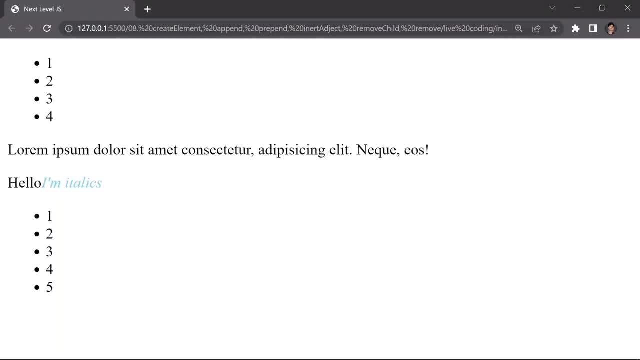 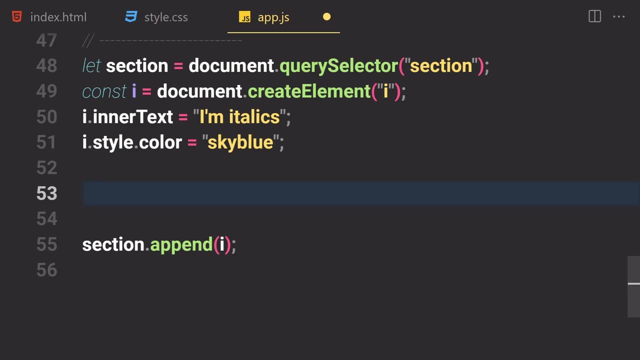 here you can see it will now append this: uh, i metallic with the hello. so we are now appending this. i tag on this section right here so we can just create another one like: let's suppose const h4 will be now equals to document dot. create element. uh, create element. oh, my goodness, come on create. 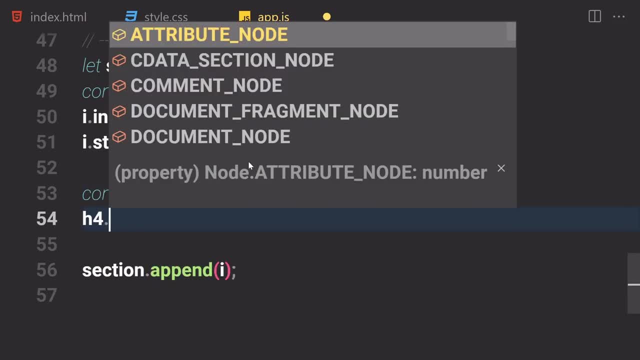 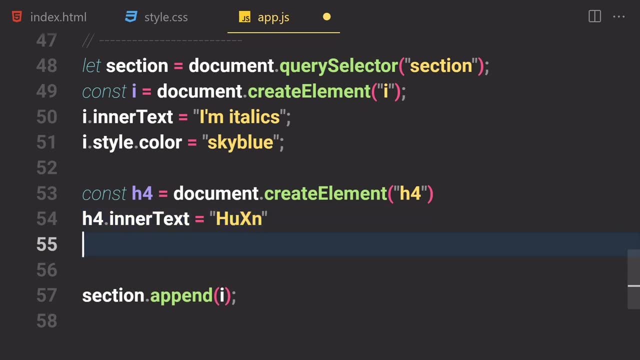 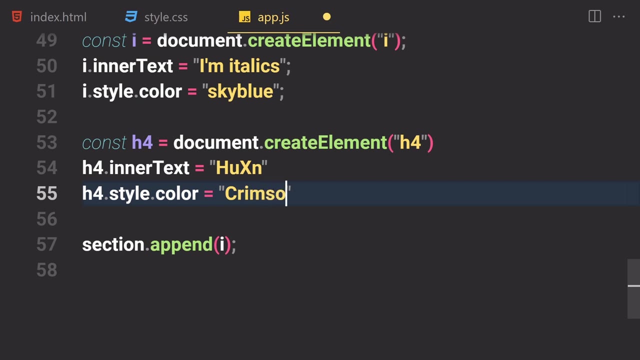 element of h4, and then h4 will have the text of, like i don't know, inner text will be now set to maybe my own name, like hussein. and now let me just uh change the four dot style, dot color to be, uh, crimson, crimson. and now let's just append that as well at the same time. so i'm going to just 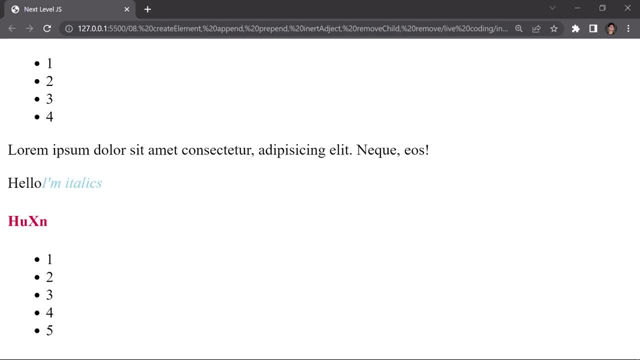 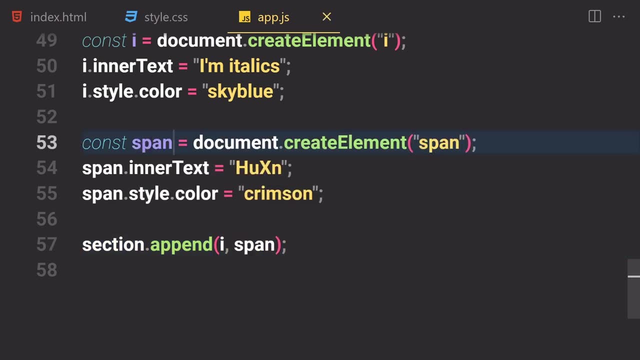 write h4 and now if you save that and boom, here you can see it will now append this one as well. so if you just change that to span and also change these two spans, and now if you save there- and it will, now you can see it will now be in line right here. okay, so this is how we can append multiple. 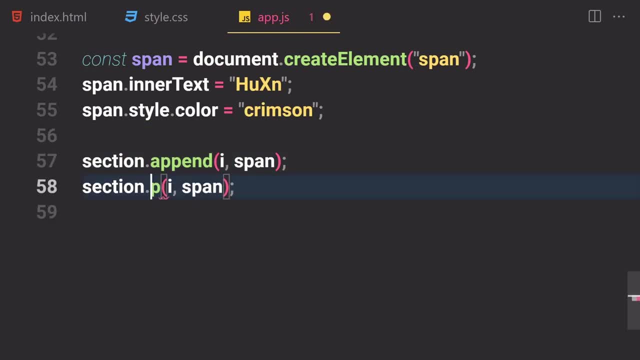 things at once. so then the next thing which we have: we have pre-pens. so now if you sell a file and say it will now append it at the beginning of that section, and if you just use that append, so it will just push it at the end of that selection. so if you save that, it will now push it to the end. 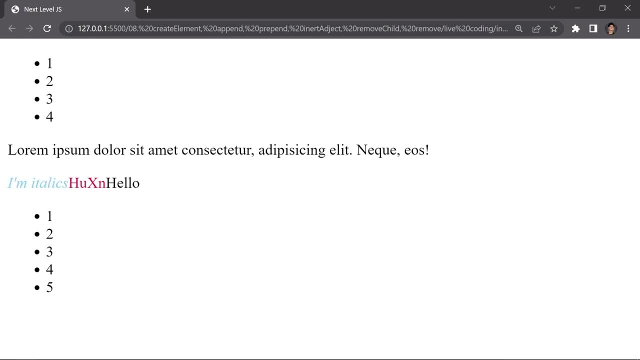 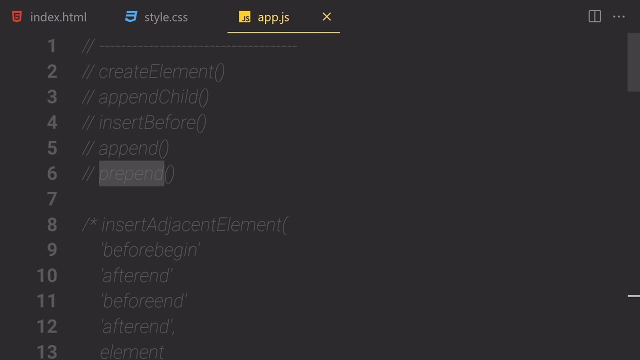 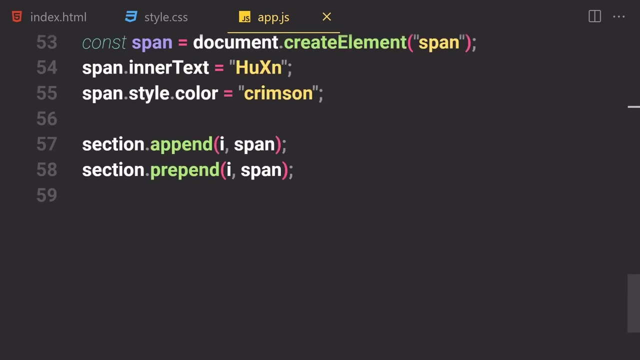 and this prepin will just push it at the beginning right here. okay, so that's it about. uh, create element, the append child before append prepin and suggestion. now let's just learn about remove child and remove. okay, so it's kind of a self-explanatory. so if 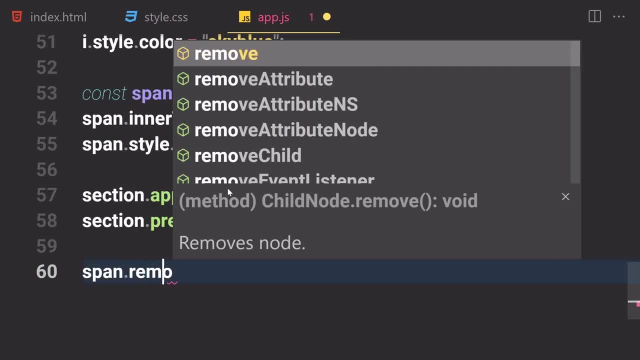 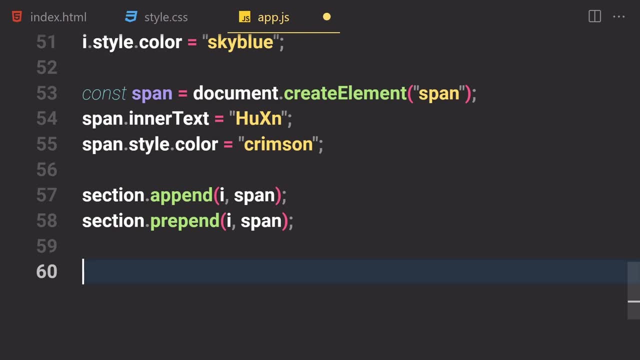 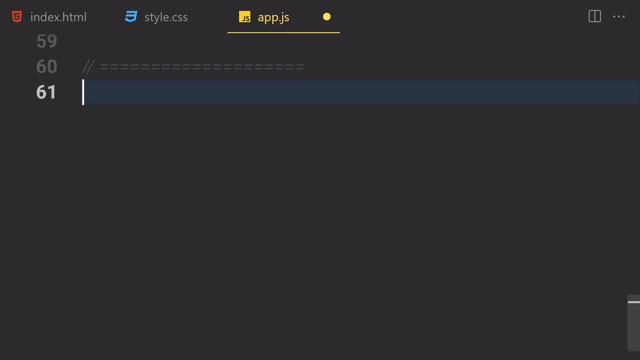 you want to remove that um span, so you can just write spanremove. you know what? not span? let's just see. uh, we have a new list. first of all, let me just get my new list real quick and i'm going to comment all of this code right now. create a separator for myself and now let me just write: 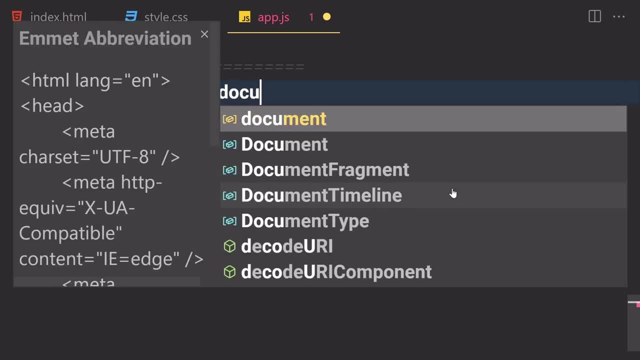 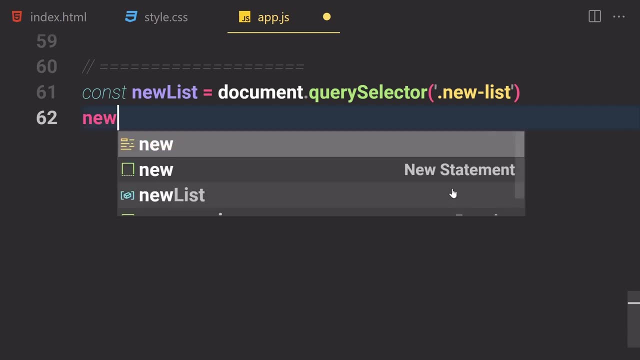 a new list first of all const new list and it will now equals to document that query selector of new list. okay, so we have different kind of elements inside this new list. so i'm going to write new list, dot- remove child c, h, i, l, d, and which child we want to remove. so we want to remove. 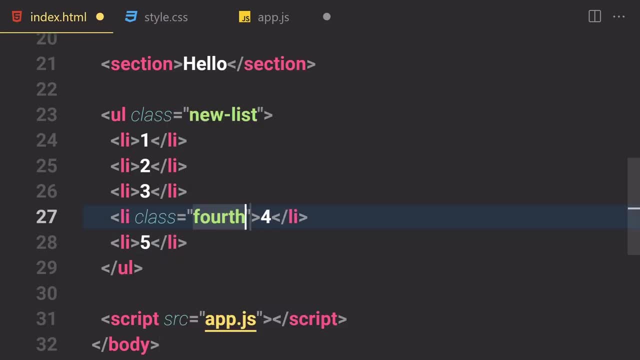 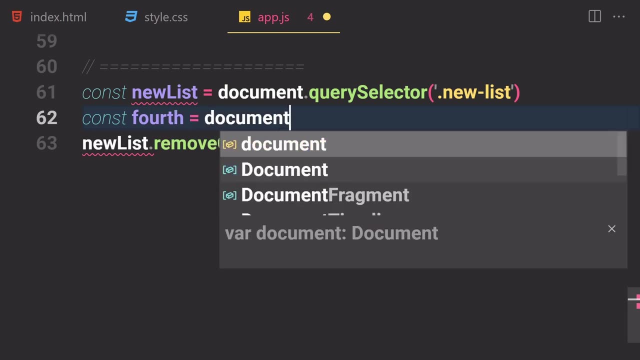 this one. oh, you know what? this one, fourth one- i'm going to give a class of fourth, so copy that and let's just get order fourth as well. so const fourth will be now equals to document that query. selector of fourth. okay, so we have to just specify this fourth in it. so 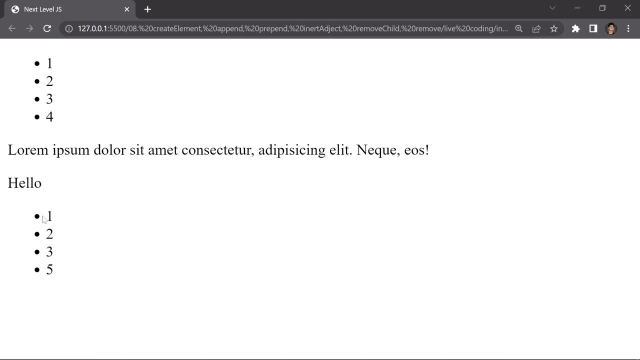 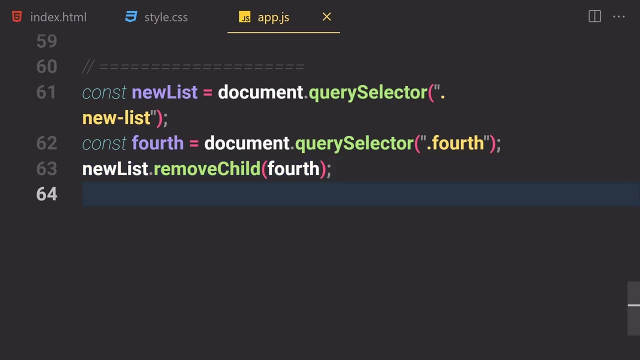 let's just write fourth and now, if you save that, it will now just remove that fourth from here. so we have one, two, three and five. we don't have that fourth one, and if you want to remove all of them at once, like if you want to remove all of that list, so for that we have. 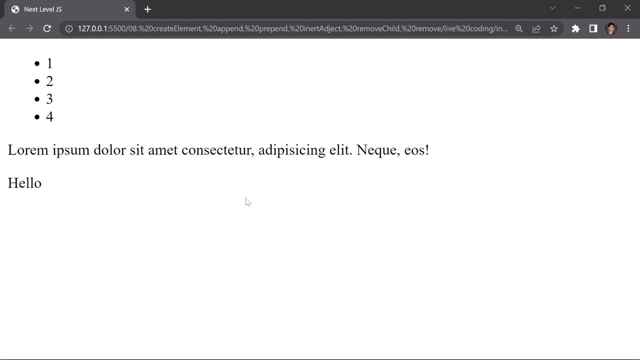 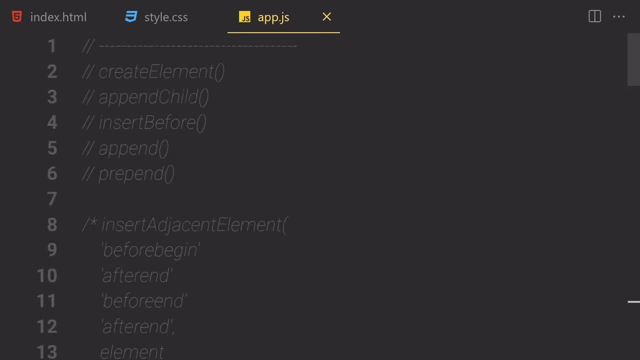 new list, dot remove and boom, okay, so we'll just remove. so if you want to remove the other stuff, so you can just use this remove method and we'll just remove it totally from the dom. so in this section we learn about different kind of methods, like we learn about create. 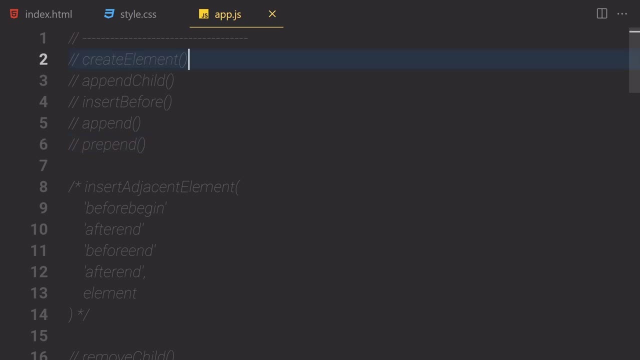 element method and create element method, as the name suggests that it allows us to create element. then we learn about append child. it will just push or anything we just created at the bottom of the page, at the bottom of the list, and then we have insert before. it will just. 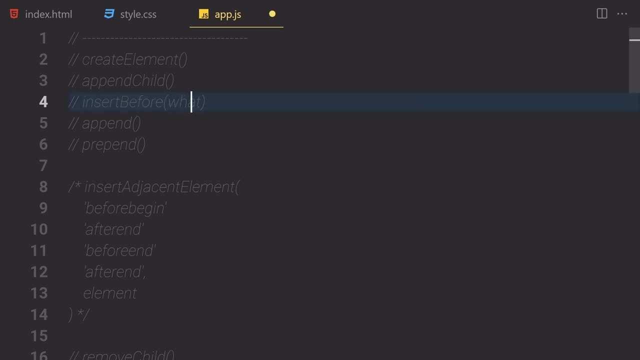 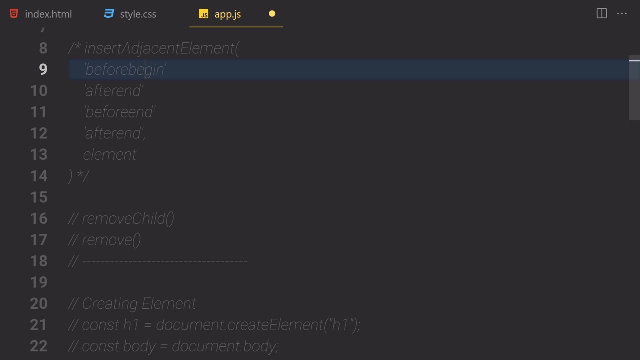 insert it before and let me just put like what and where. okay, then we have append method and append will append or element at the end of the list and prepend will append or element at the beginning of the list. we also learn about insert, adjust an element before we have a few properties for that. 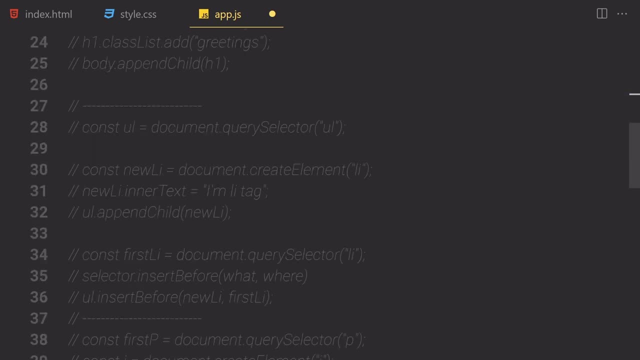 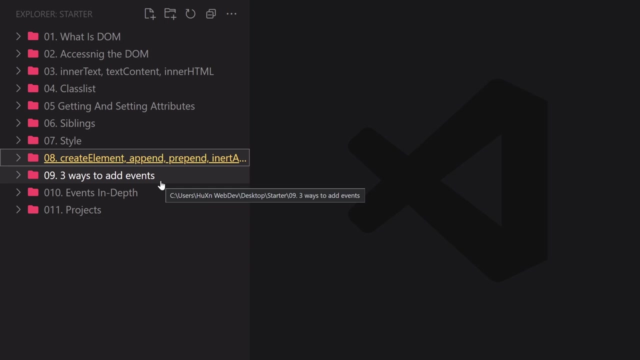 and we also learn about removing child and also the remove method. so we learn enough about in this section, so what else do we have to learn? so now, the next thing which we are going to be learning is something called event listener in the dom. all right, so now that we are totally done with creating element appending and 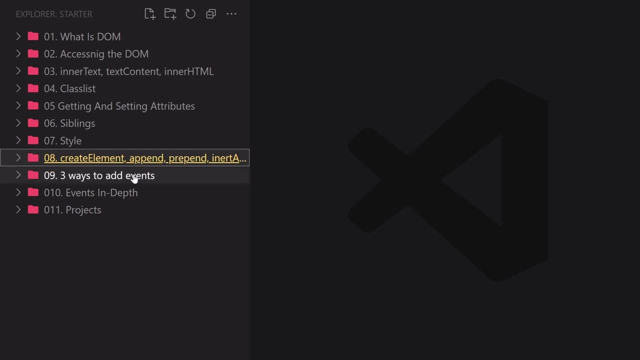 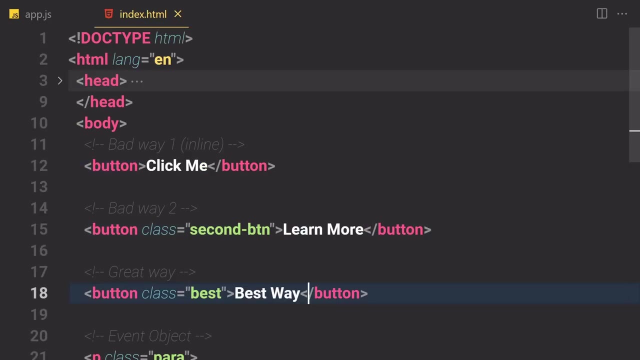 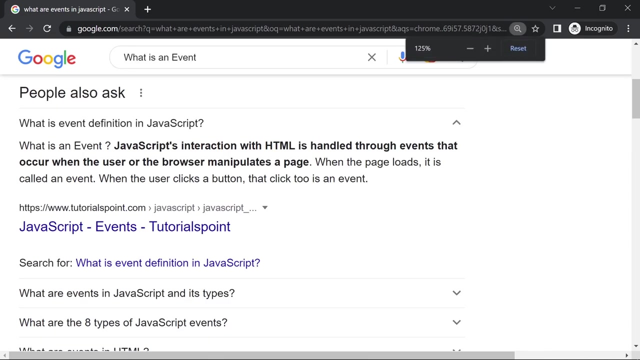 prepending and all of that kind of good stuff. so now let's just learn about something called events in javascript. so, uh, this is our html coding. it's not that much. but before we get into all of these coding, let's just ask our good old friend: like: what in the world is even so, what is even javascript? 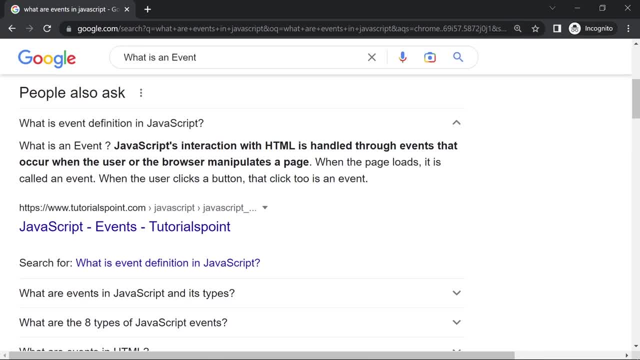 interaction with html is handled through events. that occurs when the user or the browser manipulate a page. so when the page loads, we have different kind of events for different kind of things, which we are going to be learning in this video. so like in, for example, when the web page door, it can call: 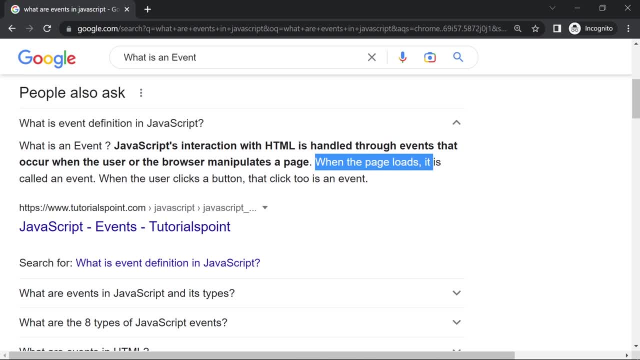 an event the user can. if the user click on some button, the specific event can be called. or if the user drags something, if we just click on somewhere else, if we move our mouse to somewhere, so we have different kind of events for that. so i just kind of want to give you the definition of what event is. 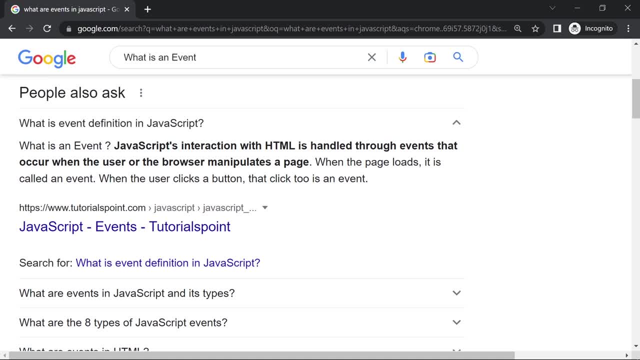 so let me just say that one more time. javascript, interaction with html, is handled through events. that occurs when the user or the browser manipulates a page. when the page loads, it is also called event when the user click on the button, that click is also an event as well. so 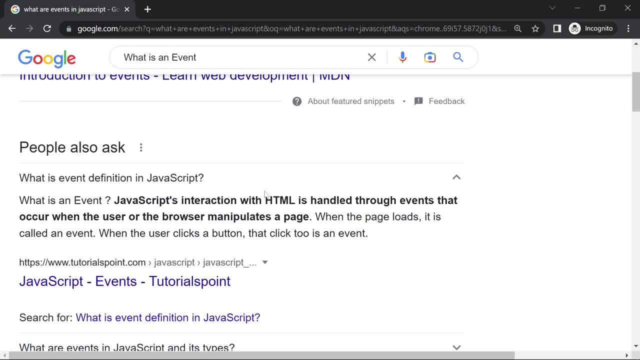 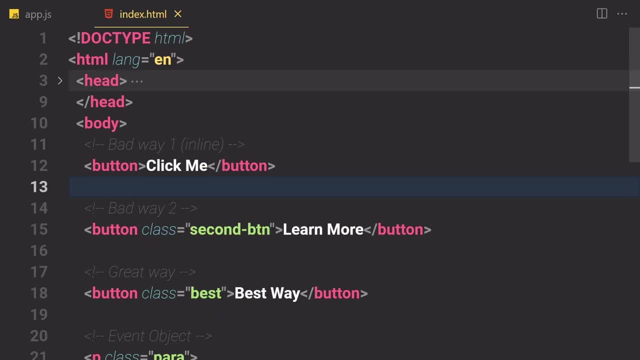 that was just kind of a definition of our events. so now we're going to be learning about how to jump into our coder and let's just see what we have. so first of all we have our doctype html, just a structure of that. then we have our button with no classes, nothing inside there, but we just have 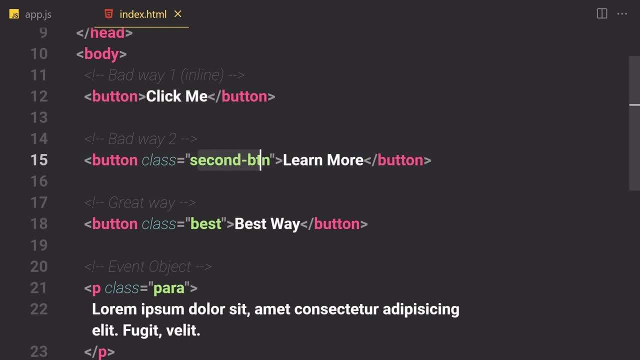 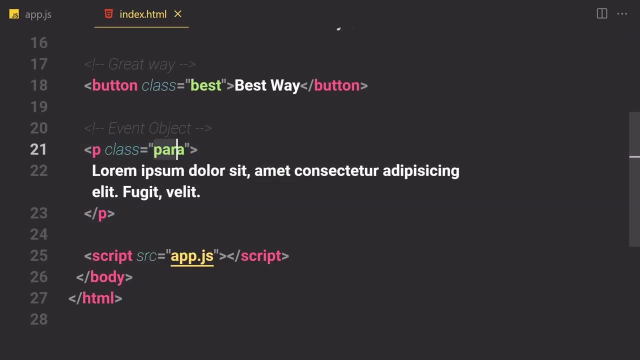 a level of click me. then we have another button with the class of, second button with the text of learn, or you know what bad way would be fine, so with the text of bad way. and then we have a button with the class of best and best way and finally we just have our paragraph with the class of para. 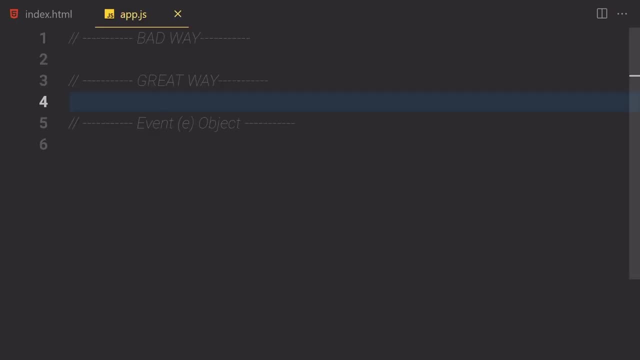 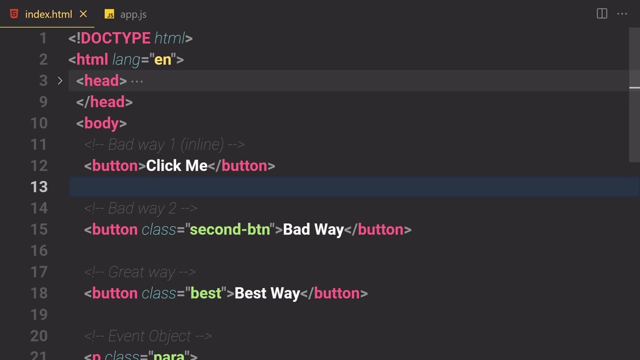 so this is it for our html. now let's get into our javascript. and now let's just start working. oh, you know what? we're not going to be just jumping into a javascript straight. first of all, we have to learn about the inline event. so how would you attach inline events to inline, or? 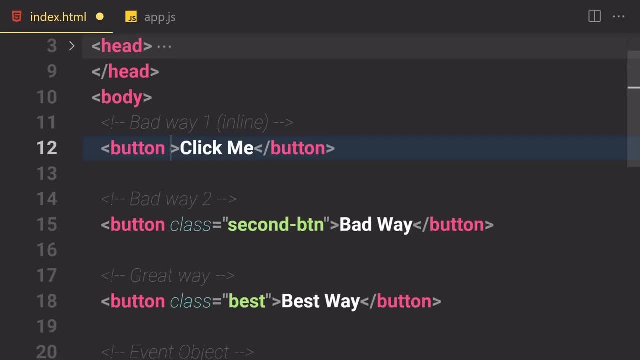 specific element in your web page. so now, in this case, we are going to be learning about inline event, but my suggestion will be to never use that. so if you want to attach inline events, so first of all you are going to be writing on, and then we have a click and we have 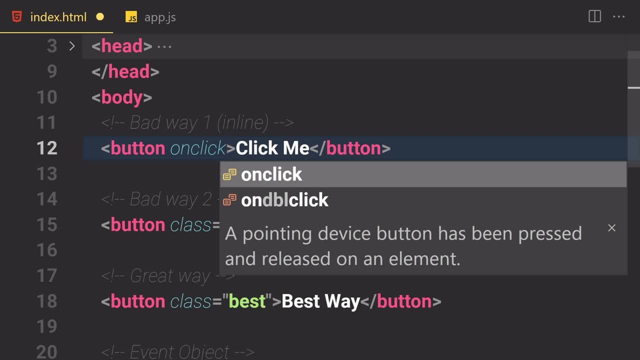 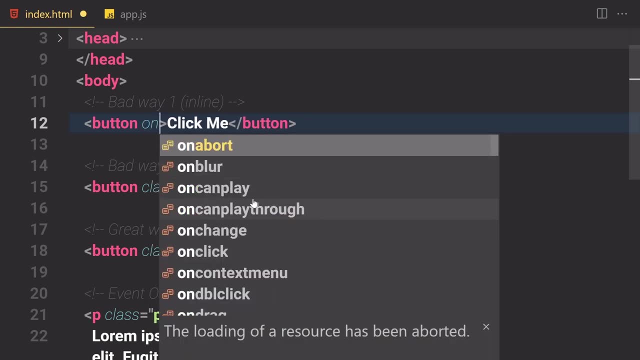 a lot of events for a lot of different kind of things. if i zoom out, if i just zoom out a bit like so, if i just write on, so we have on a board on blur on, can play on, can play through change click context menu, double click, drag, and we have different kinds of events right here for different 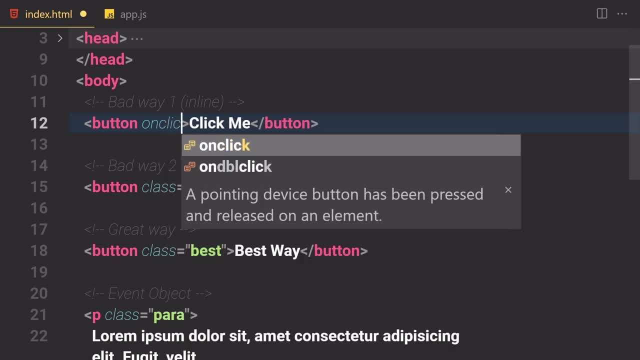 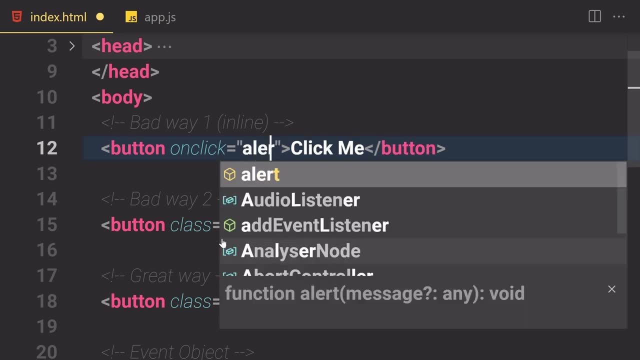 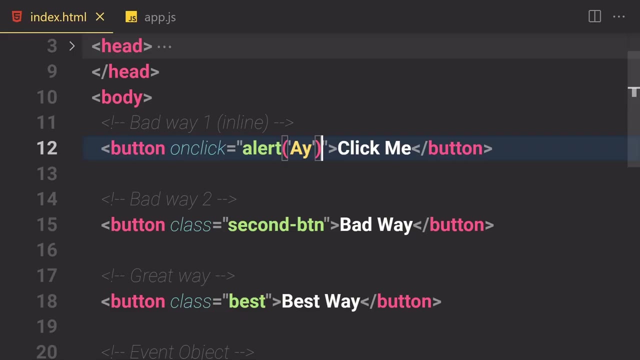 kind of things, but in this case we are just interested in the click one, so we are going to be just working with the on click event right here. so now, what do we have to do? let me just write alert in here and i'm going to just put the value of like a: okay, so if you save our file and let's just launch this, 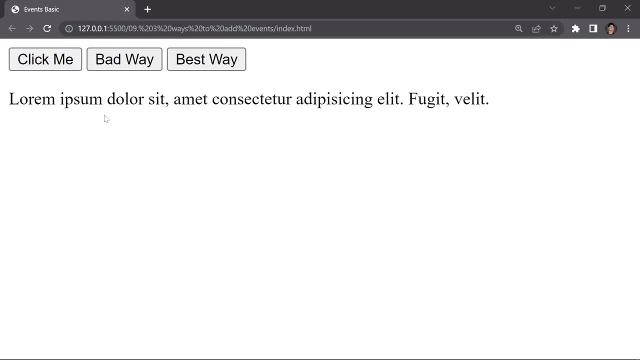 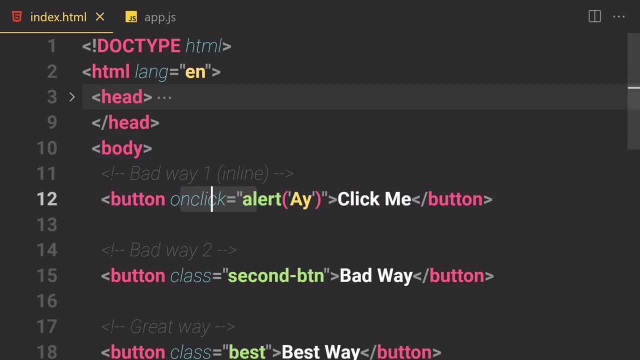 in or live server so it will not just launch it all right. so now if i click on this click me button right here, so here you can see it will not give us this a right here. that's because of this event like on click. so whenever we click on this button, so something will happen. so we just attach alert. 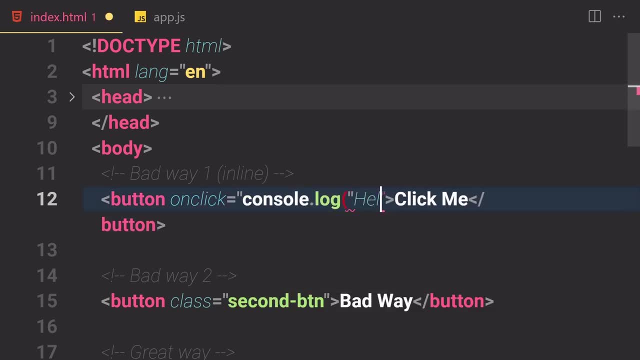 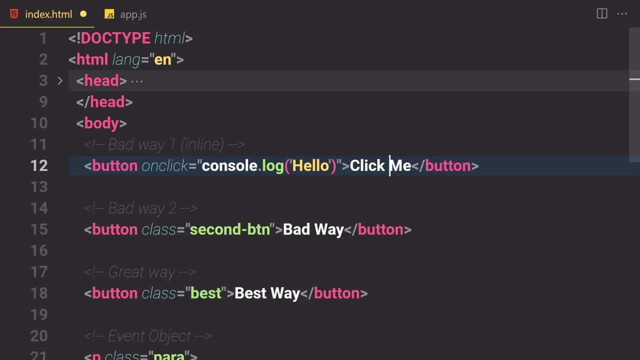 we can also just write like i don't know consolelog of, like hello, so let's just do that, oh you know what. or single code would be fine, so that it doesn't give us an error like so: if you save our file, open our developer tools. if you click on this, click me so anytime. 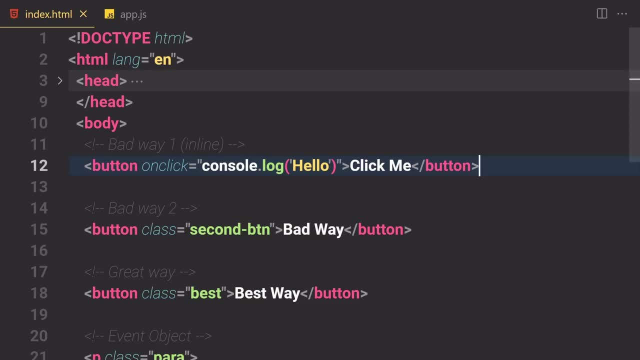 we click on this button, it will now give us this hello right here. that's because of this button and my suggestion will be to never ever use inline uh javascript like that and never ever use inline uh events. but i just kind of want to show you like for some cases, if you just see like 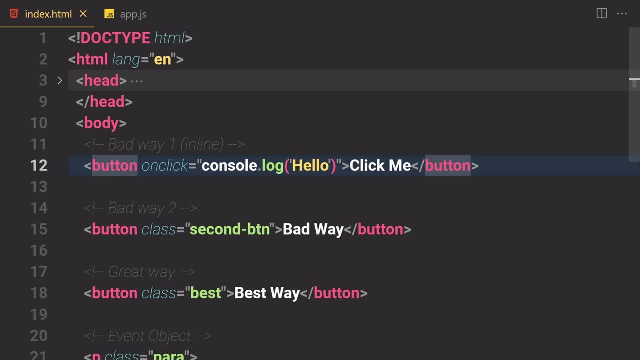 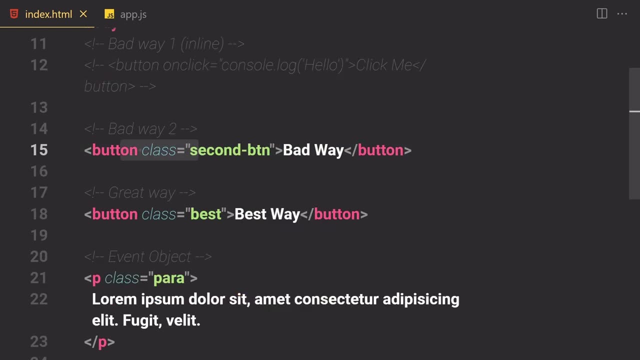 old code bases, so you will find this on click inline events, so be aware of that. so i'm going to just comment this line for now. and now, what else do we have? so we have a second button and we are going to be learning about yet another bad way, and then, finally, we are going to be learning 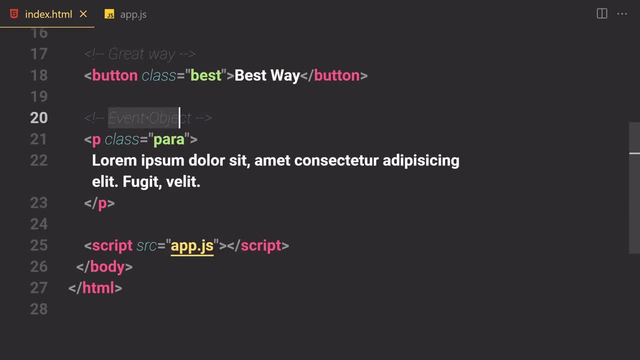 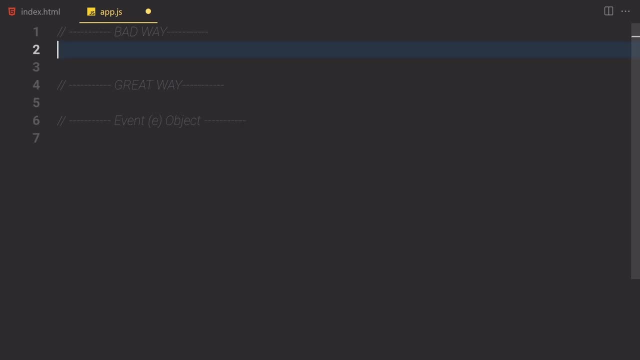 about a great way to attach even a listener, and we are going to be also learning about event object. okay, so now let's just write or bad way. so first of all, if you want to work the bad way, first of all we have to select something so that we can attach or even listener on there. so let's just 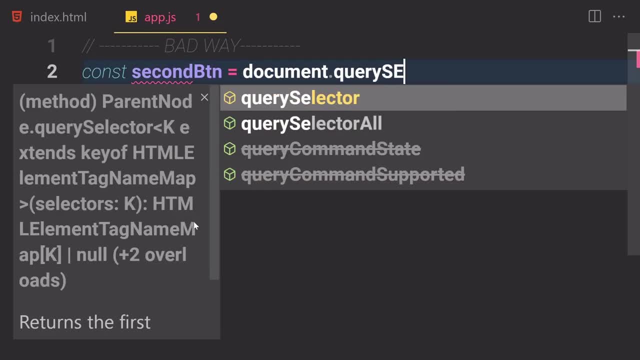 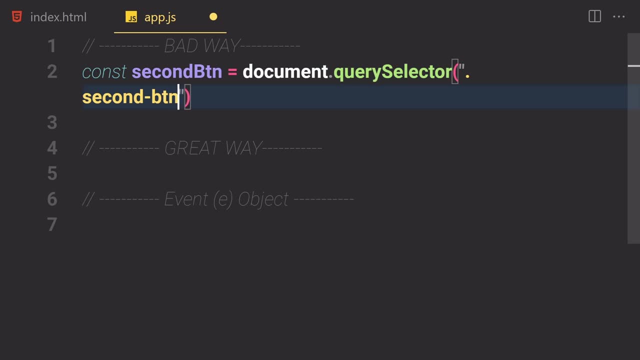 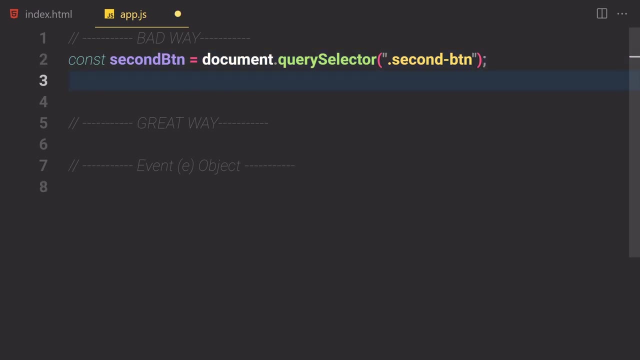 select our second btn and let me just write documentquery query selector- this one- and let me just get my second btn zoom out, which is this second btn right here. okay, so now we totally select our second button. now, if you want to attach your event listener- and this is the second bad way to- 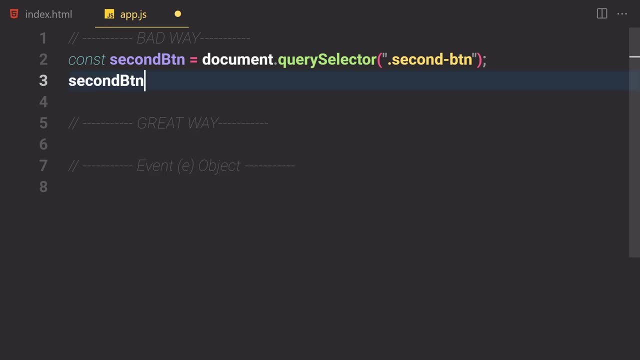 attach your event listener. so first of all, we have our selector like second button, and then we have our second btn. so what do we have to do? we are going to be just firing this function right here, or you can just put alert in here. and, by the way, if you just put alert alert right here, and if i 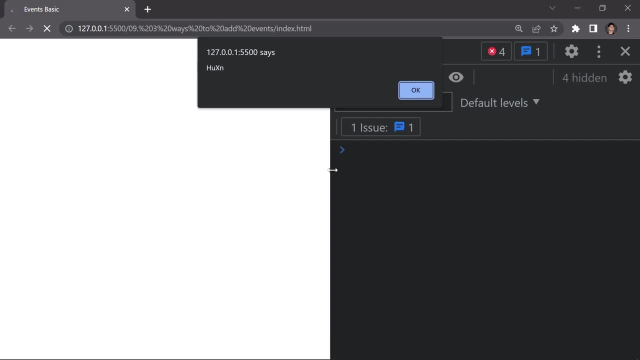 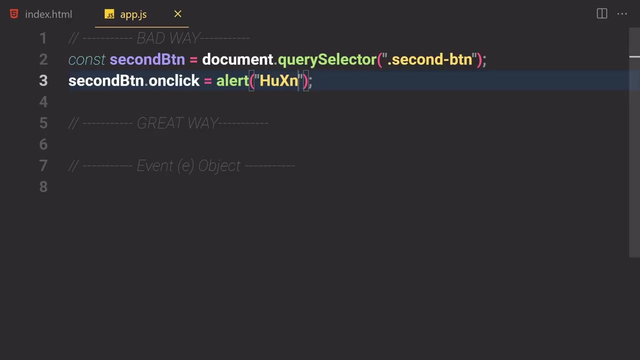 just put my own name and if you save a file, it will now gives us that alert right here and our web page does not loads up. this is another story, but i want you to know that it will block our web pages from execution. so if i just click on ok, it will just paint our browser right here, but never. 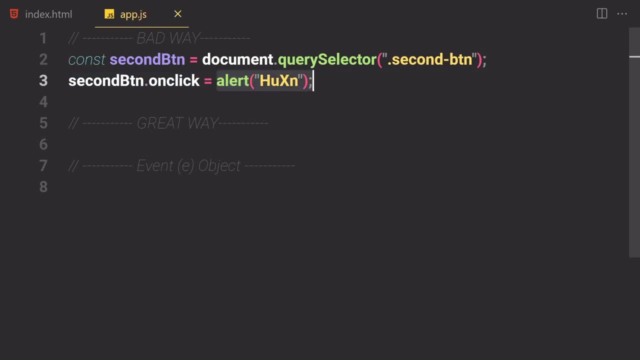 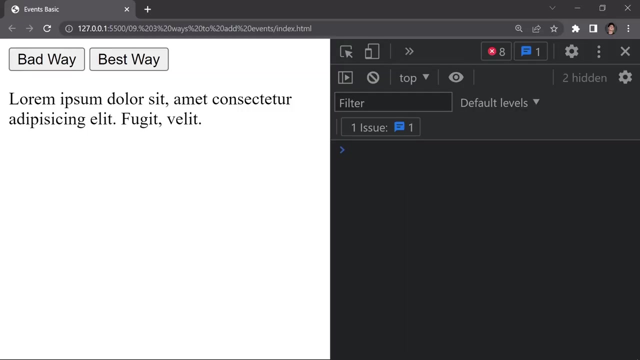 use this alert and this kind of a bad stuff. so instead we can just use a function. if you just use a function like so and if you just write consolelog of uh, huzzain, maybe then web dev, web dev. and now if you save our file, and now if i just 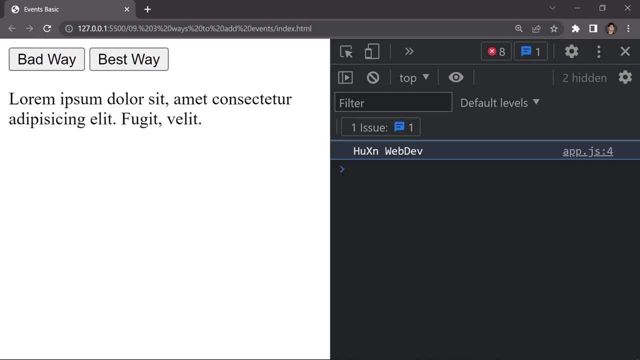 click on this bad way, it will now print us that huzzain web dev right here and we have different kind of events like: uh, we have on mouse move, i guess, so server file. so now, if i move my mouse over to that button, so it will now print. 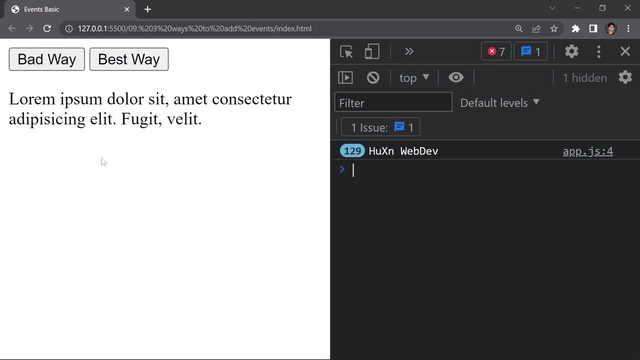 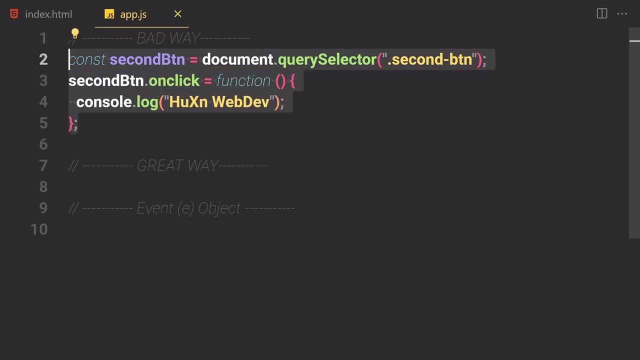 name that much time like so. here you can see countless time, so we have different kind of events, but for now i'm going to just stick to on click event, and this is the bad way to write events, so i'm going to comment this line out. okay, this coding out, and now let's just learn about a. 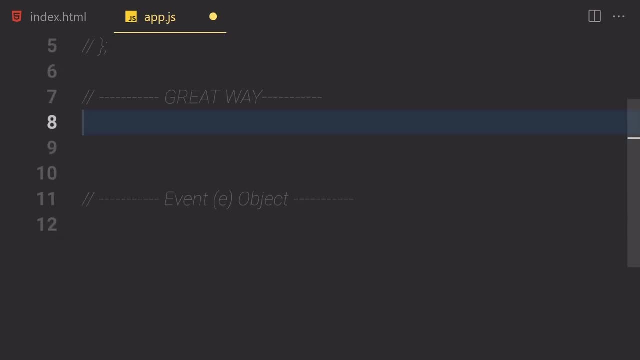 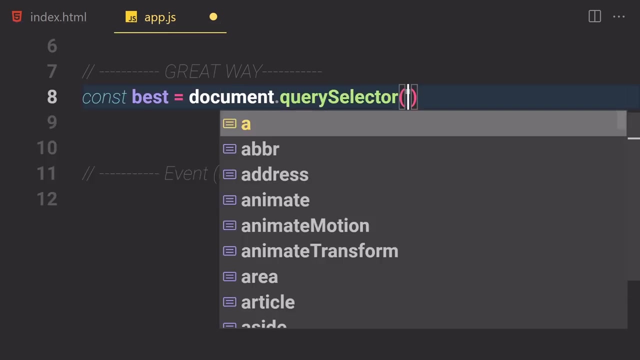 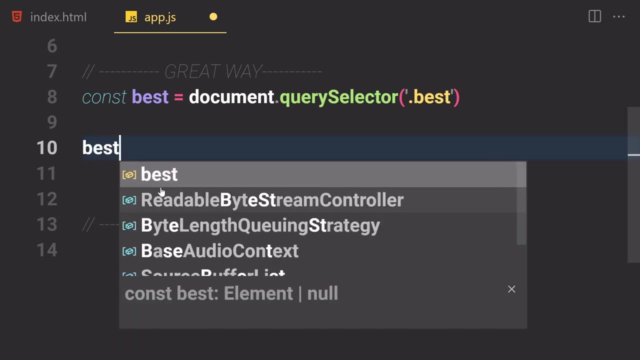 great way to attach events using javascript, dom. all right, so let's just select our best. so i'm going to just select my best documentquery selector of best. and now, if you want to attach event, listener on this best by using a best way. so, first of all, we are going to be selecting our 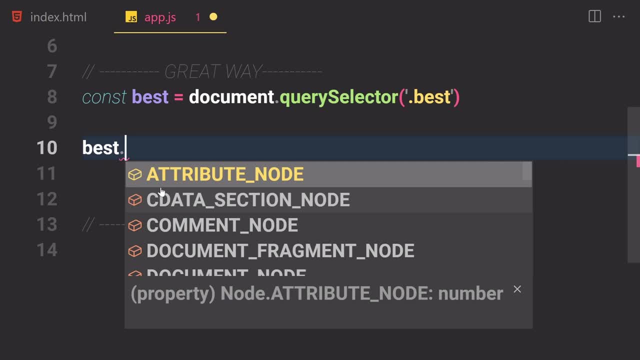 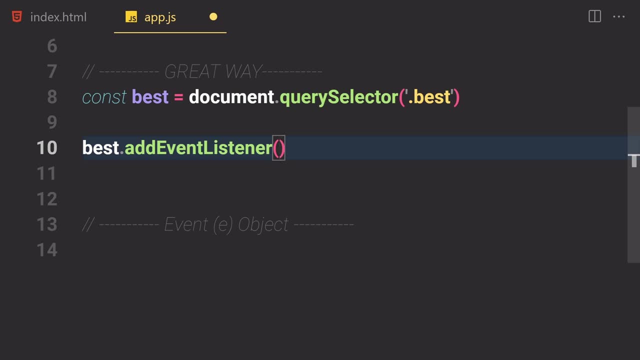 best like some sort of a selector, and then we are going to be using a method called add event listener, and this is the best way to attach your event listener to different kind of elements. so now here we have to specify, like, which kind of events we want to listen to. we have click, we have 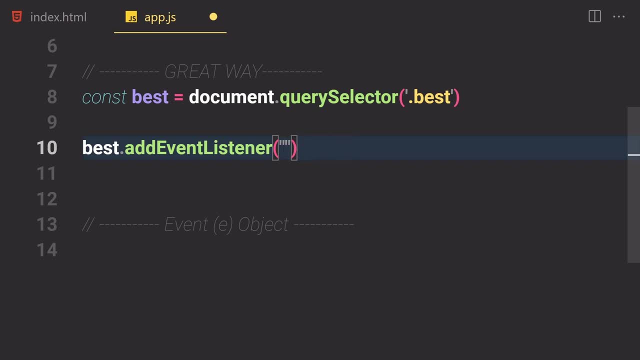 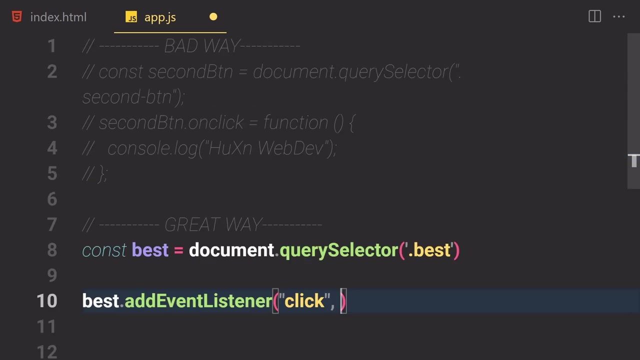 a dbl click, we have a mouse move click, we have mouse, or we have a lot kind of events which you are going to be learning just in a second, but in this case we are just interested in click event, so you'll just pass or click and then we have to pass some sort of a function. in this case, we just pass our function. 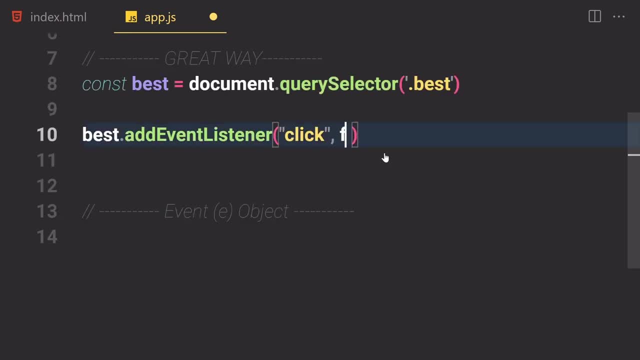 manually right here. but now, in this case we can also pass our function manually as well, like just pass an anonymous function and then just write like consolelog of hello world. and now if you save that and now if i click on this best face here, you can see it will still print that hello. 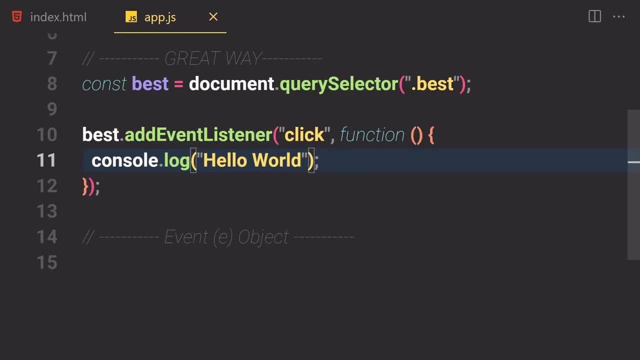 world right here in the console. but we can also just separate that function to somewhere else. so if you just copy that or cut that from here from here, and if you just put it right here and we have to give some sort of a name like greetings would be fine. now we successfully create our function. now we have to just pass the. 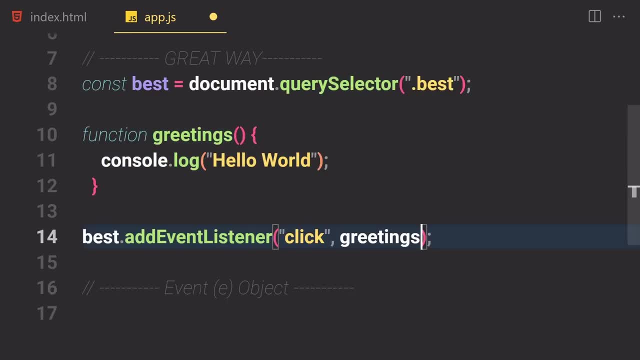 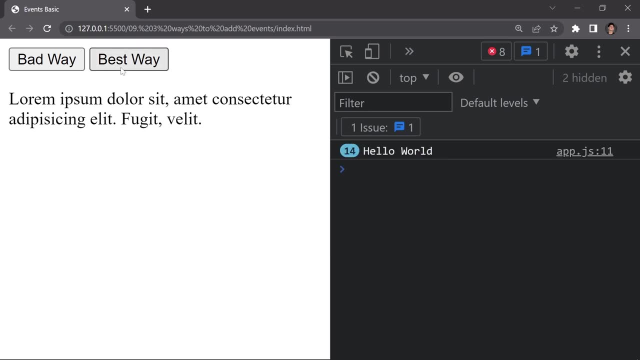 name of that function or the reference of that function inside this add event listener as the second parameter. so if you save our file and now if you click on that one more time, so it will still work right here. okay, so everything is working the way we expect it to work. so now we are going to 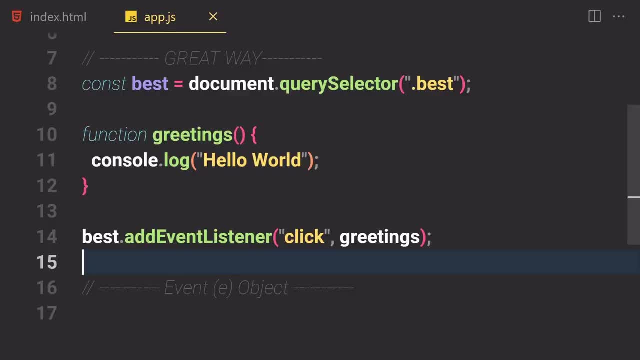 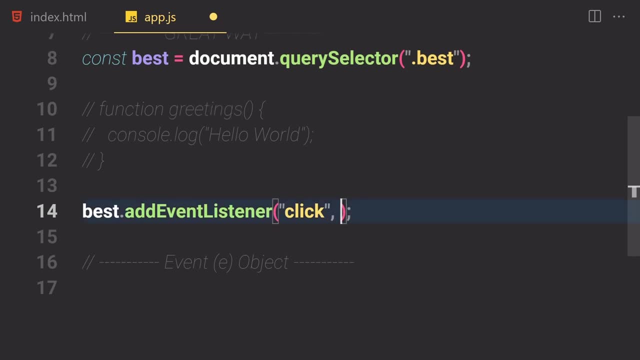 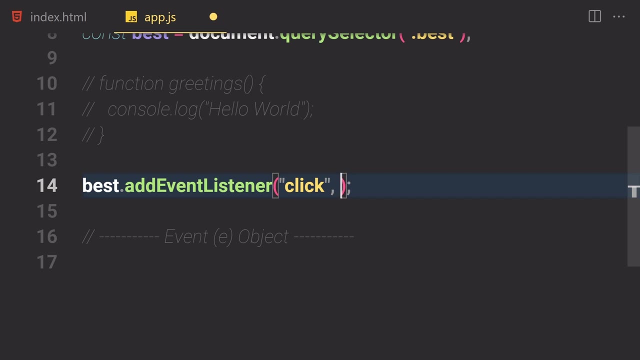 have to work and we can just still pass what we call it off- error function. so i'm going to comment this line out and let's just remove these greetings from there and we can still pass an error function. and, by the way, if you guys don't know about error function, so i've got entire course on es6 and 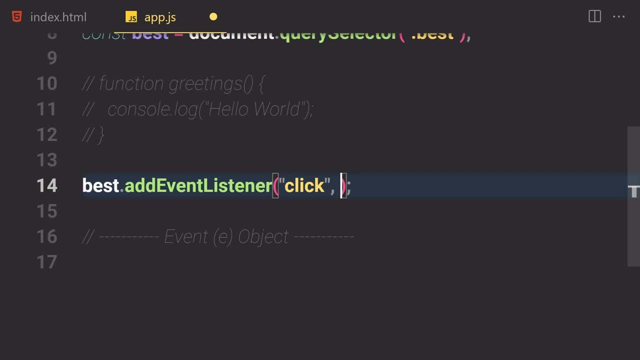 there if you want to check that out. or it's totally free on my youtube channel. so es6 through es, whatever the best way is coming up. so i have a course on. es6 is like all of these bleeding edge javascript. i have entire course on there if you want to check that. 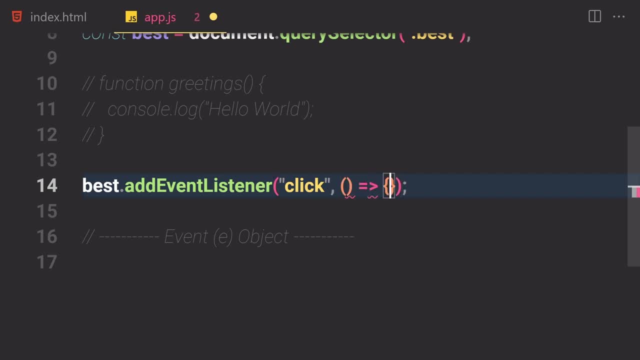 out anyways. so if you want to check out the error function where you so, feel free to do that. i've got a video on that error function as well. so this is how you can pass error function and you can just write like whatever you want to write, like: consider log of uh yellow. and now, if you save, 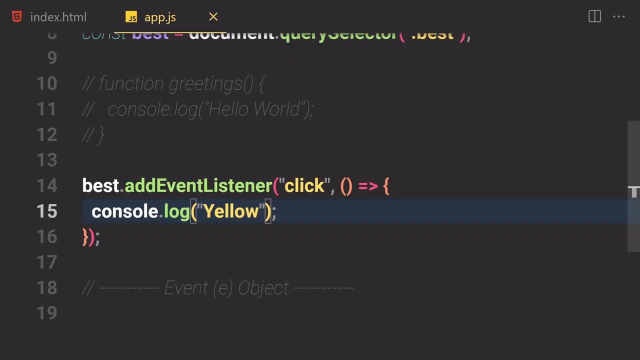 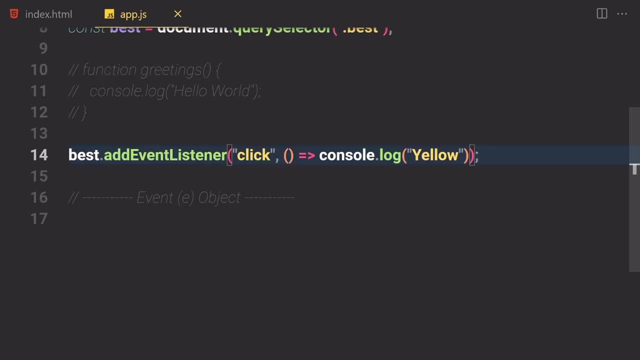 there and if you click on there it will pronounce yellow, and if you are using an error function, so you can also omit these curly braces from there. so if you save there and now here you can see, we get our one liner right here, and if you click on this best way it. 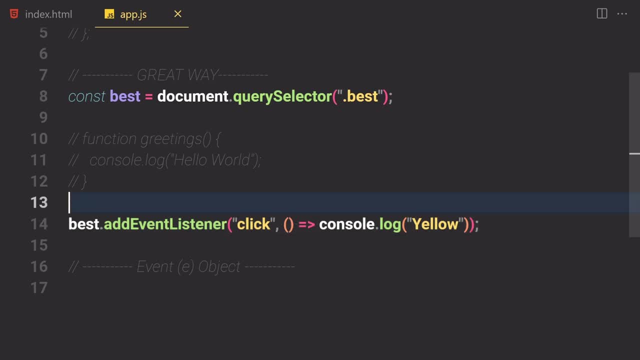 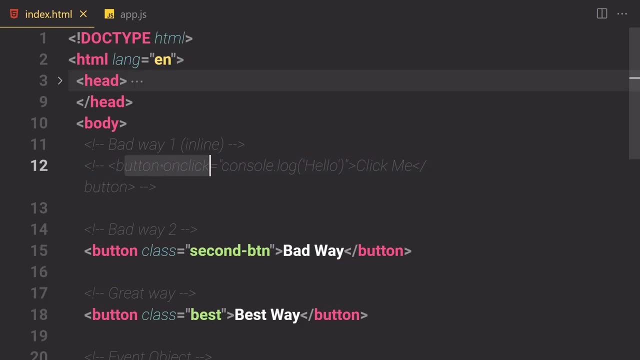 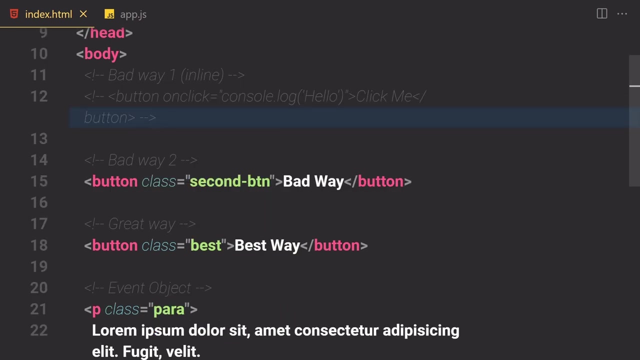 will now still print us that yellow. okay, so this is how we can attach event listener. so in this video we just learned about three ways to attach event listener. this is the first way, the oldest, like the 90s way of attaching event listener by using inline event listener. and then we learn. 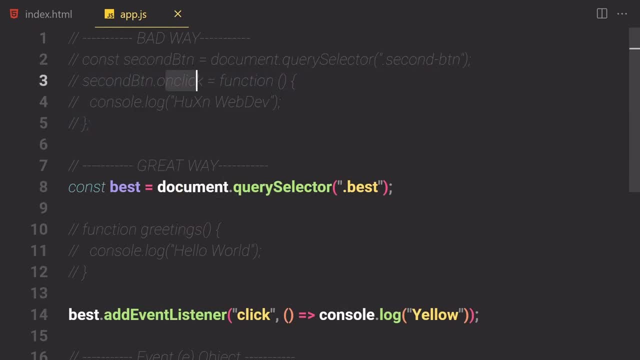 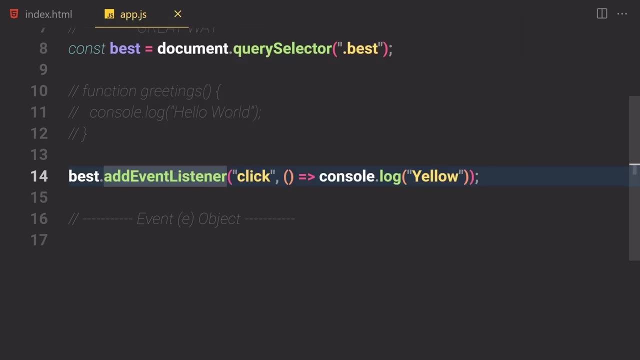 about the bad way, which is that we by using this on click methods, and then we learn about a great way, which is by using add event listener, and this is also a modern one, uh, okay. so let's just comment this line out, and i want to also comment this line out as well. so now let's just learn about something. 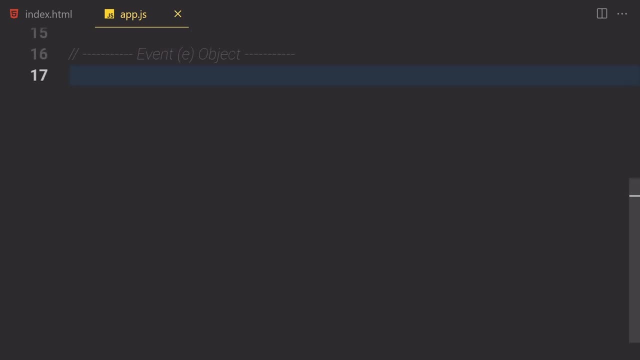 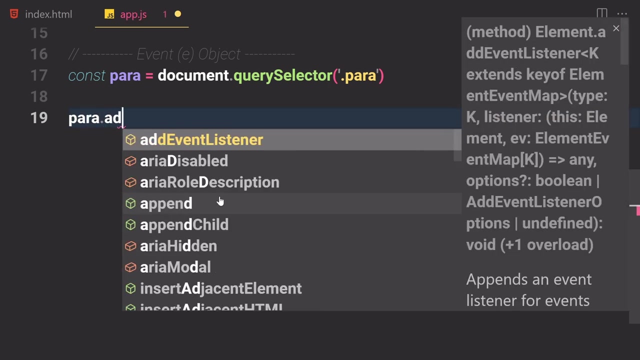 called the event object. so let me just select my para, which is this paragraph right here. so let me just select that. cons para will be now equals to documentquery. selector of para. okay, so now if you want to attach event listener on this paragraph, so we can just use like a para and then add event. 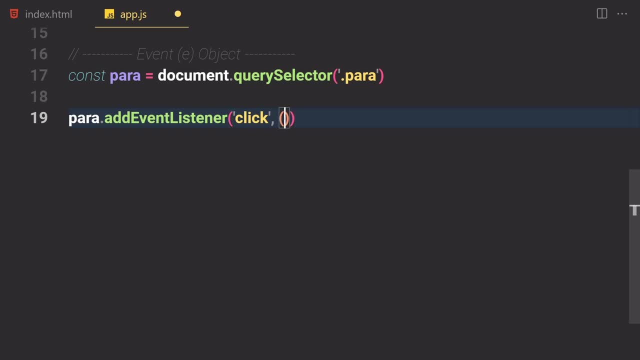 listener and we can just uh listen to a click event and here we are going to be passing our arrow function, but we are going to be also passing our event object right here. so this is going to be a special object. it's not a parameter, it's a special object. so if you just log there to the 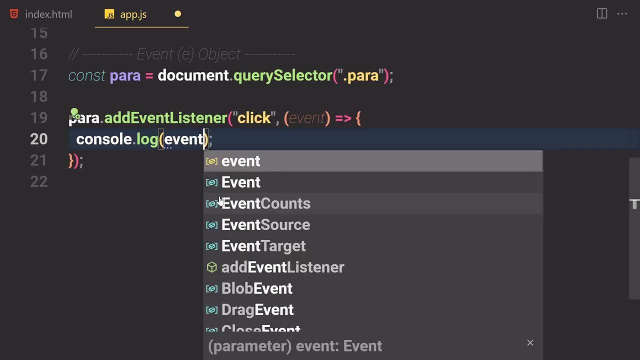 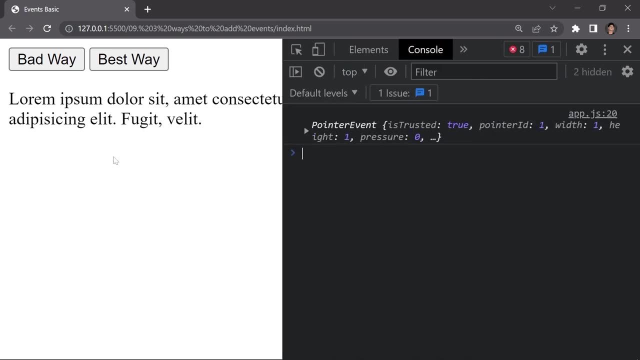 console like consolelog and event. and now if event, to be precise, if you save a file, and now, if you just click on this paragraph right here, so here you can see we are getting this event- uh, pointer event- right here. so this is going to be our event object right here and now. if you just 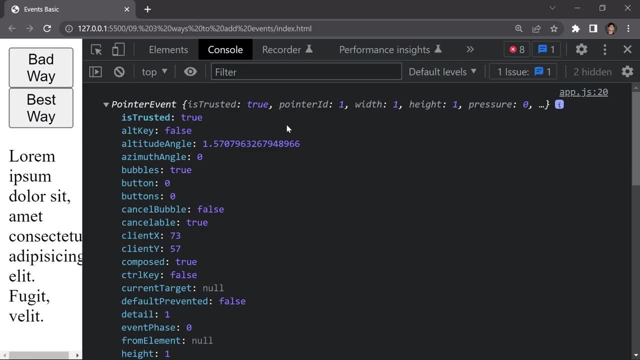 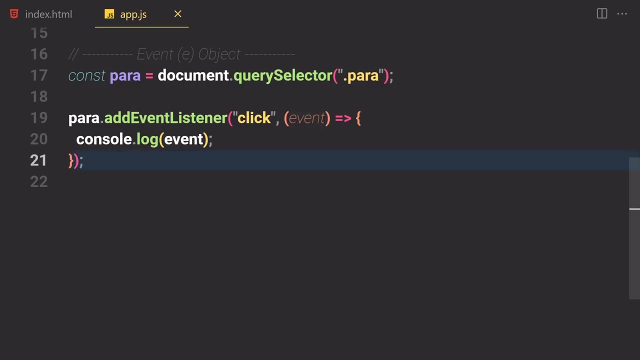 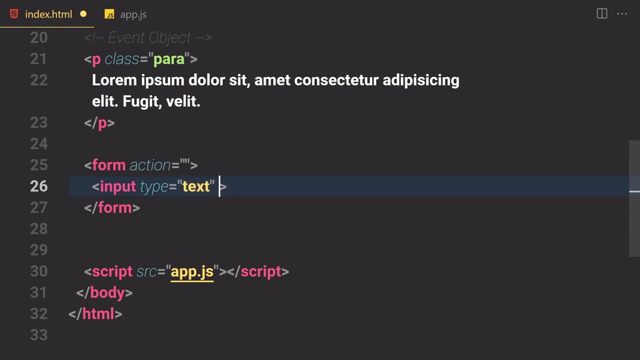 click on this DIE so we have alt key and bubbles and bottom and all of these kind of stuff. uh, let me just use that in some sort of um input right here inside this one. we have an input right here here and let me just give a value of like. uh, oh, you know we're not going to give any value, i'm. 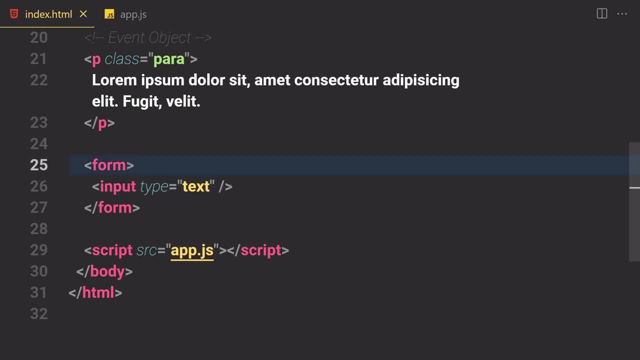 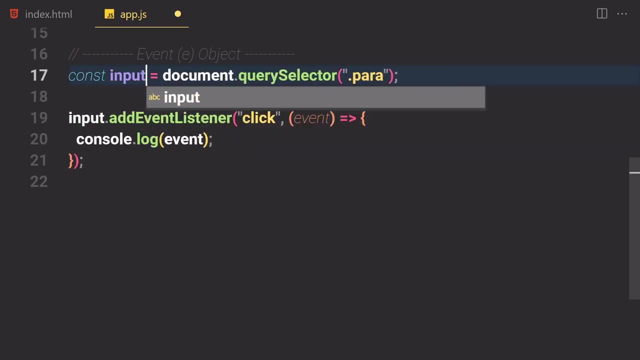 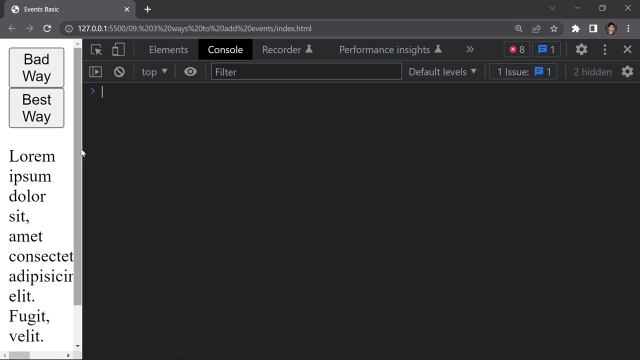 going to remove this value from here and also this action right here as well. instead of that para, i'm going to just get my input and select that as an input and this one will be also a input. so if you save that, we get our input box. uh, right here and we, okay. so if you click on there, so we'll not. 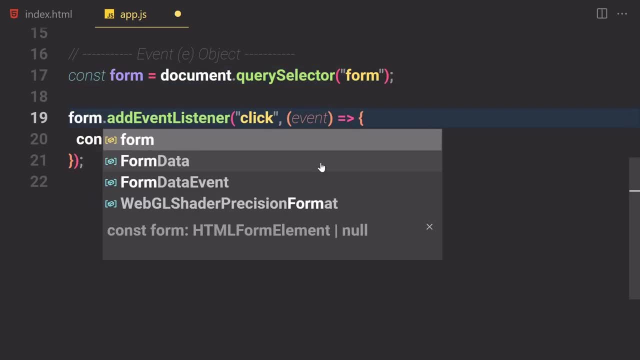 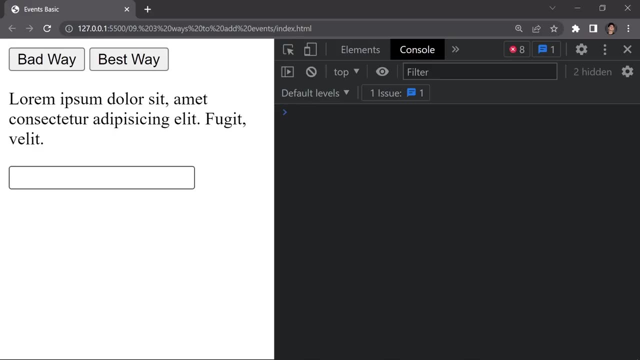 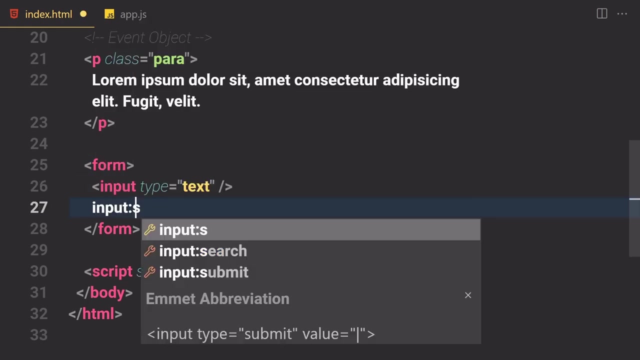 just fire there, let's just write form right here, so let's just save it. and now, once the form is submit, so you want to listen for a submit event, so we have something and we have to create a input of submit as well. come on, man, submit and no value is nothing, okay, so we have to provide. 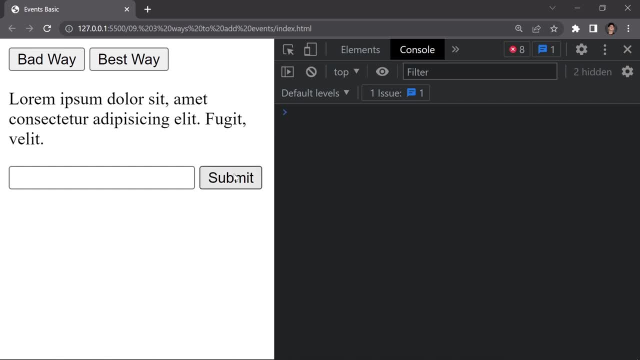 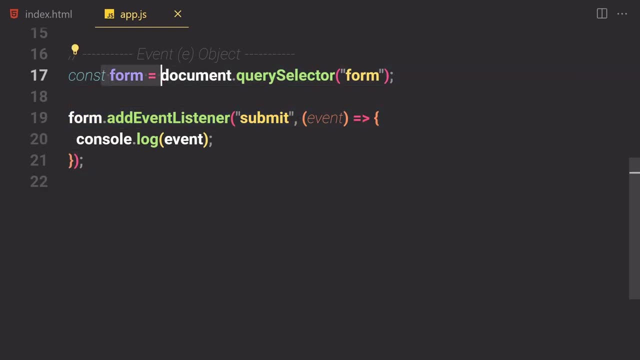 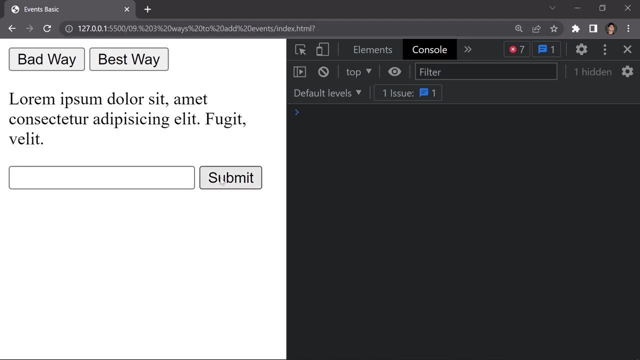 a submit value to it, like so if our form is submit, so it will just uh print something. so all of this code means that first of all, we are getting our form, like this form, right here and we are just attaching event listener of submit, like when our form is submit, like once we click. 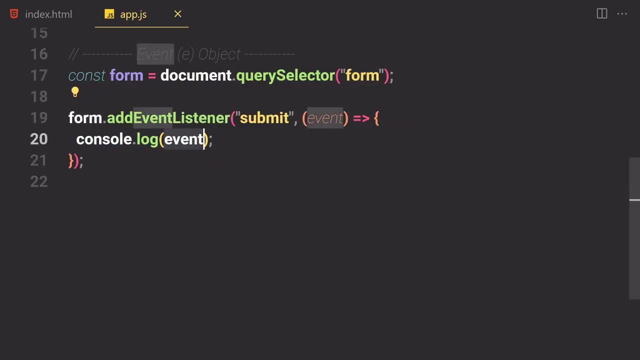 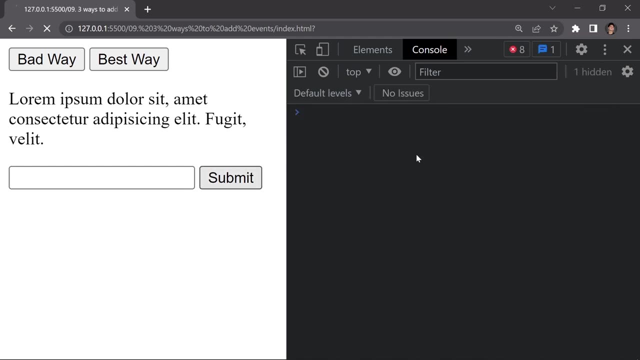 on this submit button. so we want to just print like this event object. but if you just click on this submit button right here, so did you see that? let me just click there one more time. let's just click there. did you see that flash of that event? so there's the form default behavior, like whenever. 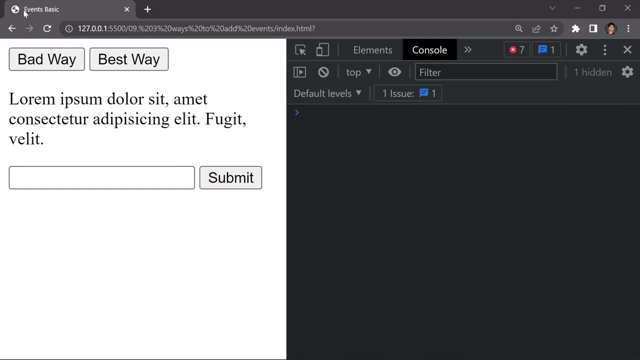 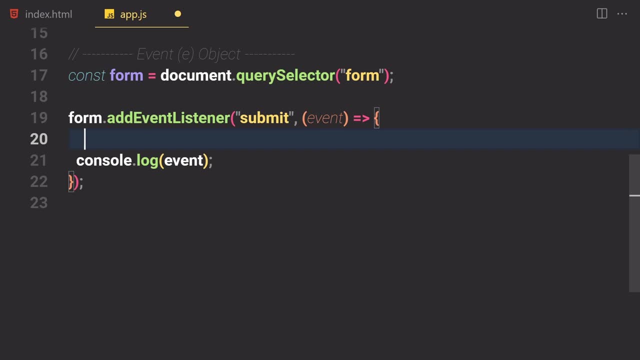 we submit our form, so it will just refresh the event. so let's just click on that and let's just refresh our browser right here. so i want you to just notice this tile and here you can see it will just refresh your browser. so if you want to remove that default behavior of the form, so for that we. 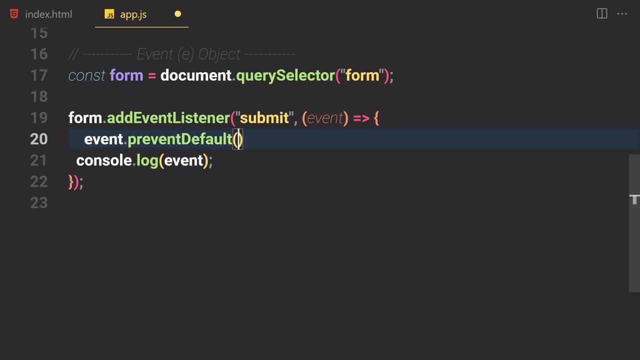 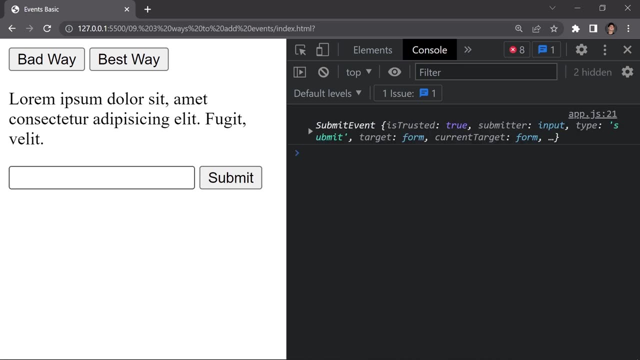 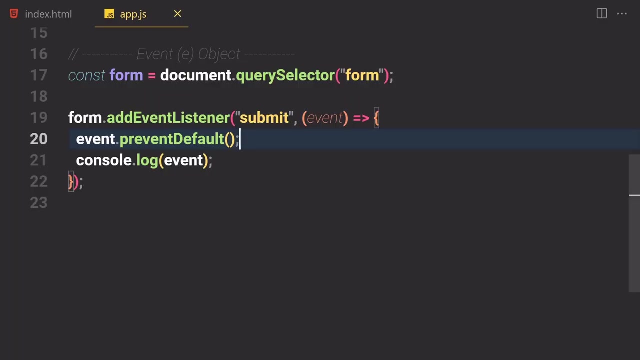 can get our event and then prevent default method right here, so we can use this method and we can just listen for that. and now, if we save that and now if i click on it here, you can see it will not refresh our web browser right here and it will gives us that uh data specific about that submit. 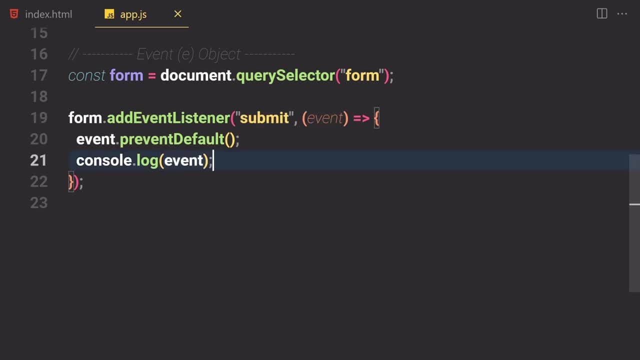 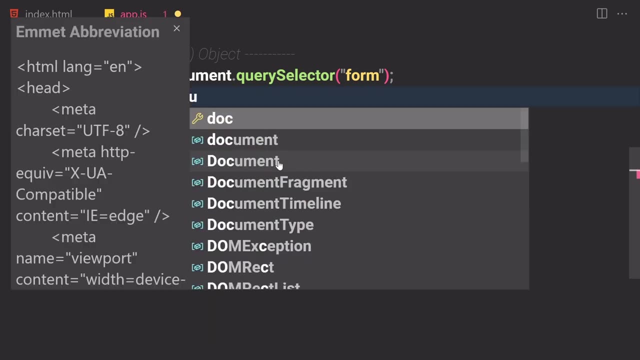 event right here. okay, so we have different methods. so let's just click on that and then we can see we have different kind of events and we can also get a values, if you want to. so let's just get our input area. let me just write const input and it will be now set to documentquery selector. 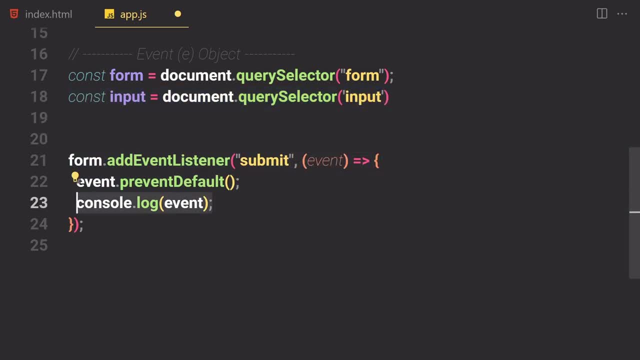 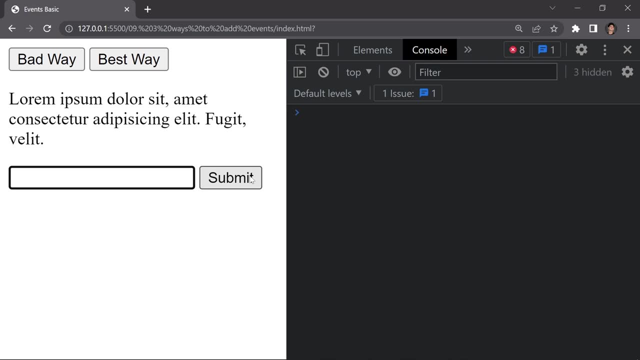 of input. so now we get our input right here and let me just write input and we can also get a value of that input. so if you save that and let me just write apple, and now if you click on the form, and we are now getting apple, if you just write banana and if you click on this banana, it will not. 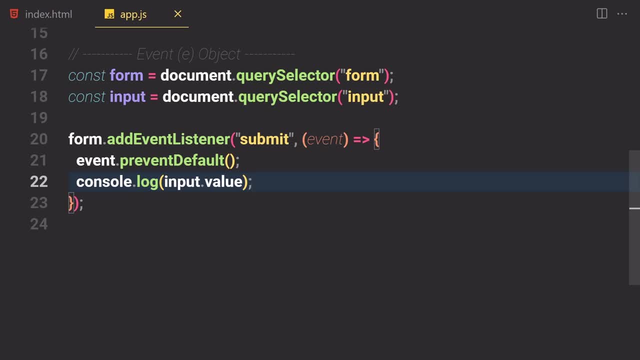 this banana right here. okay, so we can do crazy stuff by using forms and events. so we can also shorten the to instead of writing events. so we can just uh, change that to e and we can also change this one to e. so that's there. let's just uh. you know what we are going to. i'm not going to give. 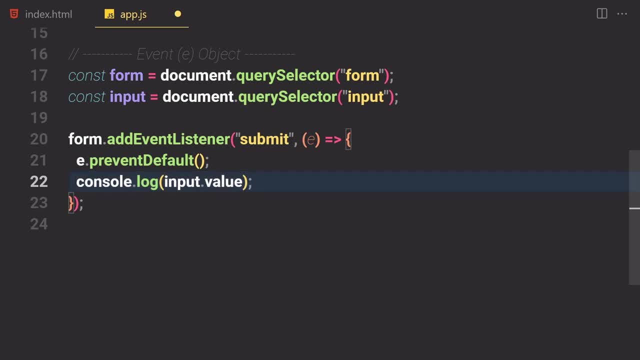 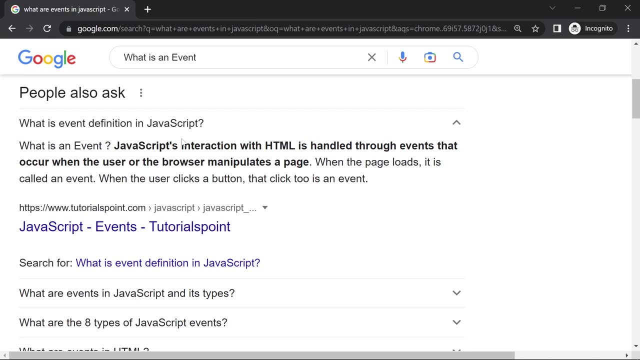 that much of other example, but i guess that would be about how we can attach event listener and what is event. so let me just review that one more time and then we are going to be jumping into different of things. so so javascript interaction with html is handled through events. that occurs when the 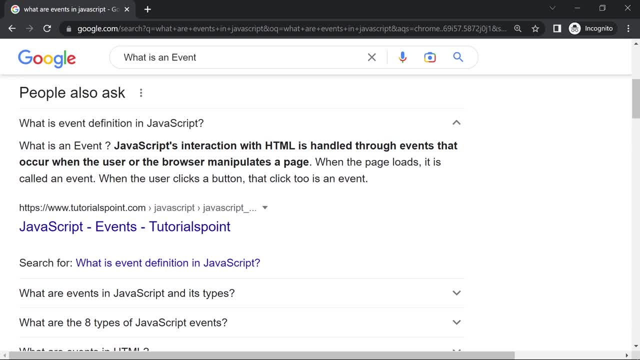 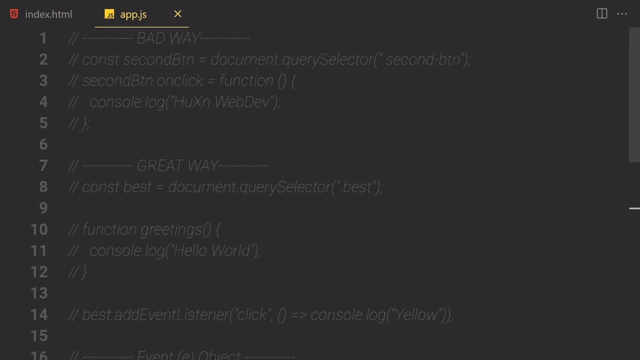 user or the browser manipulates the page when the page loads. so we have different kind of events. for page loads, like dump counter loaded, it is called an event, and when the user click on a button, so there is also an event. so let's just say bye to that page or that site and we learn about a few. 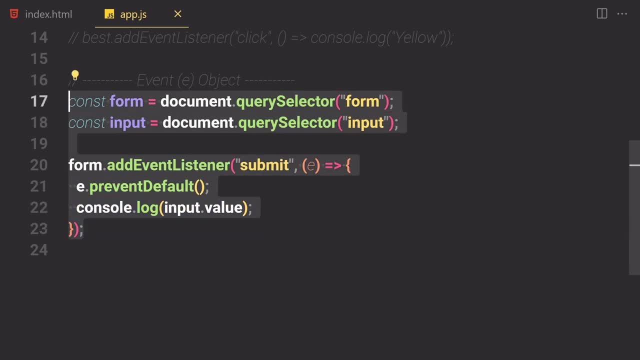 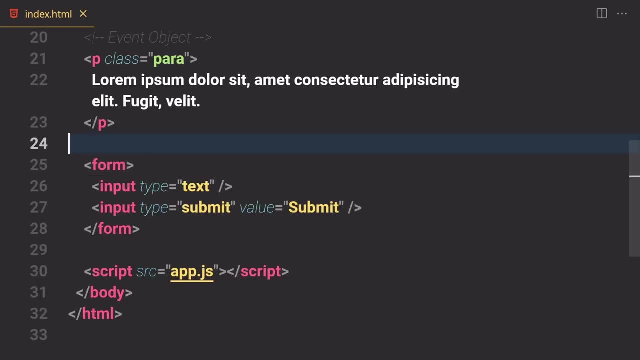 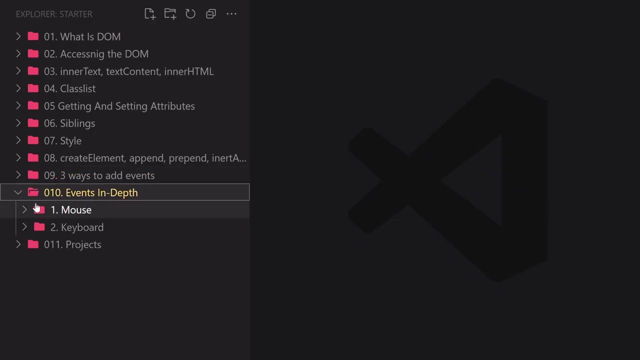 or not a few, but we just learned about three ways to attach even listener, and we also learned about a few other ways to attach event, so let's just say bye to that page or that site. okay, so i guess that would be it for this section, and now let's just get in towards new section. 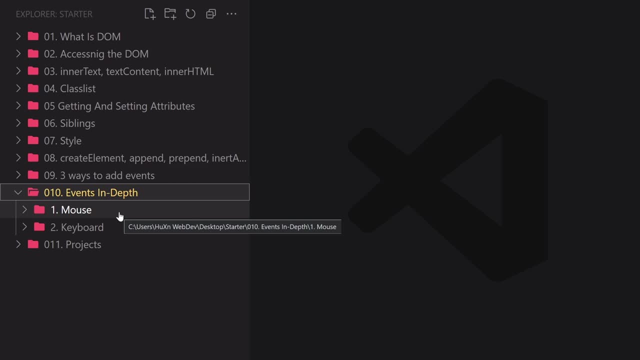 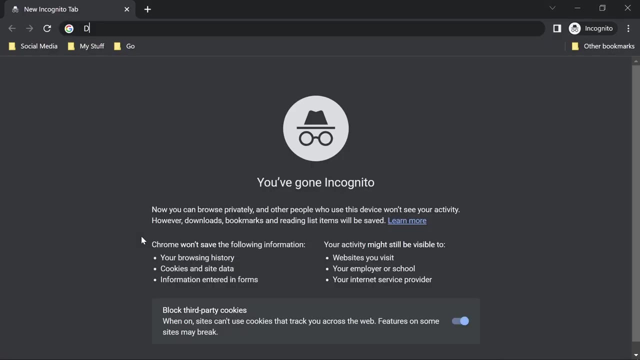 called event in depth. so we have mouse event and we have keyboard event and i'm not going to be going into that much detail. like we have different kind of events for like let's- let's just quick google search that um dumb events. so it will now give us different kind of events. so we have 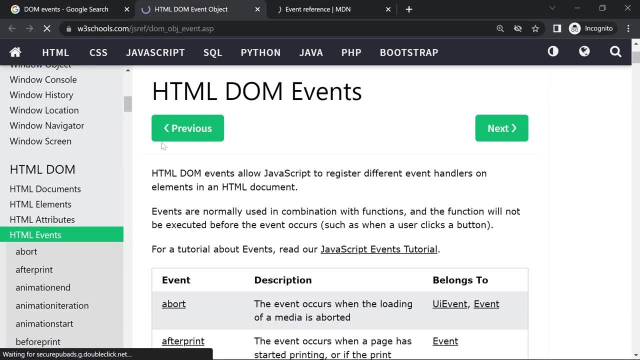 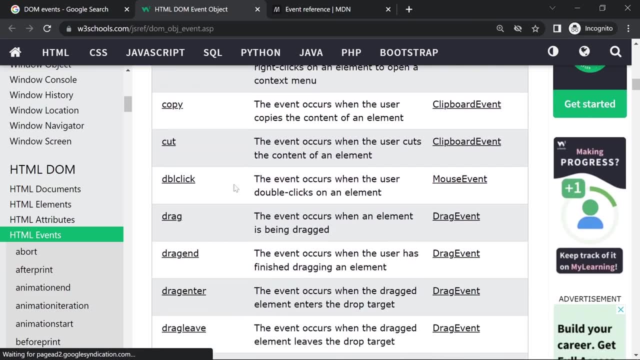 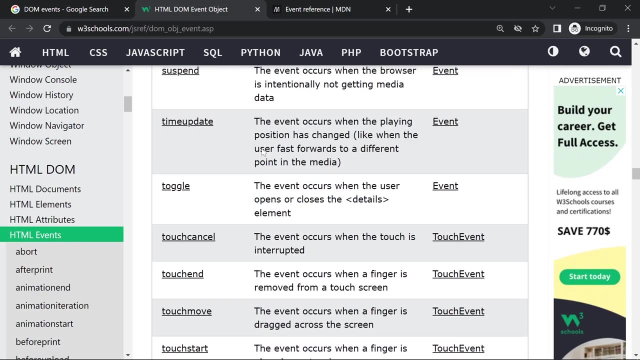 form events. we have keyboard events, we have mouse event. we have a lot of them like here you can see: animation and blurriness can play, change, click, copy, double click, drag, drop, and there are countless events like here you can see. i i can like show you all of them. it will take like. 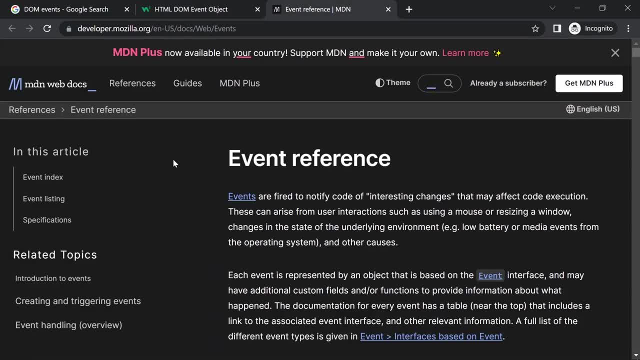 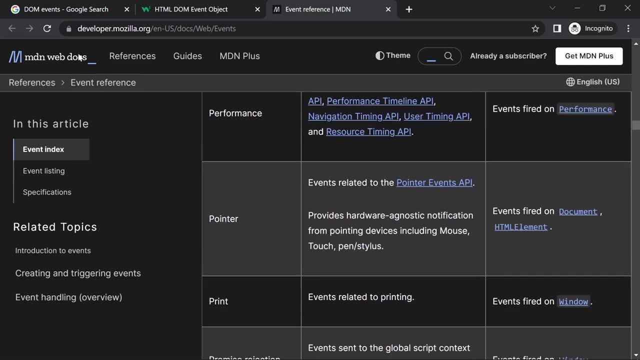 new course to show you all of them, but i'm going to just show you a few of them, like those which you would need in every single day, or not even sing every single day, but one time in a month. so i'm going to just show you the important one and you can explore others if 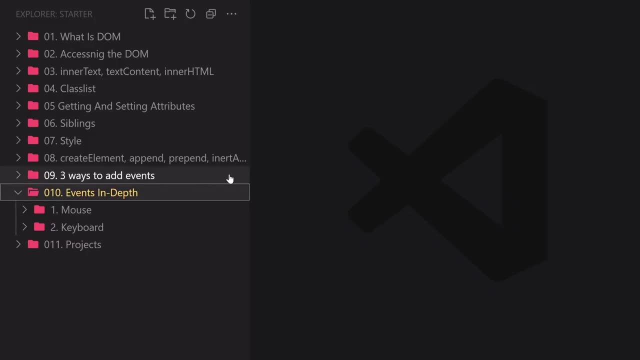 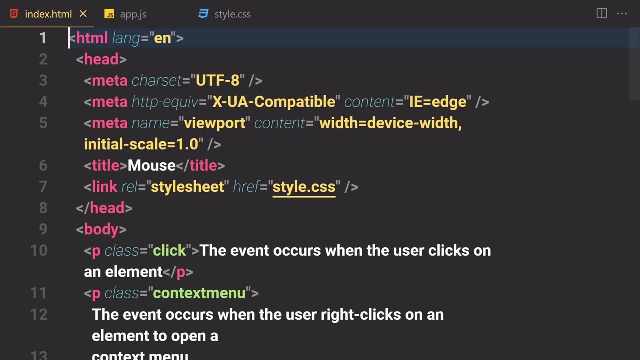 you want to in your spare time. okay, so say goodbye to that one. and now, in this video, we are going to be starting working on our mouse image. so first of all, we have indexhtml file and we have a mouse event. so now let's just collapse this area. so first of all, we have 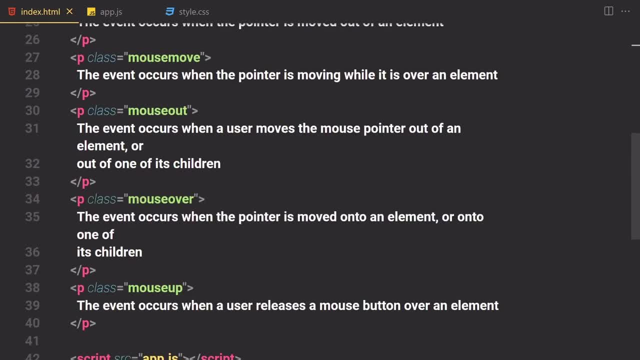 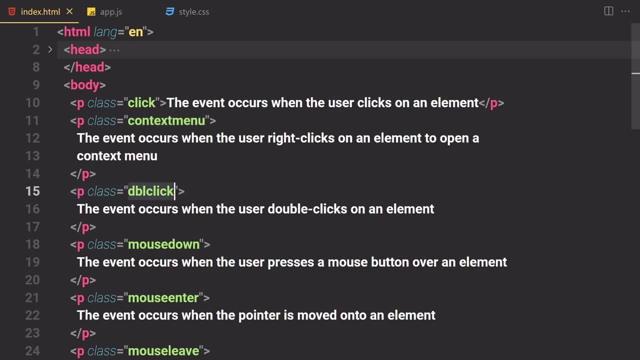 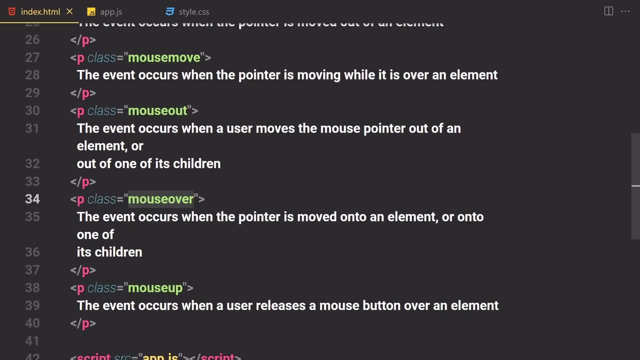 our body. then we have a paragraph, not one, but we have a lot of paragraphs inside there and we just give a classes of different kind of events, like click and uh, right click, one double click, mouse down, mouse enter, mouse leave, mouse move, mouse out, mouse over, mouse up, for different kind of events. 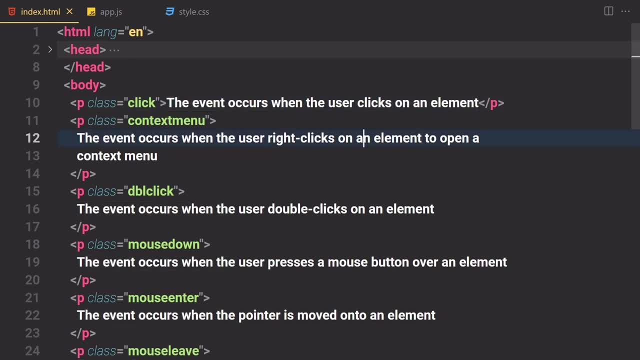 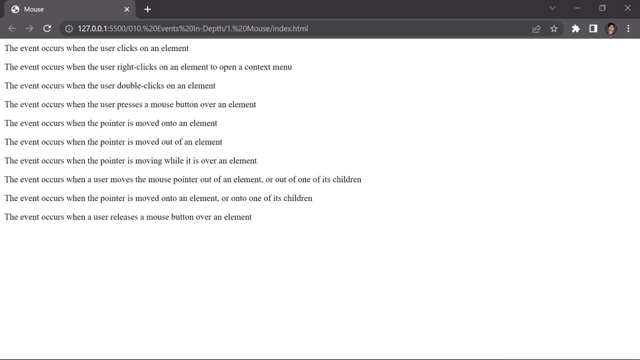 we have different kinds of uh definition of them, so i'm going to right click on there and open it with the live server, and this is how everything looks like right now. i'm going to open my dev tools as well. all right, so we have our definition for the first one. 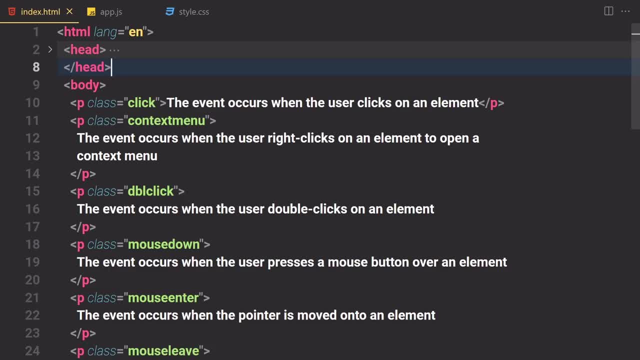 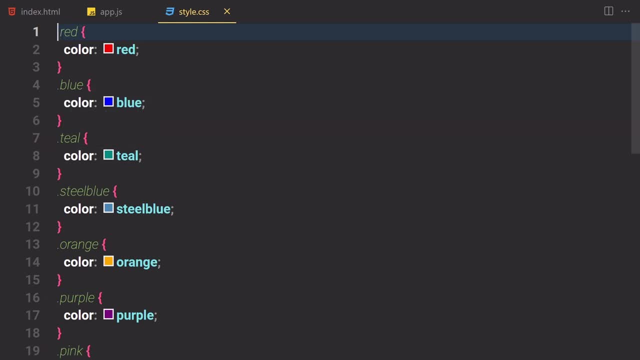 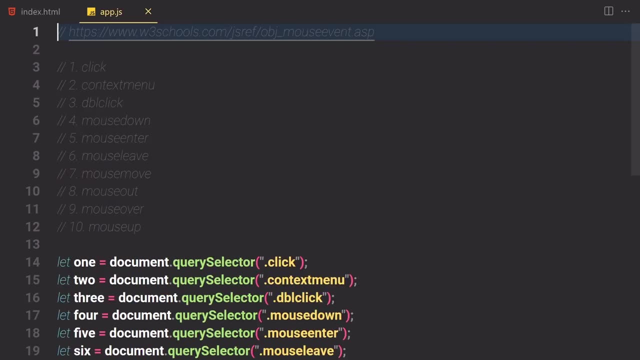 event occurs when the user click on the elements. so let's just start working on that. and, by the way, we have a few colors like red, blue, teal, steel blue, orange, purple, pink, crimson, chocolate, aqua, so we have different kind of uh colors right here, so we are going to be using that. 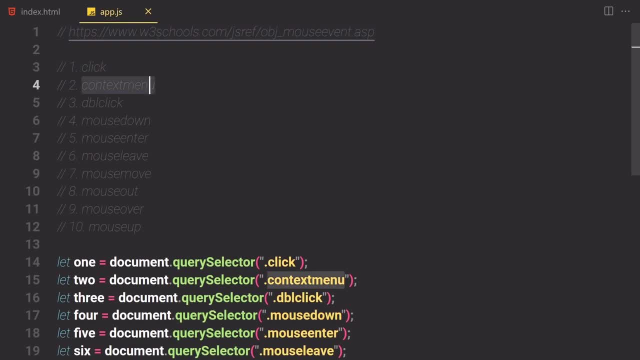 uh, in or appjs. so we have click event, we have context menu, double click, mouse down and all of their events which you are going to be exploring in this video, and we also have a reference. so like all of these events came from this w3 school, so if you want to go there, you just have. 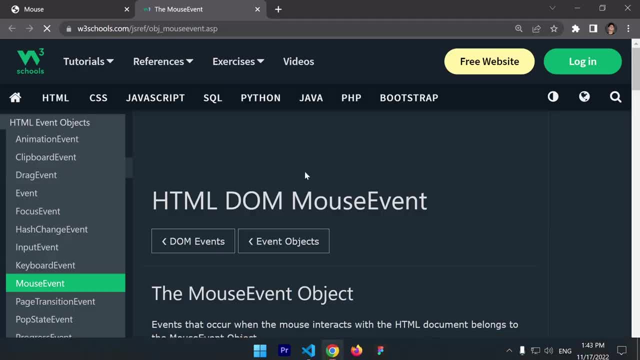 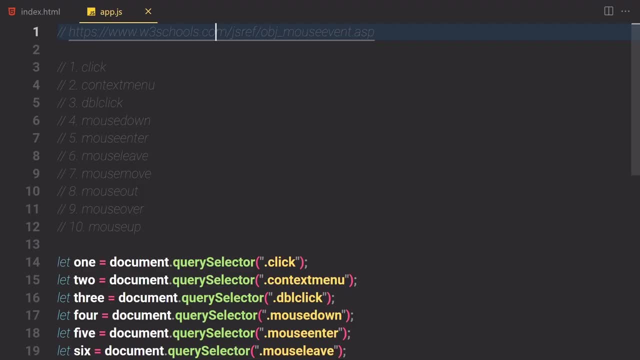 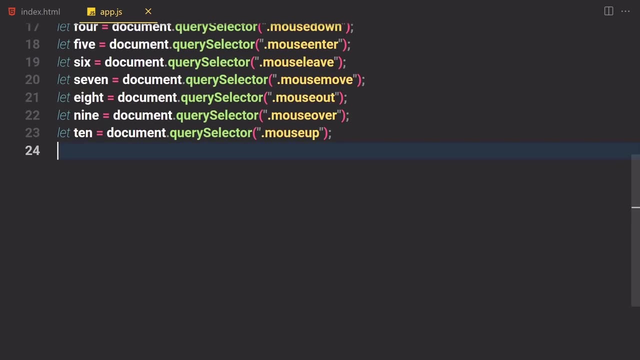 to hold ctrl and click on this link so it will just open it right here inside of google chrome for you. so if you want to learn more about this, you can in your spare time, but in my case i'm going to just show you all of them one by one. so let's just attach event to our first element, like: 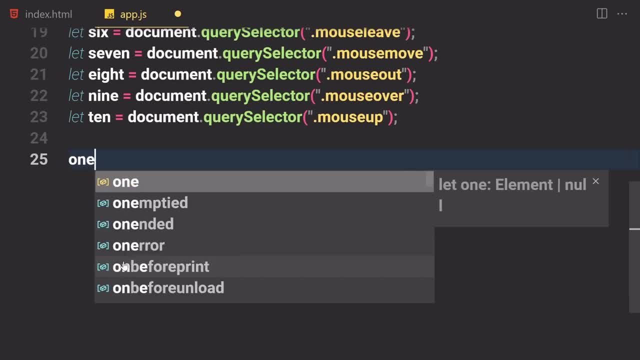 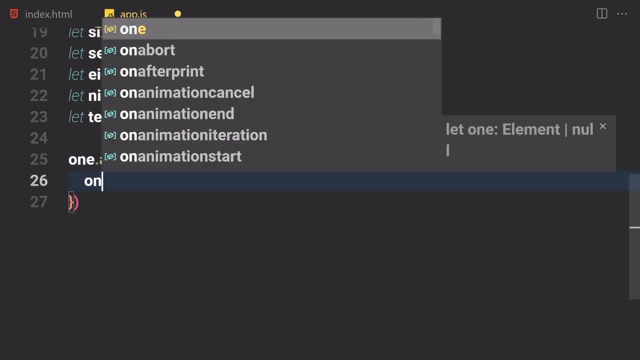 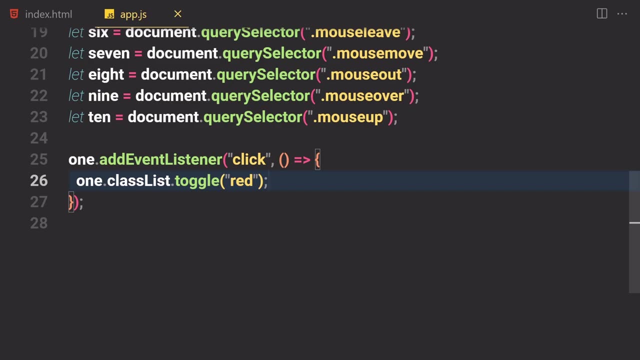 one. so i'm going to zoom in a bit and i'm going to just write, like 1.8 event, listener off, click, so clicks on that element. so what do we have to do? on or not on? but one, not class list dot toggle, and we want to just toggle this right. so now if you sell file and now if you click on this element. 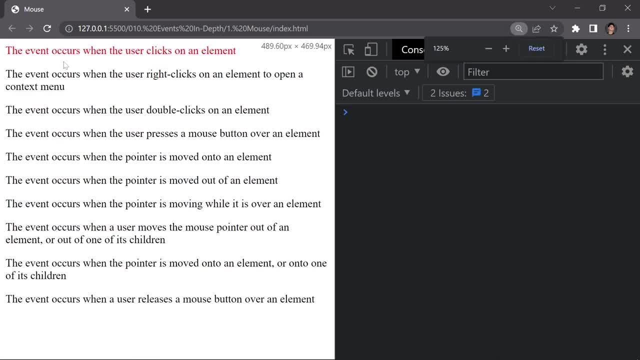 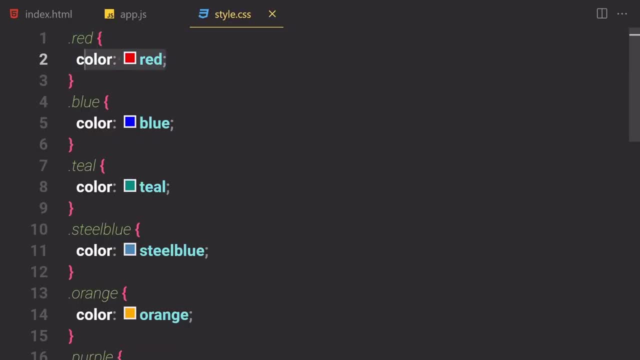 right here. so here you can see that text color is changed to red. that's because we are toggling this red clause and we have that red clause right here inside or css file right here. so we are just toggling this class and we are going to also toggling the other classes just in a second. 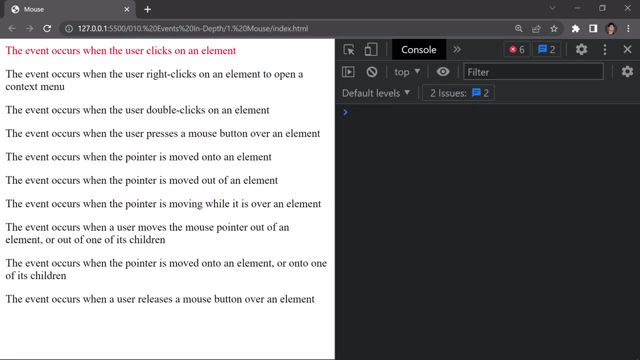 all right so so that was quite simple and easy. so like, if somebody clicks on the element, so this event will fire. the next event we have is that when the user right click on the element so to open the context menu, so we have that one as well. so let me just write two dot add, or, you know, i don't. 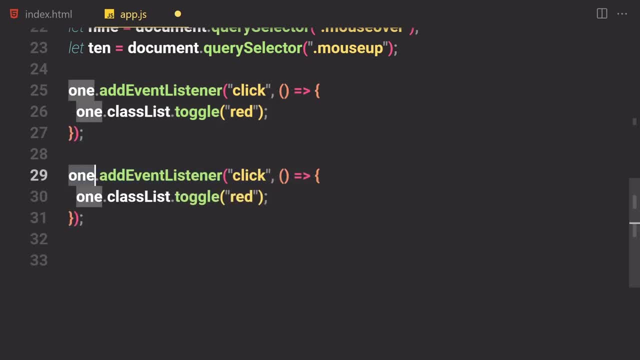 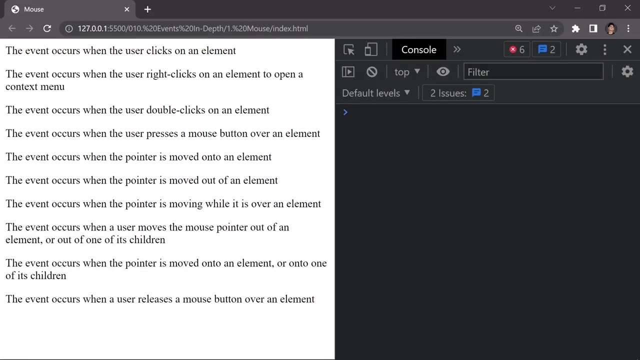 want to waste your time, let me just duplicate that. change these two to like two. and now let's just change the event name to be context menu. okay, so we want to attach or we want to change the color. so if you just save our file and if i just click on there, can you listen to that? if i just click on. 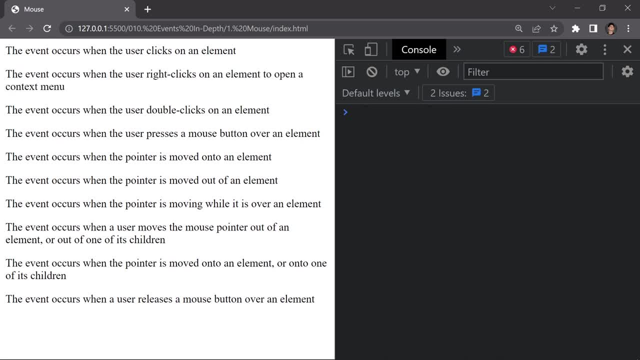 there, nothing will happen. but if i just right click on it- so here you can see- it will now change the color to that kind of a blue color. so if you just right click on it one more time, it will just toggle that class again and again. so if you just right click on it and now- here you can see, it will just 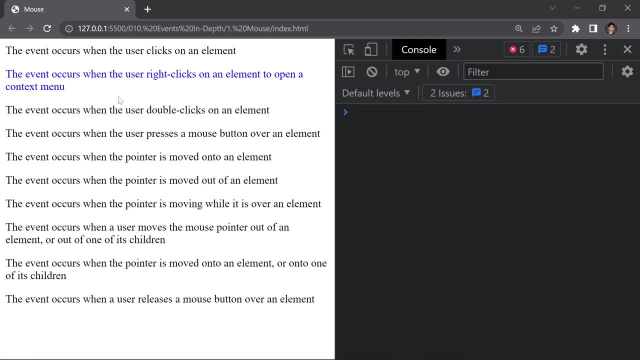 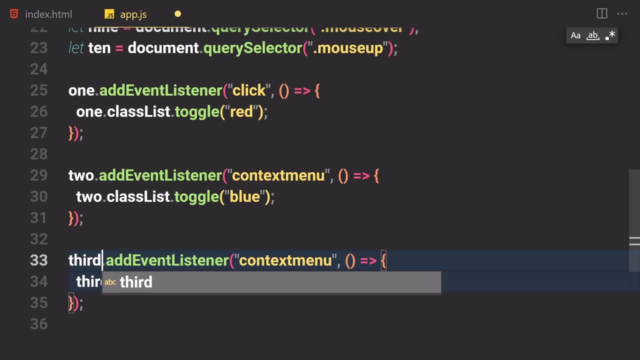 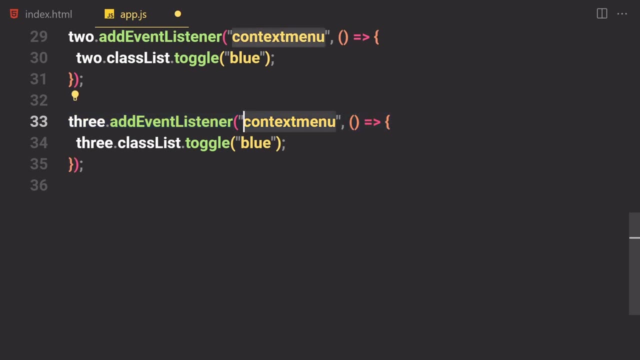 work like that: right click on it and it will just attach or fire that function. so let's just duplicate that one more time and change that to the third. one, third is that third or three? okay, so three, three, and change the event name to what, uh, dbl, and click. 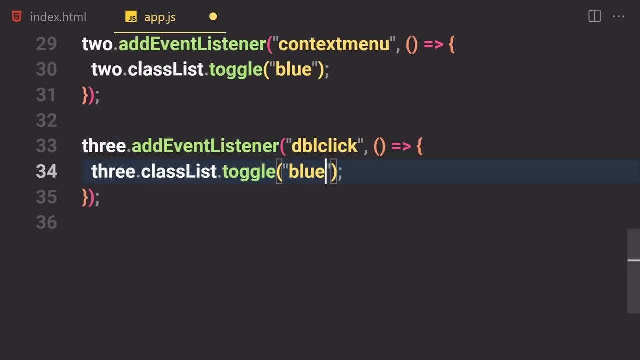 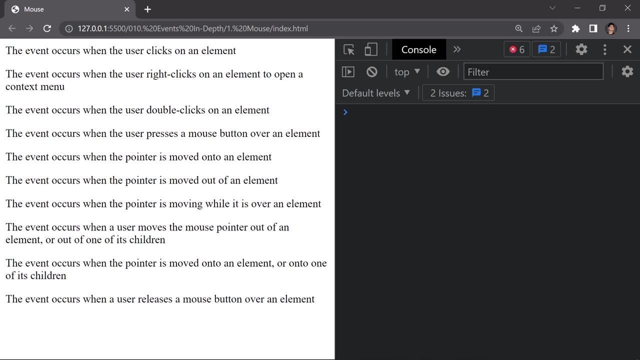 uh, as the name suggested, it will just um if you use a double click on there. so then this event will fire. so change the color to teal several file. if you just click on it one time, nothing will happen if you click on it double uh time like double click on it. so here you can see this event. 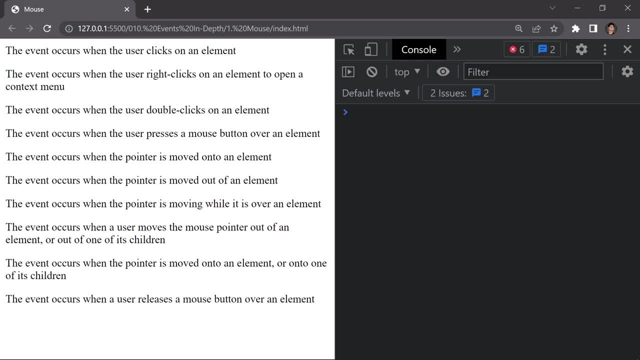 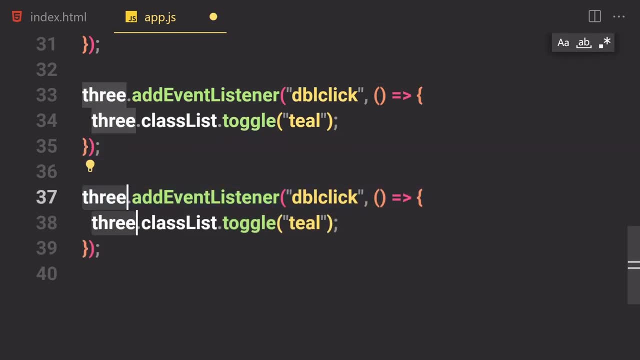 gives this kind of a teal color if you double click on it one more time so that class will be gone because you're doing toggling. let's just duplicate that one more time and change that one to what? four, and also change the event name to mouse down and also change this color to be steel blue. 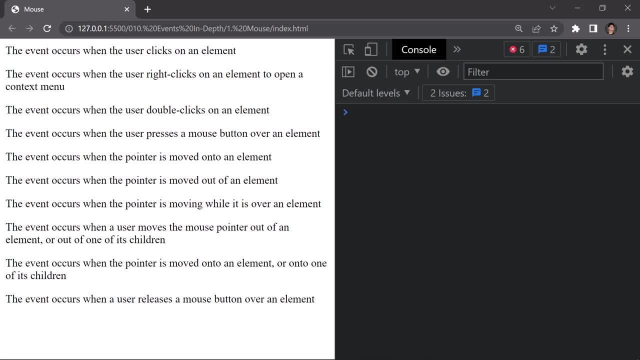 and now, if you several files, so first of all, let's just learn about that. even a curve, when the user presses a mouse button over an element, if you just click on it and then you can see that it click on it, so here you can see this will and this event will fire. it's kind of like a click. 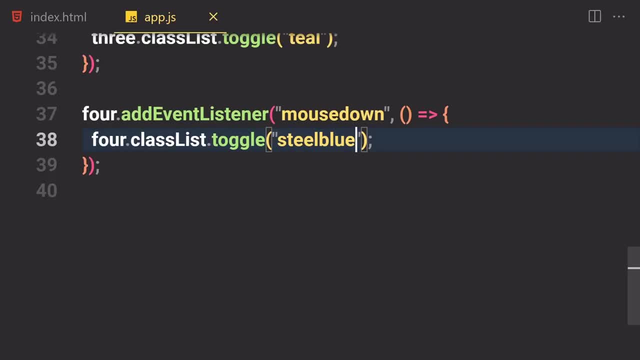 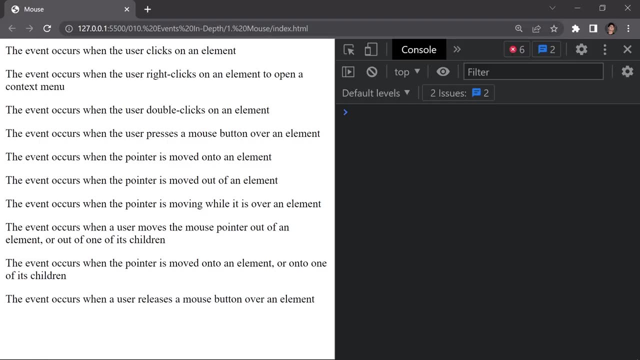 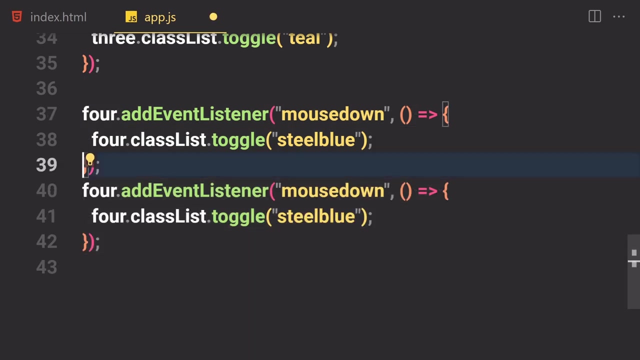 event. but this is another way to use the mouse down. come on, man, all right. so then we have another one, which is the event occurs when the pointer is moved on to the element. and this one, and i guess the mouse move, or both of them are the same. let me just show you that one by one. so we have a four. 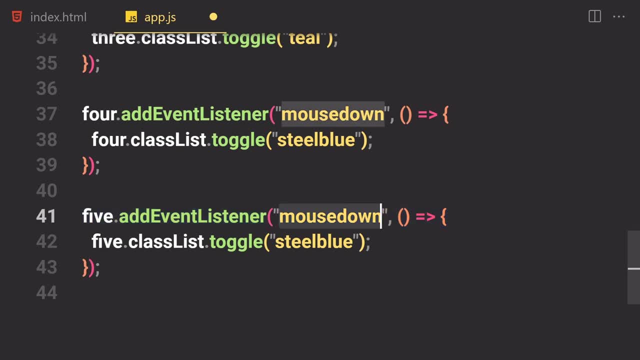 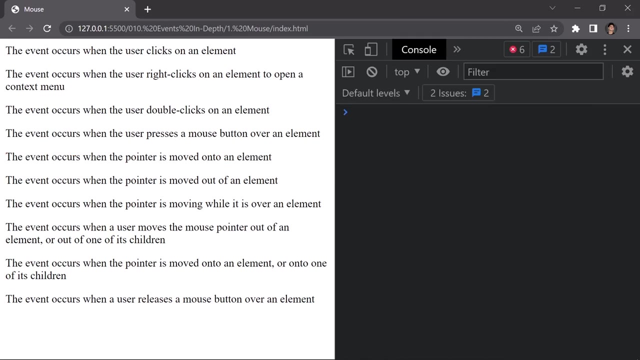 then we have a five and let's just change that to, instead of mouse down, we have mouse enter, like so, and change the color to be orange and save our file. so what do we have? okay, so once i hover my mouse over to it, it's kind of like a css hover once you hover your mouse over to it. so 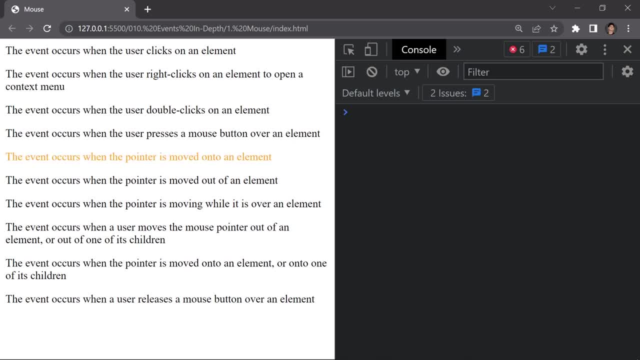 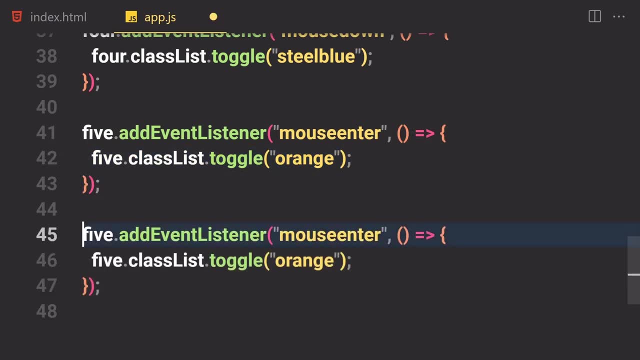 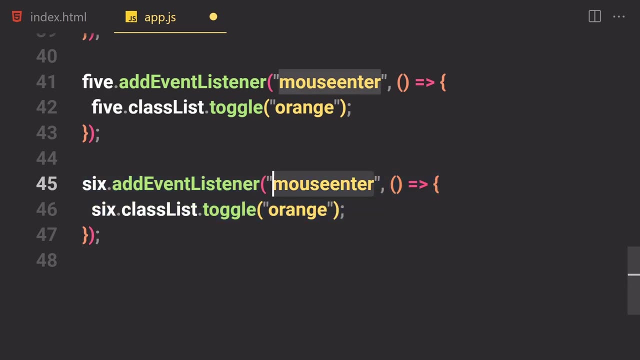 something will happen. so in this case we are doing a toggling. so this what's happening right now? okay, so so this is a mouse enter- it's kind of same like a hover one- and let's just change that to six, one, so sixth- and also change this event to mouse leave. so let me just write mouse leave and change the. 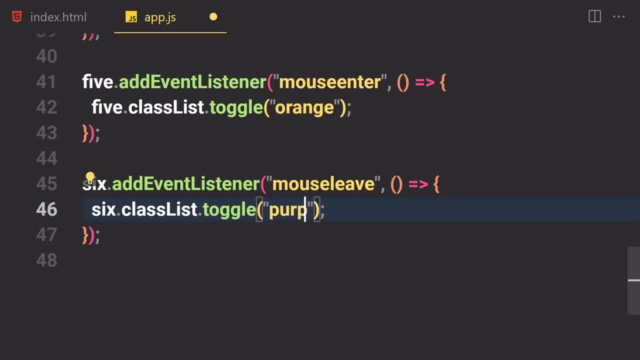 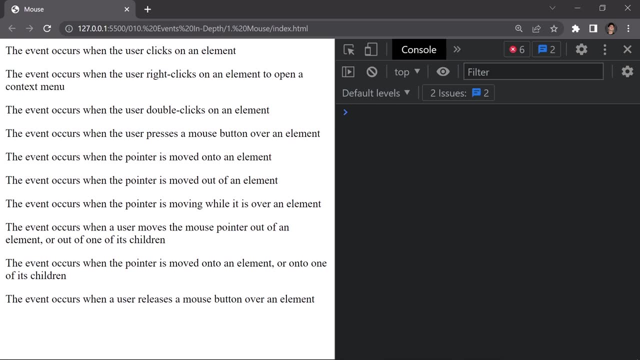 name or not a name, but the color to purple, purple, like so. and now, if you save there, if you just hover mouse over to it, nothing will happen. but if you just mouse leave here, you can see that event will fire. and if you just hover over it, 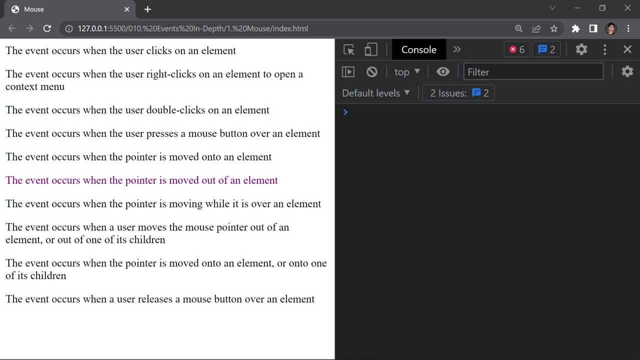 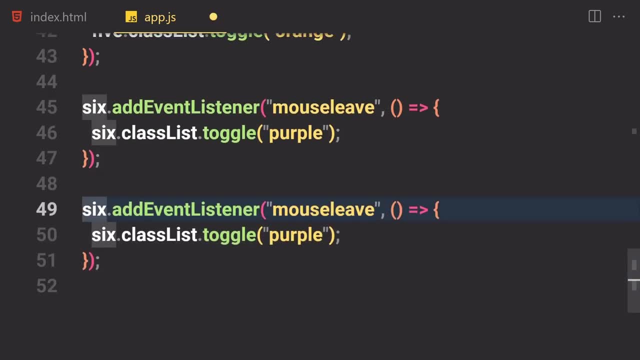 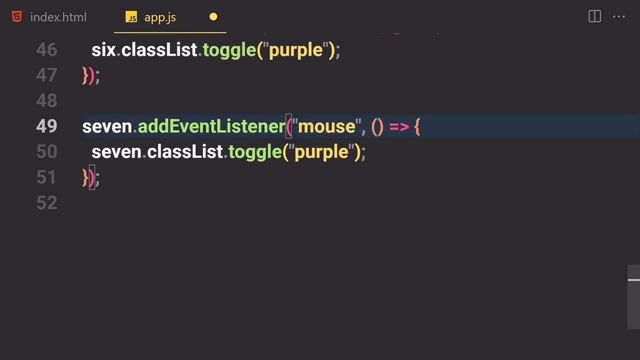 that event will. nothing will happen. but if you just hover mouse out like mouse out, so this event will fire. okay, so let's just duplicate that and you can learn more about that in your spare time. and s-e-v-e-n mouse move and mouse enter, it's kind of like the same one mouse move. let me just 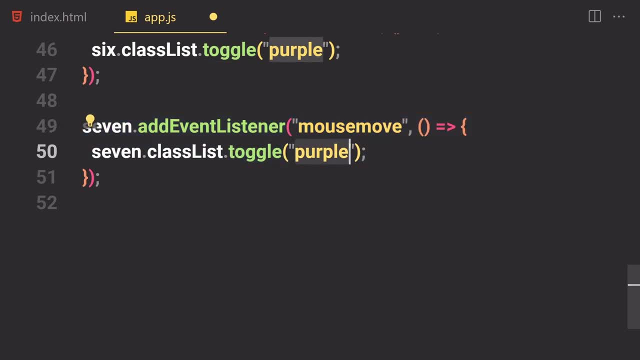 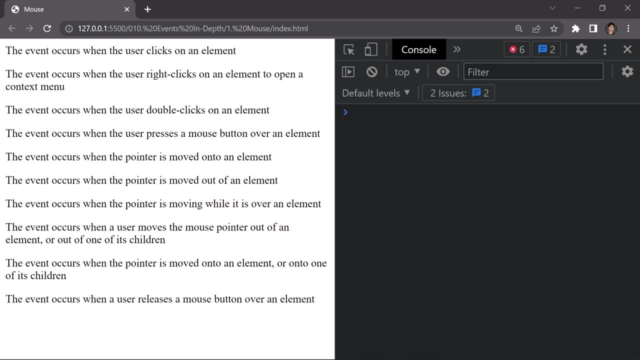 show you that one as well. so we have purple, we have a pink. so if you save that, and now if you move, not that one, so if you mouse move, so first of all, if you mouse smooth, so it will now take this pink color. if you mouse out, so it will. 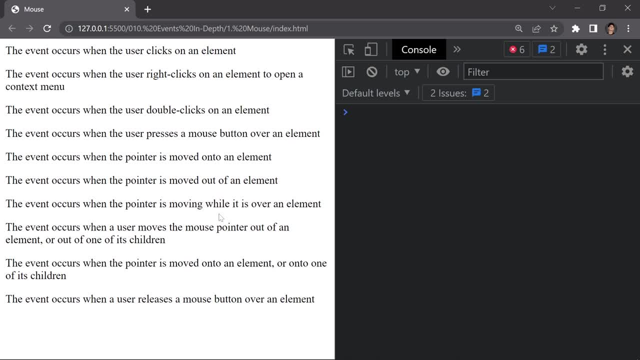 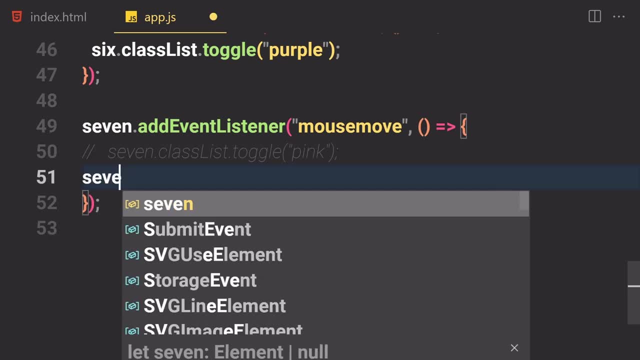 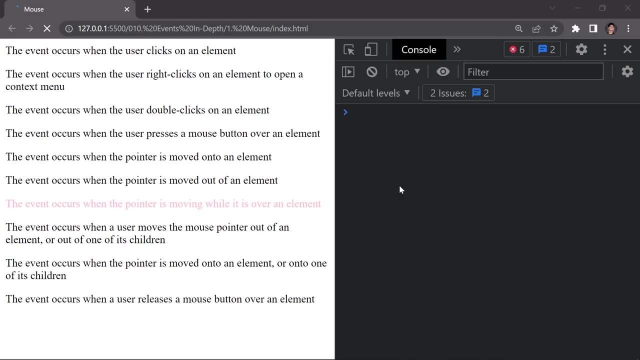 just remove that color from it. that's because you are doing a toggling, and this is how everything looks like. you know what? instead of mouse move seven, let's just comment this line out seven. now come on seven dot text content. let me now set to hello. and now, if you save that, 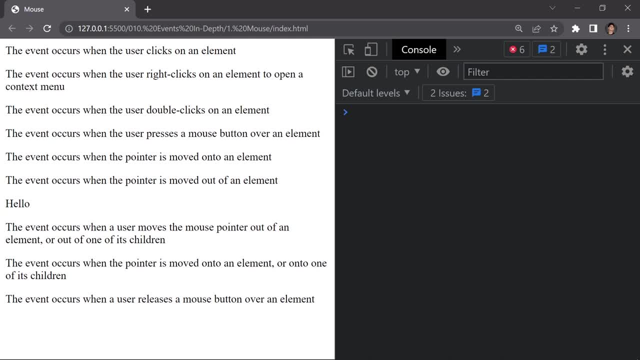 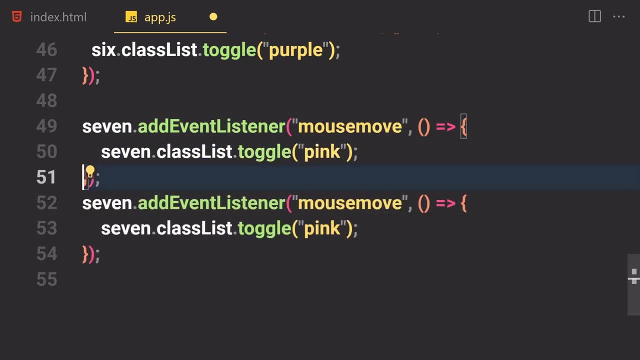 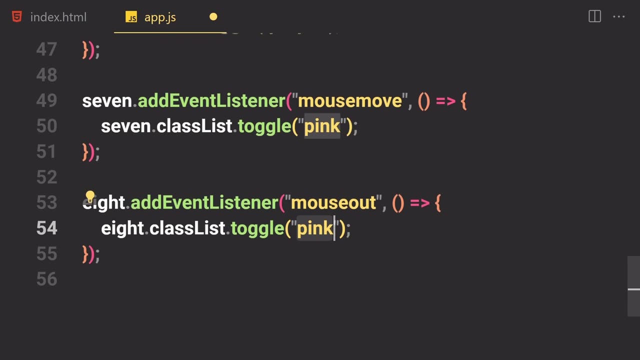 and now if you hover our mouse over to it, it will not give us that hello. all right, here i'm gonna comment that one, cut that one, to be precise, and duplicate this one, and then we have a eight. also change this one to mouse out. so once we mouse out it's kind of like the same one. so 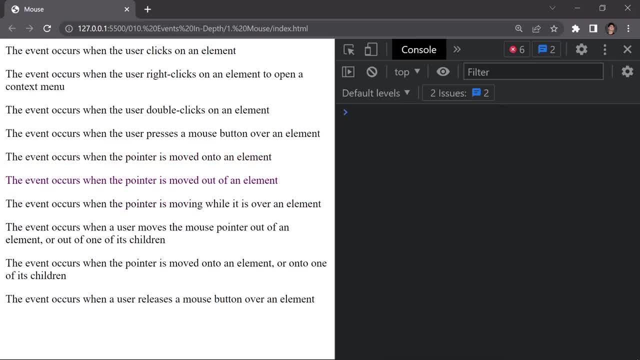 change the crimson color to be crimson, so this one, not that one. so once we mouse up, so let me just refresh this page. and now, once we hover our mouse over to it, nothing will happen. if we just hover it back and this event will fire like so nothing is happening. 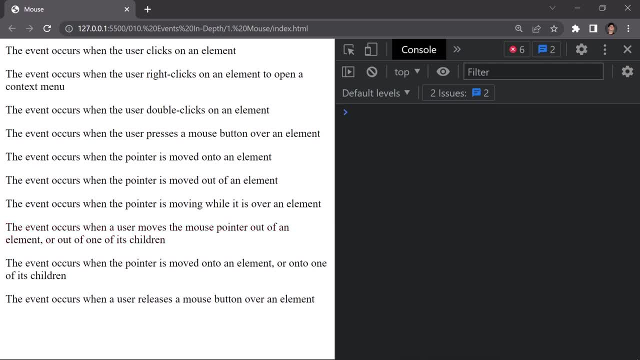 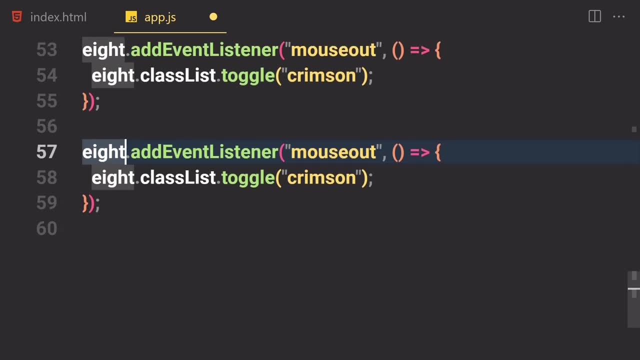 uh, if you just go back, so that event will fire like: so okay, so you can just play around with that if you want to, but all of them are the same kinda. so let's just change that one to nine and mouse over, we already learned about, uh, c-h-o-c-o-l-a-t-e. 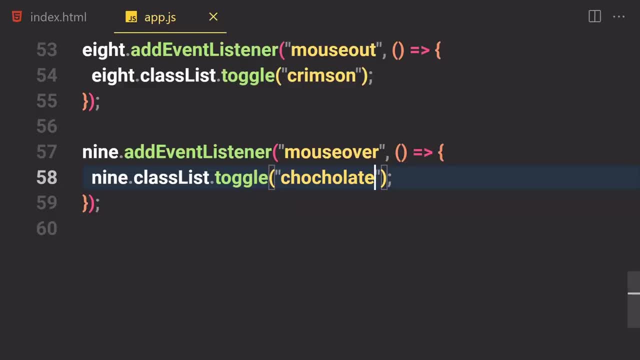 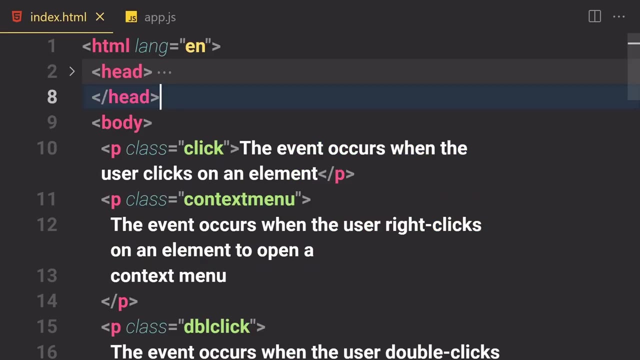 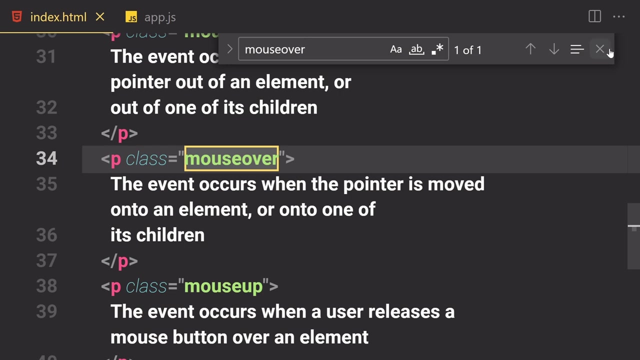 why did i include that again and again? once we mouse enter, is that a mouse enter, m-o-u-s-e over? okay, this one is not working. n-i-n-e, n-i-n-e okay, so mouse over. uh, mouse over, okay. so we gave a class of mouse over and we swore that in the ninth one. 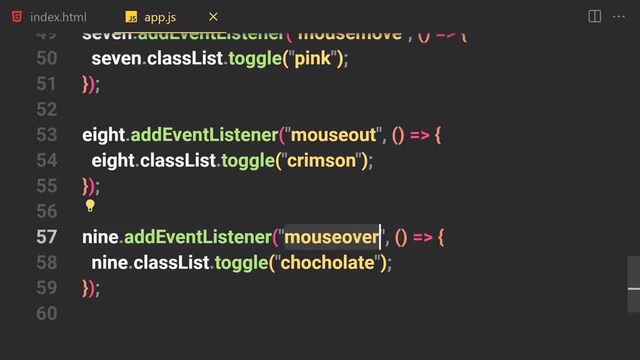 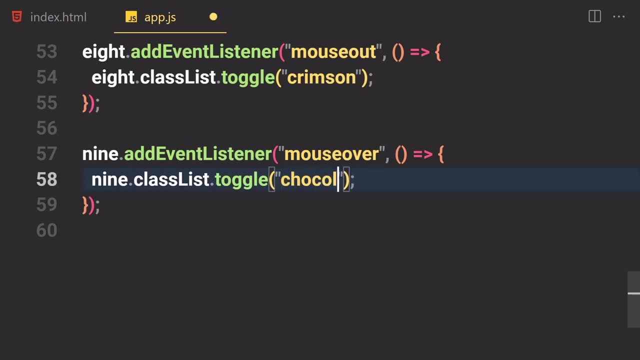 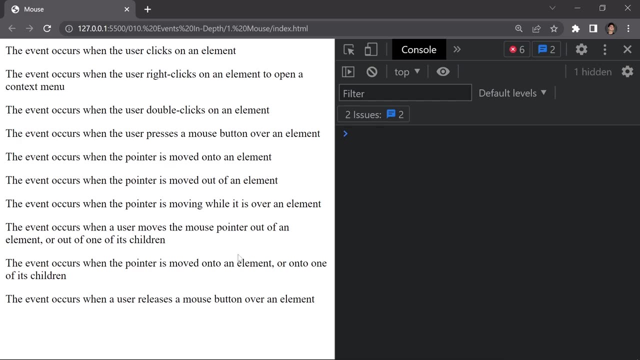 and i-n-e mouse over and we just toggle the clause is c-h-o-c-o-l-a-t-e like. so now, if you mouse over it, so everything is working that way, we expect him to work, and then the final event we have is mouse up. it's kind of a stupid one, i don't know. 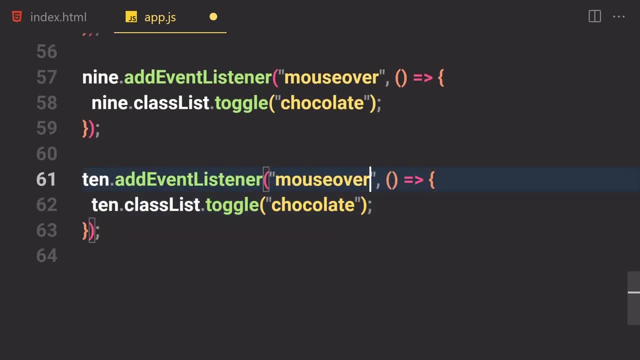 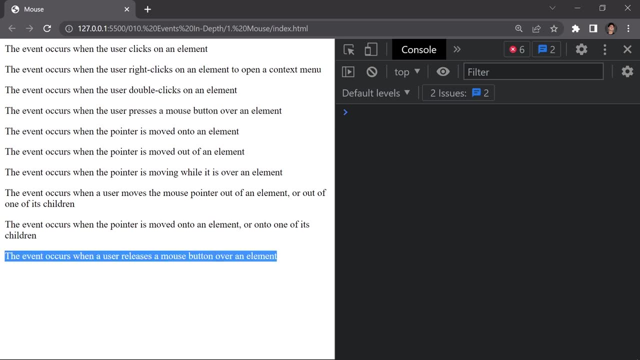 why people would create such an event like that 10 and then mouse up: all of them are the same. you know aqua, and now if you click on it, so here you can see, all of them are kind of the same, like i mean, like what's the point of just making two events like sam, click on this, one click on that. 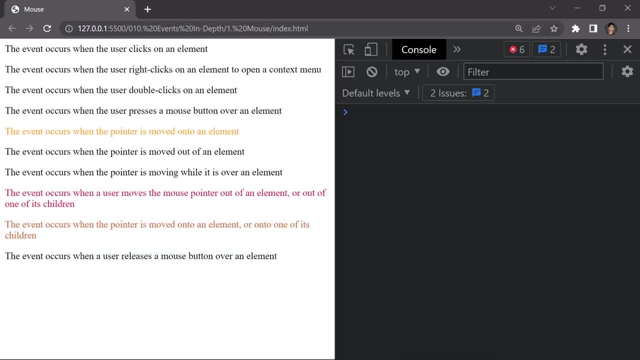 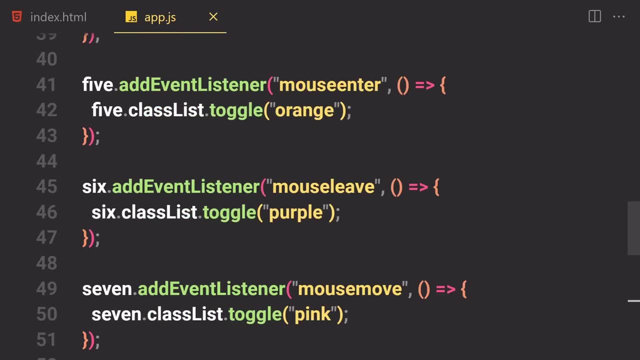 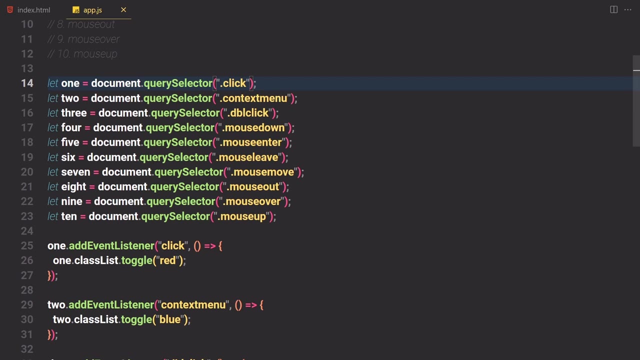 one and it will do the same thing. the event occurs when the user releases a mouse button or an element. okay, we have to click on the kind of a stupid anyway. so that was or um mouse event. so we have or click. then we have a on context click menu. then we have a double click: mouse down, mouse enter, mouse leave, mouse. 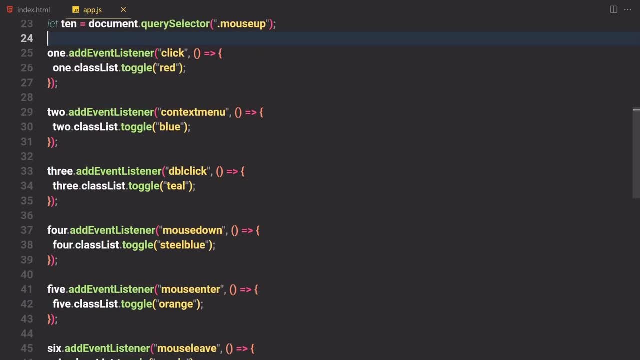 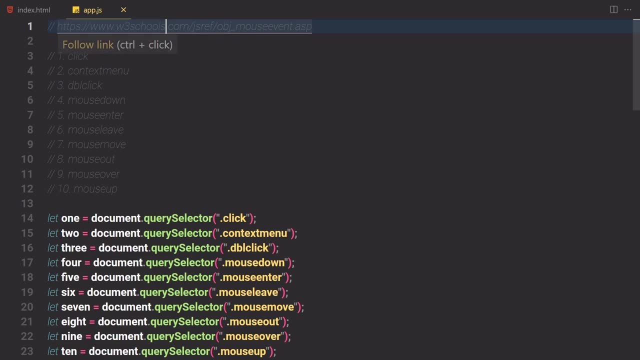 move mouse, mouse out, mouse over, mouse up. so we have different kind of events and we already learned all about that and if you want to learn more, you just have to hold control and click on that. it will bring you to this w3 school documentation and you can even learn about. 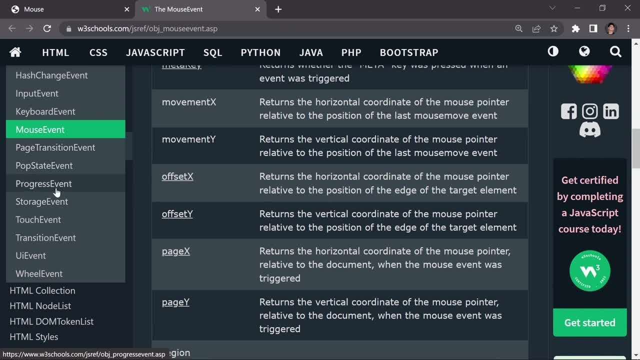 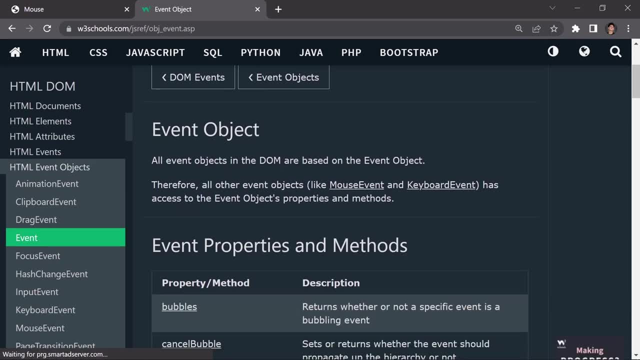 a transition page, transition event- you can learn about a pop stat event, progress, and there are countless of them. if you want to learn more about that, let's just click on this one and all, even objects of the dome, are based on the event. blah, close that one. close that one as well. 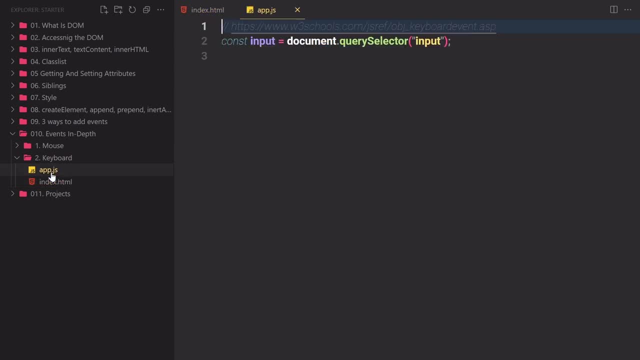 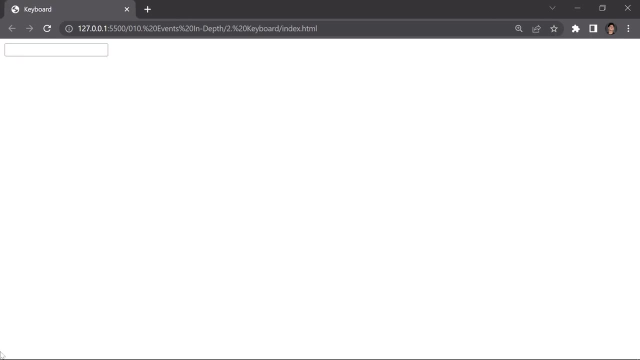 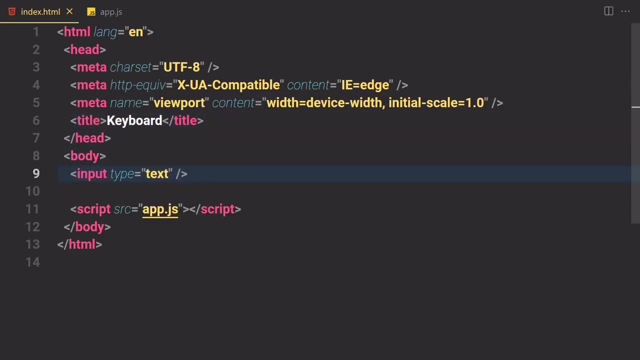 and now let's just learn about a keyboard event. so i'm going to launch my indexhtml file, right click on it and open it with the live server and open our developer tools right here, or dev tools, and let me just zoom into it. inside this body, we just have our input with the type of text and we don't have nothing special in our html. 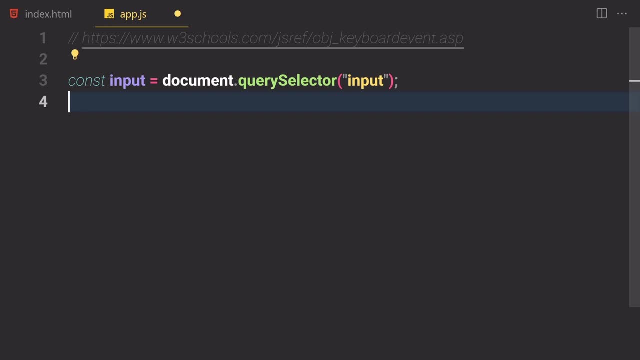 okay, so we just have a link. you can learn more about the keyboard events by going to w3 school if you want to. but we have a cons input dot query selector and we select our input. all right, so now let's just start work on our first event, which is a key press. so once we press some 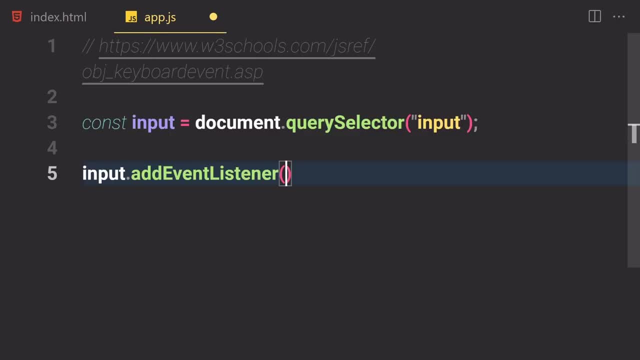 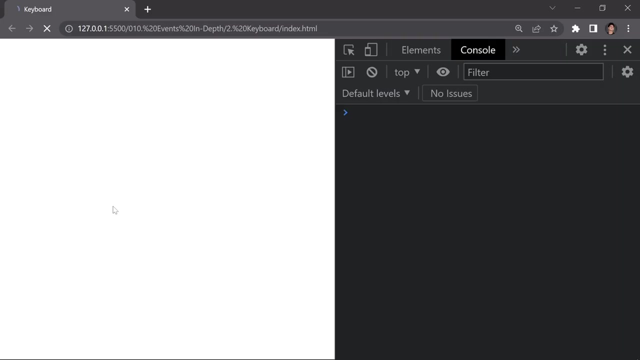 sort of a key so that add event listener. and let me just write a key press and here we just have to fire some sort of event, like i don't know. i'm gonna just write uh consolelog of key pressed if. if you just press some sort of a key, so this event will not fire until we press some keys. so 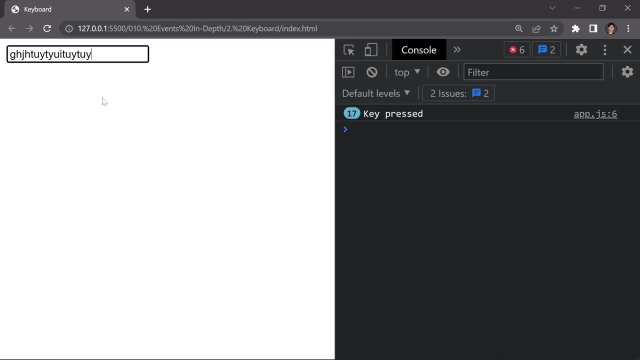 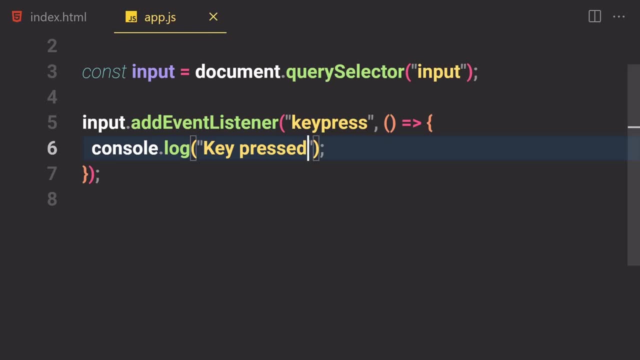 i'm going to just press some random key right here. so these are random keys i'm pressing right now and that event will fire that much time, like so. so that was the first one. let's just duplicate that and change this one to. you know, i'm going to come in this out and change this event to key up, if so. 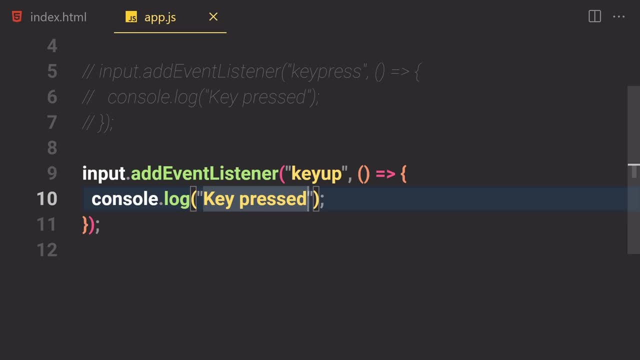 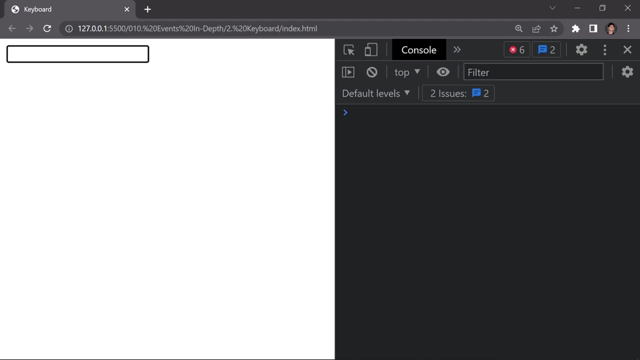 if you just hold or key, so that event will not fire. if you just release or key, so that even will fire. so key up, kind of a stupid one. and if you just, um, let me just hold some button, you know i'm going to hold this edge, so i'm going to hold this edge and that event will not fire. but if i just release that, 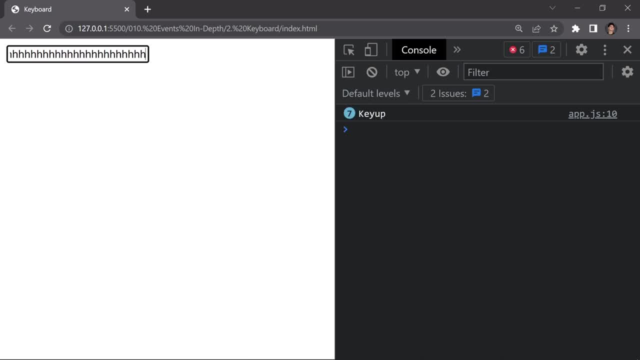 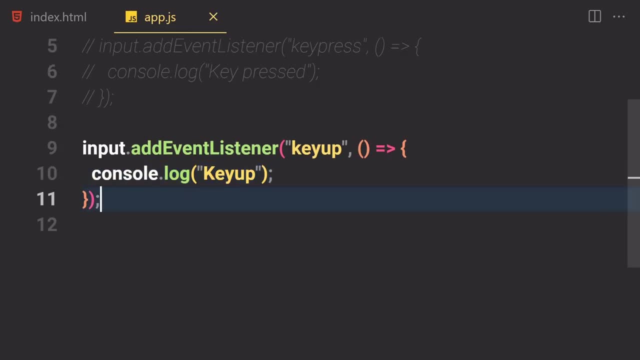 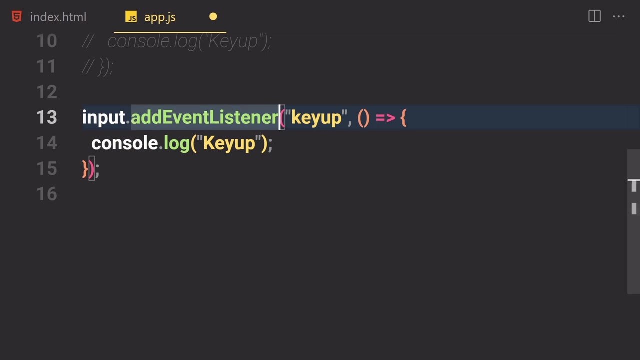 and here you can see, that event will fire. so if i just presses, and here you can see, that will fire that much time, that event will fire that much time anyways. so that was a key up, and then we have the final one. let's just duplicate that and learn about something called a key down. so if 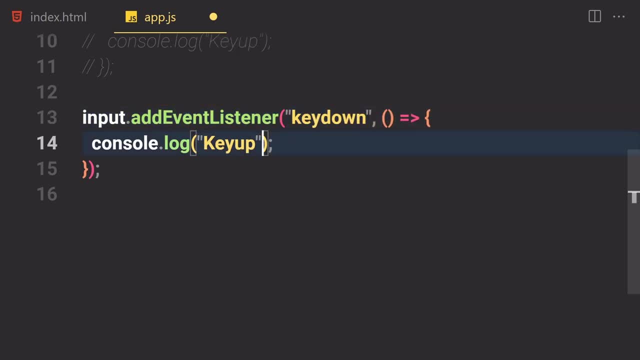 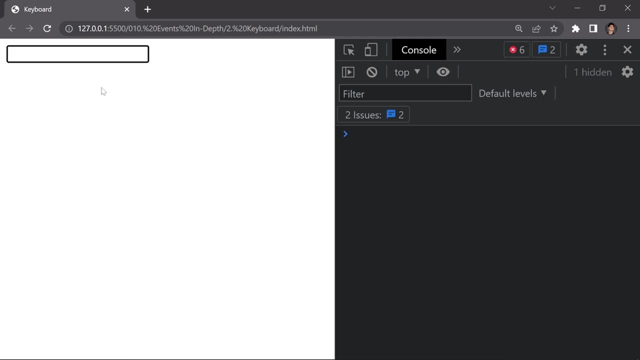 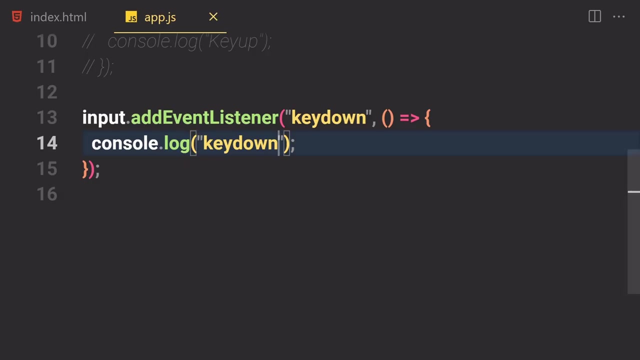 the key is down like key down, key press and key down is kind of a same like key down server file, and if you just key down, like if you just hit some key, so it would, this event will still fire like that much time anyway. so that was just at about four keyboard events, and now let's just learn. 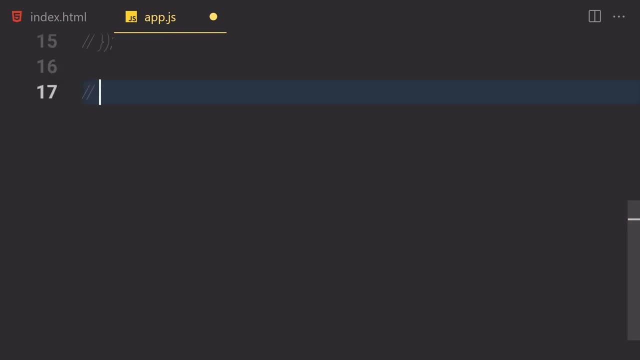 a few useful properties and methods related to this uh keyboard event. so i'm gonna just write like useful properties is and methods like so. so now let's just use that, let's just get our input, not that one input, and use add event listener. and once we press some key, so we want to get or eat because this 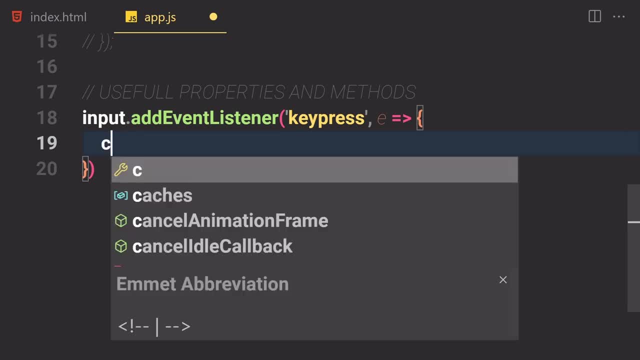 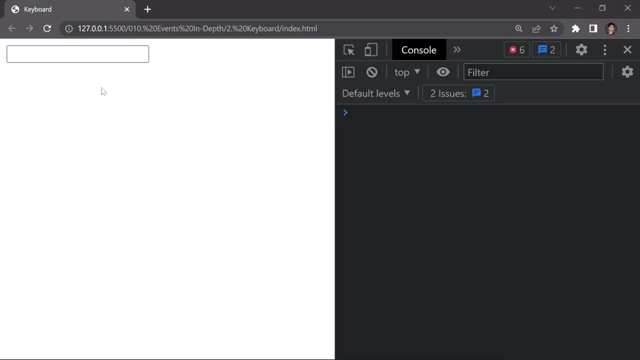 is important. and now let's just write console, console dot log of e and then char code: certain log uses that character code. so if you just type something like if i just type, a certain log uses the character code of 97, and then b98, c99, d, e, f and blah, blah, blah. okay, so any, any key, i press. 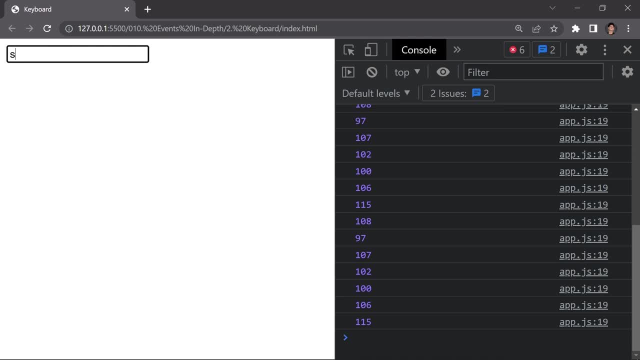 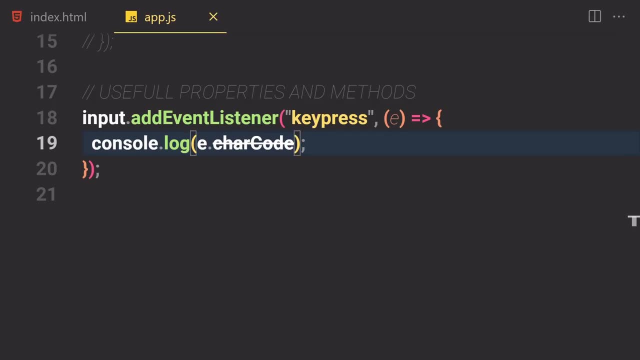 it will give us different kind of character code based on the specific key which i'm pressing right now. okay, like so, and we are going to be building a project by using this char code and code and stuff like that. let me just duplicate that and change this one to code and i'm going to come. 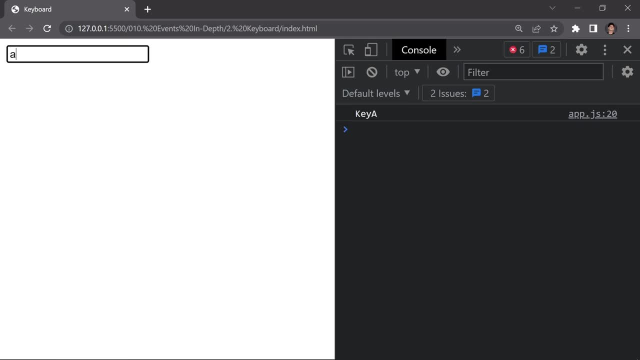 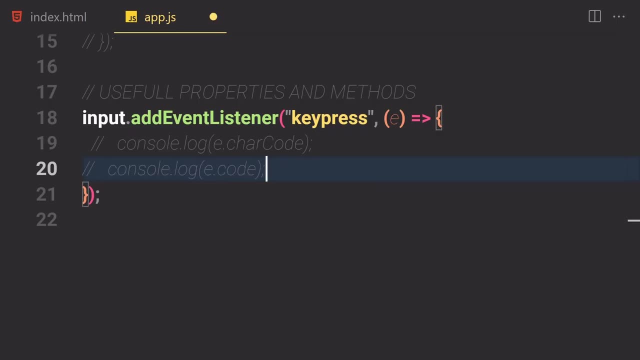 with the other one line, so cell file. and now if i hit and change it to that, and if i hit a certain log, it gives us key a. if i hit b, c, d, a, f, g, it will just give us key and the specific key name and then let's just use consolelog of e, dot, c, t, r l key. 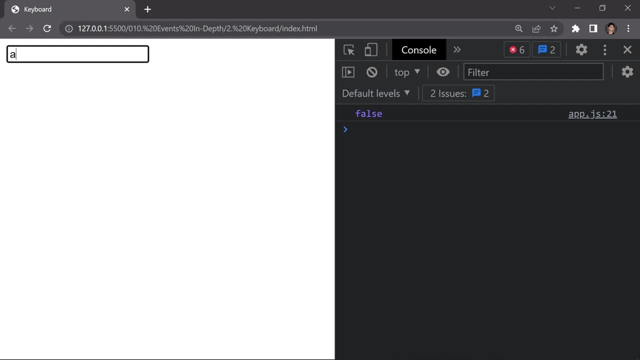 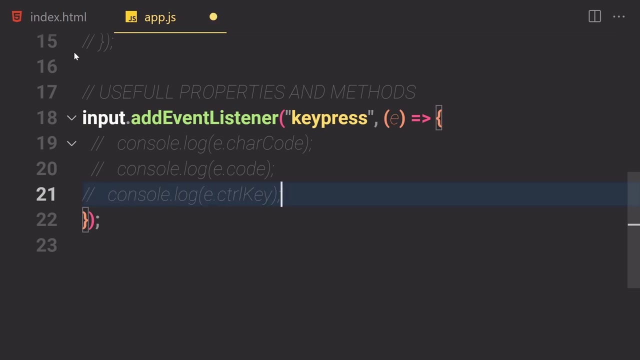 it will just check. did the user hold that key while pressing some sort of a key? so let me just write a certain like: uses false, b, still false. but if i just hit control and if i hit cam, so the long not gives us true. it will just give us true if the control key was hold. but if it will give us, 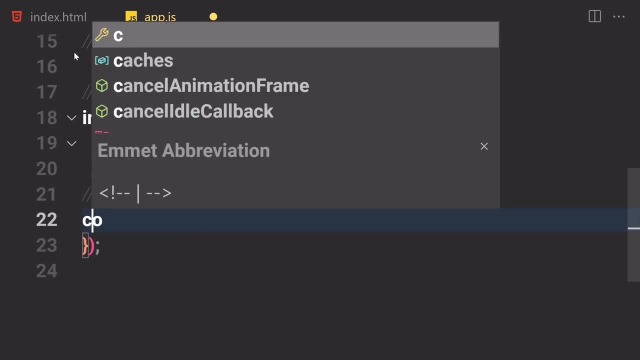 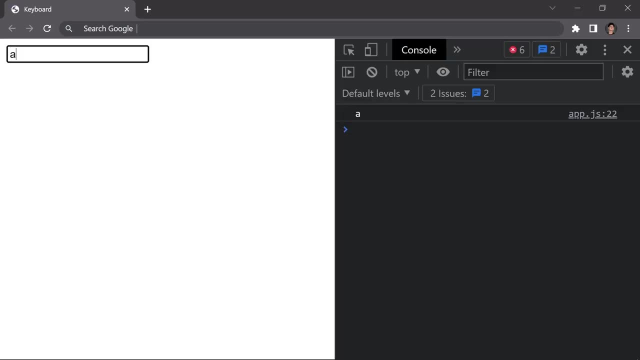 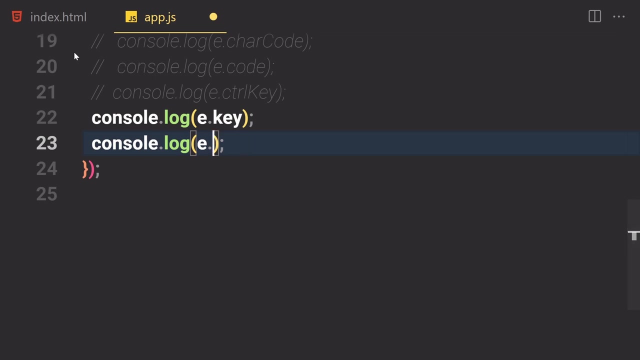 false if that wasn't the case. so now let's just log that to the console like key, not keyboard ekey. and now if you save that, if you just write a, so it will not give us a, b, c, d, e, f, g and blah, blah, blah, it will just print us all of the keys which you are pressing right now and then we have. 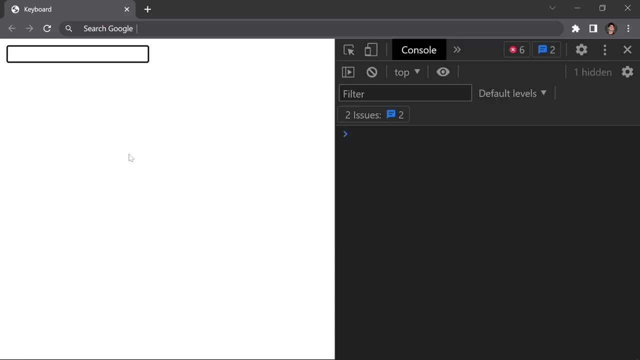 a shift key, so it will just check: did the user hold a shift while hitting on that key or not? so if i just write a, so nothing will happen, it will give us false. if i just hit uh, i don't know- b, it will give us still false. but if i hold shift and hit q, so it no longer gives us true. and if i 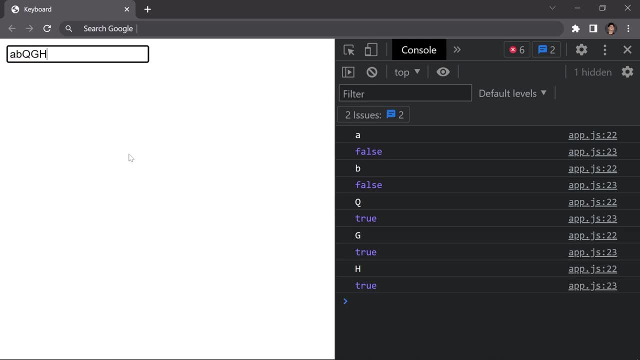 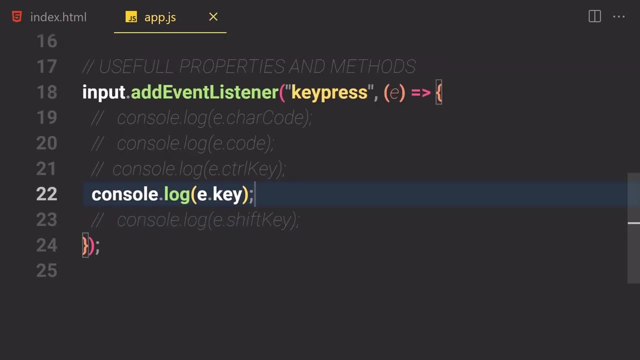 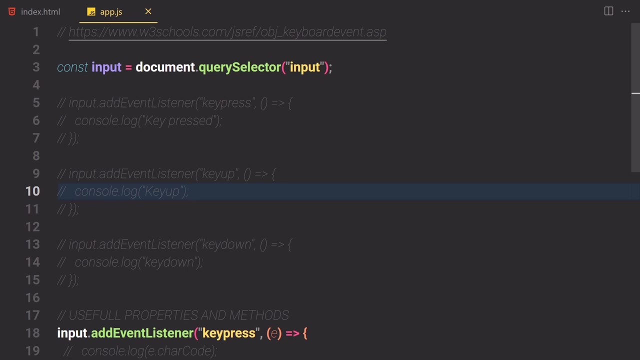 just hold shift and hit g, it will also give us true and so on and so forth. okay, so these were just a few methods and uh properties which you can use throughout, and we are going to be also building a project by using these keyboard events and stuff like that. all right, so now we are. 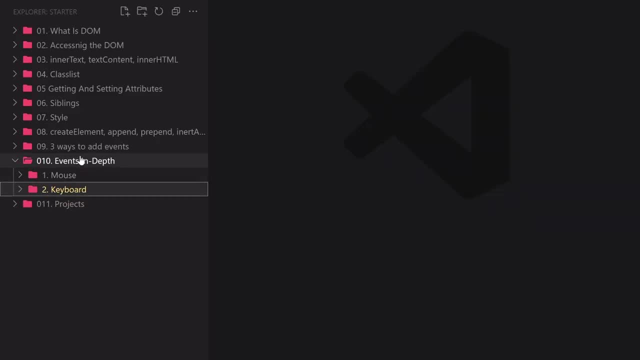 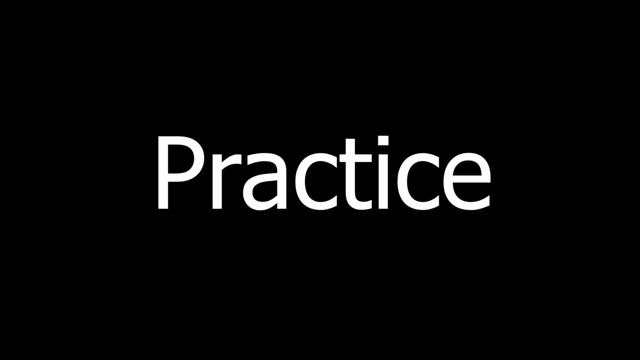 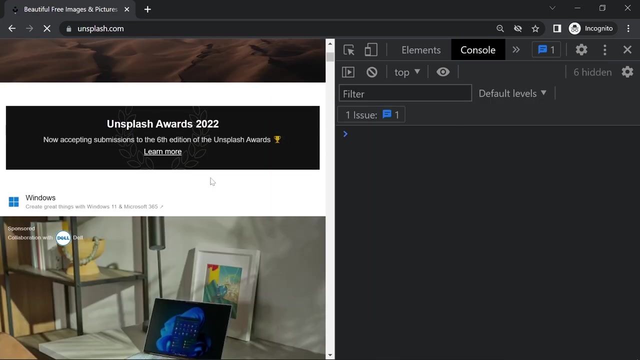 totally done with our dom, course, but you can practice that by going to like random websites. if you want to like, uh, in my case i'm going to just go splashcom and i can just explore that. like, i can just play around with the dom, i can change the things, i can even change the images. 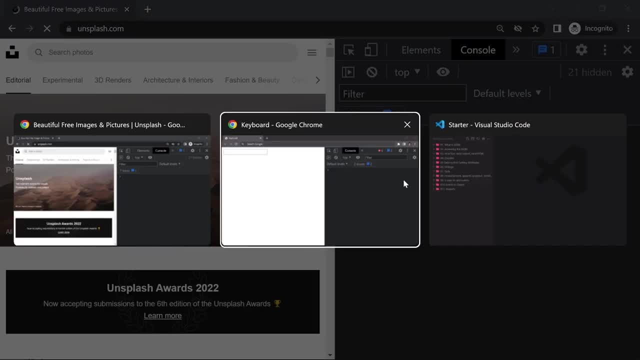 if i want to, and i can do a lot sort of stuff with that, and i'm going to be working on a lot of stuff with that, and i'm going to be working on a lot of stuff with that and i'm going to be also giving you a project, like we are going to be building this sixth project in this video, but my 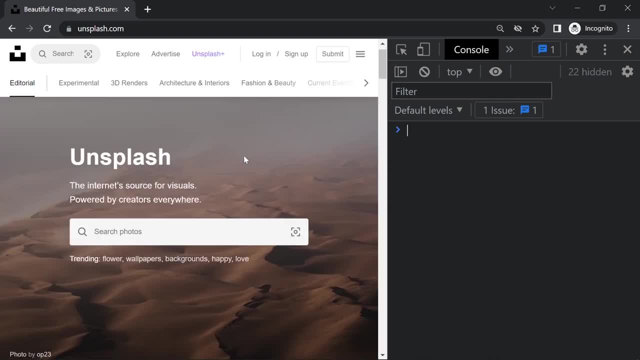 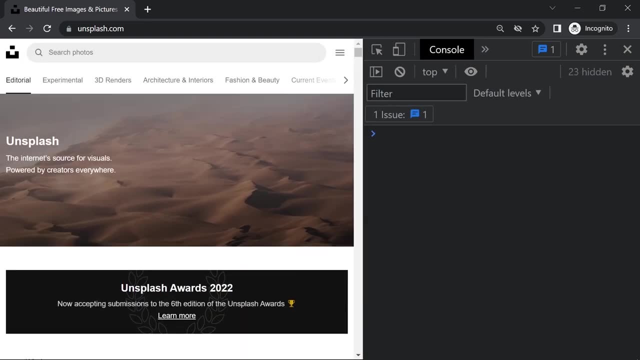 recommendation will be to first of all go to random website like i don't know. in my case, i just came to unsplash. you can go to google and you can just play around with there. you know, just select something by using a query selector. check out its code like: go to the elements panel. 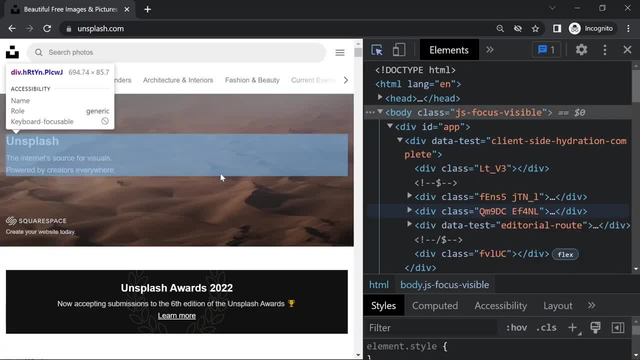 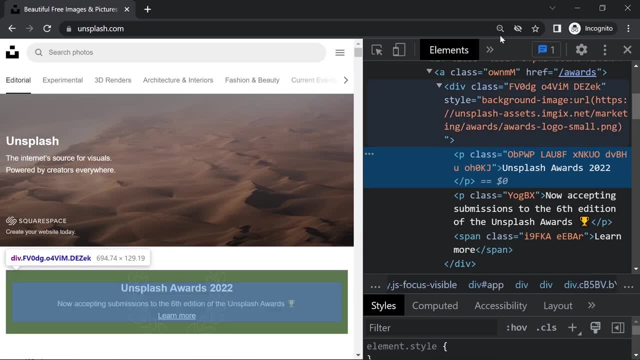 and go to the body, like the app or you know what. you can just click on that and click around, like anywhere you like and it will give us different kinds of like uh classes. so you don't have to. let me just show you a quick, real quick uh trick. so now that we click on this, 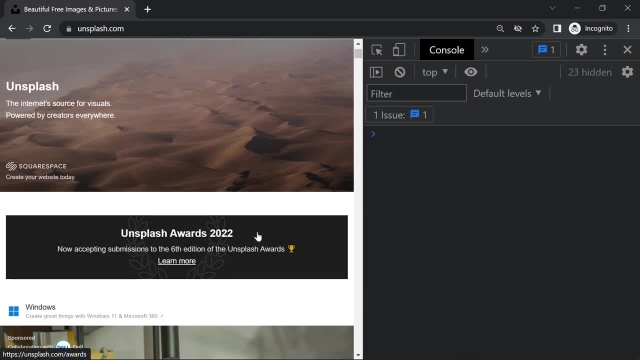 unsplash. oh, like, we just selected that unsplash award 2022. but if you just hit dollar sign and zero, and if you hit enter and here you can see, it will not just select that paragraph for you, but this will only work on developer tools. so now, if you just select uh, this unsplash right here and 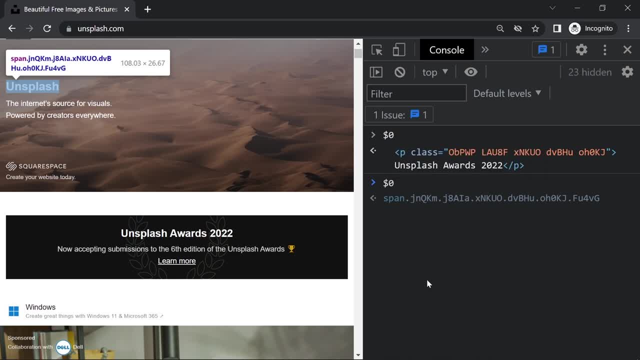 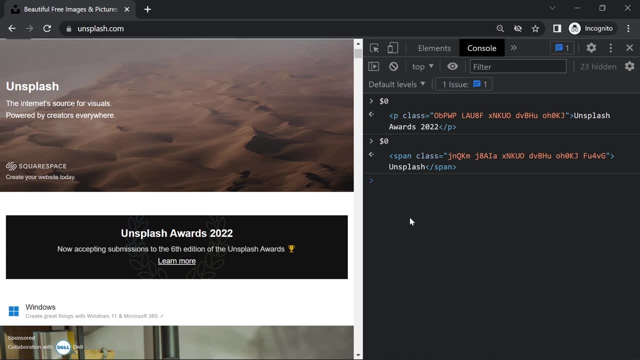 if you go to our console and then dollar sign in zero and if you hit enter, so it will not just select that unsplash right here, so we can just store that to some variables and stuff, like, uh, i don't know, uh, what can i do? i'm 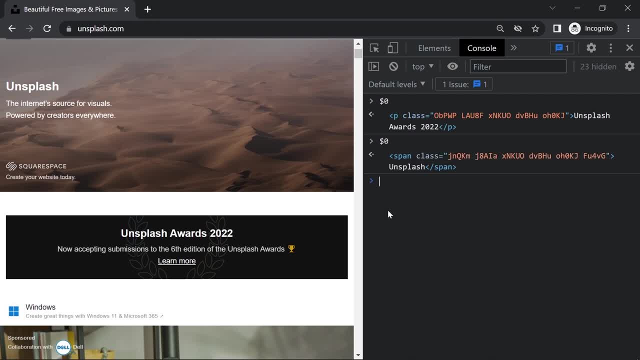 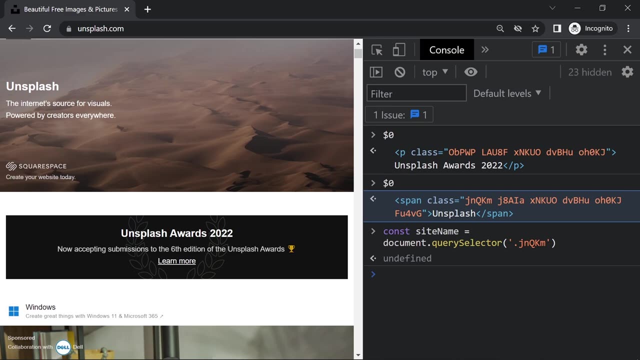 going to copy just a single class of it and i'm going to just store that to like const uh site name and it will now equals to documentquery selector of that site name. and, by the way, don't forget to include their period, because it's a class. and now we selected their site name, let's 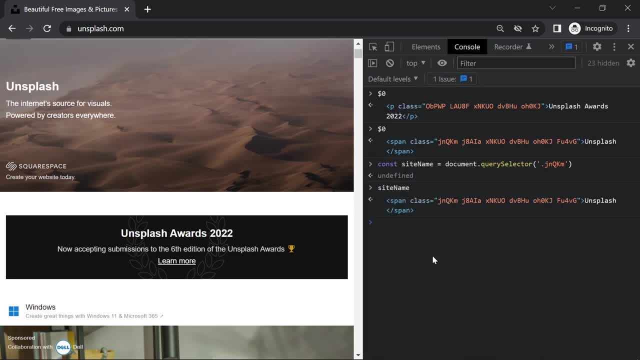 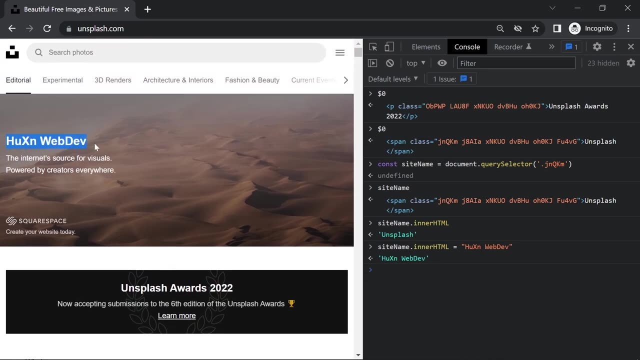 just see site name and if you hit enter, okay, so we can just use site name dot enter text, we can check out that one. or we can also change it to our own name, like huzzain web dev, and if you hit enter and here you can see, it will now change the unsplash to: 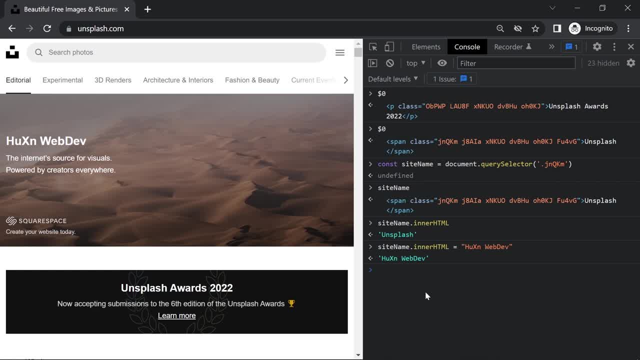 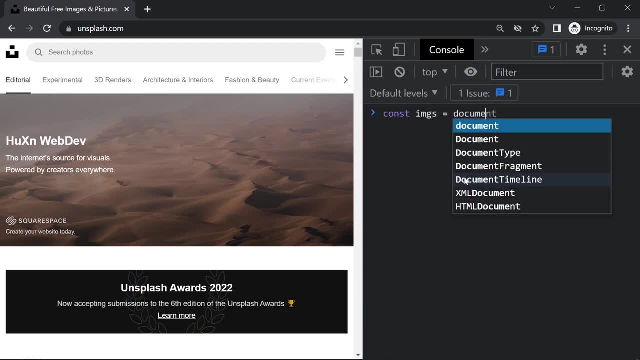 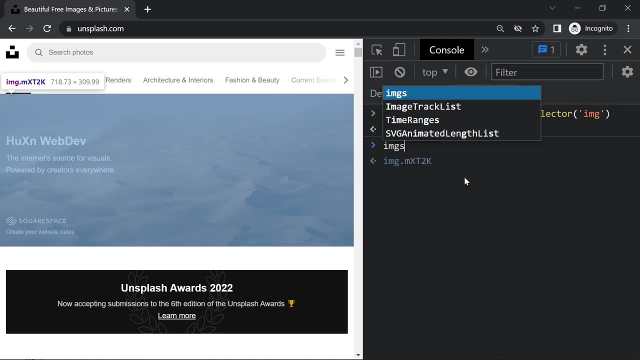 huzzain web dev, you can also find out how many images we have inside this all uh website. so we can just use like const imgs for documentquery selector of just use img and if you hit enter. and now, if you just explore this imgs and if you hit enter, certain now just gives us the first one because, oh, come on. 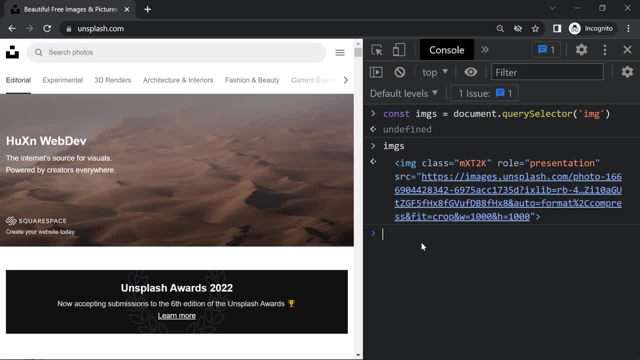 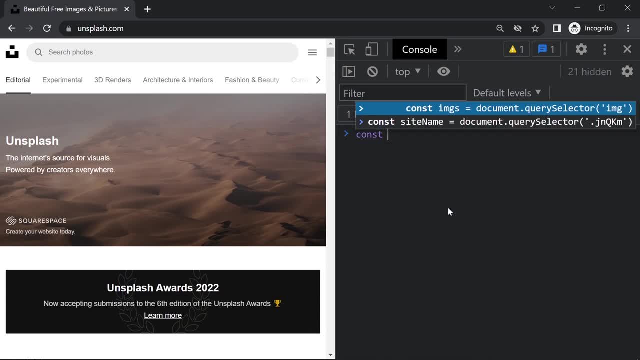 because we just use a query selector, not query selector. let me just refresh that one more time. and now let's just use or query selector all. in this case i'm going to just use const imgs and document dot query selector all. and let's just use or img. and if you hit enter. 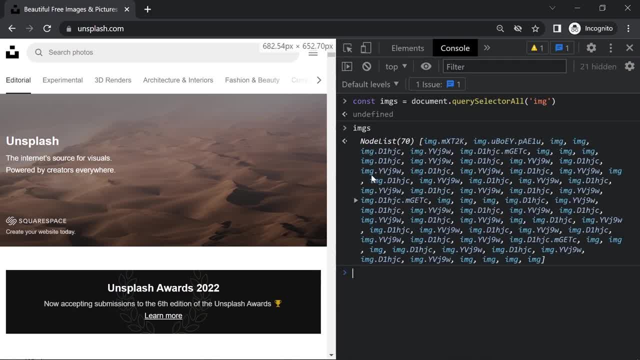 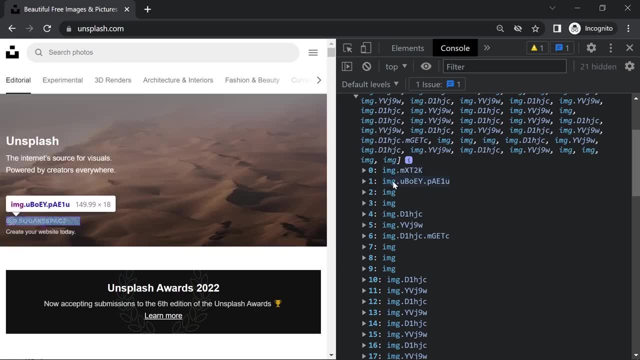 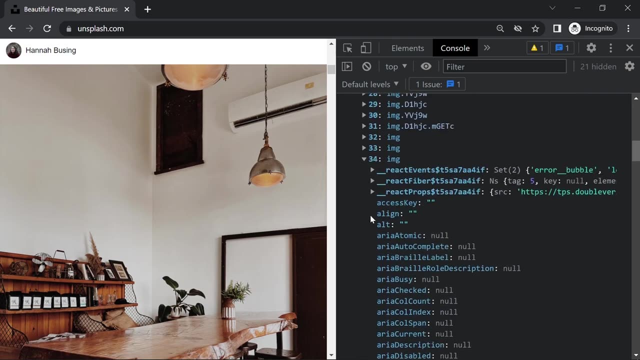 and if you just hit on img, so we have 17 images on just this one landing page right here. so if you just click on that we can explore more. like we have this image, that one. we have other images down here. we can explore that. we can get a classes of them. we can do a lot sort of stuff with them. 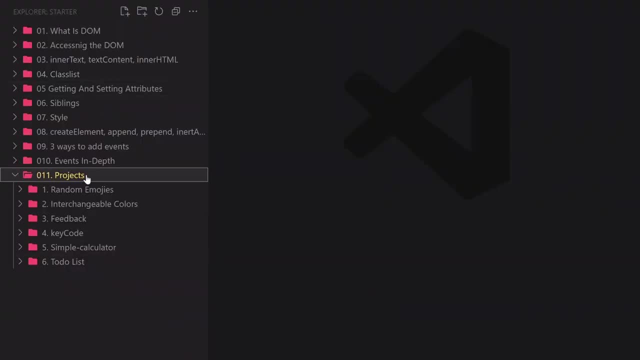 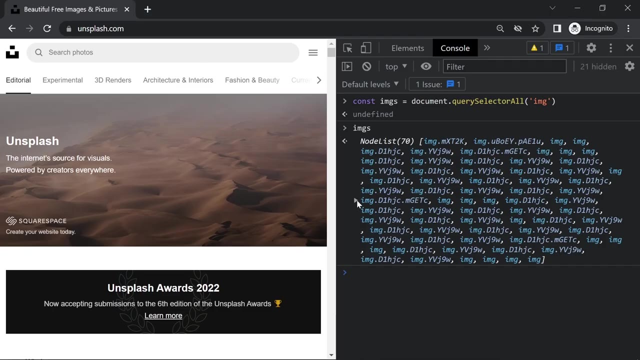 like we learned enough stuff. we learned crazy stuff throughout the schools, so my recommendation will be to just spend a few seconds and not seconds. i shouldn't have the second second, but my recommendation would be to just spend a few hours. uh, just going to random sites and 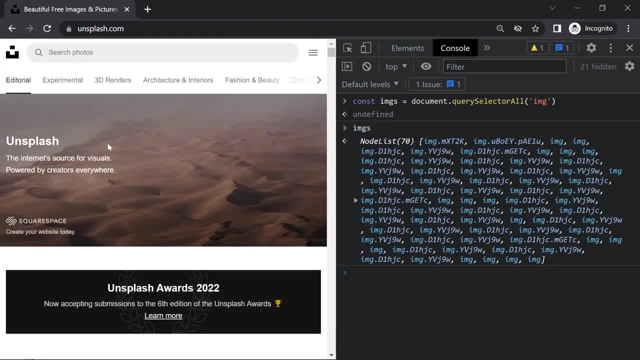 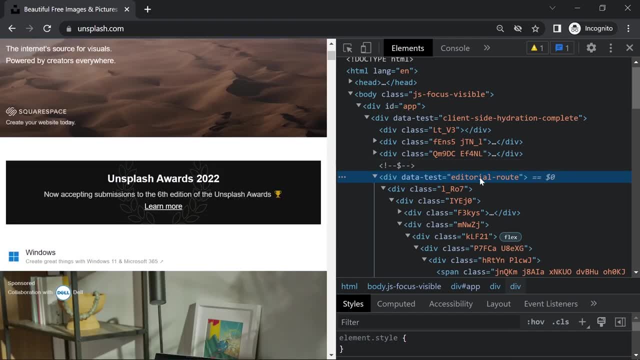 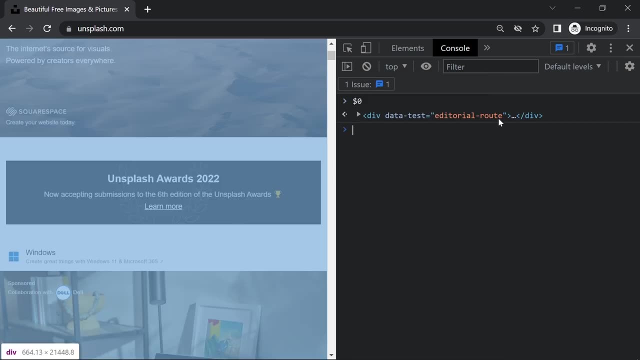 just exploring with that, like you can even change the background color of this site. let's just get into. you know i'm going to click on here somewhere and okay, rower, additional row, let's just select that real quick. i'm going to hit dollar signs and dollar sign in zero. and now let's. 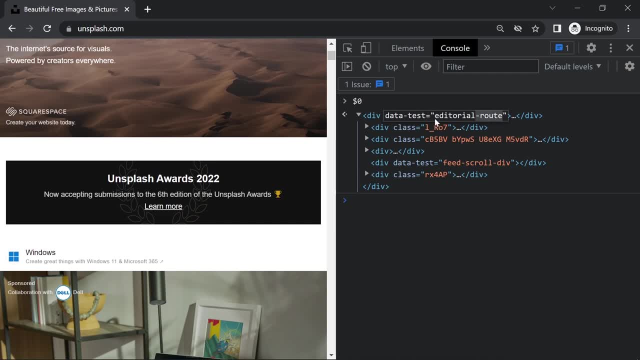 just get this class. i'm going to cut that or copy this class and we can even change the classes like, um, we can even change different kind of stuff, like i don't know const, uh, header or you know what, sex section, but now it goes to document that query, selector of that um element or whatever, and 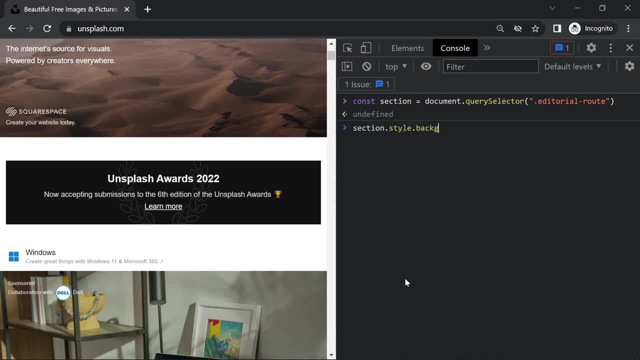 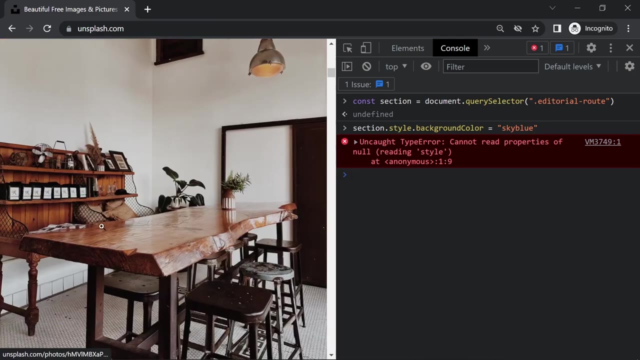 section dot style: dot background color: let me know, set to sky blue if you hit. okay, so something is. there cannot read a property of un null, uh-huh, so we did miss something in here. you know you can change the color of something else like i don't know, excuse me so. 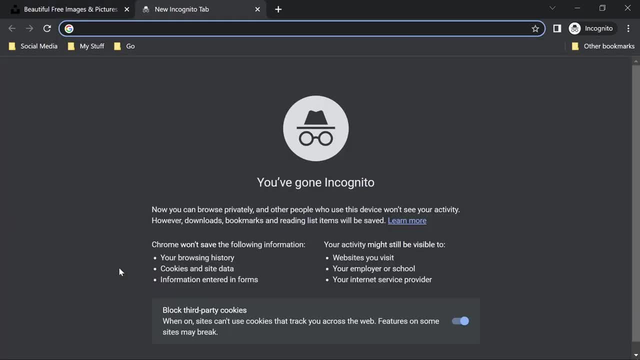 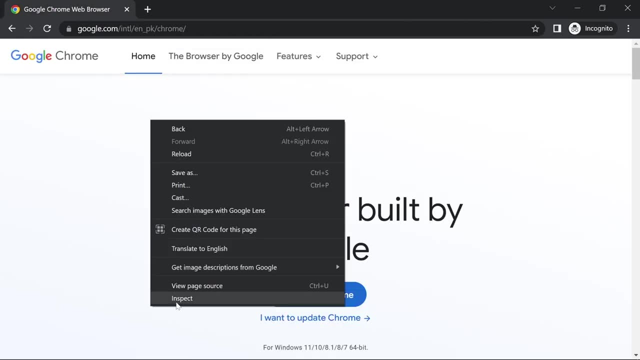 what should we do? you know, i'm going to go to some other site, like let's just go to google chrome site official web page, and now let's just play around with that. i'm going to right click on it and go to the inspect area, go to the console and select. 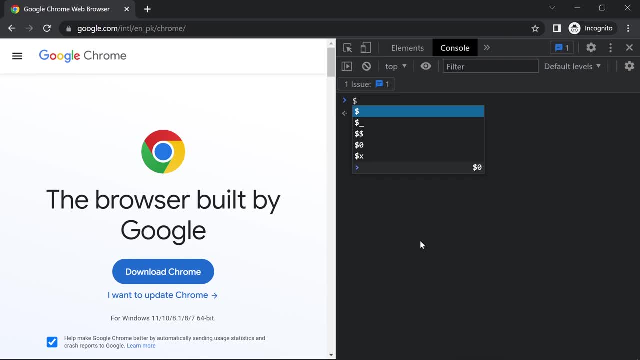 their body and let's just use dollar sign and zero hit enter and let's just copy that and what do we have to do? i'm going to just store that variable like section or header- would be fine. document dot query selector of that kind of a weird selector. and if you just check the header, 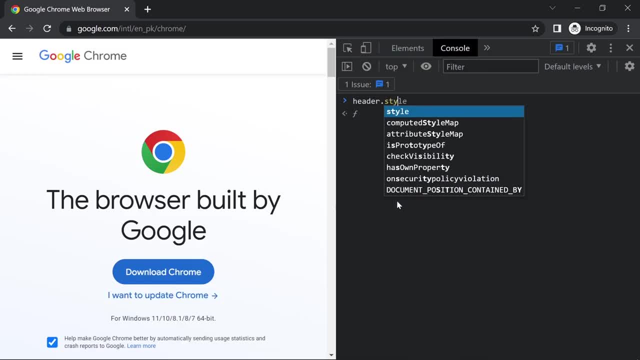 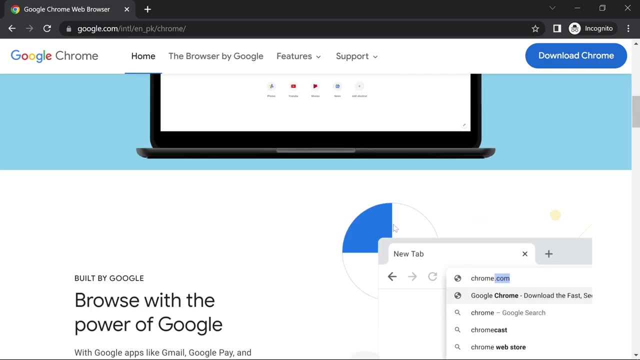 it will now give us the header. we can change the background color of that header: dot style, dot. background color of that like something else, like maybe sky blue. and if you hit enter and there we go, your google is now totally sky blue. you can even remove this stuff from here. let's just right. 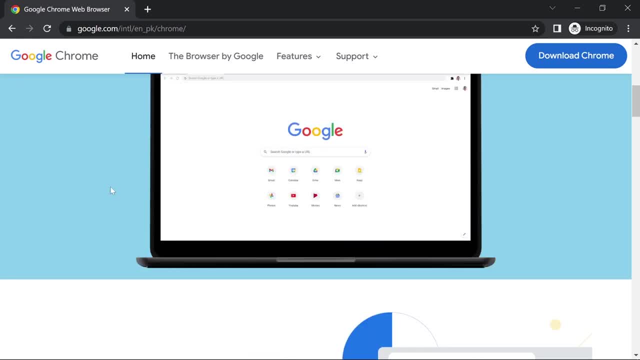 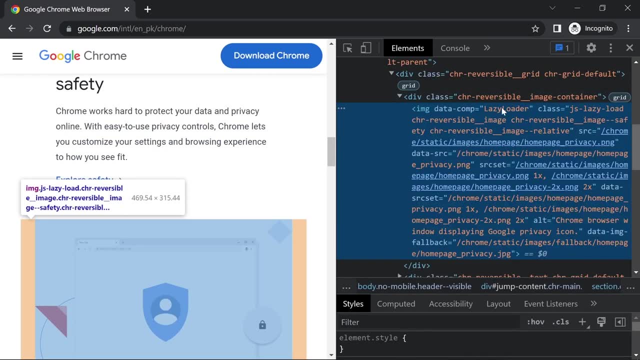 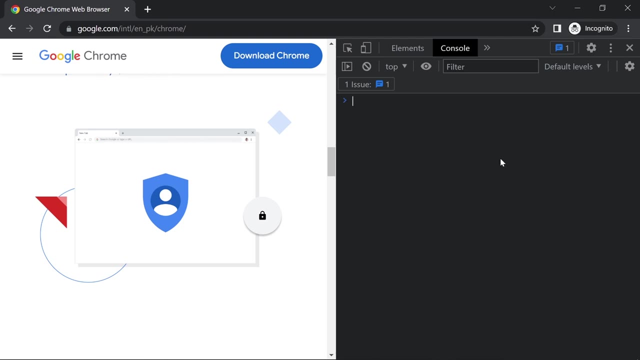 click on it. uh, oh, you know what let's just, what can we do with that? let's just remove this svg from there selected. okay, so we have different kind of lazy loading and stuff. okay, this image- i thought it's an svg, but it's an image. so now let's just use dollar sign zero, hit enter and oh my god this. 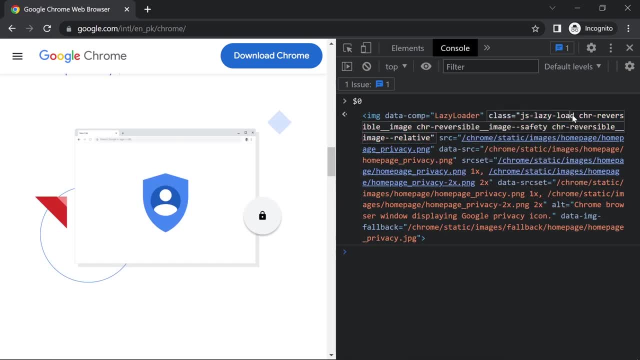 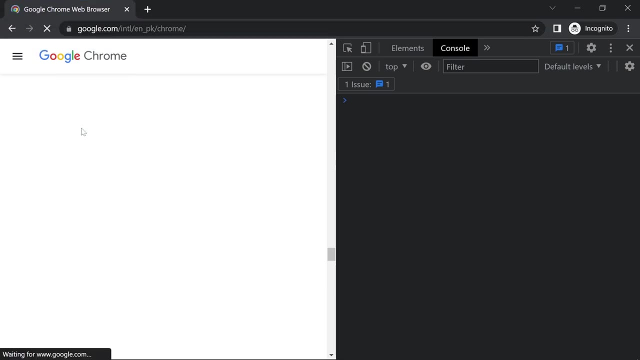 is a huge clauses. let's just- oh my god, let's just select this, just lazy loading. let's just select this, just lazy loading. oh my, hmm, oh, you know what? we can also remove all of these images at once, i guess. let's, let me just refresh this browser. let me just refresh that one more time and go to the top. let's just get all of. 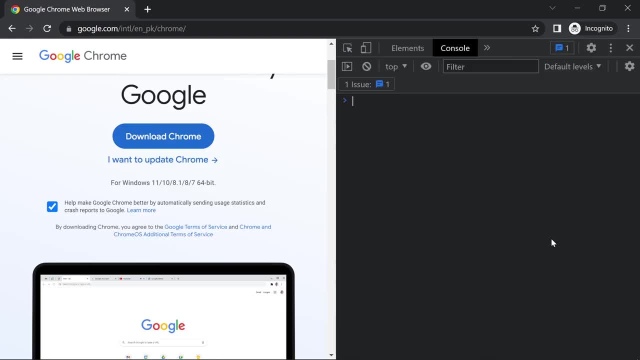 the images which we have, like i don't know const or not, consulate imgs and let me know, equals documentquery selector. all let's just get all of the images and img, imgsforEachImage, and what do we have to do for each image? so for each image we want to remove imgremove. 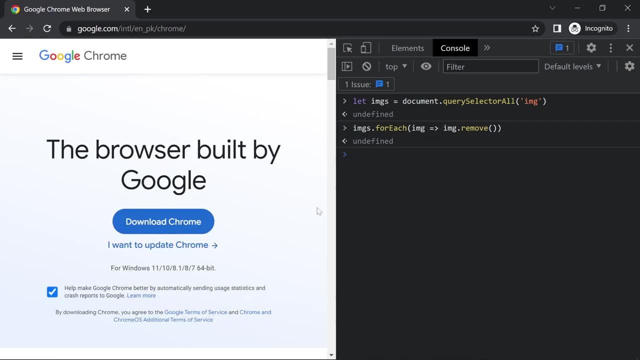 okay, so all of the images are now gone from this google chrome right here. so you cannot find any images that are missing from this google chrome right here. so you cannot find any images that are missing from this google chrome right here. so you cannot find any images that are missing from this google chrome right here. image right here you can change. 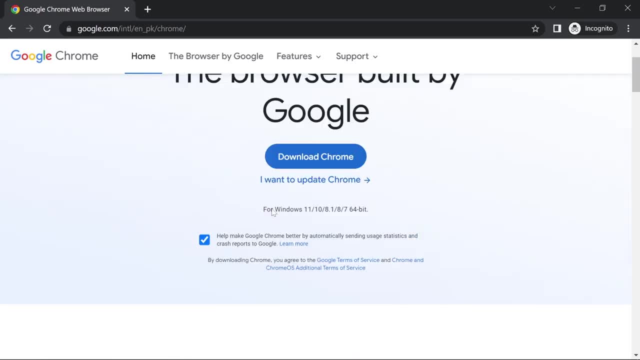 image. right here you can change image. right here you can change the name. you can change the text. you can the name. you can change the text. you can the name. you can change the text. you can replace. you can even put your own image replace. you can even put your own image. 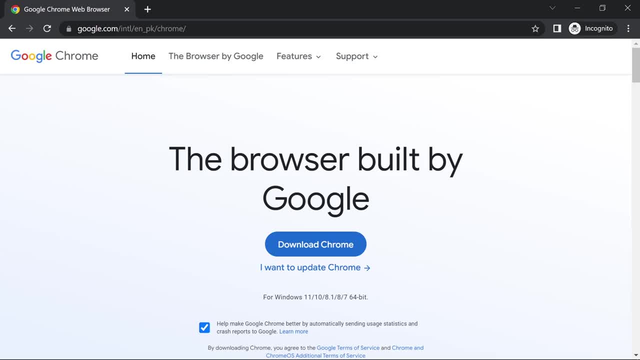 replace. you can even put your own image, if you want to. you can do crazy stuff if you want to. you can do crazy stuff if you want to. you can do crazy stuff with that. so i will highly recommend you with that. so i will highly recommend you. 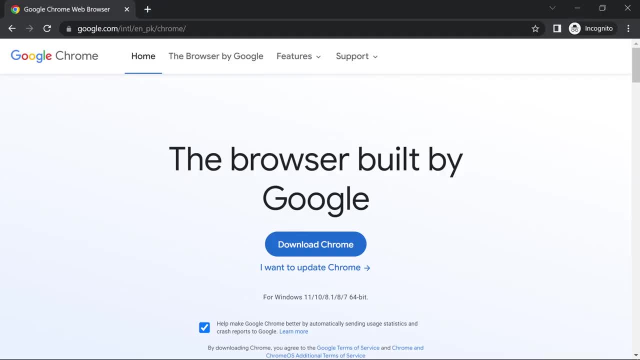 with that. so i will highly recommend you to go to any site. you want your own to go to any site. you want your own to go to any site. you want your own site. like i don't know, you can go to any site. like i don't know you can go to any. 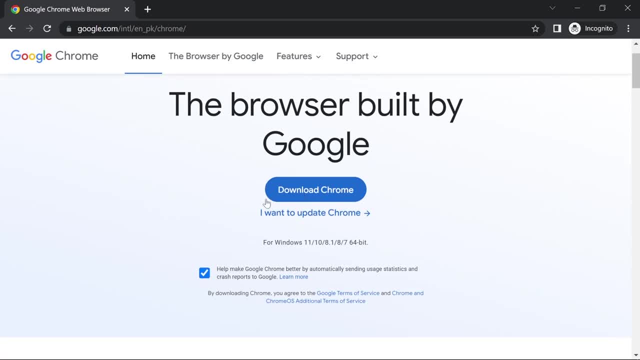 site like i don't know. you can go to any site you want and just pair on with site you want and just pair on with site you want and just pair on with that. you can even change the background that. you can even change the background that. you can even change the background color of this button. you can increase or 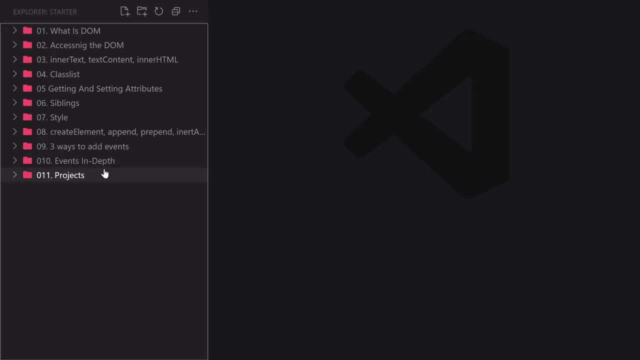 color of this button you can increase or color of this button you can increase or decrease. that you can provide animation. decrease that you can provide animation, decrease that you can provide animation and all kind of a good stuff like that, and all kind of a good stuff like that. 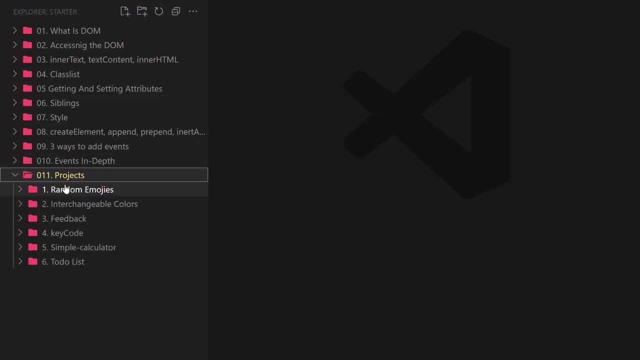 and all kind of a good stuff like that. okay, so, finally, let's just jump into. okay, so, finally, let's just jump into. okay, so finally, let's just jump into this project and start building our this project and start building our this project and start building our first project. 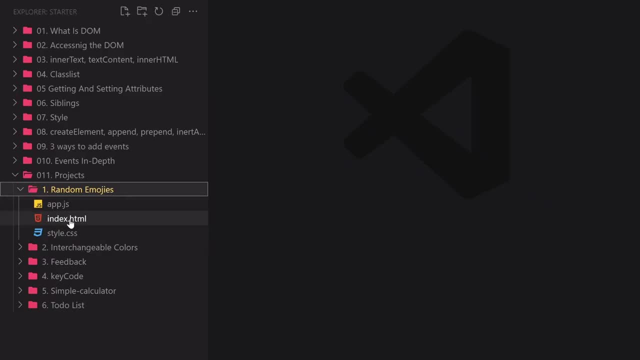 first project, first project, so we have our first project, which is so we have our first project, which is this: random emojis and we have index this random emojis and we have index this random emojis and we have indexhtml file in there. we have this css html file in there. we have this css. 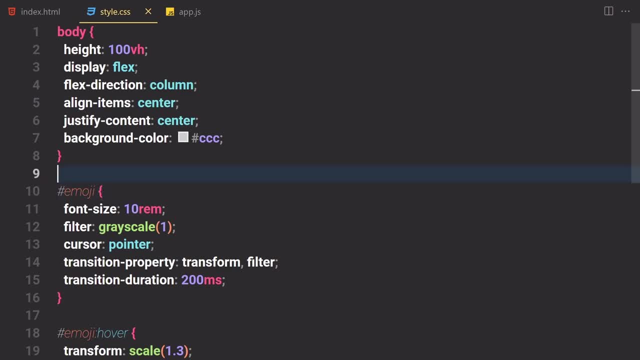 html file in there. we have this css file and we have this javascript file file and we have this javascript file file and we have this javascript file. so i will already give you this um. so i will already give you this um. so i will already give you this um css as well, so you don't have to type. 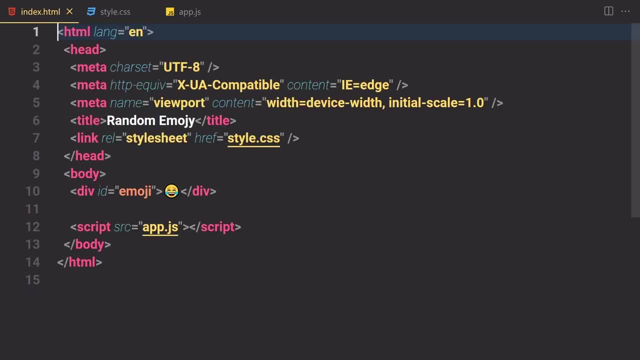 css as well. so you don't have to type css as well, so you don't have to type this css again and again by yourself, this css, again and again by yourself, this css, again and again by yourself. so here you can see, we have like just a. so here you can see, we have like just a css, again and again by yourself. so here you can see, we have like just a. so here you can see, we have like just a basic doc type html, but we just have one basic doc type html, but we just have one. 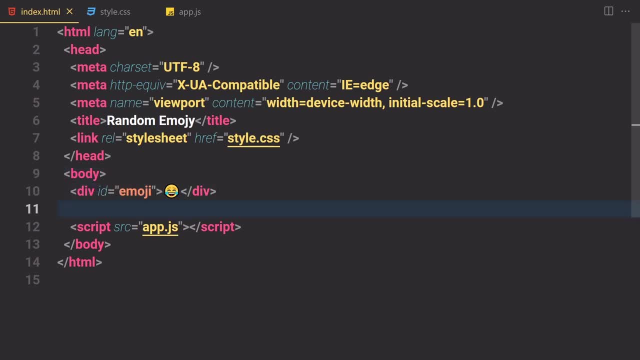 basic doc type html. but we just have one div, div, div. and we have this smiley emoji and by the, and we have this smiley emoji and by the, and we have this smiley emoji and, by the way, if you want to get emoji, way, if you want to get emoji. 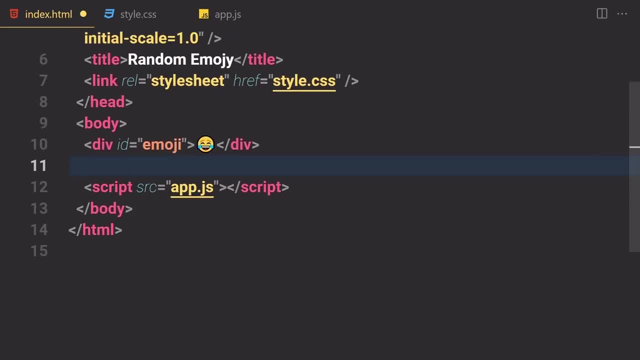 way, if you want to get emoji- i'm not sure about a mac user, but if i'm not sure about a mac user, but if i'm not sure about a mac user, but if you are a windows user, so i want you to. you are a windows user, so i want you to. 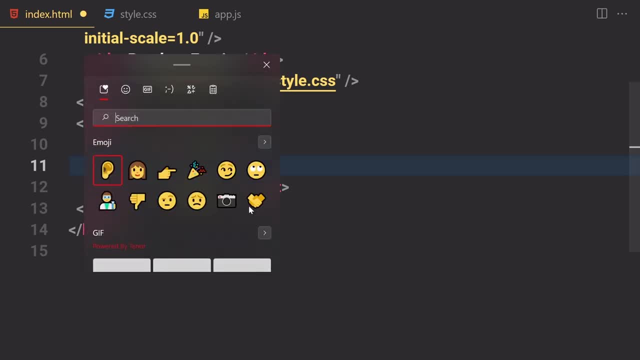 you are a windows user, so i want you to just hold a windows button and hit dot. just hold a windows button and hit dot. just hold a windows user. so i want you to hold a windows button and hit dot. just hold a windows user. so i want you to hold a windows button and hit dot. so it will now use a different. 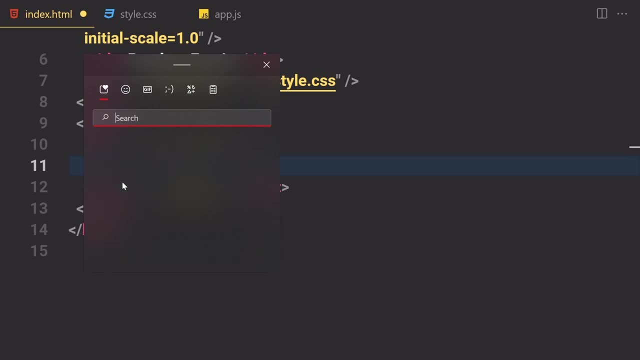 so it will now use a different. so it will now use a different kind of emojis right here. so you can kind of emojis right here. so you can kind of emojis right here. so you can just give a name of the emoji and it. just give a name of the emoji and it. 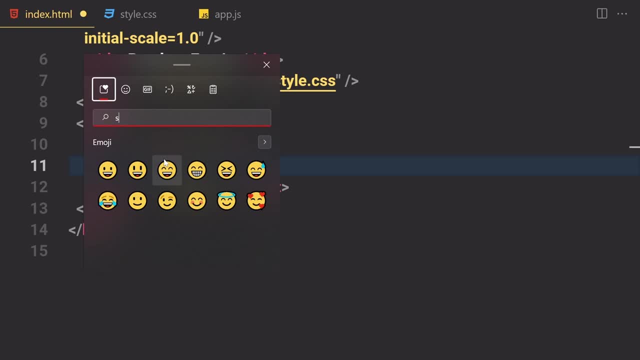 just give a name of the emoji and it will give you that in my case, if i just will give you that in my case, if i just will give you that in my case, if i just hit s, hit s, hit s. kind of a weird guy. so that's why we are kind of a weird guy, so that's why we are kind of a weird guy, so that's why we are getting kind of a smiley faces. so if you getting kind of a weird guy, so if you getting kind of a weird guy, so if you just select that, 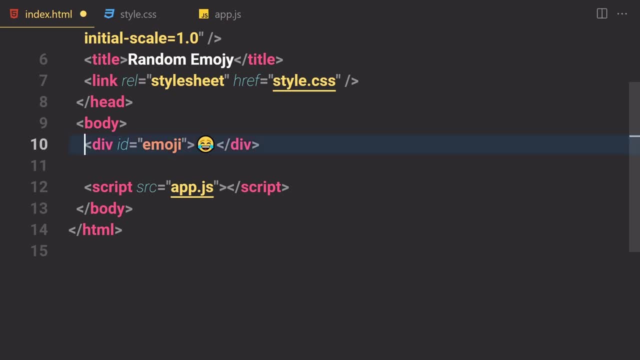 just select that, just select that. and there we go, you get your svg. and there we go, you get your svg and there we go, you get your svg. i'm going to remove that, and this is how i'm going to remove that, and this is how i'm going to remove that, and this is how we provide our 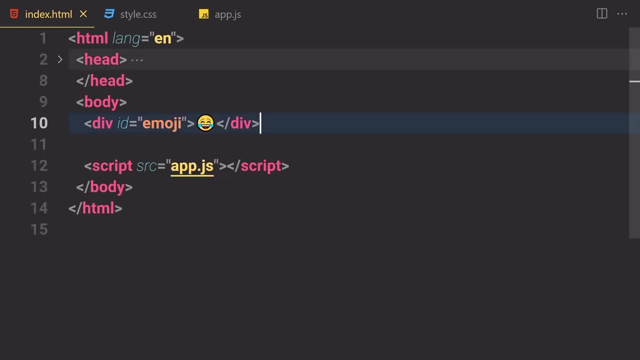 we provide our. we provide our text or text, or text or or image. you can also provide uh, what do? or image? you can also provide uh, what do or image. you can also provide uh, what do we call it? we call it, we call it a font. awesome, if you want to, you can. 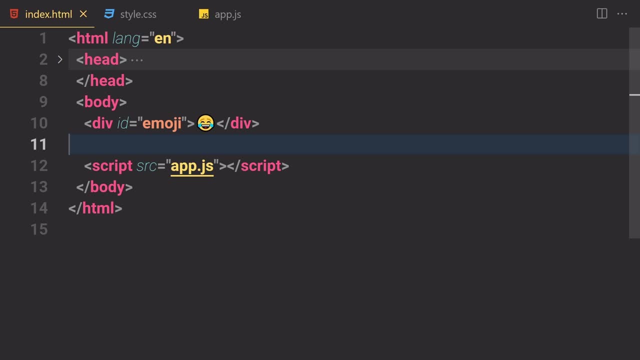 a font awesome if you want to, you can. a font awesome if you want to, you can also probably render different kind of also probably render different kind of, also probably render different kind of things. but in my case we just have a div things, but in my case we just have a div. 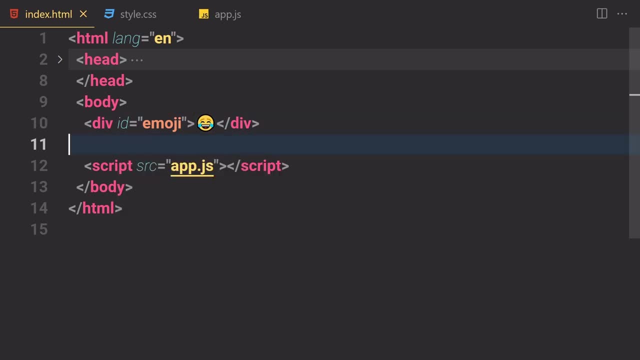 things. but in my case we just have a div with the id of emoji and we just have one with the id of emoji and we just have one with the id of emoji and we just have one: emoji inside there, emoji inside there, emoji inside there and now inside the css. we are just 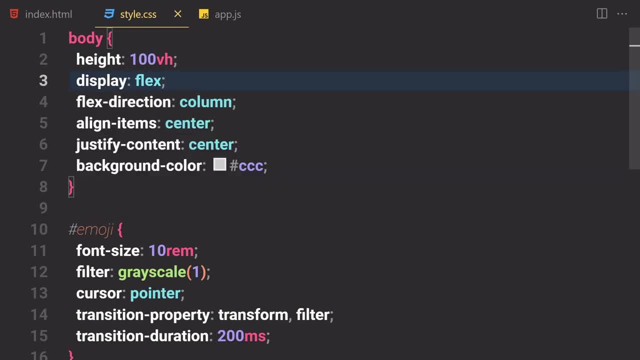 and now inside the css. we are just and now inside the css. we are just providing 100 pixel of height and providing 100 pixel of height and providing 100 pixel of height and displays: uh, flex flex direction is displays. uh, flex flex direction is displays. uh, flex flex direction is column align. items is centered center. 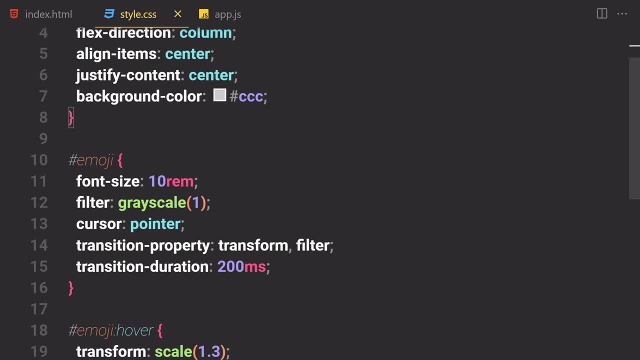 column align items is centered center. column align items is centered center and background is kind of a grayish kind and background is kind of a grayish kind and background is kind of a grayish kind of a background, and then we have our of a background and then we have our. 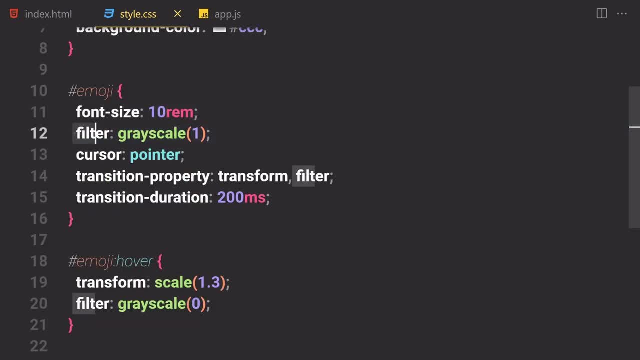 of a background. and then we have our emoji, the font size. we just increase the emoji, the font size, we just increase the emoji, the font size, we just increase the return rim and we just provide a little return rim. and we just provide a little return rim and we just provide a little bit of filter of gray scale of one and 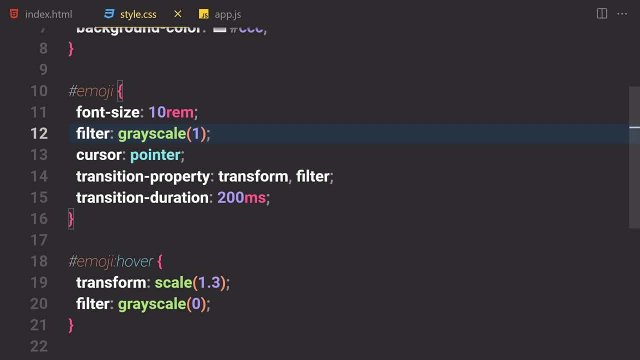 bit of filter of gray scale of one and bit of filter of gray scale of one and cursor will be a pointer once we hover, cursor will be a pointer once we hover, cursor will be a pointer once we hover over to it. and transition. we are just over to it and transition. we are just. 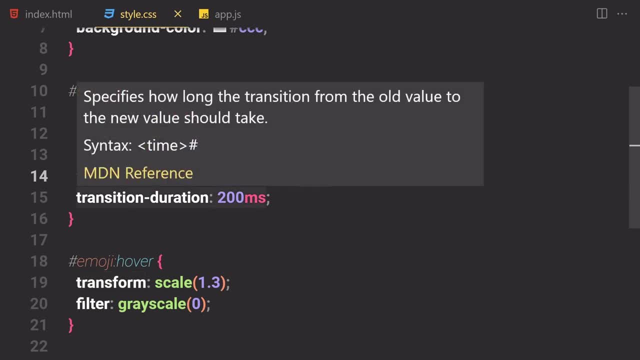 over to it and transition. we are just providing a transform of filter and then providing a transform of filter, and then providing a transform of filter, and then we have a transition duration. it will we have a transition duration. it will we have a transition duration. it will take 200 millisecond and once we hover, 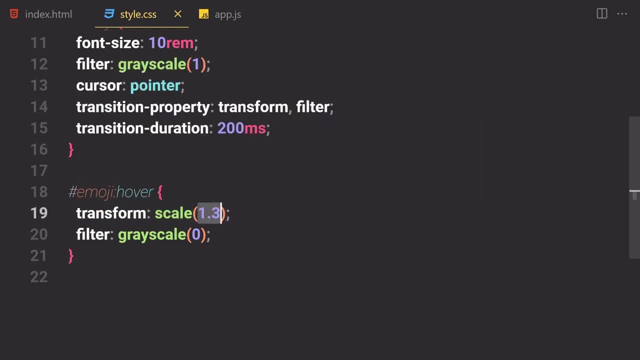 take 200 millisecond and once we hover take 200 millisecond and once we hover over it. so it will just scale for its uh over it. so it will just scale for its uh over it. so it will just scale for its uh size to 1.3 and the gray scale will be: 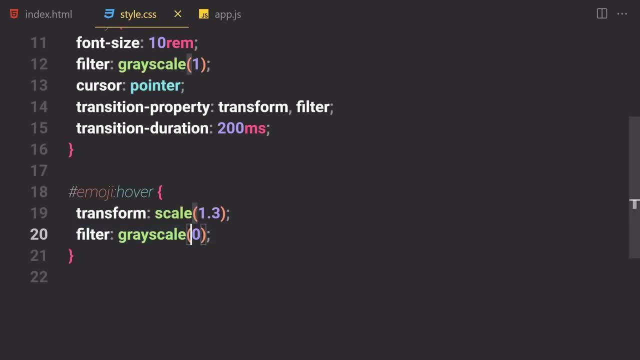 size to 1.3 and the gray scale will be size to 1.3 and the gray scale will be now set to zero. this is now set to one. now set to zero. this is now set to one. now set to zero. this is now set to one, so once we hover over to it. so the gray so once we hover over to it, so the gray. so once we hover over to it, so the gray scale will be set to zero. i'm going to scale will be set to zero. i'm going to scale will be set to zero. i'm going to launch that real quick. 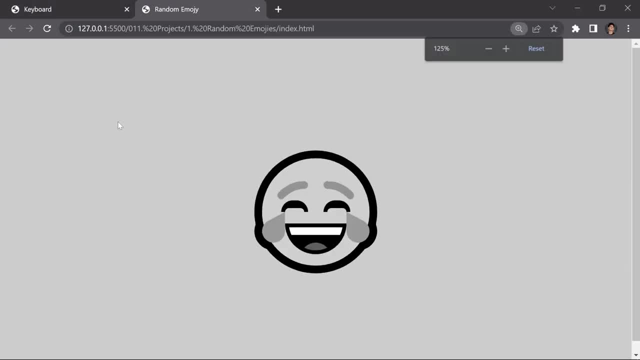 launch that real quick, launch that real quick. uh stop the live server and open it for uh. stop the live server and open it for uh. stop the live server and open it for the live server. and now, here you can see the live server. and now, here you can see. 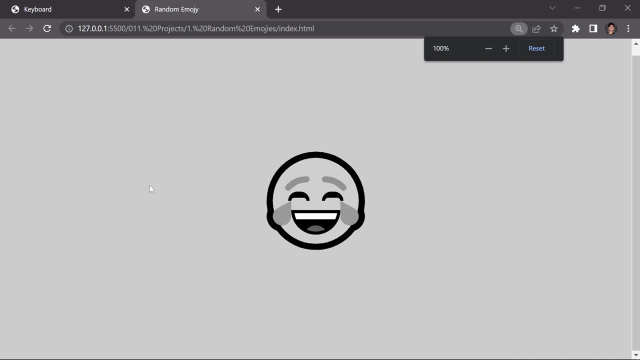 the live server. and now, here you can see, we have this image right here. we have this image right here. we have this image right here. if i just zoom out, and now if i hold my, if i just zoom out, and now if i hold my, if i just zoom out, and now if i hold my mouse over to it, so here you can see. 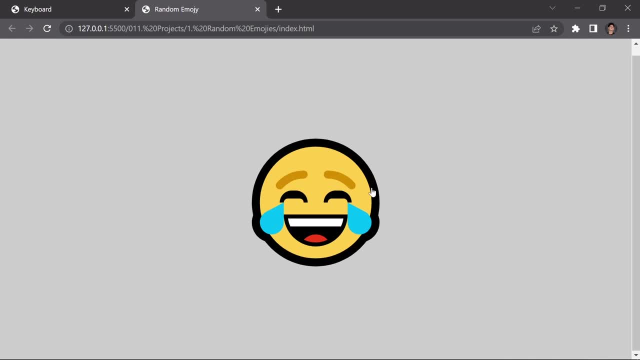 mouse over to it. so here you can see. mouse over to it. so here you can see that gray scale is setting to zero and that gray scale is setting to zero and that gray scale is setting to zero and this image is taking. i mean like this, this image is taking, i mean like this: 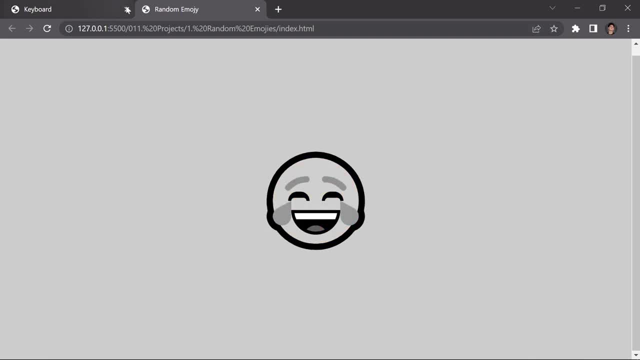 this image is taking. i mean, like this emoji is growing just a little bit, like emoji is growing just a little bit. like emoji is growing just a little bit like 1.3, 1.3, 1.3. all right, so you're scanning everything. all right, so you're scanning everything. all right, so you're scanning everything. is working the way we expand to work, but is working the way we expand to work, but is working the way we expand to work. but first of all, let me just show you we. first of all, let me just show you we. 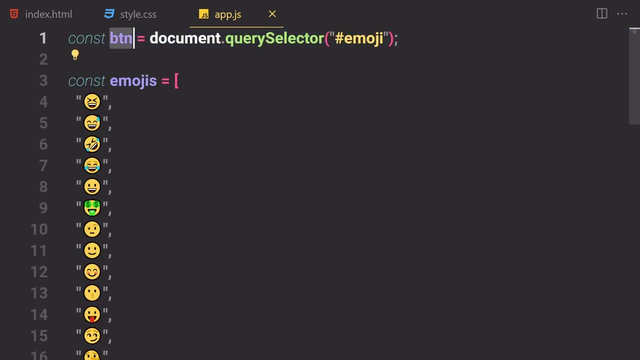 first of all, let me just show you: we have a few things, so we are first of all have a few things, so we are first of all have a few things. so we are first of all selecting our button or emoji to be, selecting our button or emoji to be. 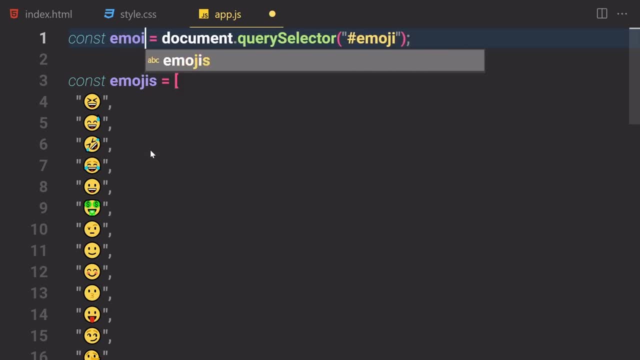 selecting our button or emoji to be precise. not a button precise. not a button precise. not a button. emoji: emoji like so: and now, here you can emoji. emoji like so: and now, here you can emoji. emoji: emoji like so: and now, here you can see. we have different kind of emojis. see, we have different kind of emojis. see, we have different kind of emojis right here. i don't want to waste your right here. i don't want to waste your right here. i don't want to waste your time. so that's why i provided all of time, so that's why i provided all of 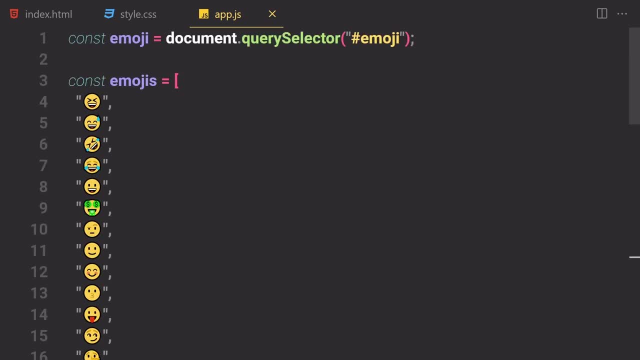 time. so that's why i provided all of these emojis, these emojis, these emojis by myself. if you want to get some other by myself, if you want to get some other by myself, if you want to get some other emojis, so feel free to choose whichever emojis. so feel free to choose whichever. 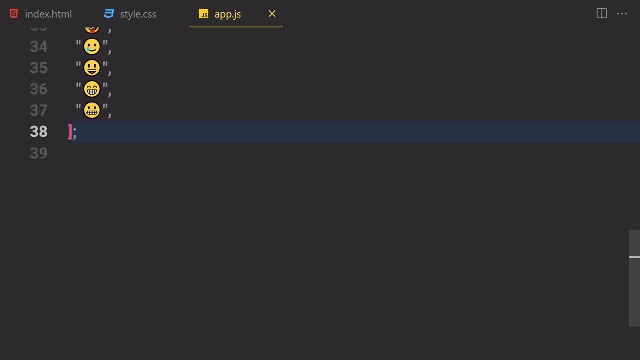 emojis. so feel free to choose whichever kind of emojis you like. but here you can kind of emojis you like. but here you can kind of emojis you like. but here you can just sort of mouse over, so once we mouse, just sort of mouse over, so once we mouse. 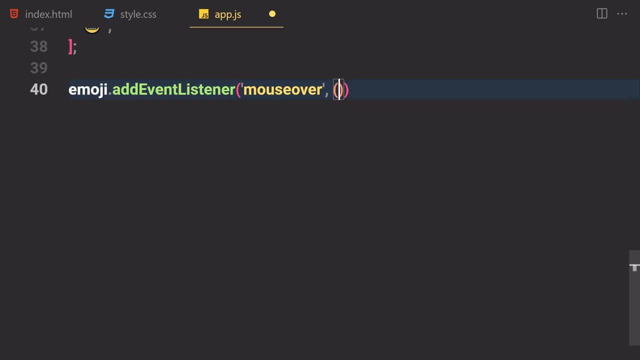 just sort of mouse over. so once we mouse over through that emoji, so what do we over through that emoji? so what do we over through that emoji? so what do we have to do? have to do, have to do. we want to just fire this um function. we want to just fire this um function. 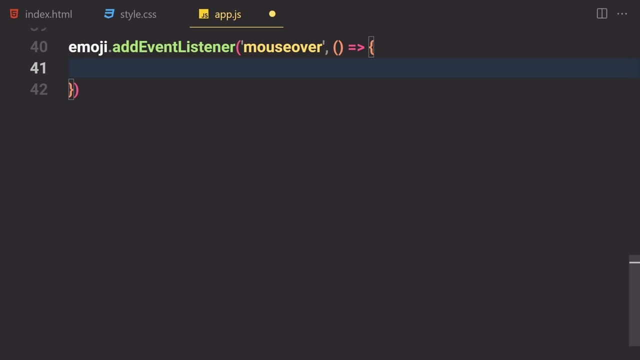 we want to just fire this um function right here. so what do we have to do right here? so what do we have to do right here? so what do we have to do? inside this uh function, we want to select. inside this uh function, we want to select. 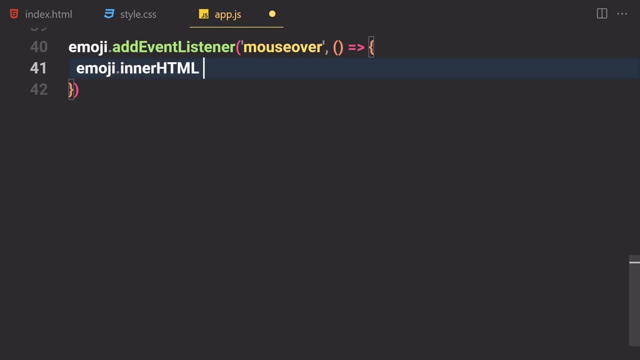 inside this uh function. we want to select that emoji and we want to just change that emoji and we want to just change that emoji and we want to just change the inner uh text of that emoji to these. the inner uh text of that emoji to these. the inner uh text of that emoji to these emojis. we want to get these emojis. 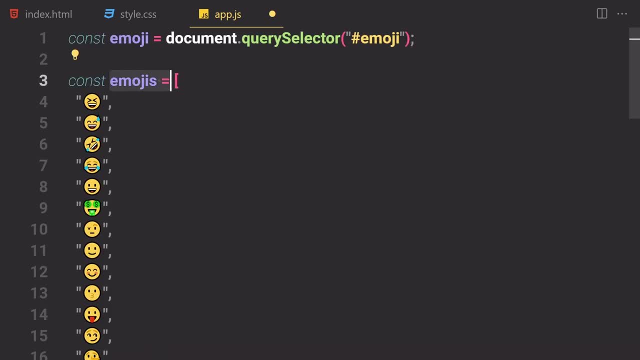 emojis. we want to get these emojis emojis. we want to get these emojis like a plural uh and which we store like a plural uh and which we store like a plural uh and which we store inside this emojis variable right here, inside this emojis variable right here, inside this emojis variable right here. so you want to get there and we want to. 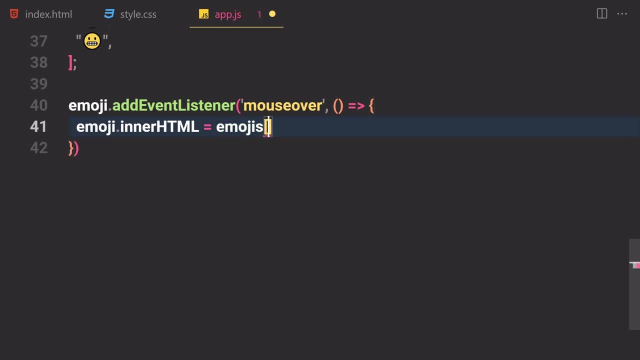 so you want to get there and we want to. so you want to get there and we want to just get a random emoji. so in javascript, just get a random emoji. so in javascript, just get a random emoji. so in javascript, if you want to get a random numbers, 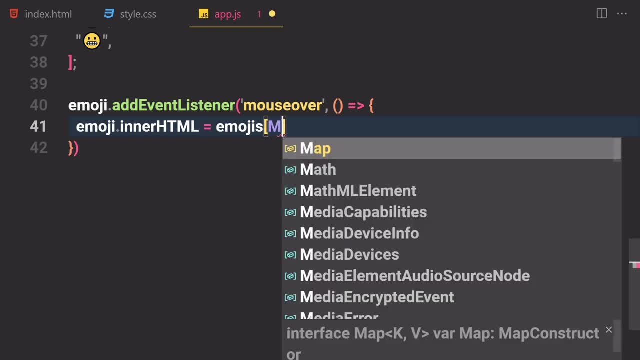 if you want to get a random numbers, if you want to get a random numbers, random colors, random emojis or whatever random colors, random emojis, or whatever random colors, emojis or whatever. so, first of all, you're going to be. so, first of all, you're going to be. 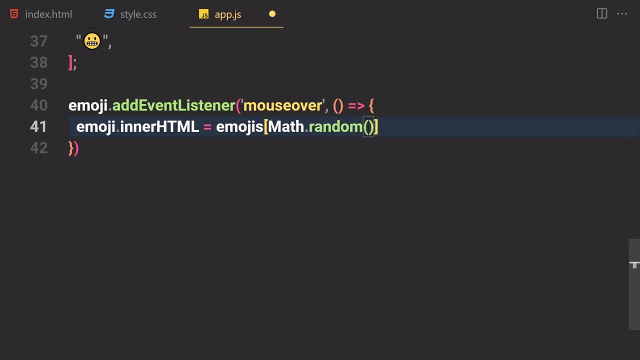 so first of all, you're going to be just writing a math dot random and then just writing a math dot random, and then just writing a math dot random, and then you're going to be just writing like: uh. you're going to be just writing like uh. 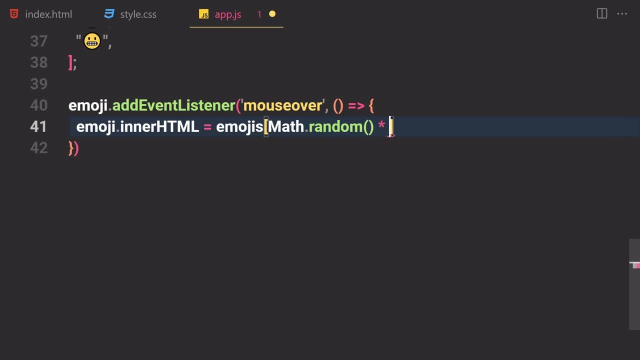 you're going to be just writing like: uh times, uh, whatever you want, so times and times. uh, whatever you want, so times and times, uh, whatever you want, so times. and then emojis, then emojis, then emojis. emojis- dot length. okay, and yeah, i'm emojis- dot length. okay, and yeah, i'm. 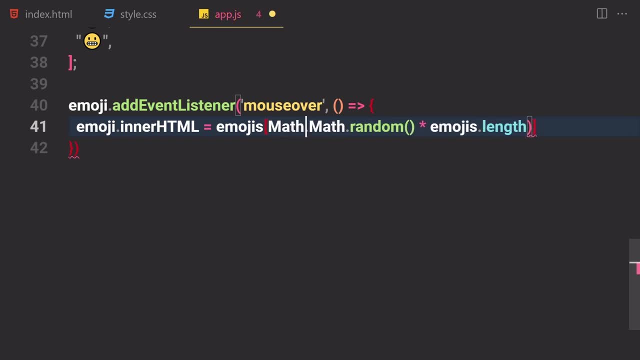 emojis: dot length. okay, and yeah, i'm gonna also wrap that inside. gonna also wrap that inside. gonna also wrap that inside: uh math dot floor as well. okay so, just uh math dot floor as well. okay so, just uh math dot floor as well. okay, so, just zoom out a bit and this everything. 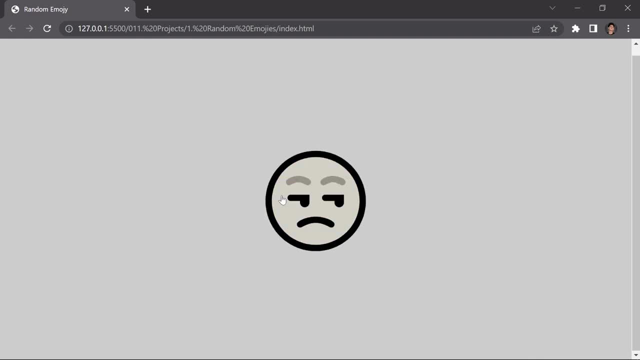 zoom out a bit and this everything. zoom out a bit and this everything looks like. and now if you save our file looks like. and now if you save our file looks like. and now, if you save our file, and now if i hover my mouse over to it, i 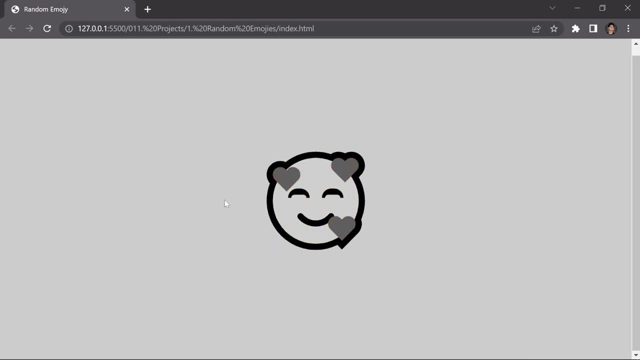 and now if i hover my mouse over to it, i. and now if i hover my mouse over to it, i know that was just a one-liner code, but know that was just a one-liner code, but know that was just a one-liner code, but it's now giving us different kind of 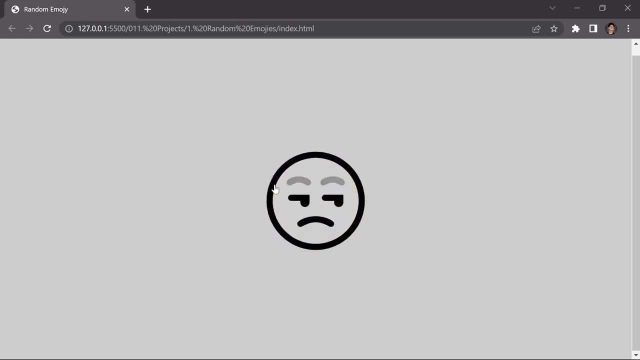 it's now giving us different kind of. it's now giving us different kind of frizzle right here and we can achieve frizzle right here and we can achieve frizzle right here and we can achieve different kind of different kind of different kind of result like we are now getting. 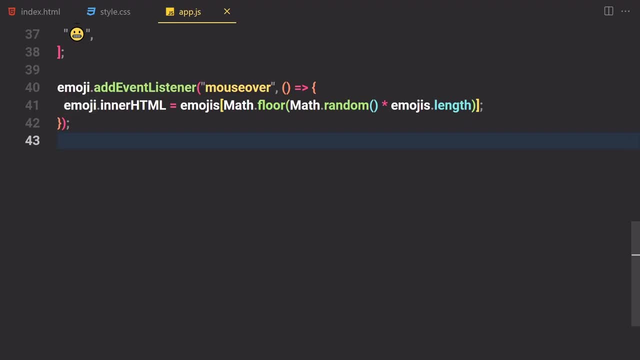 result. like we are now getting result. like we are now getting different kind of emojis first of all, different kind of emojis first of all. different kind of emojis first of all. we are just attaching our event listener. we are just attaching our event listener. we are just attaching our event listener of mouse move and once we hover our 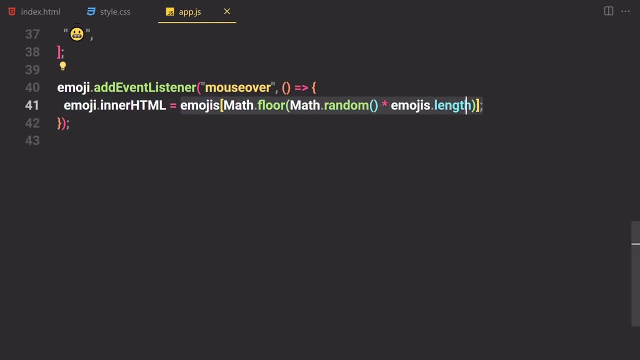 of mouse move and once we hover our of mouse move, and once we hover our mouse over to it, so that event will fire, mouse over to it, so that event will fire. mouse over to it, so that event will fire. and it will now give us random emojis. 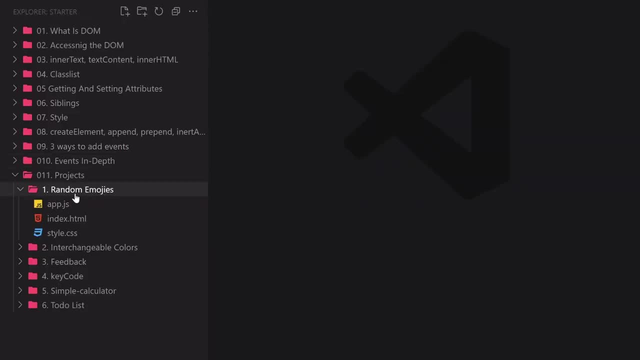 and it will now give us random emojis. and it will now give us random emojis. okay, so that's the first project. i'm okay, so that's the first project. i'm okay, so that's the first project. i'm going to, just going to, just going to just remove everything. 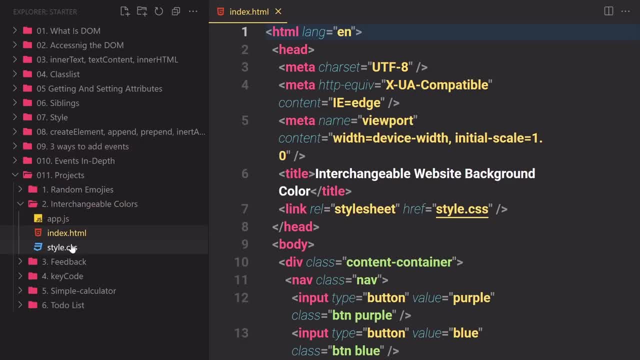 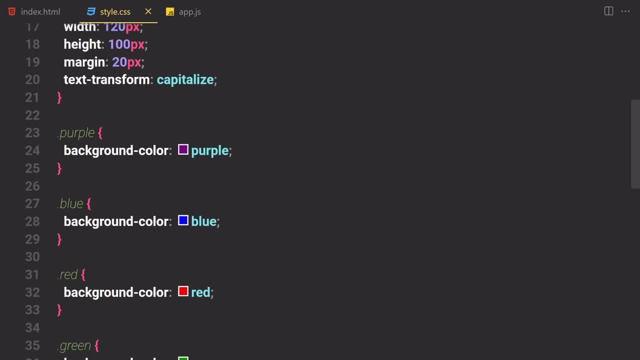 remove everything, remove everything. and now let's just get into our second. and now let's just get into our second. and now let's just get into our second project. by the way, i've already built project. by the way, i've already built project. by the way, i've already built this project, so you can check out all of. 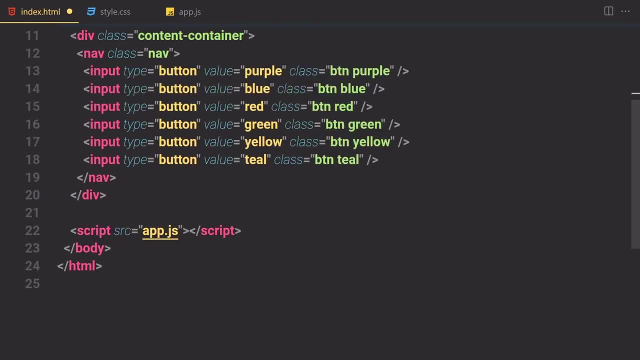 this project, so you can check out all of this project. so you can check out all of this project, plus 100 more projects on this project, plus 100 more projects on this project, plus 100 more projects on my youtube channel. so i have already my youtube channel. so i have already. 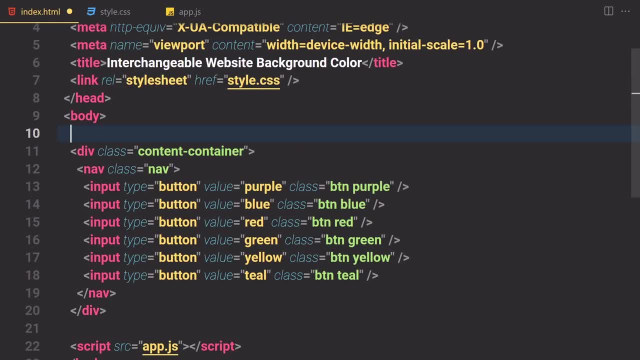 my youtube channel. so i have already built like 100 projects. so built like 100 projects. so built like 100 projects. so that will give you a huge and that will. that will give you a huge and that will. that will give you a huge and that will give you a lot, a lot practice. 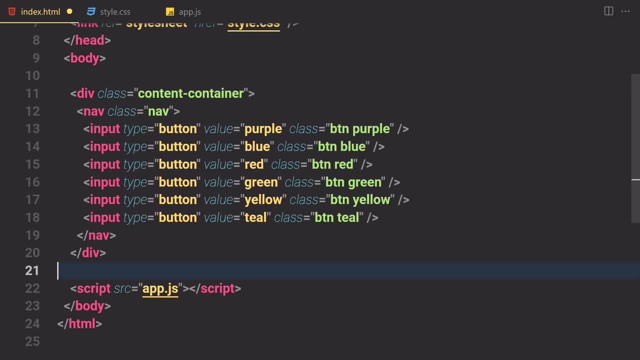 give you a lot, a lot practice. give you a lot, a lot practice if you want to sharpen your dom skills. so, if you want to sharpen your dom skills. so if you want to sharpen your dom skills. so i have already covered 100 projects on. i have already covered 100 projects on: 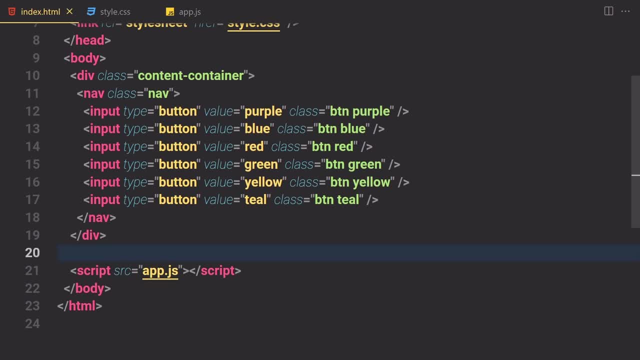 i have already covered 100 projects on my youtube channel. if you want to check my youtube channel, if you want to check my youtube channel, if you want to check that out, that out, that out anyway. so inside this html file, we just anyway. so inside this html file, we just. 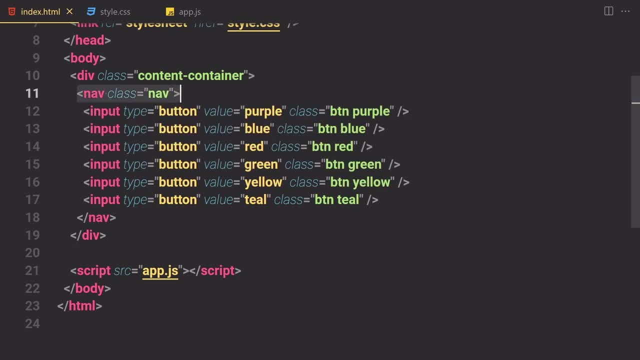 anyway. so inside this html file we just have our content container, have our content container, have our content container inside this content container. we have inside this content container we have inside this content container. we have our navigation, our navigation, our navigation. inside this navigation we have a few. 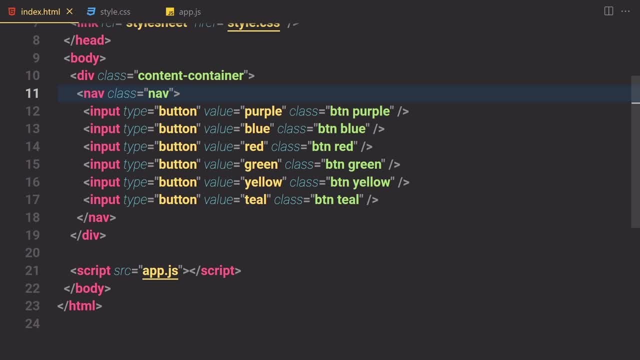 inside this navigation. we have a few inside this navigation. we have a few inputs right here like button button. all inputs right here like button button. all inputs right here like button button. all of them will be button of them will be button button. all of them will be button button. all right, green, yellow and teal. so this is. 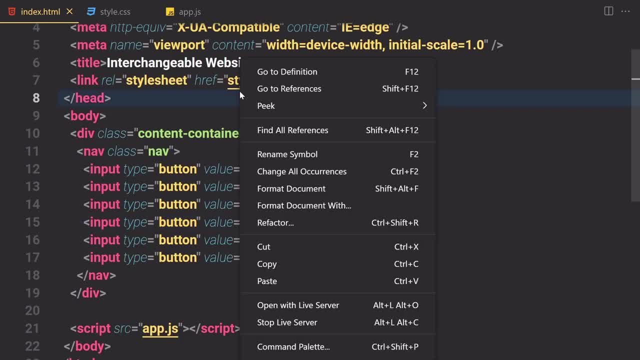 right: green, yellow and teal. so this is right: green, yellow and teal. so this is going to be it for the html. so what going to be it for the html? so what going to be it for the html? so what about the css? i'm going to just right. 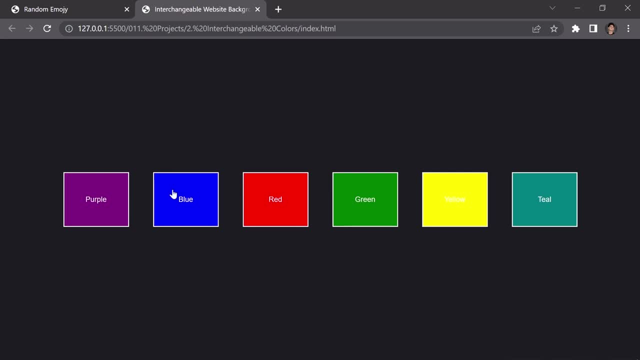 about the css. i'm going to just right about the css. i'm going to just right click on it and open it for the live click on it, and open it for the live click on it and open it for the live server. and this is how everything looks. 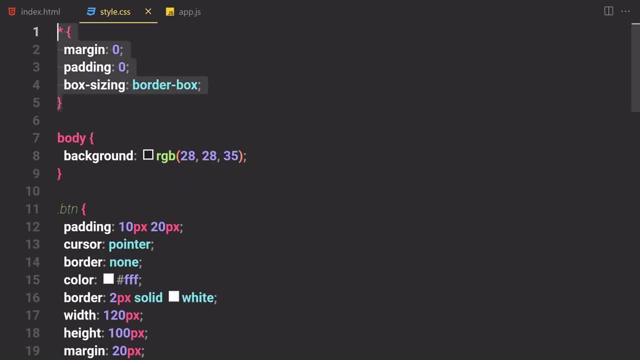 server and this is how everything looks server. and this is how everything looks like right now. so what about a css like right now? so what about a css like right now? so what about a css? we just first of all write our research. we just first of all write our research. 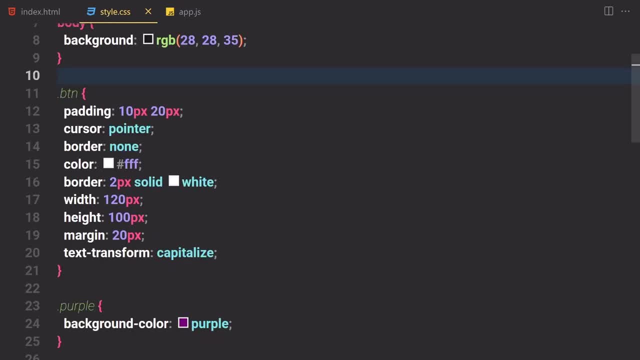 we just first of all write our research, then we change the background color. to then we change the background color, to then we change the background color to that kind of a bluish kind of a, that kind of a bluish kind of a, that kind of a bluish kind of a background. then we select all of our 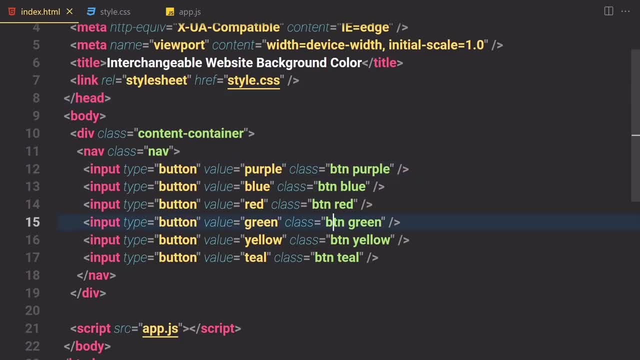 background, then we select all of our background, then we select all of our button, which we give this class right button, which we give this class right button, which we give this class right here, button, button, button, button and all here, button, button, button button and all here, button, button, button button and all of them. of them. of them, and we provide a padding of 10 pixel for, and we provide a padding of 10 pixel for, and we provide a padding of 10 pixel for a top and bottom. left and right will have a top and bottom, left and right will have. 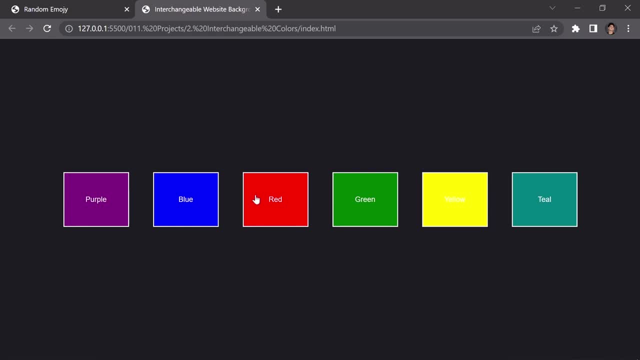 a top and bottom, left and right, will have 20 pixel cursor will be pointed like 20 pixel cursor will be pointed like 20 pixel cursor will be pointed like once i hover my mouse over to it. so once i hover my mouse over to it. so 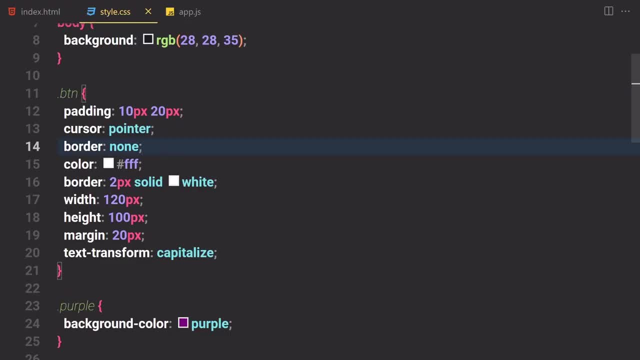 once i hover my mouse over to it. so cursor will be a pointer. we remove the cursor will be a pointer. we remove the cursor will be a pointer. we remove the background. i mean like the border, we background. i mean like the border, we background. i mean like the border. we change the color to totally wide the. 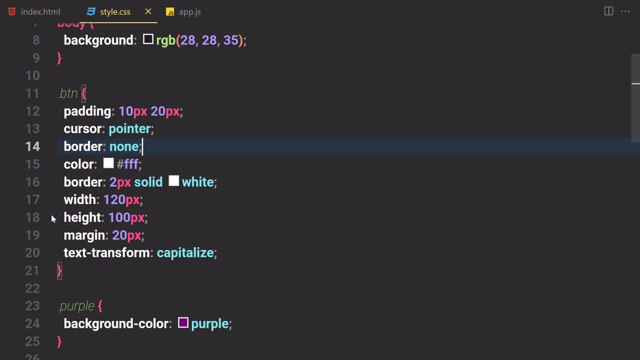 change the color to totally wide. the. change the color to totally wide. the border: we provide two pixels solid wide border. we provide two pixels solid wide border. we provide two pixels solid wide. we give a width of like 120 pixels the. we give a width of like 120 pixels the. 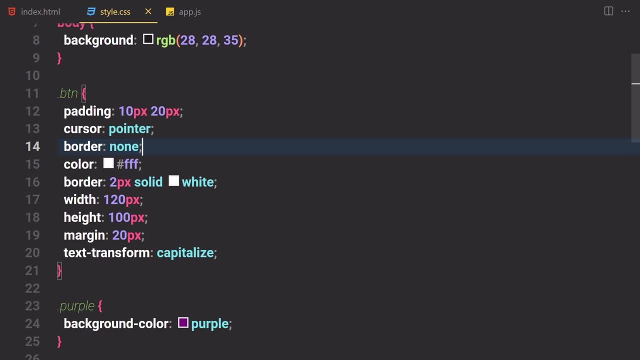 we give a width of like 120 pixels, the height will be 100 pixels pixel. the height will be 100 pixels pixel. the height will be 100 pixels pixel, the margin will be 20 pixel and text margin will be 20 pixel and text margin will be 20 pixel and text transform will be capitalized like so: 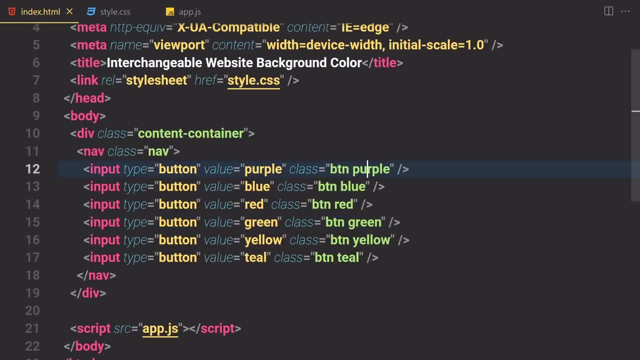 transform will be capitalized like so. transform will be capitalized like so: okay, then we select each of the color. okay, then we select each of the color. okay, then we select each of the color. like this one, so we have purple blue red. like this one, so we have purple blue red. 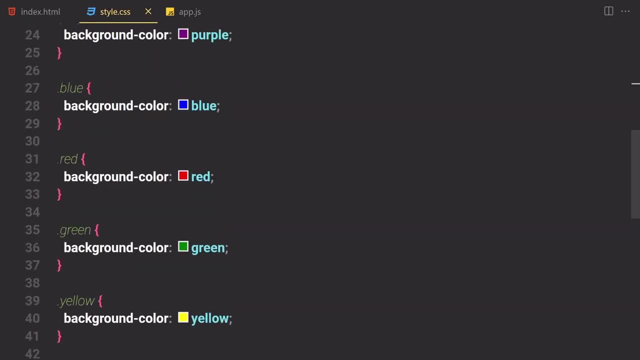 like this one. so we have purple, blue, red, green, yellow and teal. we select each of green, yellow and teal. we select each of green, yellow and teal. we select each of them and we just change the background them and we just change the background them and we just change the background color of them too, like that, and finally, 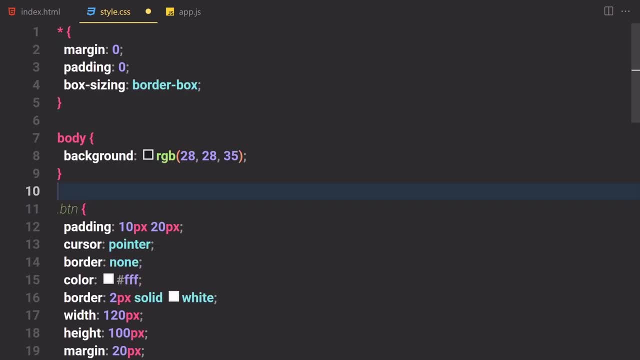 color of them, too, like that, and finally, color of them, too, like that, and finally, we just have our content container. i'm, we just have our content container. i'm, we just have our content container. i'm gonna have to put that up. gonna have to put that up. 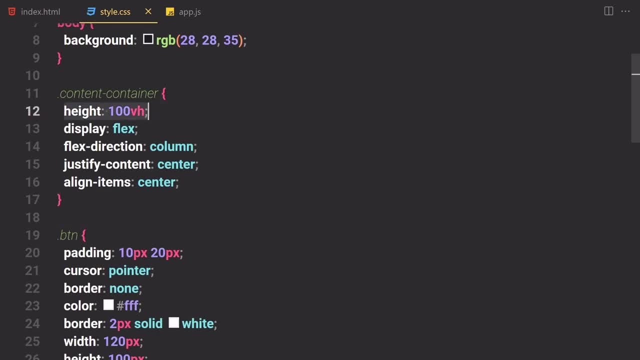 gonna have to put that up above, like here, and we just give a height above like here, and we just give a height above like here, and we just give a height of 100 vh and everything is now totally of 100 vh and everything is now totally. 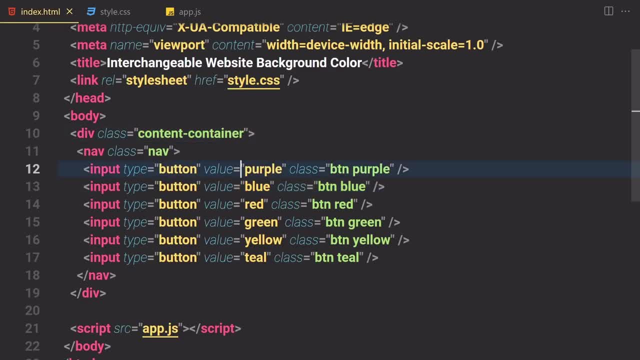 of 100 vh and everything is now totally at the center, and that's why we provide at the center, and that's why we provide at the center and that's why we provide this content container close to it, all this content container close to it, all this content container close to it. all right, so we are totally done with our. 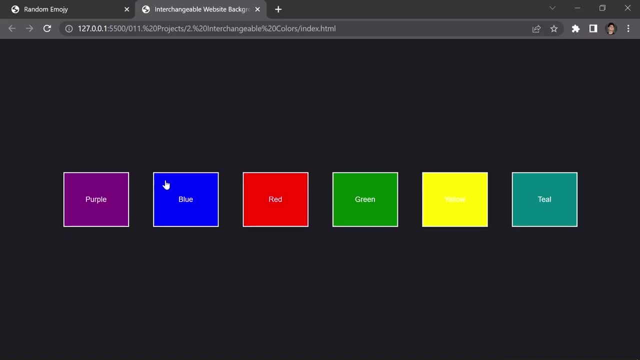 right. so we are totally done with our right. so we are totally done with our html and css. so now let's get into our html and css. so now let's get into our html and css. so now let's get into our javascript and provide our javascript and provide our. 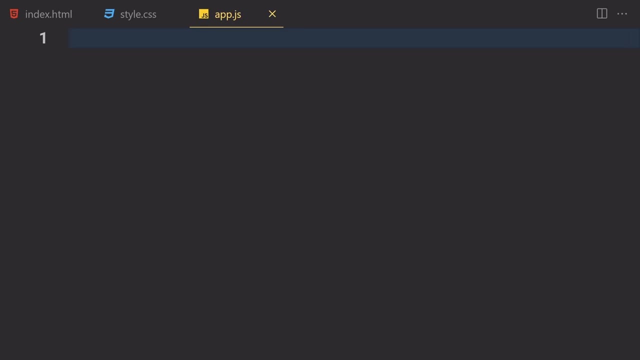 javascript and provide our interactivity to it. so what do we need? interactivity to it. so what do we need? interactivity to it? so what do we need for this project first of all? we would for this project first of all. we would for this project, first of all, we would need a button and a body. so, first of all, 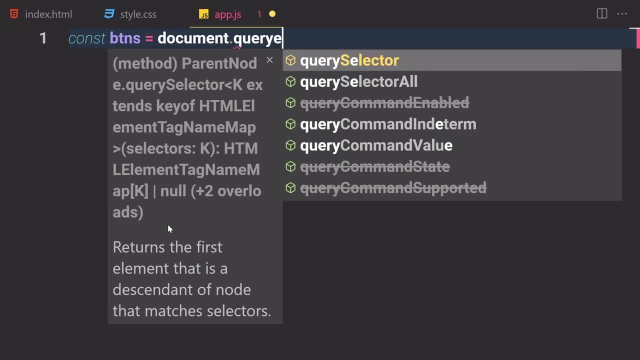 need a button and a body. so, first of all need a button and a body. so first of all, let's just get all of the buttons. so let's just get all of the buttons. so let's just get all of the buttons. so document, dot, query, selector, and all so. 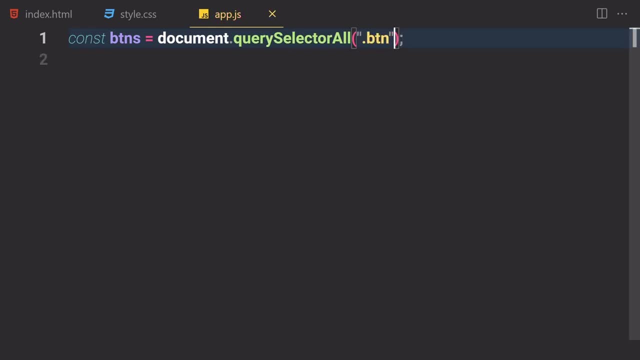 document dot- query selector and all. so document dot- query selector and all. so we have to just get all of these buttons. we have to just get all of these buttons. we have to just get all of these buttons. okay, not btns, but just a btn, so we have. 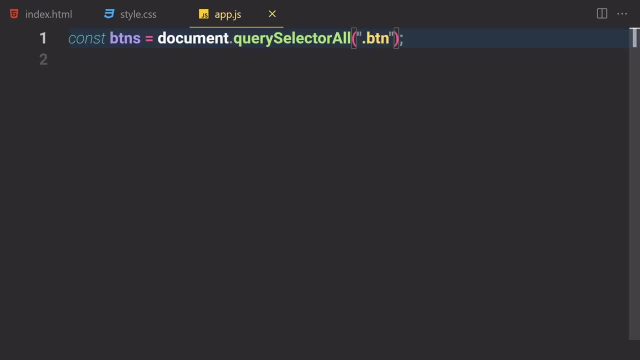 okay, not btns, but just a btn. so we have, okay, not btns, but just a btn. so we have this button, this button and all of this, this button, this button and all of this, this button, this button, this button and all of this button right here, okay so? button right here, okay. so button right here, okay. so the next thing we would need is a body. the next thing we would need is a body. the next thing we would need is a body. so you're going to be just writing. so you're going to be just writing. 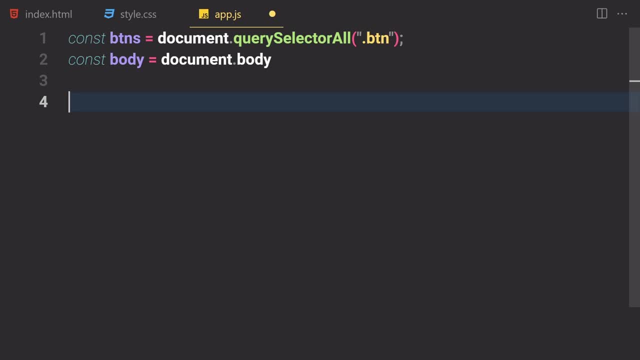 so you're going to be just writing document dot body. okay, so now word: document dot body. okay, so now word document dot body. okay, so now word selection is done now. what else do we? selection is done now. what else do we? selection is done now. what else do we have to do? we have to iterate over. 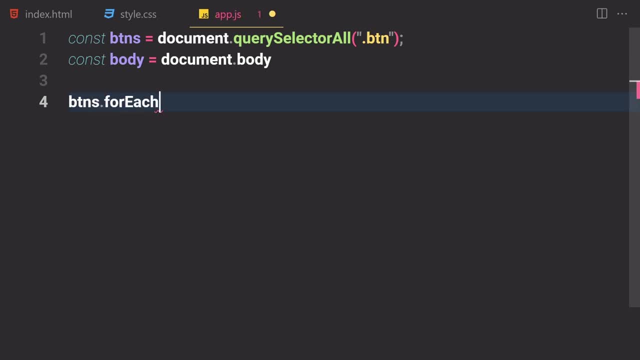 have to do, we have to iterate over, have to do, we have to iterate over through all of these buttons. so we want through all of these buttons, so we want through all of these buttons, so we want to just use like for each, to just use like for each. 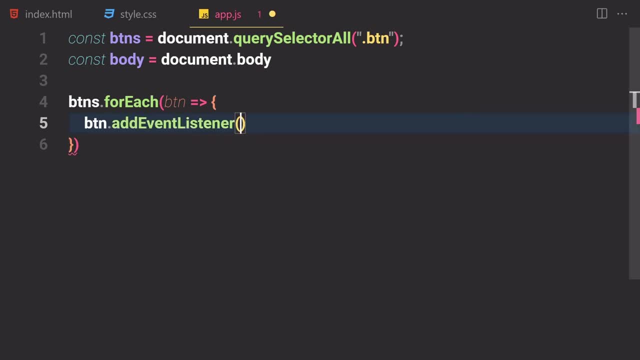 to just use, like for each. so for each button we want to attach. so for each button we want to attach. so for each button, we want to attach event listeners. so once we click on each event listeners, so once we click on each event listeners, so once we click on each button, so what do we want to do with? 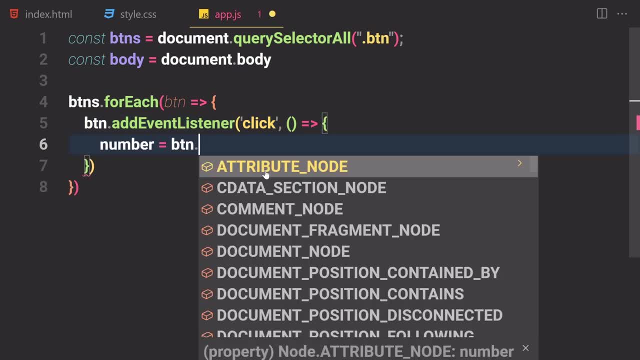 button. so what do we want to do with button? so what do we want to do with that? so you want to change the number that? so you want to change the number that. so you want to change the number to be like btn dot value- okay, so, to be like btn dot value- okay, so. 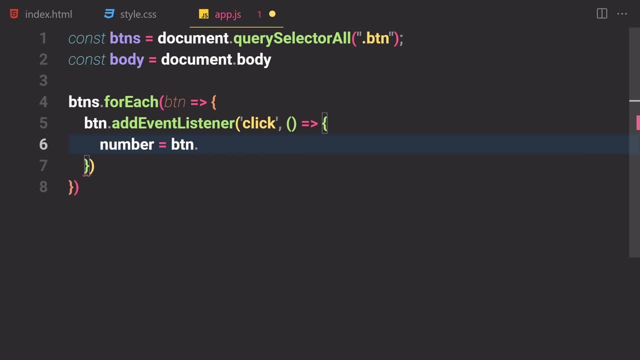 to be like btn dot value. okay, so whatever the button value is, we want to. whatever the button value is, we want to. whatever the button value is, we want to change that, to change that, to change that to a number. so this is writing value come a number. so this is writing value come. 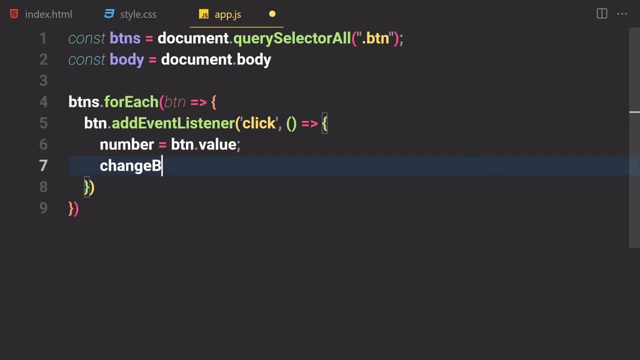 a number. so this is writing value. come on, man on man, on man, and also we are going to be using change and also we are going to be using change, and also we are going to be using change background. uh, yeah, change background background. uh, yeah, change background. 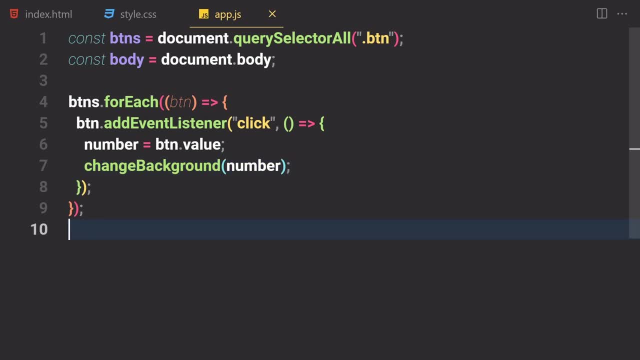 background. uh, yeah, change background function, which we are going to be function, which we are going to be function, which we are going to be creating just in a second, and we are creating just in a second and we are creating just in a second and we are going to be passing that number in there. 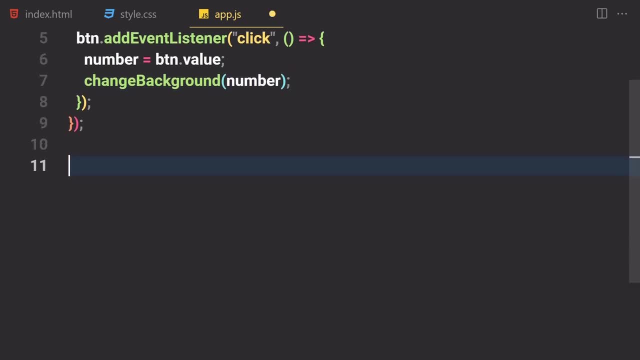 going to be passing that number in there. going to be passing that number in there, all right. so that's that, all right. so that's that, all right. so that's that. and now let's just create their function. and now let's just create their function. and now let's just create their function real quick, so i'm going to just create. 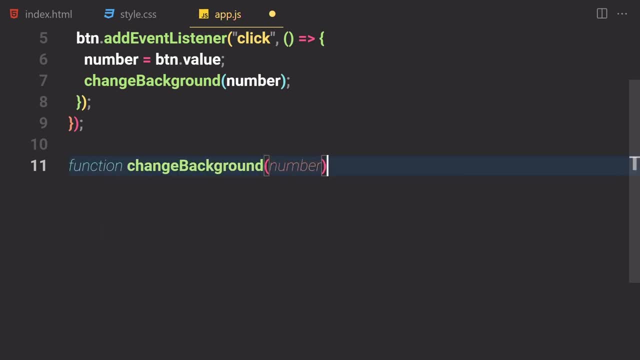 real quick, so i'm going to just create real quick. so i'm going to just create that function like change background, that function like change background, that function like change background, and it will also take the parameter of and it will also take the parameter of and it will also take the parameter of number. okay, so let's just write a body. 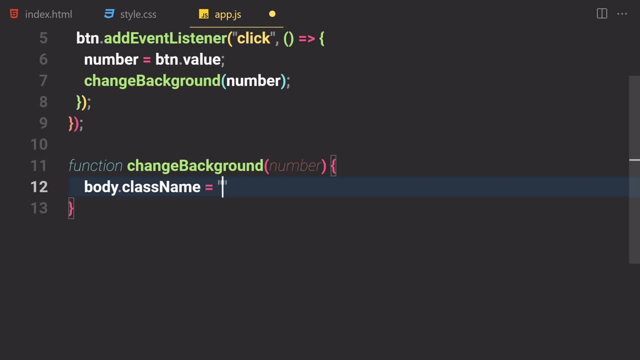 number. okay, so let's just write a body number. okay, so let's just write a body and the body class and the body class and the body class name will be now set to empty. clause name will be now set to empty clause name will be now set to empty clause because we don't want to provide any. 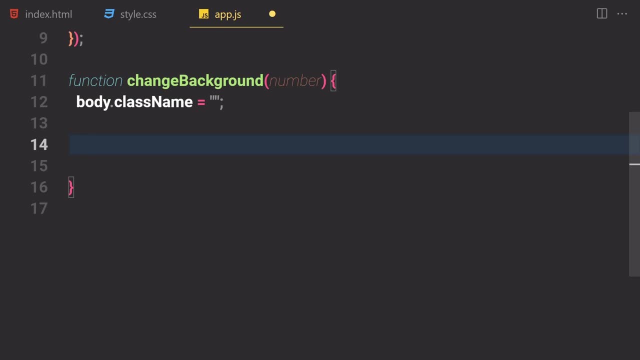 because we don't want to provide any, because we don't want to provide any clauses and stuff clauses and stuff clauses and stuff for the body. so now let's just use switch for the body. so now let's just use switch for the body. so now let's just use switch and cases and you can also use. and cases and you can also use and cases and you can also use uh fnl statement if you want to, and we uh fnl statement if you want to, and we uh fnl statement if you want to, and we are going to be working on the. 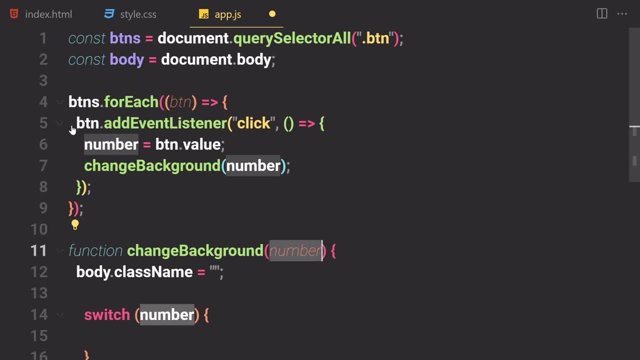 are going to be working on the are going to be working on the parameters. so, like this number which is parameters, so like this number which is parameters, so like this number which is coming from this one and we are going to coming from this one and we are going to 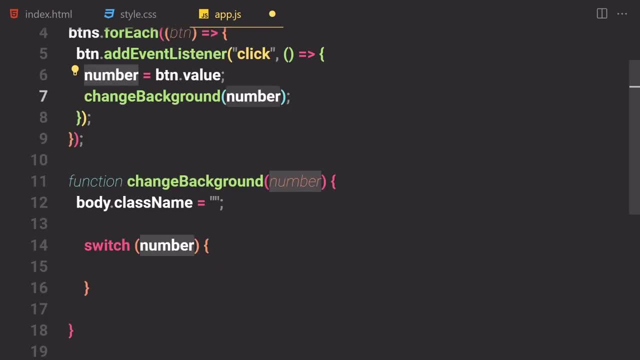 coming from this one and we are going to be passing the button value inside this. be passing the button value inside this. be passing the button value inside this: change number unlike change background change number unlike change background change number unlike change background. right here, okay, so you get the idea. so 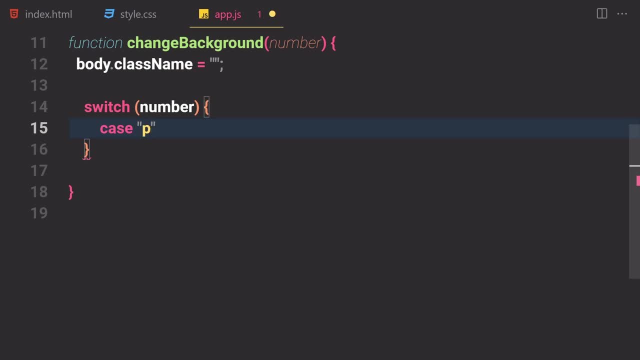 right here. okay, so you get the idea. so right here, okay, so you get the idea. so now we have to write our first case. like now, we have to write our first case. like now: we have to write our first case like purple, if the color or the number is: 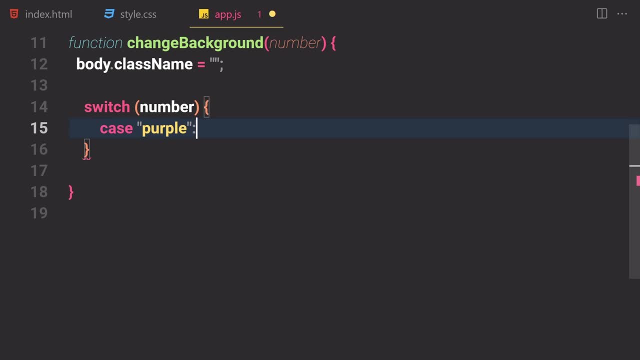 purple, if the color or the number is purple. if the color or the number is purple, so p-u-r-p-l-e like so purple. so p-u-r-p-l-e like so purple. so p-u-r-p-l-e like so. uh, oh, you know what. instead of number, 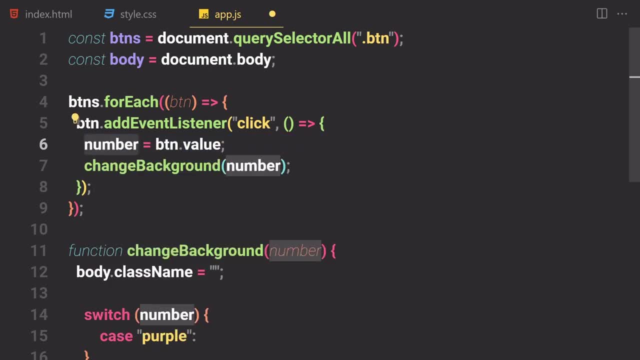 uh, oh, you know what, instead of number? uh, oh, you know what, instead of number, it should be a color, isn't it? so i'm? it should be a color, isn't it? so i'm? it should be a color, isn't it? so i'm going to just change that to: i'm going 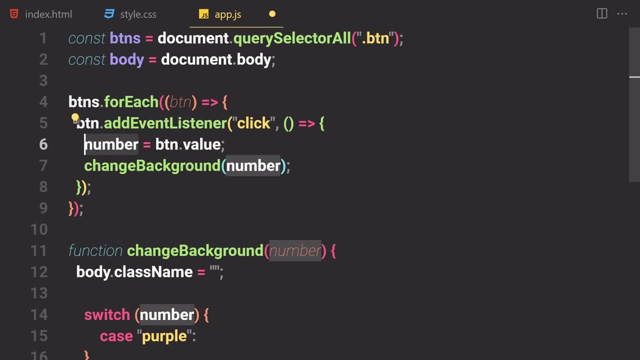 going to just change that to. i'm going going to just change that to. i'm going to hit f2, to hit f2, to hit f2. okay, it's not taking that f2, so i'm okay, it's not taking that f2, so i'm. 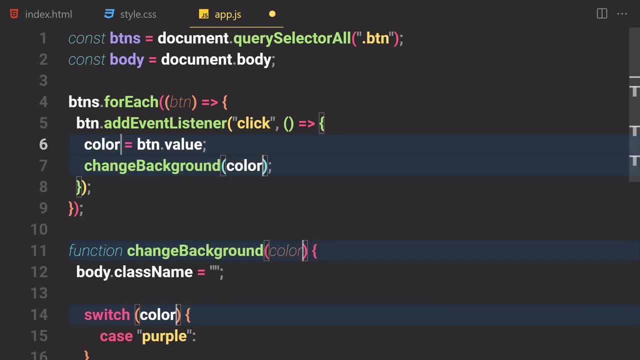 okay, it's not taking that f2, so i'm going to select that manually. it should going to select that manually. it should going to select that manually. it should be a color. i guess that color would be be a color. i guess that color would be be a color. i guess that color would be fine. why the hell do i just write? 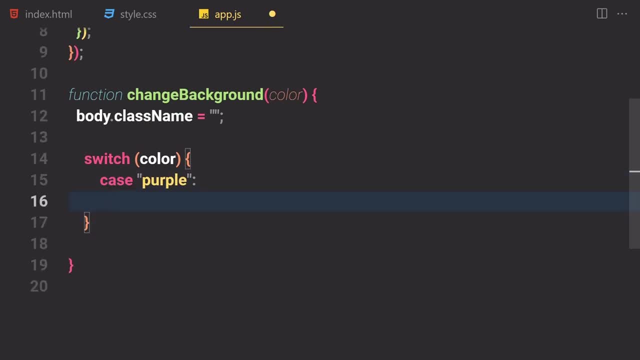 fine. why the hell do i just write fine, why the hell do i just write number? if the color is uh purple, so we number. if the color is uh purple, so we number. if the color is uh purple, so we want to just set the body. want to just set the body. 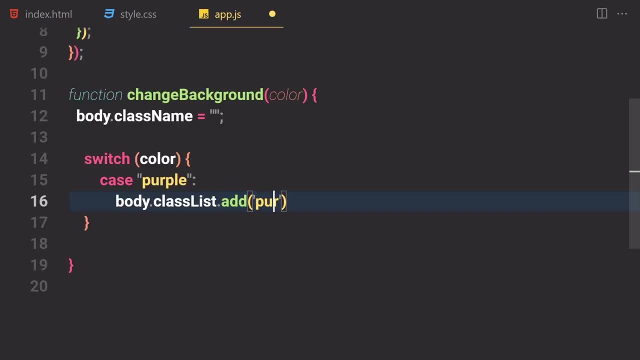 want to just set the body dot, class list dot. and we want to dot class list dot. and we want to dot class list dot and we want to attach this purple, attach this purple, attach this purple. p-u-r-p-l-e clause to it, so p-u-r-p-l-e clause to it, so. 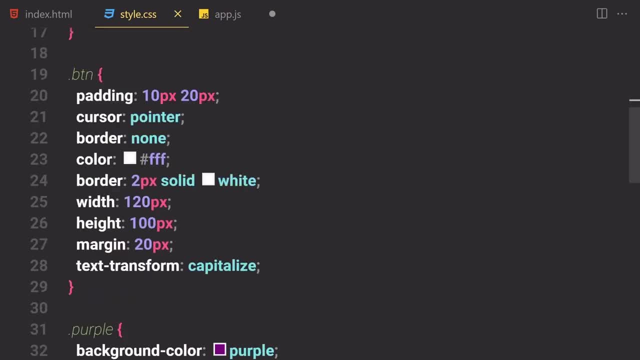 p-u-r-p-l-e clause to it. so, and then we want to break out from this, and then we want to break out from this, and then we want to break out from this loop, and we have this loop, and we have this loop and we have this purple clause right here. so, right here. 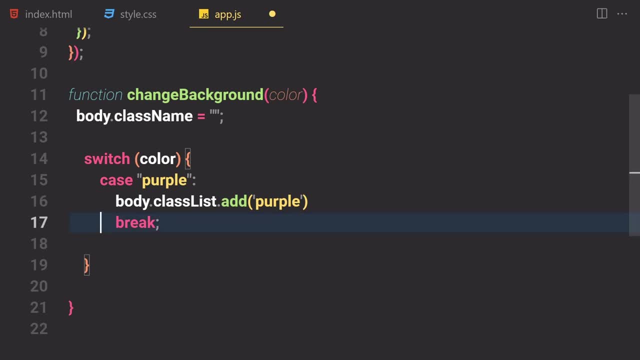 purple clause right here, so right here, purple clause right here, so right here. you can see that, you can see that, you can see that and we want to break out from this loop and we want to break out from this loop, and we want to break out from this loop. and you know what i'm gonna? oh, you know. 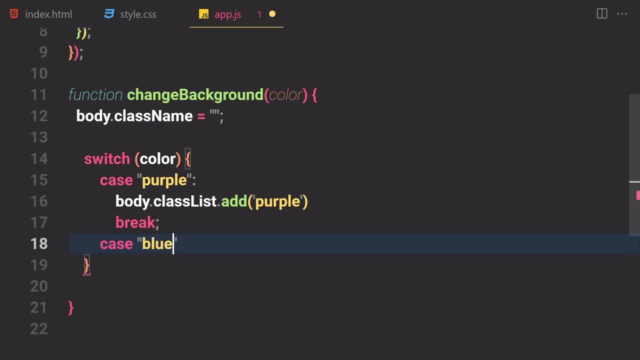 and you know what i'm gonna. oh, you know, and you know what i'm gonna. oh, you know, i'm not gonna do duplicating there. so i'm not gonna do duplicating there. so i'm not gonna do duplicating there. so then we have another case for a blue. so 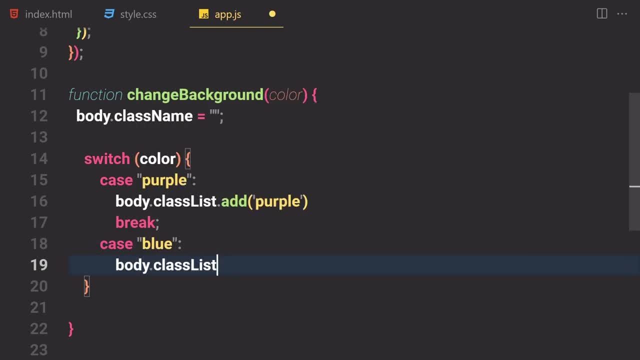 then we have another case for a blue, so then we have another case for a blue. so if our case is blue, so what do we have? if our case is blue? so what do we have if our case is blue? so what do we have to do? we want to just write a body dot. 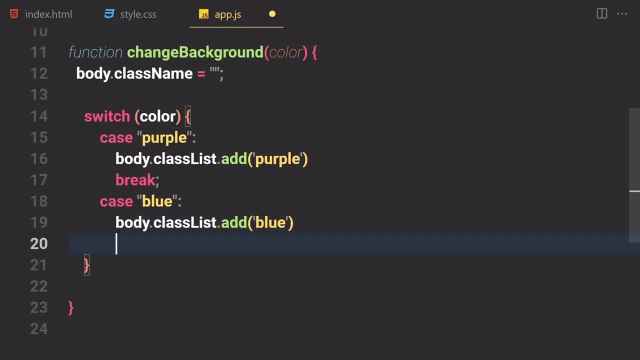 to do? we want to just write a body dot to do. we want to just write a body dot: clause list dot: add the color of blue. clause list dot: add the color of blue. clause list dot: add the color of blue to it. and we already wrote that inside. 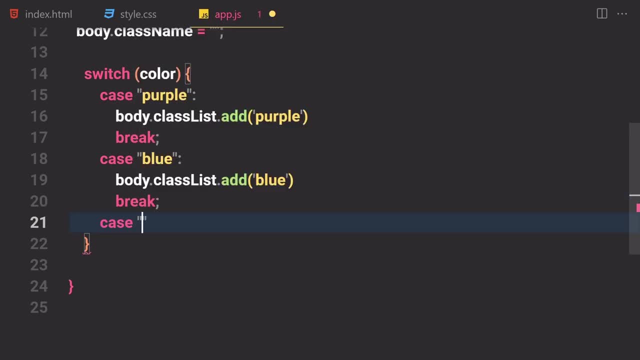 to it and we already wrote that inside to it and we already wrote that inside word css. if you want to check that out, word css. if you want to check that out, word css, if you want to check that out, so you can. and then, if the case is set, 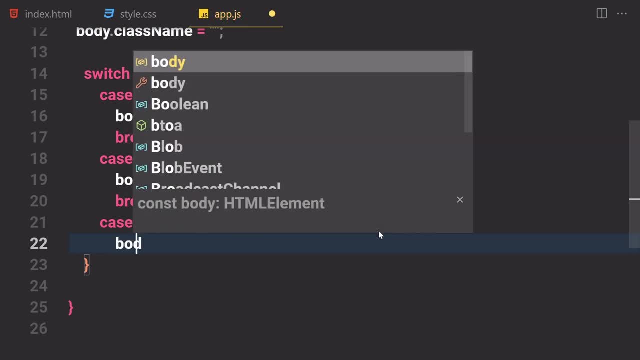 so you can. and then, if the case is set, so you can. and then, if the case is set to rent, so you want to just write um to rent, so you want to just write um to rent. so you want to just write um body dot. uh. clause list: dot add. 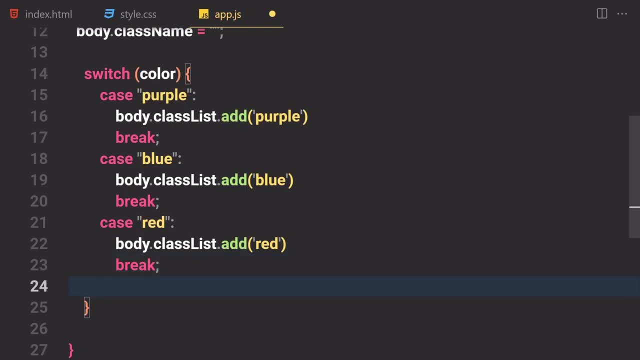 body dot- uh- clause list dot. add body dot- uh- clause list dot. add the color of red to it, and we also want the color of red to it, and we also want the color of red to it, and we also want to break out from this loop. and then we 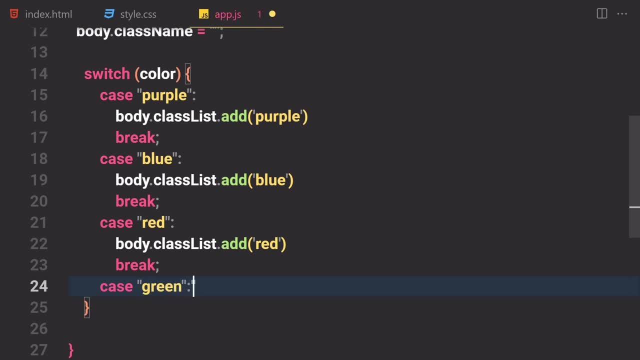 to break out from this loop, and then we to break out from this loop, and then we have a case of green. okay, so let's just have a case of green. okay, so, let's just have a case of green. okay, so let's just write a green case. 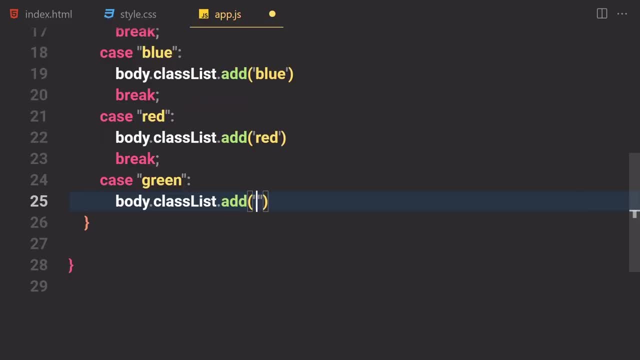 write a green case. write a green case and body dot clause list dot. add. and body dot clause list dot- add. and body dot clause list dot. add uh green color to it and we also want uh green color to it and we also want uh green color to it and we also want to break out from it. 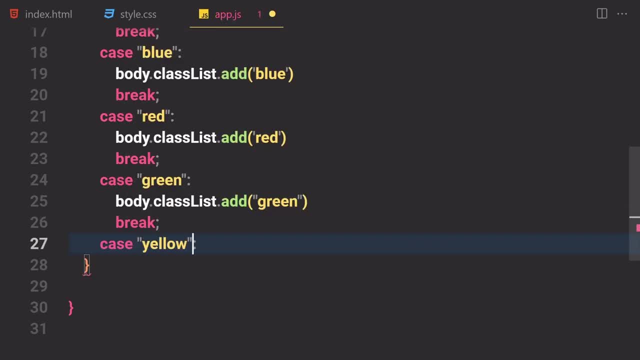 to break out from it. to break out from it. then we have another case for a yellow, then we have another case for a yellow, then we have another case for a yellow. yellow like so yellow, like, so yellow, like so. embody that clause list: dot. add uh. embody that clause list: dot. add uh. 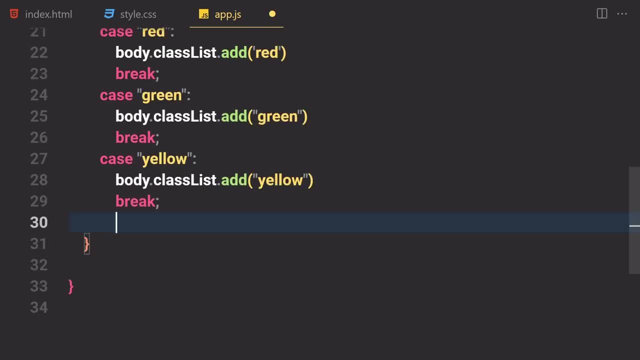 embody that clause list: dot. add uh. color of yellow and breakout. color of yellow and breakout. color of yellow and breakout. and finally we just have a lost case for, and finally we just have a lost case for, and finally we just have a lost case for the teal color. 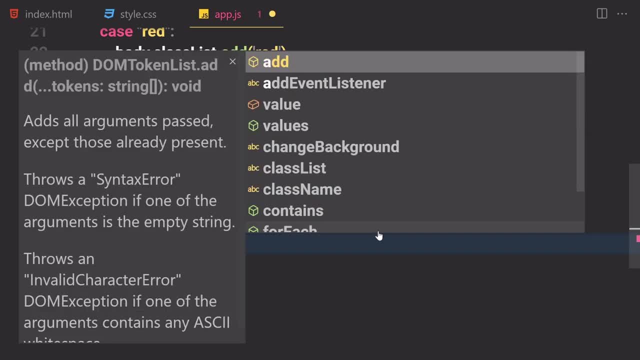 the teal color, the teal color, and we are going to be just setting the and we are going to be just setting the and we are going to be just setting the body dot clause list dot add. body dot clause list dot add. body dot clause list dot add. and we are going to be changing the color. 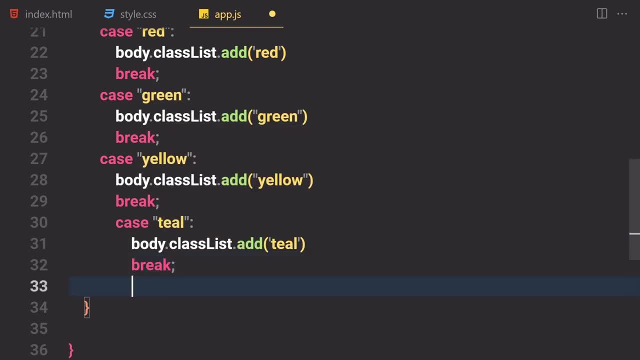 and we are going to be changing the color. and we are going to be changing the color to be teal and let's just break out to be teal and let's just break out to be teal and let's just break out from this loop break. and we also want to. 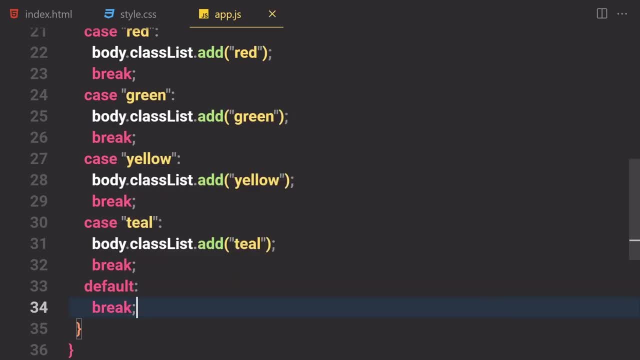 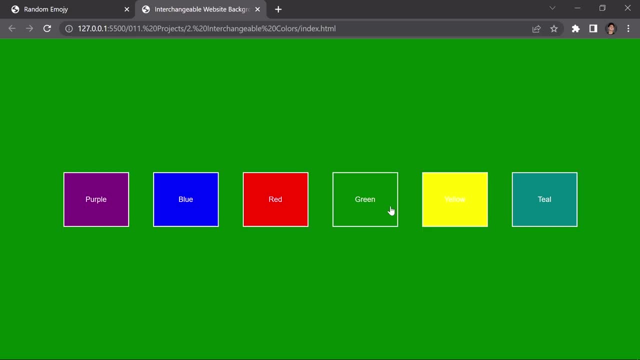 from this loop break and we also want to. from this loop break and we also want to. everything is working, but we have a few. everything is working, but we have a few. everything is working, but we have a few cases. we can also use if and l statement. 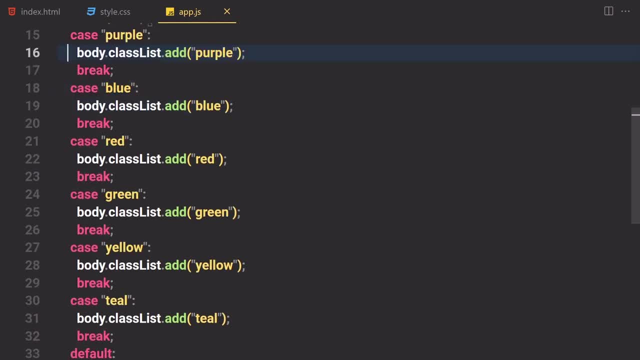 cases. we can also use if and l statement cases. we can also use if and l statement for that, for that, for that if you want to, but i guess their if you want to, but i guess their if you want to, but i guess their switching cases are looking a bit better. 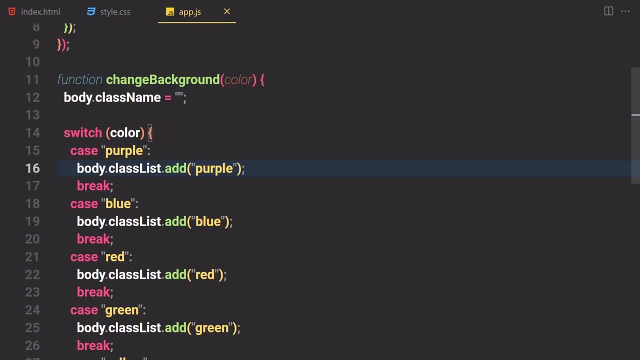 switching cases are looking a bit better. switching cases are looking a bit better, so i'm going to just go with that. so, if so, i'm going to just go with that. so if so, i'm going to just go with that. so if the case is purple, so you want to just the case is purple, so you want to. just the case is purple, so you want to just change the background color to be purple. change the background color to be purple. change the background color to be purple. if the case is blue, so you want to. if the case is blue, so you want to. 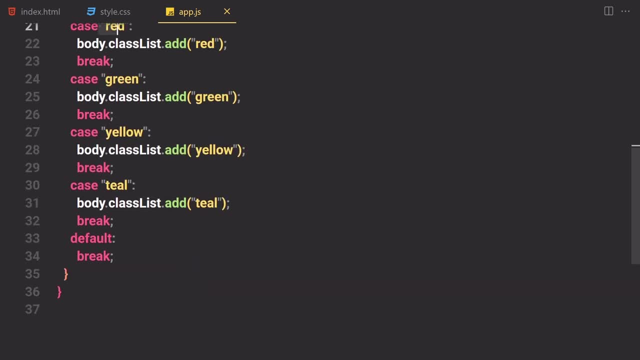 if the case is blue. so you want to change that to blue, change that to blue, change that to blue, to the red to green yellow teal, and to the red to green yellow teal, and to the red to green yellow teal, and finally, we just, finally, we just. 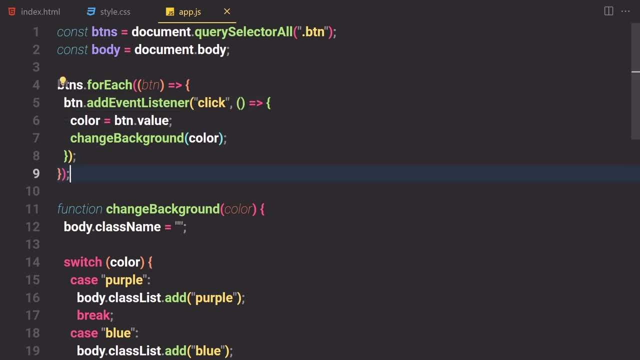 finally, we just want to break out from the loop. okay, so want to break out from the loop. okay, so want to break out from the loop. okay, so this is the second project, this is the second project, this is the second project and we are now totally done with our 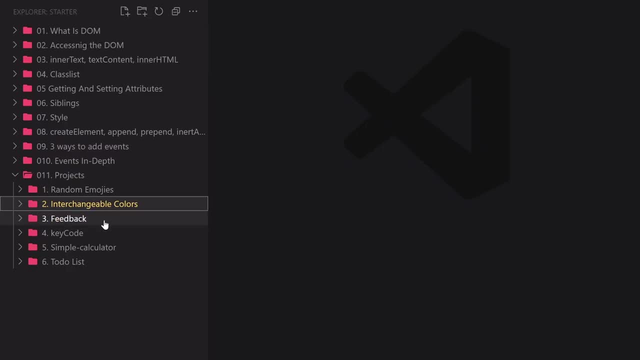 and we are now totally done with our. and we are now totally done with our second project as well. second project as well. second project as well. now let's just start working on our now. let's just start working on our now, let's just start working on our third project. so i'm going to just 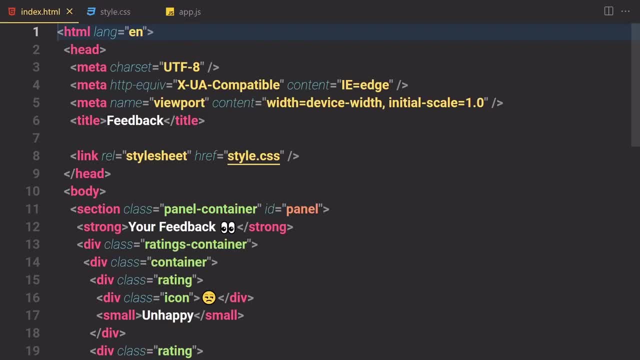 third project, so i'm going to just third project, so i'm going to just open all of these files, open all of these files, open all of these files, and we are going to be building a and we are going to be building a and we are going to be building a feedback ui. so, first of all, let me just 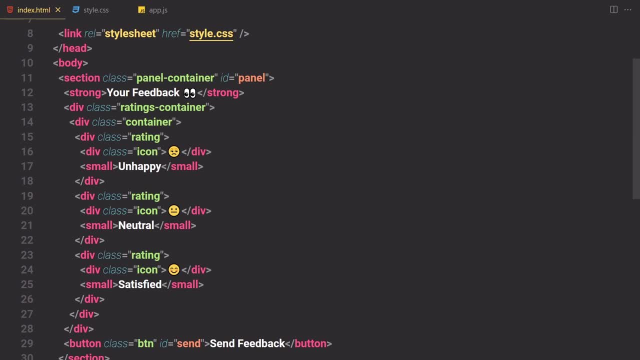 feedback ui. so first of all, let me just feedback ui. so first of all, let me just show you the feedback ui. show you the feedback ui. show you the feedback ui: coding, so we have html. so for html, we. coding, so we have html. so for html, we. 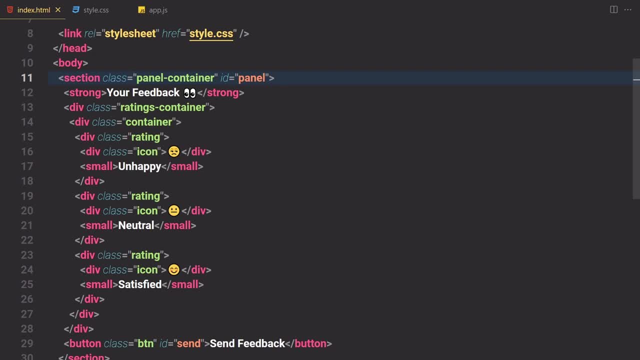 coding. so we have html. so for html, we have a section with the class of panel, have a section with the class of panel, have a section with the class of panel container and we also have id of panel container and we also have id of panel container and we also have id of panel. then we have our strong uh. then we have 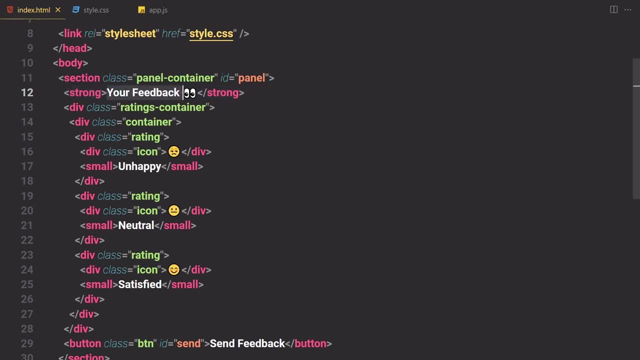 then we have our strong uh, then we have, then we have our strong uh, then we have our strong tag, our strong tag, our strong tag, with your feedback, uh as level, with your feedback, uh as level, with your feedback, uh as level. and then we have our div with the class. 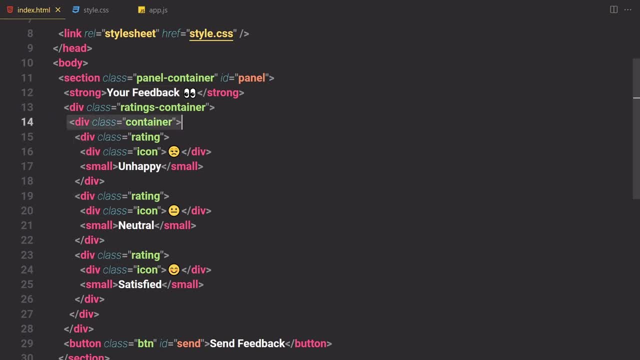 and then we have our div with the class, and then we have our div with the class of rating container. and inside this of rating container and inside this of rating container, and inside this rating container, we just have our rating container, we just have our rating container. we just have our singular rating. i mean like singular. 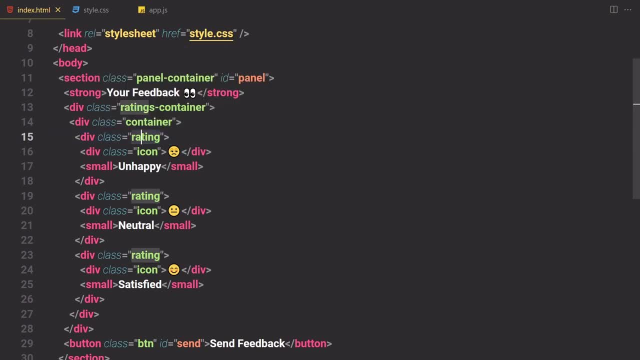 singular rating. i mean like singular. singular rating i mean like singular container, and then we have different container and then we have different container and then we have different kind of ratings for it, like we have a kind of ratings for it, like we have a kind of ratings for it, like we have a rating, then we have an icon for that. 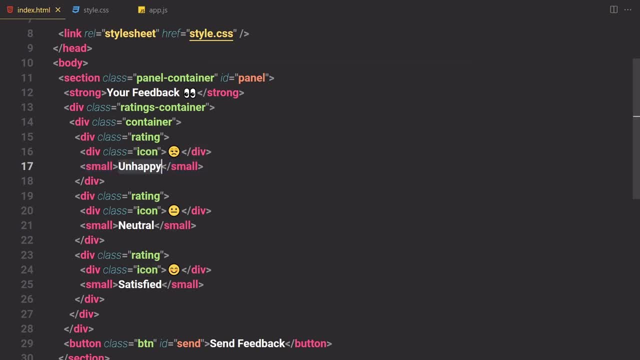 rating, then we have an icon for that rating, then we have an icon for that specific rating, specific rating, specific rating- and we have a small tag of unhappy then and we have a small tag of unhappy, then and we have a small tag of unhappy, then we have a neutral. 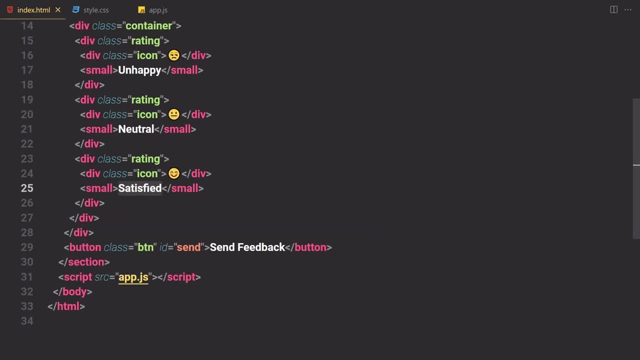 we have a neutral, we have a neutral, and then we have a satisfied right here, and then we have a satisfied right here, and then we have a satisfied right here, okay. so finally we just have a button at. okay. so finally we just have a button at. okay. so finally we just have a button at the bottom. 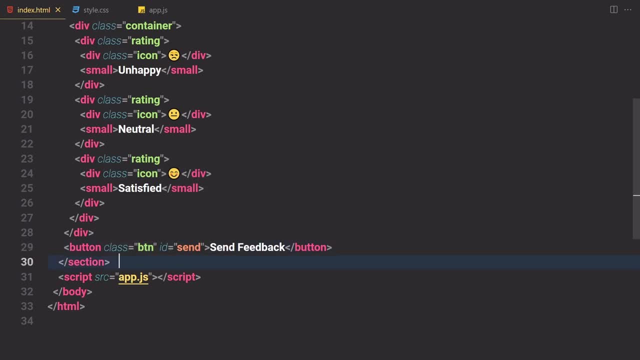 the bottom. the bottom and the class will be button and the id and the class will be button and the id and the class will be button and the id will be sent and it will just say like will be sent. and it will just say like will be sent and it will just say like: send feedback. and now, if you right click, 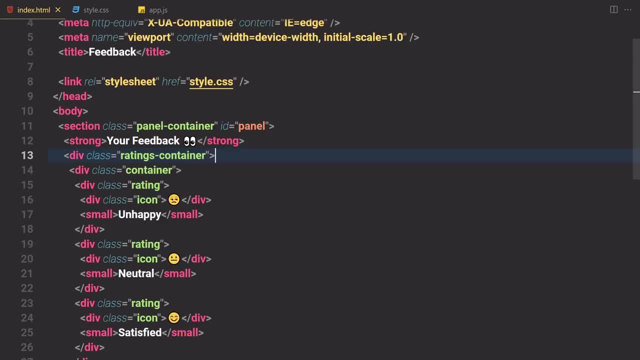 send feedback. and now, if you right click, send feedback, and now, if you right click on that, and open it with live server on that, and open it with live server on that, and open it with live server. and once again, i'm saying that once again, and once again, i'm saying that once again. 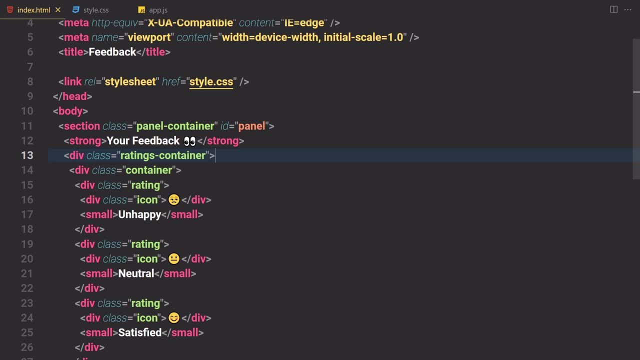 and once again i'm saying that once again, if you want more practice on the dom, so if you want more practice on the dom, so if you want more practice on the dom, so i have, i have i have 100 projects on my youtube channel, 100 projects on my youtube channel. 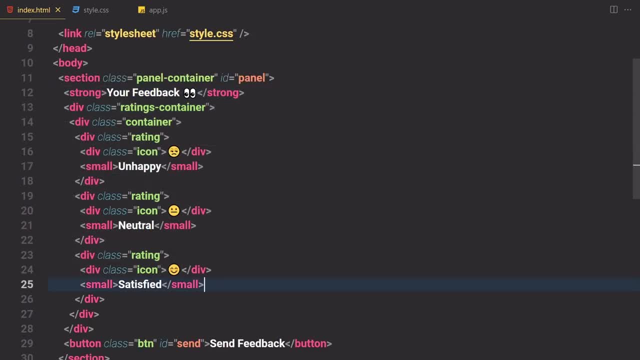 100 projects on my youtube channel, which also include all of these projects, which also include all of these projects, which also include all of these projects. like i've already covered all of this, like i've already covered all of this, like i've already covered all of this project in a real great depth in my 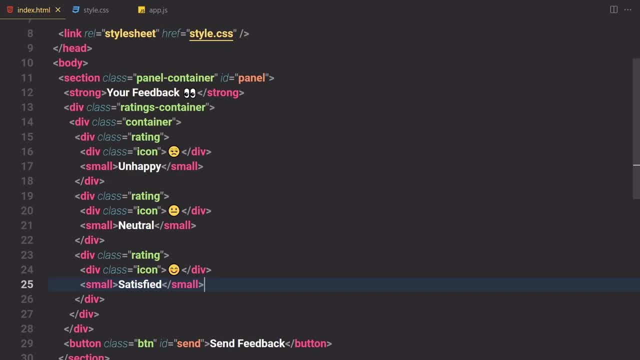 project in a real great depth in my project, in a real great depth in my course. like 100 projects in 100 days course. like 100 projects in 100 days course. like 100 projects in 100 days course, if you want to check that out. 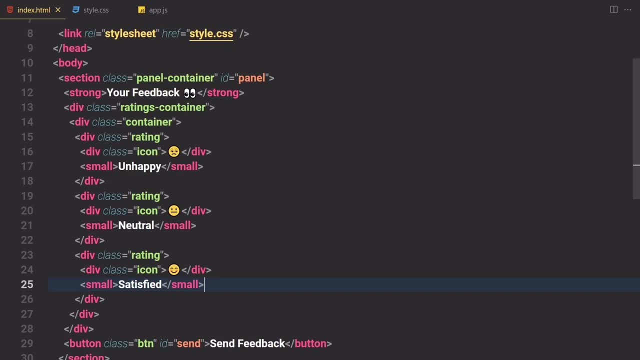 course, if you want to check that out course, if you want to check that out, i'm just skipping through all of this. i'm just skipping through all of this. i'm just skipping through all of this html because i have already have a html, because i have already have a. 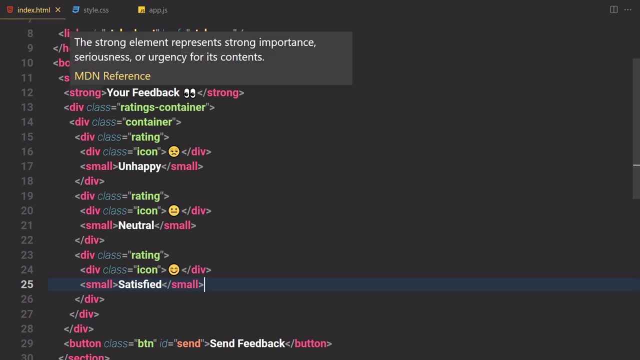 html, because i have already have a radius like entire section of the videos. radius like entire section of the videos. radius like entire section of the videos on these uh projects as well. so if you on these uh projects as well, so if you on these uh projects as well, so if you want to check that out, that would be a. 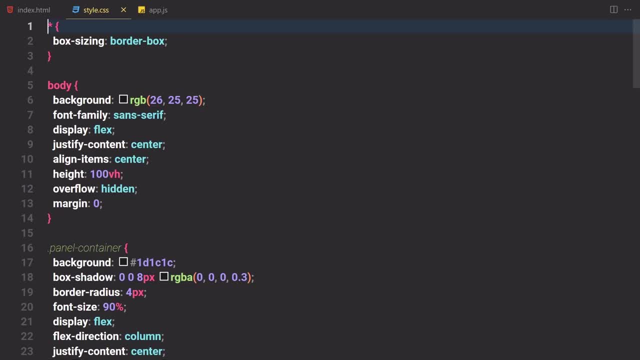 want to check that out. that would be a great fit for you. and then we have a great fit for you, and then we have a great fit for you, and then we have a style share, style share, style share. so we have, like, first of all reset, then 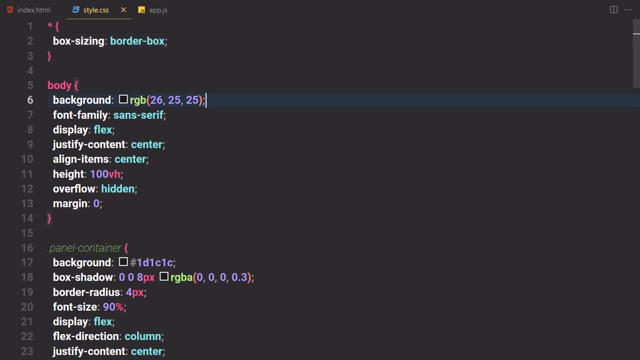 so we have like first of all reset then. so we have like first of all reset. then we have a body, we just give him a color. we have a body, we just give him a color. we have a body we just give him a color of. uh, we just change the color to kind. 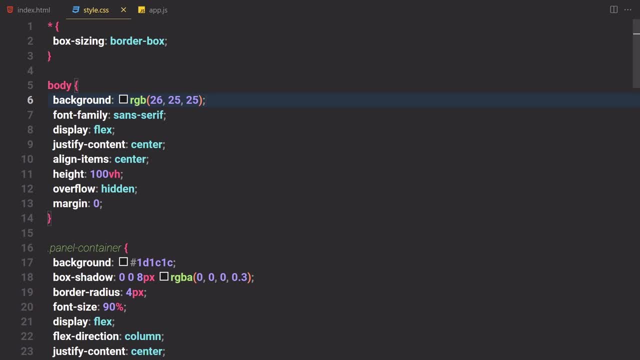 of uh, we just change the color to kind of. uh, we just change the color to kind of a blackish, kind of a blue color, then of a blackish kind of a blue color, then of a blackish kind of a blue color. then we have four family of center serve and 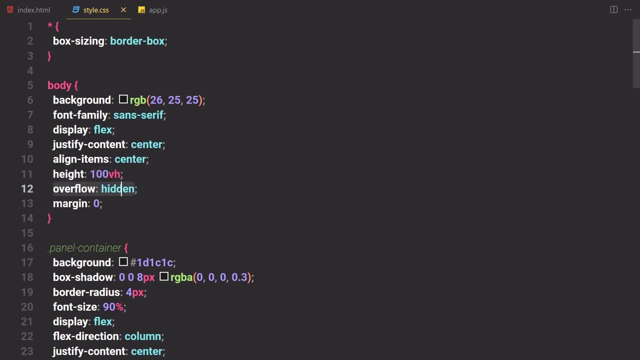 we have four family of center serve and we have four family of center serve and we want to center everything we provide. we want to center everything we provide. we want to center everything we provide. the height of 100 vh, we want to overflow the height of 100 vh, we want to overflow. 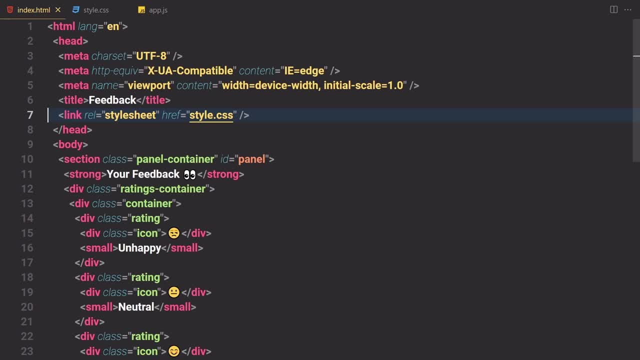 the height of 100 vh. we want to overflow. hidden and margin will be zero. then we hidden and margin will be zero. then we hidden and margin will be zero. then we have our panel container, which is this. have our panel container, which is this: have our panel container, which is this panel container. so we just give him a. 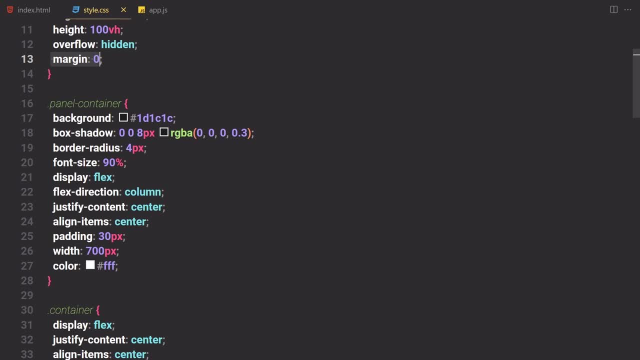 panel container. so we just give him a panel container, so we just give him a background of that 1d1c kind of a background, of that 1d1c kind of a background of that 1d1c kind of a bluish kind of background. then we also 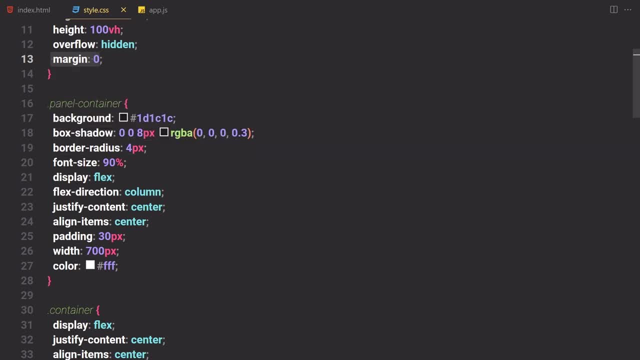 bluish kind of background, then we also bluish kind of background, then we also give him the box shadow and we also give give him the box shadow and we also give give him the box shadow and we also give him a border radius of 4 pixel and we 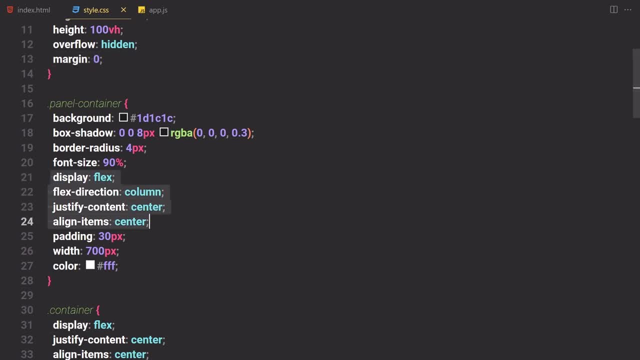 him a border radius of 4 pixel and we him a border radius of 4 pixel, and we have font size of 90 percent, and we also have font size of 90 percent, and we also have font size of 90 percent, and we also set out everything to the center and we 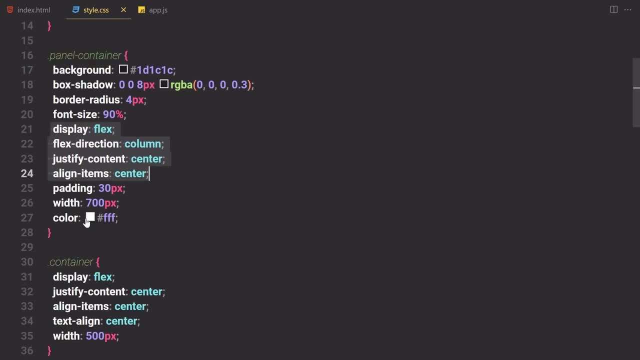 set out everything to the center and we set out everything to the center and we have a padding of 30 pixel width will be have a padding of 30 pixel width will be have a padding of 30 pixel width will be 700 pixel and the color will be totally. 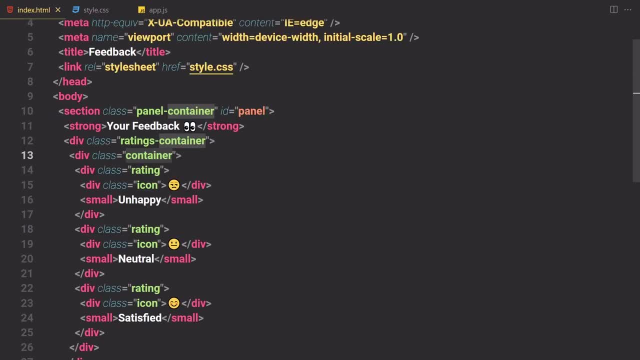 700 pixel and the color will be totally 700 pixel and the color will be totally white. then we have our container, which white. then we have our container, which white. then we have our container, which is that container right here which is. is that container right here which is. 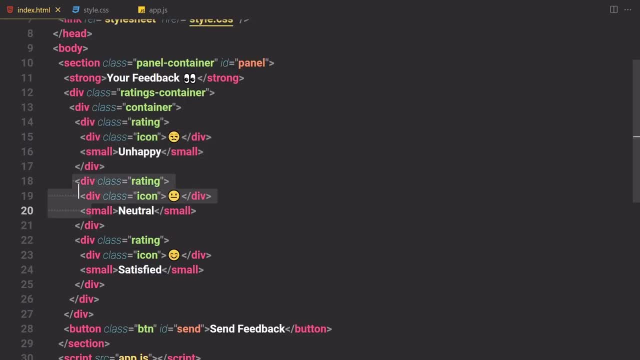 is that container right here which is holding all of these ratings. so like we holding all of these ratings, so like we holding all of these ratings, so like we have rating one, rating two, and then we have rating one, rating two, and then we have rating one, rating two, and then we have a rating three right here. okay, so 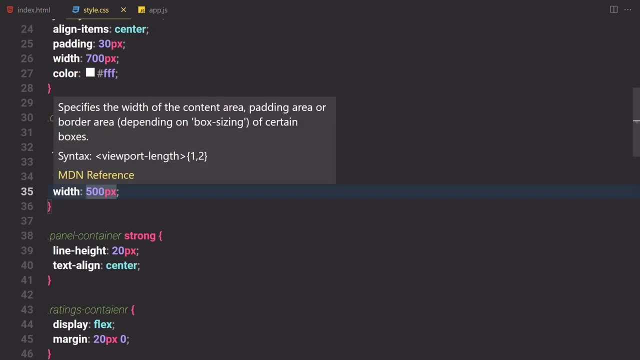 have a rating three right here, okay. so have a rating three right here, okay. so then we are just first of all centering, then we are just first of all centering, then we are just first of all centering everything and we give the max width of 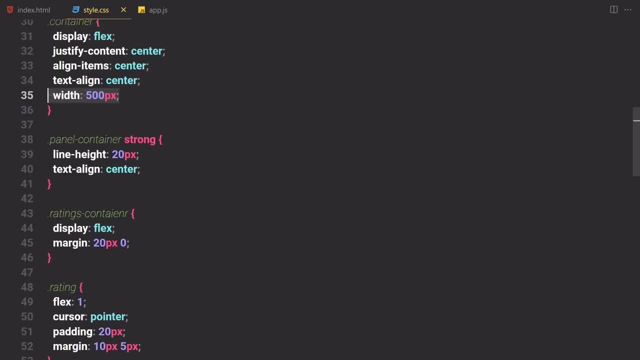 everything and we give the max width of everything and we give the max width of 500 pixel on there, then we have a panel 500 pixel on there, then we have a panel 500 pixel on there, then we have a panel container and which is holding a strong 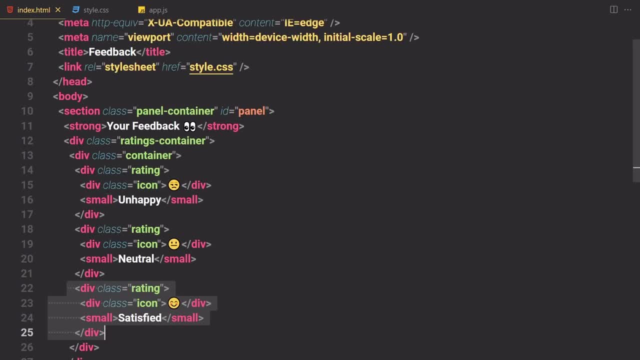 container and which is holding a strong container, and which is holding a strong, which is the come on strong. oh my god. which is the come on strong, oh my god. which is the come on strong, oh my god. all right, this is a small one. yeah this. all right, this is a small one, yeah this. 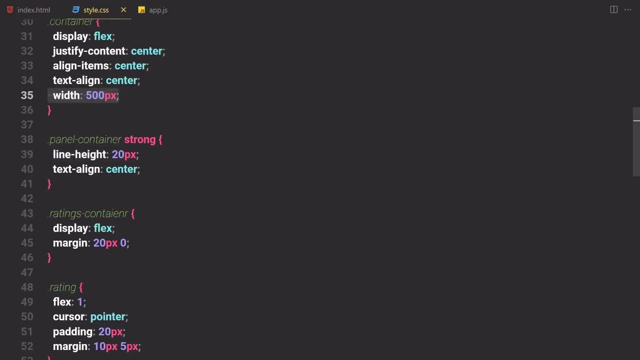 all right, this is a small one. yeah, this one your feedback. so we are just giving one your feedback. so we are just giving one your feedback. so we are just giving a line out of 20 pixel and text, a line out of 20 pixel and text. 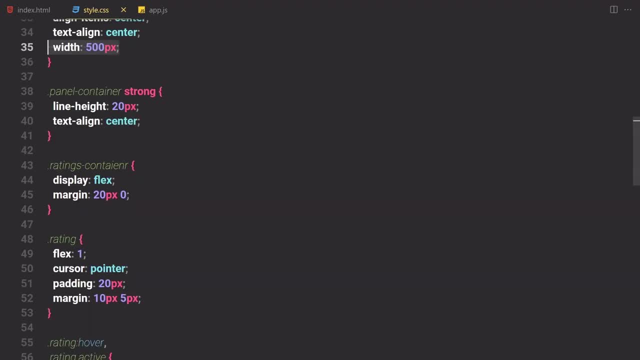 a line out of 20 pixel and text alignment will be totally centered. so alignment will be totally centered. so alignment will be totally centered. so it's now center. then we have a rating: it's now center. then we have a rating: it's now center. then we have a rating container- ratings container, which is this: 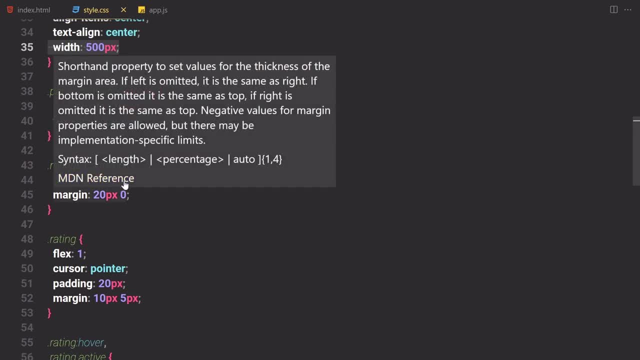 container ratings container, which is this container ratings container, which is this one, one one, and we're just using display of flex and we're just using display of flex and we're just using display of flex and margin of 20 pixel for top and bottom, and we're just using display of flex. 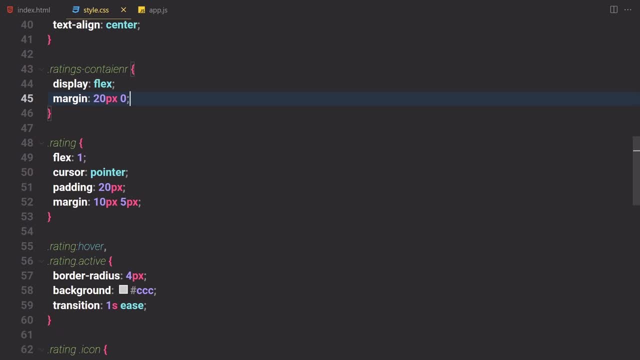 and we're just using display of flex, and for left and right we have a zero pixel, and for left and right we have a zero pixel, and for left and right we have a zero pixel. and then we have a rating- just a singular. and then we have a rating, just a singular. 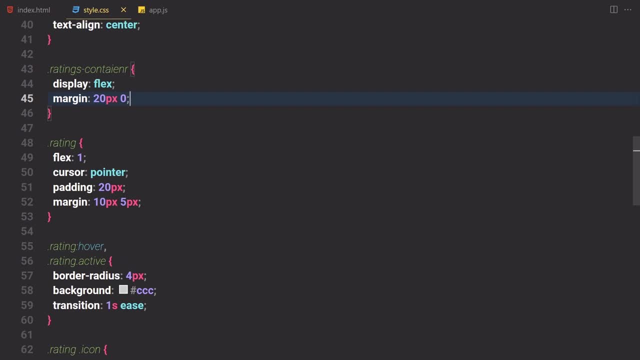 and then we have a rating, just a singular rating. which rating? which rating? which is that one we are just giving a flex? is that one we are just giving a flex? is that one? we are just giving a flex of one cursor pointer. padding will be 20. 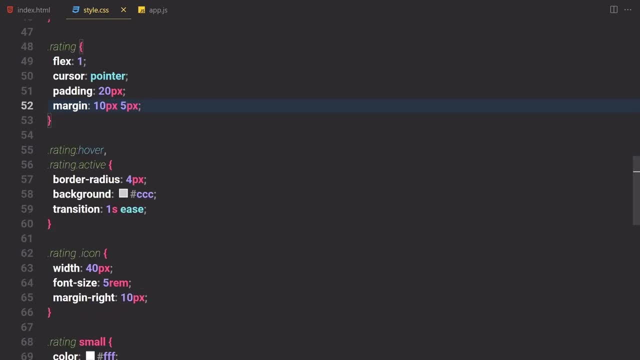 of one cursor pointer padding will be 20 of one cursor pointer padding will be 20 pixel margin. top and bottom will 20: 10 pixel margin. top and bottom will 20: 10 pixel margin. top and bottom will 20: 10 pixel pixel pixel. left and right will be five pixel and. 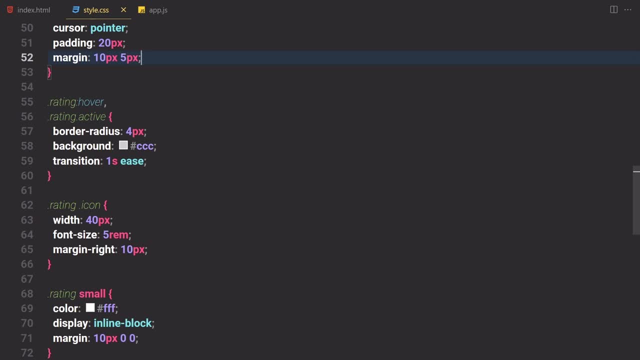 left and right will be five pixel and left and right will be five pixel and once you hover over to it and if our, once you hover over to it and if our, once you hover over to it and if our rating is active. so you want to provide. 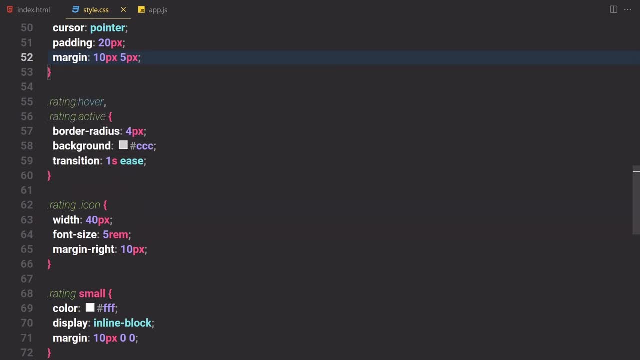 rating is active, so you want to provide. rating is active, so you want to provide a border radius of four pixel and a border radius of four pixel and a border radius of four pixel and background color to be that ccc and background color to be that ccc. and 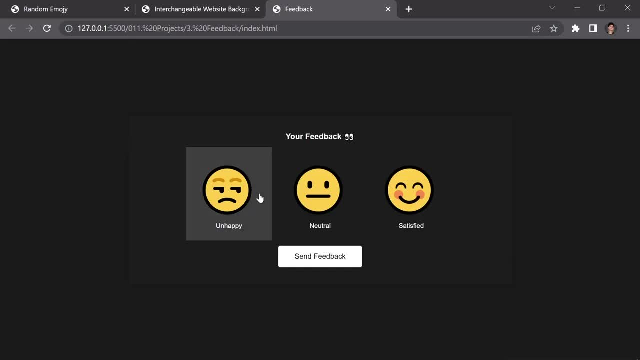 background color to be that ccc and transition will be taking one second. transition will be taking one second. transition will be taking one second ease, so if you just hover over it and if ease, so if you just hover over it and if ease, so if you just hover over it and if you click on it, so like one when it's. you click on it, so like one when it's. you click on it so like one when it's become active. we are going to be become active. we are going to be become active. we are going to be providing the active functionality once, providing the active functionality once. 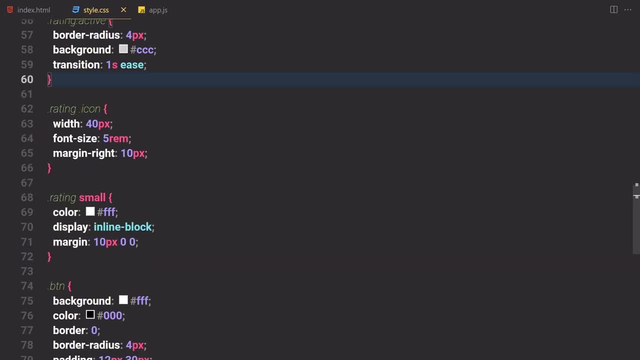 providing the active functionality once we jump into our javascript. but i just we jump into our javascript, but i just we jump into our javascript, but i just kind of want to tell you that kind of want to tell you that kind of want to tell you that. and then we have a rating icon which is 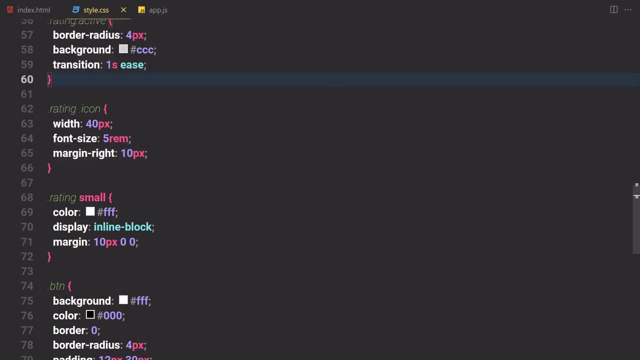 and then we have a rating icon which is: and then we have a rating icon which is that one, and we'll give him a width of that one, and we'll give him a width of that one, and we'll give him a width of like 40 pixel and the font size will be. 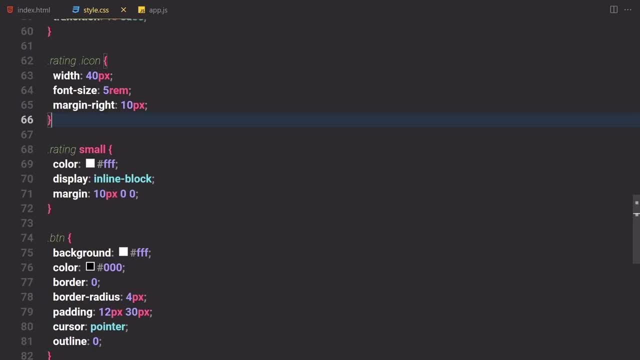 like 40 pixel and the font size will be like 40 pixel and the font size will be five frame and the margin for the right five frame and the margin for the right five frame and the margin for the right will be 10 pixel. and then we are just. 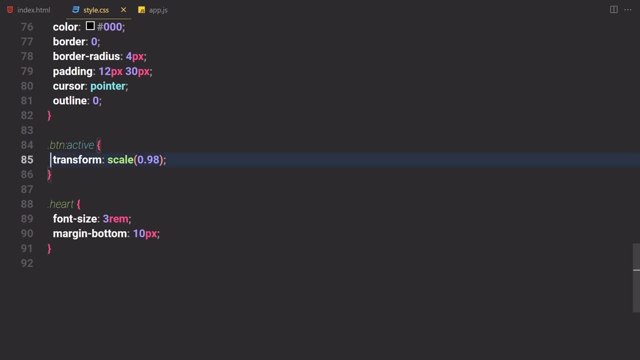 will be 10 pixel and then we are just will be 10 pixel and then we are just styling our small tag and our button, styling our small tag and our button, styling our small tag and our button, just a little bit, just a little bit, just a little bit, and if our button is active. so we want 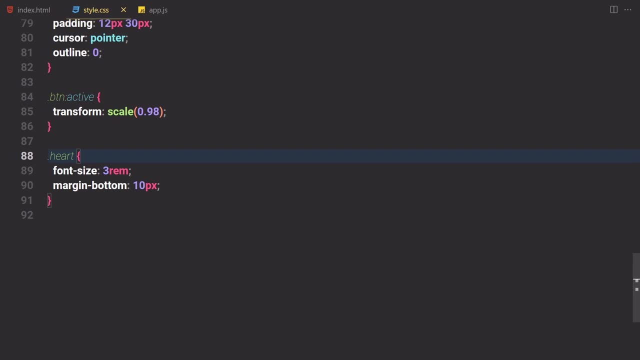 and if our button is active, so we want, and if our button is active so we want to use a transform of scale, we want to to use a transform of scale. we want to to use a transform of scale, we want to just scale it a bit. kind of lost my 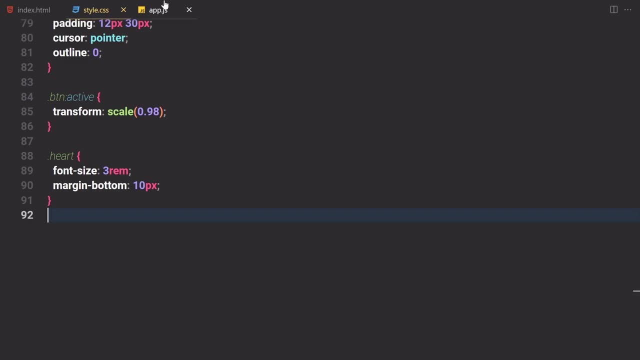 just scale it a bit kind of lost my just scale it a bit kind of lost my mind- okay. so we have a hard once we mind okay, so we have a hard once we mind okay, so we have a hard once we submit our feedback anyway. so now let's. 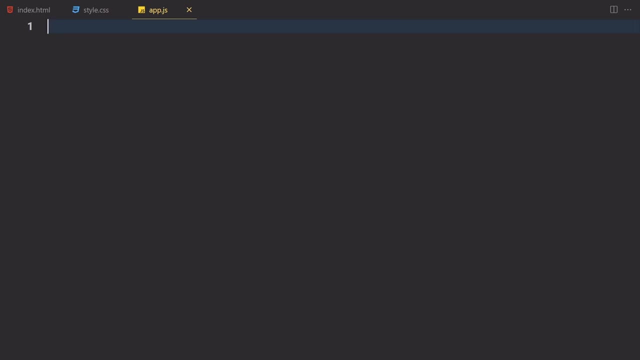 submit our feedback anyway. so now, let's submit our feedback anyway. so now let's just get into our javascript and write: just get into our javascript and write, just get into our javascript and write our code first of all, and then you will. our code first of all, and then you will. 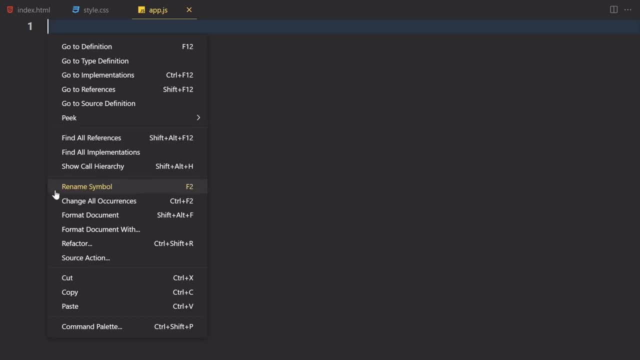 our code first of all, and then you will get to know, get to know, get to know how this project will look like. so first, how this project will look like. so first, how this project will look like. so, first of all, let me just zoom in a bit so you 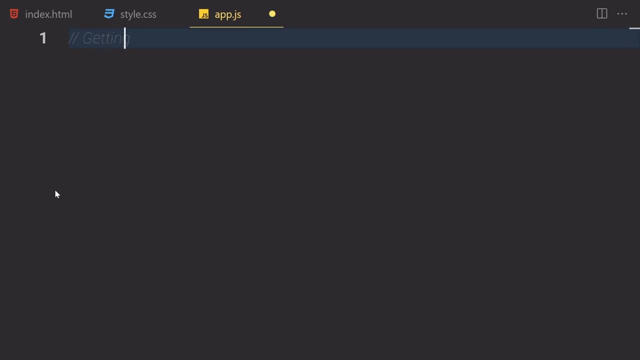 of all, let me just zoom in a bit. so you of all, let me just zoom in a bit so you guys can see everything a bit better. guys can see everything a bit better. guys can see everything a bit better. and getting and getting and getting elements from the dom. so you need a few. 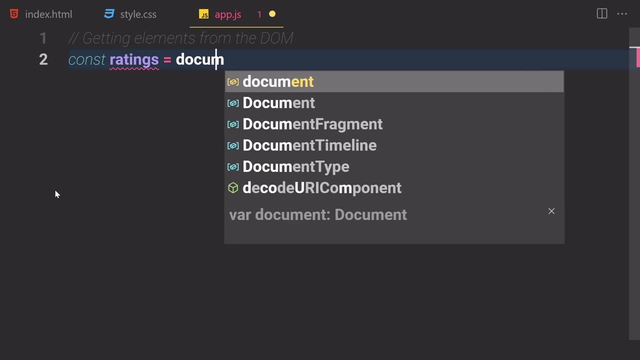 elements from the dom. so you need a few elements from the dom. so you need a few things. so we will just first of all need things. so we will just first of all need things. so we will just first of all need a ratings, and it will be now equals to: 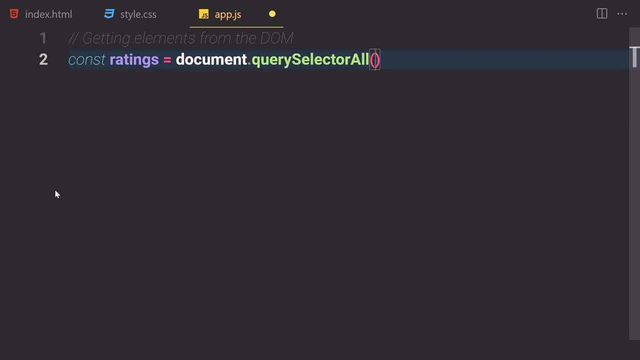 a ratings and it will be now equals to a ratings. and it will be now equals to document that query selector of all. and document that query selector of all. and document that query selector of all. and you want to get all of the ratings. okay, you want to get all of the ratings, okay. 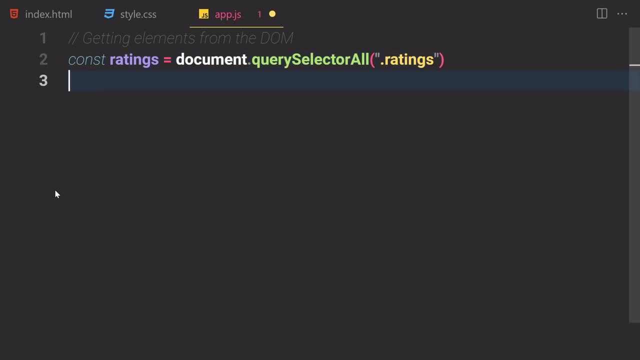 you want to get all of the ratings. okay, not a singular rate, but ratings like- not a singular rate, but ratings like- not a singular rate, but ratings like plural. and then we have a cons ratings plural, and then we have a cons ratings plural and then we have a cons ratings container. it will be now equals to: 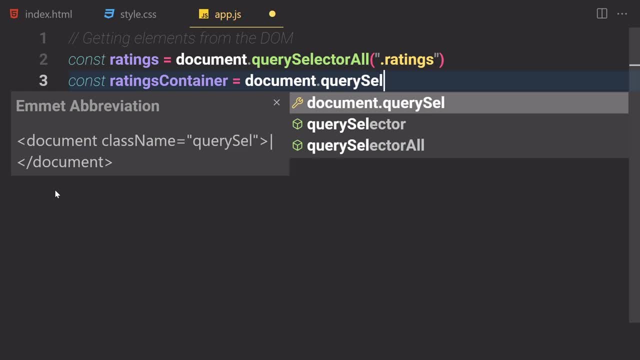 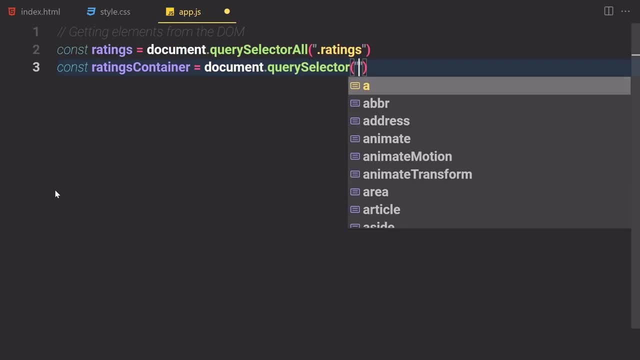 container. it will be now equals to container. it will be now equals to document. that queries document. that queries document. that queries query selector. uh query selector, uh query selector, uh query selector. just a singular query query selector. just a singular query query selector. just a singular query selector. and we are going to be selecting. 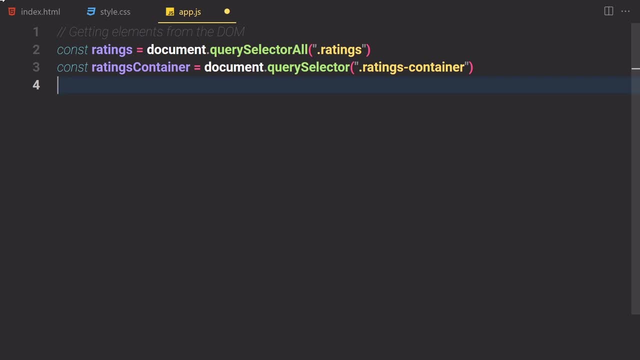 selector and we are going to be selecting selector and we are going to be selecting our ratings, our ratings, our ratings container, which is this ratings container, which is this ratings container, which is this ratings container right here, and then we have container right here, and then we have. 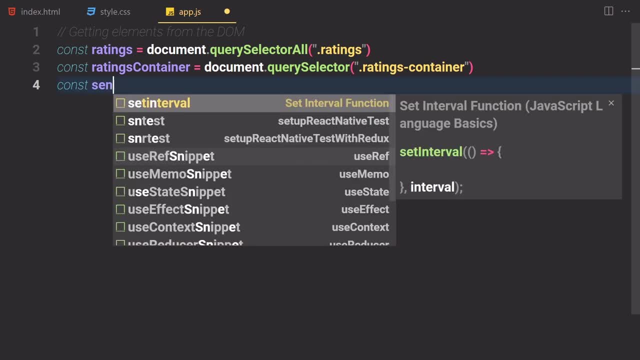 container right here. and then we have our send button. so consent, our send button. so consent our send button. so consent, consent bt and it will be now equals to consent bt. and it will be now equals to consent bt and it will be now equals to document dot query. selector query: 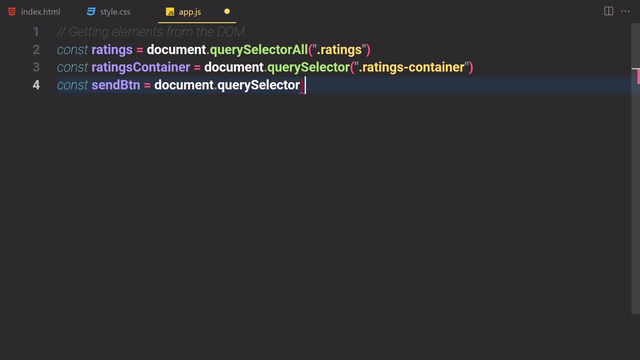 document: dot. query selector. query document- dot. query selector. query selector. come on, man selector. come on, man selector. come on, man, like so. and we are going to be using a like so, and we are going to be using a like so and we are going to be using a pound symbol of. 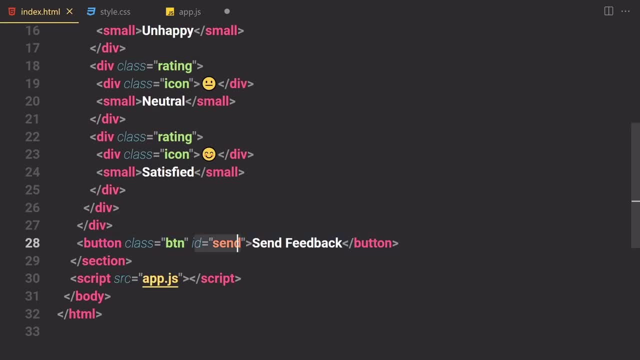 pound. symbol of pound. symbol of send, which is id. i guess, yeah, we are send, which is id. i guess, yeah, we are send, which is id. i guess, yeah, we are going to be selecting that one, going to be selecting that one, going to be selecting that one. and cons panel available now equals to: 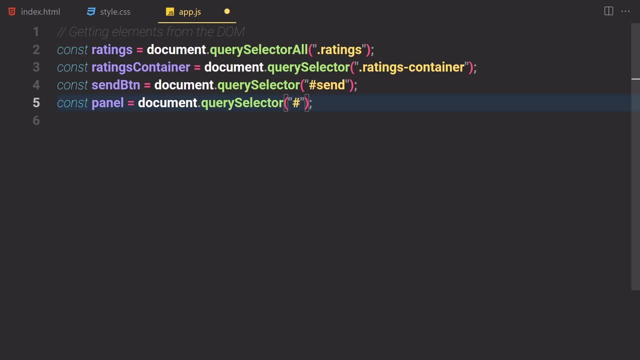 and cons panel available now. equals to: and cons panel available now. equals to: document dot query selector. document dot query selector. document dot query selector of panel like so. all right, so we are of panel like so. all right, so we are of panel. like so. all right, so we are totally done with. 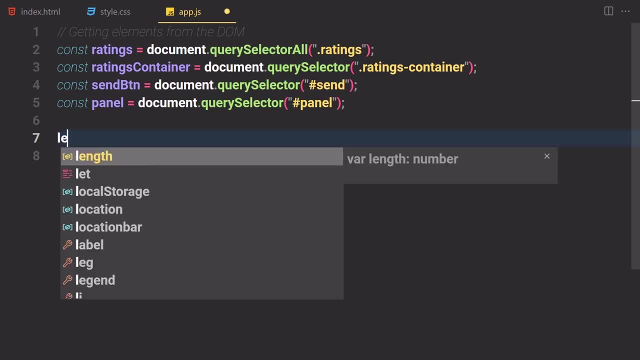 totally done with, totally done with or selection. so now the next thing, which? or selection. so now the next thing, which? or selection. so now the next thing which we have to do is that we have to select. we have to do is that we have to select. we have to do is that we have to select or selected. 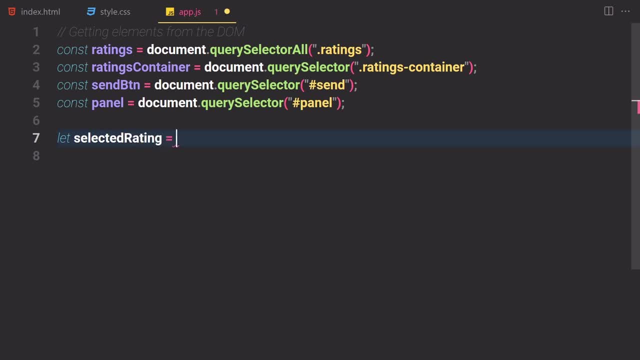 or selected or selected: uh right thing. this kind of this is uh right thing. this kind of this is uh right thing. this kind of this is going to be our default, going to be our default, going to be our default. selection like said this. selection like said this. 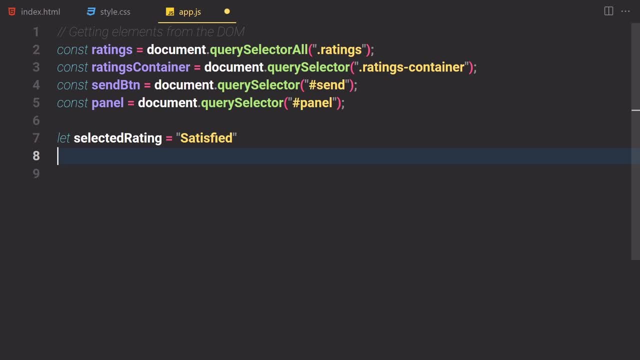 selection, like said this: fired okay, fired okay, fired, okay, zoom out, zoom out, zoom out. it will be now set to satisfied. and now, it will be now set to satisfied. and now, it will be now set to satisfied. and now, let's just attach. let's just attach. 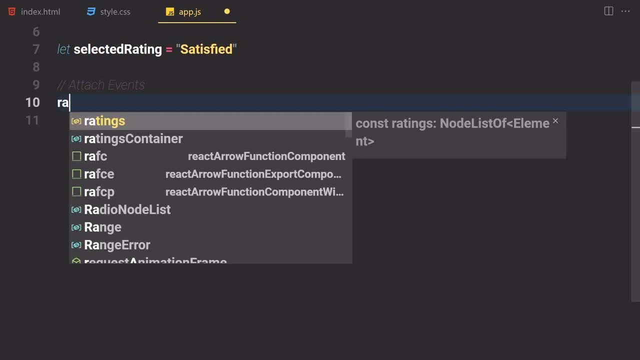 let's just attach events to events to events to that ratings container. so we have a that ratings container. so we have a that ratings container. so we have a ratings ratings container. so we have a ratings container. and if you just uh provide container and if you just uh provide, 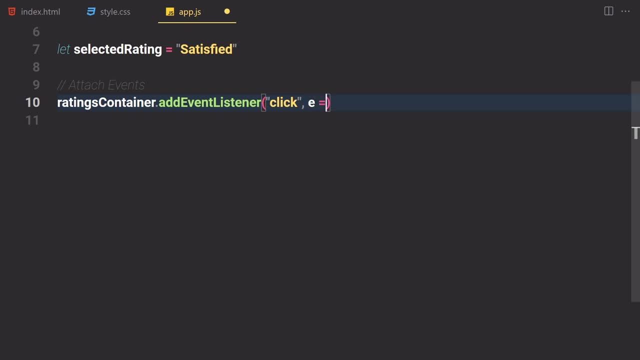 container and if you just uh provide add event listener to it, if you click on add event listener to it, if you click on add event listener to it, if you click on it, so then we want to get our event it, so then we want to get our event. 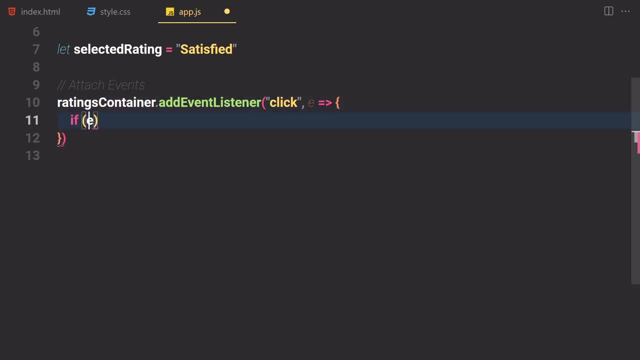 it. so then we want to get our event object, object object, and now let's just check if or e dot, and now let's just check if or e dot, and now let's just check if or e dot, target dot, target dot, target dot. parent node that class. 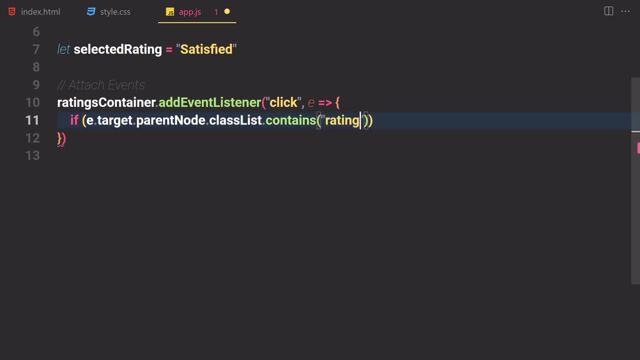 parent node that class. parent node, that class list. or contains uh ratings, so let's list. or contains uh ratings, so let's list. or contains uh ratings, so let's just check for that. if that contains, just check for that. if that contains, just check for that. if that contains ratings. so what do we have to do? we are. 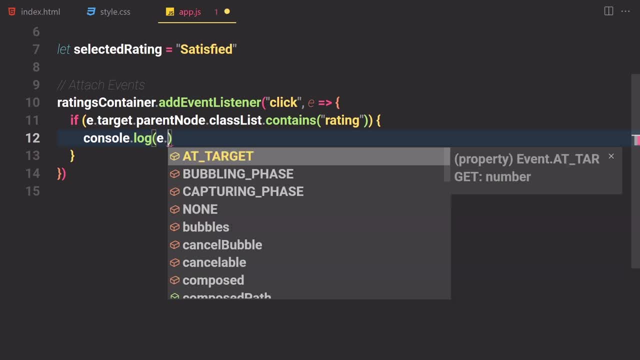 ratings. so what do we have to do? we are ratings, so what do we have to do? we are going to be first of all logging that. going to be first of all logging that, going to be first of all logging that to the console, like e dot target. 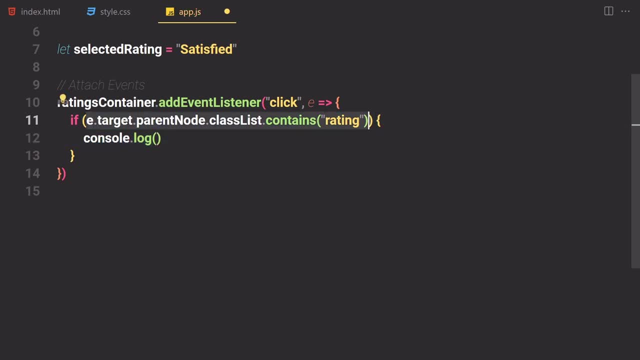 to the console like e dot target. to the console like e dot target. uh okay, let's just uh okay, let's just uh okay, let's just copy that from here so you guys can see. copy that from here, so you guys can see. copy that from here, so you guys can see everything. and i want to paste that. 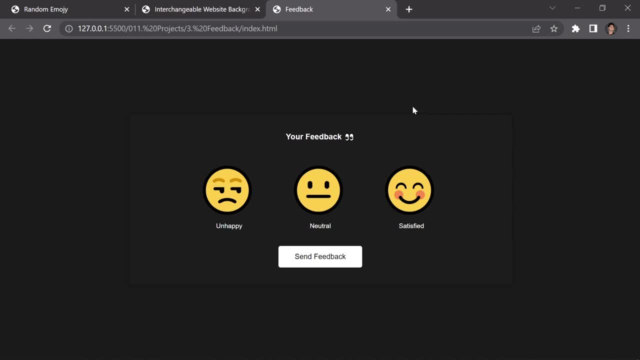 everything and i want to paste that everything, and i want to paste that right here, right here, right here, and now let's just save that and open. and now let's just save that and open. and now let's just save that and open: our developer tools, our developer tools. 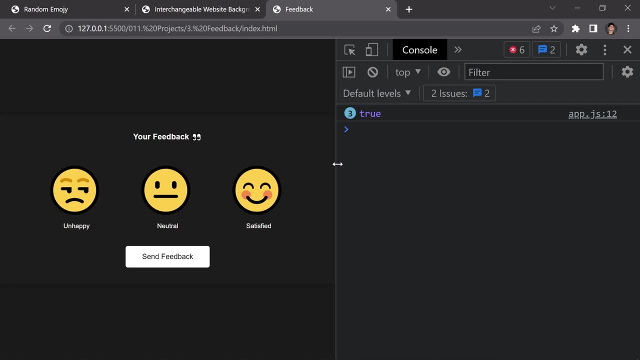 our developer tools. click on it. so true, true, true, everything. click on it. so true, true, true, everything. click on it. so true, true, true. everything is working. yeah is working, yeah is working. yeah, it is including that, so let's just. it is including that, so let's just. 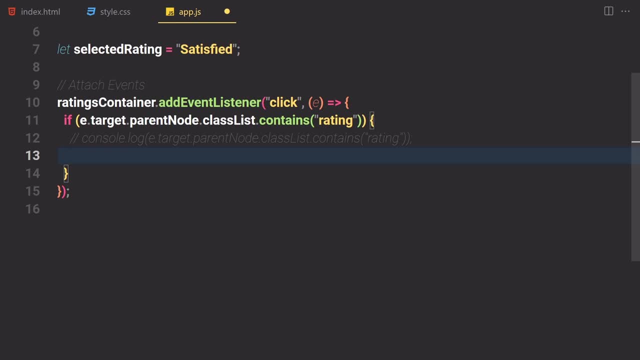 it is including that. so let's just comment this line out, comment this line out, comment this line out. and we are going to be passing over a and we are going to be passing over a and we are going to be passing over a function which we are going to be. 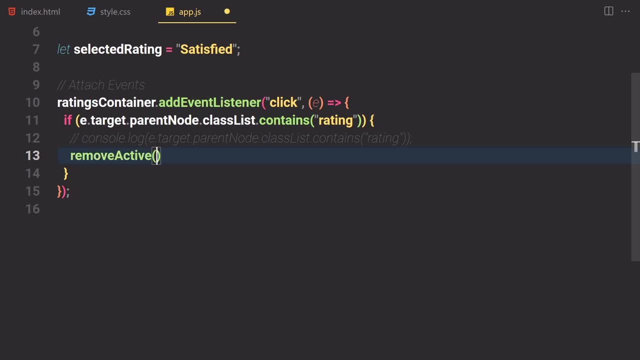 function which we are going to be, function which we are going to be creating just in a second, like remove. creating just in a second like remove. creating just in a second like remove- active. okay, so we are going to be active. okay, so we are going to be. 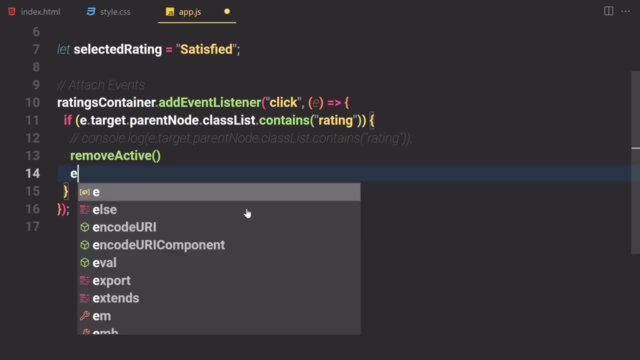 active. okay, so we are going to be passing our function and then we just passing our function, and then we just passing our function and then we just have to use like uh e dot target. have to use like uh e dot target. have to use like uh e dot target that parent. you know what i'm going to. 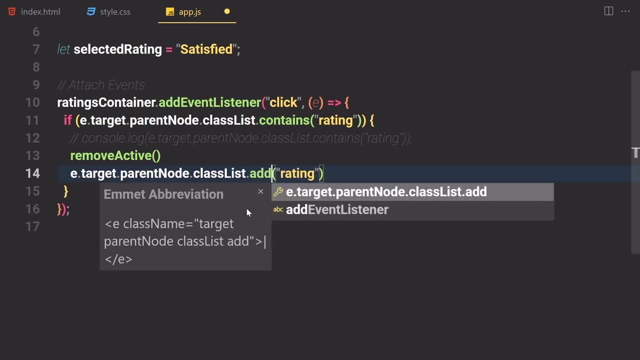 that parent. you know what i'm going to that parent. you know what i'm going to place that right here instead of that. place that right here instead of that. place that right here. instead of that contains, i'm going to just write add contains. i'm going to just write add. 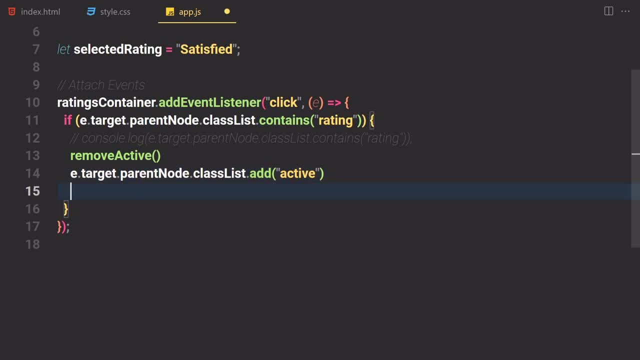 contains: i'm going to just write add and and. and. let's just write active. let's just write active. let's just write active instead. and then selected ratings which instead? and then selected ratings which instead, and then selected ratings which we've created, this variable right here. 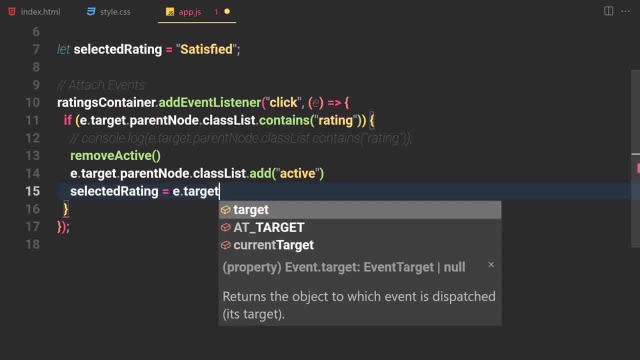 we've created this variable right here. we've created this variable right here, up above, and will be now equals to e dot up above and will be now equals to e dot up above and will be now equals to e dot target dot. next target dot. next target dot. next uh element. sibling element. 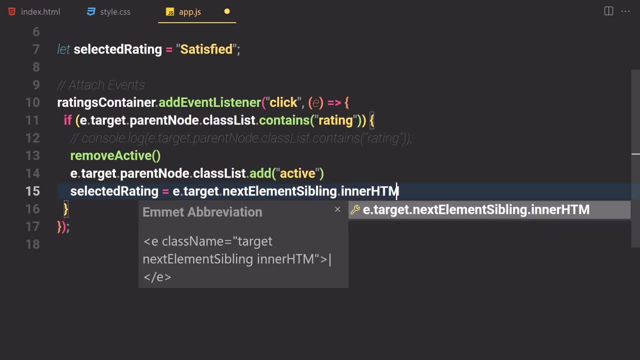 uh element sibling element. uh element sibling element: s i b l i n g, and then inner html: s i b l i n g, and then inner html: s i b l i n g and then inner html: like. so it will be now equals to there. like, so it will be now equals to there. 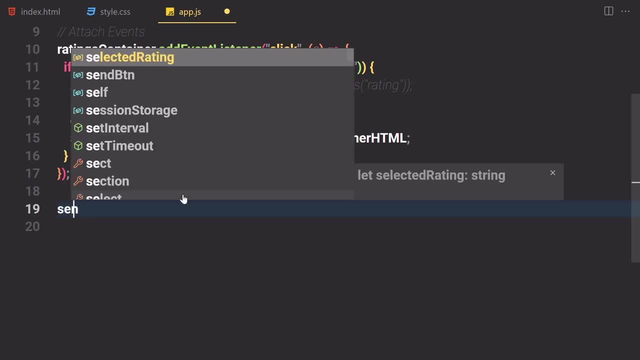 like, so it will be now equals to there. underneath all of that, let's just attach underneath all of that, let's just attach underneath all of that, let's just attach our event listener on the send button. so our event listener on the send button. so our event listener on the send button. so symbol on that: add event listener. and. 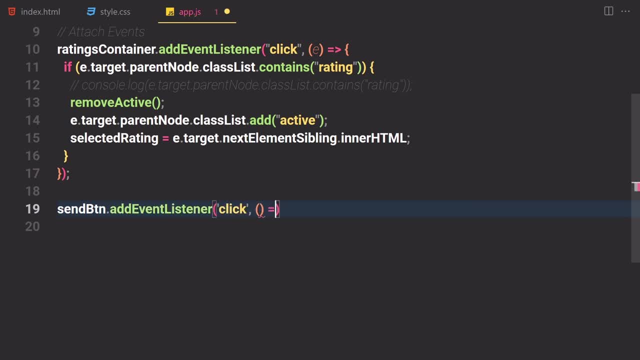 symbol on that- add event listener. and symbol on that- add event listener. and once we click on it. so what do we have once we click on it? so what do we have once we click on it? so what do we have to do? we have to just fire this function. 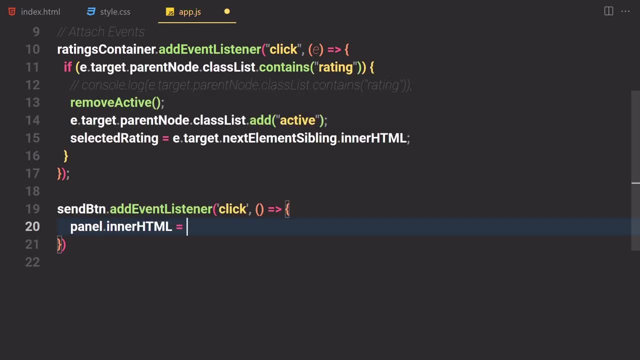 to do. we have to just fire this function to do. we have to just fire this function. so panel dot inner html will be now so. panel dot inner html will be now. so panel dot inner html will be now. equals to this template literal and we. equals to this template, literal and we. 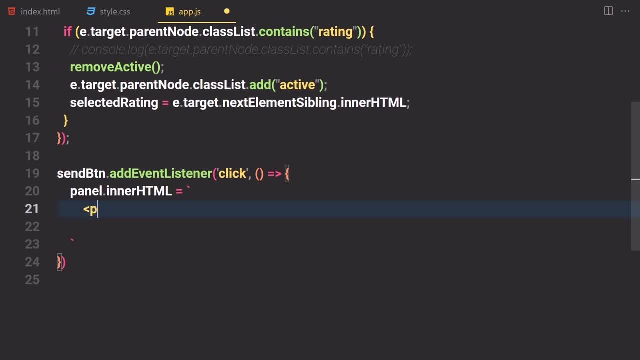 equals to this template, literal, and we are going to be placing our own html, so are going to be placing our own html, so are going to be placing our own html. so we have our paragraph with the class of, we have our paragraph with the class of, we have our paragraph with the class of heart and we already style this heart. 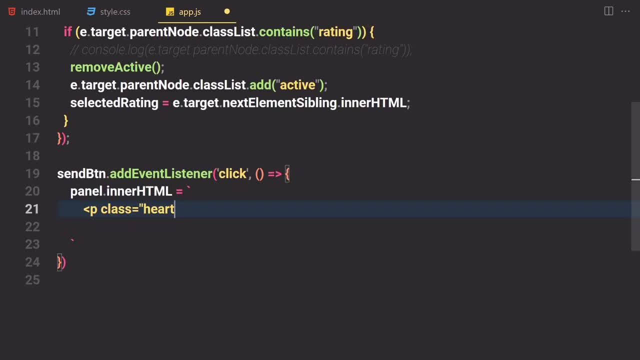 heart, and we already style this heart, heart, and we already style this heart right here, right here, right here, as i forgot just a second ago. and let's, as i forgot just a second ago, and let's, as i forgot just a second ago, and let's just put our 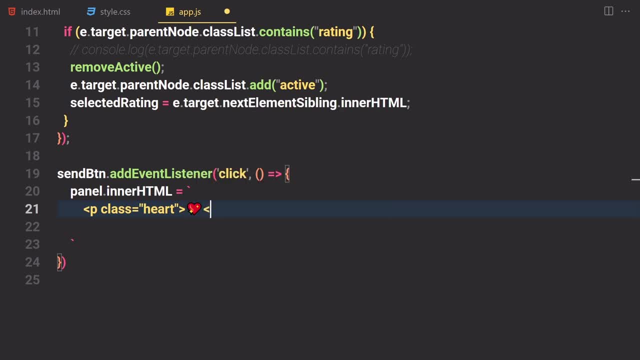 just put our, just put our heart in it. so we have a heart right here, heart in it, so we have a heart right here, heart in it. so we have a heart right here and let's just close that paragraph tag and let's just close that paragraph tag. 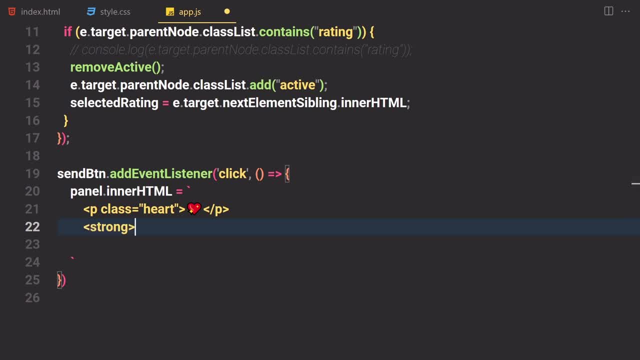 and let's just close that paragraph. tag right here, right here, right here: write a strong, write a strong, write a strong, and thank you and thank you, and thank you. close that strong right here, close that strong right here, close that strong right here, and then we have a br for breaking and. 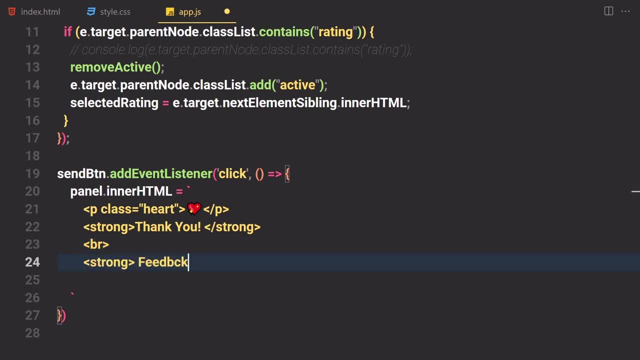 and then we have a br for breaking, and, and then we have a br for breaking, and finally we have another strong. finally we have another strong. finally we have another strong: feedback feedback feedback a, b, a, c, k, and then selected feedback rating, and and then selected feedback rating, and. 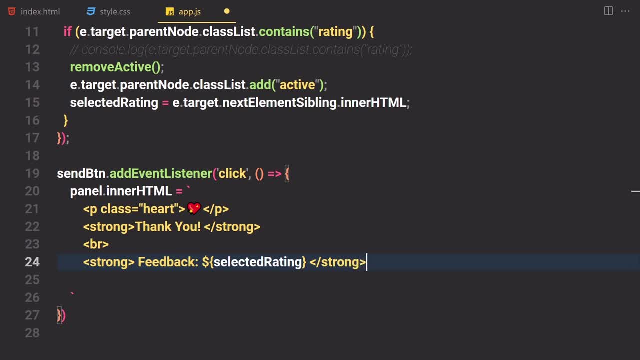 and then selected feedback rating. and now let's just scroll. now, let's just scroll. now, let's just scroll. crow, let's just close that strong tag as crow. let's just close that strong tag as crow. let's just close that strong tag as well. all right, so now we are totally. 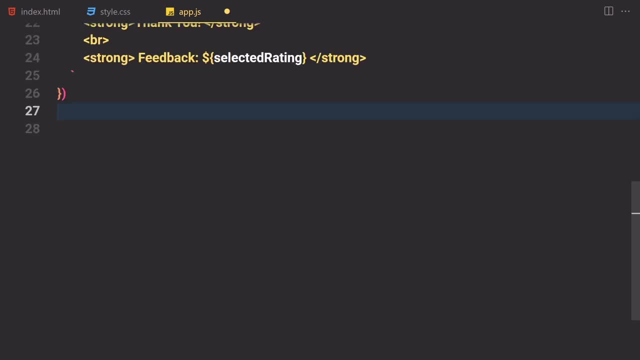 well, all right. so now we are totally well, all right. so now we are totally done with that. but now let's just create: done with that. but now let's just create. done with that. but now let's just create this remove active function, and we are this: remove active function, and we are. 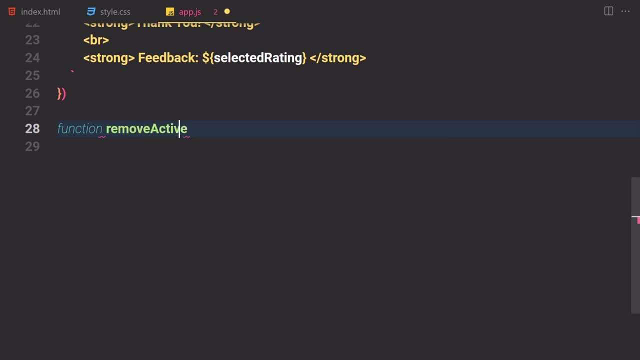 this remove active function and we are going to be totally done with this, going to be totally done with this, going to be totally done with this project as well. so remove active. okay. so project as well. so remove active. okay. so project as well. so remove active- okay. so it will not take any parameter or 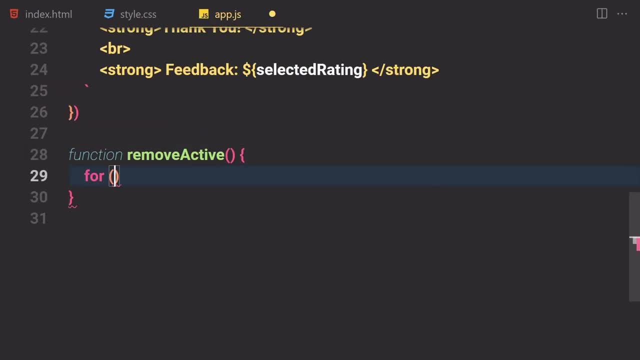 it will not take any parameter, or it will not take any parameter, or nothing, but inside that we are going to nothing. but inside that we are going to nothing, but inside that we are going to be iterating over through, like, let i be iterating over through, like, let i. 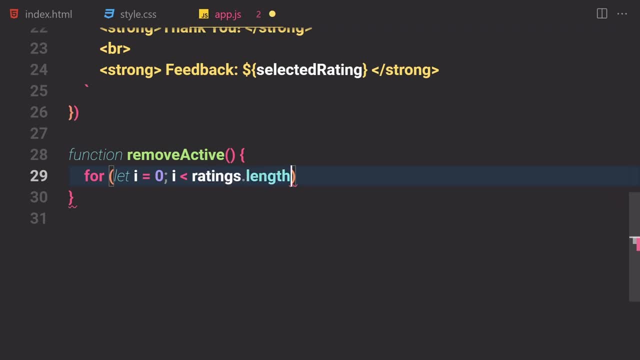 be iterating over through like let i: equals to zero. i is less than ratings. equals to zero. i is less than ratings. equals to zero. i is less than ratings dot length. so we are just iterating dot length. so we are just iterating dot length. so we are just iterating over through this. 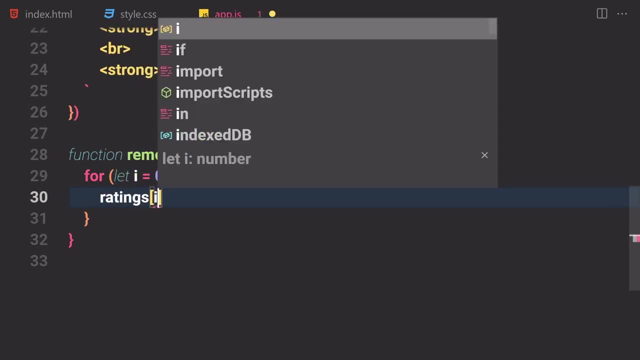 over through this, over through this: uh ratings length and then ratings dot uh ratings length and then ratings dot uh ratings length and then ratings dot uh index. uh index, uh index. dot class list or remove. so you want to. dot class list or remove, so you want to. 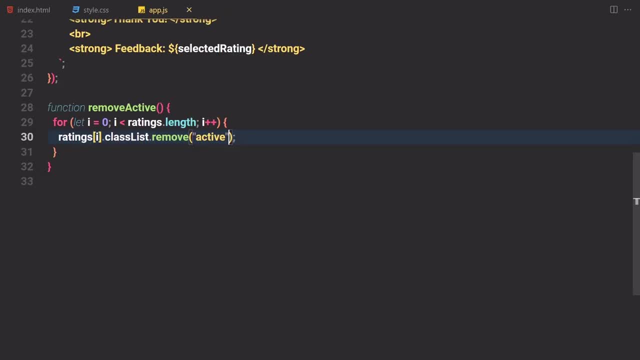 dot class list or remove. so you want to just remove that active from it, just remove that active from it. just remove that active from it. so now, if you save that, and let's just so, now if you save that, and let's just so now if you save that. and let's just zoom out a bit, and this is how. first of 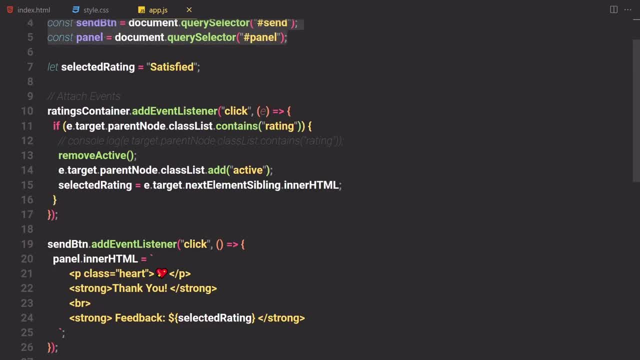 zoom out a bit and this is how, first of zoom out a bit and this is how: first of all, we have a selector, then we are just all. we have a selector, then we are just all we have a selector, then we are just attaching our first event: listener and 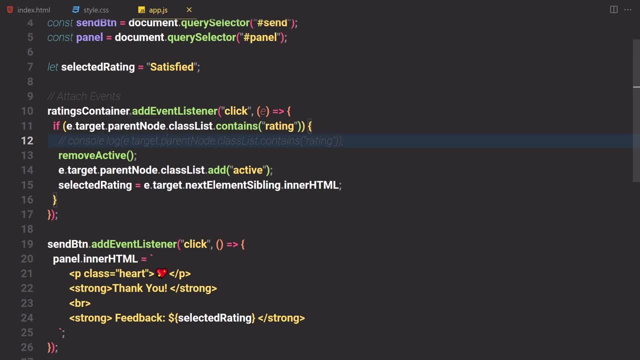 attaching our first event listener and attaching our first event listener and we are just checking if either target- we are just checking if either target, we are just checking if either target dot parent element class test contains dot parent element class test contains dot. parent element class test contains the class of ratings. so if that's true, 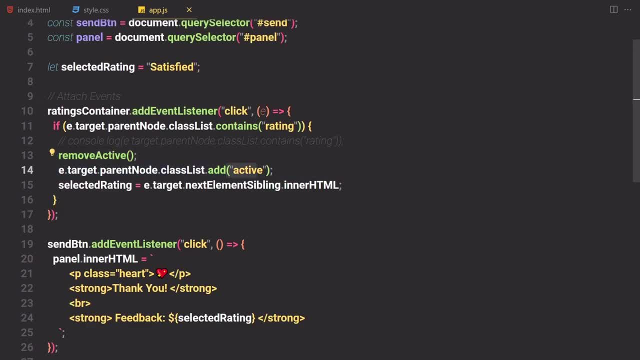 the class of ratings. so if that's true, the class of ratings. so if that's true, so you want to remove that egg and we so you want to remove that egg and we so you want to remove that egg and we want to add that active clause on it. and 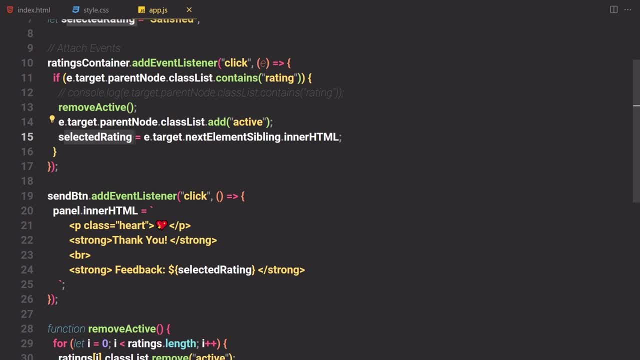 want to add that active clause on it. and want to add that active clause on it and we want to set the selected rating to. we want to set the selected rating to. we want to set the selected rating to this next element parent, this next element parent, this next element parent. so we want to select this selected. 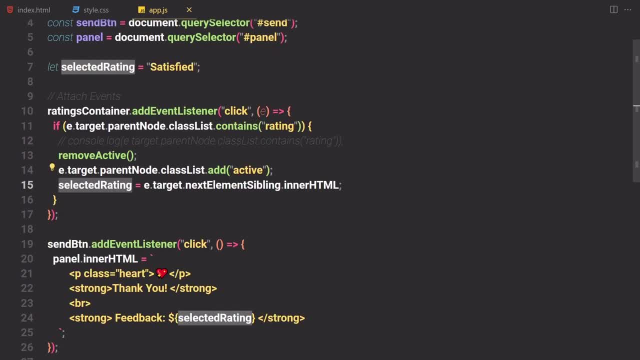 so we want to select this selected. so we want to select this selected. ratings ratings: ratings which we've created up above. so we which we've created up above, so we which we've created up above, so we want to select it there too, want to select it there too. 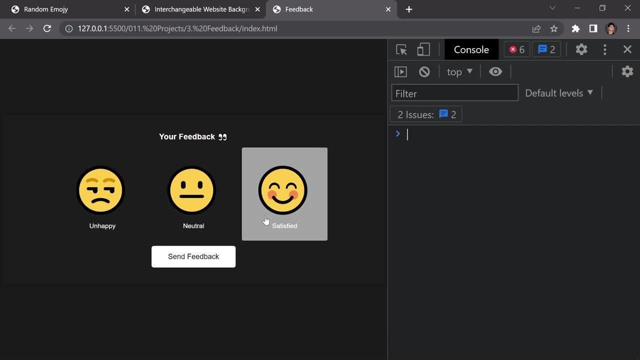 want to select it there too: uh selected rating, which is like either: uh selected rating, which is like either uh selected rating, which is like either neutral, unhappy or satisfied, and then if neutral, unhappy or satisfied, and then if neutral, unhappy or satisfied, and then if you just click on the select, 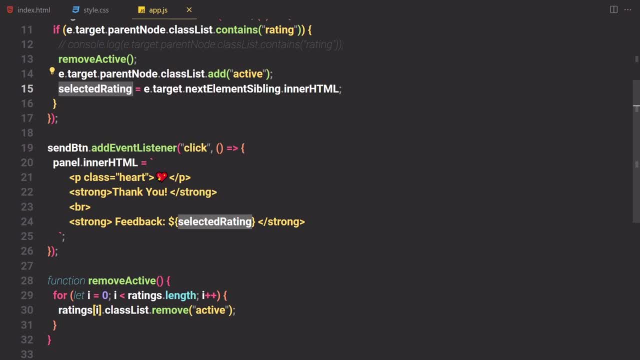 you just click on the select. you just click on the select send feedback. so we are just attaching send feedback. so we are just attaching send feedback. so we are just attaching even listen around there and we create even listen around there and we create even listen around there and we create our own panel and we just change the. 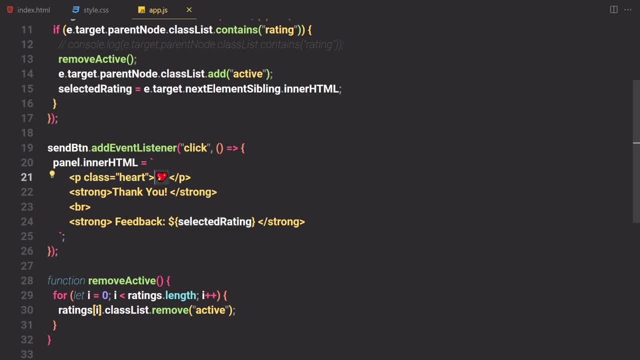 our own panel and we just change the our own panel and we just change the inner html to like first of all. they inner html to like first of all. they inner html to like first of all: they will get like hard, they will get like will get like hard, they will get like. 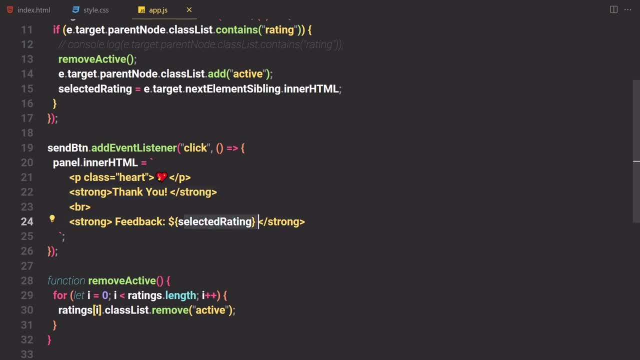 will get like hard. they will get like strong tag of thank you, then you have strong tag of thank you, then you have strong tag of thank you. then you have our feedback, so it will just show up our feedback. so it will just show up our feedback, so it will just show up that kind of a feedback for them, and we 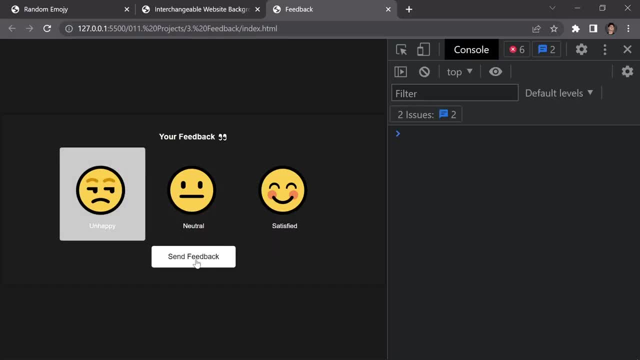 that kind of a feedback for them and we that kind of a feedback for them and we are iterating over through that now are iterating over through that, now are iterating over through that now. let's just check him out- unhappy send. let's just check him out- unhappy send. 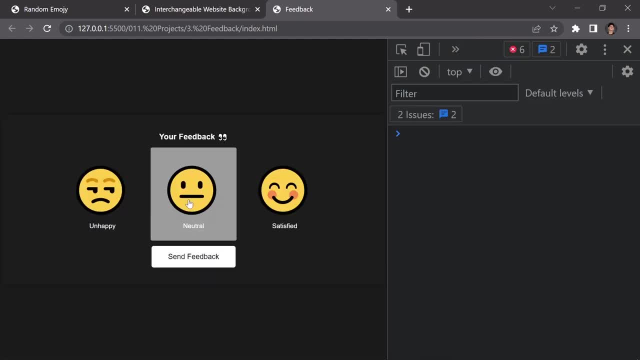 let's just check him out. unhappy- send feedback. thank you, feedback, unhappy and feedback. thank you, feedback, unhappy and feedback. thank you, feedback, unhappy. and now let's just click on neutral. send it now. let's just click on neutral. send it now. let's just click on neutral. send it one more time. thank you, feedback neutral. 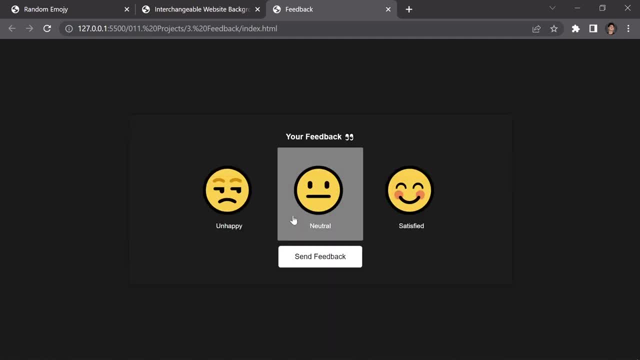 one more time. thank you, feedback neutral. one more time, thank you, feedback neutral. now, let's just click on the satisfied. now, let's just click on the satisfied. now, let's just click on the satisfied and satisfied. so everything is working and satisfied. so everything is working and satisfied. so everything is working the way we expect them to. 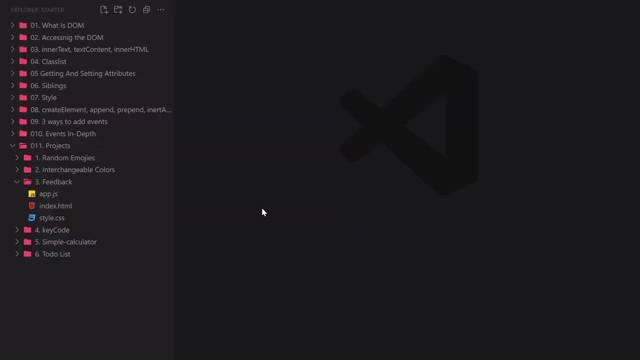 the way we expect them to, the way we expect them to work- all right. so now we are totally done: work all right. so now we are totally done- work all right. so now we are totally done with our third project as well. the next project is kind of a simple uh you. 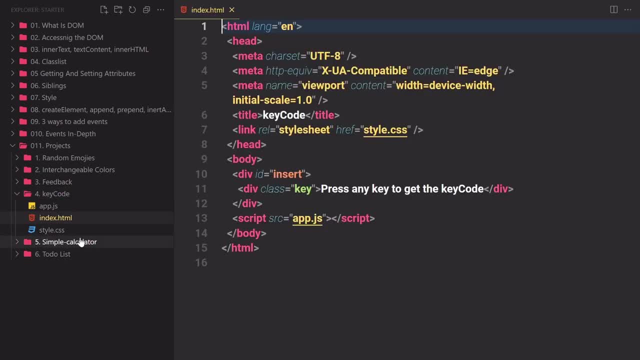 the next project is kind of a simple: uh, you. the next project is kind of a simple: uh, you already have everything which you need, already have everything which you need, already have everything which you need and we are going to be linked there, just. and we are going to be linked there, just. 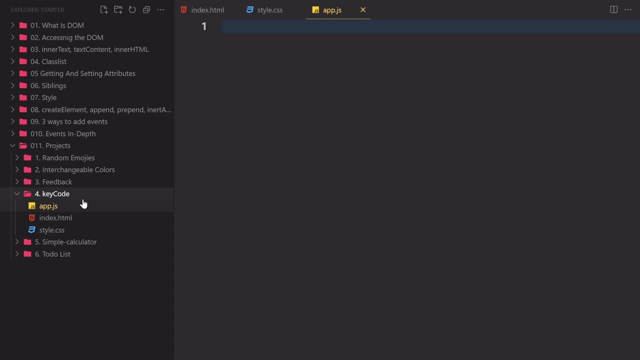 and we are going to be linked there just in a second, in a second, in a second. it's not that much hard. this one, the key, it's not that much hard. this one, the key, it's not that much hard. this one, the key code, is the most simple one i should. code is the most simple one. i should. code is the most simple one. i should have put that in the first one. i just have put that in the first one. i just have put that in the first one. i just want you to know that this one is simple. 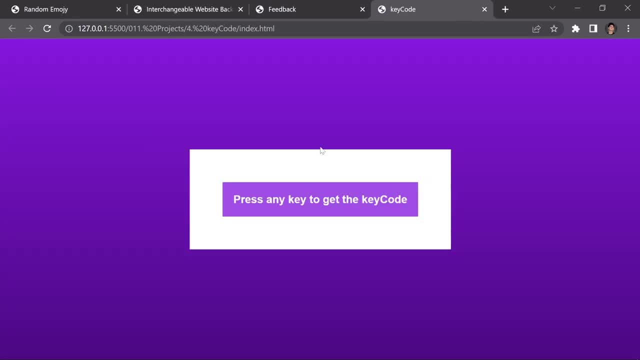 want you to know that this one is simple. want you to know that this one is simple one. that's what i meant. right click on one. that's what i meant. right click on one. that's what i meant. right click on it. open it with live server and if you 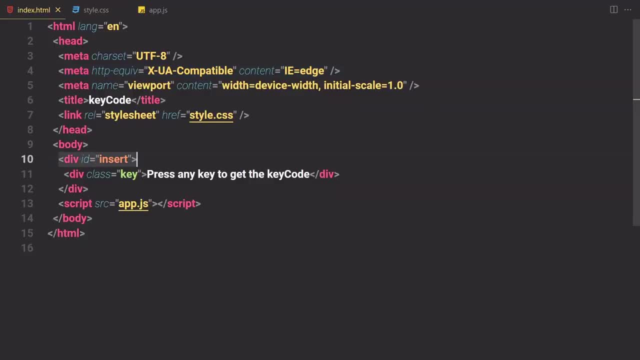 it, open it with live server. and if you it open it with live server. and if you press some key, nothing will happen. press some key, nothing will happen. press some key, nothing will happen. inside the body, we have first of all a. inside the body, we have first of all a. 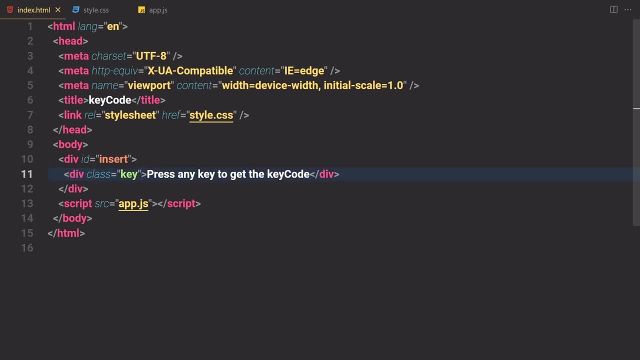 inside the body we have first of all a div with a class of insert, and then we div with a class of insert, and then we div with a class of insert, and then we have a div with a class of key and then have a div with a class of key and then 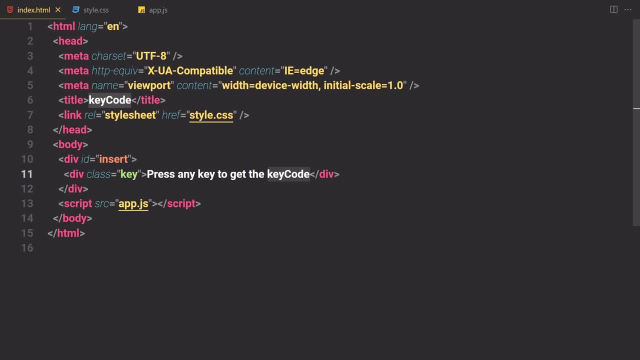 have a div with a class of key and then the level of press- any key to get the. the level of press any key to get the. the level of press any key to get the key code. so we are going to be just key code. so we are going to be just. 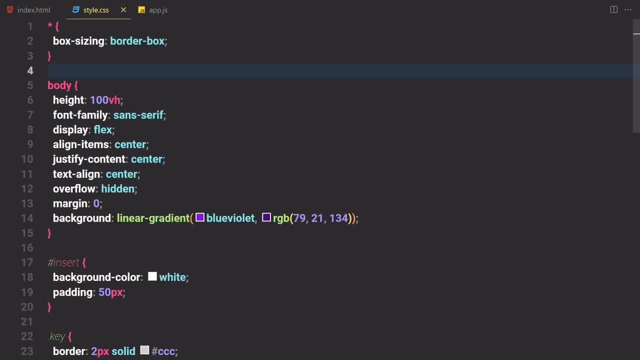 key code. so we are going to be just getting a key codes and all of that kind getting a key codes and all of that kind getting a key codes and all of that kind of a good stuff. we are just providing a of a good stuff. we are just providing a. 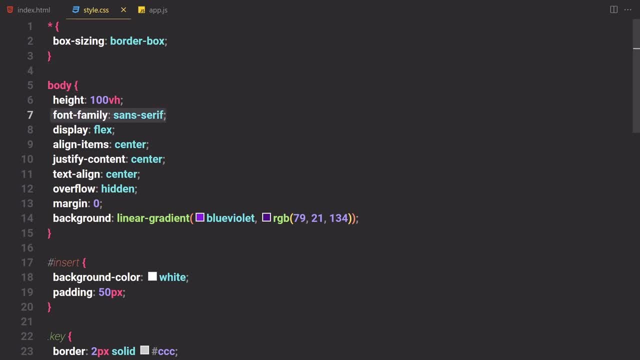 of a good stuff. we are just providing a research for it. we have a height of 100. research for it. we have a height of 100. research for it. we have a height of 100 pixel. we have sensor of and everything. pixel. we have sensor of and everything. 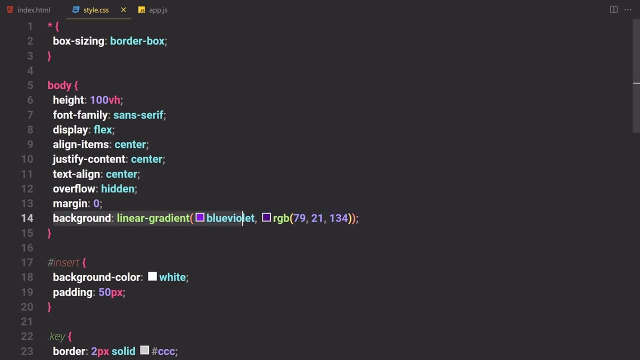 pixel. we have sensor of and everything the center, and then we have overflow is the center, and then we have overflow is the center, and then we have overflow is zero. we are just providing background of zero. we are just providing background of zero, we are just providing background of linear gradient to it and we are 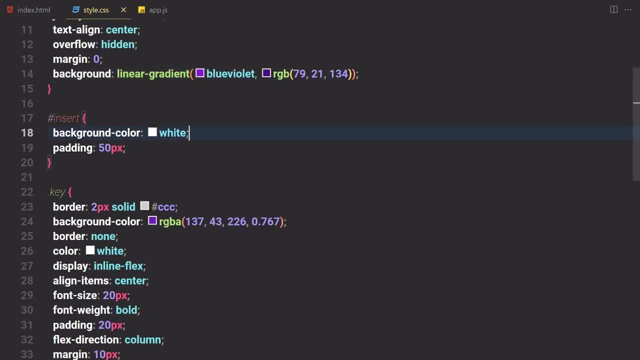 linear gradient to it and we are linear gradient to it and we are selecting that insert id right here and selecting that insert id right here, and selecting that insert id right here, and the background color will be white. like the background color will be white, like the background color will be white, like so this one and padding will be 50. 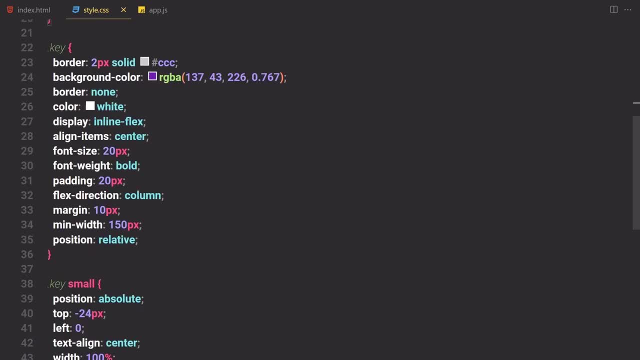 so this one and padding will be 50. so this one and padding will be 50 pixel. and we are now getting a key which pixel and we are now getting a key which pixel, and we are now getting a key which you will see just in a second, and we 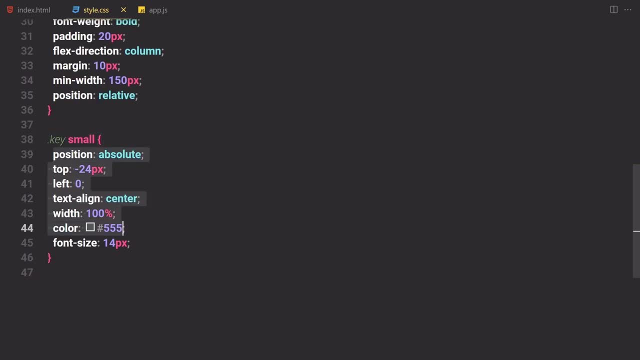 you will see just in a second, and we- you will see just in a second- and we are styling that key, are styling that key, are styling that key and also there's small text inside that and also there's small text inside that and also there's small text inside that key. so that's it for html, and that's it. 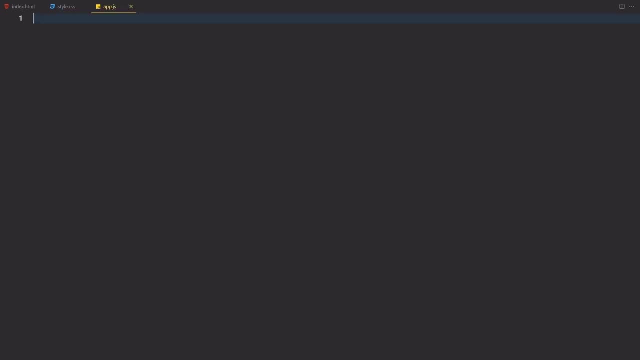 key. so that's it for html and that's it key. so that's it for html and that's it for a css. and, by the way, you can check for a css. and, by the way, you can check for a css. and, by the way, you can check out my 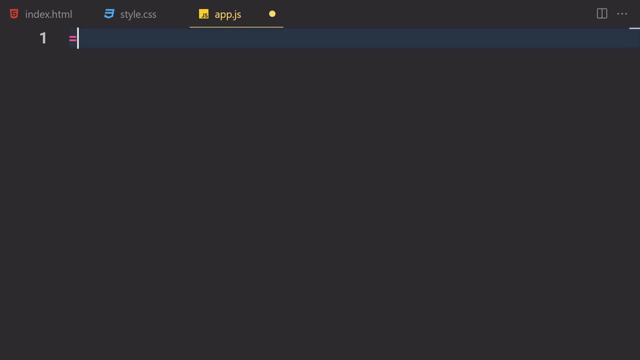 out my, out my hundred project for more details. if you hundred project for more details, if you hundred project for more details. if you want to, all right, so for javascript. want to all right, so for javascript. want to, all right, so for javascript. you will get or insert key, first of all. 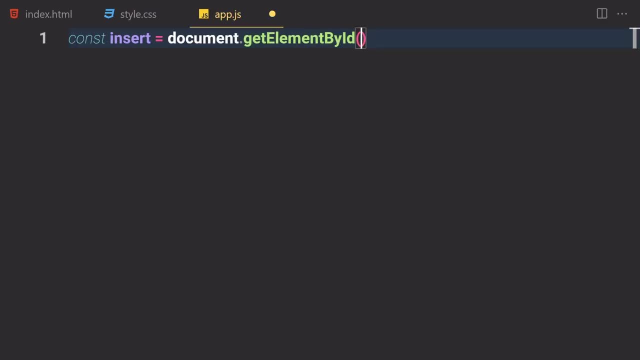 you will get or insert key first of all. you will get or insert key first of all. so documentget element by id. we didn't. so documentget element by id, we didn't. so documentget element by id. we didn't use that for a while. so now let's just 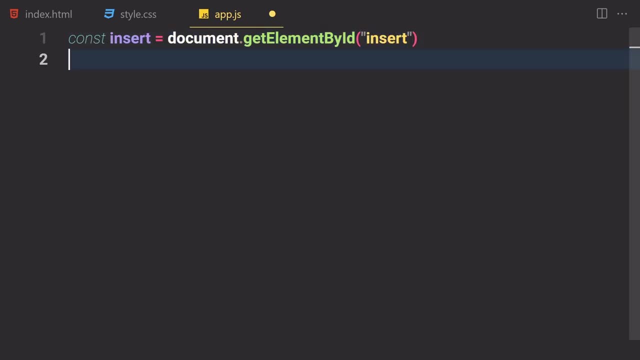 use that for a while. so now let's just use that for a while. so now let's just use: get element by id of insert. okay. so use get element by id of insert. okay. so use get element by id of insert. okay. so now let's just attach our event listener. 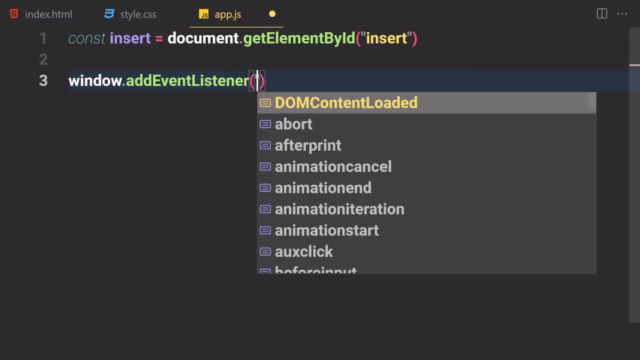 now let's just attach our event listener. now let's just attach our event listener on a window. so if we just on a window, so if we just on a window, so if we just attach event listener of on a window, if attach event listener of on a window, if 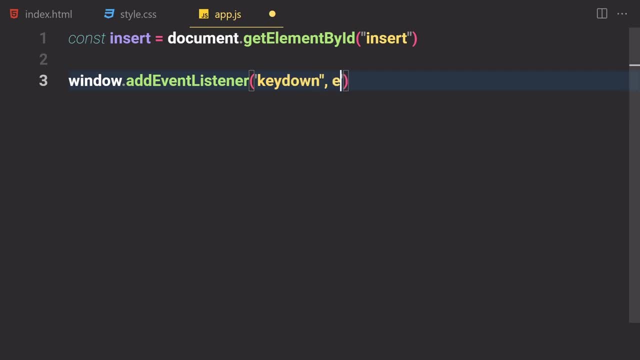 attach event listener of on a window. if we just hit key down so we want to get. we just hit key down so we want to get. we just hit key down so we want to get our event, our event, our event, like uh event and it or event will be. 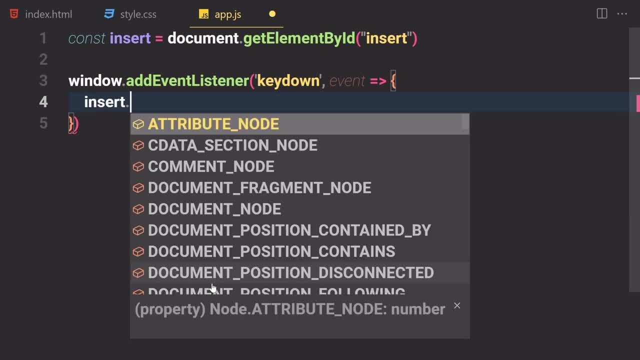 like uh event and it or event will be like uh event and it or event will be now equals to now equals to now equals to: uh insert dot inner html will be now uh. insert dot inner html will be now uh. insert dot inner html will be now equals to. 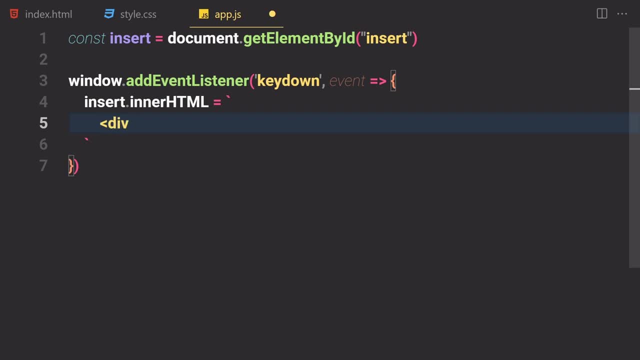 equals to equals to this back text right here. so we are going this back text right here, so we are going this back text right here. so we are going to be just rendering, or to be just rendering, or to be just rendering. or david the class of key. 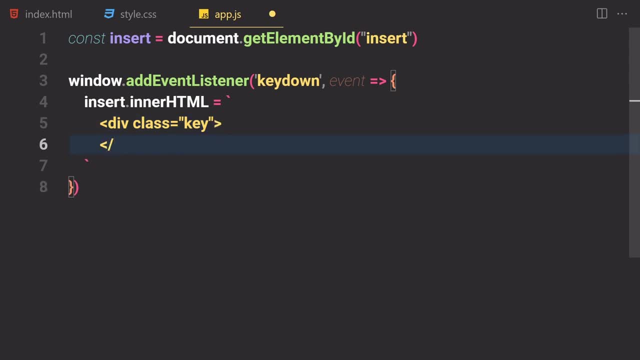 david the class of key. david the class of key, and let's just close that real quick. so, and let's just close that real quick. so, and let's just close that real quick. so, hmm, let's just close that. hmm, let's just close that. hmm, let's just close that. now, let's just render our data inside. 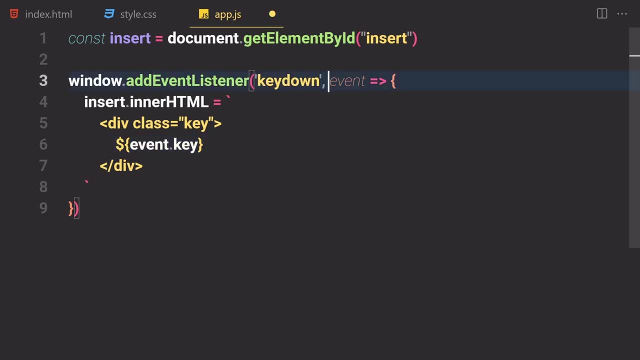 now let's just render our data inside. now, let's just render our data inside there like event there, like event there, like event dot key. so we are getting that event and dot key. so we are getting that event and dot key. so we are getting that event and we are just getting a key which you 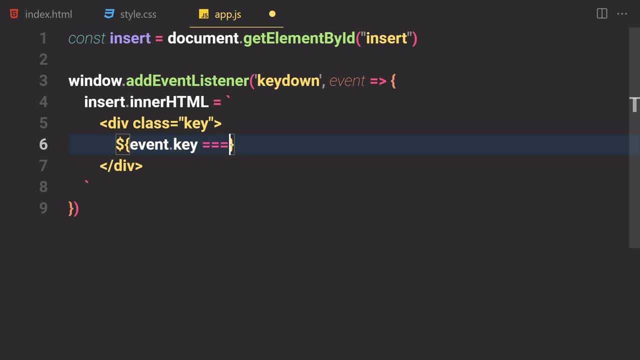 we are just getting a key which you. we are just getting a key which you learned just in a second ago. learned just in a second ago, learned just in a second ago in a keyboard event. so if that's equals in a keyboard event, so if that's equals. 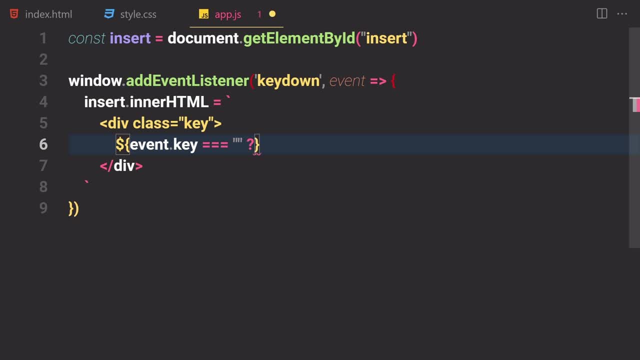 in a keyboard event. so if that's equals to empty strings, so to empty strings. so if that's equals, we are just using ordinary operator, we are just using ordinary operator. we are just using ordinary operator, right here, if that's equal to. right here, if that's equal to. 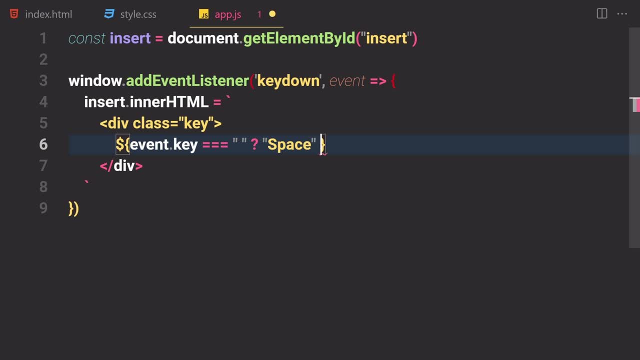 right here. if that's equal to space. if we just write a space, so we space. if we just write a space, so we space. if we just write a space, so we want to just get a space, want to just get a space, want to just get a space. and if that's not equal to space, we. 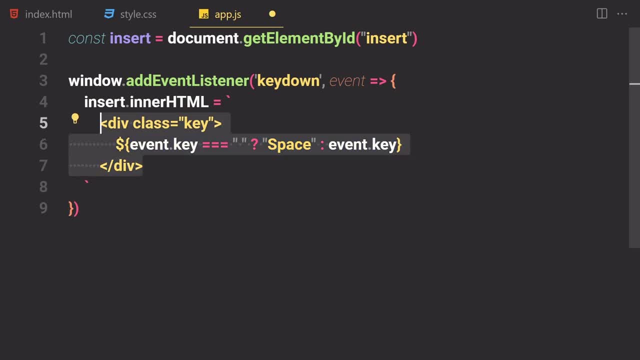 and if that's not equal to space, we, and if that's not equal to space, we want to just get. or a key, want to just get, or a key, want to just get, or a key. let's just duplicate that, or you know. let's just duplicate that, or you know. 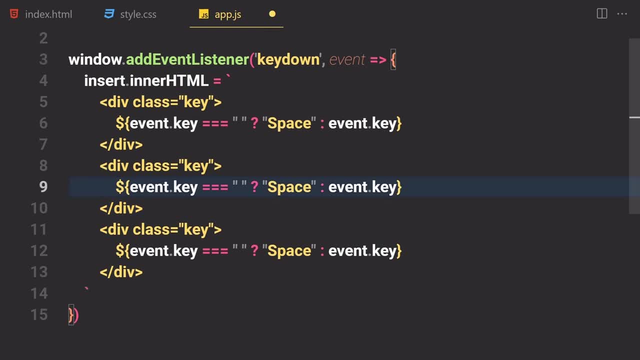 let's just duplicate that. or you know what, what, what? yeah, i'm going to just duplicate that. yeah, i'm going to just duplicate that. yeah, i'm going to just duplicate that two times, so the id will be key two times, so the id will be key. 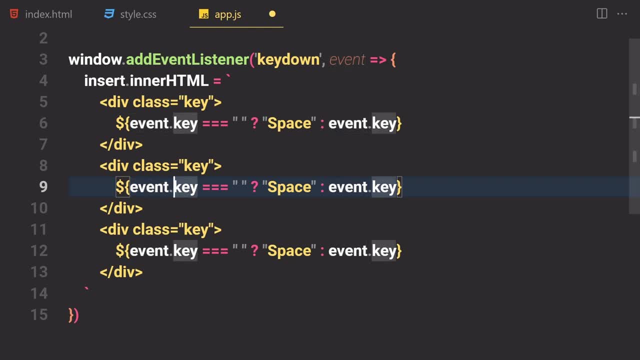 two times. so the id will be key or the class will be key, and then we or the class will be key, and then we or the class will be key, and then we have event dot. let's just remove the. have event dot. let's just remove the. 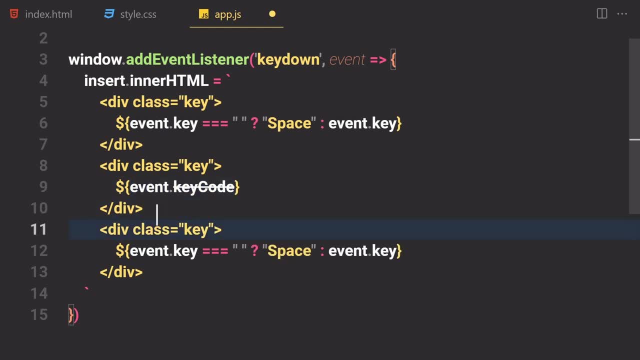 have event dot. let's just remove the other stuff. it will be now set to key other stuff. it will be now set to key other stuff. it will be now set to key code and this one will be now set to code. and this one will be now set to. 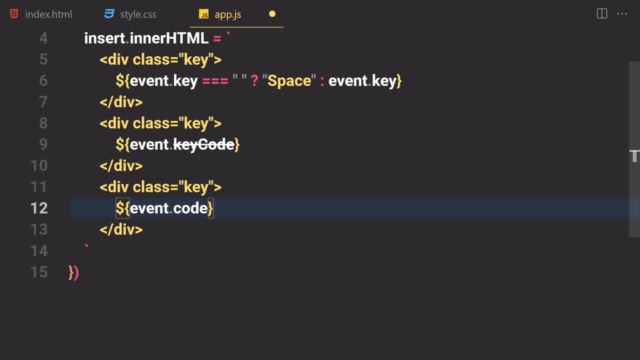 code, and this one will be now set to just a code, simple code. i'm going to just a code, simple code. i'm going to just a code, simple code. i'm going to write a code in here. write a code in here, write a code in here, and i'm going to also put a small tag. 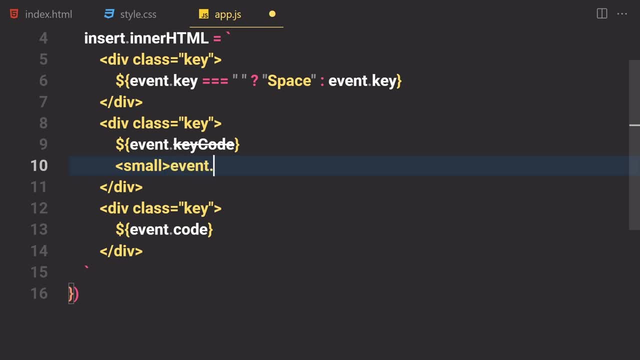 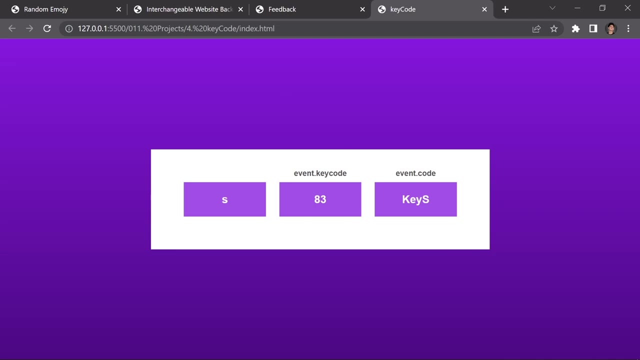 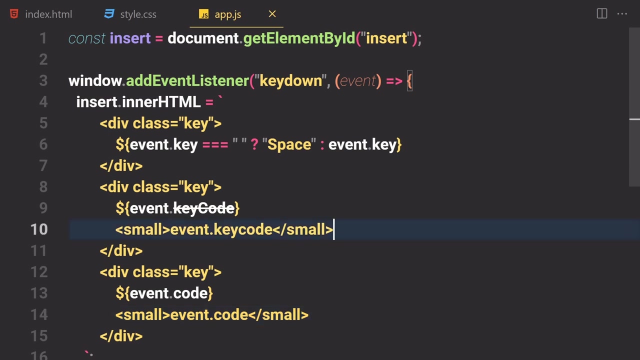 in here as well, so small. and then event dot key code. copy that and pass it right here. and event dot code would be fine. and now if you save that, and now if i hit uh, any key and now here you can see it- unlock uses the key name okay, so we are missing something right here, so copy that one. 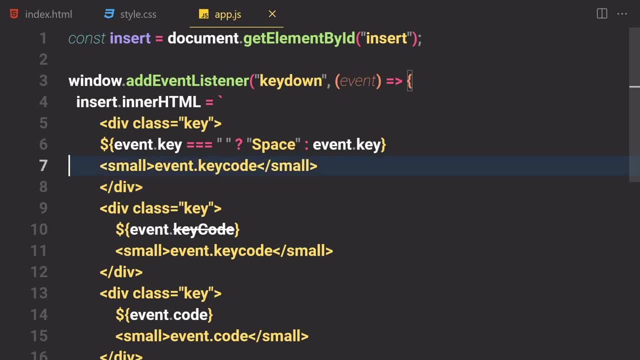 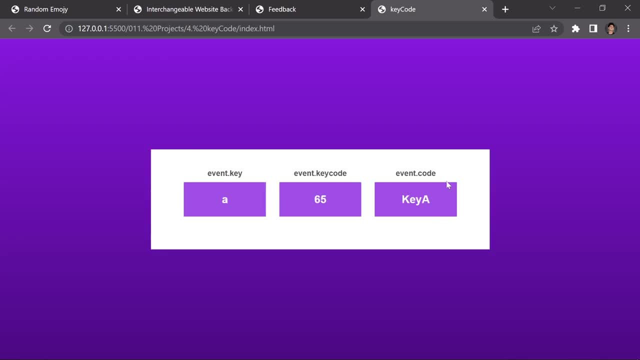 and i want to pass it underneath that one and this should be just a key. so if you save that, and now, if i just hit, a certain log uses the key of a, the key code of 65, and the code will be just key a. if i hit b, it will not use this b and 66 and the key code will be b, c, d, e, f, g and everything is. 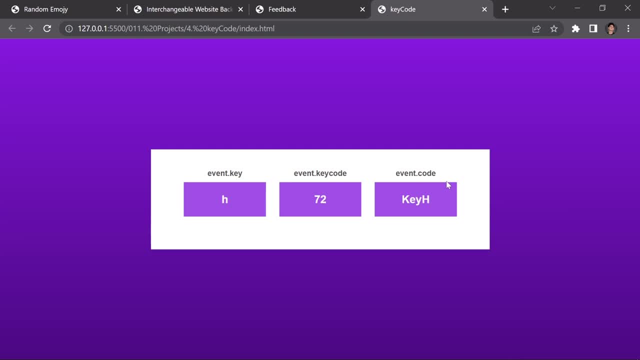 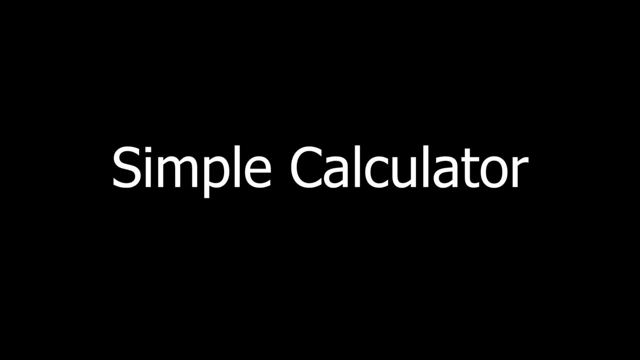 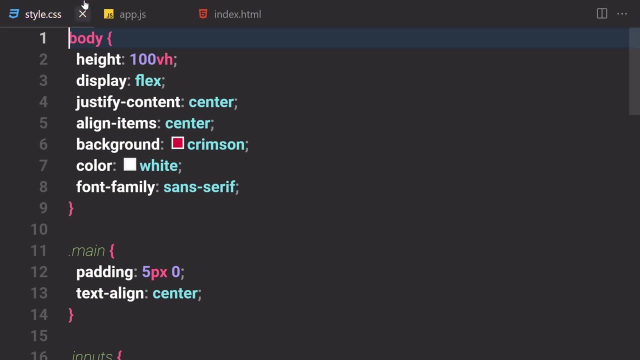 working the way we expect them to work. okay, so we have just interactive function or interactive project right here, so we have not already done with this project as well. so now the next project which we are going to be building is a simple calculator. so you already have a styling and you already have your uh html code and i have already built. 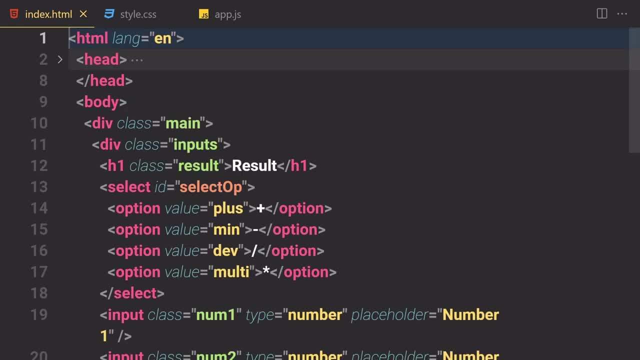 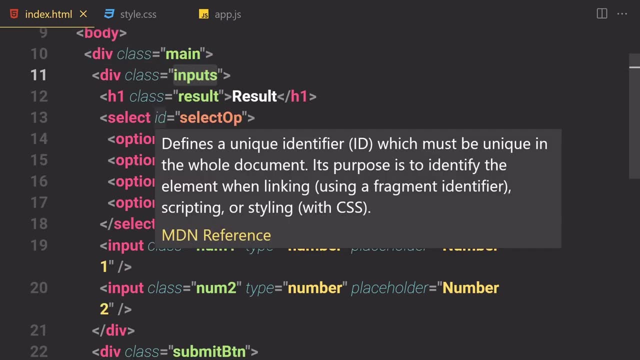 this project in my hundred projects as well. so if you want to check that out, first of all we have our div with a class of main, then we have a div with a class of input, so we are going to be storing different kind of inputs in there, and then we have our h1 with the class of results. 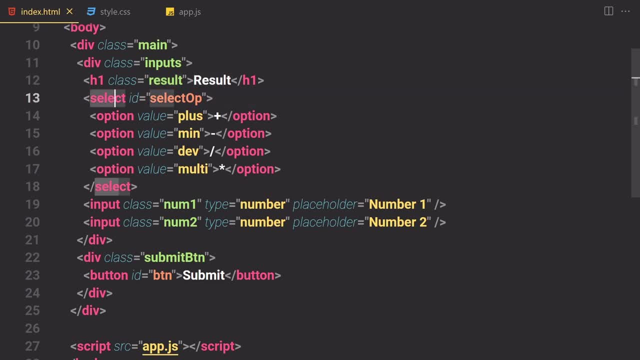 so we are going to be printing our results in there and then we have our select options. so we have different kind of options right here. so plus, minus, division, multiplication. then we have two inputs with the class of number one and number two, and both of them will take that type of input. 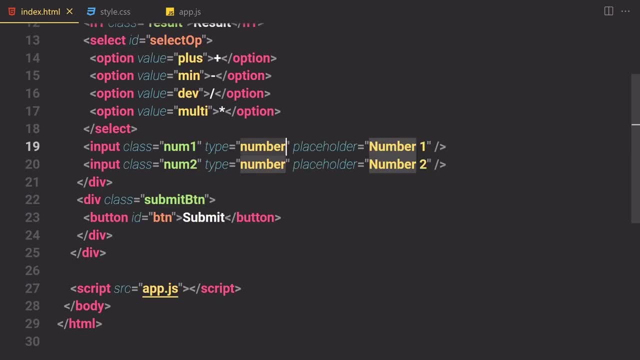 and placeholder will be number one and number two, and then we have a div with the class of submit button and then we just have one button with the id of ptn and the label of submit. submit in there and as a css, first of all we have a hundred pixel of height and we are just 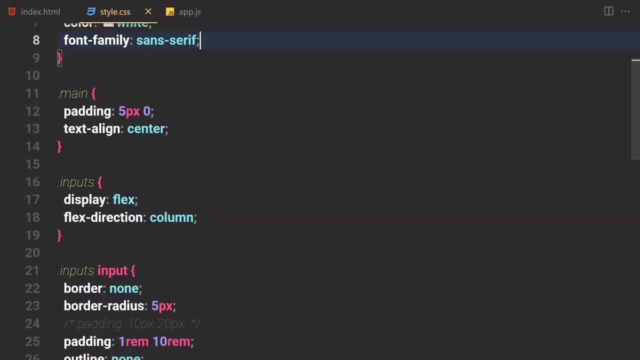 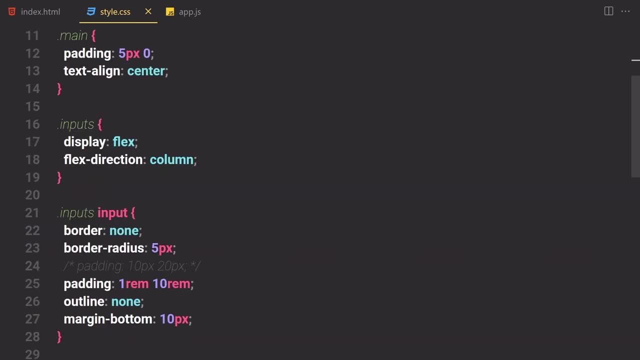 centering everything. background will be crimson, text will be white and font will be sans serif. we are just getting a 10: 5 pixel of padding for top and bottom, and left and right will be zero text and our alignment will be set to center. input will be flex. everything will be a flex. 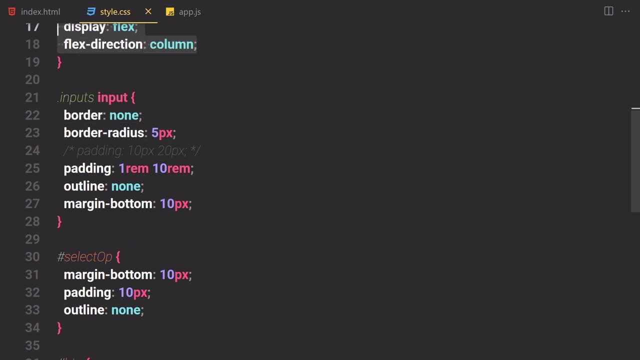 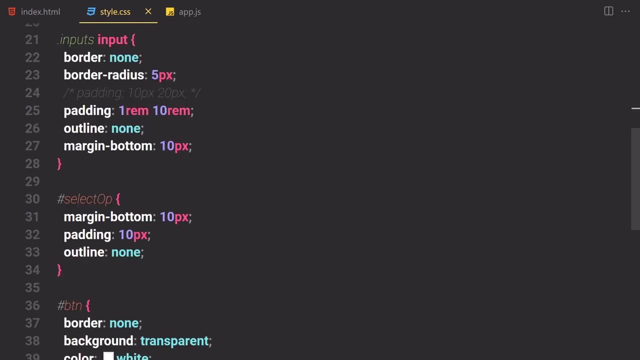 direction will be column. and then we have for input: border will be none, border radius will be five, padding will be- we just comment that out. padding will be one rim at the top and bottom and 10 ram for the left, right and outline will be none. margin will be. margin for bottom will be. 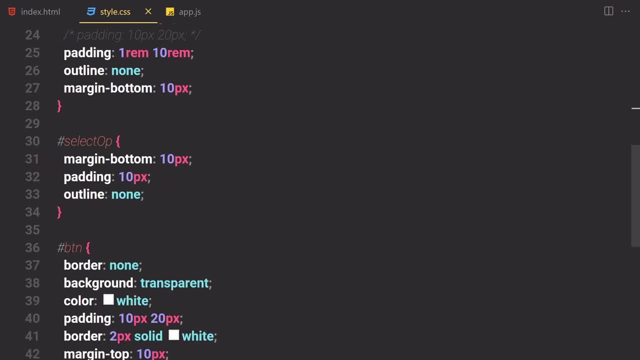 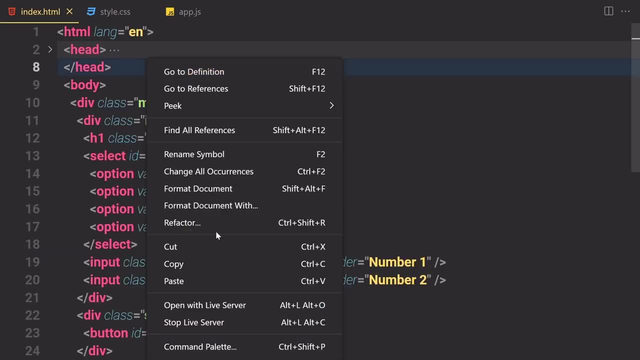 10 pixel for select option. we have margin bottom of 10 pixel and padding of 10 pixel and outline will be none, and we have a button, a little bit of styling for that button- right click on it and open it with the live server, and this is how everything looks like. okay, so now let's jump into our general 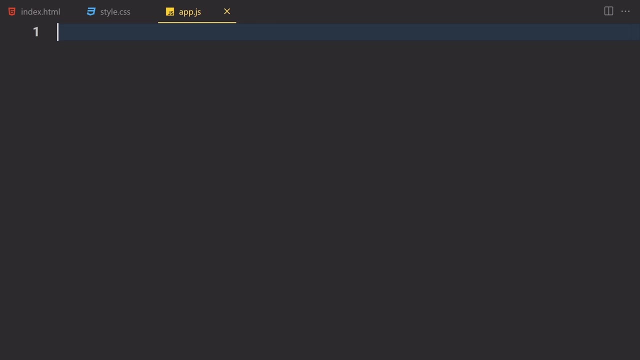 script and provide our interactivity to it. so first of all, let me just write my document documentget element by id, and i want to get my button first of all, and i'm going to just attach or event listener straight in. okay, and let's just fire this function. okay, let's just zoom out a bit. 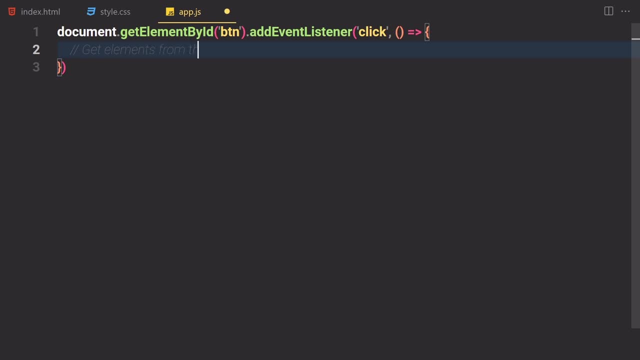 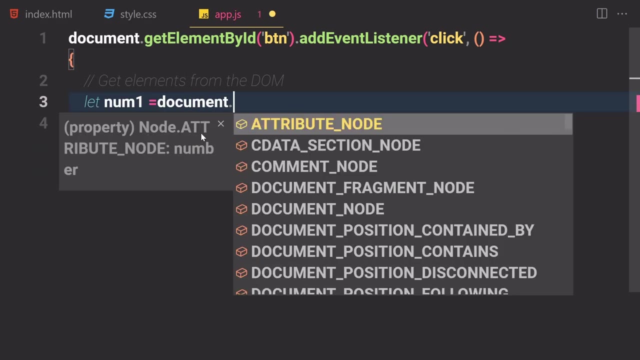 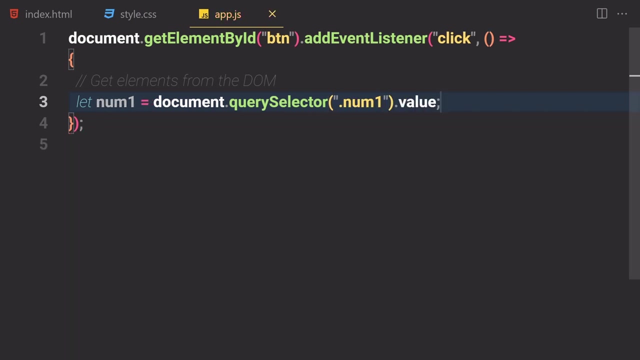 and first of all let's just get elements from the dom, zoom in a bit and let's just get our elements so like: let num1 will be now equals to document dot query, selector of dot or period number one. and now let's just duplicate there and change this one to number two and this one will be also. 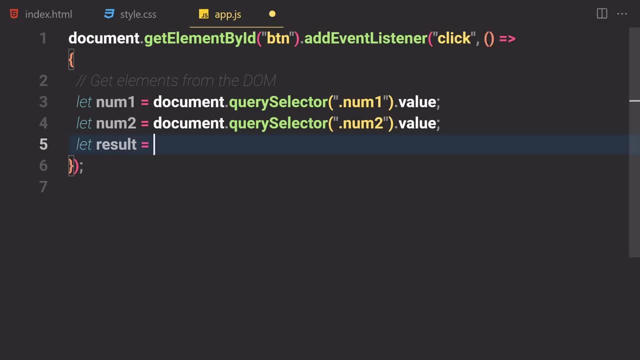 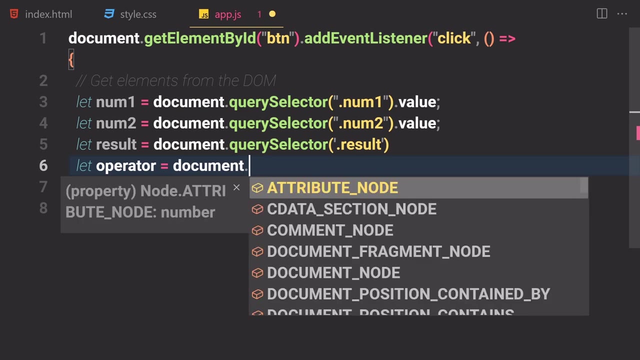 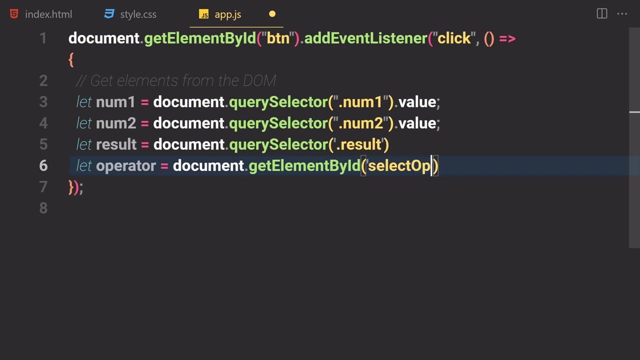 num two. then we have results, or result to be precise, and then we have a document dot query, selector of result, like so. then we have operator o-p-e-r-a-t-o-r of document dot. what document dot get? element by id or select op- yeah, not t, but just op, and you want to get the value of that one as well. so now we totally get. 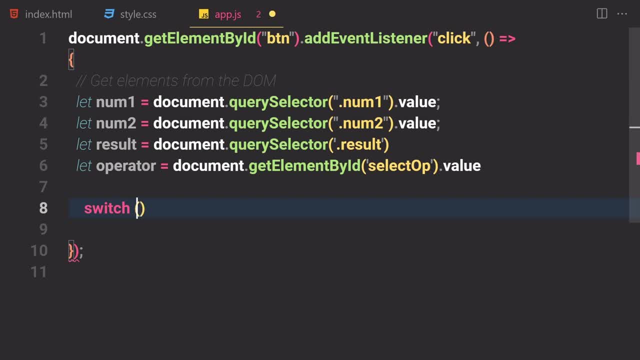 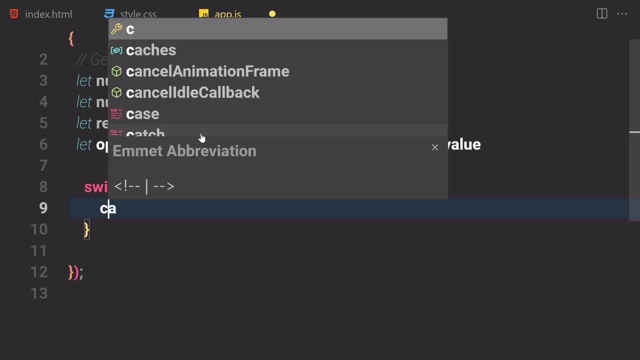 elements from a dom. and now let's just use our switch and cases and you can use um, what do we call it? if? and else statement if you want to. but in my case i'm going to just stick to the switch and cases. so the first case we have if the operator is plus. so we want to just get the results. 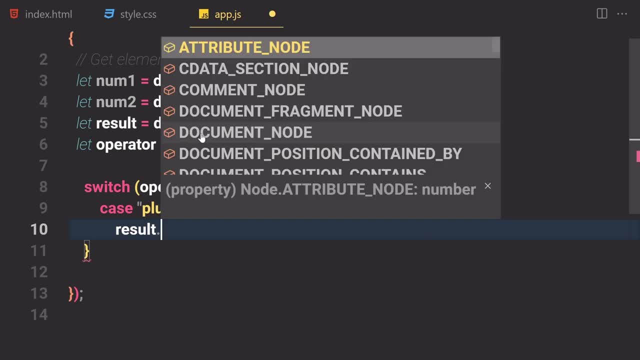 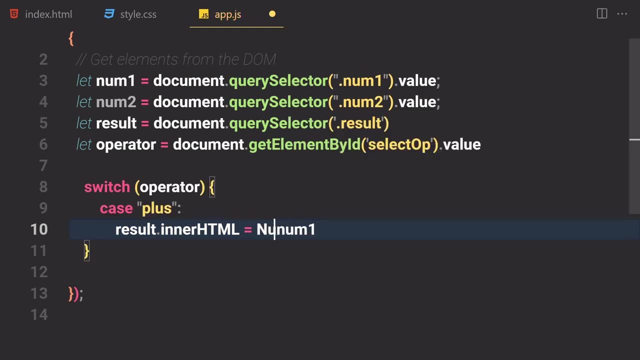 uh, come on, uh. result: dot inner html will be now set to just plus and then num one. so this just simply means it will now convert one number or string to just a number, like so, and then we have a number to num two. okay, you know, first of all i will just write it that way, and then we will. 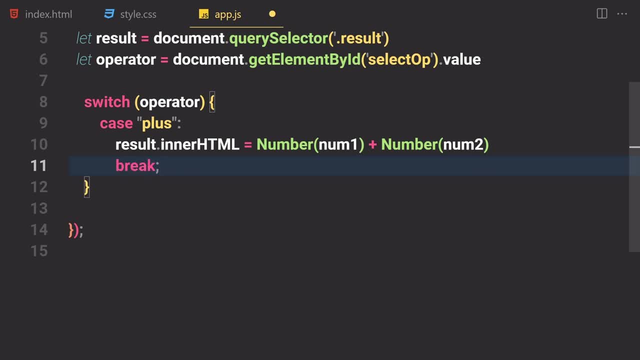 refactor our code. if that's a plus, so we want to just get that result. if the operator is not plus but it's minus, so we want to get a result for the minus. so instead of plus i'm going to change that one to minus and break out from a loop, and then we have a case for the division, and then let's just place. 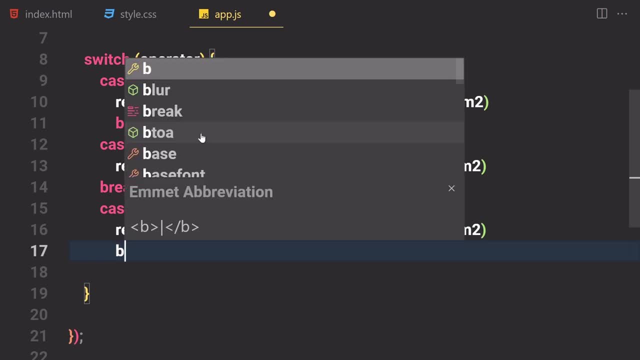 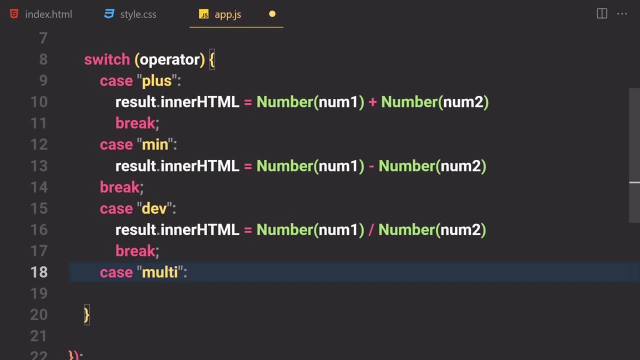 that to divide and also break out from it. and then we have another case for multiplication. so i'm going to just write multi in here, m-u-l-t-i like so, and i'm going to pass this one right here and change that one to multiplication sign. 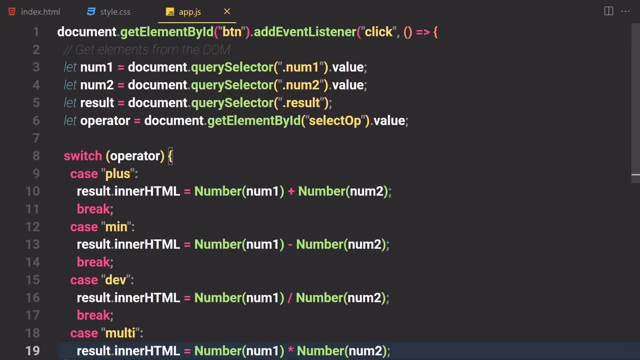 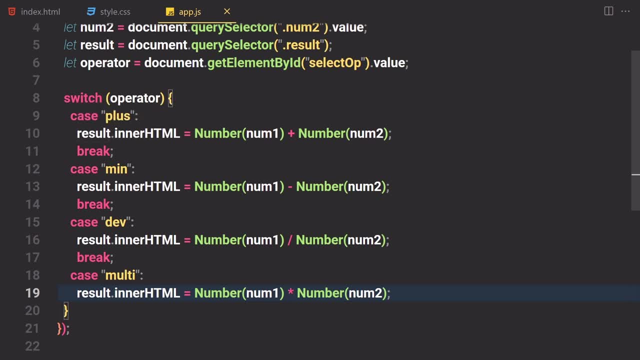 so our file, zoom out of it and now this is how it looks like. so we have a few statements like: if the case is plus, so you want to change the result, that inner html, to the just a number one string and number two string, and we are converting that string to a number and we have a operator of plus. 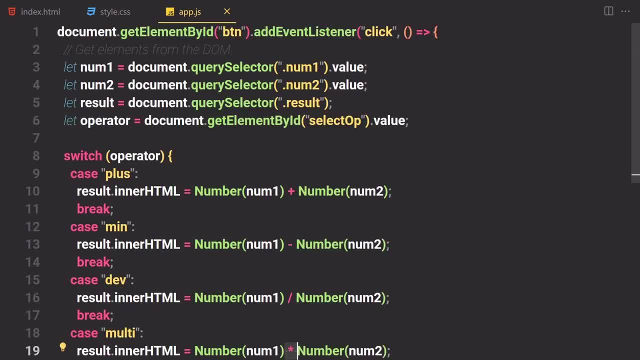 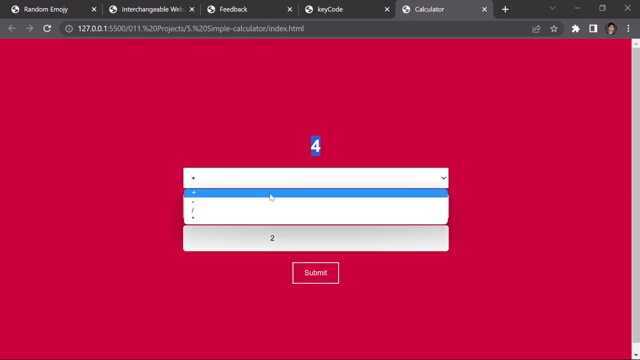 then we have minus, then we have division and then we have multiplication right here. so now let's just check them out. so we have two and two and if you click on this, submit certain log uses four. and if you change the operator to minus, and if you change the operator to minus, and we have two and two, and if you change the operator to plot, so that would make a lot more sense, and you can get this one and get a number two, and we also have someone out there, so do it right here and we will just go ahead and we'll just take the first value to the first value and we'll see how it looks like here. 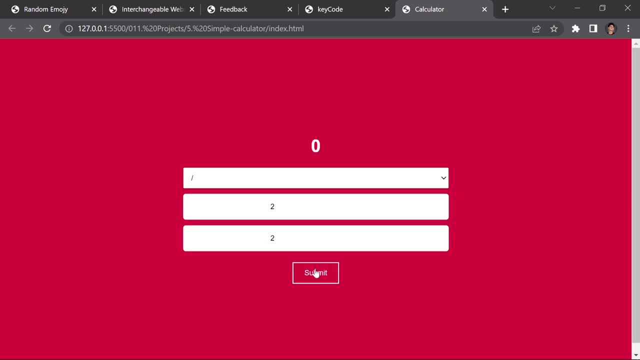 two minus two will give us zero, and then two divide by two will give us one. two times two will give us four. okay, so everything is working the way we expect to work. now let's just try it on 10 and 10. uh, let's just start. let's just try it on plus and 20 minus zero. and divide is one. 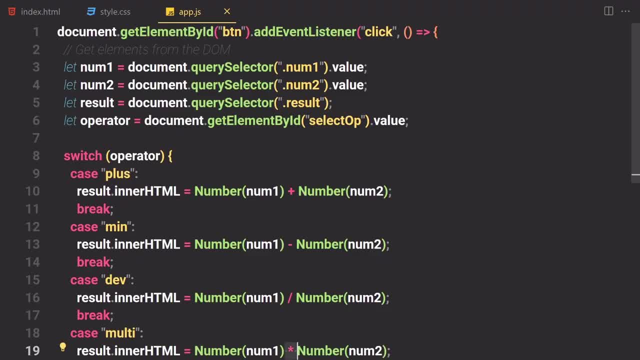 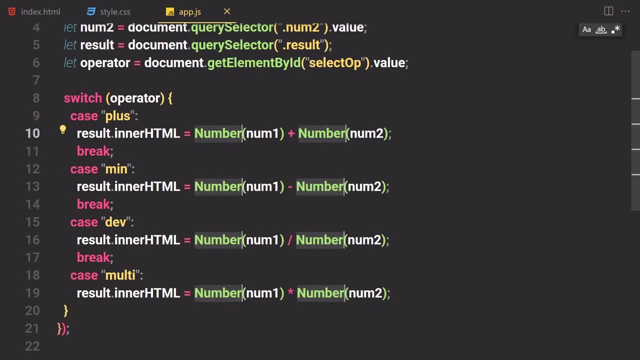 and times will be 100. yeah, everything is working the way we expect to work. so now what i'm going to do. i'm going to select all of these numbers by holding ctrl and hitting d. i'm going to remove that, remove the other one as well, and now let's just put a plus right here, so it will also work. 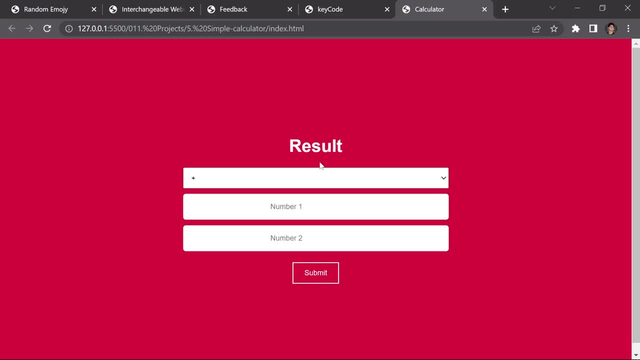 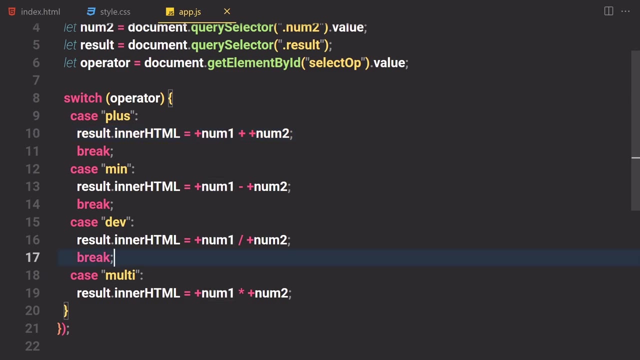 the same, like it will also convert or string to a number. so let's just put a two and two in here, so four. then we have two minus two. then it will give us zero two. two divide by two will give us one, and two multiply by two will give us four. everything is working the way we expect to work. 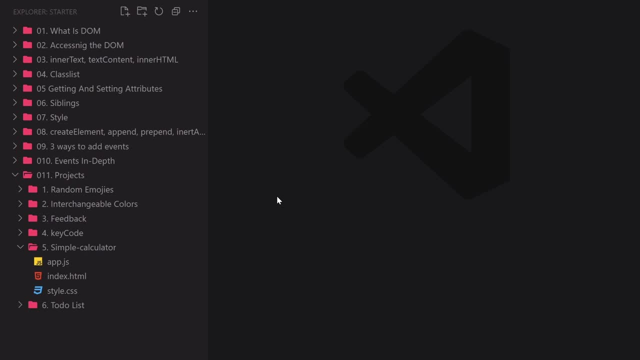 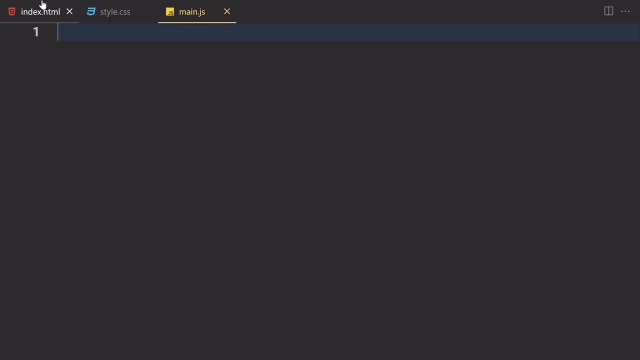 all right. so now let's just start working on our final to-do application- and that's going to be the last project, of our course. okay, so right click on it and open it with live server. and there we go, we have our to-do list right here. uh, let's just change that one to to do to-do list, okay, so. 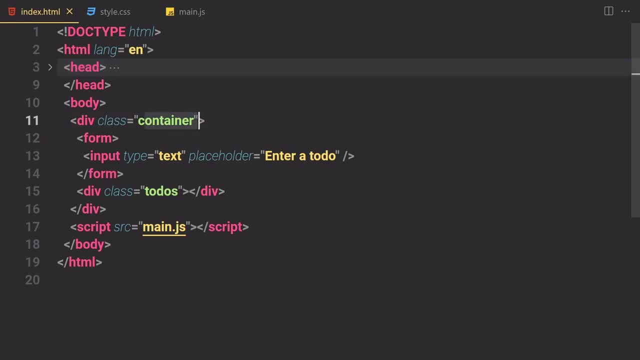 collapse this head area. so first of all we have our div with a class of container. then we have, and inside this form we just have one input with a class, with a type of text and the placeholder of enter to do, and then outside from there we just have our to do's container right here. all right. 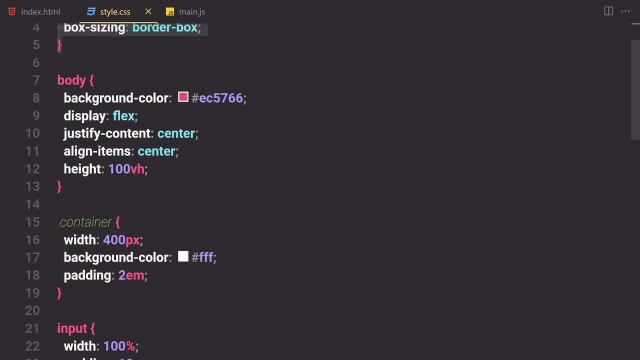 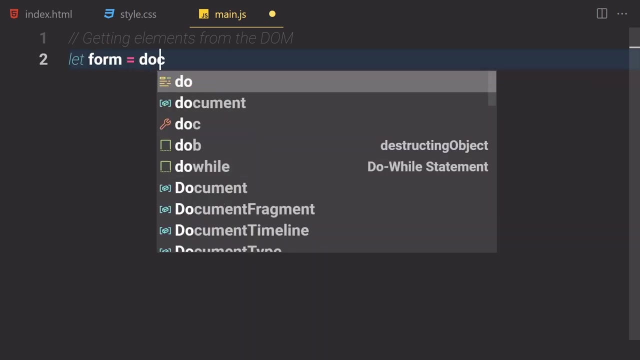 so then we have a styling for reset, then we have margin. i mean, like a body will be totally crimson the background. first of all, we have to get our elements from the down. so getting elements from the down, let me just write a form first of all, and it will be now equals to double, so double. 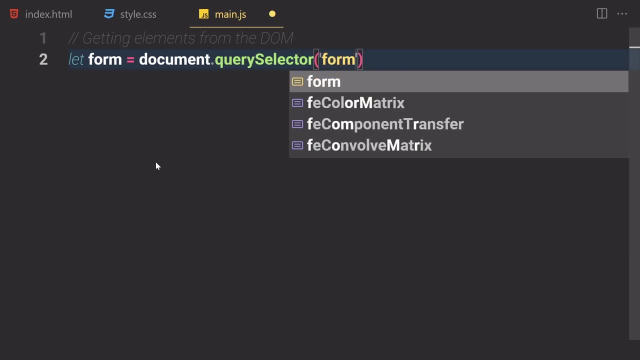 documentcreateSelector of form. okay, so duplicate that a few times, so then we have our input and then, finally, we have our to dos. okay, so change this variable names to be like input and also this one to be to dos like. so all right, so now let's just create our function and give a name. 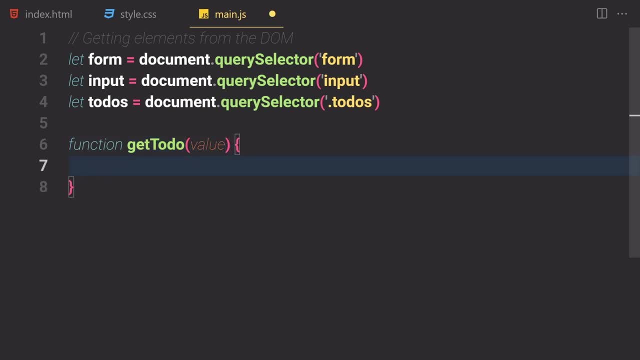 of like get to do and let's just put a value inside that- and creating new elements. so, first of all, we are going to be creating our new elements. so if you want to create new elements, like to do in this case, we are going to be using documentcreateElement, as we learned that just in. 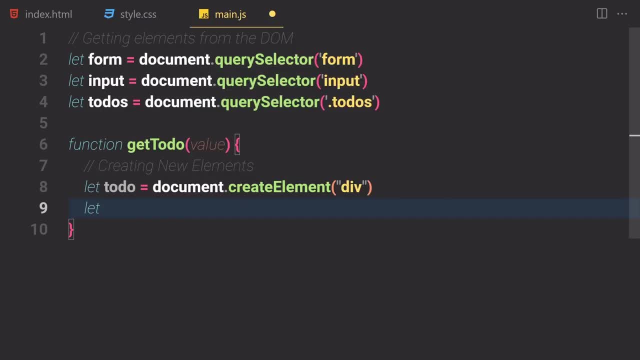 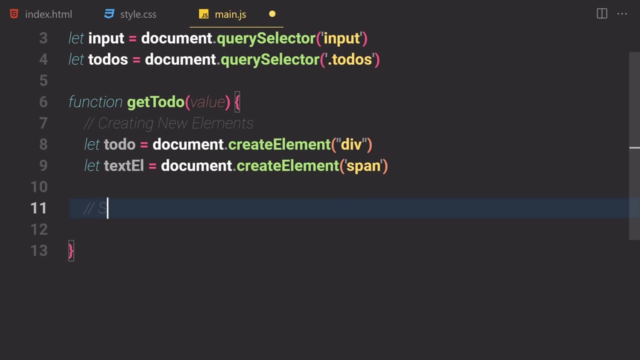 a second and we want to just create a simple div and we want to also create our text element. so we are going to be using documentcreateElement and we are going to be just passing our span in there. all right, so that's it for creating our to dos. oh, now let's just write setting values and. 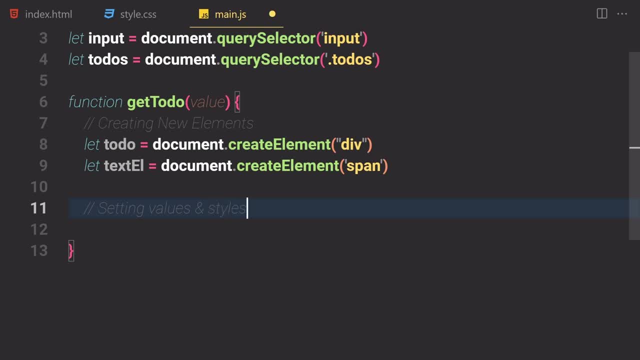 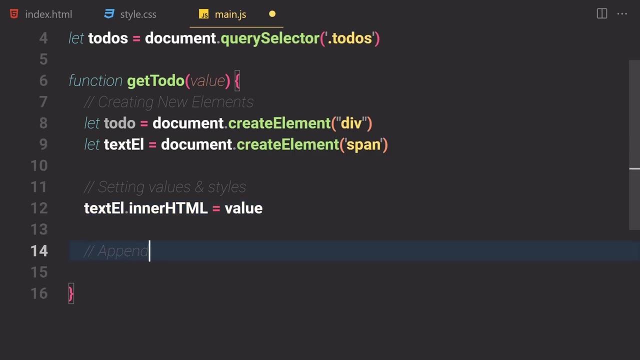 setting values, style and styles for or text element. so i'm going to just write text element dot inner html and it will be now equals to the value, whatever the value we provide like value. all right, so now let's just append the append or element to the dom. okay, so we are going to be using to do dot. 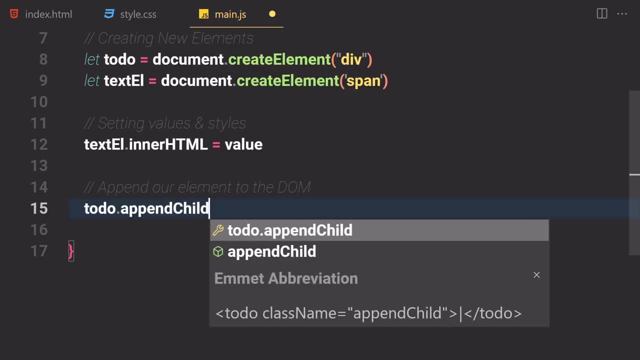 append child. we are going to be using append child c, h, i, l, d, like so. and then text element: d dot. add. pass last base: dot n dot. and then we are going to apply this bound difference and we are going to apply this button. Now let's just create our close button real quick. 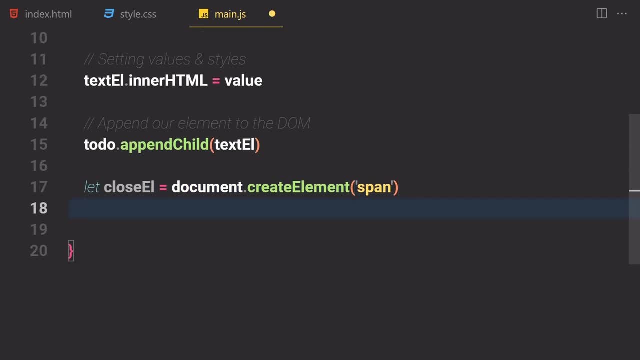 like, let close lmn. it will be now equals to documentcreateElement. our span this course is getting longer and longer, so that's why I'm just going a little bit of fast. inner html will be now equals to this html entity. so, first of all, we are going to be placing our and symbol. 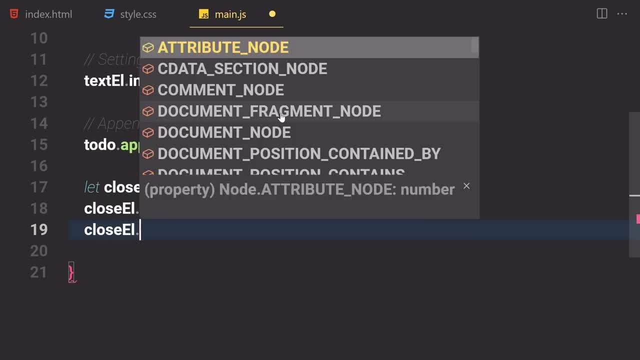 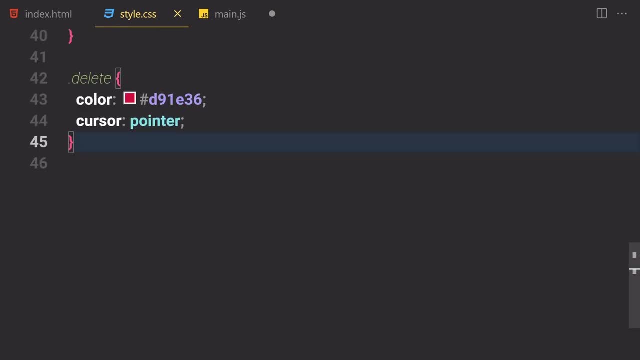 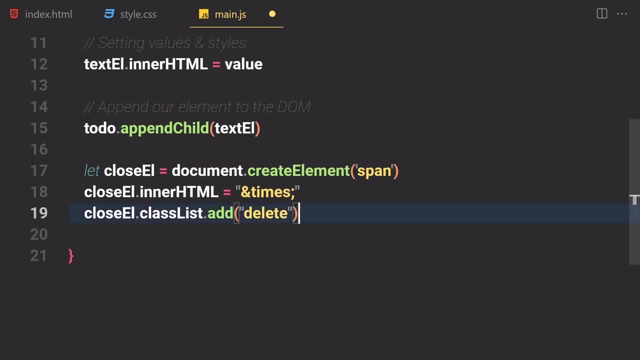 then we have our times and then close it like so list, let's just attach or add and delete class delete, which we have right here inside word css, this delete class, and we also have a class for to do, which we created right here, this to do all. 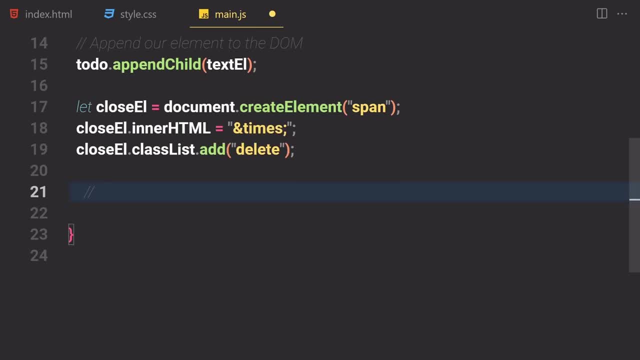 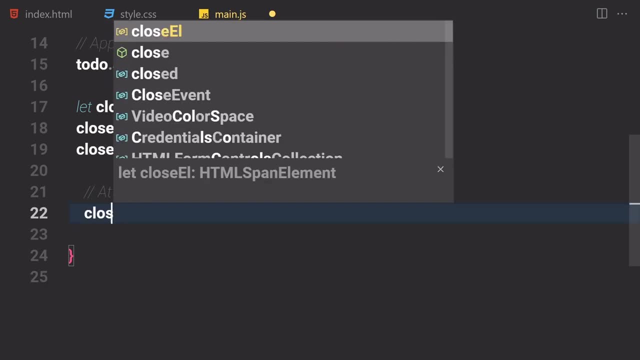 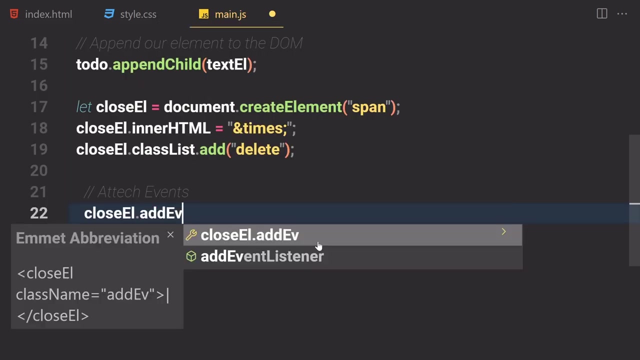 right. so cell file, let's just attach. or event listener to us, attach events like so: and now let's just attach even listener on close element and if you click on it, so add even: oh my god, event listener. oh my god, close element. dot. add event listener like so. now, if you click on it. so 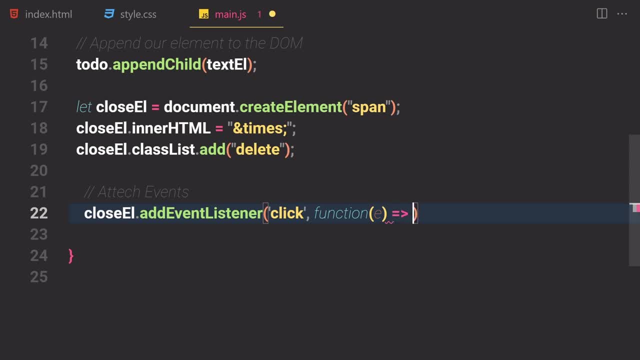 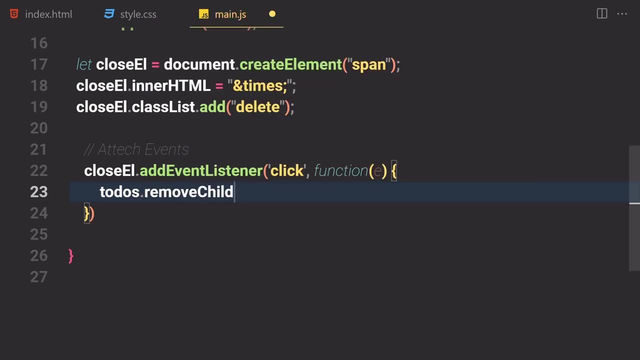 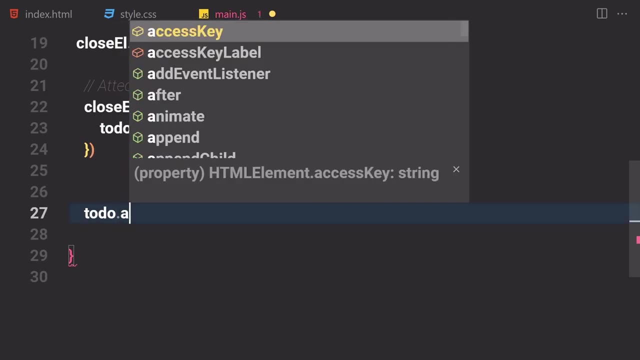 what do we have to do? we have to just create a function and we want to get our object and to do's, uh, dot, remove child, and we want to just remove that, to do from it if you click on that close element. and what else do we have to do? so you want to just write to do: dot, append. 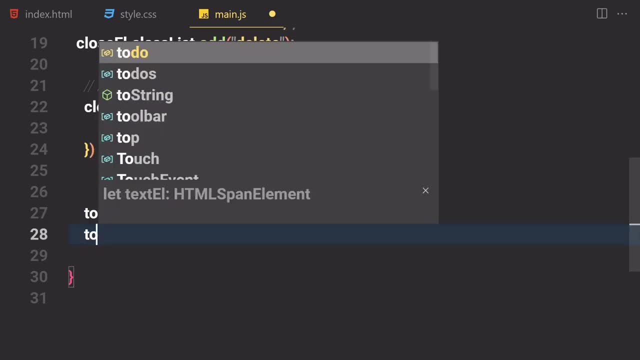 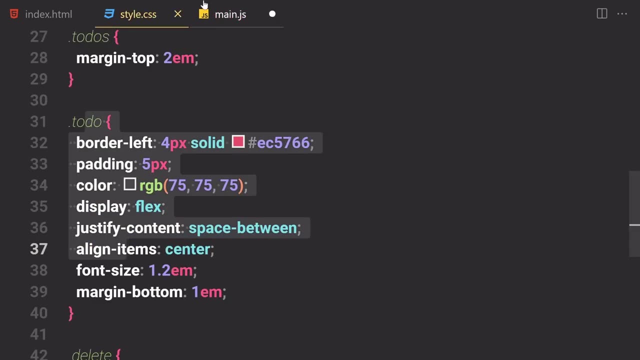 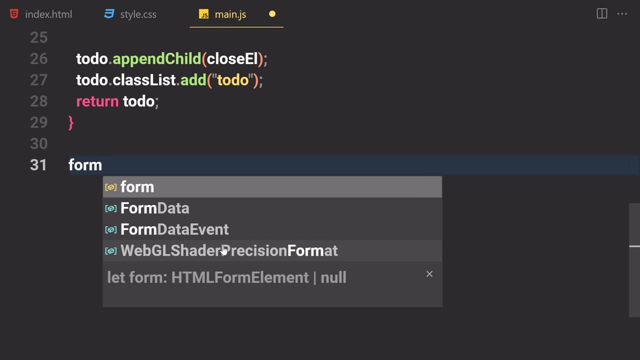 append child of close close element, and we also want to just provide a class of add and then the to do clause which we've created right here. okay, so then let's just return to do cell file. everything is working. now let's just get our form that add event listener and once that form is submitted, so then 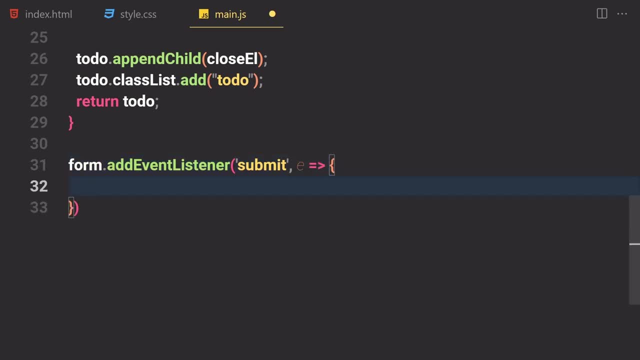 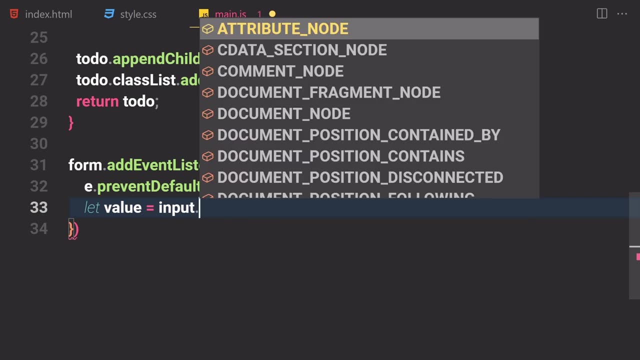 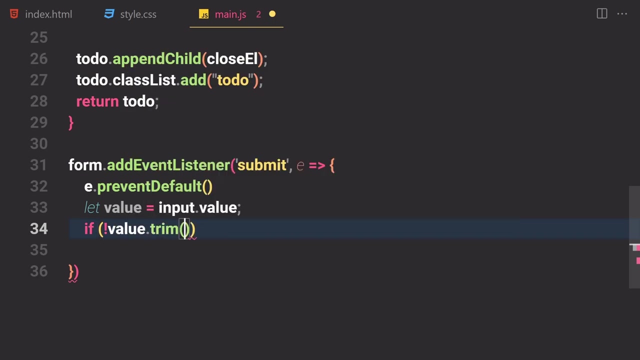 we want to get our element, our object, and let's just get our prevention, let's just set that to d4, let's get our value and input dot value, so whatever we have or value, and then now let's just check if value dot rim because we want to remove that empty spaces from there. so then we want to just return, in this case,